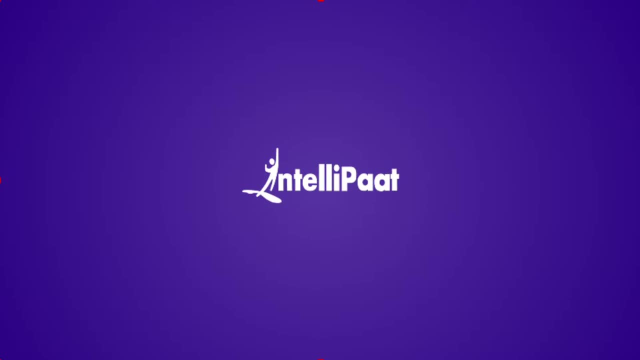 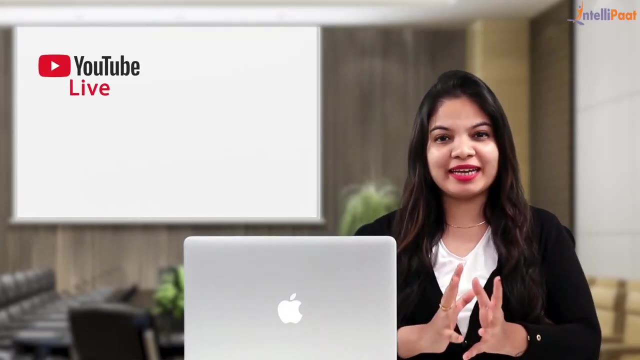 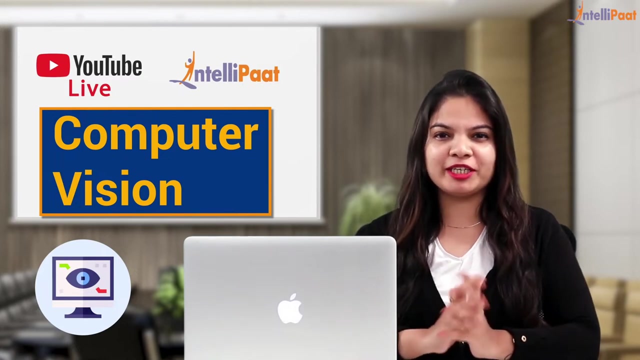 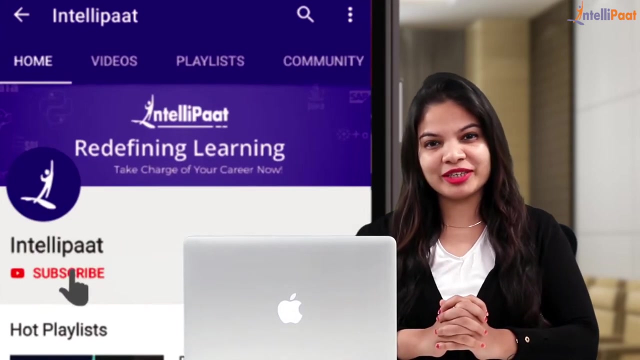 Hey everyone, I welcome you all to the live session on Computer Vision by Intellipaat. This session is conducted by multiple experts who will be teaching you everything about computer vision, from basics to advanced level. Before we begin the session, make sure to: 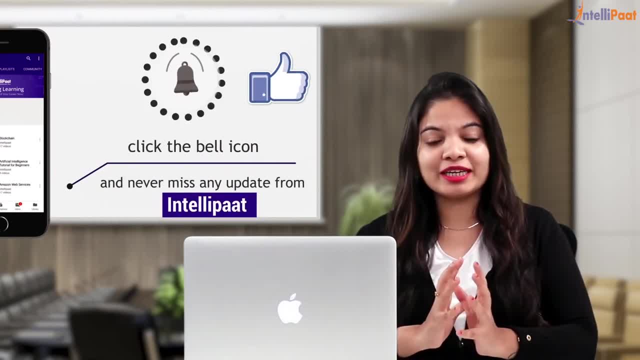 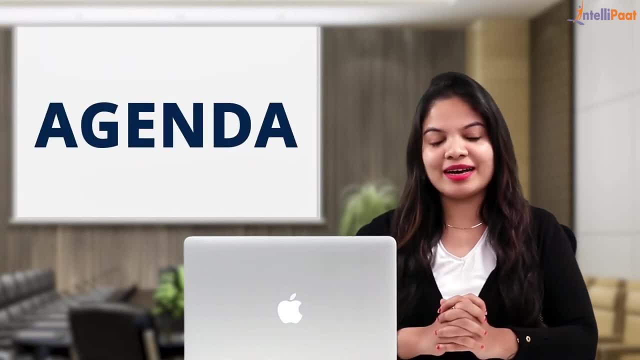 hit the subscribe button and also like our videos, so that it will motivate us to come up with more such interesting live sessions in future as well. On saying that, let's see the agenda of today. Firstly, we will begin with Introduction to Computer Vision, in that we will tell you. 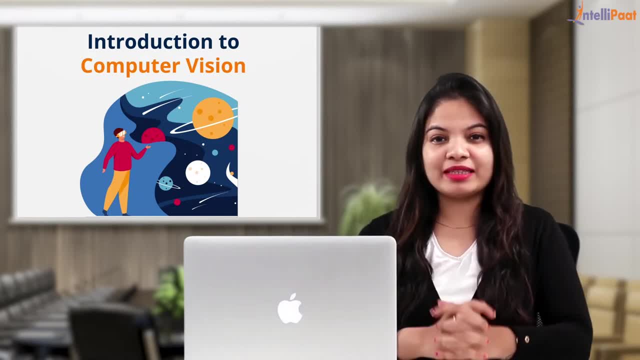 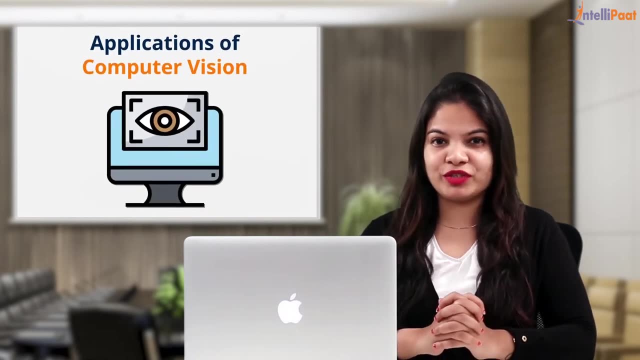 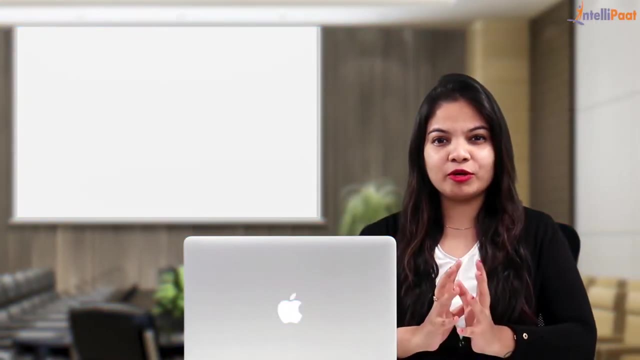 what is computer vision and why do we need it? After that, we will learn about the use cases of computer vision. Then, later on, we will see the applications of computer vision. Post that we will learn about. image resizing and cropping Post that we will learn about. 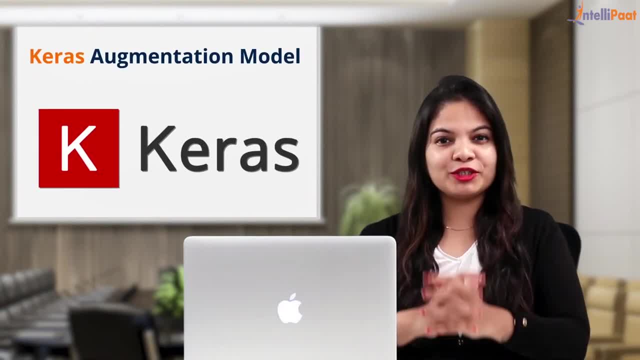 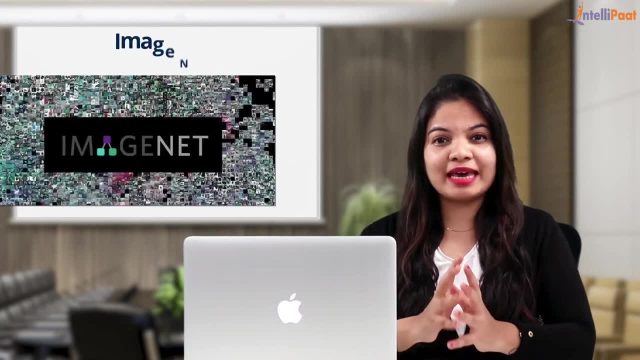 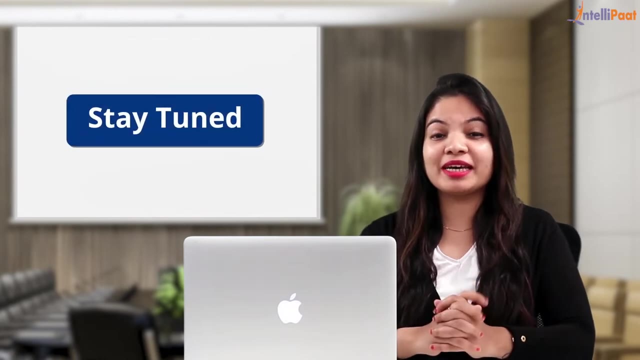 Kiraz and Kiraz Augmentation Model. Then later on we will learn about Implementation Convolution with Augmentation. Then, finally, we have covered ImageNet. So this is the agenda of the video. This session is going to be very interesting, so stay tuned and watch the video till the end. Now let's begin the 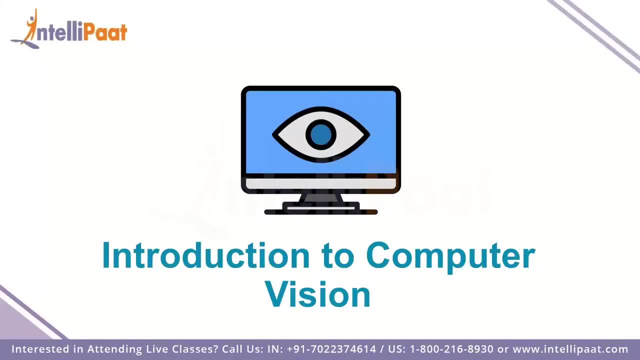 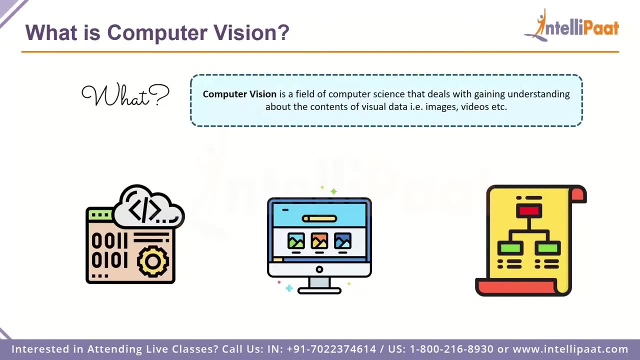 session. So what is computer vision? The question is quite natural to appear in our mind, and we have to understand what computer vision actually entails. Let's take a look at that. Computer vision is a field of computer science that deals with gaining understanding about the contents of a visual data. This 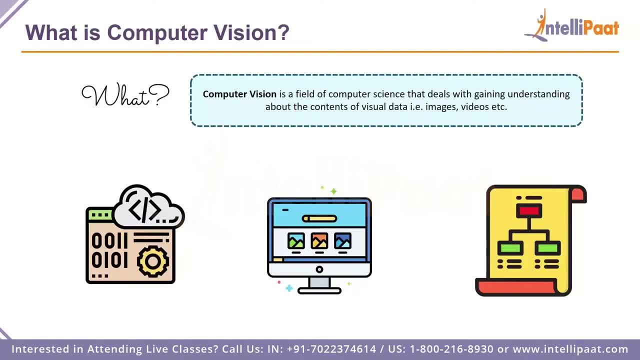 visual data includes things such as images, videos, GIFs and many more. The reason why it's called computer vision is because before computer vision we had access to images. Our computers can understand and process the image, but the processing essentially just meant converting some data into other formats. 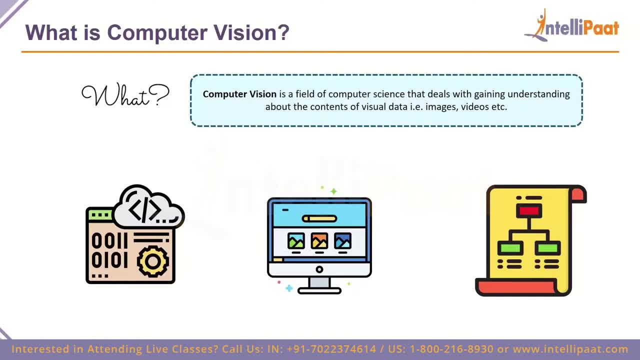 So, for instance, if we had a colored image, we can convert it into a black and white image. The computer had no idea about the contents of the image, whether it contains the face of a person, a person you know, a famous personality, whether it is the image of a tree, a mountain, some kind of an animal, so on, and 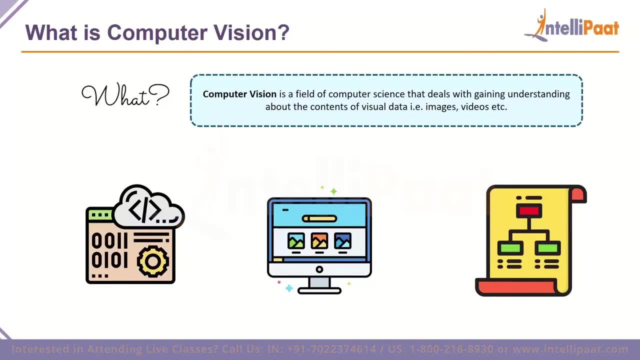 so forth. So that was not very useful, mainly because this allowed us to manipulate the data that lies beneath the images, but it does not allow us to provide any contextual information about the images. So, for instance, if I wanted to look for an image out of the images that I have on my phone, give me an image. 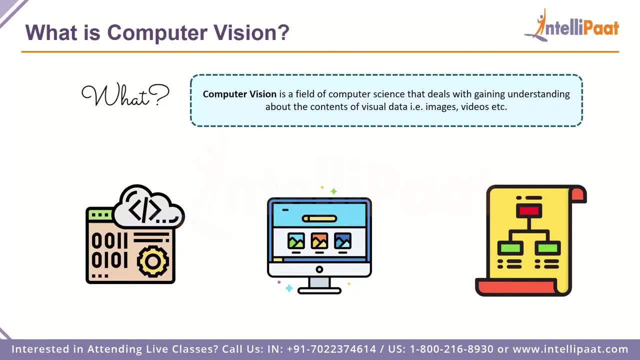 where there is a photo of me inside it. It could be a selfie, it could be any kind of image, but I should be present inside that image. Before computer vision, our computers, our applications were just not able to do that because they had no. 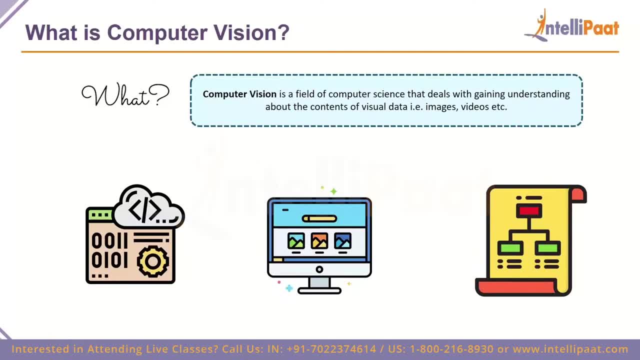 idea what an image contains. The part of the problem was that image data is very complicated. It may look simple on the outside, but because images are made up of several colors, gradients and they can be, they can be manipulated in several ways. it can be. 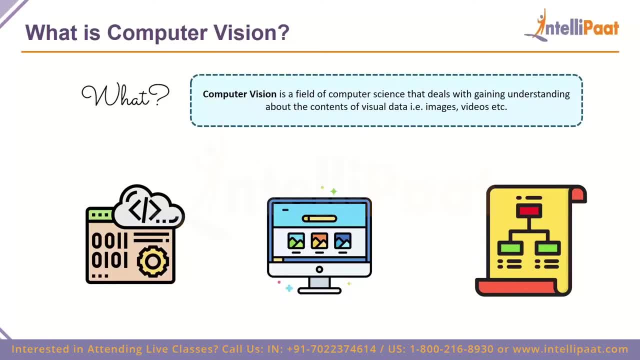 really difficult to understand well what computer vision actually is. So in cases like this, when we're trying to understand what computer vision is, an important idea to understand is that our brains are much better and much more capable of understanding visual data. We do it all the time. We take a look at a. 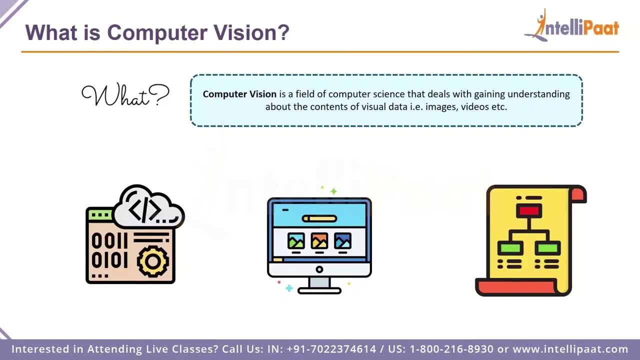 mobile phone. we understand what the phone is. we can understand contextual information about the phone, that is, how large the screen is, what's the weight, how does it look, what color of the mobile phone is there, what company brand, so on and so forth. But computers were not. 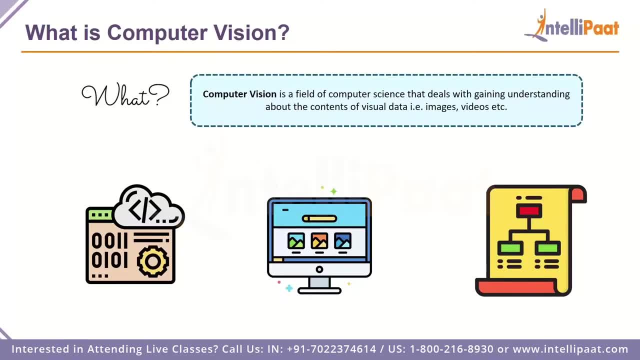 able to do so. With the advent of machine learning and data science, now this is very much possible. Now we can teach computers what a mobile phone looks like and then, when the mobile phone is seen in any of the images of videos, we can. 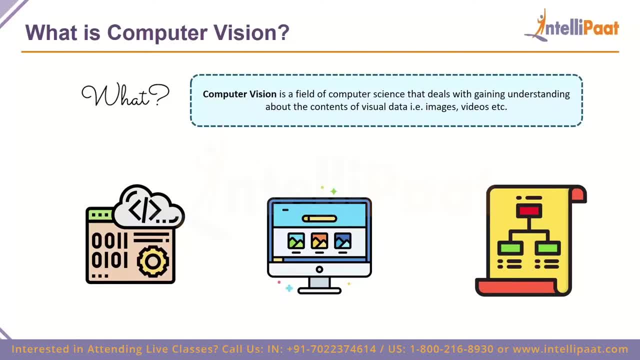 very easily understand what it actually means. Now, that is a very narrow understanding of what computer vision is, because in computer vision, you might want to not just be able to do it with a mobile phone, but there are several fields such as, if you are trying to analyze the video for traffic, you might 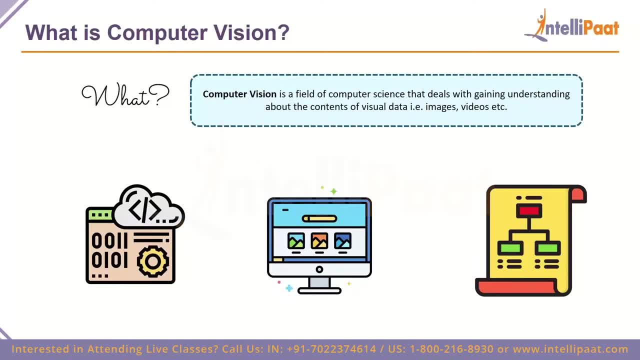 want to know which of the images or which of the people in the traffic or vehicles in the traffic are moving at a pace that is not suitable for them, and so on and so forth. So that's what computer vision is Basically: it allows computers to understand visual data, such as data contained inside an image. 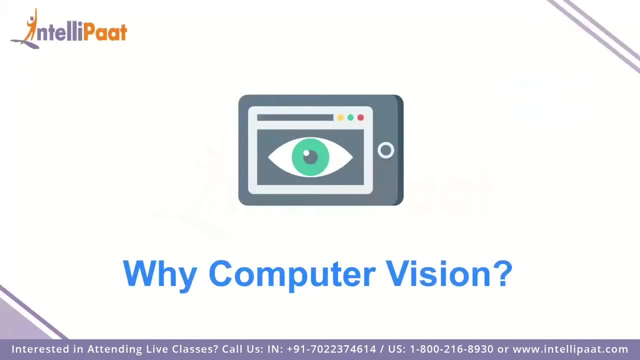 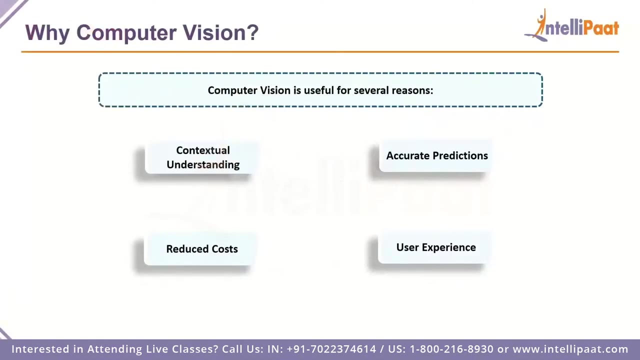 video, so on and so forth. Let's take a look at why computer vision is useful. We have understood what computer vision is and what it is useful for, but let's understand why it is useful and what benefits are there. Computer vision is useful for several reasons. Let's understand these reasons I have mentioned. 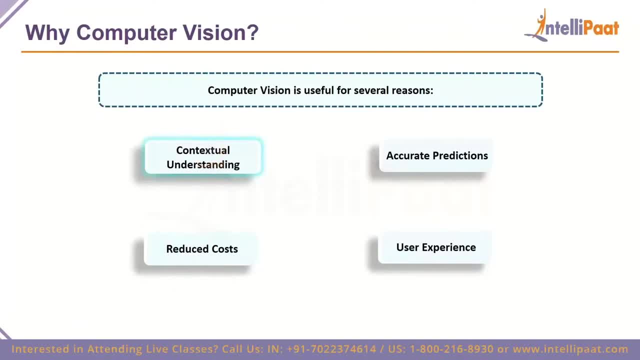 only a few, but let's understand them one by one. The first one is contextual understanding. This is by far the greatest achievement of computer vision, which is contextual understanding of images and visual data. I'll give you an example. contains a person that is or inside a vehicle, that is in an image that a computer vision can. 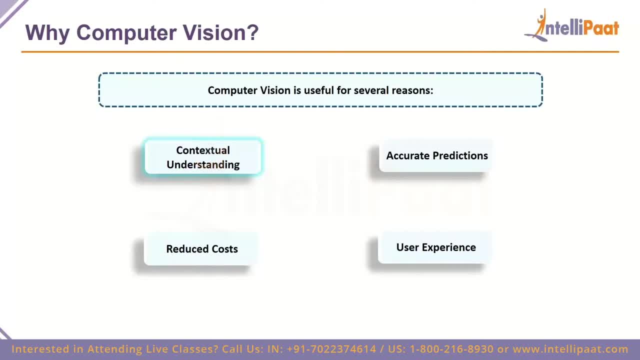 understand and, depending on how the computer vision algorithm is set up, it could even understand whether the person is driving or is just a passenger. That's the contextual understanding that we're talking about. Before this, all we had to do we had to process the image on our own, and 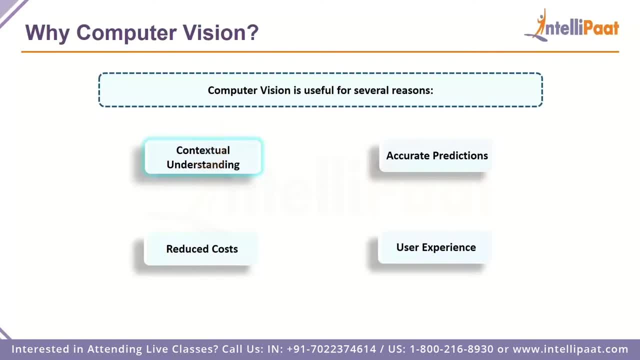 then we could label it on our own, but there was no way of it being understood by the computers automatically. Computers had no idea because they could not see the images. they had no vision per se, so that's why computer vision was helpful in providing contextual understanding. Another: 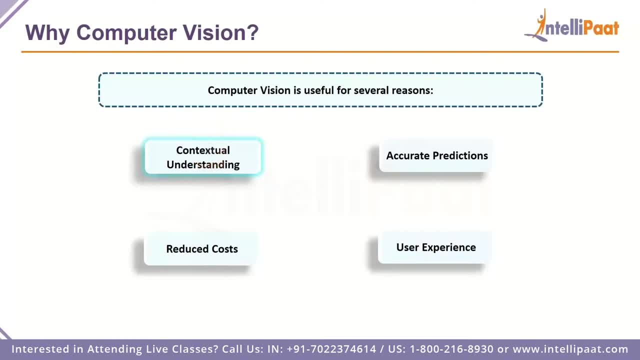 good information would be. another good use case for this would be, or a good benefit of this would be, that, since contextual understanding is built using computer vision, we can even use it in different areas, such as security, where one person might be allowed to do some things, but not the 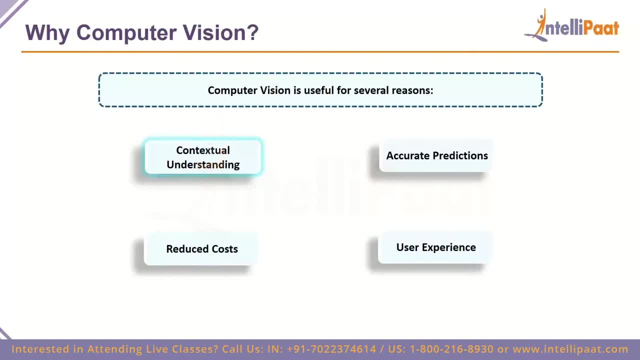 other things And so on and so forth. So that's what we mean by contextual understanding. Then comes accurate predictions. Before computer vision, predicting which data in visual data was very tiresome, very cumbersome and was not very accurate as well. We got around the accuracy of 60 percent, but that was 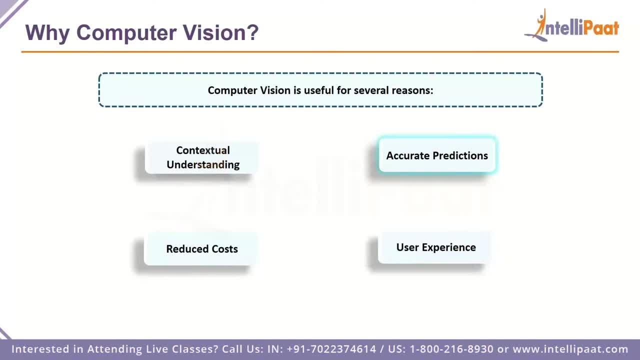 not really desirable. So to get over that hurdle, computer vision makes, processing videos, live streaming data, images, gives, so on and so forth, and segregating them, classifying them automatically. So that's what we mean by contextual understanding. Then comes accurate predictions before computer vision. thevuid doesn't need visual support, or 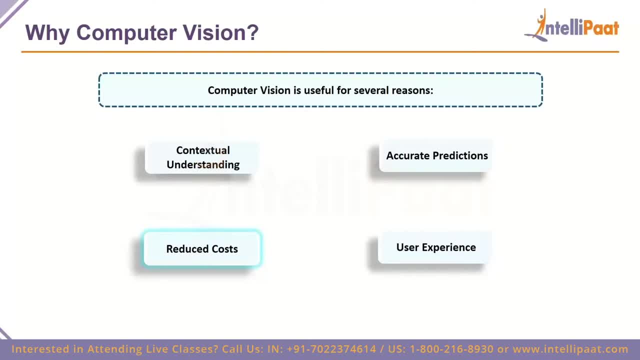 powered mobile phone, be it a high powered mainframe. computer vision applications can run on several applications or several platforms. so the cost that we sort of invest in creating computer vision system gets paid over time because of the wide variety of platforms and the wide number of users that it can be accessed by. when comes user experience? there are several things that a. 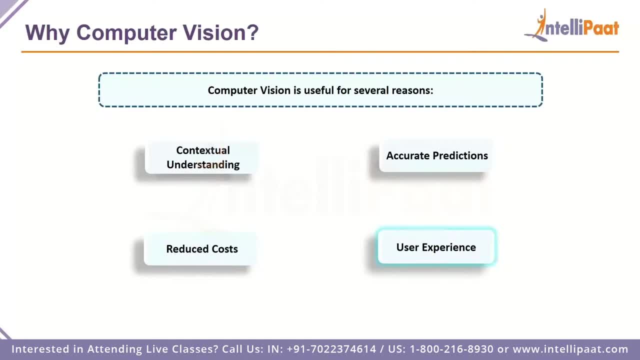 computer vision system you can do to enhance user experiences, for instance, a very useful use case of computer vision is: you have an image or you have some product in front of you that you want to get some information about now. before this, what you would have to do is you would. 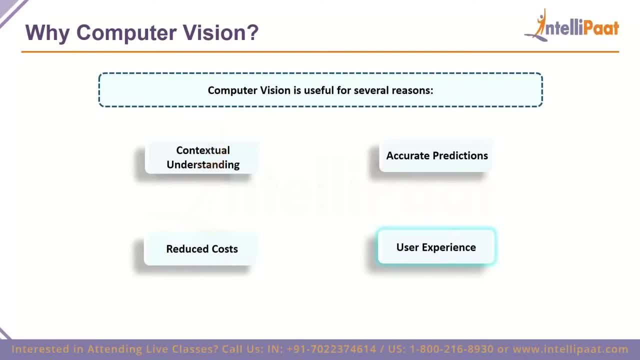 have to use a textual interface in which you would have to type in the text depending on the image that you have. now, on the other hand, you could. what you could do is now use your computer vision system camera to point at the product that you want to buy, and the computer vision system will take it. 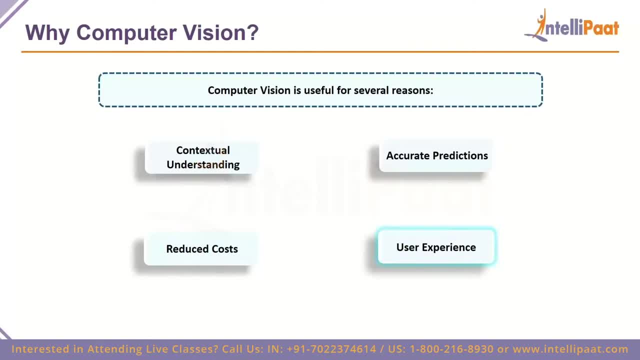 over from there and will give you all the information that it can find on the internet, based on the product that it has. that's the real advantage of using computer vision. it enhances the user experience to a level that was not possible before. computer vision was a thing, so computer 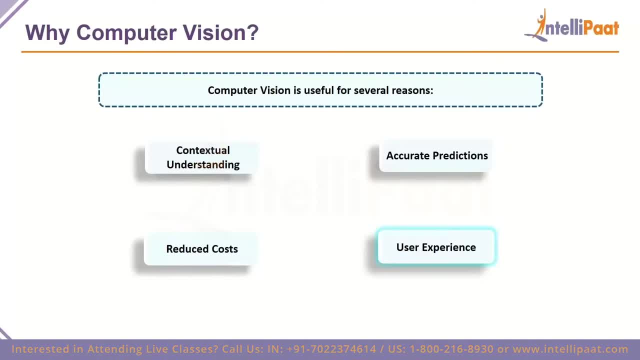 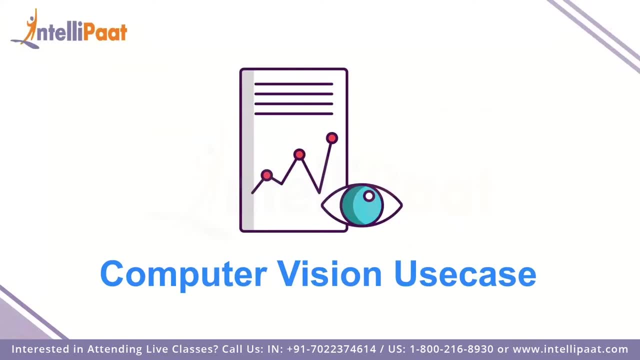 vision can be really useful for other aspects as well. but these are the four major uh advantages of using computer vision. now let's take a look at some of the use cases of computer vision. uh, these use cases are just a mere list of things that can tell you what. 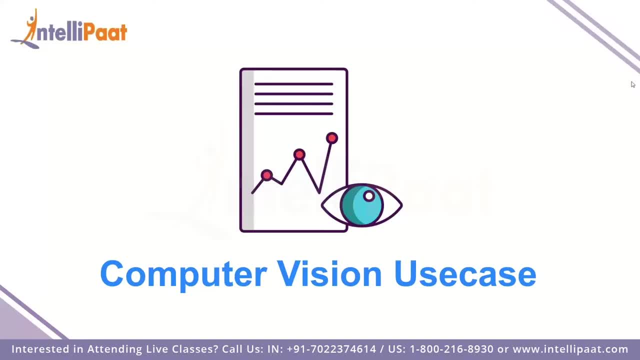 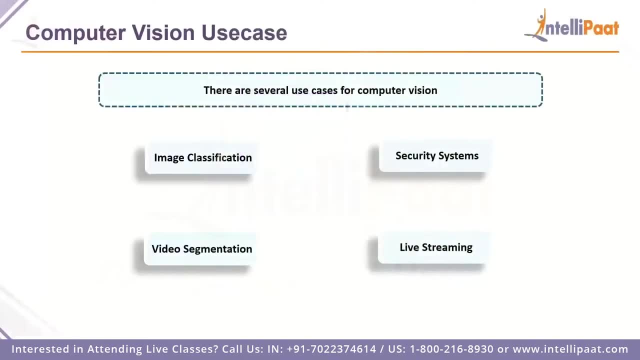 other kinds of things where you can use computer vision. uh, obviously, you can use computer vision for other things as well- more things than i have mentioned here- but let's take a look at the things that we have mentioned. so there are several use cases for computer vision. first one is image. 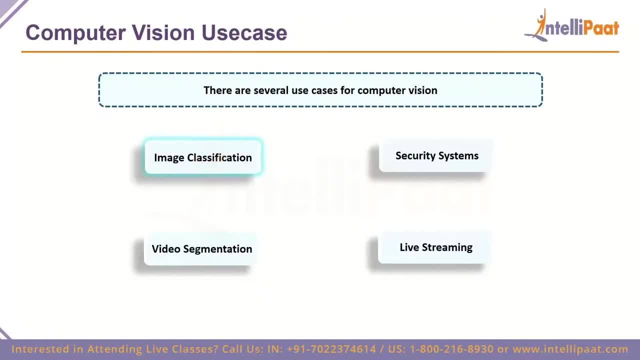 classification, image classification is by far the most primitive way or the most primitive use case of computer vision. the first thing that comes to mind when we're talking about computer vision is this primitive understanding, which is where you get an image and you try to, basically, after getting the understanding of what it actually is, what you do is you. 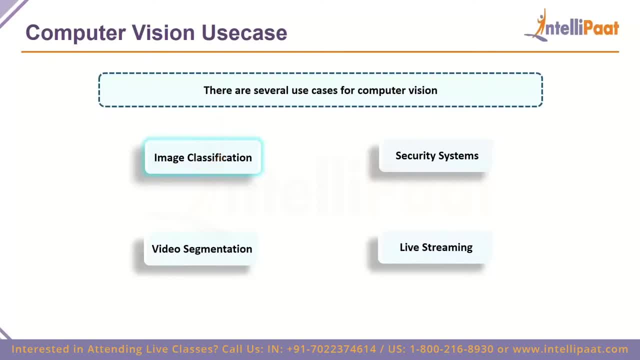 classify that image, provide a label on it. so, for instance, it could be a label based on some binary classification, whether the image contains something or not, or it could be a more broader aspect of classification in which we are trying to label the image with all the things that 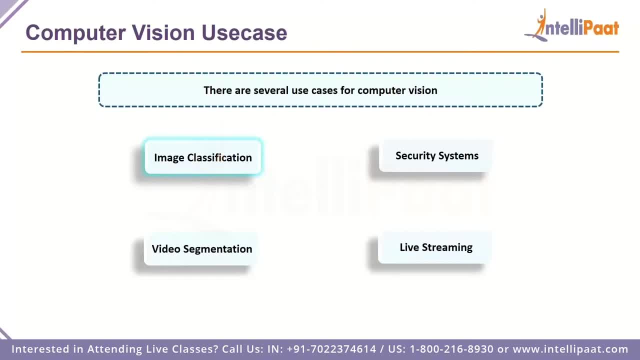 it contains. for instance, if it's an image of a person driving on a mountain, then the labels could be: person, car, road, mountains, driving, vacation, so on and so forth. all of this is now useful and feasible using computer vision. uh, then comes security systems. computer visions play a major. 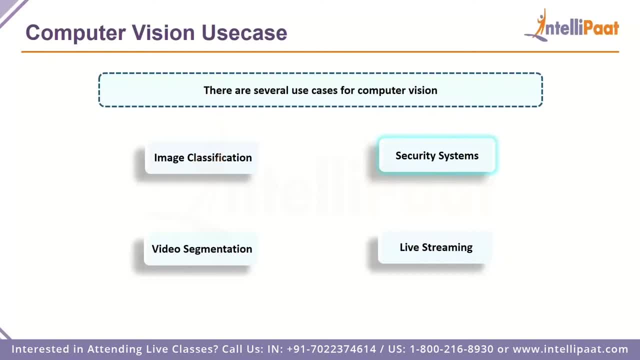 role in security systems, as you can, for instance, put in the faces of the employees that you want, want to have access to a particular resource and then, when the computer vision system activates, any person that is not inside the database of the persons who should have access to the images or to the resources is not going to gain access, because 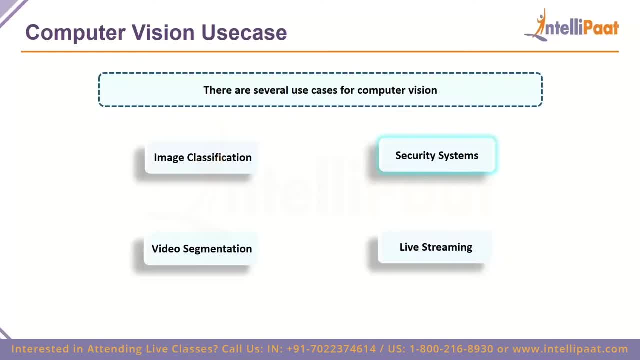 computer vision is able to classify the person as being authorized or not. computer vision systems also allow you to basically just log the information about who came in and who went out, so the security systems can be really sophisticated as well. video segmentation is also a really huge use case for computer vision. 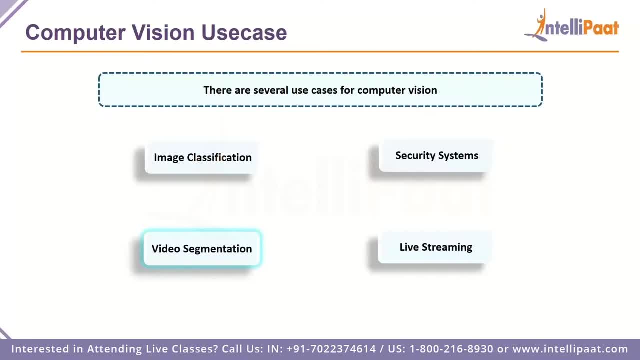 vision, since we are able to derive contextual understanding of images. we can segment videos into several portions. we can pick out portions, we can pick out people that are present inside the video and we can separate the videos based on what data it contains. google uses video video segmentation using computer vision quite a lot, so you can take a look at that as well and then 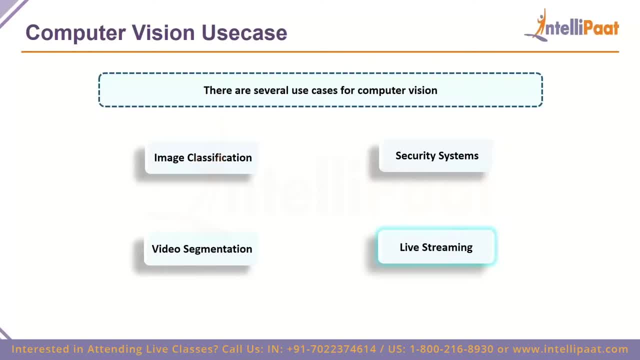 there's live streaming. computer vision systems are also now capable of processing live streaming data. so, for instance, if you have um certain certain use cases in which you don't want certain images, copyrighted contacts, anything to be shown on the screen, even when you're live streaming and you 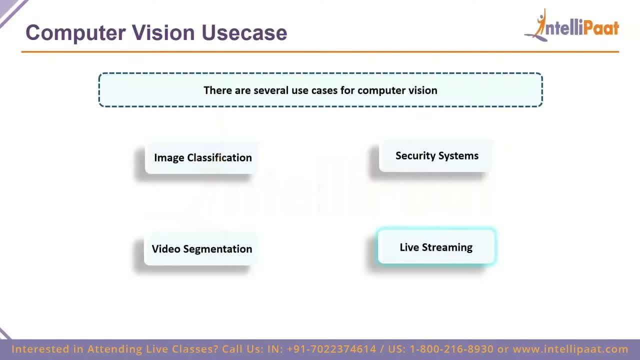 don't want to do it, even by mistake, the computer vision systems that can allow you to do so. so, basically, your data. instead of going directly from the from your computer to the streaming service and from the streaming service to the person who should get the data, what happens is the streaming. 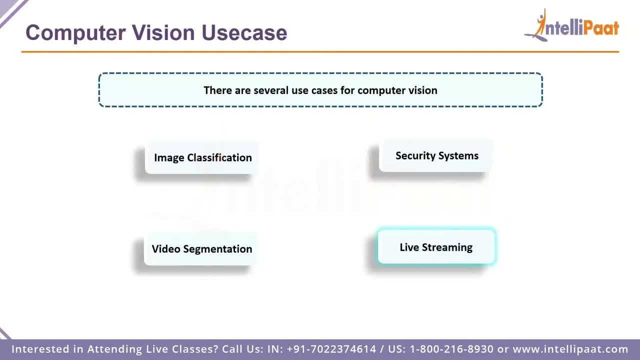 service firstly processes the data and then the streaming service processes the data and then the data. maybe it offloads it to some other computer vision system and that will analyze each frame of the video, see if there is anything that is worth clipping out or pixelating and that will 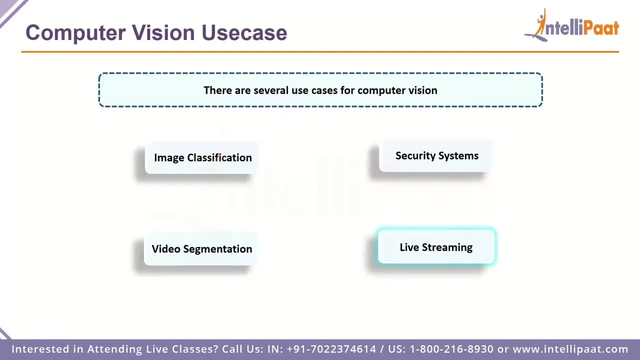 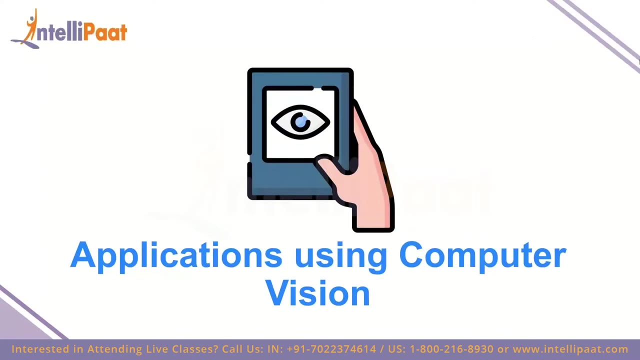 be done automatically. it does take a lot of processing power to do so, so this could be a little costly, but that really is a use case, a valid use case for computer vision. now let's take a look at some applications that use computer vision. uh, these applications are applications. 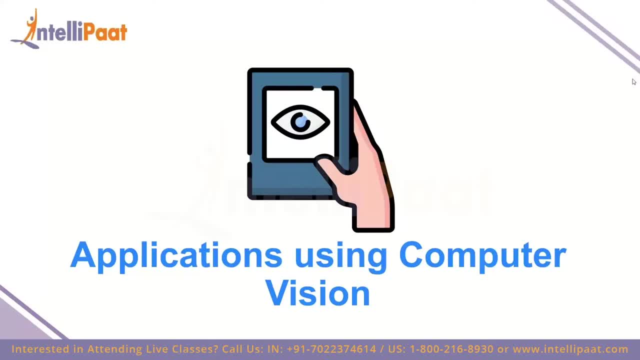 that are used for computer vision. so let's take a look at some applications that use computer vision, are very famous and use computer vision quite often and quite a lot. so let's take a look at these one by one and understand where is it? where the user? you may be familiar with some of those, so 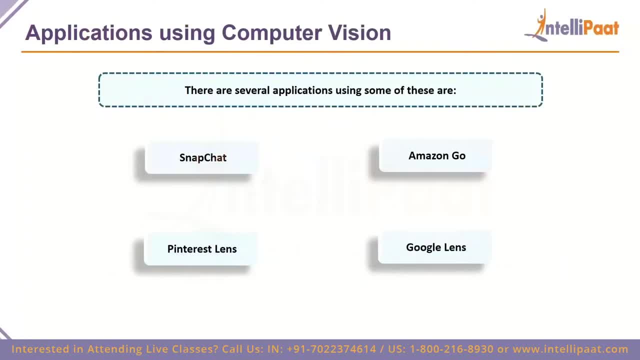 let's dive in. there are several applications nowadays that use, uh, the computer vision system. some of these are snapchat, amazon go, pinterest lens and google lens. let's take a look at them one by one. so for snapchat, if you have ever seen the filters that are provided by snapchat, and now 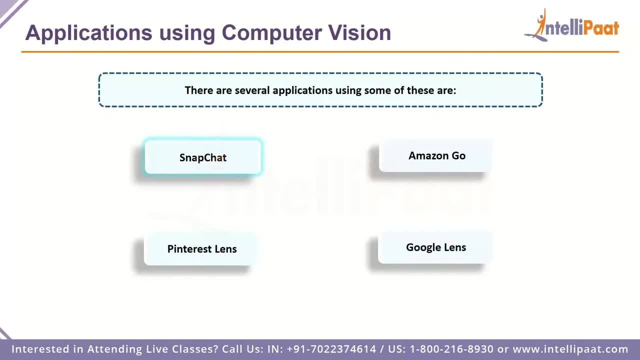 uh is a feature that is available in several applications such as facebook and instagram as well. well, these features are implemented using computer vision. all you might consider it to be an augmented reality feature. well, that does come under computer vision. so, if you are trying to understand augmented reality, where you are able to put something or inside a video that they are, 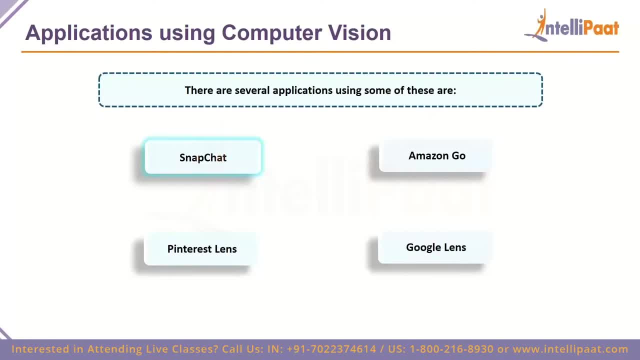 not there, then? snapchat is a good example, filters are a good example of that, and computer vision is useful in that regard. then comes amazon go. amazon go is a amazon store in which you can walk in, buy something and just leave, and the amount of the products that you have bought. 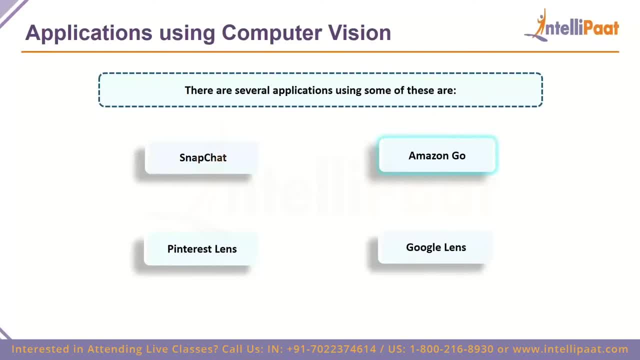 will be deducted from your payment system. uh, this is a convenience store. it is, uh, very popular, it's. no, not a lot of branches are available there, but it makes heavy use of computer vision systems, along with other systems such as cryptographically secured sensors. save money, so you don't have to butcher these all up so you can do any other kinds of things. 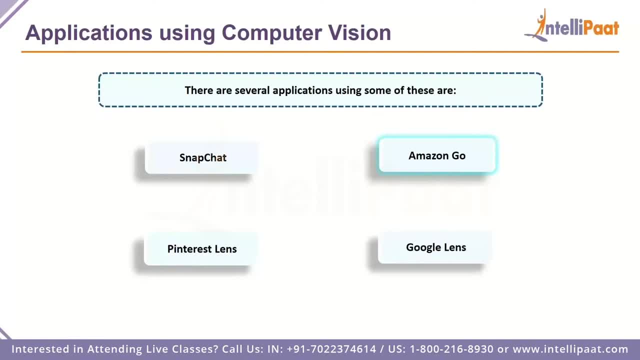 but at the end of the day it makes the shopping experience much easier, and amazon go is a very heavy user of computer vision systems. then comes pinterest lens. pinterest lens is actually a very uh important tool if you use pinterest, when which, basically, you can point it to any of the things that you want to be searched on pinterest. so, for instance, 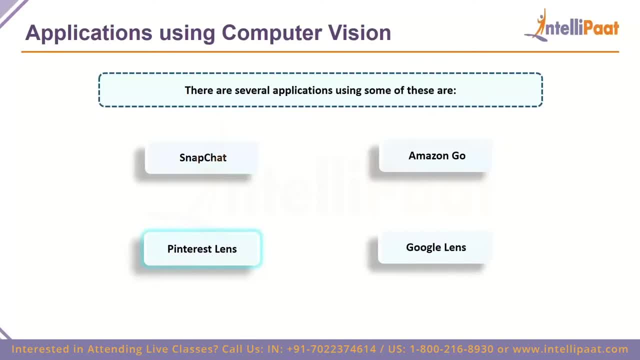 do is point it towards the dish. the pinterest lens will find all the images that look similar and then you can choose one and look at the recipe of that that image. similarly, there are many other things that pinterest lens could do and that's why it's so useful and it makes heavy. 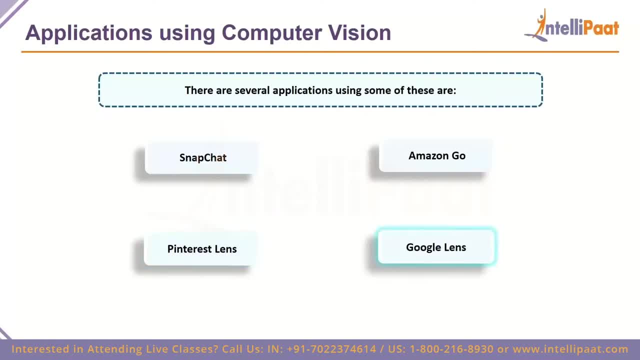 use of computer vision as well. finally, there's google lens. google lens allows us to basically perform a whole variety of tasks, ranging from scanning barcode, identifying products, identifying images, identifying things inside images, people inside images. make google search, image search. all of that, and that is one of the most popular use cases for computer vision. this. 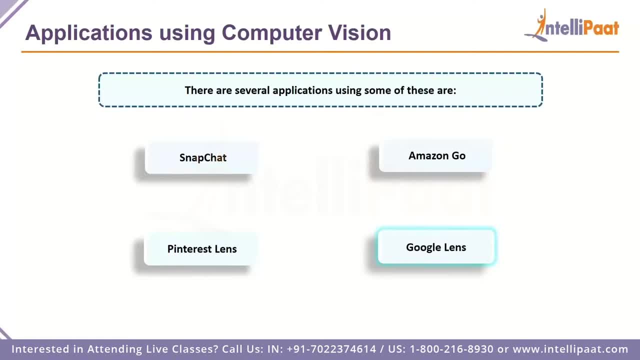 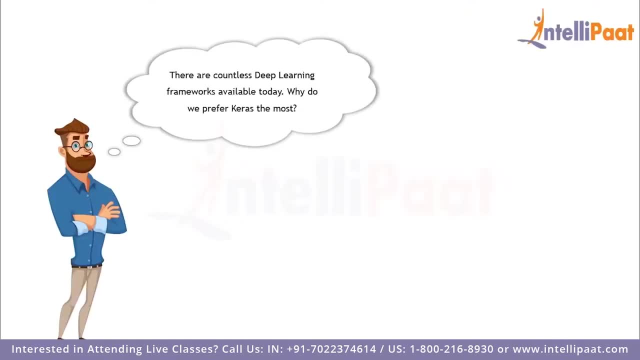 application is by far the most popular one among the bunch that we are discussing. that uses google, that uses computer vision heavily, so there are a lot of deep learning frameworks available today. so now my question to you guys would be: why should we use scaras out of all of these? 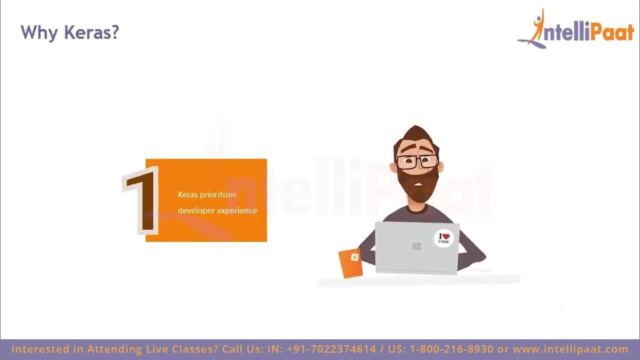 deep learning frameworks, and why should we use scaras out of all of these deep learning frameworks libraries? well, let's understand. so the number one reason to use caras would be: it prioritizes developer experience. so caras is a framework which is developed for humans and not machines. 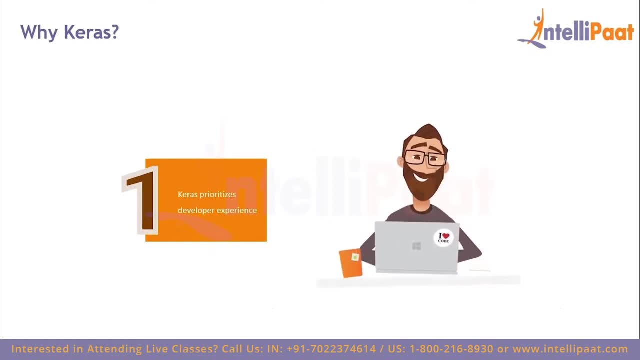 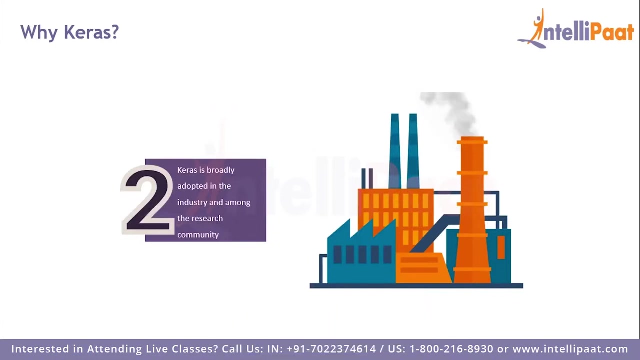 that is, it is very easy to code with caras. you just have to keep on adding layers which you can invoke with functions and you can keep on building neural networks. so it is that easy to work with caras. and then caras is also broadly adopted in the industry and also a 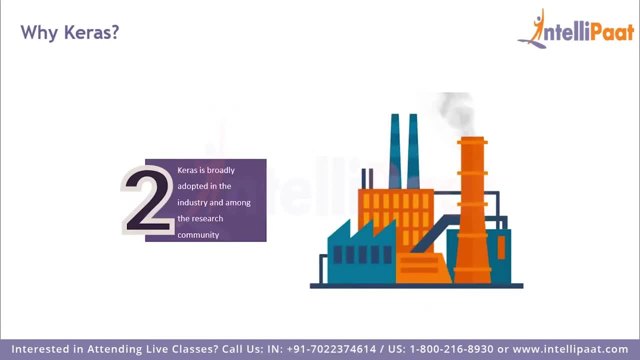 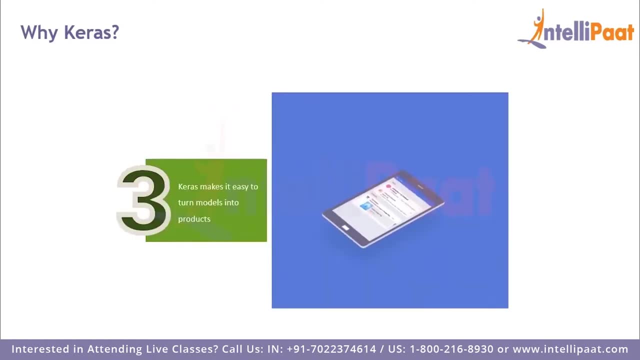 common feature among the research community. so all of the phd scientists over there and all of the data scientists, their most widely preferred deep learning framework is caras. and the next reason would be: it is very easy to turn all of these caras models into end-to-end products. so let's 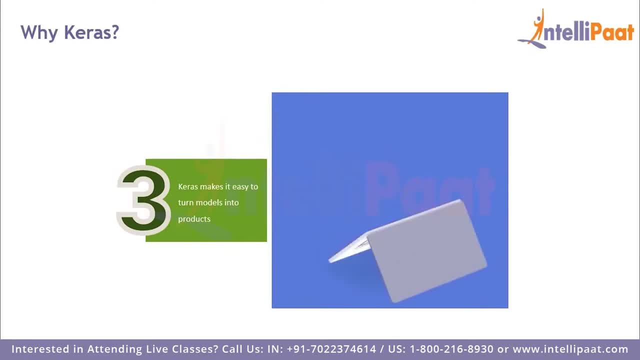 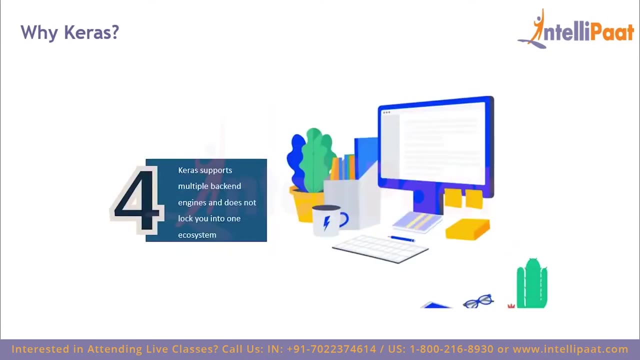 say, if you develop a simple prototype with caras and if you want to launch it on some platform, then you can easily do it. so you build a model and then you can easily launch it on, let's say, android, ios or any other operating system as an end-to-end product, and caras also supports multiple back-end. 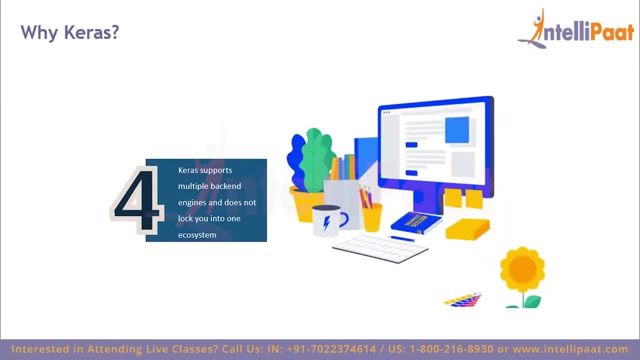 engines and does not lock you into one ecosystem. now, what do i exactly mean when i say that caras supports multiple back-end engines? well, caras is basically a high-level api, and this high-level api can run on a lot of low-level apis, such as tensorflow, cntk and theano. so now caras is what? 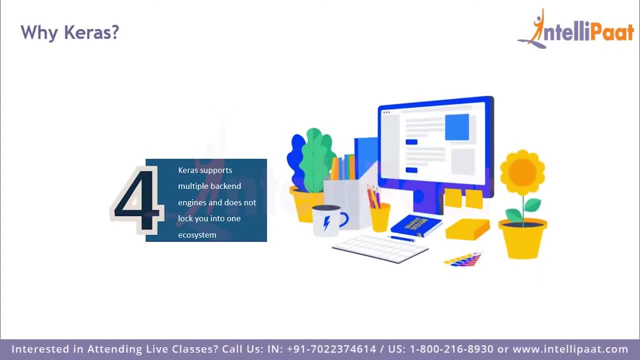 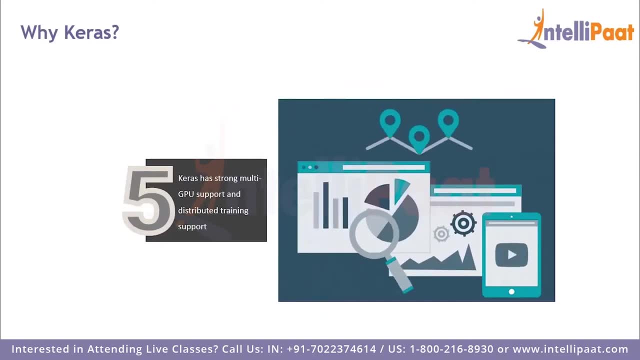 works at the front end and at the back end you have either tensorflow cntk running. right now. caras also has a strong multi-gpu support. so when i say caras has a strong multi-gpu support, what i mean is you can basically divide the data or you can basically train the data. 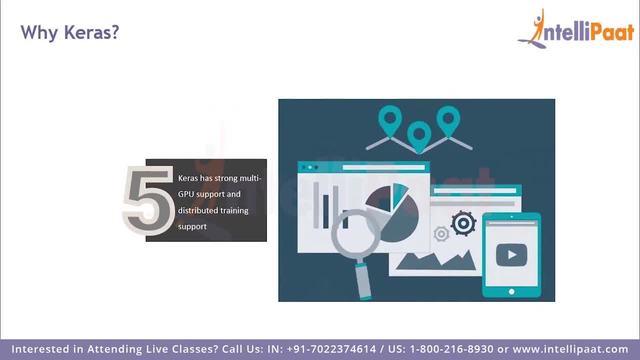 on multiple gpus. so let's say you have an input data which comprises of 100 records and you divide into five mini batches. now you can train these, each individual mini batches, on separate gpu's. so let's say you have a model and you have the input data. now you'll be making copies of this. 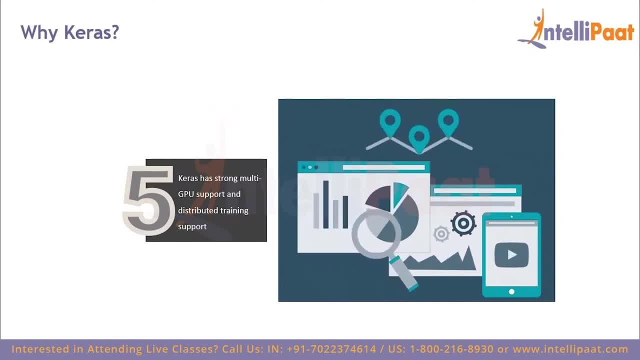 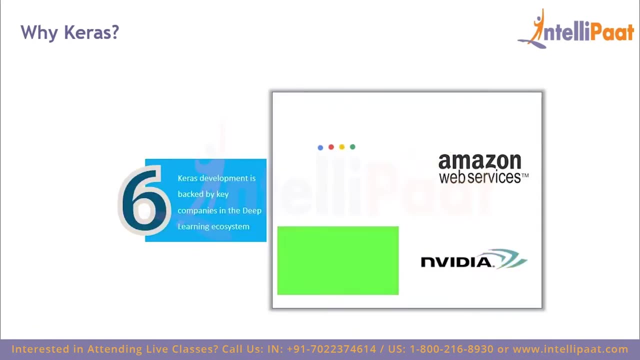 input data and each individual copy would run on each single gpu and each of that gpu would give you an individual result which is aggregated and you'll get the final result. so this basically speeds up the model building process, and caras development is also backed by all the major 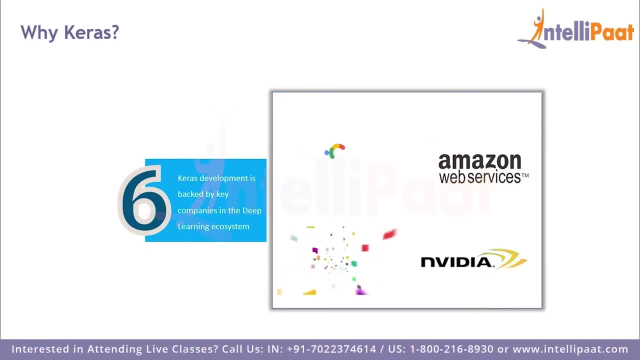 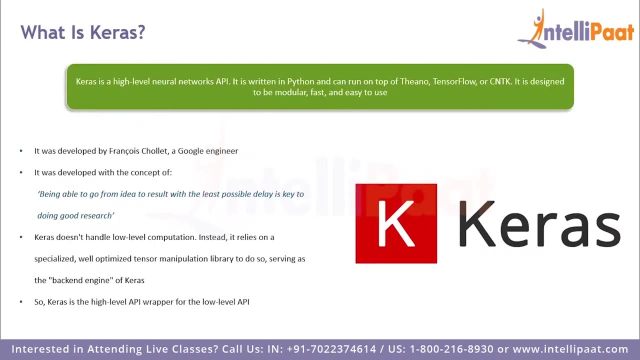 companies out there, such as google, amazon and nvidia, right. so now that we've understood what, why should we use keras? let's actually understand what is caras. so, as i've already told you guys, caras is basically a high level api and it is written in python, and this high level api can 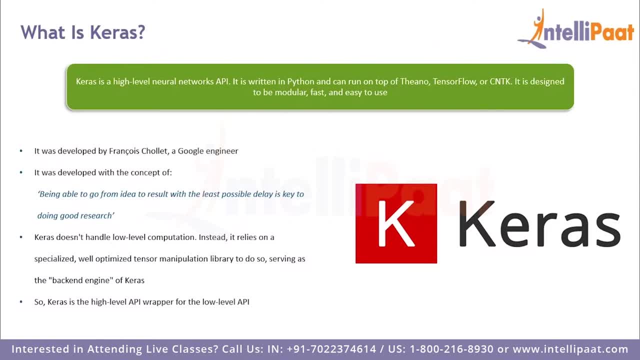 run on top of theano tensorflow or cntk, and it is very easy to work with caras. so you have individual modules and you can invoke each of these individual modules to keep adding layers on the neural network. so just as easily. well, on the cntk side, then the onto cntk side is very easy to execute. you've got. 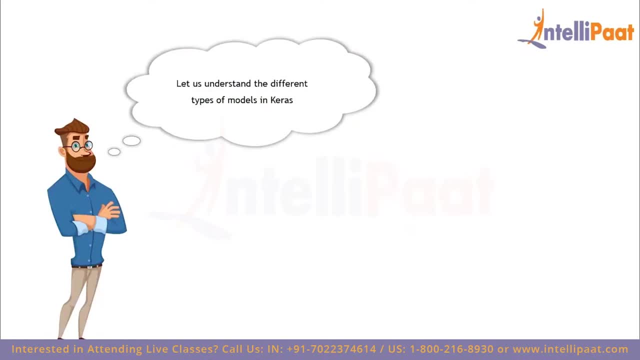 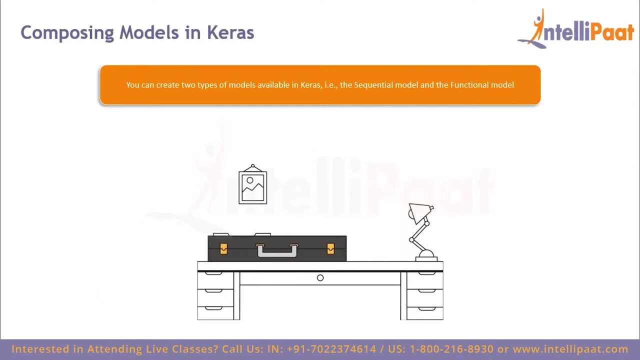 many largerانaccounts that there's some baby modules of this sui that is very vulnerable as that to work with Keras. So now that we understand what is Keras, now let's have a look at the different models in Keras. So there are basically two types of models available in Keras, which are: sequential model. 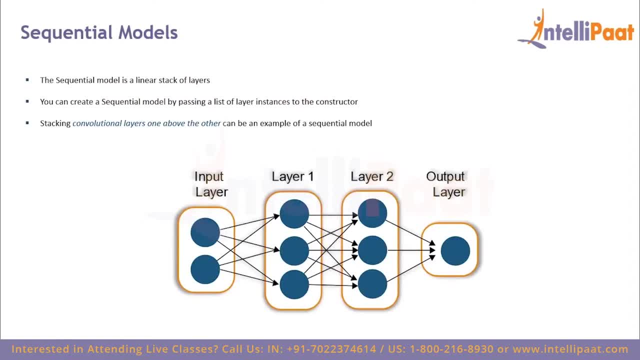 and functional model. So let's start with the sequential model. So simply put, sequential model is just a linear stack of layers. So you have one layer on top of that one layer, you add another layer. On top of the second layer, you add the third layer. 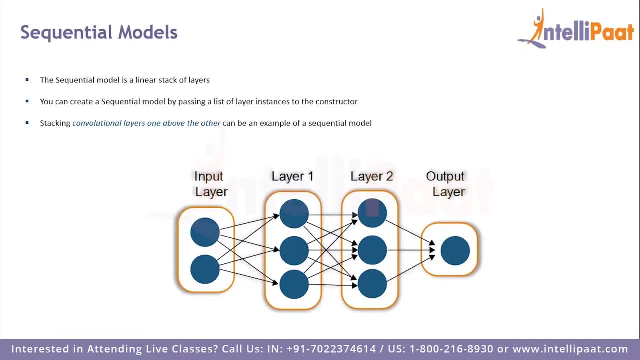 On top of the third layer you add the fourth layer, So it is basically a sequence of layers. So, as we see over here, this input layer would be our first layer And on top of this input layer we'll add the first hidden layer. 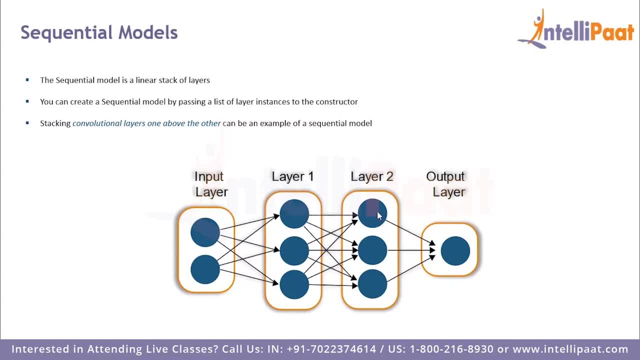 And on top of this first hidden layer we'll add the second hidden layer And finally, on top of the second hidden layer, we'll add the output layer. So, simply put, a sequential model is just a linear stack of layers which processes. 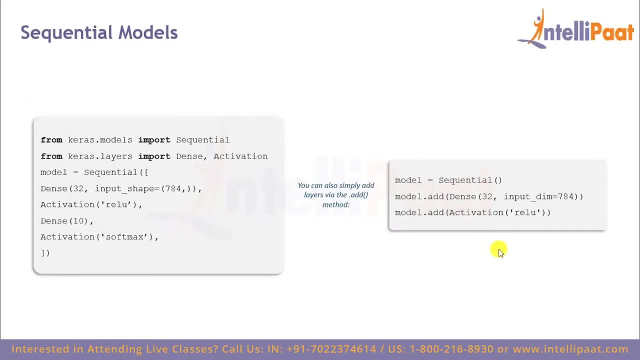 the data and gives out the final output through the output layer Right, And this is how we can invoke a sequential model through Keras. So first we'd have to import sequential from kerasmodels And then we'd have to import whatever layers that we require. 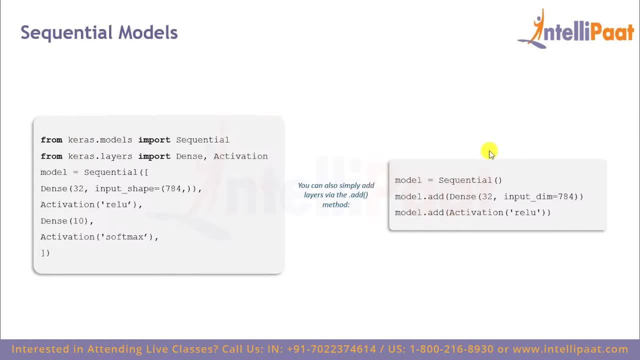 So the first step in creating a sequential model would be to create an instance of this. So we have to use the sequential method and we'll create an instance of it. So now that we've created a model, so with this model we can keep on adding layers. 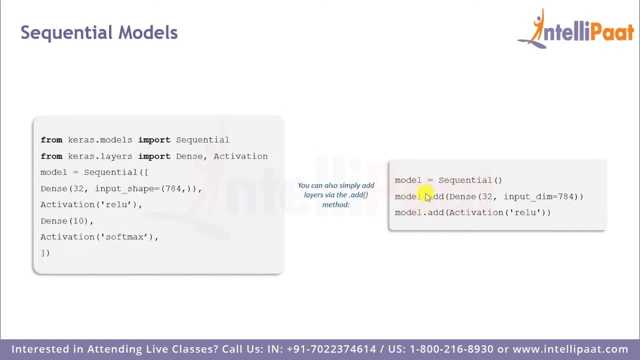 So what we are basically doing is, for this instance, I am adding the first layer. So this first layer is basically a dense layer and it comprises of 32 nodes and the dimension of the input which this first layer takes is 784.. And we are also adding an activation function to this first layer. 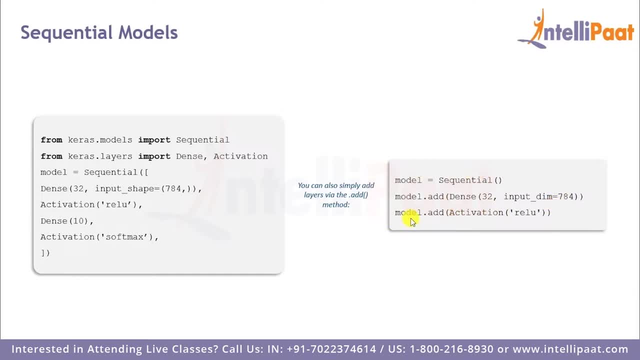 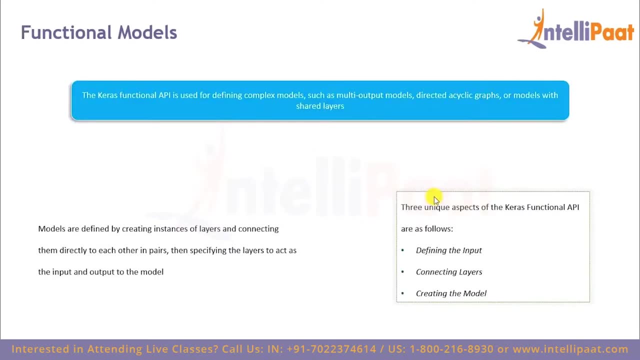 It is as simple as that. First you create a model and then whatever layers you want to add, you can just add it with the help of the add method. So this is how we can create sequential models in Keras. Now we'll head on to the second type of models, which are functional models. 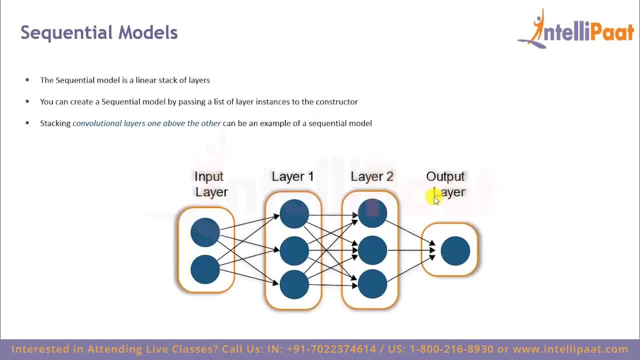 Functional models help us to create complex models. Now the problem with sequential models is you can give inputs only at the beginning stage over here. So let's say, if I want to add new inputs for the second layer, that wouldn't be possible. So once if you give the inputs, you cannot add anything else in between. 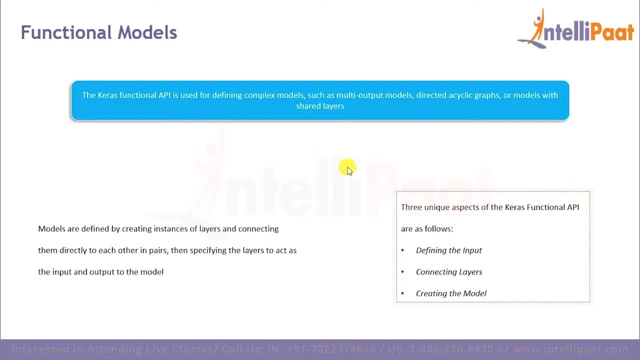 So this is where functional models differ. So in functional models it is not necessary to follow the same sequence. So when it comes to functional model, any layer can be connected to a functional model. So this is where functional models differ. So in functional models it is not necessary to follow the same sequence. 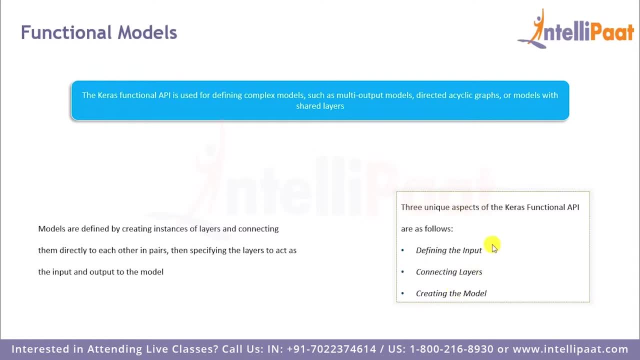 But as soon as an input is created, it will not be connected to any other layer. And these three steps which you see, these are the three steps which have to be followed to create a functional model. So we start off by defining the input. 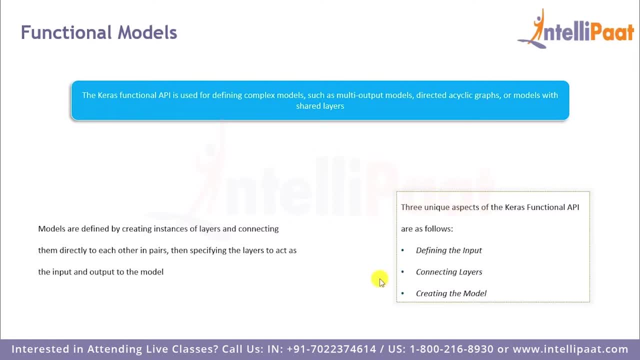 And once we define the input, we start off by building a set of layers and these layers can be connected anyway. So I can connect the first layer with the fourth layer or the second layer with the 10th layer. So I start off by defining the inputs and then I'll create the layers and then I'll. 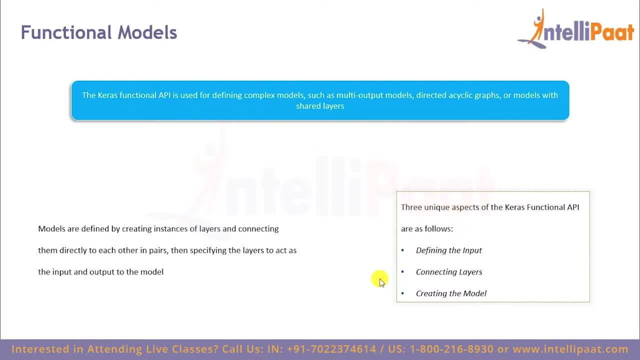 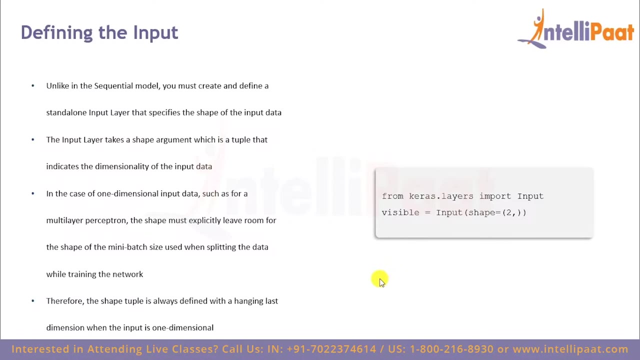 connect those layers. Finally, I will build a model. So these are the three steps involved: First, define the input. Second, build the layers and connect the layers. and then, finally, build a model, Right? So let's understand each of these steps properly. So, when it comes to a sequential model, 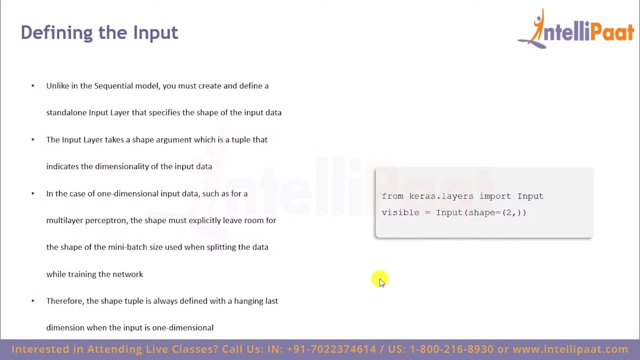 we actually have to create and define a standalone input layer that specifies the shape of the input data. So, as you see over here we are importing input method. So from Keras dot layers we are importing input and we are defining the shape of the input data, And this is extremely important. 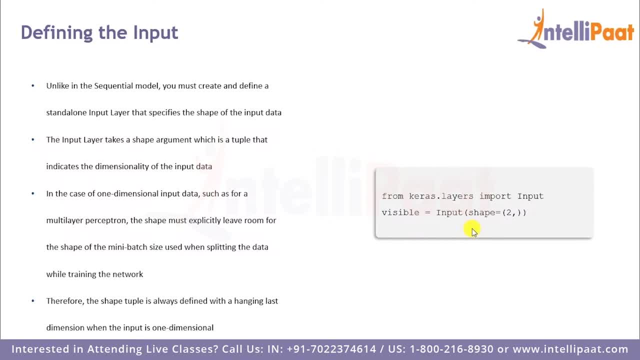 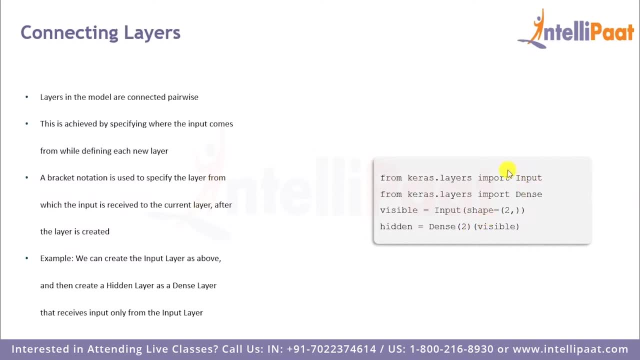 when it comes to functional models. So first we have to start off by creating the input layer, And once we create the input layer we can keep on adding other layers. So, as we see over here, first we import input method And after that we are importing the next layer, which is basically. 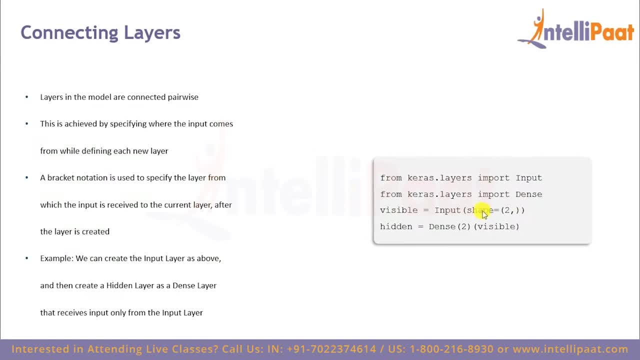 a dense layer. So, as we see over here, first we create the input layer using the input method, and the shape of the input is two And I'm storing it in visible. After that I'll add another layer. So this is basically a dense. 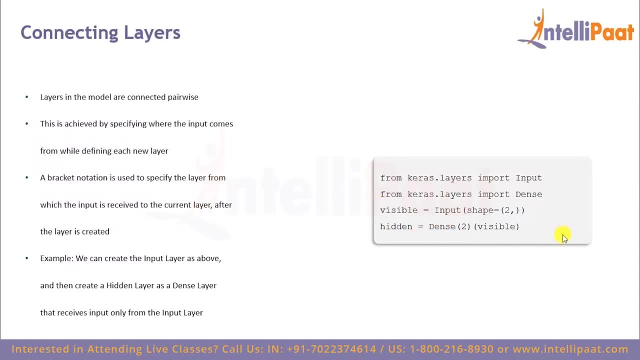 layer. Now, this dense layer has two nodes in it and it is connected with the visible layer over here, Right? So we give out the name of the previous layer after we create the first layer over here. Or, in other words, layers in functional model are basically connected pairwise. So this: 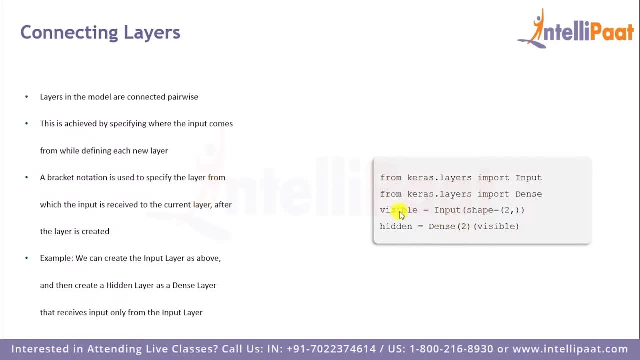 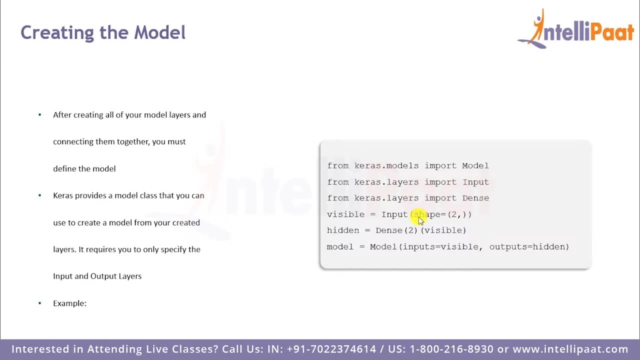 is the dense layer, and this dense layer is connected with the first input layer, which is visible Right. So we're done with the first two steps. We created the input layer and then we connected the rest of the layers. Now, after that, we have 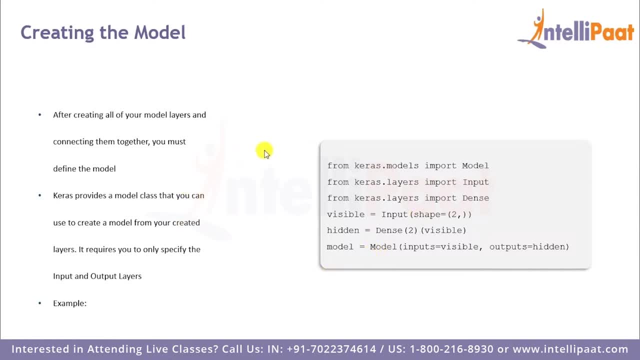 to create the model. So defining the model is extremely simple. So first we have to import the model method from garage dot models And, using this model method, all we have to do is pass in the input and the outputs. So, as we have already seen this before, input is the visible layer and 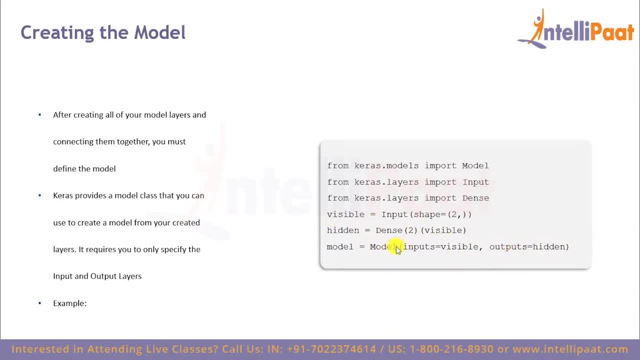 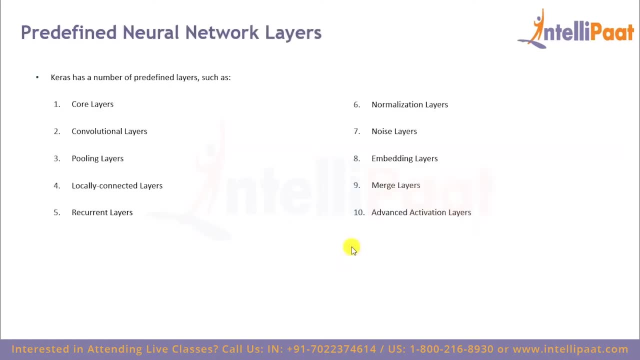 output is the hidden layer. So we are passing these two layers in this method and we are storing this in the model instance. So this is how we can create a functional model And Keras already has a number of predefined layers. So these are some of the predefined layers listed over here, So Keras can have core. 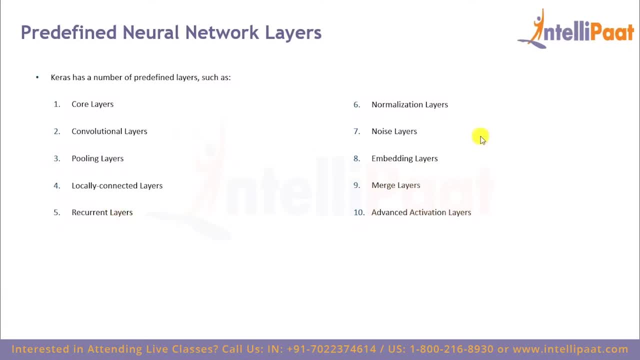 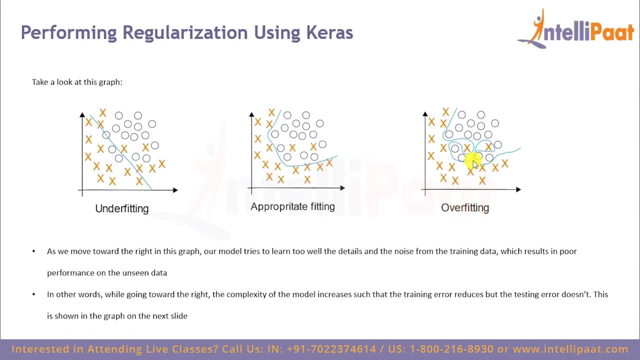 layers, convolutional layers, pooling layers, recurrent layers, noise layers, embedding layers and so on. So it has multiple predefined layers associated with it. So, now that we've understood the different models available in Keras, now let's understand some problems when we are building. 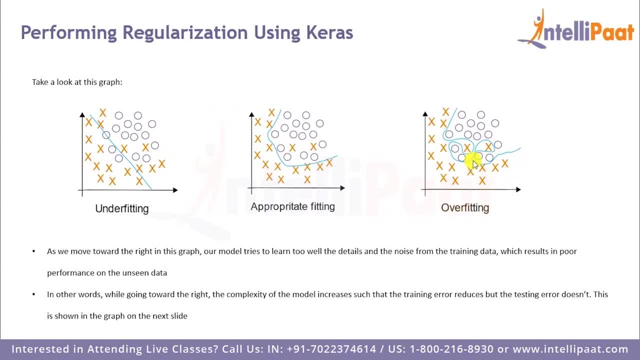 the model on top of input data. So the first problem would be to gain the maximum accuracy. But then again it is not that easy to build that perfect model. Many times what happens is our model is not able to learn the right amount of data. So let's take this case over here. So let's say we build a neural network model on top of 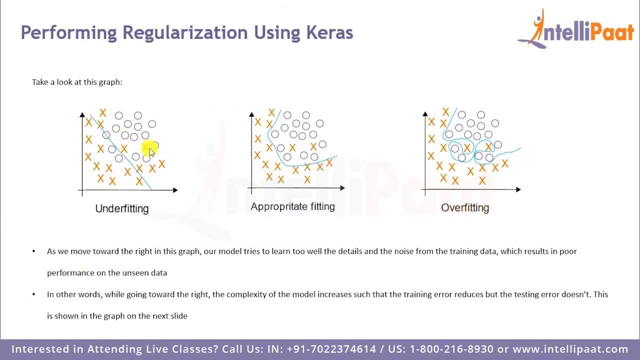 this data And our aim is to classify this data into two classes. So the first class would be this cross and the second class is the circles over here. Now, the problem with this model is learned all of the features of the data properly and since it has not learned, 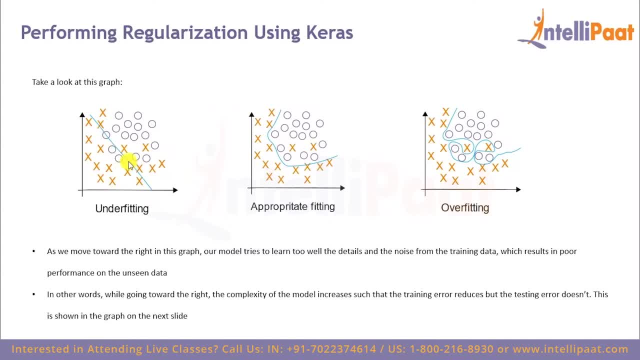 all of the features of the data properly. the misclassification over here is quite high. so these three circles, which would actually be circles, have been classified as cross and these crosses which you see, they have been misclassified as circles and this misclassification is due to the 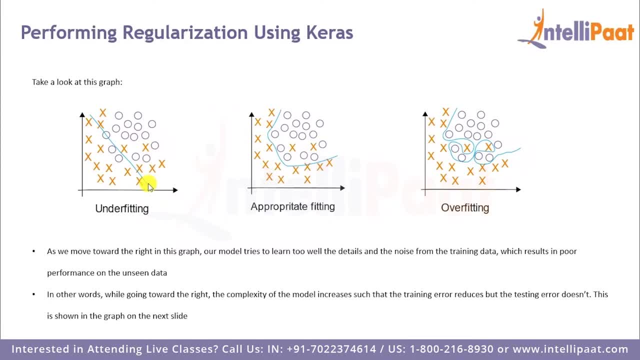 underfitting of the model. so I again restate it. so underfitting of the model basically means that it is not able to learn all of the features of the data properly. and when it doesn't learn all the features of the data properly, it is. 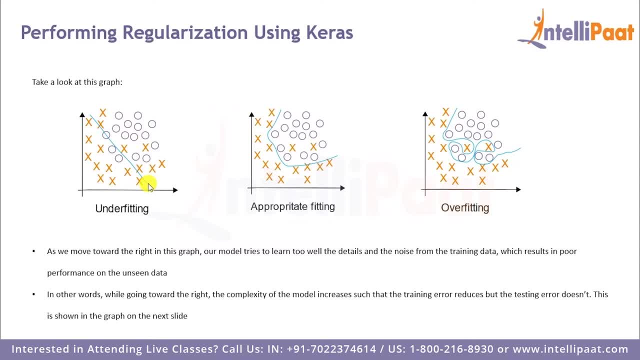 not able to predict, or it is not able to classify the problem in a correct way, or it doesn't give us the perfect accuracy. so let's see: if this model is built on the train set, then the train set accuracy would be somewhere around 65%. 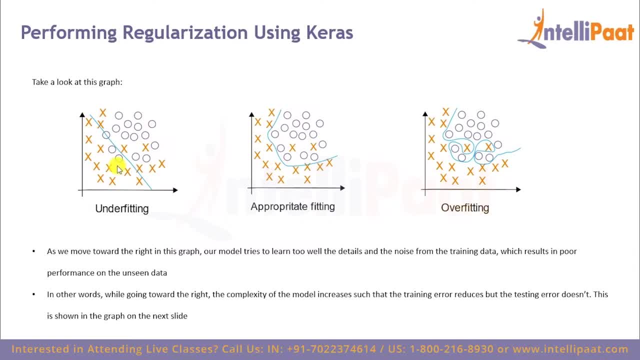 and the test set accuracy would be somewhere around 63%, which is not really that good, right. so this is basically the problem with underfitting. now, instead of drawing a straight line, what if I make the model a bit more complicated? so what I'll do? 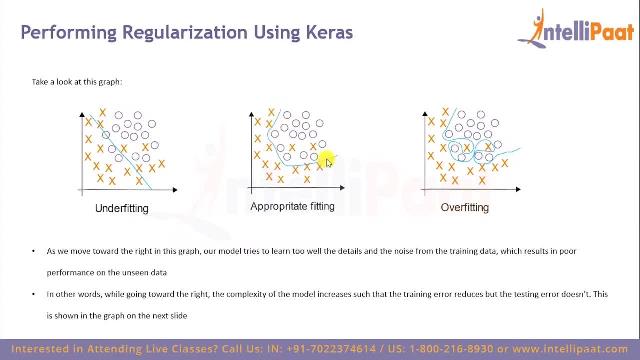 is, I'll build a polynomial curve over here. so this is a complicated model. so this complicated model is better than this model over here. so this model gives just about the right fit. so over here all of the circles have been classified correctly as circles and just these two crosses have been misclassified as. 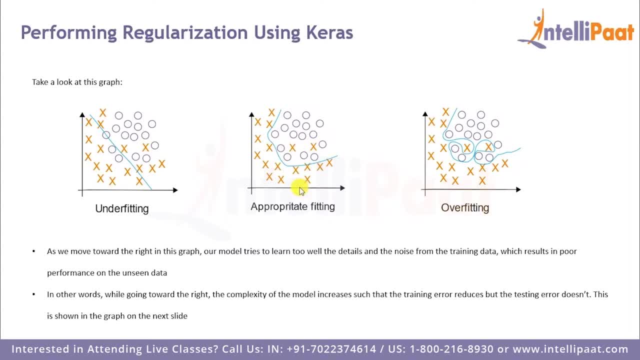 circles. so let's see, this gives an accuracy of around 95% on the train data and an accuracy offer of 93% of the test data, which is actually good enough. now what if I get over enthusiastic and build a very, very complex model with lot of? 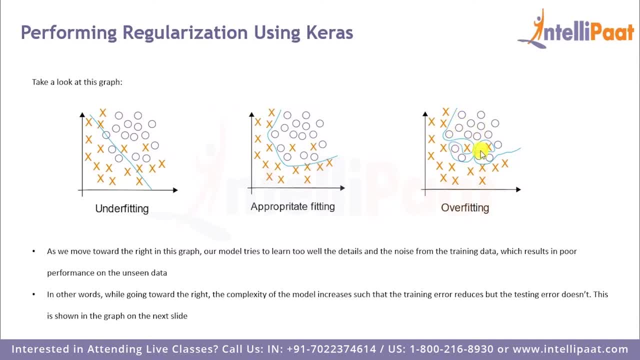 polynomial variables in it. so this would give me a curve. something like this over here: all of the crosses have been classified into one pool and all of the circles have been classified into another pool. so this basically gives a gives us 100% accuracy on top of the train set, but the problem is it fails miserably on the test. 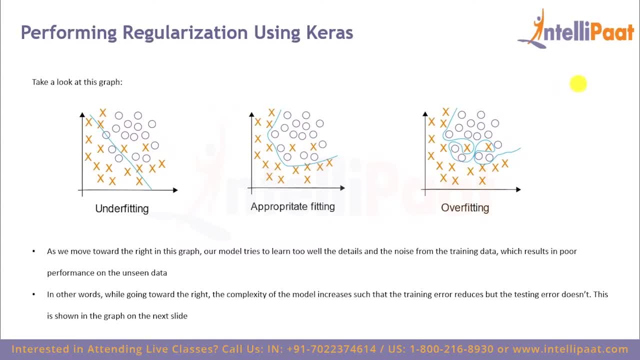 set. So the problem actually is that it fails to generalize. So when it is given the train set, it learns all of the features of this train set perfectly, and when it comes to the test set, it has not seen the test set at all and that is why it fails to perform properly on the test set. 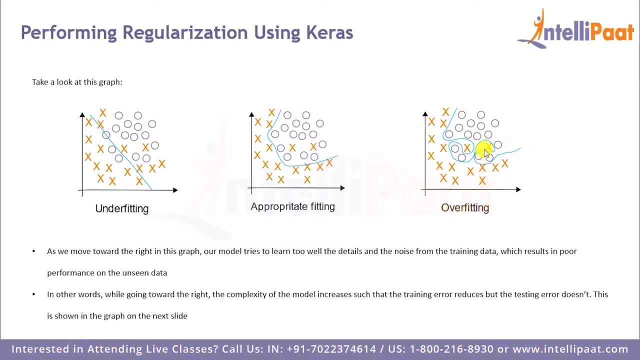 So when it comes to the train set, it gives out 100% accuracy and when it comes to the test set, it might give only around 75% or around 80% accuracy. So that is why underfitting and overfitting should be avoided and we need to find that appropriate fitting or just the right fitting. 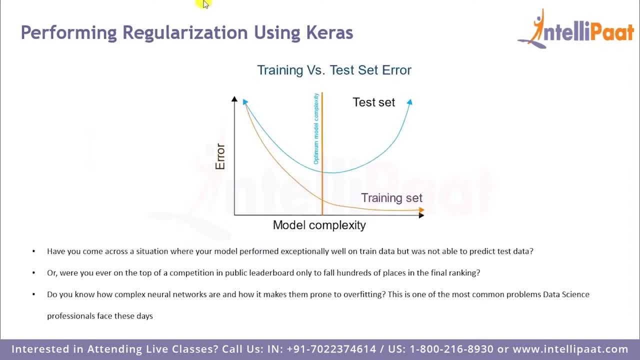 to get that ideal accuracy on top of the test set Right. so this graph over here explains this in a better way. So we have error on the y-axis and model complexity on the x-axis, As we see over here, as we keep on going, we get the error on the y-axis and model complexity on the x-axis. 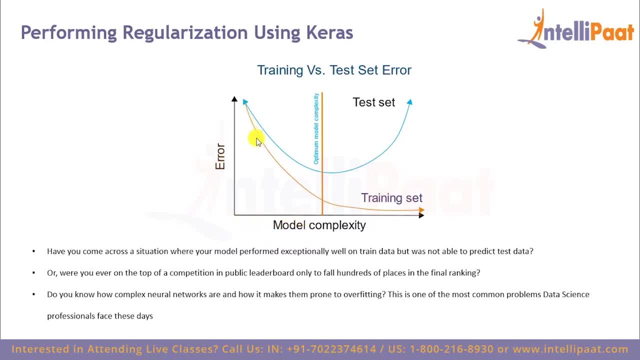 So as we keep on increasing the model complexity, the error it decreases for the training set. But what happens with the test set is as we increase the complexity the error first decreases, but then again the error increases as we keep on increasing the model complexity. Right, so to get that perfect accuracy on top of the test set, we need to find out that optimal. 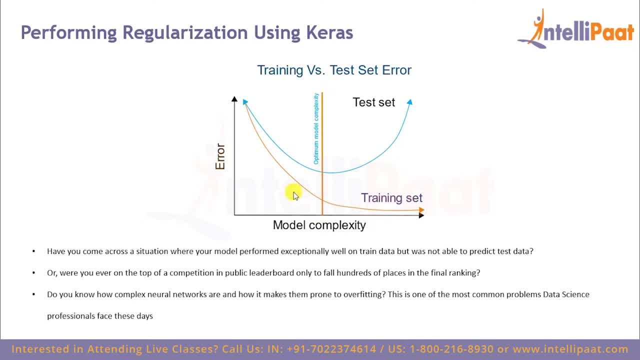 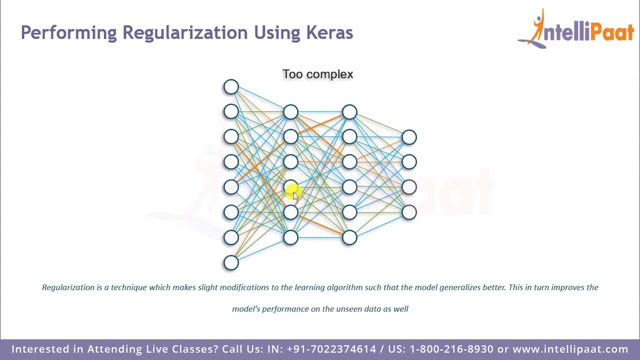 model complexity Only when we find out that optimal model complexity, that is when we're going to get the maximum accuracy Right. so now that we've understood why overfitting is harmful for our model, let's understand the solution to it. So the solution to overfitting is basically: 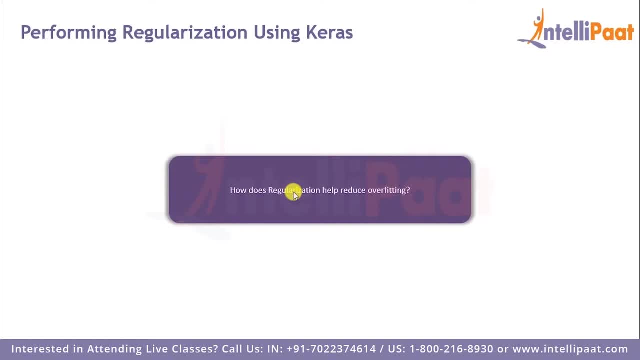 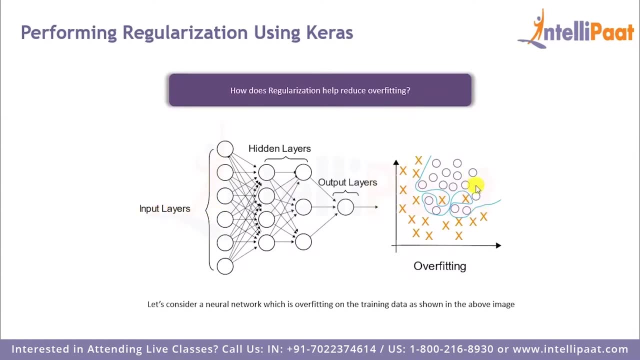 regularization. So there are some regularization techniques which help to reduce overfitting. So let's actually take this example over here. So here we see that we have built a very complex model and it learns all of the training data perfectly. But then again, since it learns all, 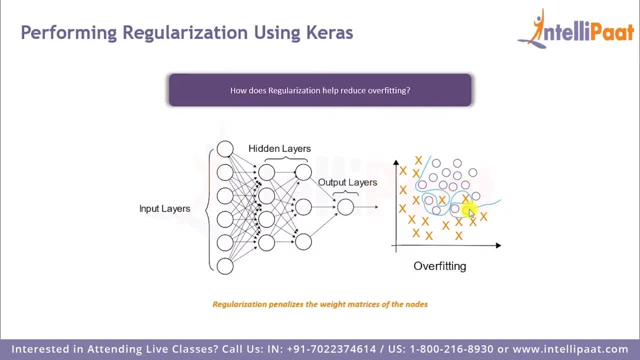 of the training data perfectly. this leads to overfitting. Now the solution to this model is would be regularization. So when we apply a regularization technique on top of this data, what happens is it penalizes the weight matrices. So when it penalizes the weight matrices, so the 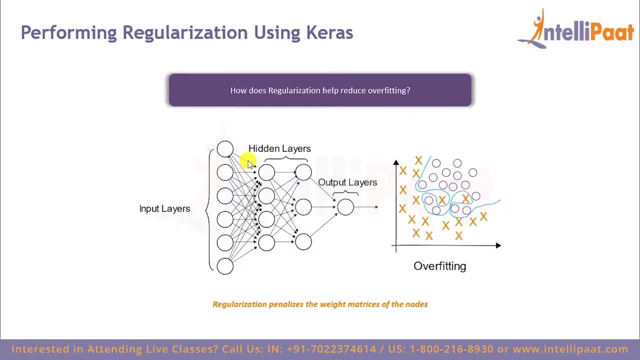 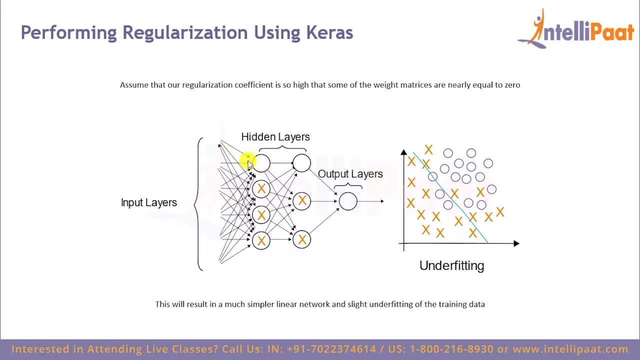 values of those weight matrices and bias matrices would change a bit and this would lead to a less complicated curve. Now also, we need to make sure that we give the appropriate value for the regularization coefficient. So if we keep the regularization coefficient to be very high, all 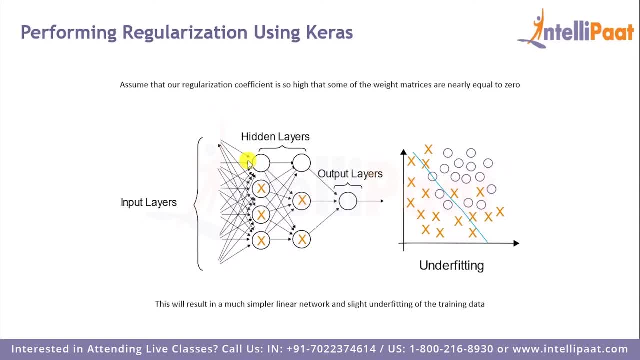 then what might happen is some of the weight matrices would become zero, and when some of the weight matrices become zero, it would basically lead to a model which is underfitting the data right. So again, when we are applying this regularization technique or when we are tuning, 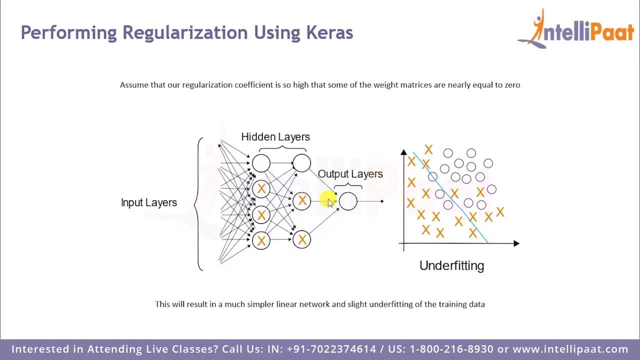 this regularization coefficient, we have to make sure that we don't alter the weights too much. and if we alter the weights too much, then we might end up actually underfitting the model, And that is something we have to avoid. So that is why we have to find out that right value of 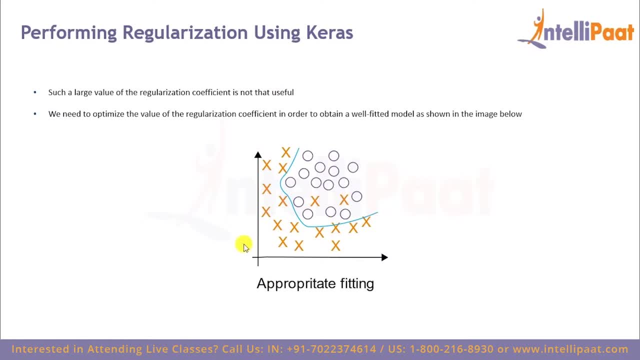 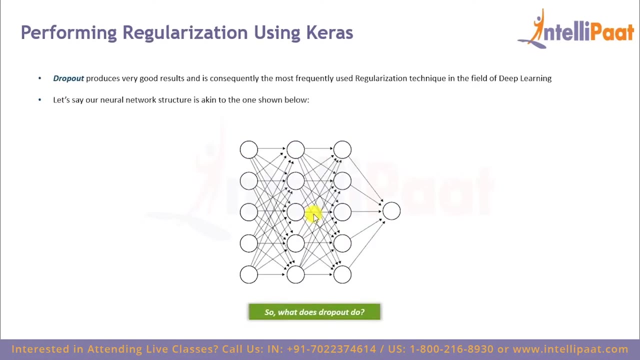 regularization coefficient which would give us this appropriate fitting. So we don't want a model which is too complex or too simple. We just want that right fitted model which is able to give us the perfect accuracy on top of the train set as well as the test set. Right now let's actually 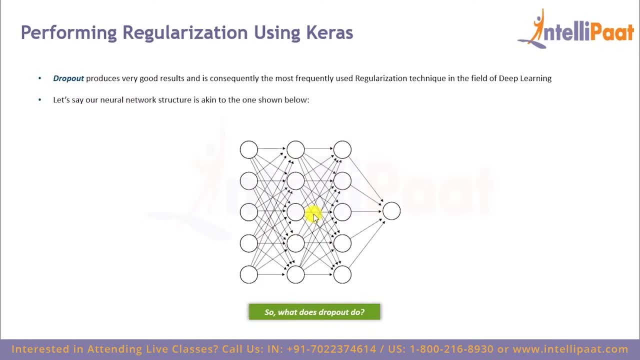 see some regularization techniques. So one regularization technique could be to add drop odds in our neural network model. So now the question in your head would be: what exactly does a drop out do? Drop out basically means that we randomly remove or cancel some nodes during each iteration. 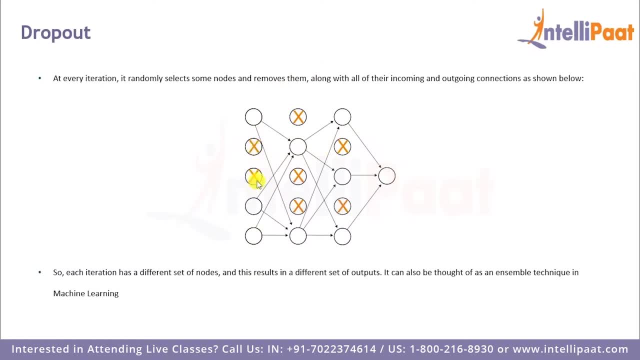 So, as we see over here, in the first layer these two have been dropped out or these two have been removed. Similarly, in the second layer, these three have been removed, and in the third layer, these two have been removed. So this again is an arbitrary choice and we can give any random value. 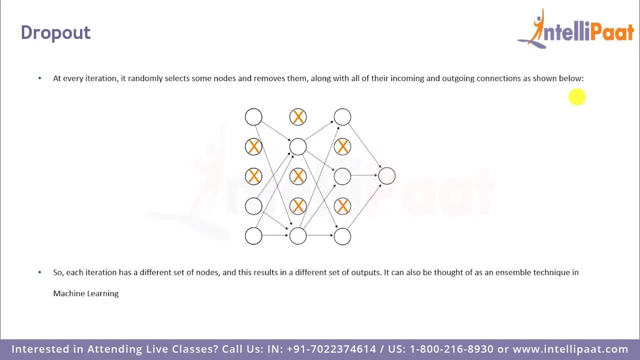 to each of these layers. So now that we know what exactly dropouts are and what exactly they are, let's understand how they are helpful. So when we cancel out these nodes during every iteration, they do not memorize the data. And when they don't memorize the data, this actually, in turn, helps in. 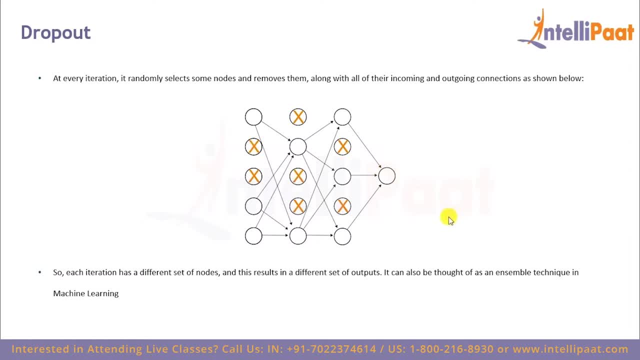 not to overfit the data. So let's actually understand this through an example. So let's say we have this training data and we are building this model on top of the training data, and this training data goes through three epochs or three iterations. So in the first iteration in this 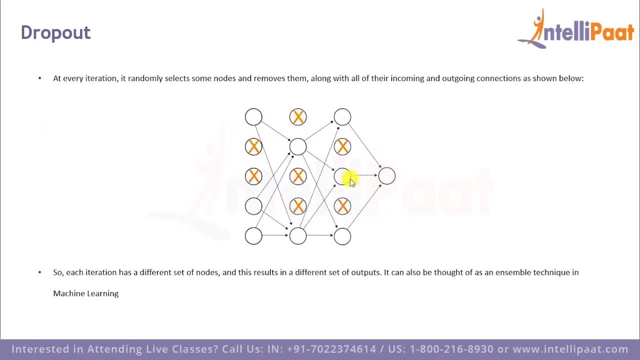 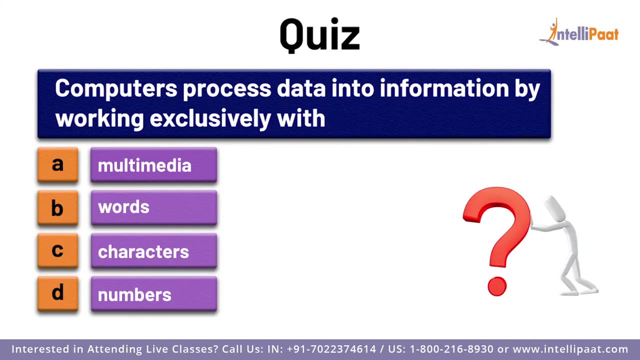 layer, these two are cancelled out. In this layer, these three are cancelled out. and in the third layer, these two are cancelled out. Just a quick info, guys. Test your knowledge of computer vision by answering this question. Computers process data into information by working exclusively with which of the following? 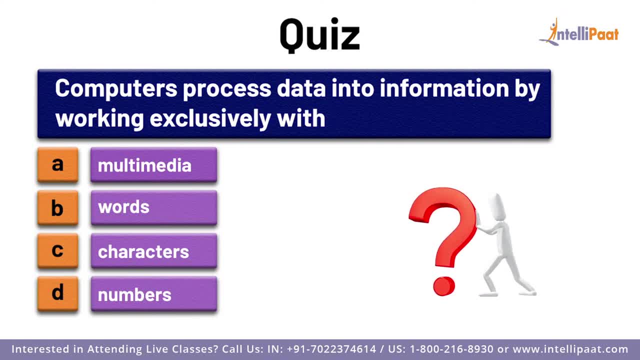 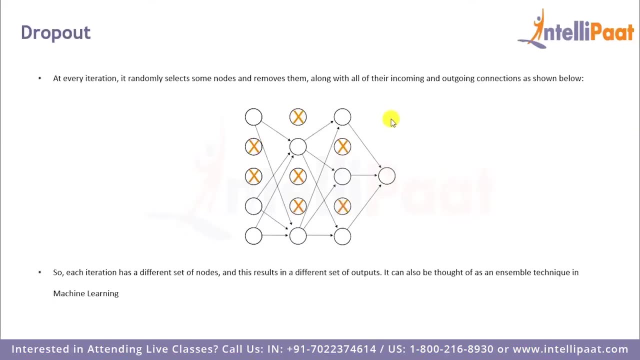 A Multimedia B- Words, C, Characters, D, Numbers. Comment your answer in the comment section below. Subscribe to IntelliPath to know the right answer Now. let's continue with the session Now. this is only with respect to the first iteration. 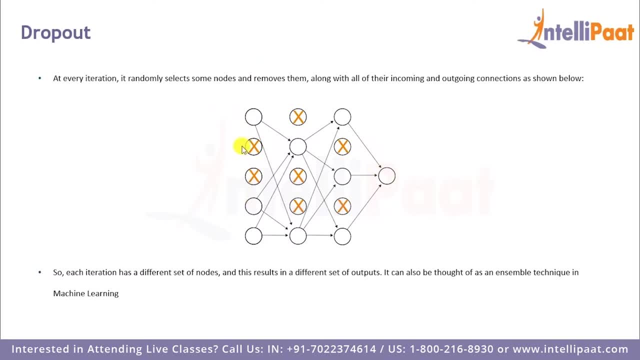 Now in the second iteration, again a random set of two nodes would be cancelled out, And it's not necessary that these would be those two nodes. So those two nodes could be either this one and this one, or this one and this one. 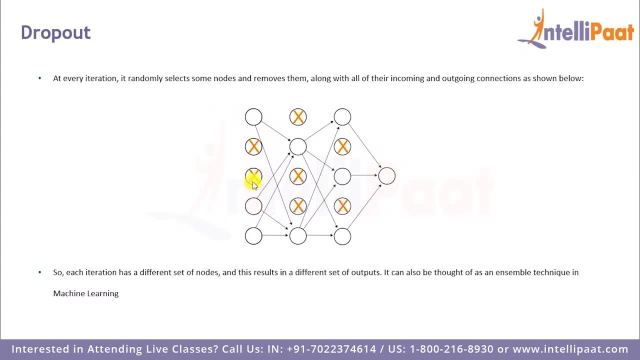 So it could be any random combination of two nodes which are cancelled out from this first layer. Similarly, again from this second layer, a random combination of three nodes is cancelled out. Again in this third layer, a random combination of two nodes is cancelled out. 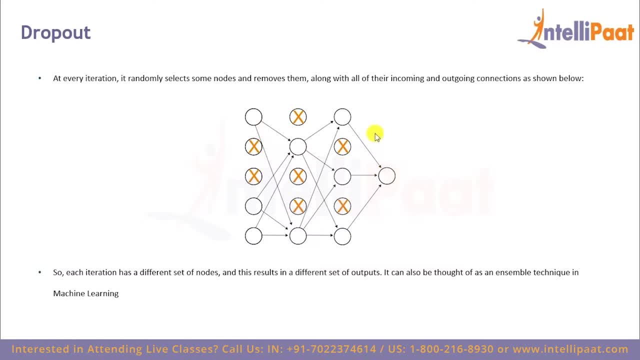 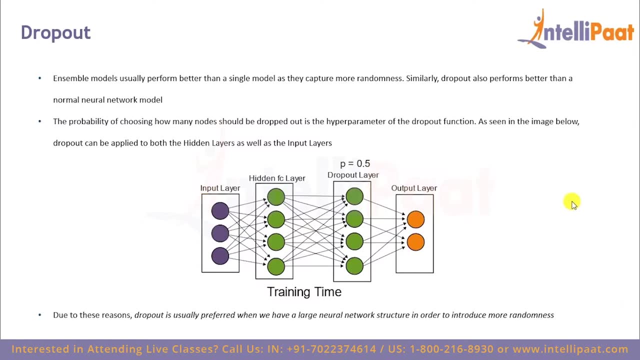 Again we'll come to the third iteration. Again the same thing happens in the third iteration. So basically, adding a dropout layer works as an ensemble model. So every iteration gives slightly different model. So in the first iteration we have different set of nodes which are giving the output. 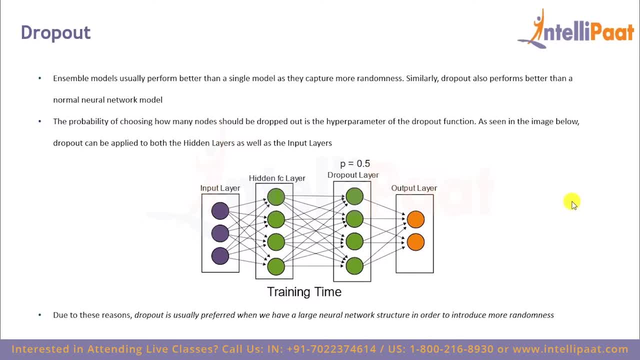 In the second iteration we have another set of nodes which are giving the output. Similarly, in the third iteration we have totally different set of nodes which are giving the output right. So a dropout layer basically works as ensemble models through each iteration. 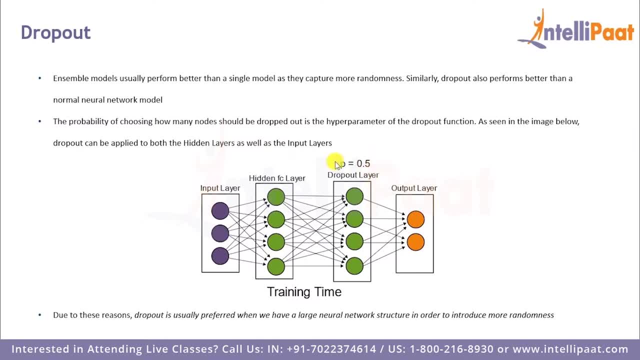 So we can basically set a probability of number of nodes to be dropped out. So over here p is equal to 0.5.. So this means that the dropout percentage would be 50%. That is, we'll be keeping two nodes and we'll be removing two nodes. 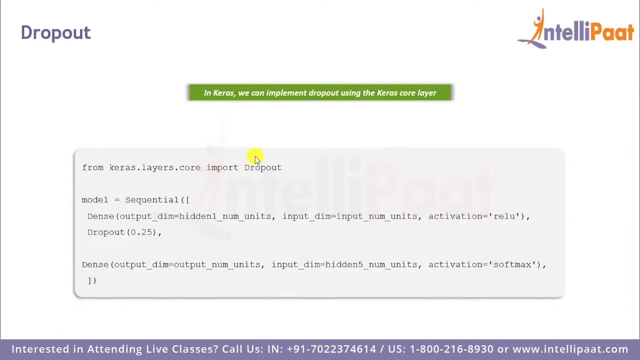 And it's extremely easy to add dropouts with Keras. So first we'd have to import the dropout method from keraslayerscore. So once we do that we'll build a model, and in this model we are adding a layer over here. 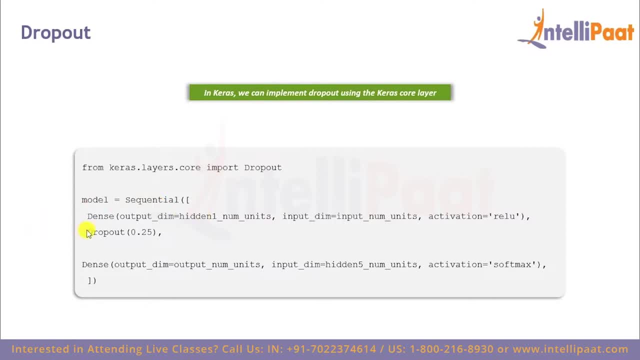 Now for this layer, for this dense layer over here, we are adding a dropout And the probability of the dropout- we are setting it to be 0.25.. So it's as simple as that. So all we have to do is use this dropout method and set in the probability of dropout. 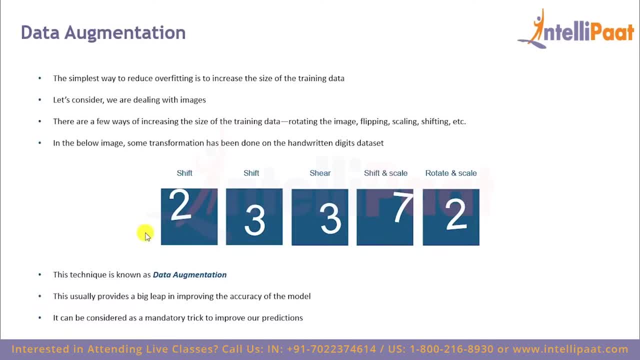 So adding a dropout layer was one regularization technique. Now we also have another regularization technique, which is data augmentation. So the simplest way to reduce overfitting is to increase the size of the training data. Now, how can we increase the size of the training data? 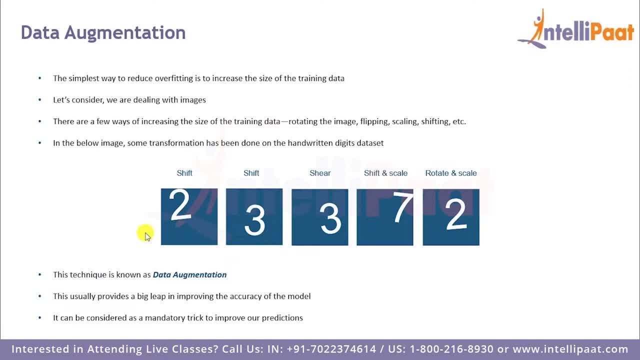 Well, we can basically modify the data to increase the size of it. So let's say we are dealing with images, or images of these numbers over here. Now, in this case, what we can do is we can augment the data. So let's say, I have the input data, which is basically image of the number two. 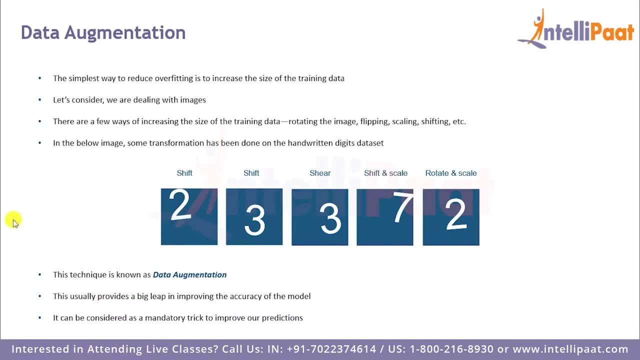 Now, if I want to create a duplicate of this image, what I can do is I can add some sort of transformation on top of it. Let's say, the initial image, which had the number two, was over here at the center. 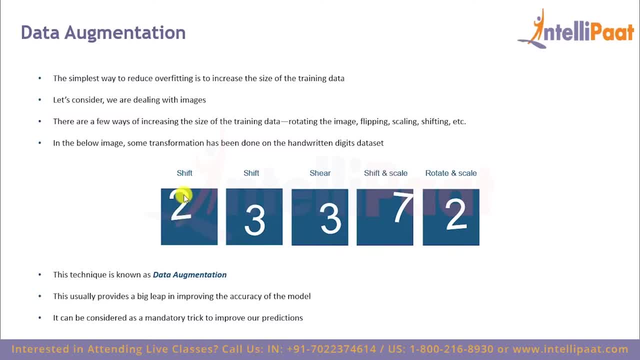 So, instead of keeping it at the center, what I'll do is I'll move it up. Similarly, let's say, if I had the number three over here in the center, I'll move it down. Similarly, over here, the number three, I'm pushing it to the right and not just. 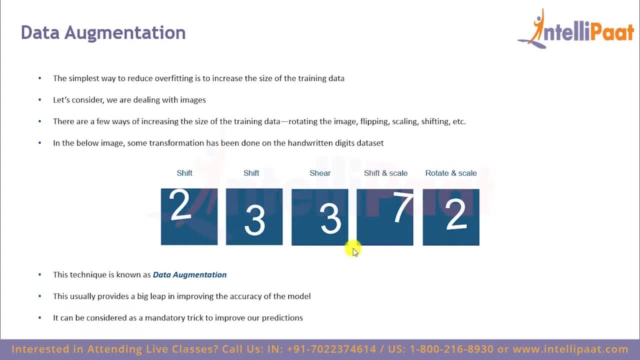 moving them to the top, bottom left. We can also flip the image. We can also scale the image. So let's say, this is my input image seven. So instead of keeping it like this, what I'll do is I'll flip it inverted like this: 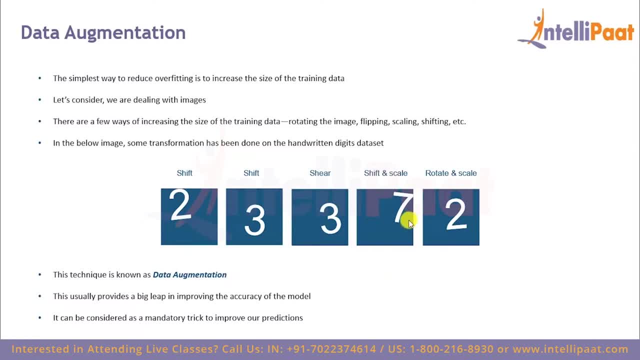 So I'll flip it and it'll be inverted, And also I can scale it up, Or in other words, I can also increase or decrease its size. So these are different transformations which I can apply on top of the input data. so 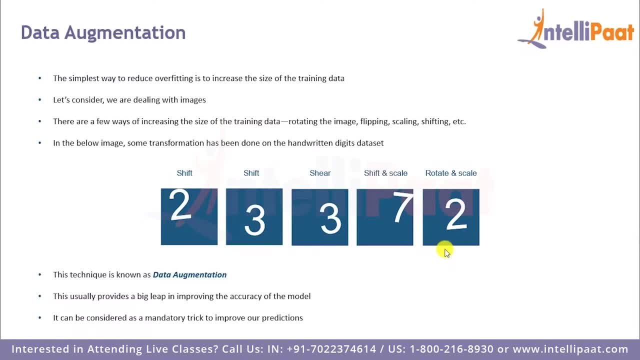 that I can create more records or records which are similar to the original records. So, let's say, if my input data consists of images of the first hundred natural numbers, Now if I want thousand records instead of hundred records, all I have to do is add. 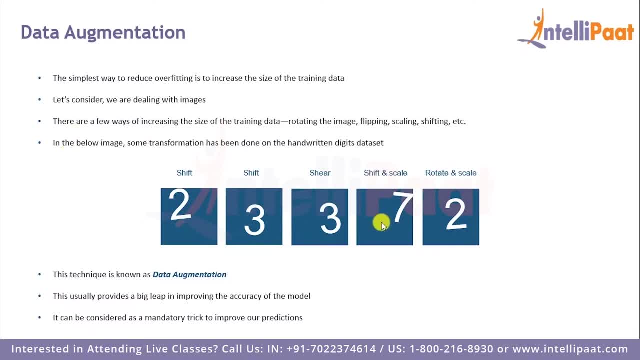 some sort of transformations on those original records, And I have records which are pretty much similar to the original records. So this is how we can augment the data. Now, what is the importance of data augmentation? Well, when we have more data, obviously it'll be difficult for the model to learn all of the features of it. 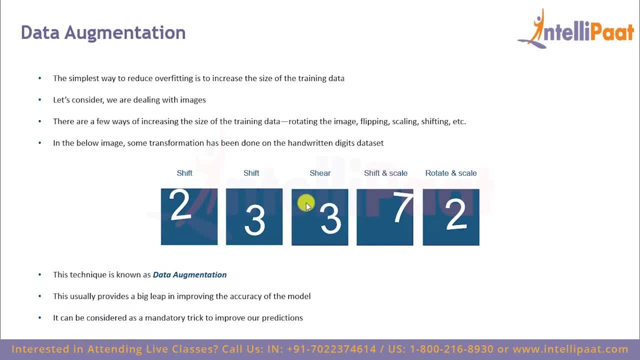 So when we have less training data, then it is very easy for the model to overfit it. And when we have a lot of data, the model will obviously take a lot of time to learn all the features And it is difficult for the model to overfit it. 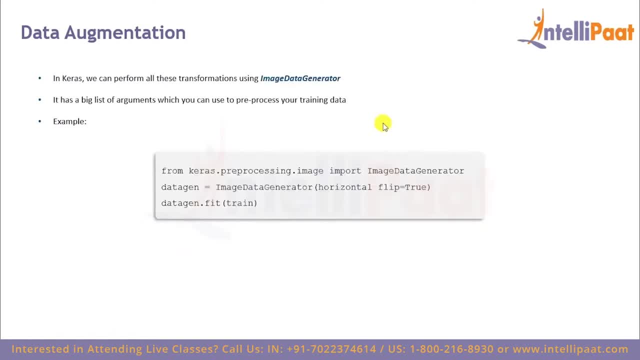 So this is how data augmentation works, And, when it comes to Keras, we can perform all of these data augmentation strategies using the image data generator method. So we have to import this image data generator from keraspreprocessingimage And it has a big list of arguments, as over here. we are setting the horizontal flip to be equal to true. 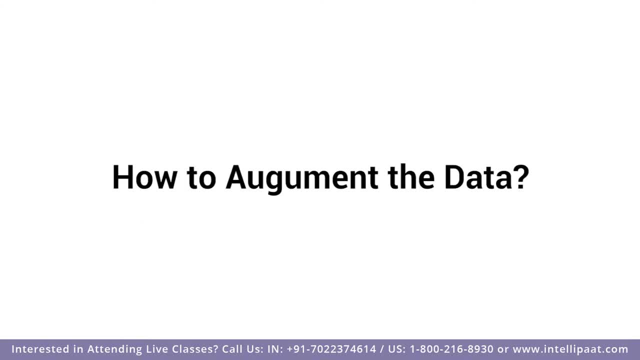 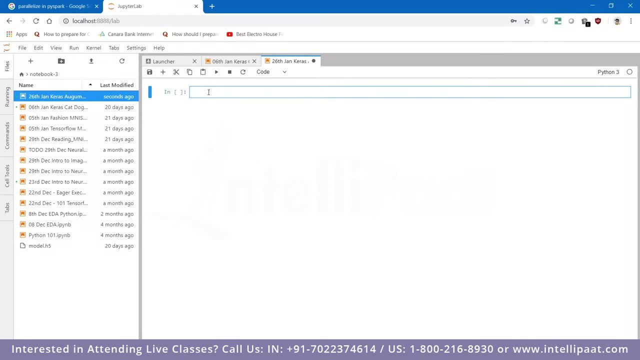 So, similarly, there are a lot of arguments which we can play with. OK, first step: what we're going to do is we are going to learn that how do you augment your data or how do you increase your data set? We have less amount of data, right? 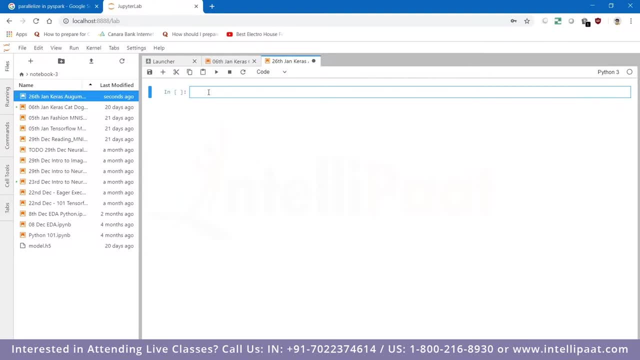 So we learned that we have only 200 images of each category, and that is not good for building a model out of it. right? We are going to augment our data. Until then, let me show you that we have this data set. 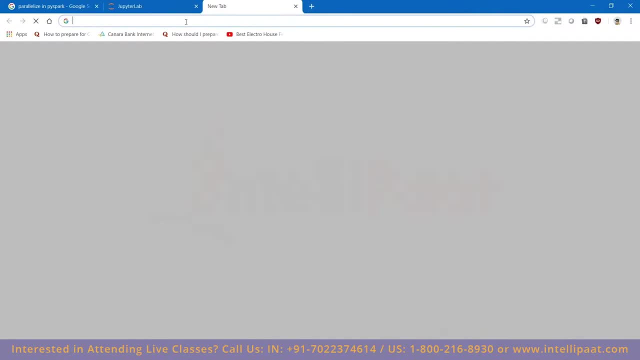 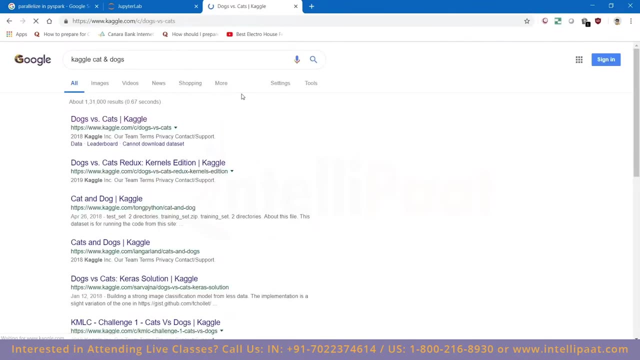 And OK, before showing you how do we get this data set, you all can also get it. Just, this is a. this was a Kaggle competition, Cat and dogs. You can download the data set from here quite easy. Let's go on this, OK. 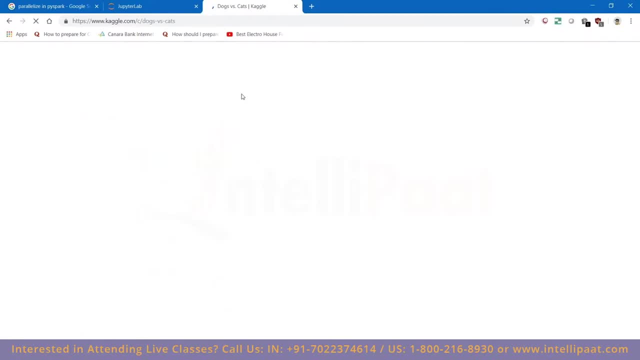 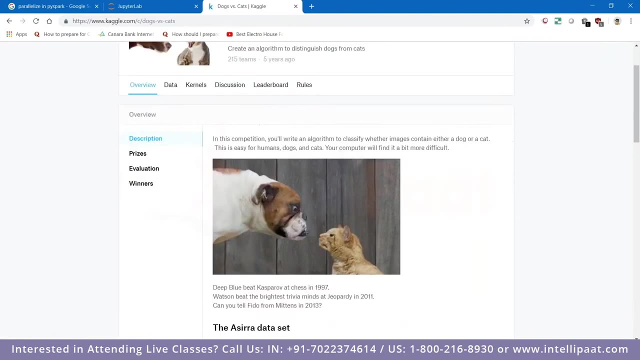 Everybody has an account on Kaggle right. If not, then now. just now, create account right, While you are listening to the class. just create account. So this competition started almost like five years ago, if I remember- Yes, five years ago. 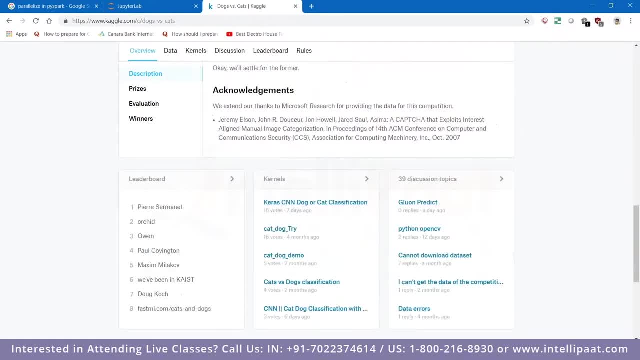 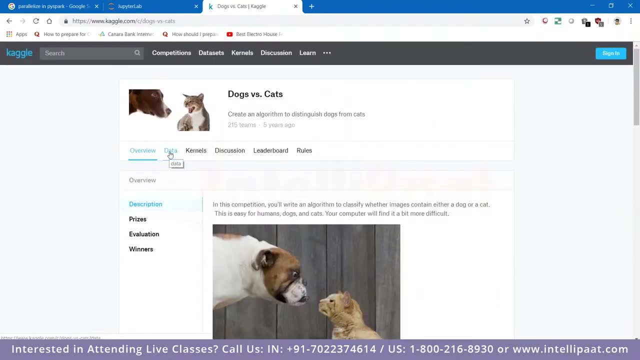 And they made the data set And this is like one of the benchmarks to start with deep learning, And people say so. people have done different things And before we even start with this problem, let me introduce you to those who don't know: Kaggle. 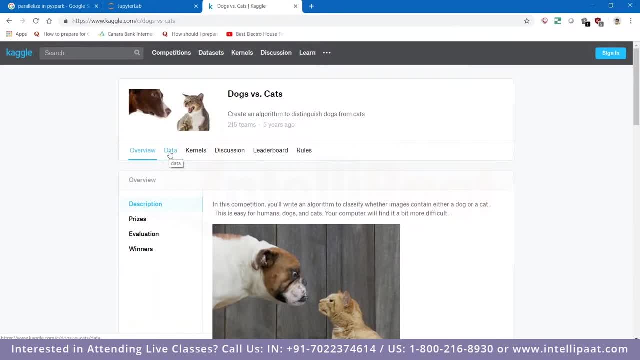 Kaggle is actually a platform. It's a platform for data science, ML, AI, competitions. Kaggle what it does is that it is in collaboration with very big, large corporations like Walmart, like Google, Facebook. So these people, they are ready to give their data. 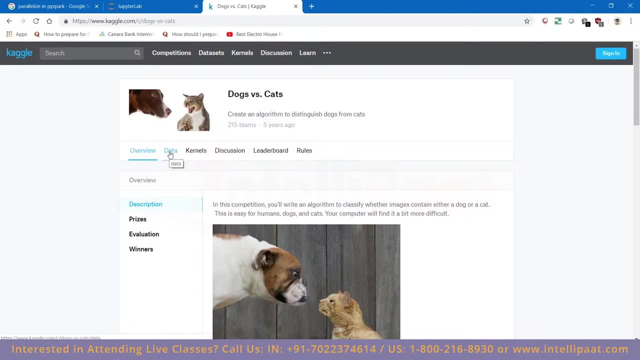 But in return they want that if they are hosting a challenge, they should come up with a solution also. So what Kaggle does is Kaggle collaborate with these big corporations. Corporations give them the data and then they host a challenge. They challenge multiple people from all over the world. 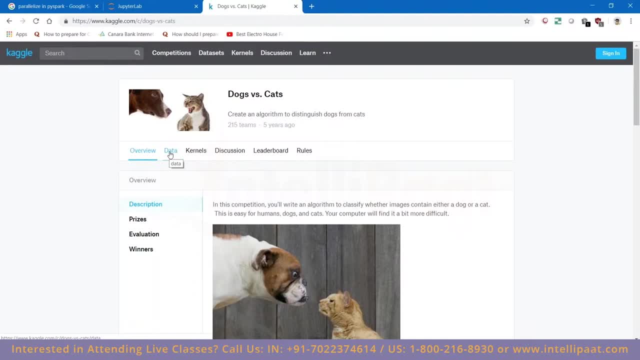 They come together and they solve the problem through this Right. So Kaggle is not just only a data solving platform, but a collaboration platform also. You'll come to know what multiple people read their problem statements. see their solving approaches. how do they solve? 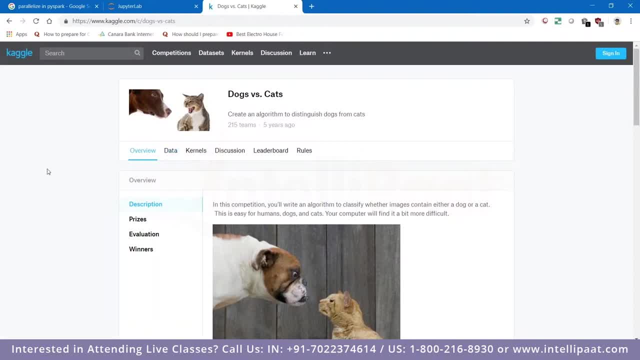 And second is that companies are also like learning new things from here. What they're doing is they're seeing people. OK, you are performing well in Kaggle. It means you're a good data scientist. You're hired. So I know two or three of my friends who 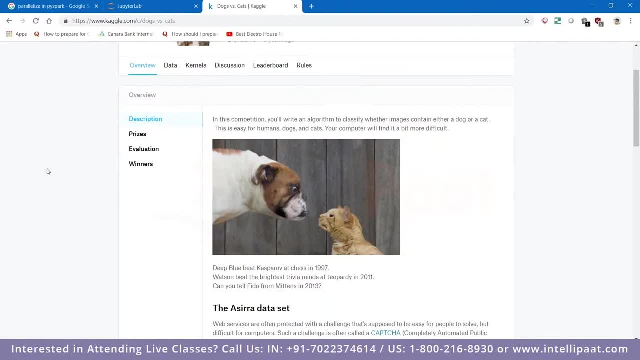 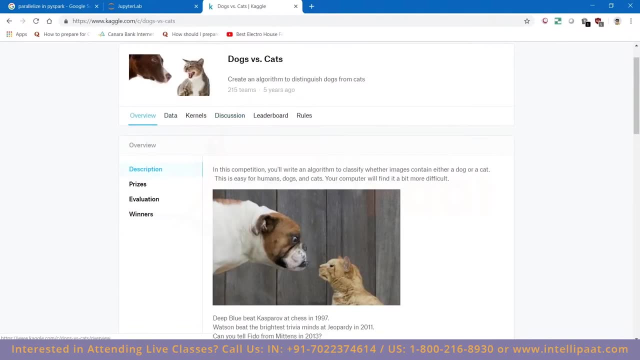 got hired just because of their Kaggle profiles. So always maintain a good Kaggle profile. Start working on this, The Kaggle problem. at every problem you'll see these six tabs. The worst one is the overview, where you read about who has given the data. 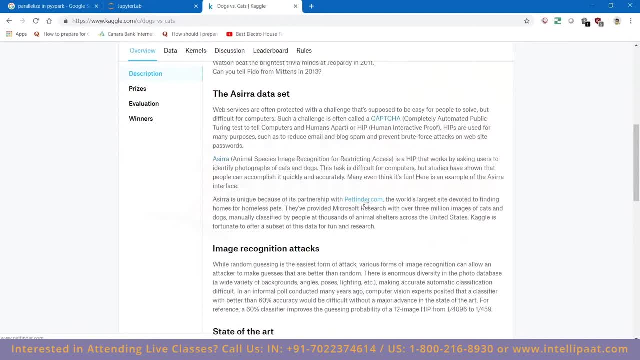 This is a Petfindercom, I think Petfindercom. they started a new competition almost like two months ago, So yeah, it is a bit in that. So actually, they actually have a team of a few teams and they want to test it out. 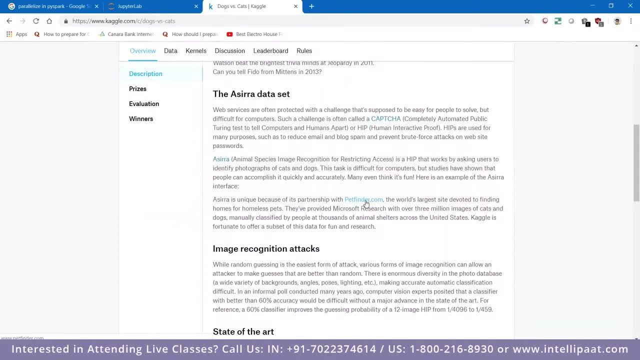 And when they do test it, they're like starting to analyze what their data looks like. who got the data? And then the thing you're going to get is: what are the rate of evolution of the data? So the answer to this question is the same. 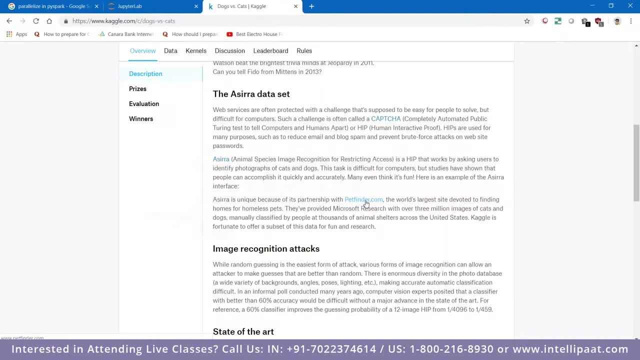 it doesn't matter. what the data you get is the same. what the data you get is the same. So what the data you get will be the same, because you get the data from the data you send to the processes. it doesn't matter what you get, the data is going to be the same. 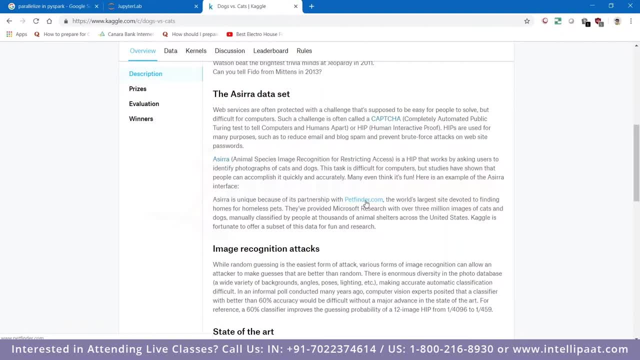 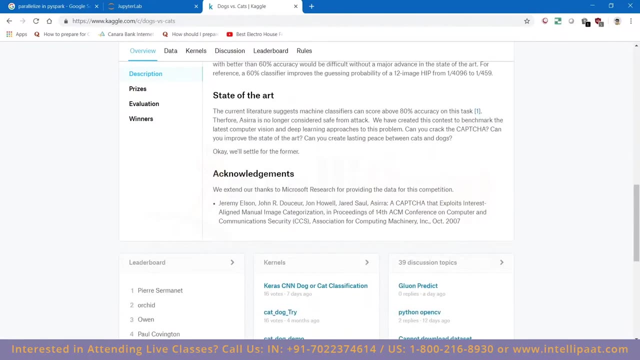 And the next thing that I mentioned is the other one, the first one, so that they can propose him or her at the very first instance. it was the recent problem and that was classical problem of NLP plus image. you should try this. this is a very old problem. the benchmark second tab comes your data tab. 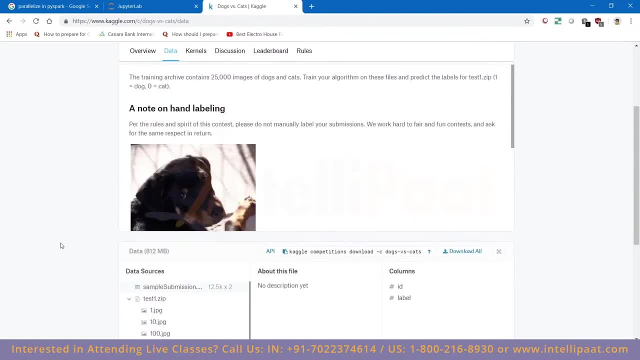 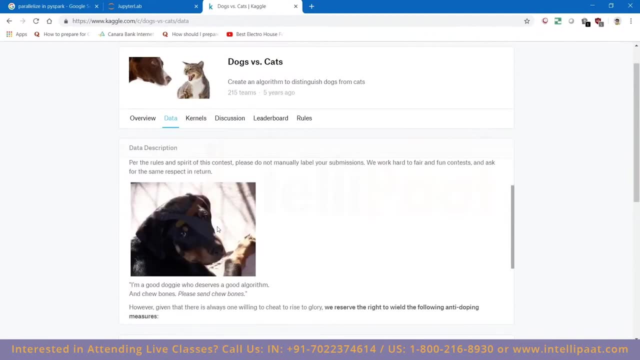 here. you can come on this tab and it's a very important app. people generally miss this tab. it is here where this thing is written. so multiple people they have come up to me and they say, okay, how do I know that this is a? so? so then you. 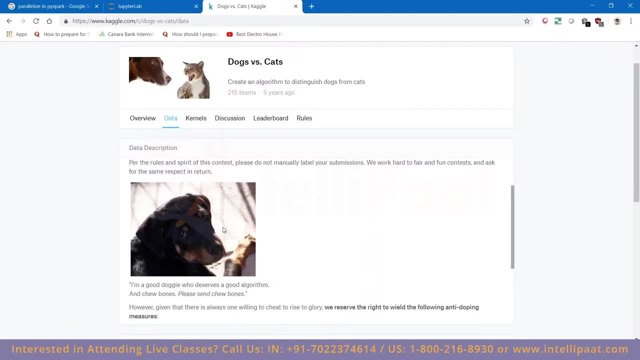 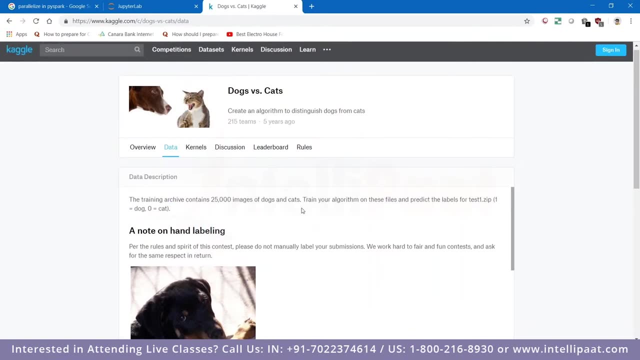 download this data, they will give you all the images. now you have got the images, how do you know which one is cat and dog? so they have written here that in your, in your dimensions, that you'll see that all the image names have a label inside them. so the image name would be cat, dog, some number, dot, jpg or. 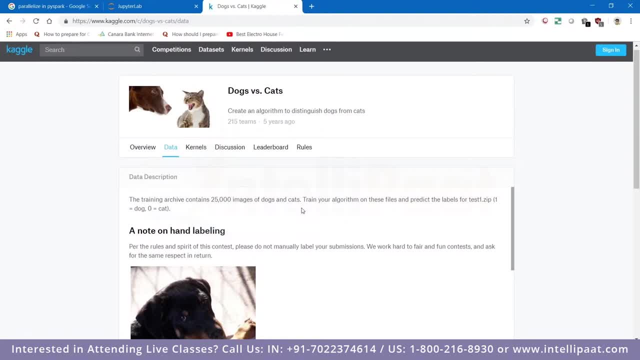 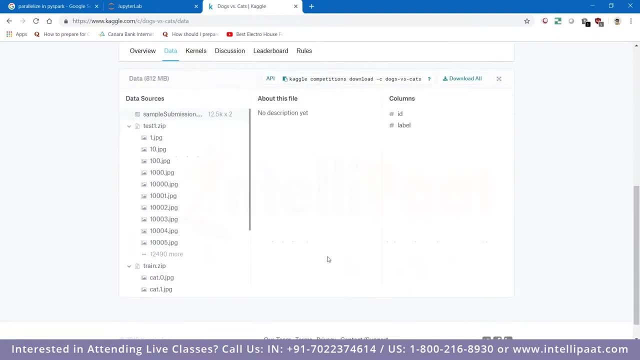 dog, dot some number dot jpg. while you're training you should keep one for dog and zero for cat right. second is all terms and conditions. but okay, you can click here, download all and it will download a data site for you right thing displays. okay, this doesn't. 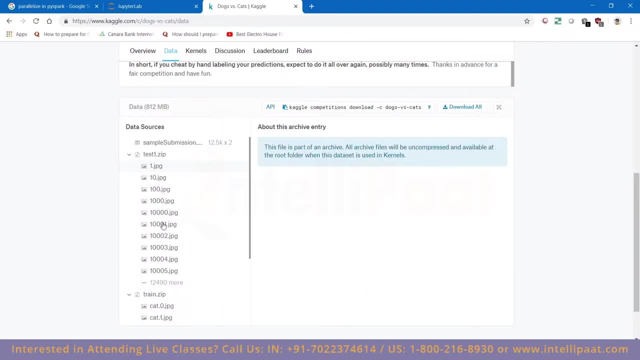 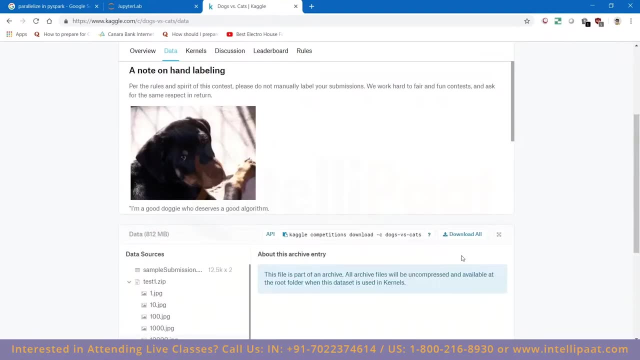 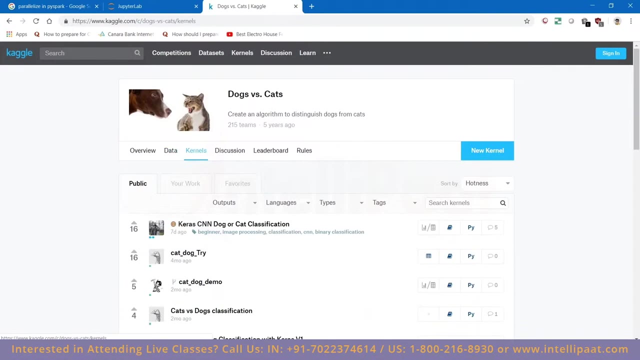 display because this is an archive file currently, otherwise you might sorry. you might also see the photo here, right, so you can download it. is it by clicking on this button called download? all right, then? second thing, is this current third thing? is this kernel thing? very important thing? so what this kernel is. 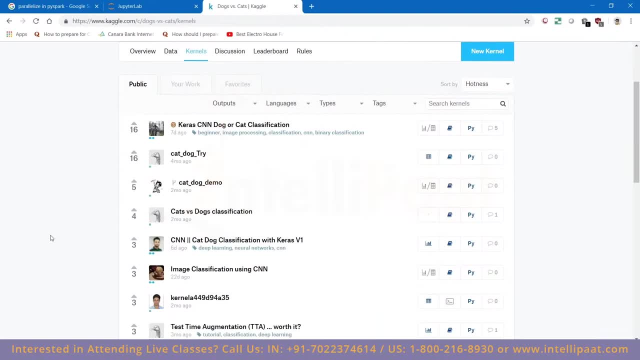 actually is that all the people who have worked on this cat and dog problem and they want to share their code. they share their code here only so you can read. okay, it says: CNN cat dog classification: Kiras one, Kiras cat and dog classification. so people, you know they do different, different things. 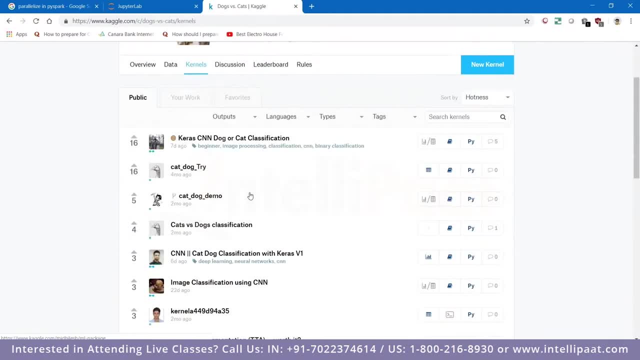 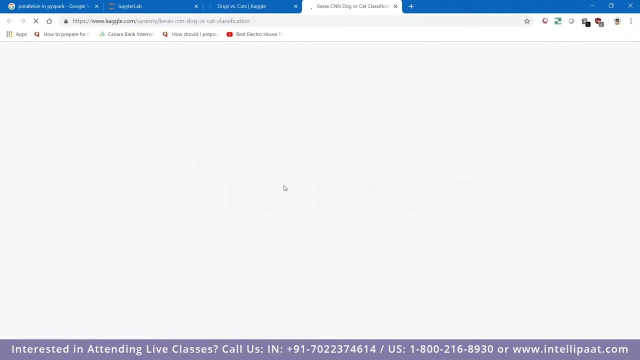 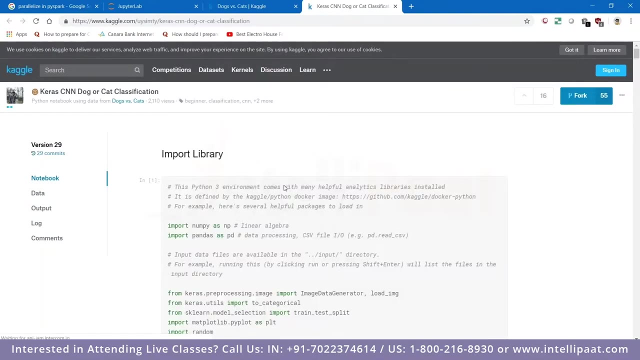 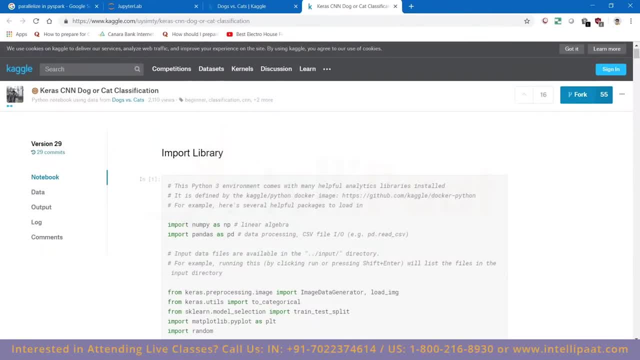 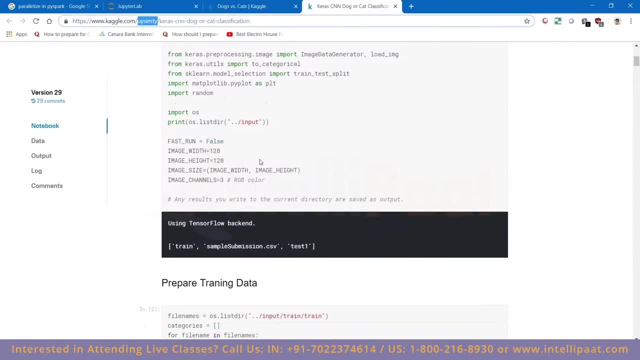 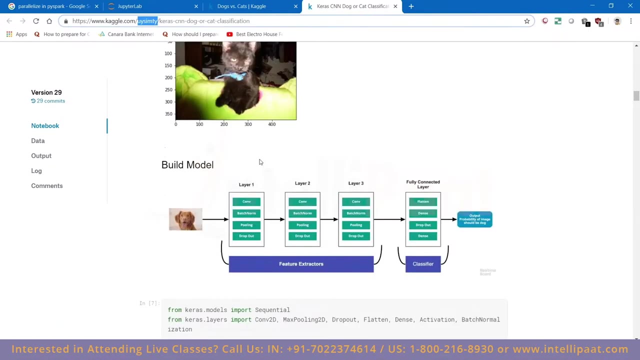 okay, see, this is a notebook, right? this notebook has opened in front of you and this guy's- his name is US MIT. you can see his code, whatever he has run and what things he is trying to say. right, so see, you can put anything you can put. 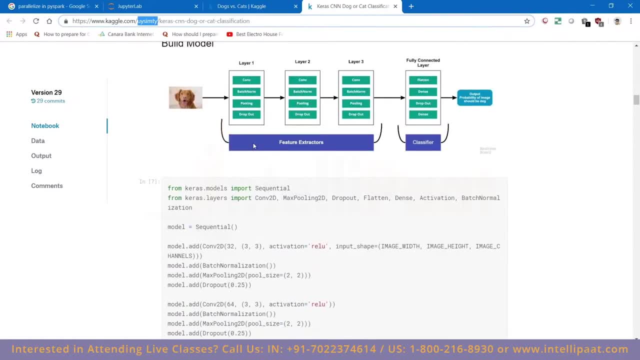 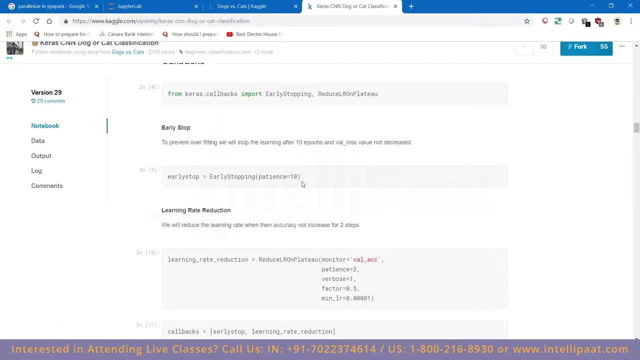 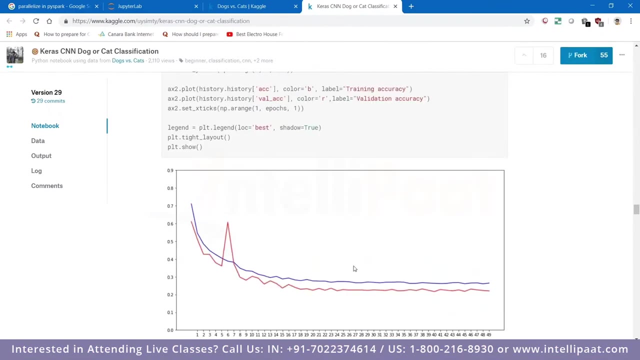 images. Lord's code is one thing that you're putting and he's putting: call back early, stopping, reduce our own black. you, it's all the code you can see right here, right, he's also producing some good graph, right, so you can read all these things here. you can do whatever you want. 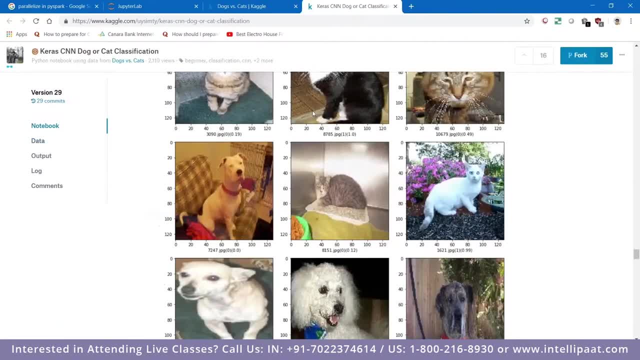 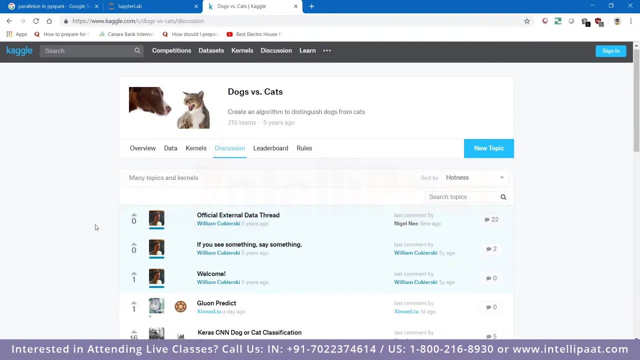 okay, this is a very good feature of Kaggle, I think. I think this is the best way. how do you contribute it? discussions, if you have any problem or people are telling new approaches. people did like they don't want to share their code but they have something that they cannot write in code but they can tell you, or 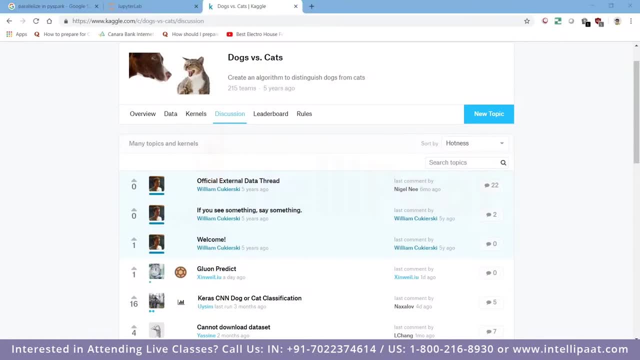 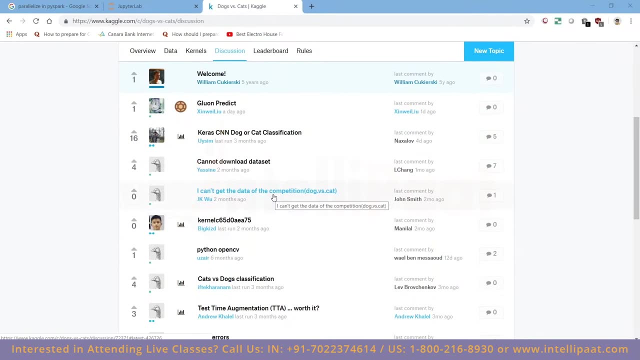 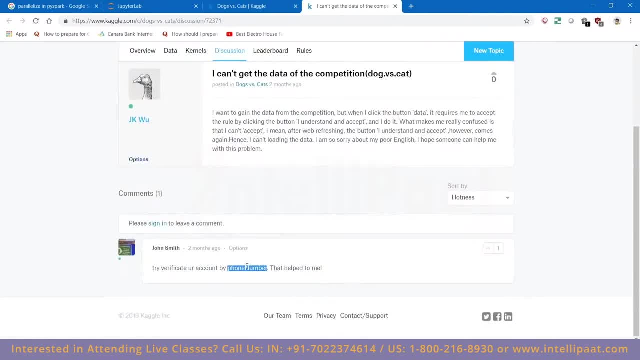 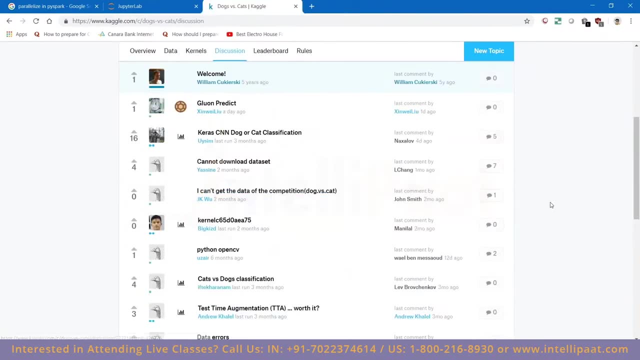 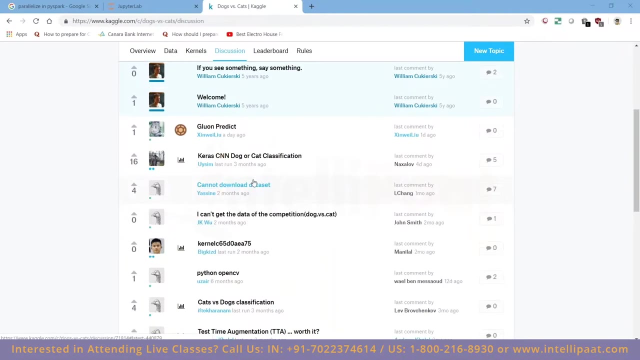 data okay. so one thing that they have written is that whenever you are making your account and Kaggle, just make sure you are verifying your account by phone number also. sometimes it's idea also sometimes it's just general idea that people post on Kaggle only, but it's very easy, it's inspiration code, so it see this. 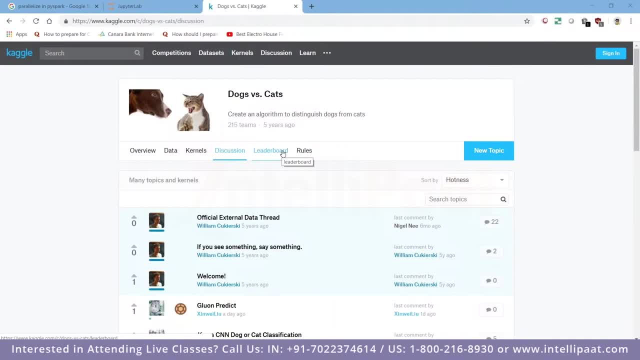 is one of the biggest problem that you know new people do on kernel. what they want to do is because they want to increase their rank. what they will do is they'll take the number one score, they'll copy paste it and they'll run. they'll get ranked 2 on the public leader board, but whenever the private 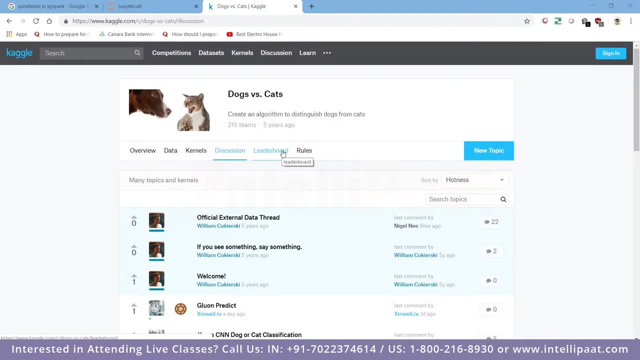 leader board comes, they fail right and this is the biggest problem. people are doing this. so this code is for the inspiration. just read the code, just get inspiration out of it and then write your own code right at the end of the day. always you have to write your. 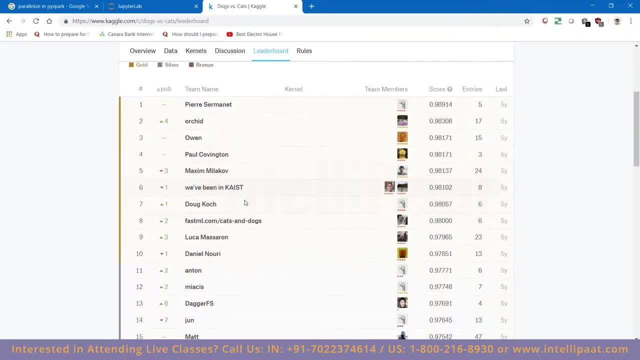 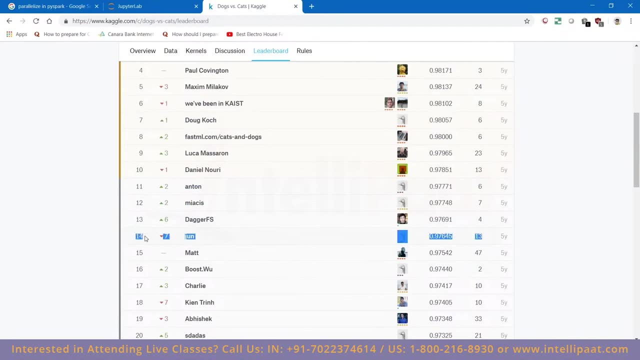 own code, right. so this is like your see now, this guy on number 14, right. so this guy, he somehow he got a rank 14 on the public board, right, if you see, this is the public board, right. and then on the private board he got minus 7. so so these guys, they fail drastically. so never copy paste someone's. 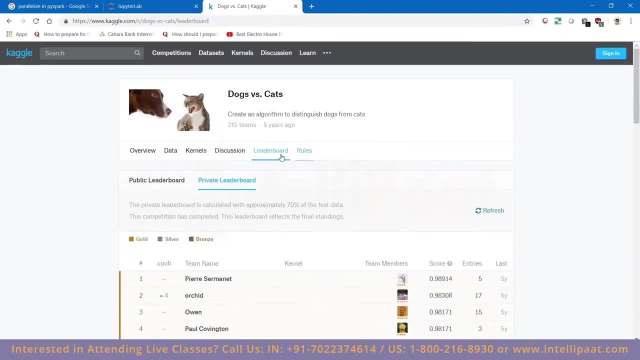 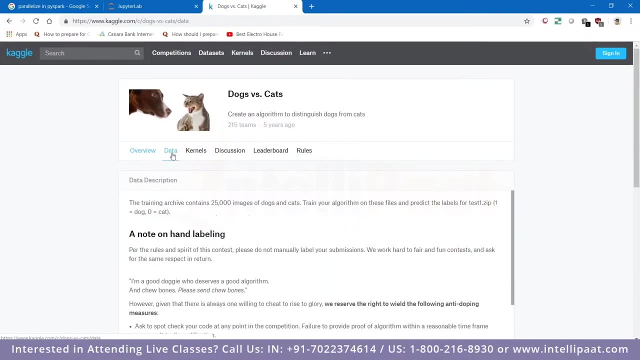 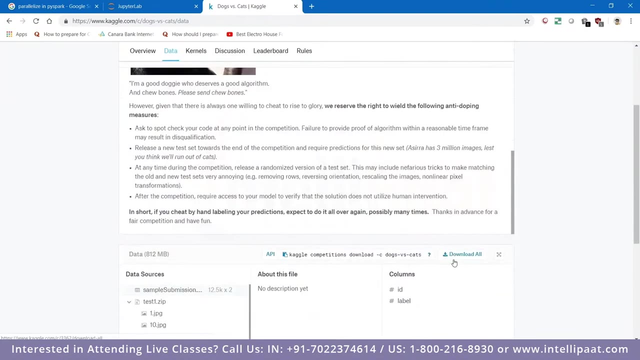 code right and get inspiration, and that's it. make your account on kaggle, verify your account with phone number and then download the data from here. data, click on this and then download all to people who are working on collab also: collab, now you can do. you can install kaggle through paper also. it's. 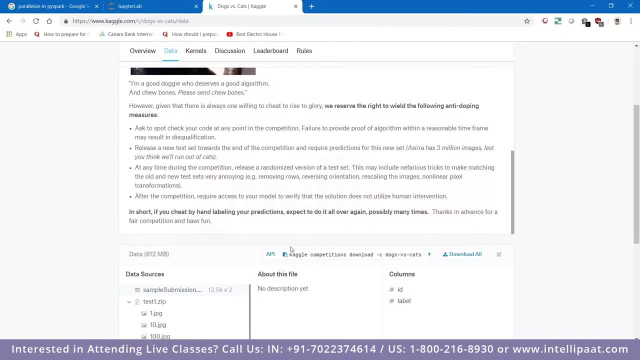 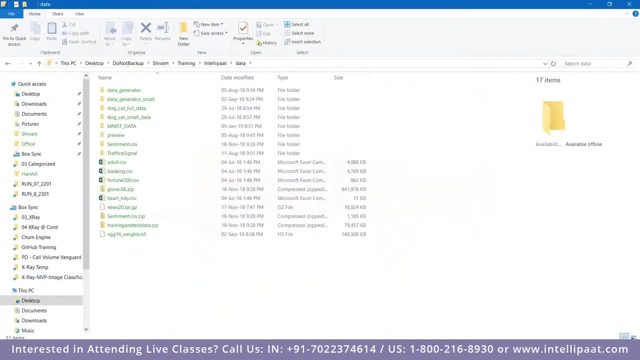 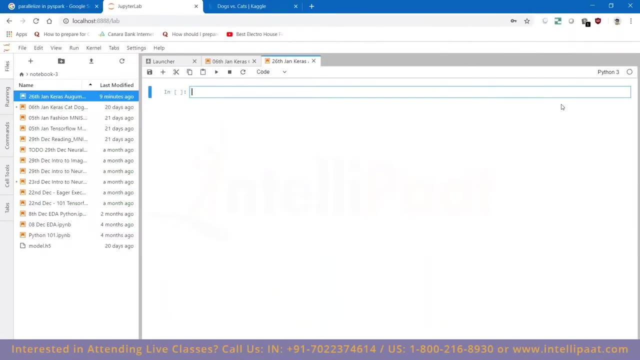 just one step, like pip, install kaggle, and then you can run this command on your collab and it will download the data for you. right now let's move back to our thing that was of cat docs augmentation. but how do we start doing augmentation on our data set? let's imagine that we have very less state of it, like 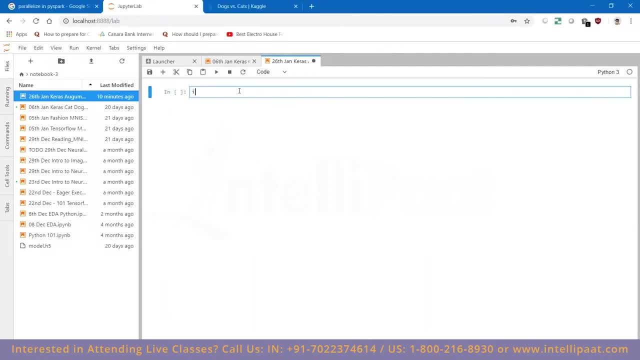 very less. let's do quickly our basic import: import keras, import number, import os. be my plot as dlt. okay, so just to check what is my version. my version is okay. let me take you to data path. i am. i will be using the relative path. see how i. 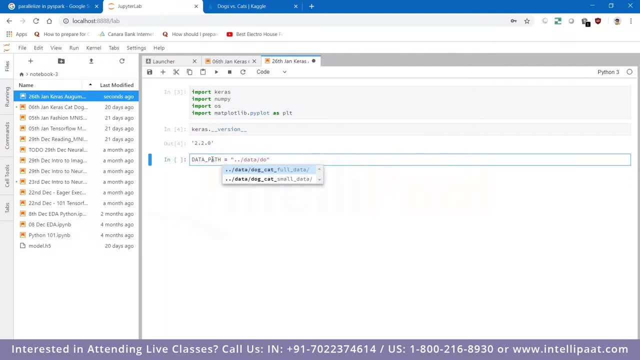 move back and then i say data and then cat doc- small data set. this will be my data set. okay, let's take a test image. test image is equal to um. okay, we forgot to import open cv- cv2- cv2.im read data path plus. let me take one file example. so i'm just doing nothing, i'm just copy pasting the. 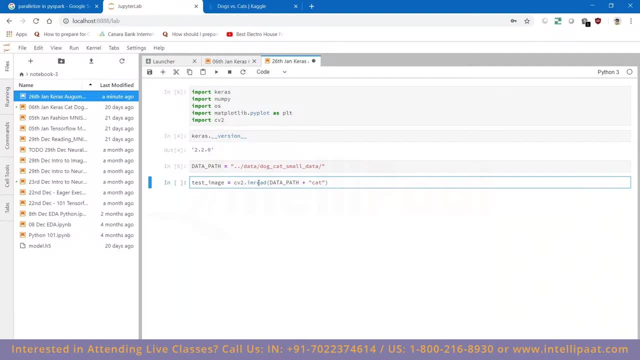 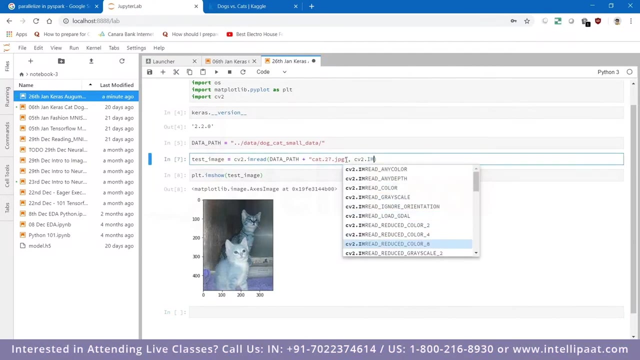 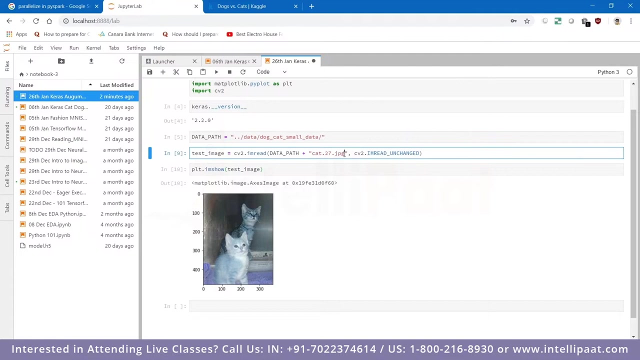 cat's name file name so that you can see it right � الم зап conductter google.com it will show you the image so what i did here is i just said i am read unchanged it means i am saying i am to i am saying to it will that please don't change any kind of color formatting just 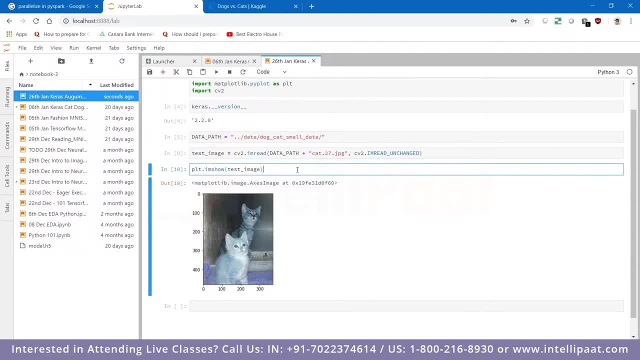 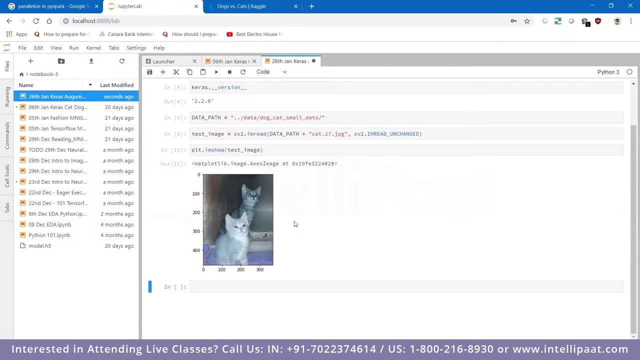 print whatever. it is right, okay. so it printed me this image. now the challenge here with us is that we have been doing the, gave it the, so now the challenge here with us is that we have. the challenge here with us is that we have a very less amount of data. we don't have a large amount of data, we are just very. 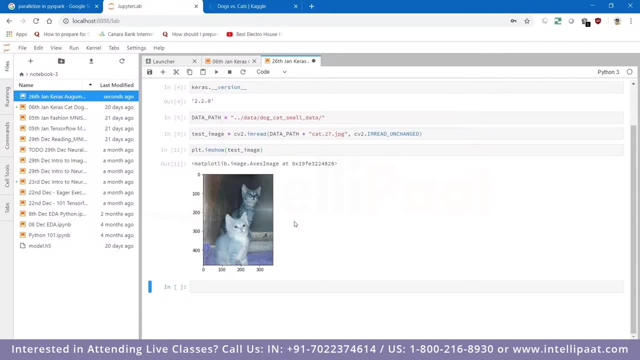 less amount of data, and this is just 200. now, how do we increase the data set? now, one of the options that you okay. before even I tell you something, let's say that I give you an example that, okay, this is cat dogs. you have to build a model and 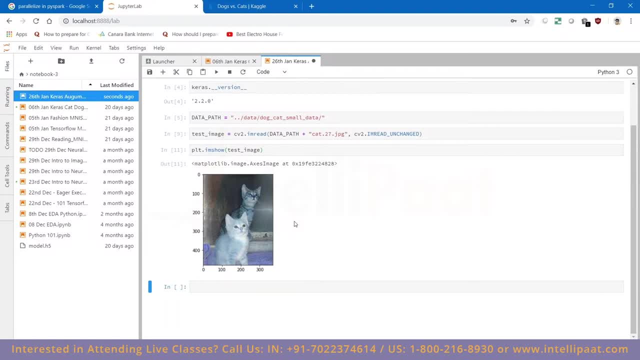 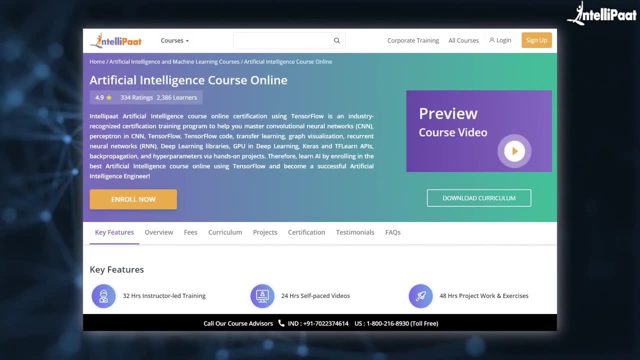 you have just hundred images. what kind of approach you will use to increase your data? just a quick info, guys. Intellipaat provides artificial intelligence online training mentored by industry experts. the course link of it is given in the description below. now let's continue with the session you have. 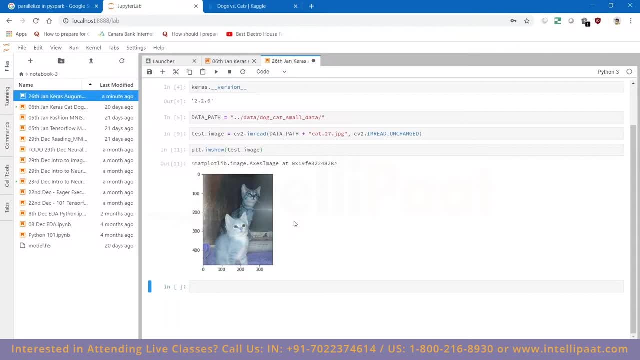 to just increase the data. nothing, do nothing, just increase the data. now let's say there is a very small kid, very small kid, right? he's like just a year old, right, and you are showing him a image of cat, the top view of the cat. now imagine: 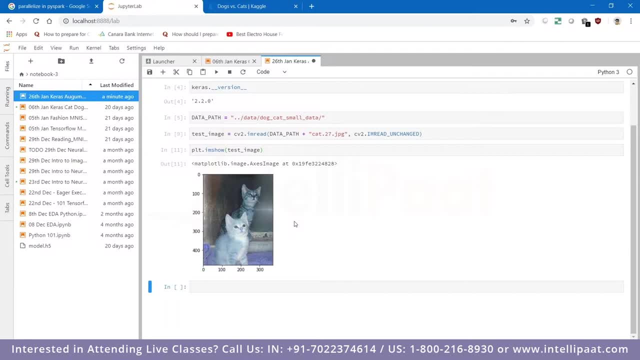 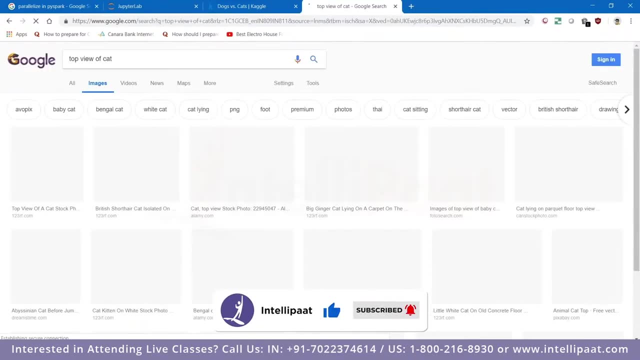 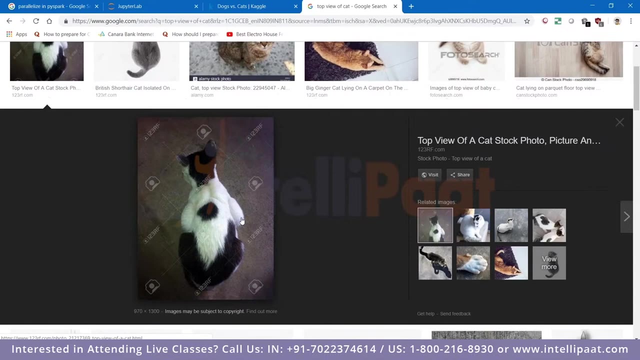 the top view of a cat how it will look like. let me check if I have a top view of a cat. okay, let's say that you show this image to that child and you show it multiple times, like ten times, and just say: this is cat, this is cat, this is that, but now the of the child he are. 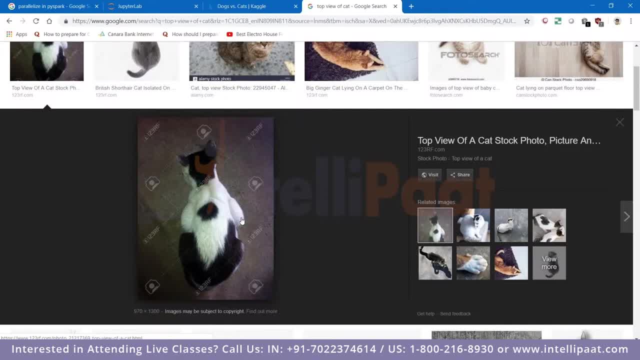 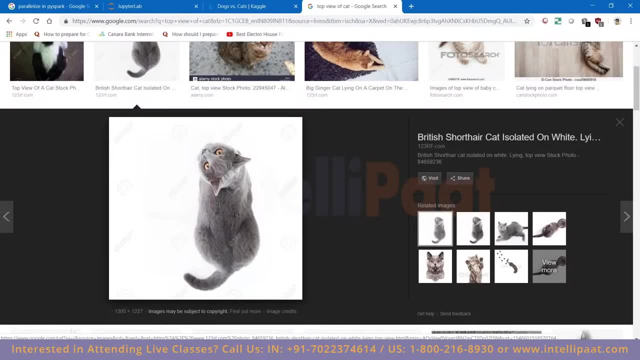 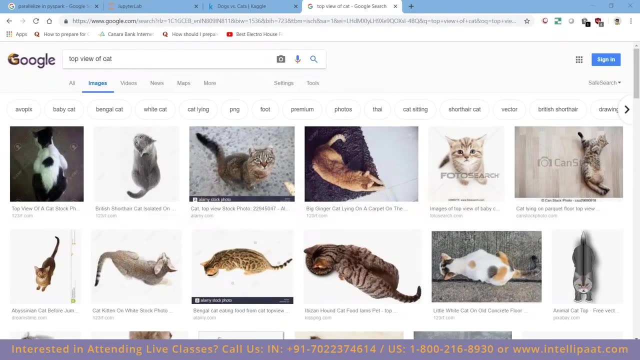 understood. okay, this is cat. next time, if you are going to show him this kind of image, he'll say: okay, this is cat. yeah, I know this is that cat. okay, I understand, this is a cat, but next time if you show him some- okay now, if you show him this kind of image- he. 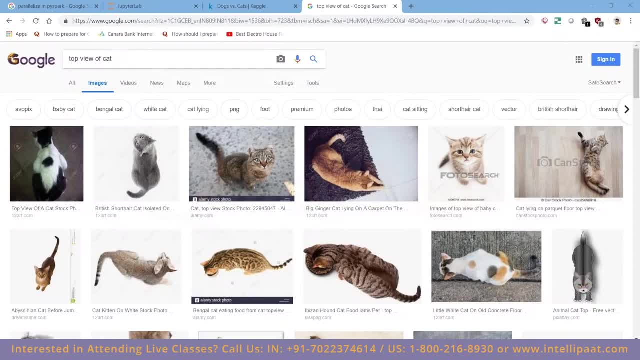 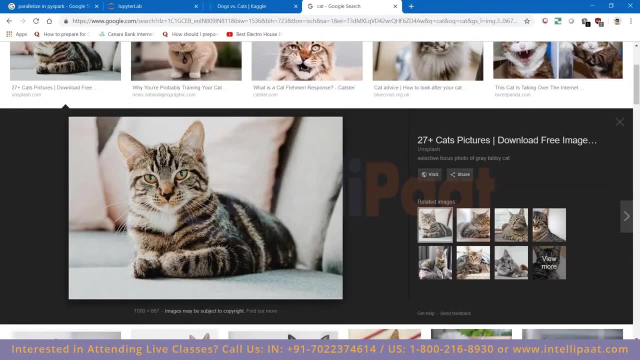 will get totally confused, right, because he hasn't learned this thing: that cats look like this. he only learned 10 times, and that to be the confidence. see, whenever you show someone one image and then say this is a cat, he gets okay, okay, this is a cat. but when you are showing it 10 times and then 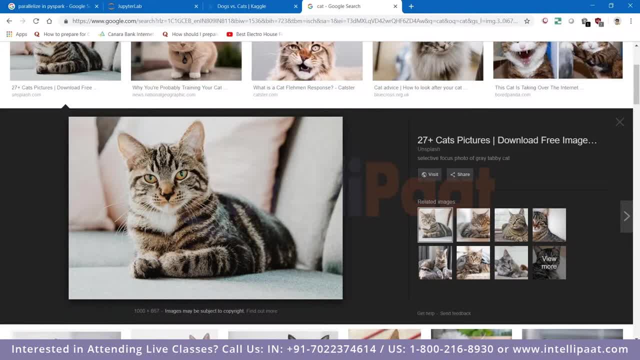 saying he's a, it is a cat. his mind learned this thing that, okay, this shape, top view, this thing is called cat, irrespective of learning about its feature. now it is mugging up the things. it is mugging up that, okay, this is a cat, this is a cat, this is a cat. next time, if you show him some, 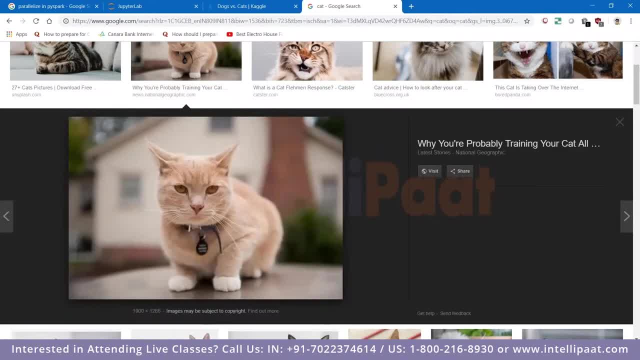 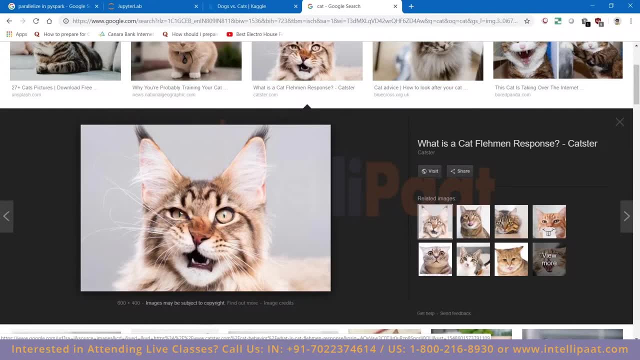 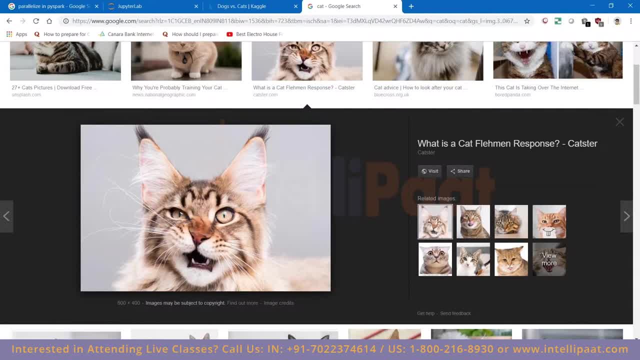 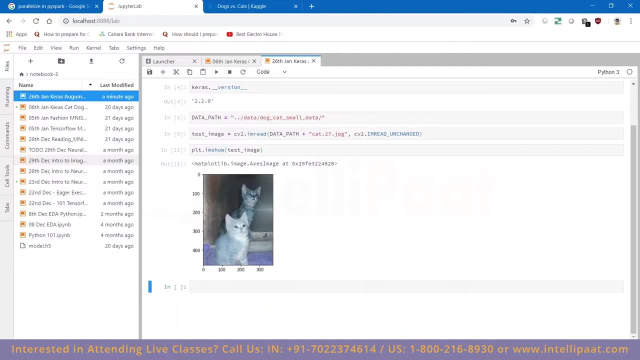 a cat. this is not a cat. this is not a cat. this is the problem. when you do a copy paste, right, whenever you are doing a copy paste of 10 times, the happen, what is the thing that is happening to you is that you are showing the exact image 10 times. problem. that's why there comes a new 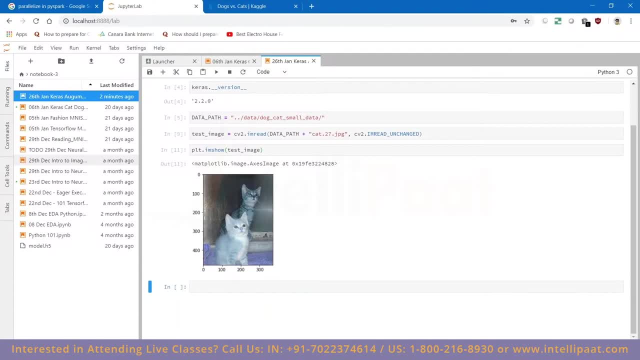 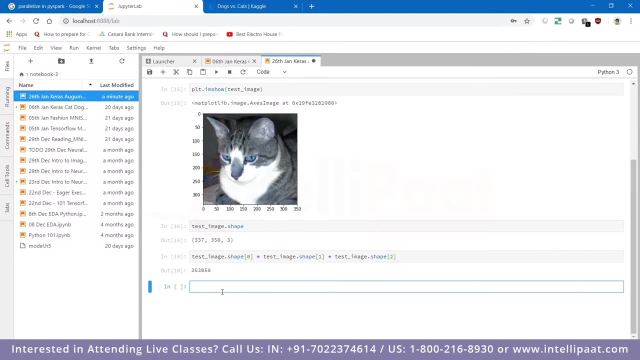 and a handy thing that helps you, that is called data augmentation. then the second thing, that break the images if it has multiple cats. okay, i understand, break the image if it has multiple cats, we can do, but if it is a single image, then then we can do nothing, right? no, still, we can still. 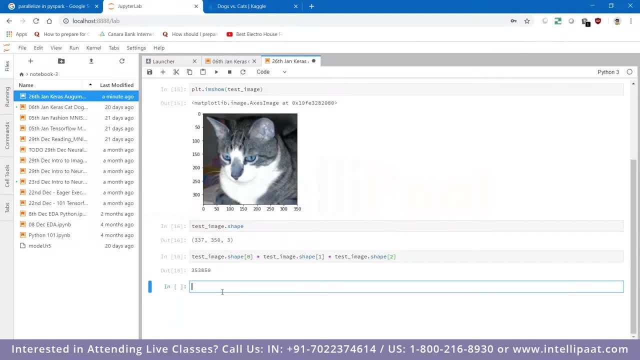 we can. this is called data augmentation. see, now, you cannot produce new kind of data, right? so this is a simple example of cat. so what you can do is you can just go to google and download multiple images of cats, right? but let's say, this is some kind of a business problem and you are dealing. 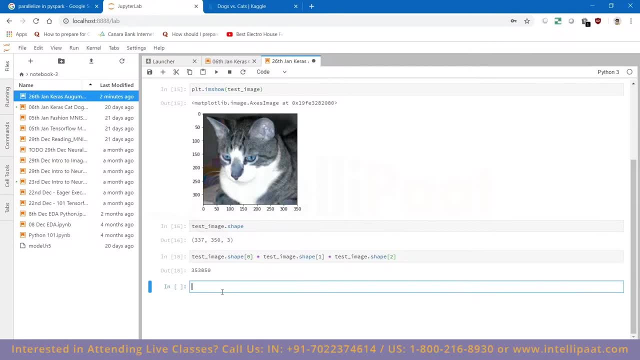 with something that is not available on internet? how will you increase the data set? this thing is called data augmentation, now data argumentation. it involves two kinds of knowledge. one is the domain knowledge that you need to understand that what kind of image you are using and what kind of a problem you are. 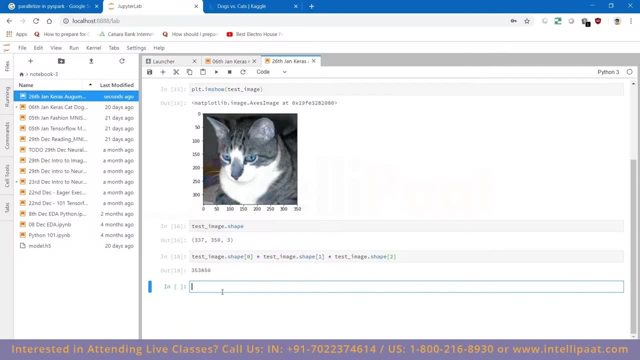 dealing with? right, so we are dealing with cats. okay, so first of all, how to do data argumentation, then i'll let me show you this thing. okay, so for data argumentation, you will use keras. keras has already given you this thing from keras dot pre-processing dot images. import image data. 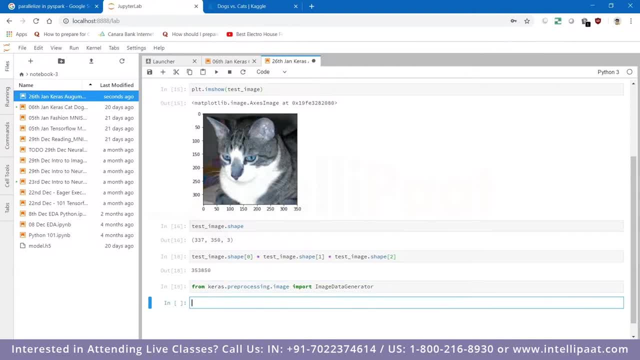 generator. now, this image data generator will generate images for you, for the image that you have given right now. when i say, let's say we make a data generator, see one thing that i might have already told you. if not, then i'm sorry that everything that starts with a capital thing. 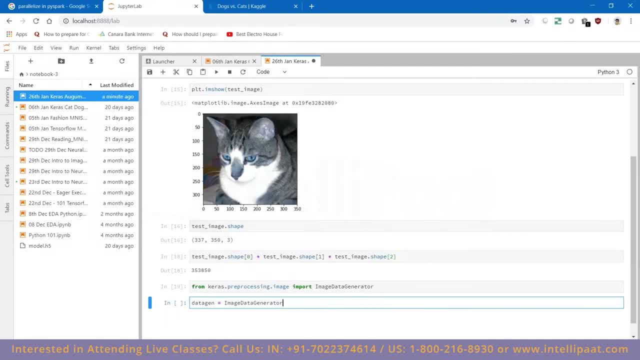 in python, and especially if you are working with a standard library like keras or tensorflow. that is the class right. it's not a normal uh function or a normal method. it's a class. so you have to first initiate a class right and then you can work on it. so, image data generator. 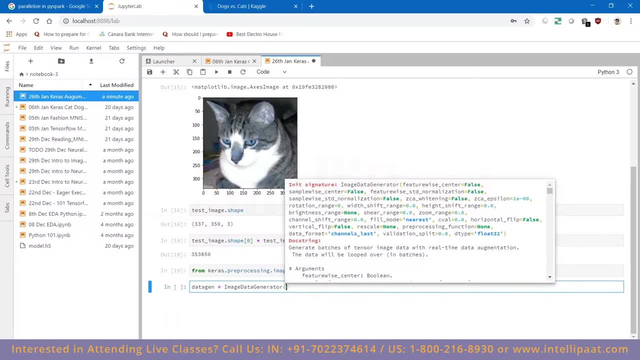 if you see its help here, if it is visible to you, this block, how did i bring this? uh tool tip shift tab is the thing that helps you to bring this out right. you so, whenever you are working in jupyter notebook, just make the function, just go to it and then. 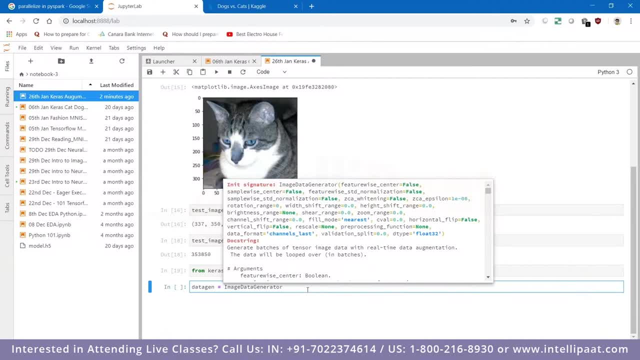 just say shift tab and you will get this. okay so, image data generator. it says. its doc string says that it generates batches of tensor images with data, with real-time argumentation, and the data will be looped over in batches. okay, so we get the small idea that some kind of a data argumentation 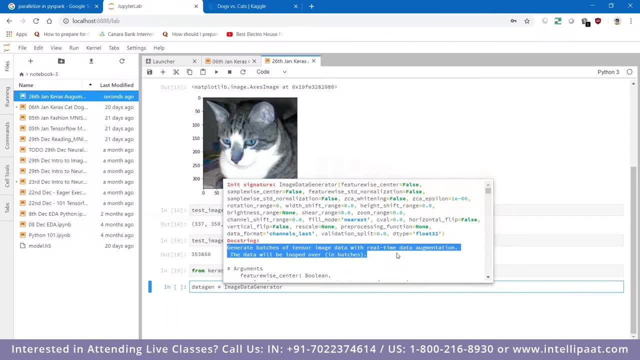 is going to happen, but it has two things. it is going to happen in real time. second, it is going to be a batch, so it's not like you have given it a folder and it will take all the images. no, it will take only some amount of images, process them, give it to you. then the second batch: process it, give it. 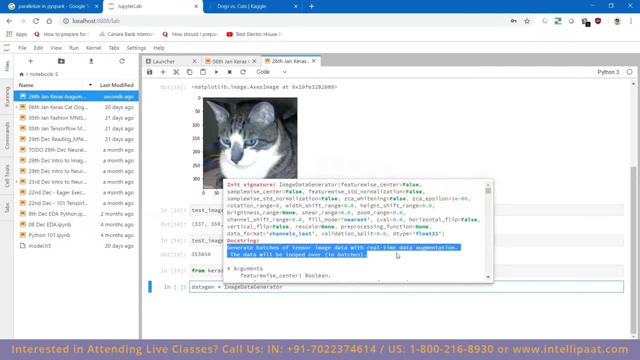 to you third batch process. it give it to you. this batch will happen until your images are exhausted. right now, when we come to the options that are available in image data generator, these are like multiple options: feature-wise centering, sample-wise centering, feature standard, normal. so so, first of, 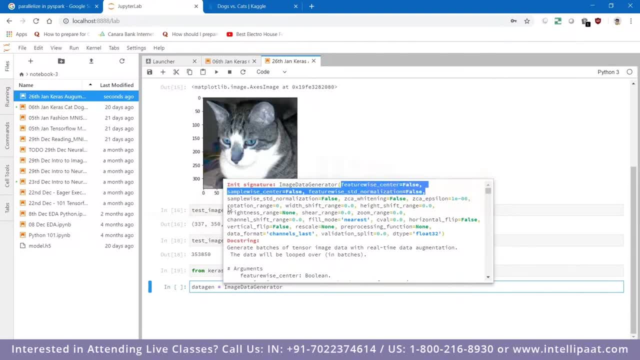 all. let me show you one successful tutorial: life management using fish c-Menu in future. so I have chosen this function already. so before I am going to use this function, I want to point out that this function is called return relief tool. now, personally, I have used it in one of 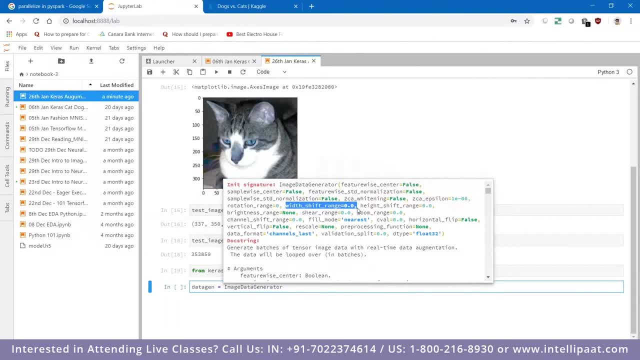 my courses and other internet courses, but recently I have been flying my browser wounded, so I am reusing it and I am using it in� September 2019, where I have uploaded this wrong successful. I am Even masterillism or bio data generation. everything is available in từ still listening. you can use it like this. now see one of the. if your business case allows you to rotate your image to certain angle, then you can use this. buy width shift range. it means, if your business use case allows you to shift your images to a left and right on the width spaces, you can do similarly for the height. up and down, you can do. brightness you can change. 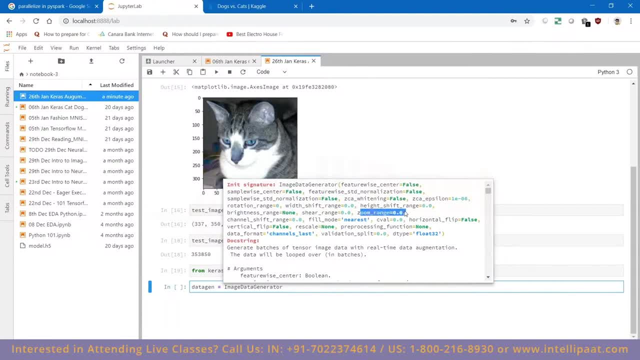 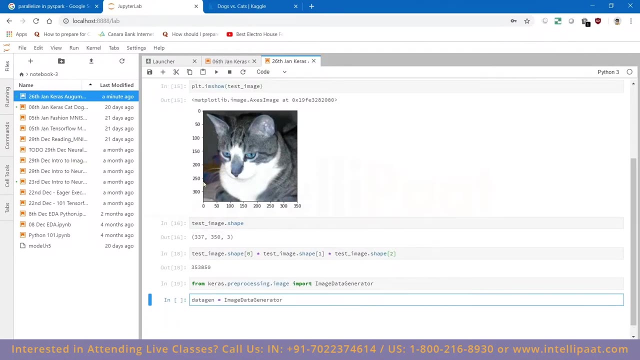 change the image, zoom you can. you can zoom into a little bit into the image. now, when I am saying your business use case is allowing you, what does this thing mean? business use case is allowing me? it means that let's say, okay, let me ask you this question: can I flip this image on a on a horizontal basis? it means to 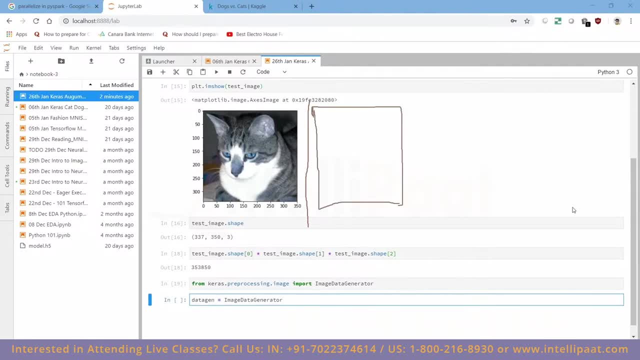 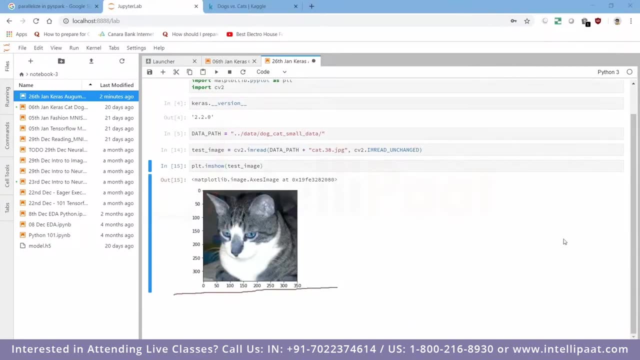 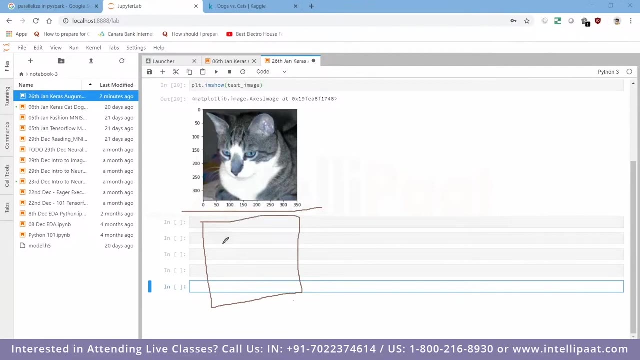 keep a mirror here, can I just okay now. but if I say, and let me say that if I put a mirror down here now, I will have a now let's say there that put a mirror somewhere here and I will have a image over somewhere here now the cat will be. 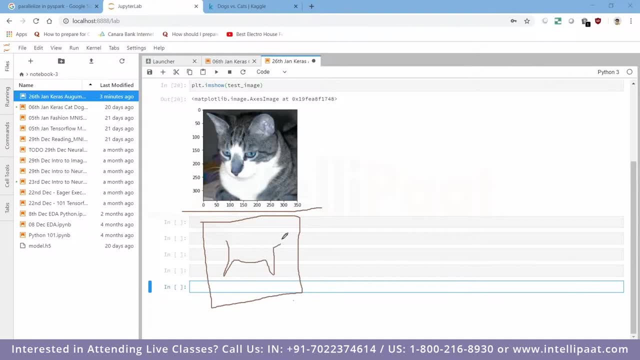 somewhere like this, with ears here and looking here right now. does this make sense to have this image inside your data set? you want to all the bad images away from the model right. only good images, real world images, right? you don't want to set wrong expectations out of your model right. rather than giving him- i think, giving- small data, 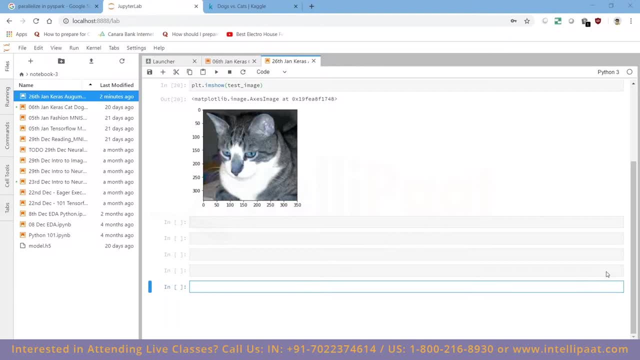 is good, rather than giving him false data and doing a overfitting over the model. right, because see if you're testing, your training accuracy is 87 and your testing is also 87. it keeps a low expectation inside in front of a client also right, so the client also knows okay training. 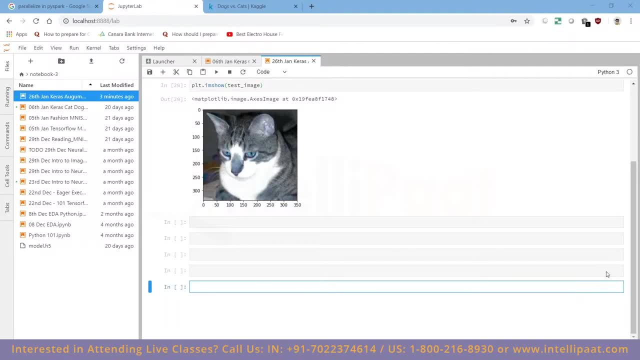 me 87, then i can expect testing also 87 or 85, right. but when you overfit your model and then you say that, okay, my model is like 97 and then you deliver somewhat like 68 it, that time you know that's a real pain in front of a client, right? so always try to so. what they say in industry is: 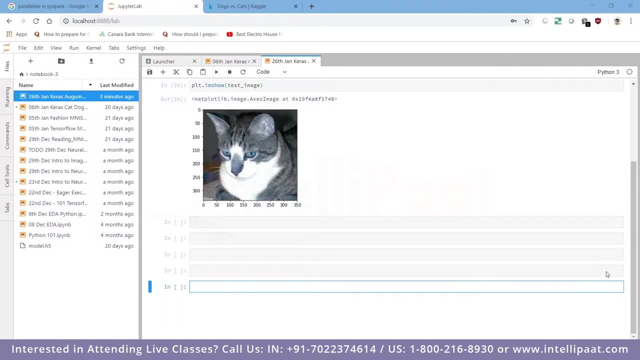 that. uh, what do they say? that under expectation and over delivery? right, so you put your model somewhat like sir, we got a training accuracy of of just 85, but now, testing me, when he gets he's at like 92. that's when he gets happy, right, if you deliver. 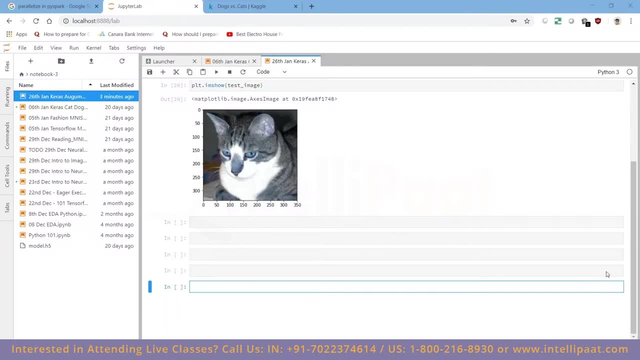 both as 92. when he's getting 92 he never gets. the client never gets happy, right. so it's all about how do you uh frame your business problem? and then you want to model your, you want to train your model, right. so this is how you do uh augmentation in kiras. let's do it. so see, kiras is one of the 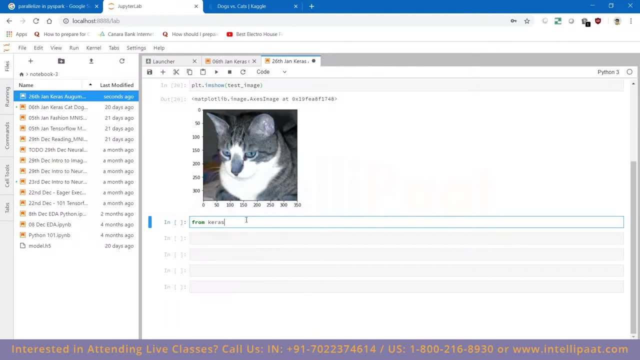 good libraries, everything is totally sorted. so when i want to do some this image augmentation, i do original augmentation, i do my picking too. it's out of the window and i have a working happens then practicing all these processes distinctly in kiras, and so there are all kinds. 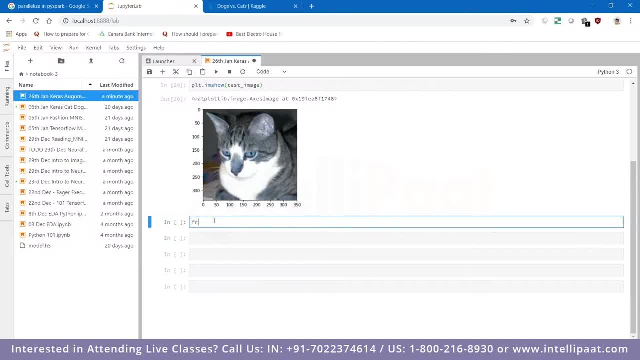 of pre-processing as well. so during trouble processing, i will just say: assign text that they would be like against one of the initial links that i would have otherwise. so, in fact, where i'm going to show you like this means like there are multiple, there are multiple. 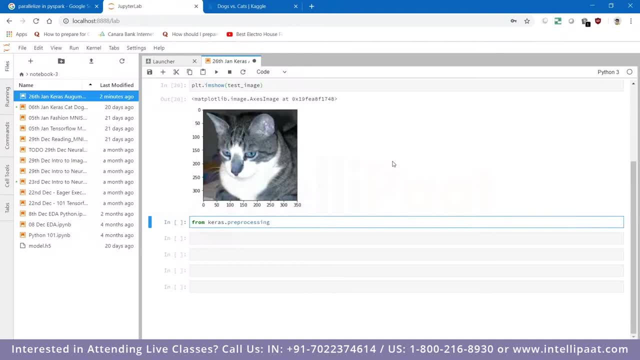 pre-processing. i'll just say i don't have to remember all these things right from kirak. pre-processing, now preprocessing, has multiple things, different kinds of pre-processing that are available to us. and then, once you have written import, then can i do something to get all the things. options, again a tab, so you get the second. 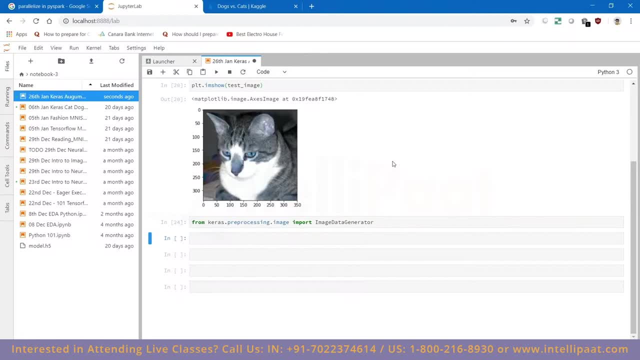 thing: image data generator. right, so you have a image data generator. we need two, three more things. one is called array to image, then image to array and load image. load image is actually a feature from kiras that helps you, uh, to load the image from a directory. okay, i'll say open cv, pil, cv2 is. 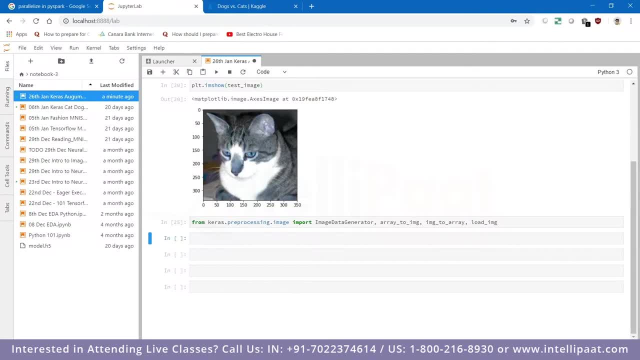 open image, right. cv2 is open, cv, right. so open cv sk image and then, uh, pil or pillow, whatever you say, and then kiras. kiras at the back end is using pillow and pil for using. so whenever you're using load image, it is actually using the pil module to load all the images. 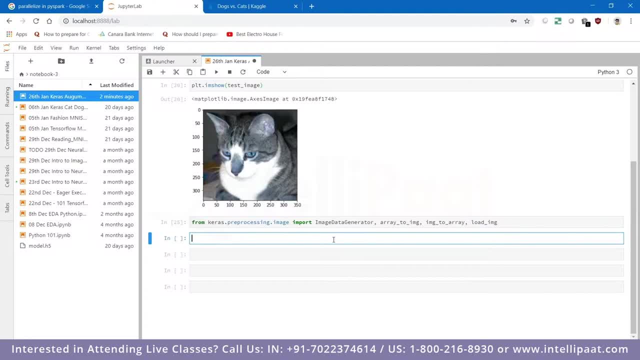 right, let me do one thing: how do you start? you have to define your data generator. you say image data generator, and then you have to say what kind of a different, different augmentation you need to choose. right, i am going to choose a rotation range. i am going to rotate my range till 40 degree. i am. 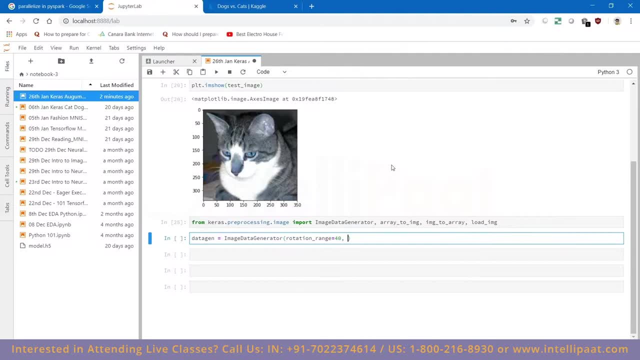 allowing it to change it. second, let me say i want to do a width shift. width shift, let me do plus 0.1 right. similarly for height width also. i want to do a width shift. let me do plus 0.1 right. similarly for height width also. i want to do. 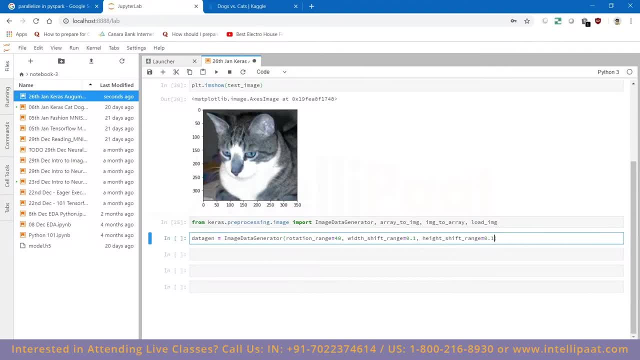 i want to change 0.1. um, i can do one more. i can do like horizontal flip that we were discussing. is equal to true, okay, it's horizontal flip. or i can do some sheer zoom. so these are the things that i've done in data generator. you can just type in data gen to get to know all the things that you have done. 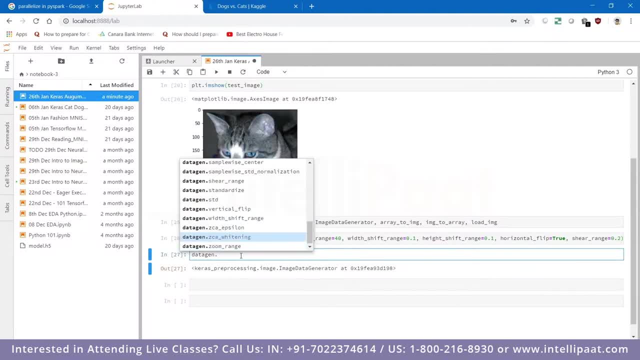 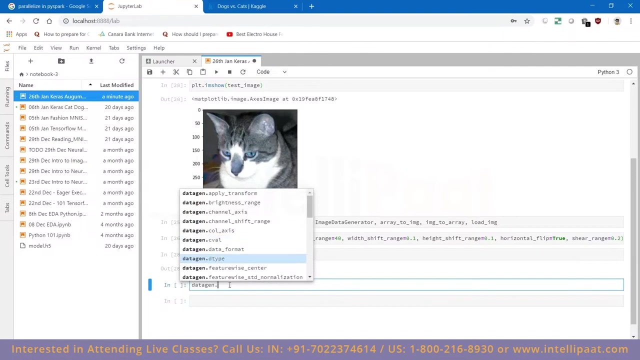 by非 um. then we did shearifmitch. if you want to know what it is, you can get through this now. so let us become it's in the constructor of the func, on the class it has written and becomes a feature, so you can later also know that what kind of a properties that you have used and if i to do this, you can get. 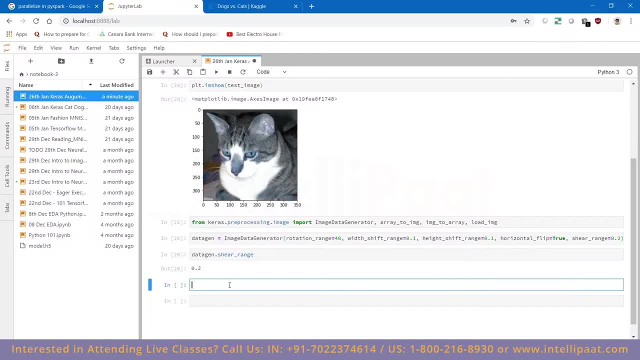 what we have done till now is that we have, uh, created a data generator. we just we have just told the model that we- these are the things that we want to do. let's do this. let's create a test image. let's create a image. image is equal to, we'll say: load image. load image from where? from data path. 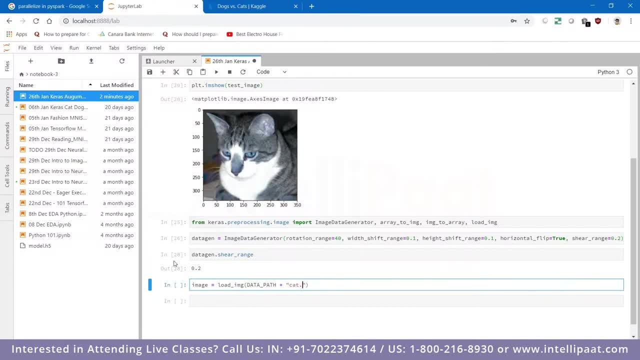 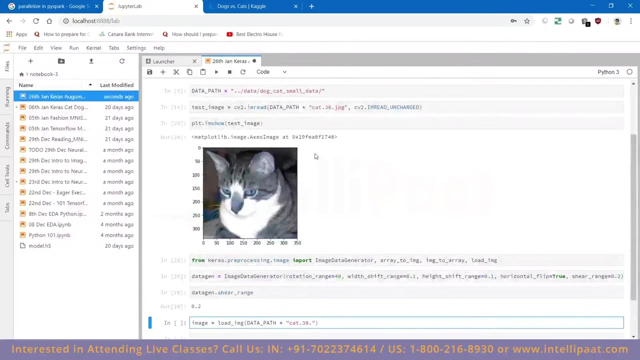 plus, let's say: we do it for cat dot. okay, let me search for a good cat. okay, i don't. okay, let's do this one only so that you get more view on this. this is 38 cat 38 dot jpg. so see what it has written. let's check that image. 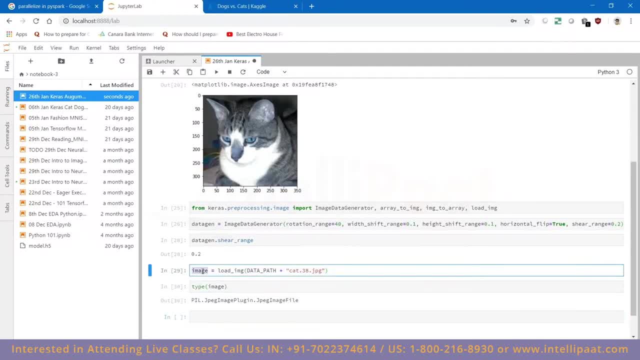 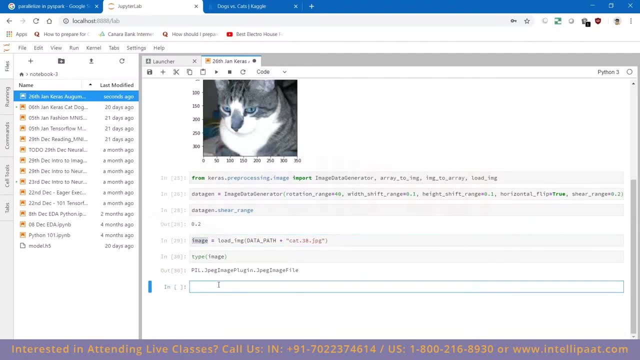 load image will not return you the. you know you will not return you the np dot uh, array matrix or matrix. it will return your pil. so what you have to do is you have to say that image, img, img to array right, and then you have to pass your image inside this. 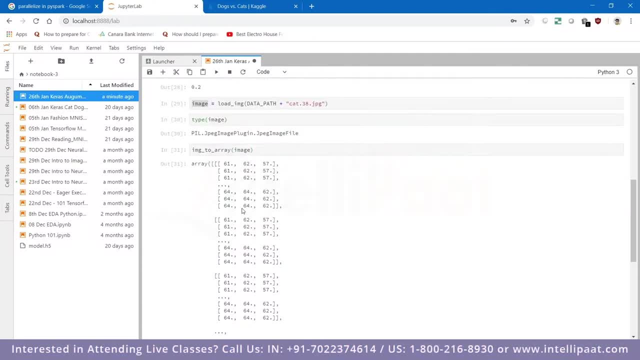 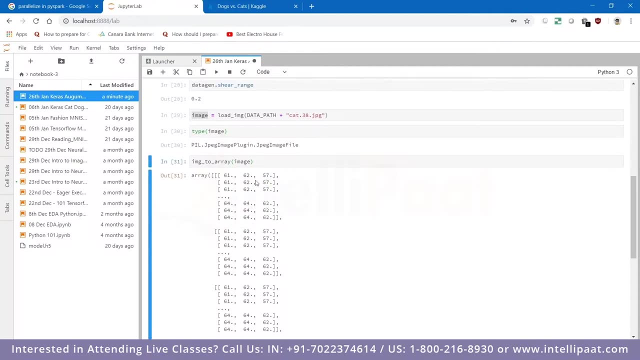 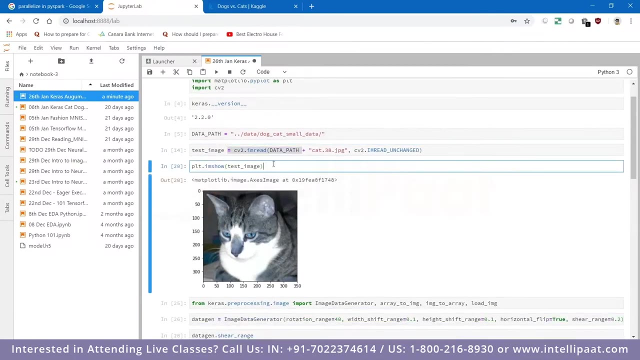 this will convert your pil image into into your matrix number right. and cv2 was directly giving you this matrix. remember when we loaded our image through cv2 dot im read it was directly giving us this uh matrix right. so there's a difference. always use which library to use for which instance. 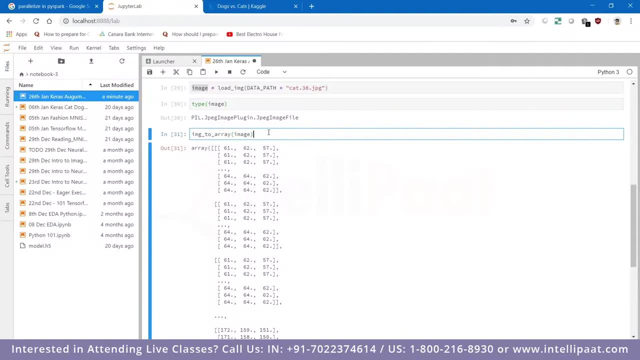 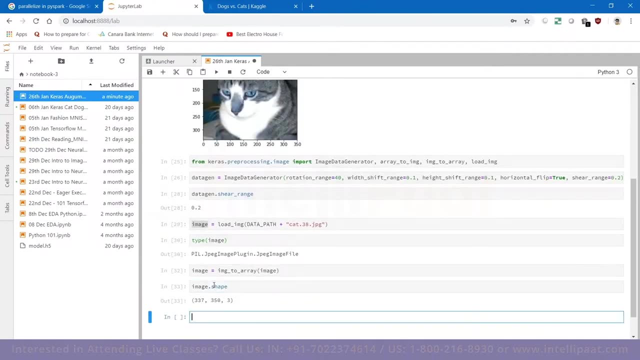 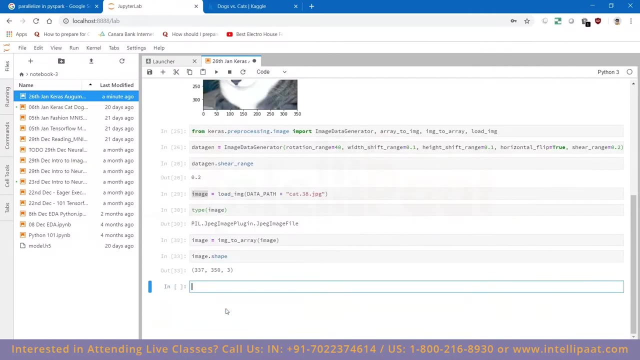 right now what we can do is, let's say, image is equal to image, dot to array. now i got this image. if we check the shape, shape is 337 dot 350, dot 3.. okay, it's all clear. right now i have the image. also, if i can do a plt dot, i am sure it will show me the image. 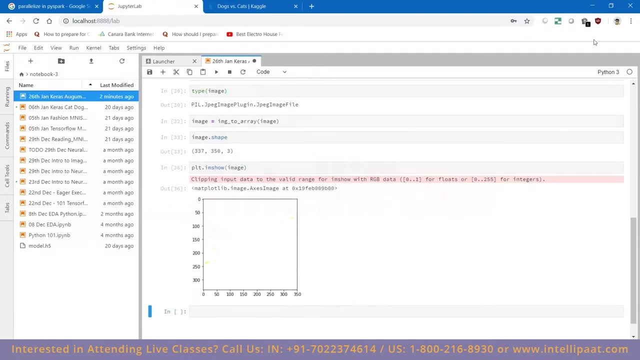 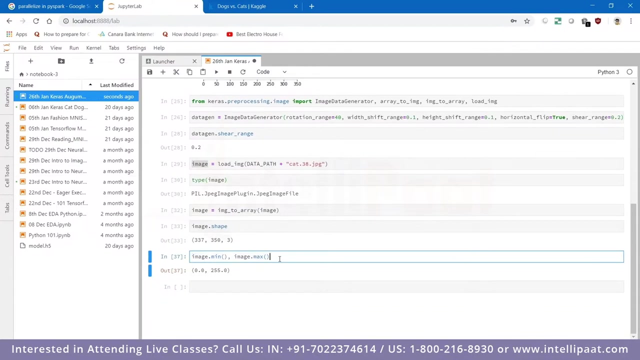 clipping input data to valid range with. i am show with rgb for float points integers: okay. so what has happened is pi has returned this thing with dot min. what they have done is they have returned something larger than expected. okay, so they are in axling floats. that's why plt is not showing you. plt believes in. 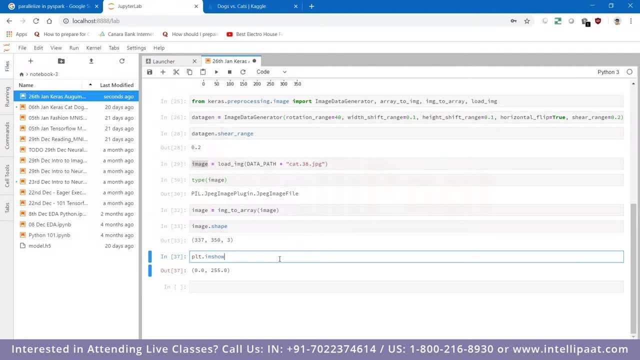 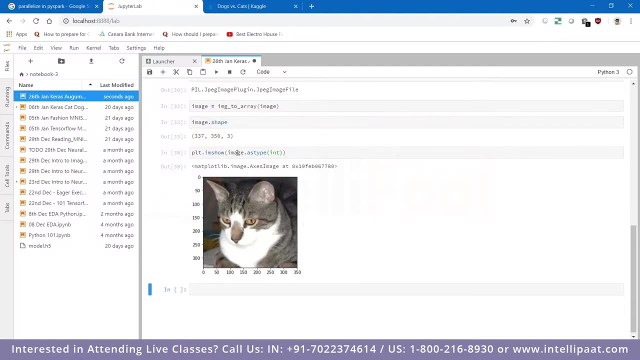 just it is there right. so what plt assumes to get? only integers. but we were returning a float. we were returning a float, but with integers only. we were just saying three co as three point, zero, zero. plt has some issues with the floats, so it only expects you to give uh, uh integers. 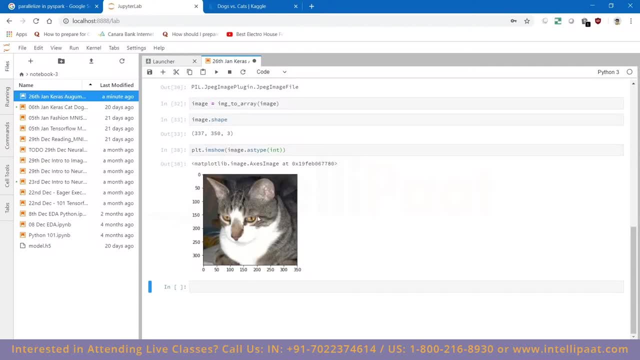 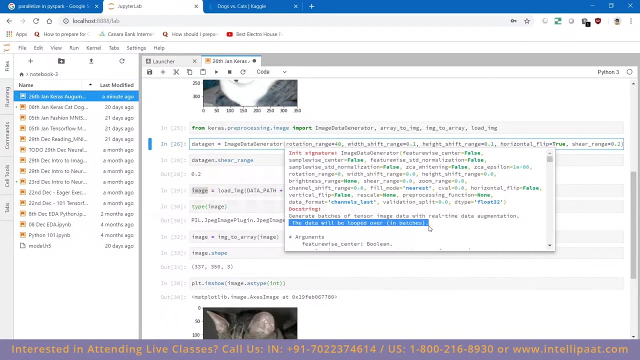 just converted into this. okay, so this was the blank image that we have. original image till we have. we have not done any kind of augmentation to it, right? but now do you remember that when we were doing this image generator, it said that the data will be looped over batches, so you have to make. 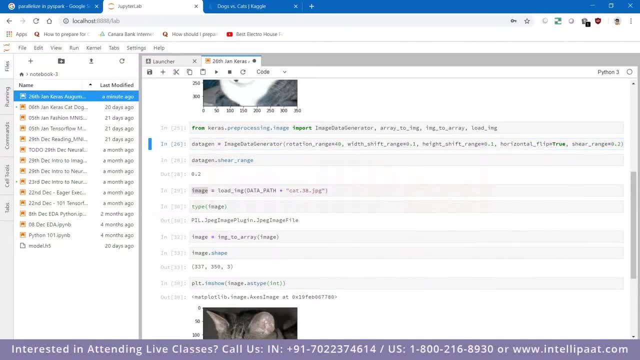 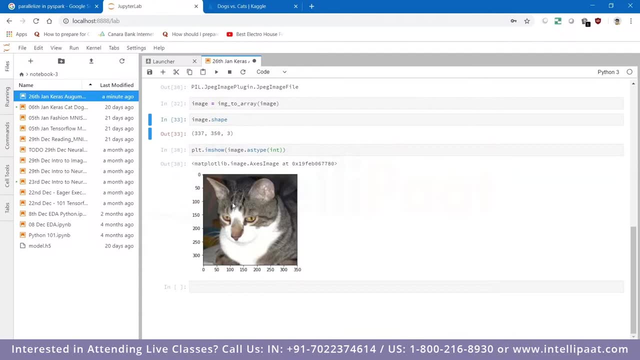 batches of the image. it will not just take single image, or even if you're giving a single image, just give it a batch, right? so what we have to do is i have to reshape this image with the batch also. so i will do not think i will just say image dot reshape dot. image dot reshape, one comma and image dot shape. okay, 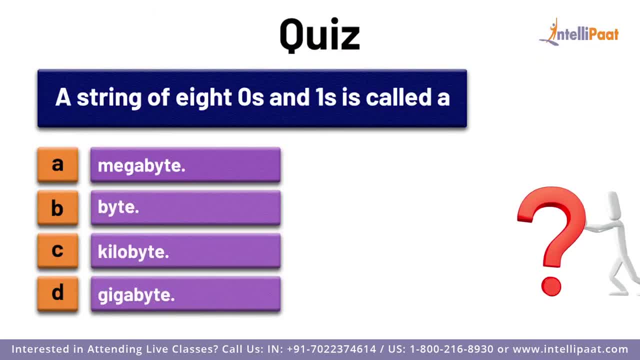 rather than doing this, i will just say: image dot shape. just a quick info, guys. test your knowledge of computer vision by answering this question. a string of eight zeros and ones is called what? a, megabyte, b, byte, c, kilobyte, d, gigabyte? comment your answer in the comment section below. subscribe to intellipaat to know. 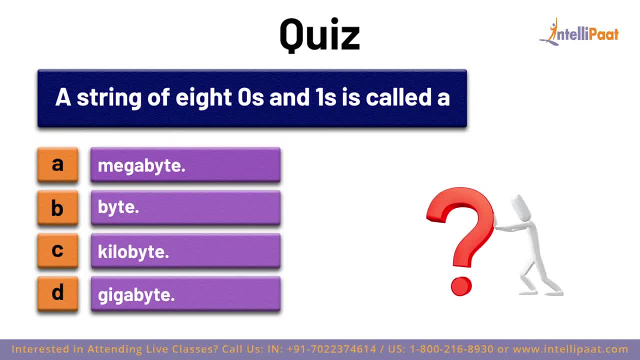 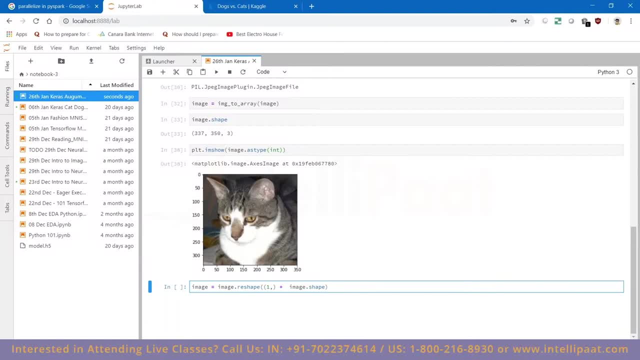 the right answer. now let's continue with the session. this will work for us, right? so what i'm doing is i'm just adding one more dimension to the image. so now, if you check the image shape, i have done nothing, but i've added one more. so it is saying that this batch contains only one image. 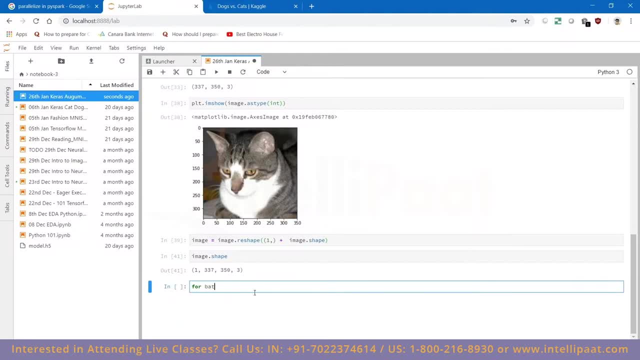 so i'm going to start this thing, we're going to say for batch in, i'm going to call this data gen function and i'm going to say: flow, simple, flow, flow. my image inside you. and this is actually not an image, but this is a batch of images. in our case it's only just one image, but it might contain 10. 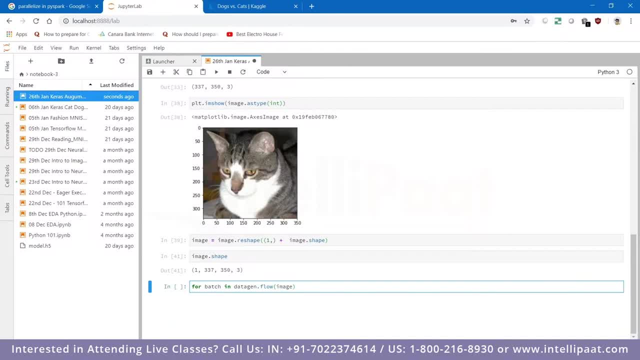 images, or 20 images, right. and then, whatever it asks you, it says: first you have to give your x, then we have the batch size. batch size is just one, we have only one image. and then it says: save to dir. uh, yes, we can say it to dir. let's say i'll give it to temp, right next. 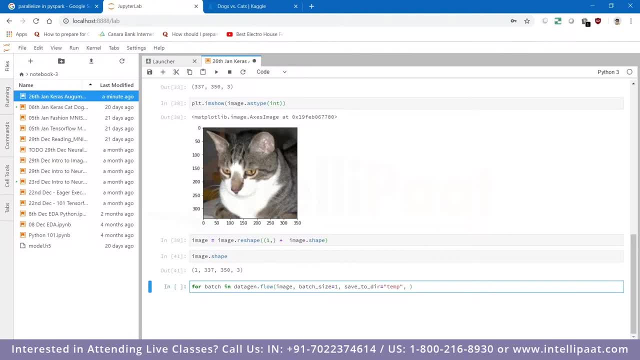 what is this asking? it's asking for seed. no, seed is for like npc, that you want to give right and next you can give it. you can give it some prefix. let's say cattle hyphen, comp, right hyphen, leave it. and what next do you have? you have save format. 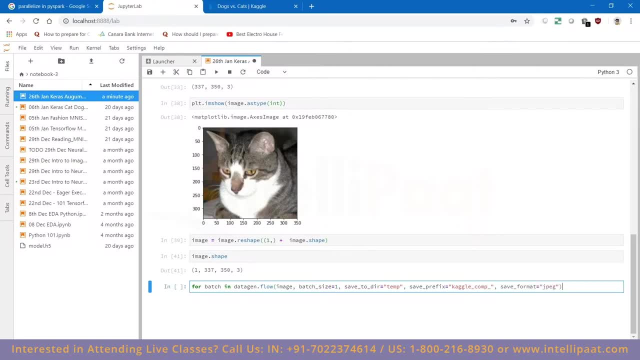 you can tell it. which format do you want to say, let's say jpg? right, these are the things that you want to start in a data generator or flow. now i want to stop this, also because this is not going to stop, uh, until and unless this thing happens. so what i'll do is i'll say index and then i'll say: 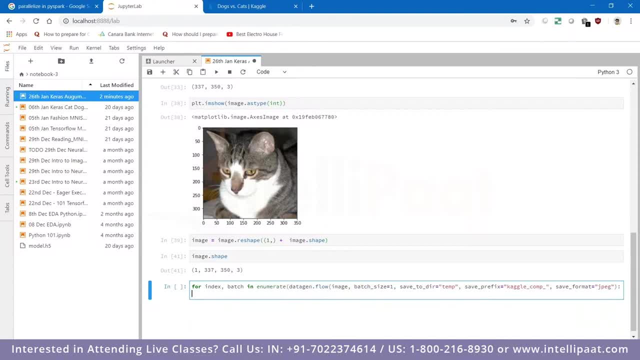 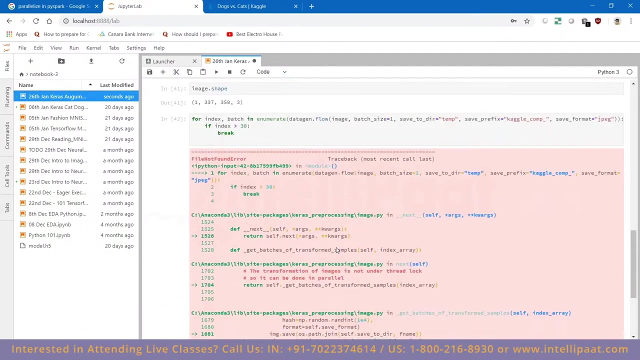 enumerate, so enumerate what it does. it will also tell you that how many times your this for loop has run. so i'll just put a thing that if index is like, uh, it's greater than 30, then do a break, okay. it says file not found. which file not found? okay, so temp folder is not there, actually, okay. 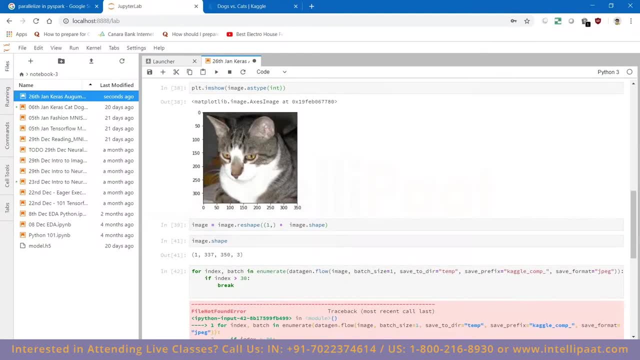 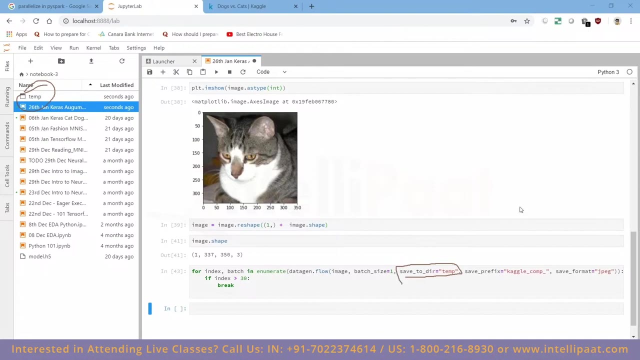 i have to create a folder. let me just jump there. i need a folder called temp. you can see, i made a folder here. you see on the screen, on the left hand section. i made this folder called temp and i have given it here save to directory called temp. and now, if i open this directory, 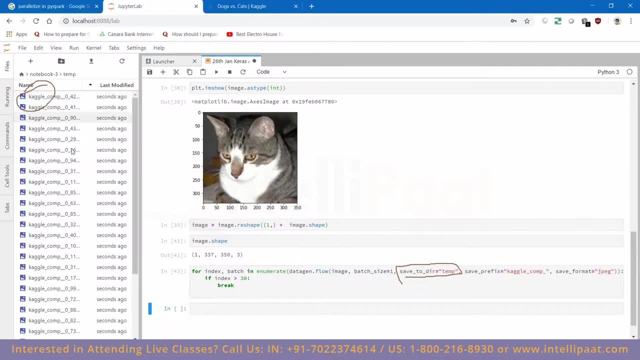 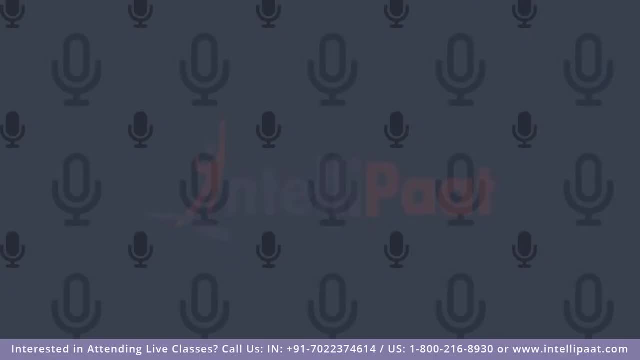 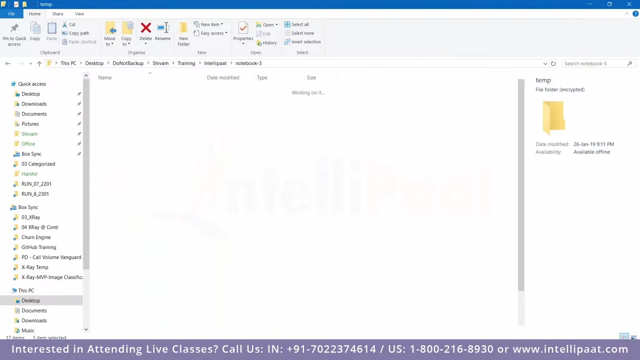 if i expand this, i have a lot of images. let's go and check it. if i go to the folder and if i go there, temp folder is here, right. so even if you can see this folder, temp folder- i go inside this temp folder. see on that particular one image. you have now these images. 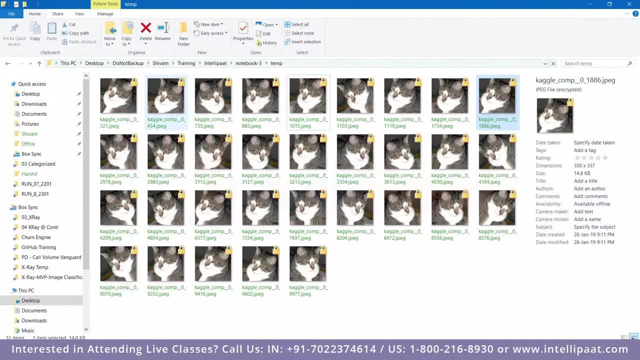 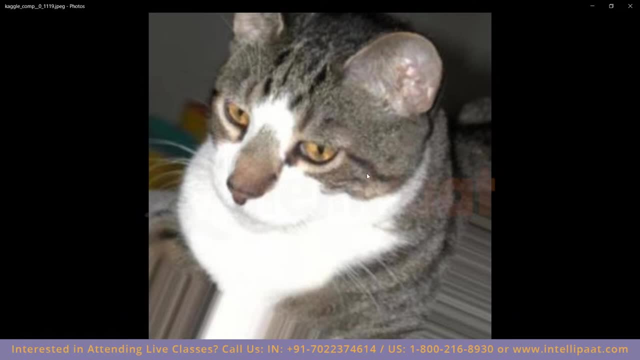 now, just think in in terms of numbers. now, does this look like the same matrix that you got in the original image? okay, yeah, see, they are different. right now, don't think in terms of image, right, for you as a human, this is still a image, right? just think in terms of numbers that. 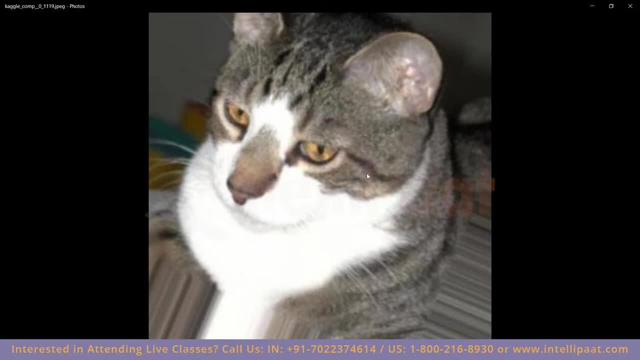 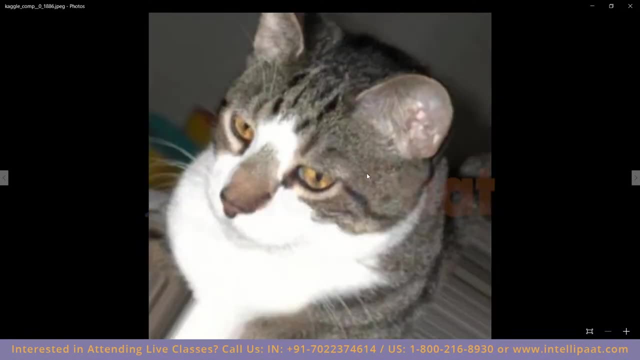 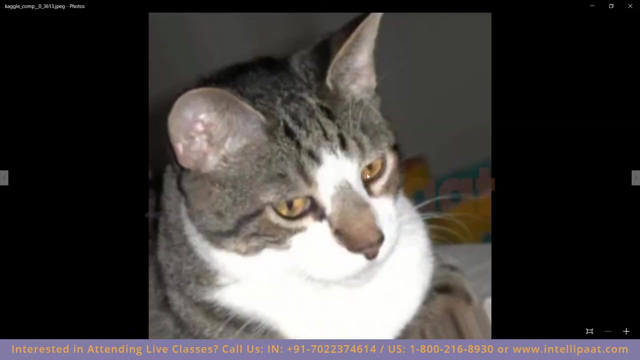 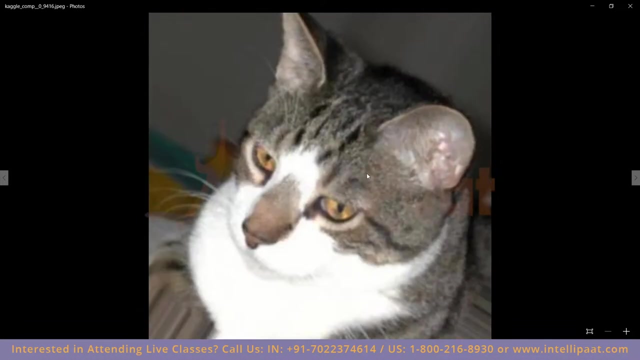 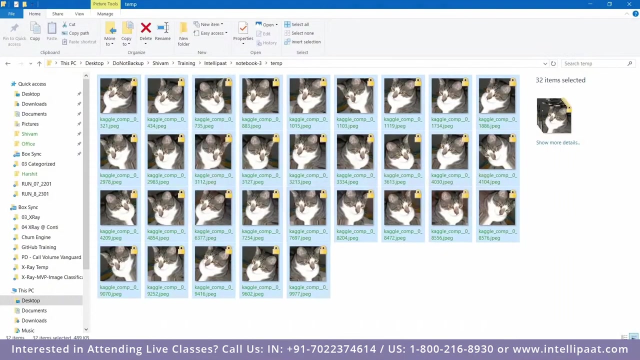 matrix that you got in 370 into 520 into three channels. now do you really think the number are going to be same? so just for one image, we got like 20 different combinations with like five to seven things right. so this is how you can like: do these things out right and then see how convenient. 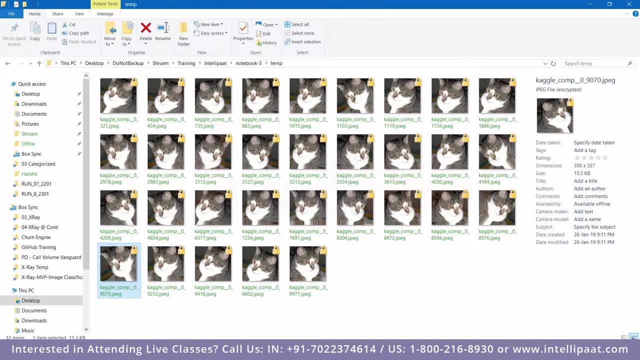 it is like it tells you that: what do you want? to give it a name like gaggle, underscore, something, something, something, and then you want to like give it some name also. so it is. it is giving you like everything inside there. this is how you can do these things, but the 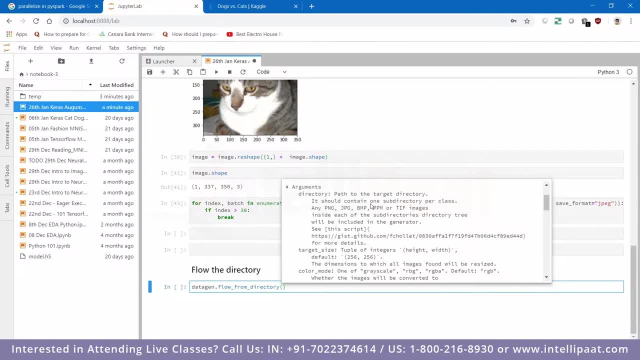 most important thing is that what kind of images you can provide to the directory right? you can give it png, you can give it jpg, you can give it dmp, you can give it ppm and tiff. if you are giving any other kind of image, no, no, no, please don't give right. 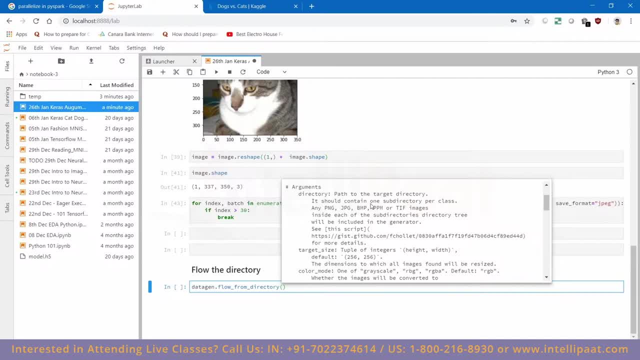 you have to obeyed by the rules, that these are the only images that you have to get inside right. next thing is the target size. let's say that you, because your images are of different, different dimensions, and we saw this in last problem also, if you guys remember, we were 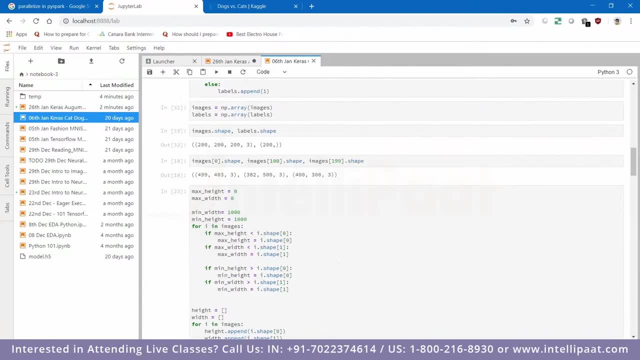 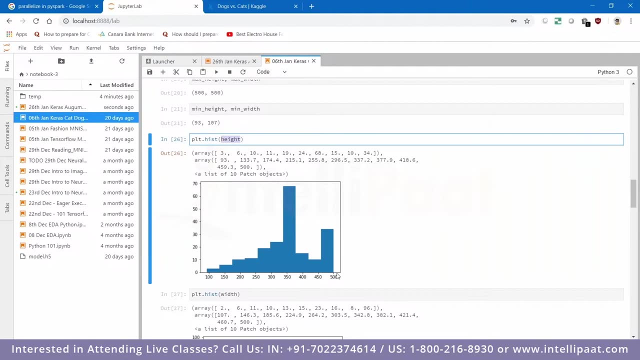 having this problem that our data had images of different, different dimensions, and this was the plot that we got for height. we had this thing right, so we came to know that three fifty one was a median height that everybody had, but our height ranged from hundred to five hundred, and 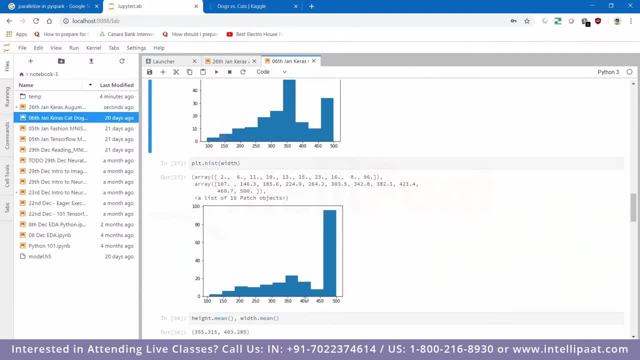 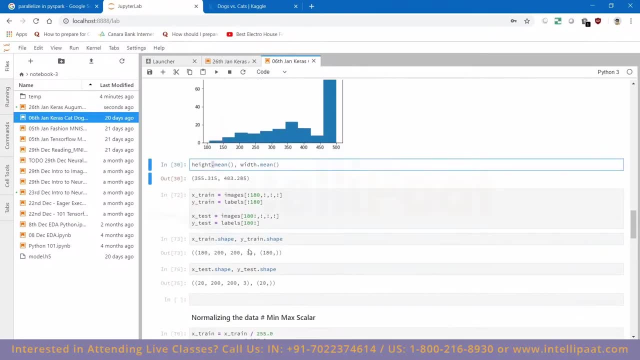 similarly in worth also, our range was from 100 to 500. so what we had to do, we had to somehow come up with the mean height and mean average, and then we have to convert our height and shape into some constant things. right, remember now here let's say you don't want to do all this thing. headaches. 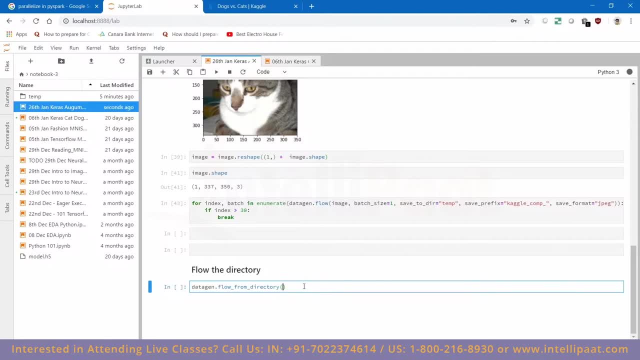 would you just simply say to the model the flow from directory. you just say to him that, okay, this is my target size. convert all my images into 140 custom images. that way, that's how you can make that. so i came up here. inthank you guys. in wireframe does being custom clothes in the? if you guys did this. 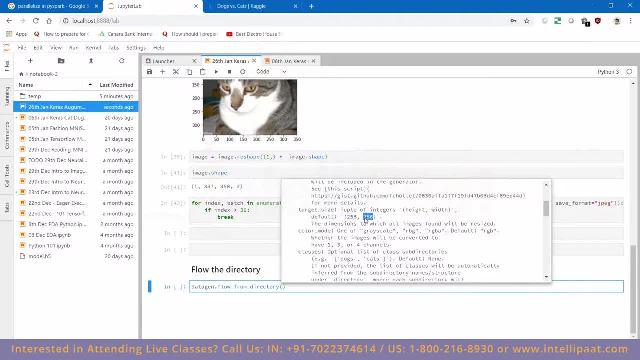 problem with Chrome? uh, i have a lot of experience with the field. style is being said because when you come to compile the data, when you build a page, if you don't have a style, EST's available exactly with the my images into this size: 256 cross, 256 or whatever you want to give right by default if you're not. 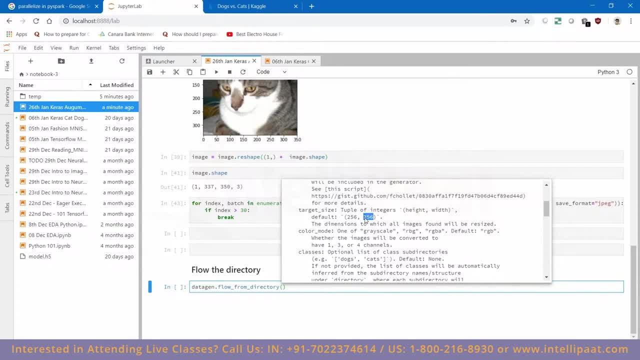 giving it anything, it will convert the images into 256, into 256, right. then you can give your color mode. also, let's say that your model is: you have a lot of images and your model- i mean it's a very small. your images are too different from each other and you don't want to take all the data. 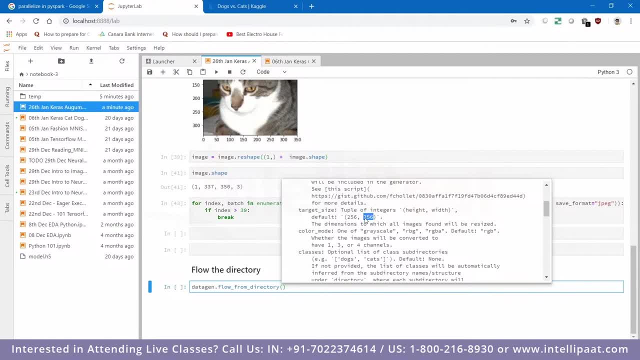 of three channels. you just want to make it into a grayscale. also, you want to make a grayscale model and you want to read the images into grayscale? don't worry, just tell it to kiraz. just say that, okay, my color mode is rgb or grayscale or rgba, whatever you want to give. 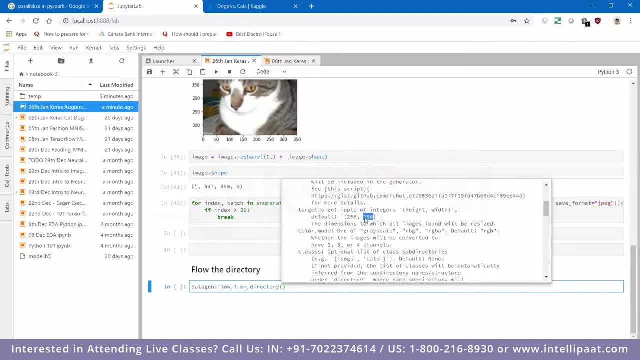 just give it right, that's all. now you might ask me this question: what is this rgba? rgba means that this is a four channel image: red, green, blue and alpha. alpha channel is also known as the transparency channel. see, if you're dealing with images, you have to know everything about images. 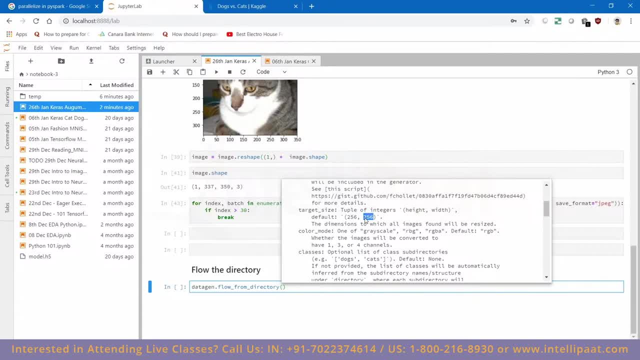 so i'll tell you my case. i was working with this client who wants to know that whenever someone is uploading an image, he's not uploading a copyrighted image. now, this is a now, this is one of the very serious problems, right, and- and this is like- everybody is facing this problem. 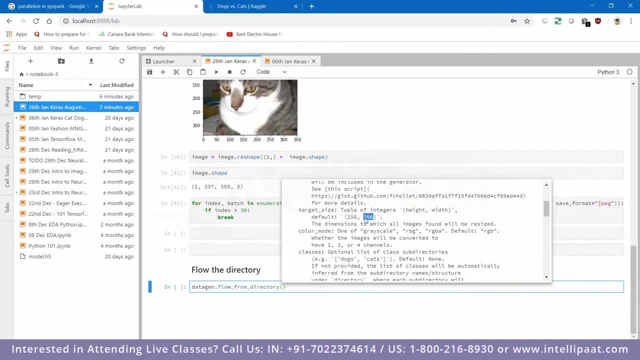 right, let's say that you have some e-commerce store and what people generally do: rather than taking their own photo, they'll take someone else's photo, like stock image photo or some image photo, and they'll upload it. now, when the user uploaded a photo on your platform, he or she doesn't care to solve this thing right, but stock image will see, he'll get. 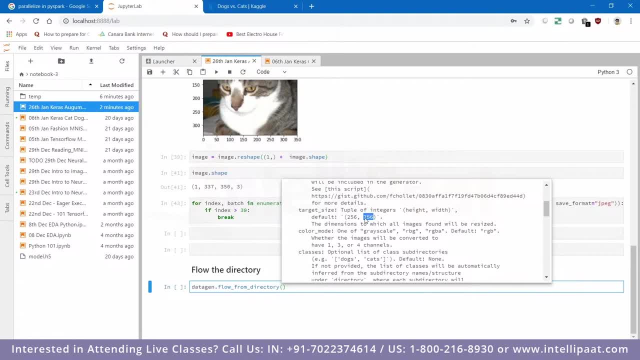 you. why is my photo on your website right? why is my image on your website? he'll catch you. he'll sue you, right? so this is a very practical problem that people are dealing right now: that they should not have someone else's copyright image in their data, right? so this is the problem that they're dealing. 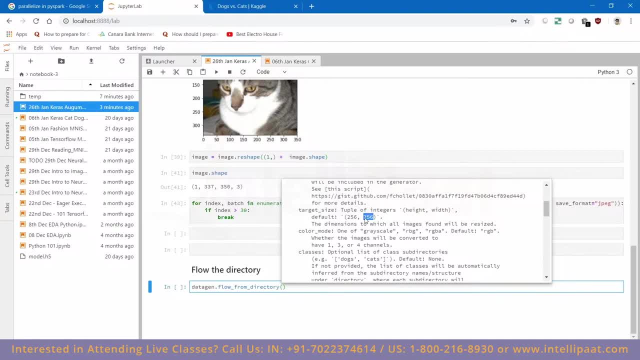 now, i was given this task. now, how do- and this was like in perry, like 2013, if i remember. so this image is in a past photo, but when they want to copy it, you have to use a file that is more transparent, right? so that means you will see that the image is not transparent and the image is not transparent. 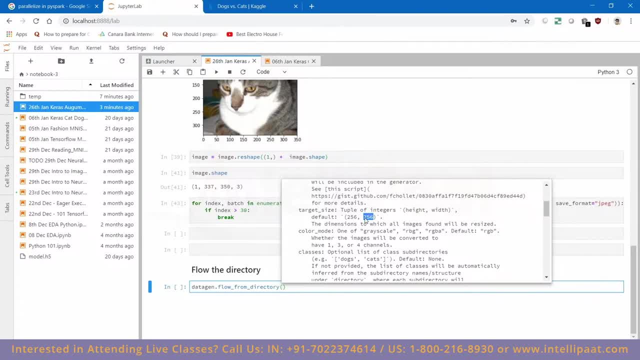 so that means if you press on this, probably that is called transparency channel. now, transparency channel means if you set this transparent 200 percent, that means you can see everything, and if you press transparency to zero or opec 200, it means that you cannot see anything. 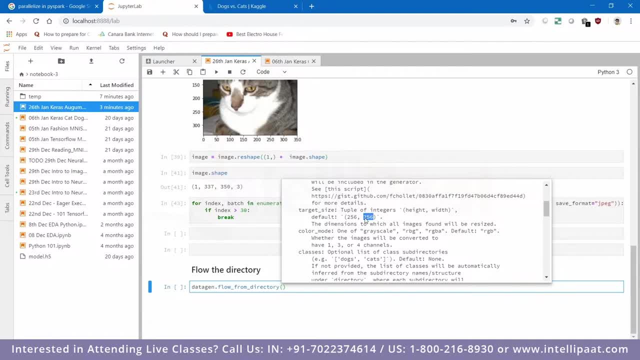 so whenever they want to copyright an image, what they do is they add one more layer of transparency and on that transparency they have their copyright seal. does it now? at that time, if i would have read this image normally, like rgb, then i would have never read the the copyrighted logo on this. i wanted my model to learn that. how are the two images? 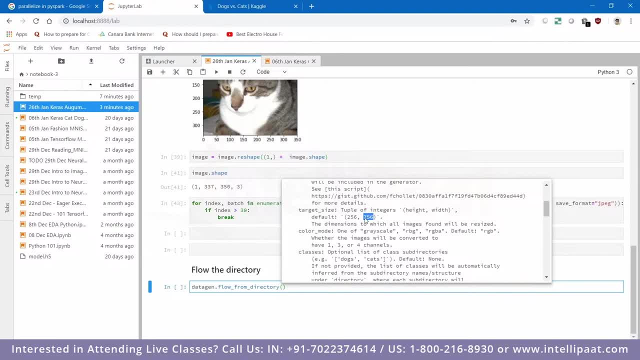 different right. one has a watermark and one doesn't have a watermark, right. so that's why i had to read both the things, and this is how you do. you read your color mode as rgba and this way you're telling your model to read the image with a alpha channel. read it and it will help you, right. 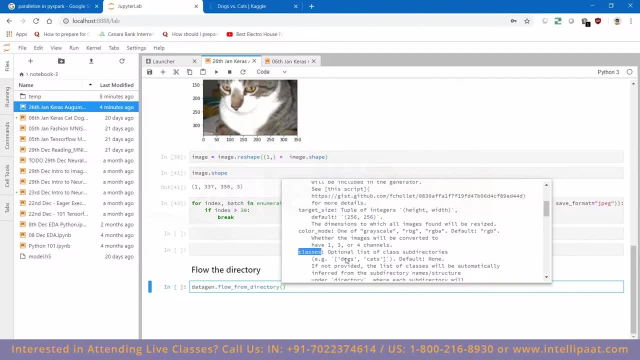 then the fourth option comes, is the classes. now let's say that this is actually an optional thing, but you should tell your model that how many classes do you have? and then, based on that, it will look for other things also. let's go to one more thing, that is, class models. so class mode. 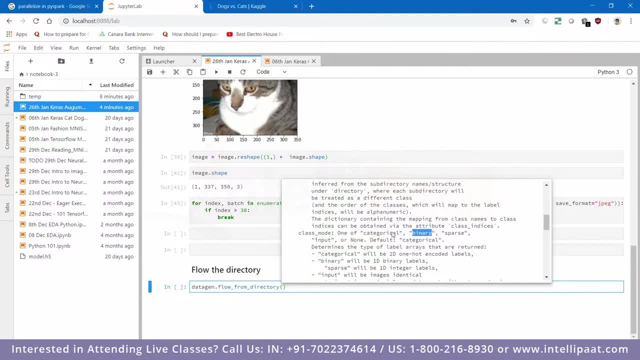 means that. is it a binary kind of a categorization or it's a categorical kind of a categorization you're looking for, like one category, true and false. categorical means that you're looking for more than two, two or more than two, like that dog elephant, i don't know. right binary would have been. 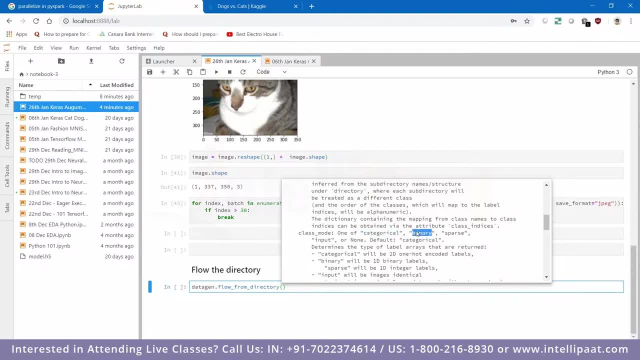 the case where you say dog or no dog, right, cat or no cat, right. then you have some sparse categories also where you have some less uh, and then some unbalanced categories also right. if no labels is needed, then it will take batch size. now, batch size is one of the important size. now you are. 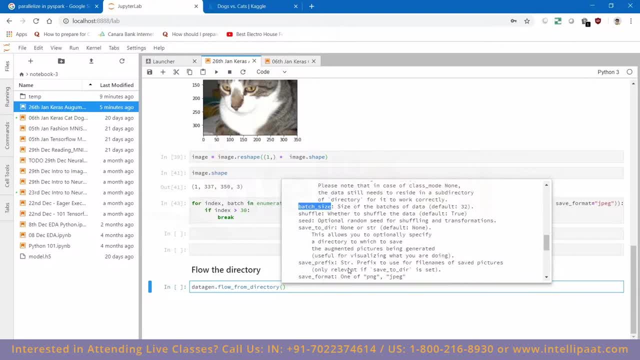 telling your model that how, if you want to- let's say that you have 100 images total- then you are telling your model that that size means 25. it means that it will create four buckets for you, each of size 25. for you, 25, 25, 25 because 25, when added four times, will become 100. that will become 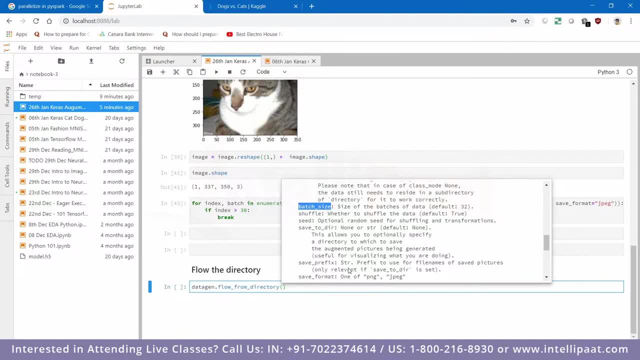 the total number of images that you have in your data set make sense. okay, then you have this thing called shuffle. now, this is a very important thing, right in my case, when i was doing this, uh, this thing called to identify if this image is a watermarked. 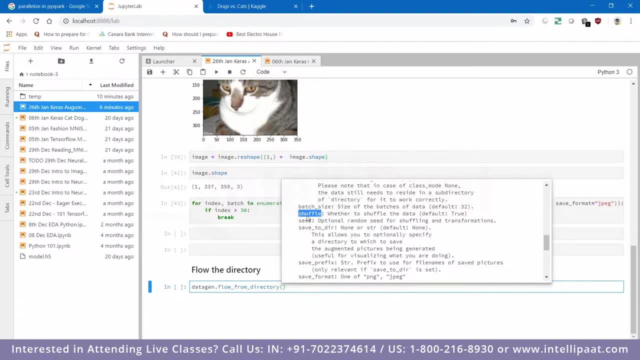 image or not. at that time i have to feed the image one by one to the model. and when i say one by one, i means one image not copyrighted, second image copyrighted, so that the model can learn that. okay, this is the difference between the two images. these are same images. there is only a small. 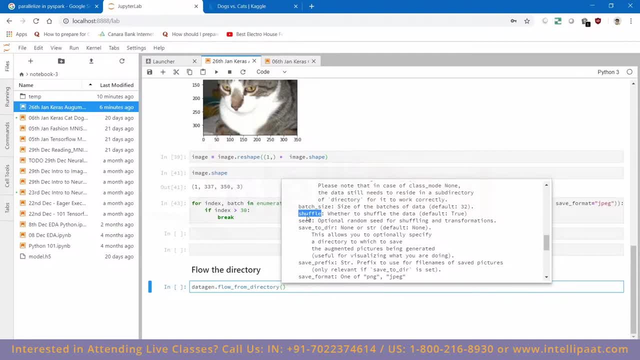 copyright logo on the left right section. so my model learned this: if imagine i would have shuffled my data set, like one image randomly is going with the other one's copyright image, then it would have made no sense to me, right? that's why i always remember: shuffle, yes or no depends on your right. and then this thing is seed. 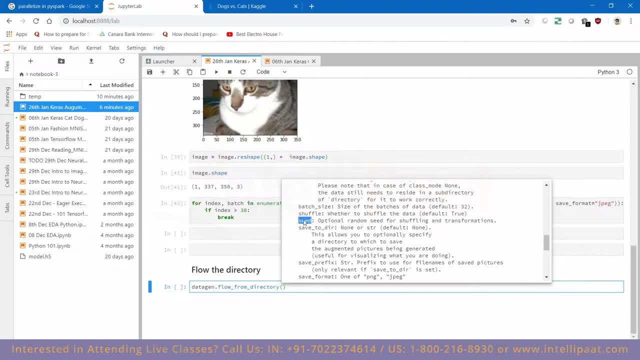 seed. you always remember nprandomc that we did right. nprandomseed ensures that. what kind of a randomization you are using. let's say that you are doing a model benchmarking and then you need to do so. all your randomizations are now constant on your particular laptop. if you provide a seed right save. 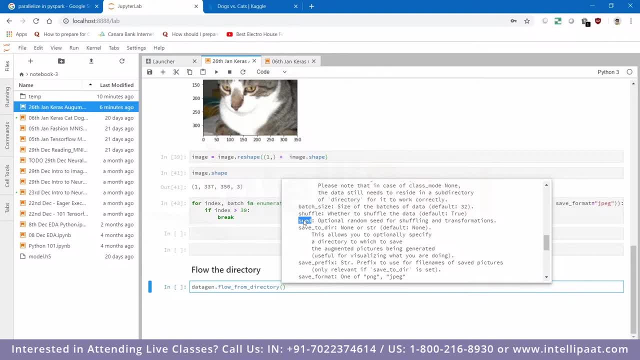 to dir means that say that you don't want to do it on the runtime. and when i say runtime, i mean that your model is running your. your model is doing the training. at that time, kiraz is doing all the augmentation, giving the images to the model. that's it. it's not saving somewhere until and unless you. 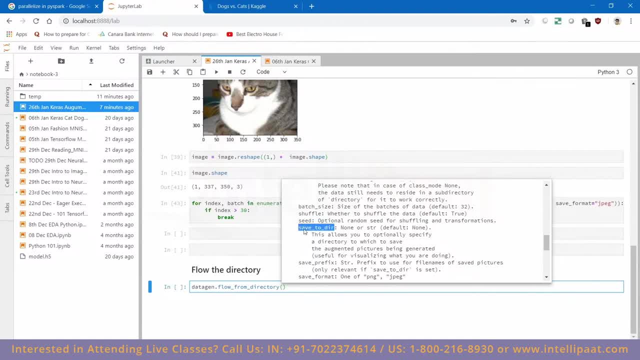 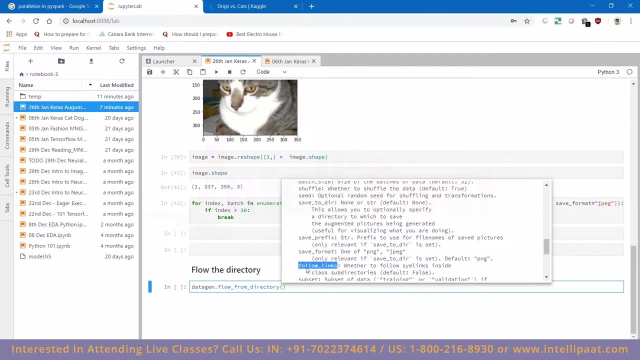 give this thing save to the ir, save to the ir, then you have this thing called save prefix. then you have, say, format that we just saw right now. right then we have follow links. follow links means that you know, you know there are like some symbolings. also, if you're working on linux or unix, you know. 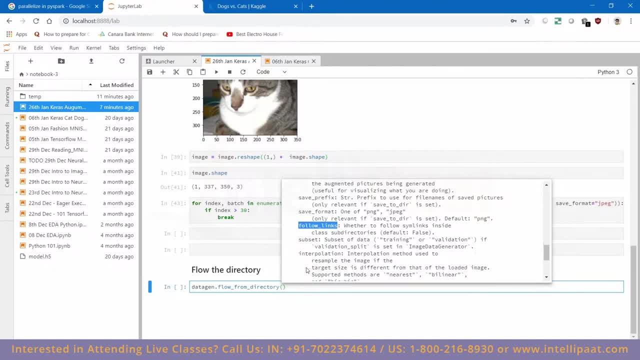 symlinks are like soft links. if you want to go inside of the data also- this we're not doing- then we have subset. let's say that you have done the augmentation but you want to do it on the uh, you know, on your validation data set also right now. sometimes people want to do it on validation. 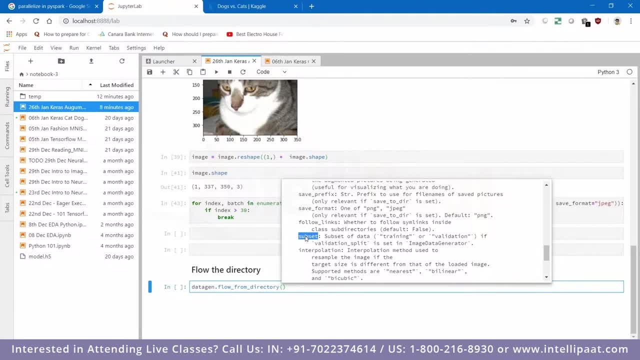 sometimes not right. sometimes people just say no, they don't want to do it, but sometimes people have. I am going to validate it only on non augmented data set only and it's fine. You know, sometimes business case things that okay. No, validation should always be done on non augmented. 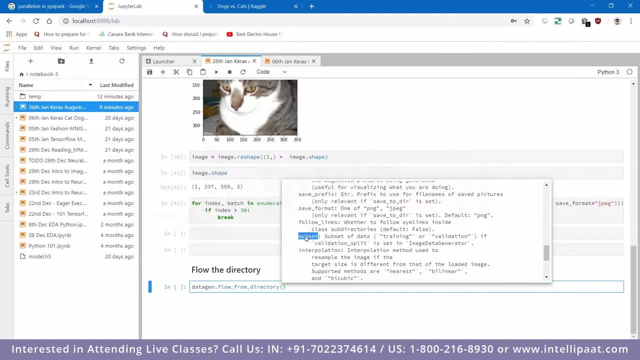 Augmented images are not the real images, So they don't do it right. So it's up to you. What if you want to do it on training or validation? you can just provide it. There's this thing called validation split. validation split means that whenever a batch is going and you say, validation split is 0.2. 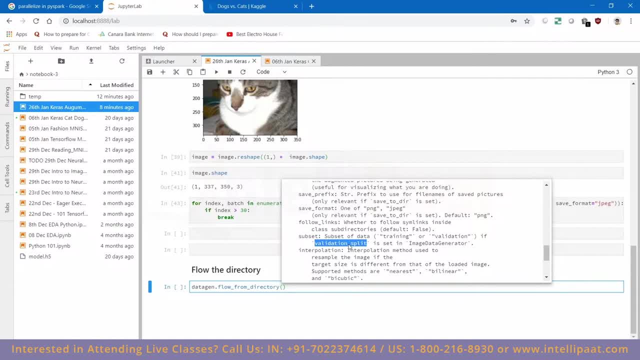 It means that point two percent, I mean it's out of ten images. two images will be kept for validation and you will get the validation score also out of it Right. and then you have interpolation. interpolation is again a different kind of a thing that you want to have, a nearest kind of. 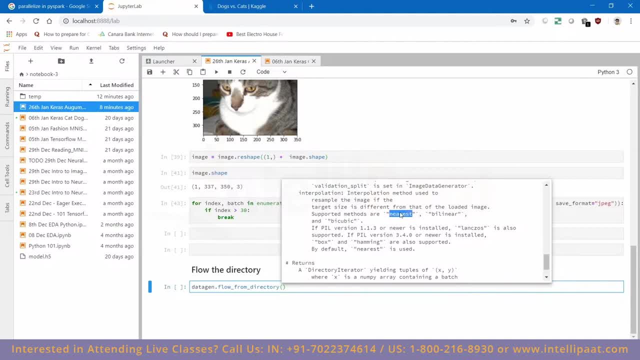 So whenever the image is loading, there are like different, different things that you can put in, like nearest color or binary color, or Bicubic color, whatever color target you want to do it. It's meaning it's just a resampling of the. so whenever you are doing a resizing, whenever you are, 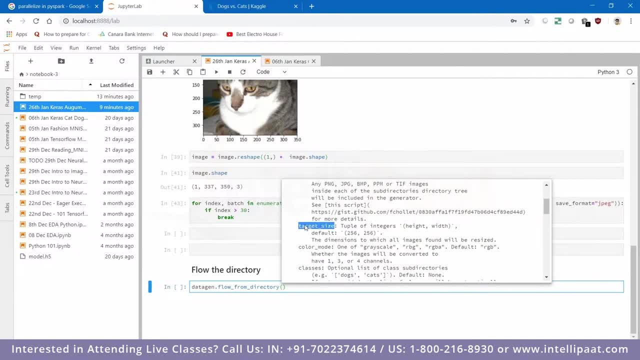 Giving this thing called. whenever you are giving a target size, It means that you want, you are wanting your image that is from the original type, to be reshaped into this thing. I 255 got to 256 or 256. now reshaping is again a very complex thing. 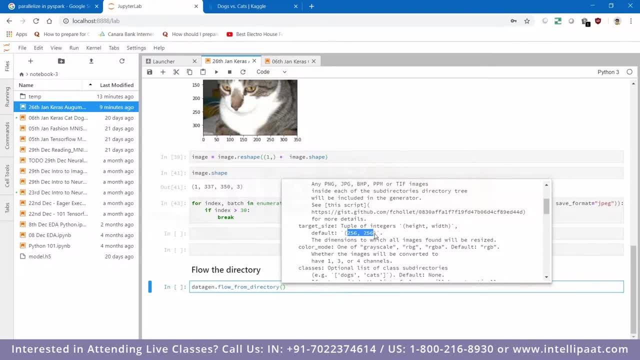 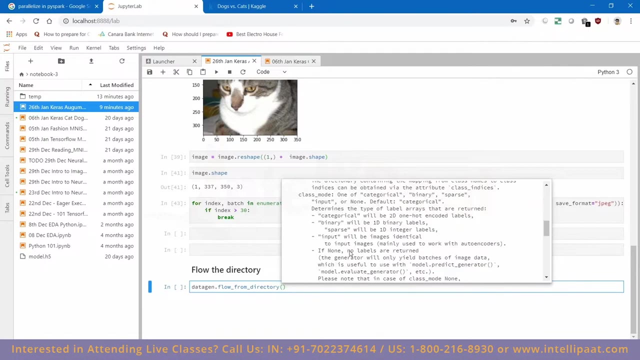 You know we, if you imagine it mathematically, then it's very complex, right? and don't compare Resizing to rescaling or cropping. cropping is simply deleting the image, right? We are not deleting the image, We are resizing the image, Right? so resizing has different, different kinds of algorithms that you can use. 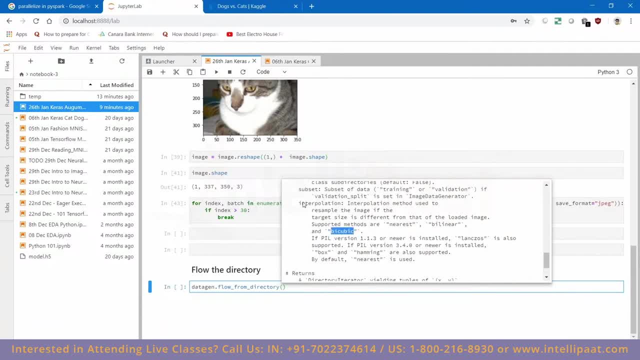 They are like bicubic nearest bilinear. all these things You can put it right. if you don't, it's like: although is a, it's always a by default thing. That is always. you have the key aspect. now What is the return thing that you are getting right in our example? what we did was in our example. 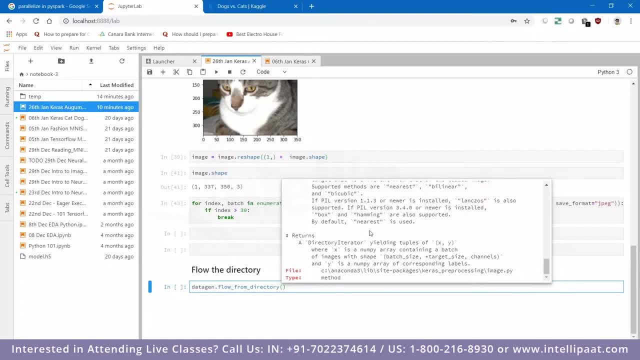 We did this thing called save to DIR. So whenever you are doing to save to DIR, It is going to save it inside the In your directory, whatever you have specified. Let's say We didn't specify that thing, then what is it is going to yield? it is going to yield two things: a tuple, a tuple. 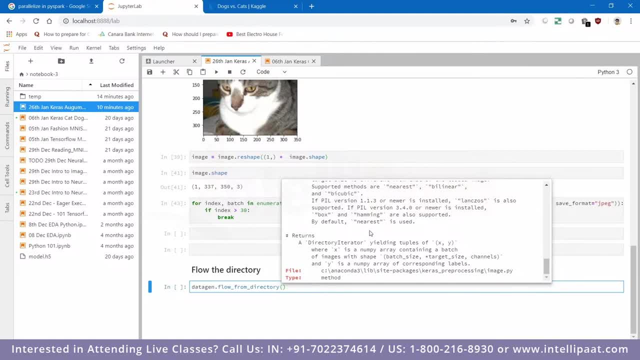 Of two things, X and Y, and it says that X is the numpy array that is containing a batch of images Which shape whatever you have given, and Y is the numpy array of the corresponding label. right, You might think that we have not done the training till yet and how it is giving the labels. 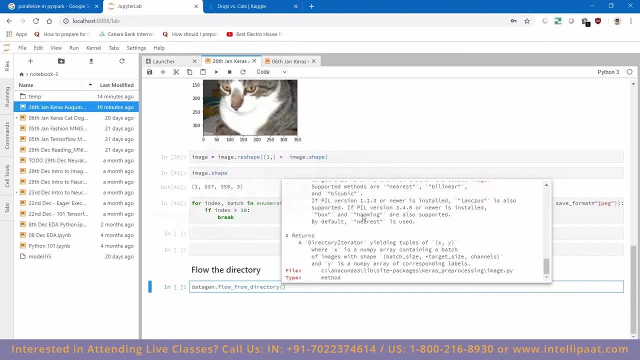 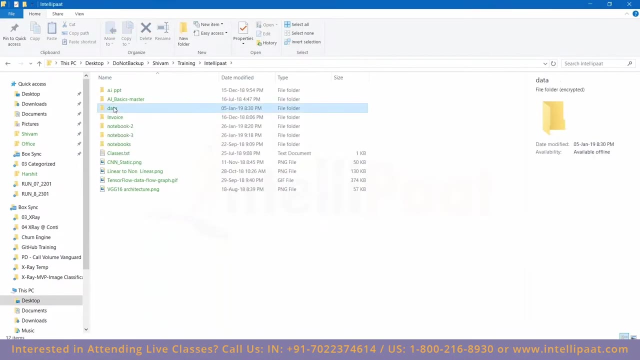 Because you specified it right and I told you that. I'm going to tell you in like five minutes that how is how You should give the directory. right now it comes the important part. Let's switch back to our folder. We have all the images, Whenever you want to read your data through generator. 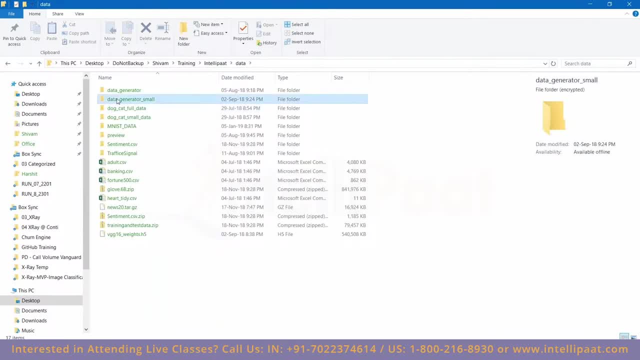 Always remember, always remember that you have to start like this: First of all, create a parent folder. Let's say I can drop a folder called data generator, small. now this folder will contain folders, not the files. this folder will contain a All the categories in which you want to divide your data. 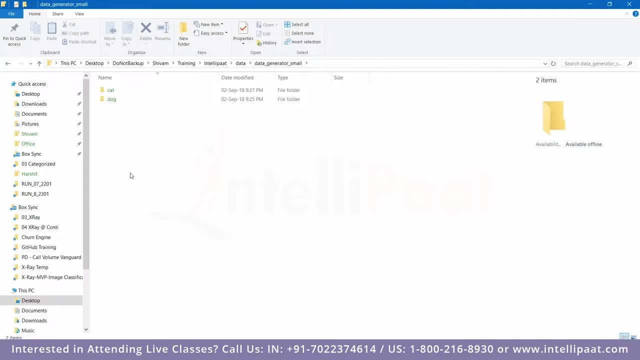 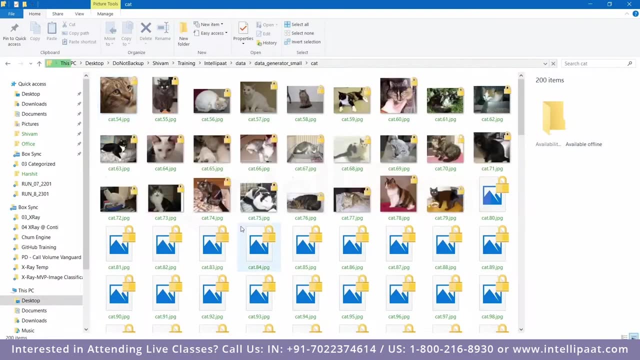 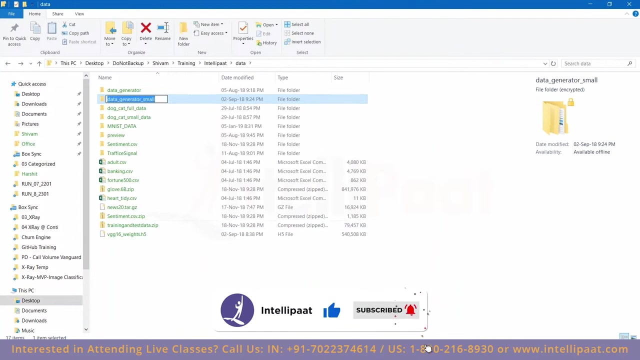 In our case, we have only two categories: cat and dog. So what I did? I created two folders: cat and dog. all the cat images are inside this folder and all the dogs images are inside This folder. right, and to Kiras, you will give the path still here. data generator small. 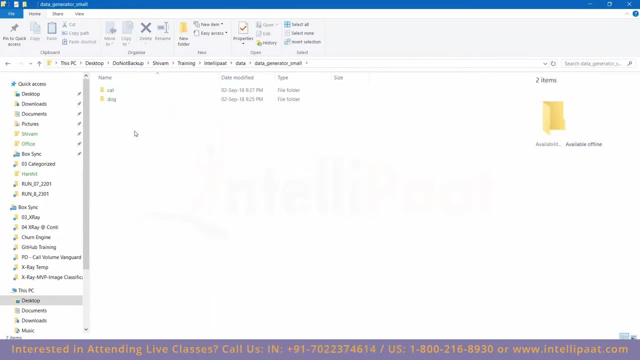 Now Kiras will go inside this data generator small folder. It will see: Okay, so the user has given me two folders. It means that it has only two classes- cat and dog- and then it will read all the images from cat and Images from dog. so now what you have done is you have read the images and it will give you. 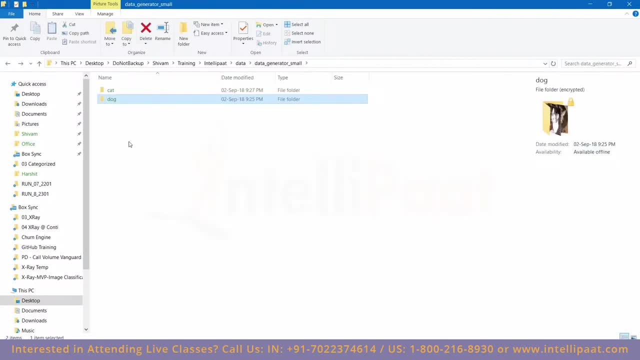 Okay, cat means zero and dog me one from here. Right, It is not necessary to name your folder. whatever I mean, whatever you can name it, This is just for Kiras to know that which category is inside which folder and which category is inside which folder. 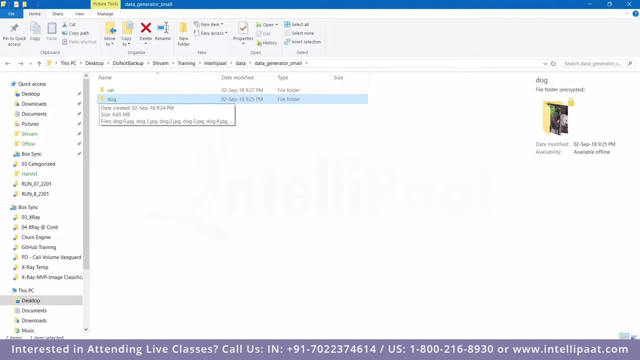 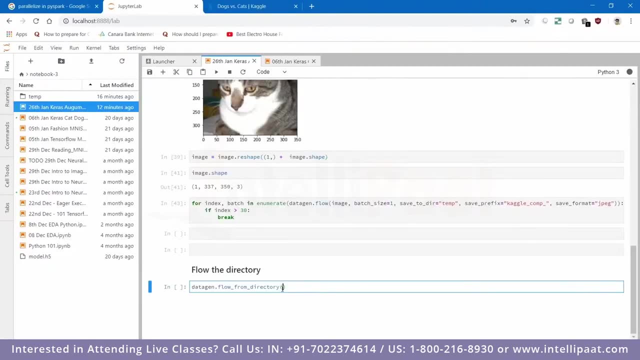 Just for the knowledge of Kiras, Let me show you then. For example, let's go back to our Jupyter Notebook. Simply, let's say nothing, but the first thing is the directory. Directory is data path. I think data path is it. 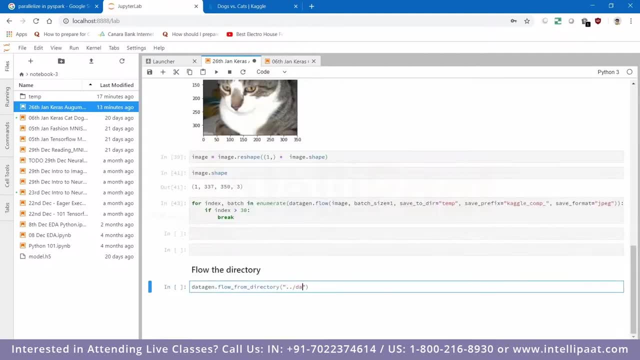 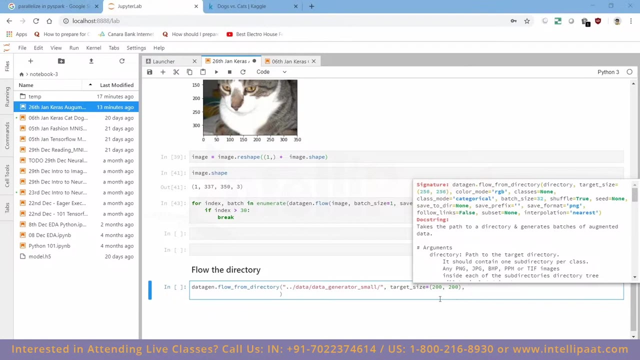 No, I have to change it. Let me type it statically. I'll say data and data generator: small. I will give it just till here, nothing. Then you have target size. Let's say our target size is 200. Then next what we can do is let me move it here. 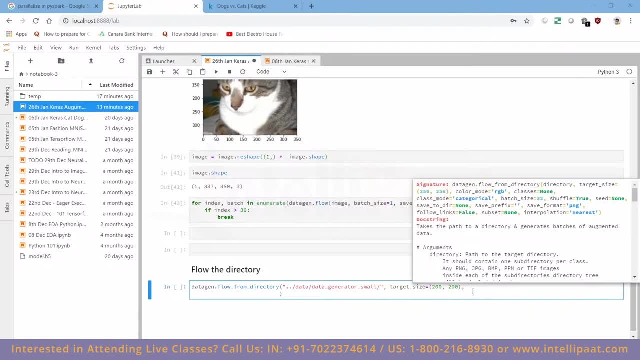 Color mode is already RGB. classes is none. class mode: categorical batch size: 32.. Okay, let's change the batch size. Batch size I only want as two, only two batch size Then we have. we don't want to save it somewhere. 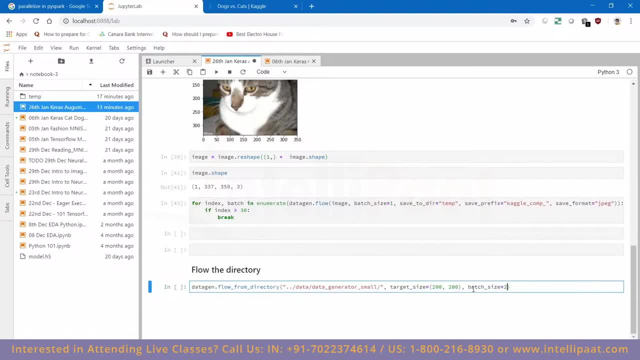 we want to shuffle, yes, we want to shuffle. We just do like this. Now, what it is going to yield is it is going to yield a tuple with X, comma, Y. Let's see what it does. right, X and B is equal to one, and then we're going to break this. 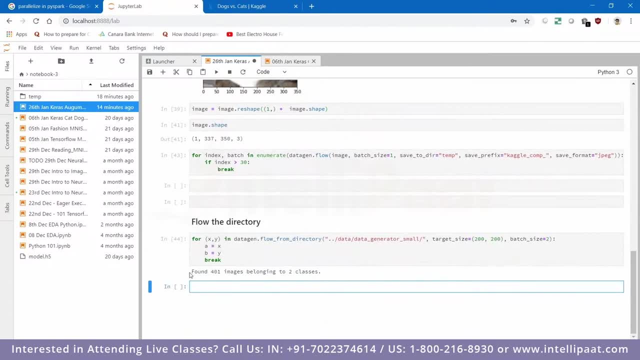 So it says: see, whenever you run this, it says that found 401 image belonging to two classes. Now how did it know that there are two classes? Because he gave two folders inside this folder, right? So it doesn't matter, whatever you give the folder name. 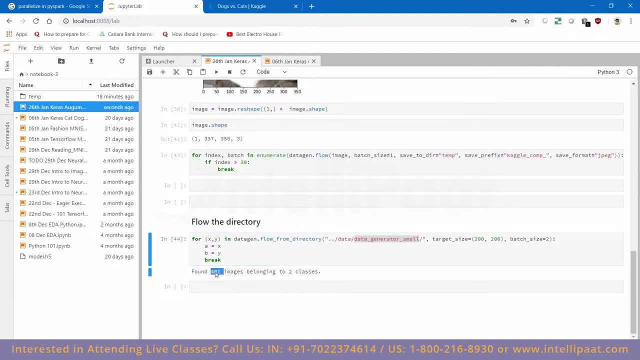 no matters, but it just want to count that which folder belongs to which. It says 401 images. so one folder contains two, right? So it doesn't matter. whatever you give the folder name, no matters, but it just want to count that which folder belongs to which. 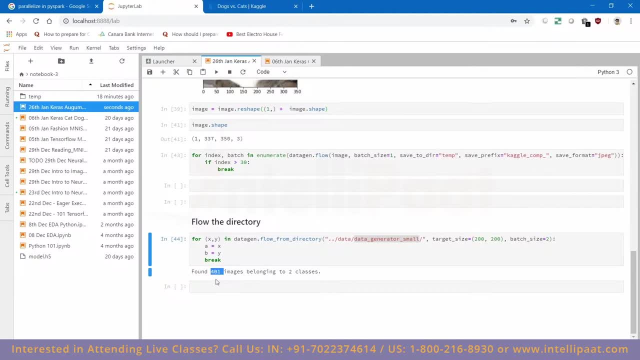 It says 401 images. so one folder contains two. So it doesn't matter, whatever you give the folder name, no matters, but it just want to count that which folder belongs to which. So it doesn't matter, whatever you give the folder name, no matters, but it just want to count that which folder belongs to which. 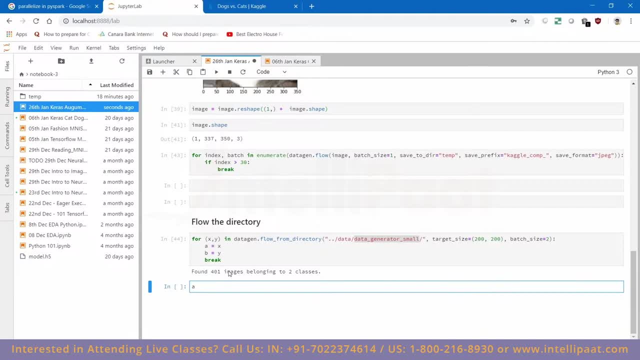 Now let's see what A and B brings to us. A should be a NumPy array, correct? Okay, let me just type in there, only so that it's for reference. And B should also be a NumPy array, right? Very good. 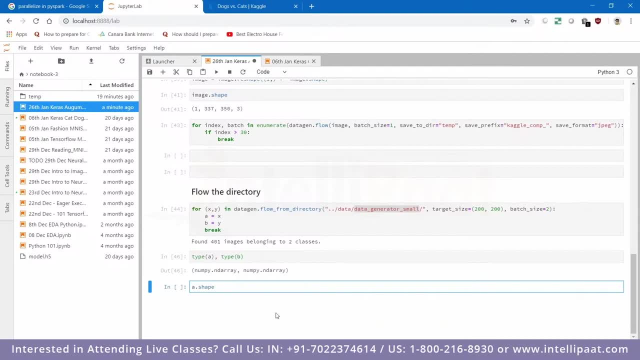 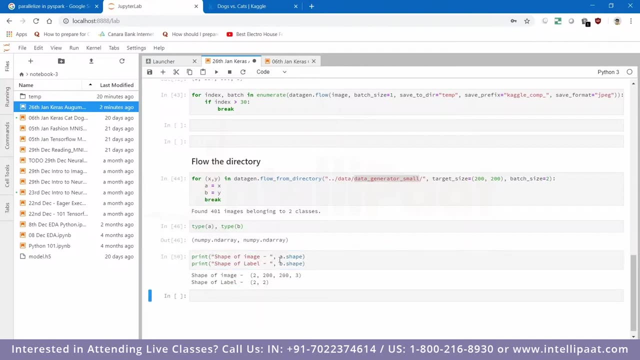 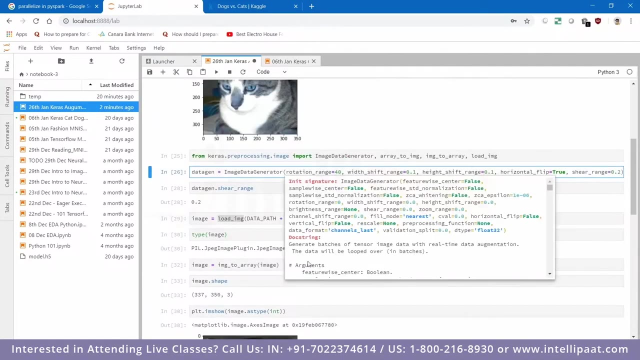 Let's just see the shape of A: Two into 200 into 200 into three. Okay, I'll take this one for the team. See you already? see, I told you that image data generator will always take this into batches. It will take it into batches, right. 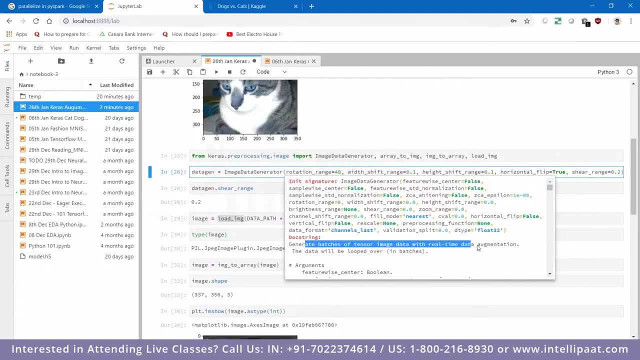 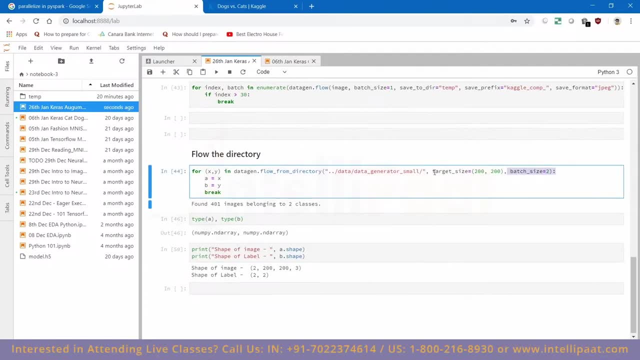 And it will generate batches of tensor images with real-time augmentation. In this time, our batch size was two. What was the expected image that you want to get out was 200 cross 200, right, And how many channel of images do you really had in the starting? 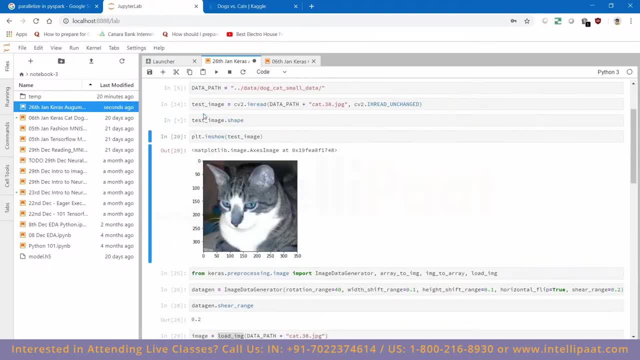 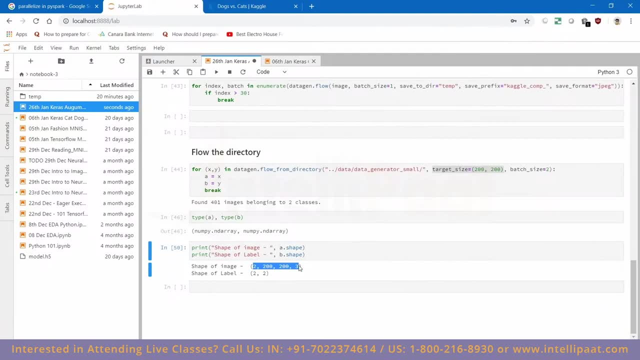 Go And if you see, It's a fundamental. that simply means that this 202 into 200 or 203 means the first two ways is the Barth size, second is the height, Third is the width and fourth is the channel right And Shape. 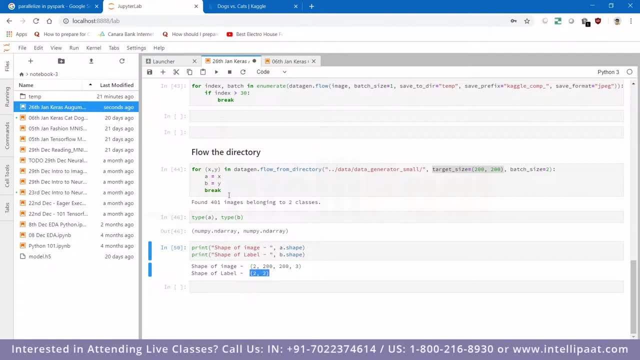 Of label means that because this thing yielded out two images, it is going to minimalize this entire sina kilogram approximately this, and that is just primero San durum and lettering littleicz to print the two labels of the initials. let's see what b is. b says the first thing is oh 101. 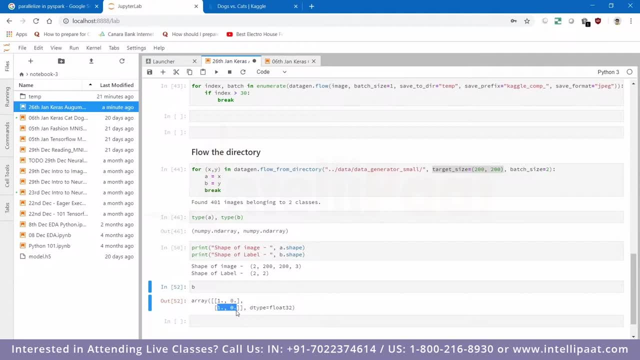 and this is the one hot encoded return. it has returned it into one hot encoding, so i imagine that this is one. so this should be a cat. let's plot this plt dot, i am sure, and we want to just print the ace first image, right, this is not going to do because it's a float type as type. 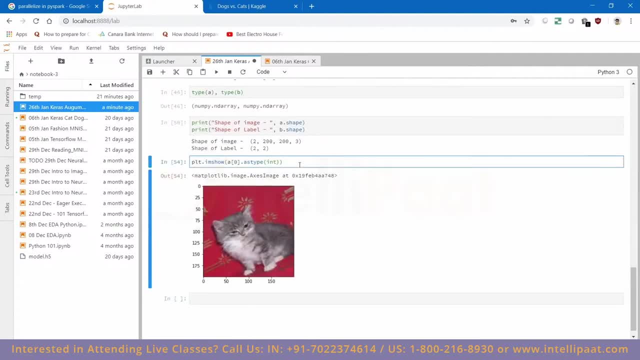 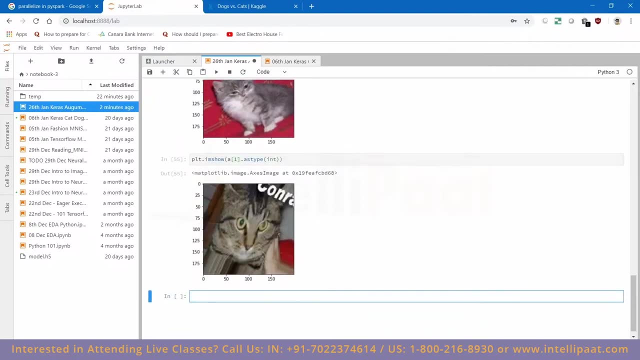 int see it's a cat, and if i print the second image, it's again a cat. so this is how what the model has done is that it is on the real time basis. it has, but it doesn't. it has, like, augmented the image and then it is going to give you. this was the method. 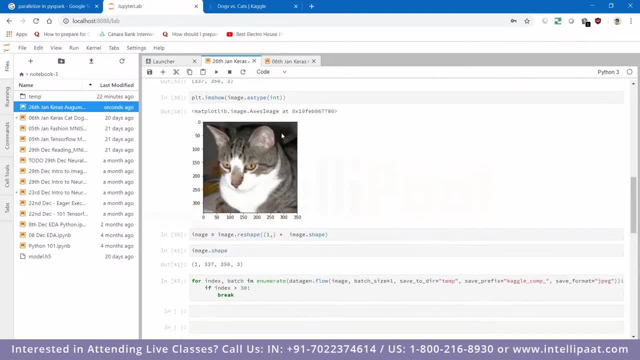 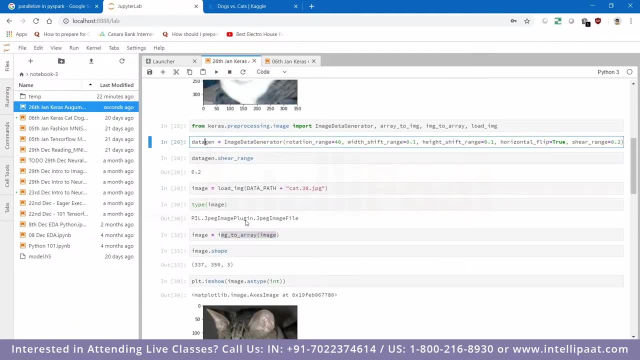 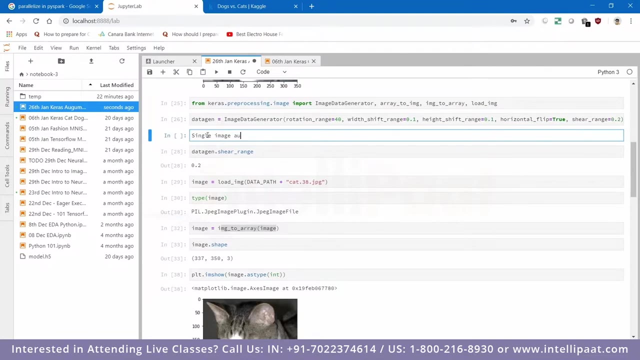 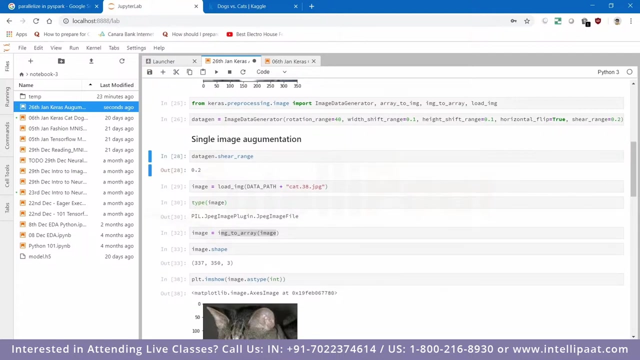 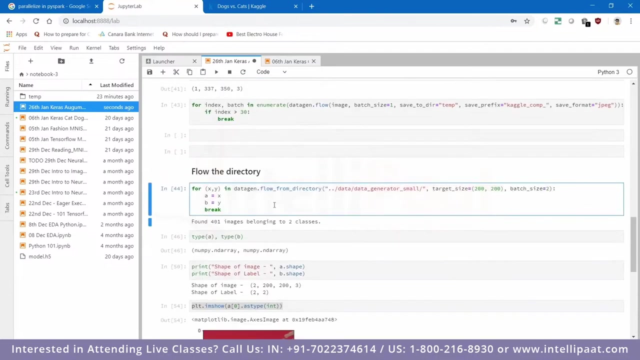 different from flow of a single image. right here you were converting, reading all the images on your own, like, let's type in here: single image augmentation. okay, and this is a flow from directory, where i just said that: read from the image and then convert it into things. right now, see, this is going to yield a. this is on a yield process, so it means 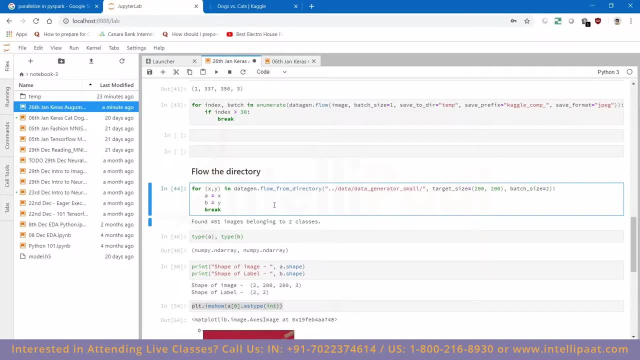 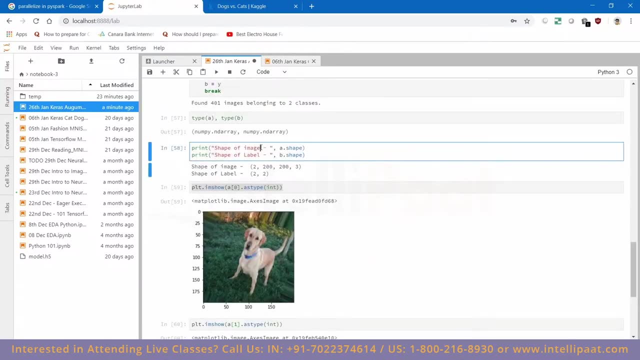 every time it is going to give me a different answer. let's say this time, if i do this, there will be new images. see, it's a dog image, it's a cat image and, if you want to see, there might be a difference. now, if this is a cat and if it's a dog and cat image, then it means that this time your 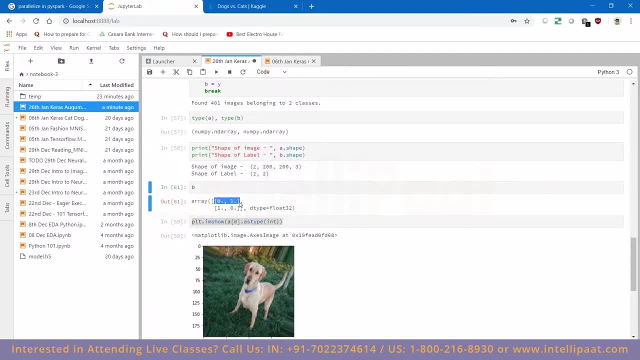 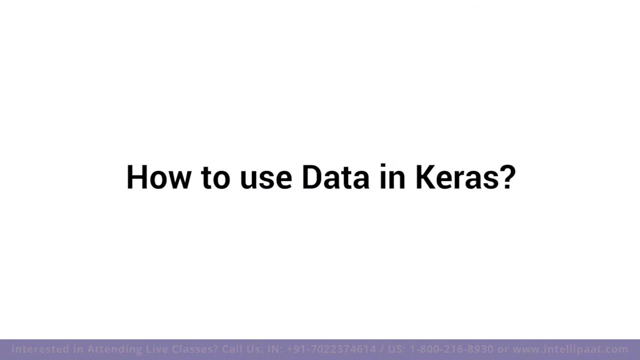 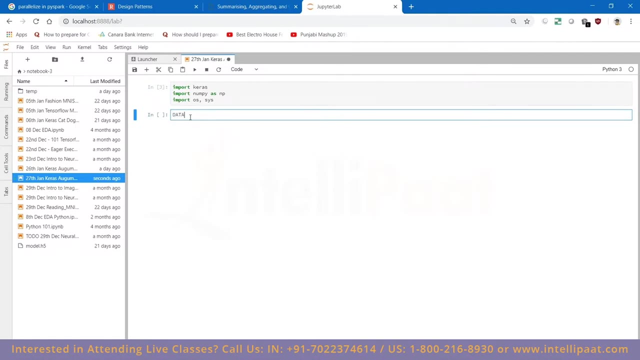 see 100 encoding is different. the first 100 encoding is zero, one it means it's a dog and one zero means it's a cat. right, how do you use this particular data inside kiraz? also, i'll quickly again load the data data path and then equal to data and then dog, cat. 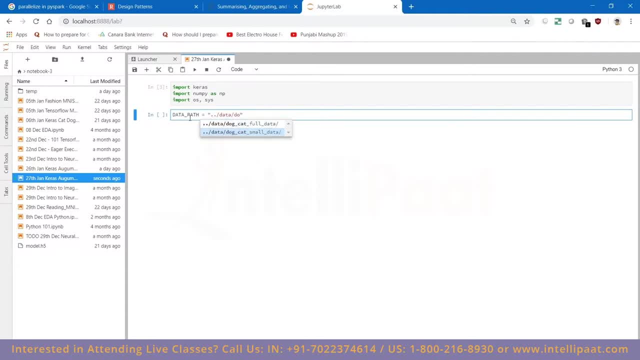 we have generator also right, where is the path? okay, here, that is control c. and then we have generated, also right, where is the path? okay, here, that is control c. okay here, that is control c. oh, yes, we have. okay, so we have data path. i have set now this data path. i'll again show you this. 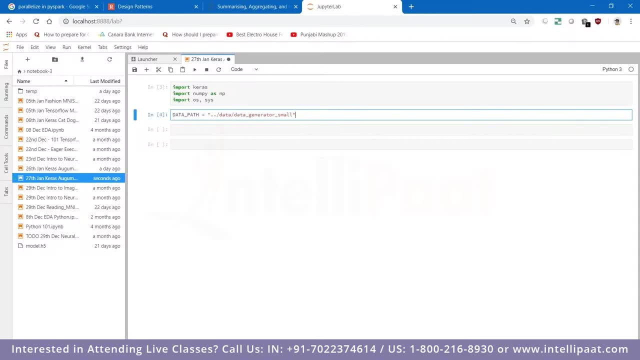 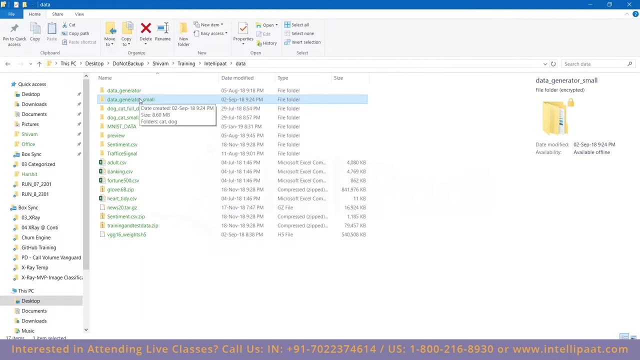 thing, and this is actually how do you set this path. very important. please see that i have made a folder here called data generator, small. now this data, this, this folder responsible to contain multiple other folders which will the categories of your model right and then inside those categories, you. 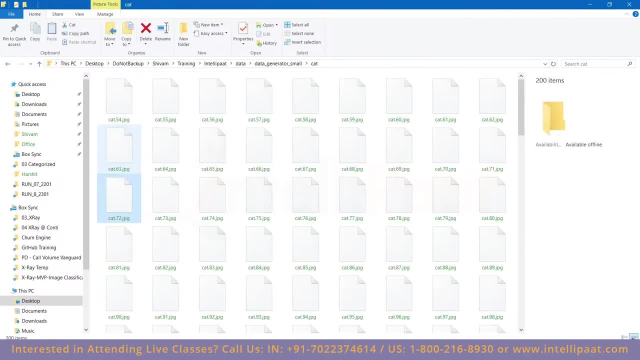 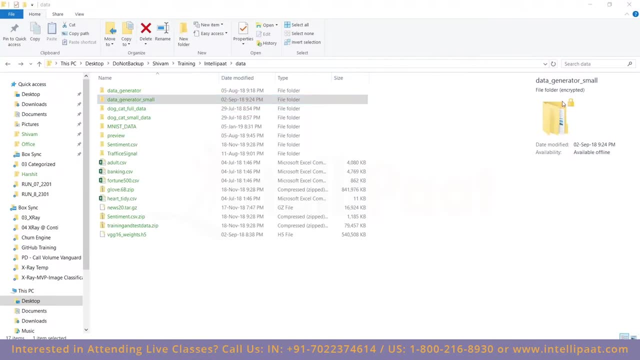 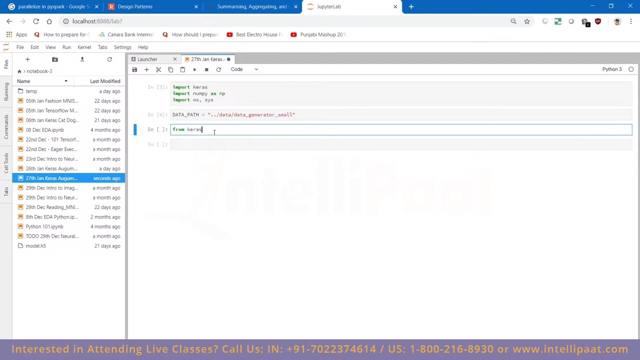 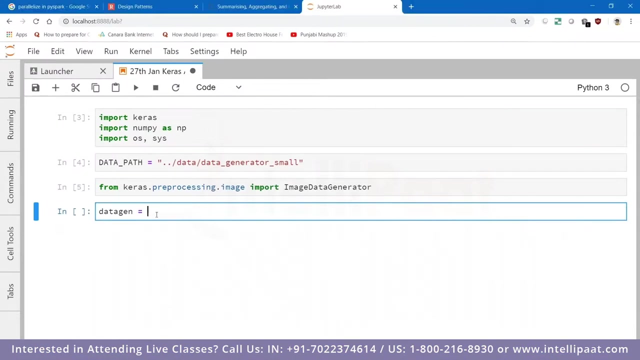 will have different different of your data sets. right, so you have to take the path till here. only data generator small, don't go inside that. right now we can see here i'll quickly do this augmentation thing from kiraz dot pre-processing. uh, let's quickly make a data gen. 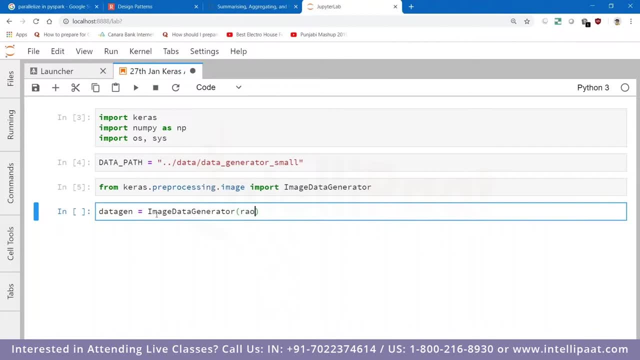 data gen would be image generator. if i do, let me do a rotation, rotation range, let's say 20, then you have. you have, your horizontal flip is equal to true. i won't do much, i'll just do this just because, so that you know, we get to know. 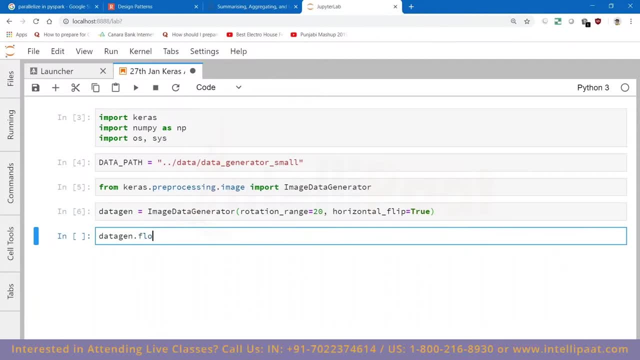 how we are doing this. then we have data gen dot flow from directory. right now we know that this is going to flow from directory. i can just simply say data path right, and it says that the data found four zero one images belonging to two classes. correct, we? 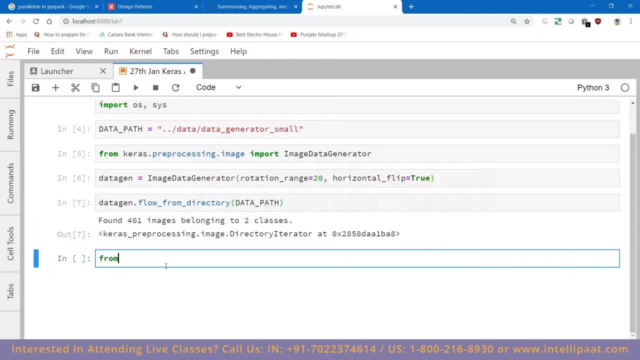 have only two classes and there are 401 images. now let's quickly build up the data. also. this is tense, this is flattened and um, what else do we have? okay, this is this. we'll add it later. from keras dot losses: import- categorical cross and droppy. from keras dot optimizers: import- rms prop. or we can use adam. 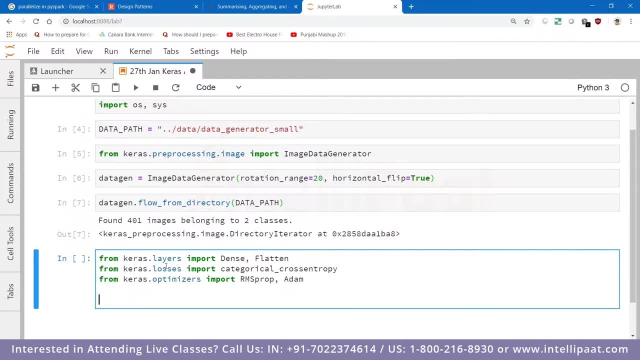 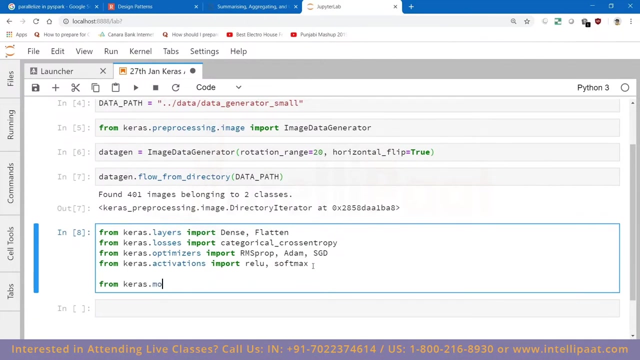 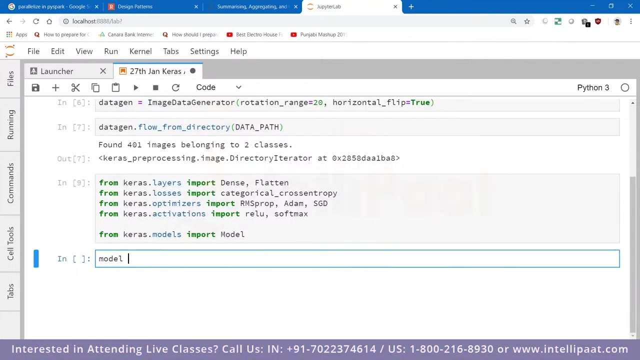 right and from, or i think we should simply use the std also- and from keras dot activations import rello right and next we need is softbox. all what we want, if you want- okay, we forgot the most important thing- from keras model input model right, let's quickly make a model. model is equal to 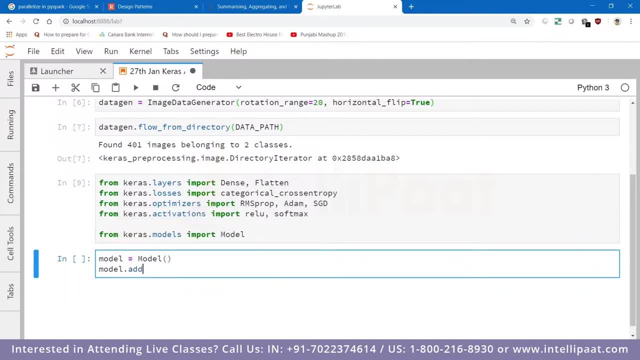 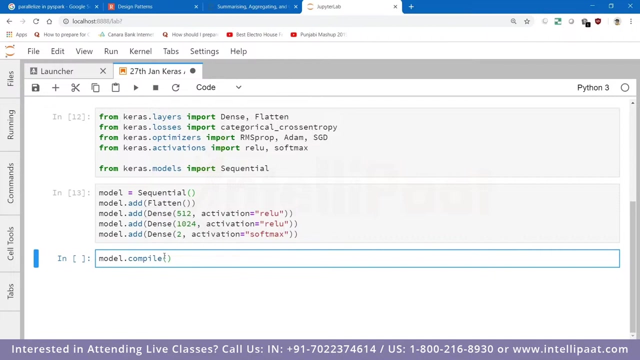 model right, model model, model, modeladd. how do you start this? What will be the next one? Okay, anybody wants to help me out here. at which thing should we use next Modelcompile, modelcompile? you say that you have optimizer as SGD right. 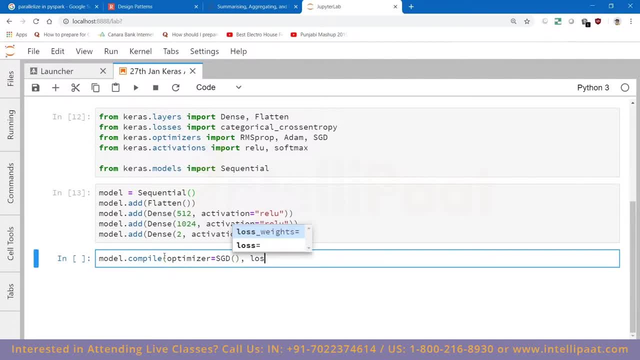 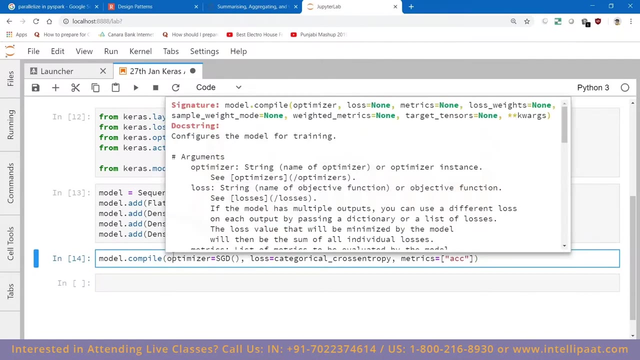 Right losses. may you have categorical cross entropy matrix. may you have accuracy, right. What else you can give here? Optimizer loss matrix, right? You've already given a lot of things. Then you say: model dot, now we do fit, right. 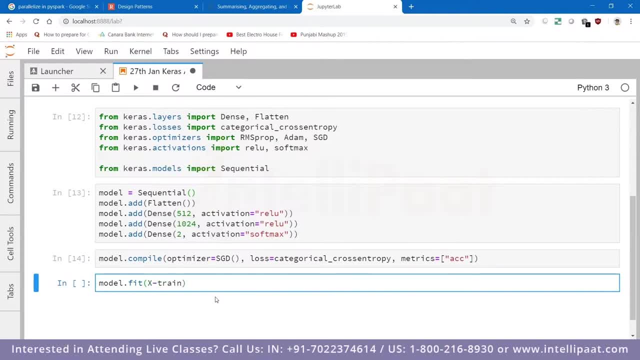 This is what we do. You give your X underscore train here and then comma Y underscore train here, But we don't have X and Y something here, right? So that's why we have to do a small change here. This is the change. 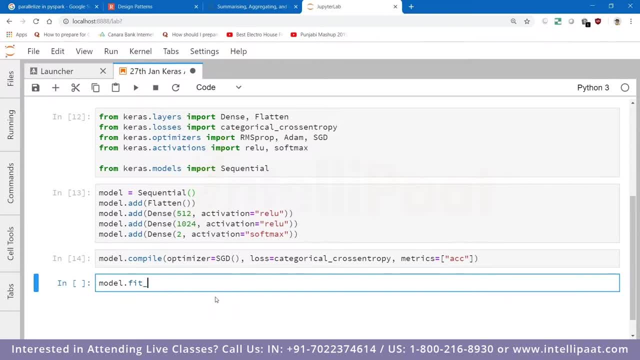 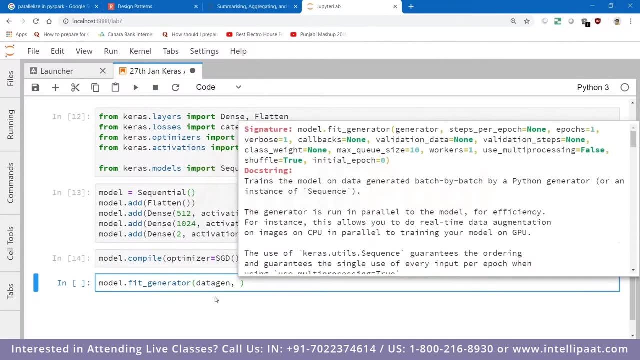 We will not use fit, We will use fit generator. Fit generator: you have to give it a generator. Your generator is data gen. Then whatever you can give is you can give. So you can give. how many steps do you want to go per epoch? 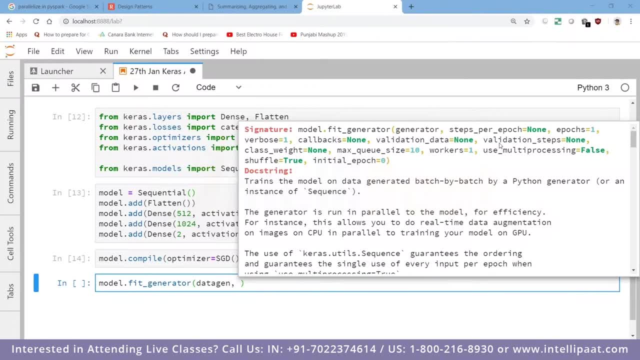 How many epochs do you want to go? Then, if you have any validation, validation steps, Then you have class rates And then don't use the workers as of now because you're not using GPU. So keep the use multiprocessing as false and workers as one only. 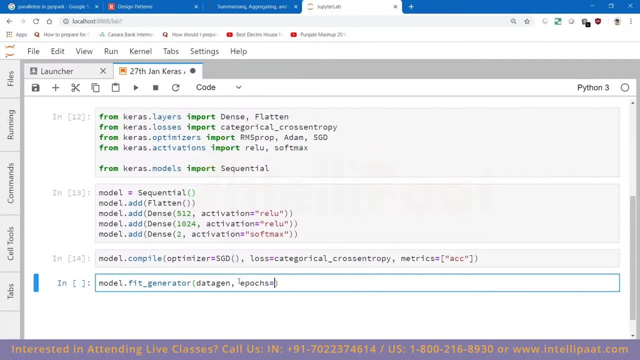 Don't do much changes, right? If you're on GPU, then you can do multiple things. Epochs, let's say 10, and let's start this. Okay, this GDN is giving hard times. What does it say? 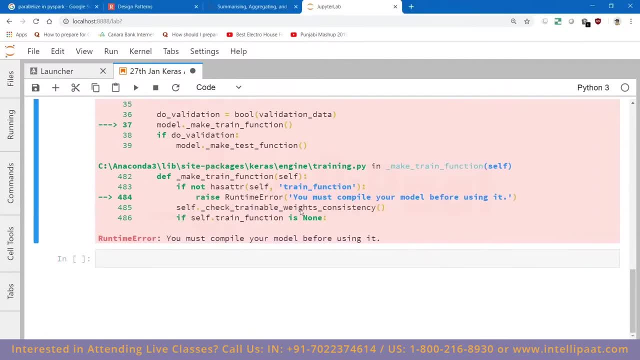 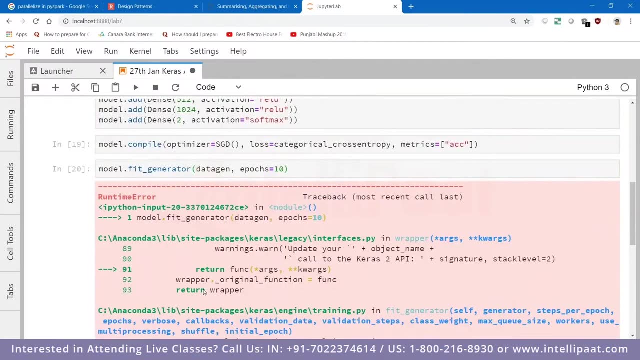 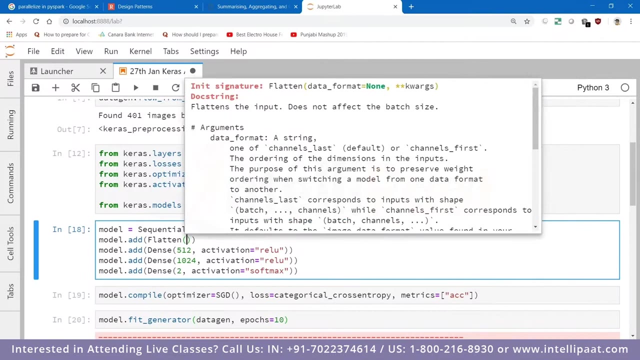 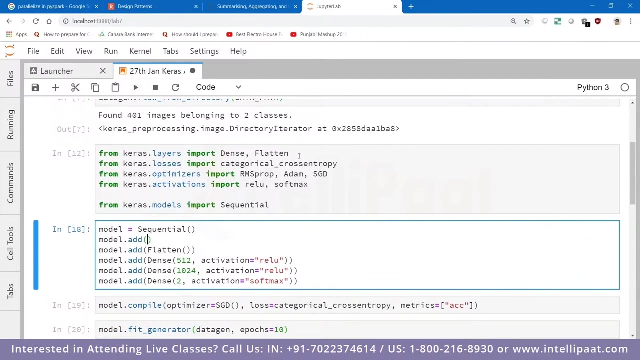 You must compile your model before using it. We have run this model dot compile. Okay, I got this issue. This issue is here, So this will take a input model dot add And then you have an input layer. Then you have an input layer. 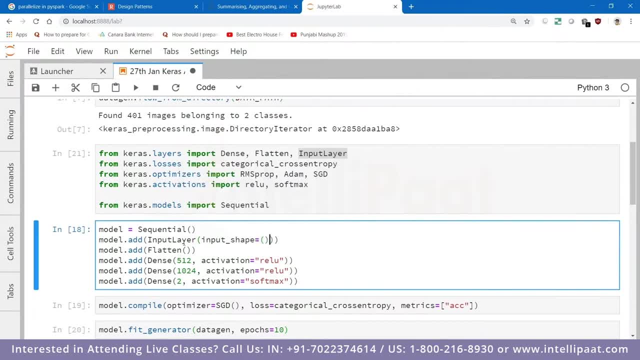 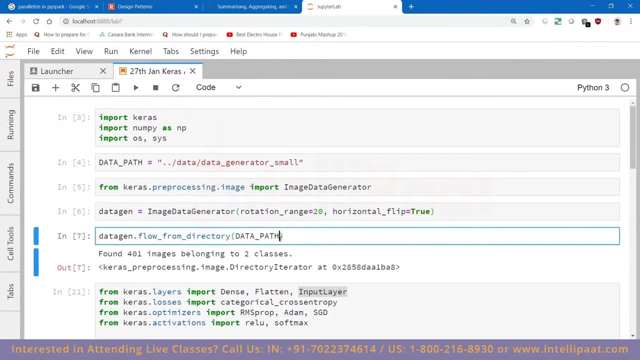 Input layer takes input shape as. So if you remember- okay, we didn't did one thing- You guys forget that we have to give it a shape also, right? So we have to give it a target shape also. Let's say, we convert it into 200 cross 200, right? 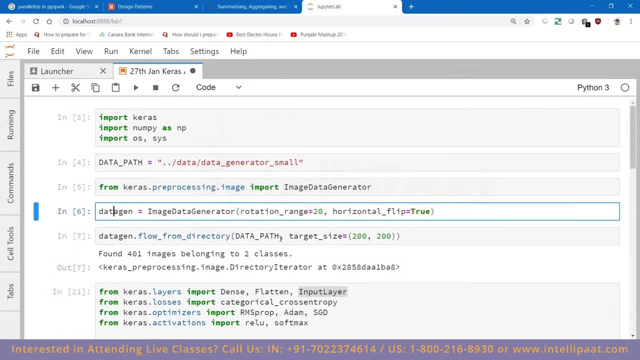 And then this is it for the upper part. Do we have something else that we're missing In validation split? let's do a validation split. Validation split of 0.2, right, Let's run everything again. Right, do this, do this. 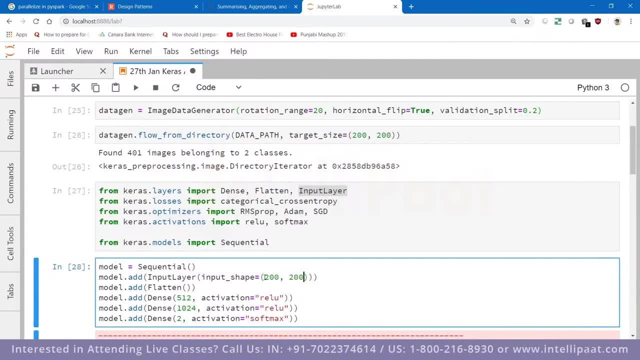 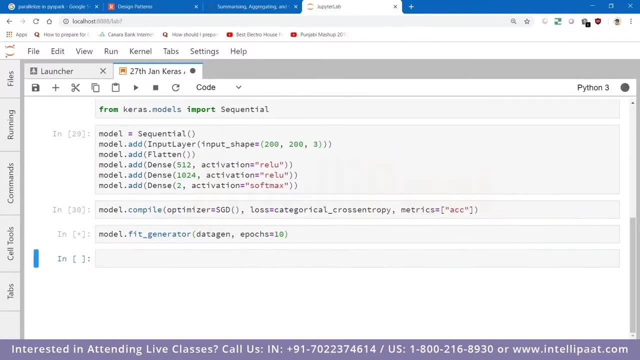 Okay, sorry, I have to fill in here 200 comma, 200 comma three. All right, now you do a compile and then you do a model dot fit. Okay, this time it's not working. Okay, so there are 10 epochs. 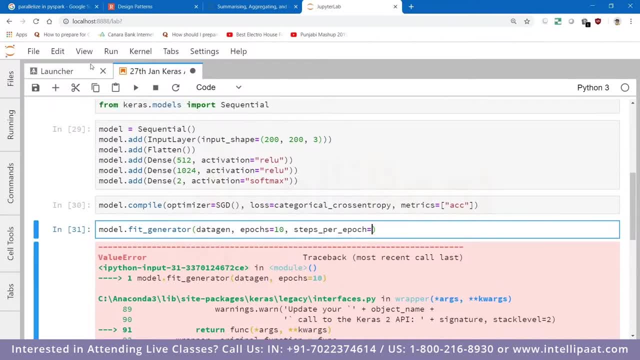 And then, how many steps do you want CC now? this is a very crucial question that it is asking. is now you understand this thing? what is a batch right? What is a epoch right? Sorry, first of all, epoch means that if you have, let's say here, 100 images, 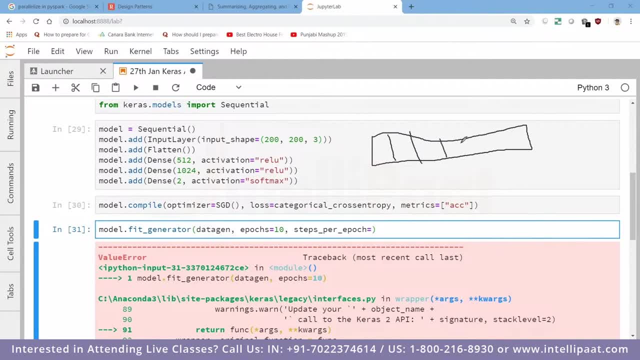 Then, once you complete all your batches, all your batches inside your total images, Once these, all, all the images, all your images, all your batches, the images have gone through the neural network funds in the forward and once in the backward right. this is called one epoch complete. now it's asking that in 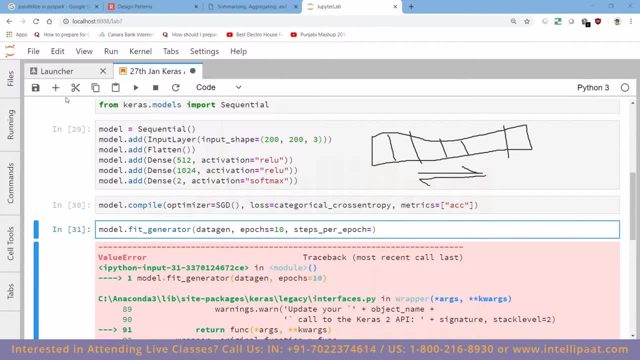 how many steps do you want to complete your epoch? right? so let's say that we want to complete in, like, let's say, three steps. right, because you have less data. three steps means that you want to perform your epoch into three cuts. so if you have total of hundred images, then 33 will go in first, 33 in second and 34 in. 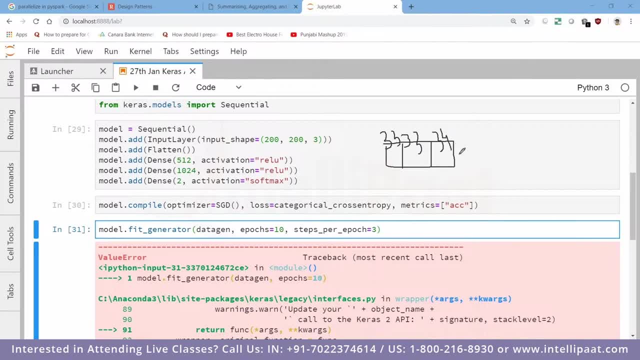 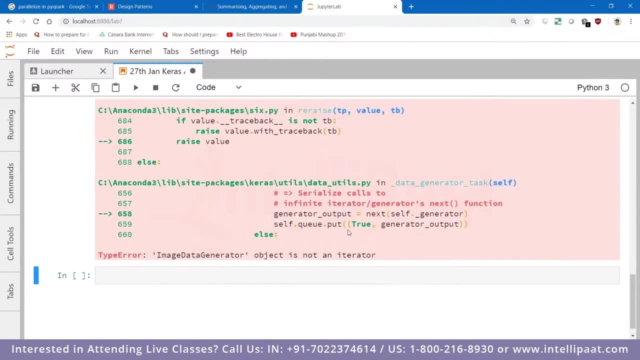 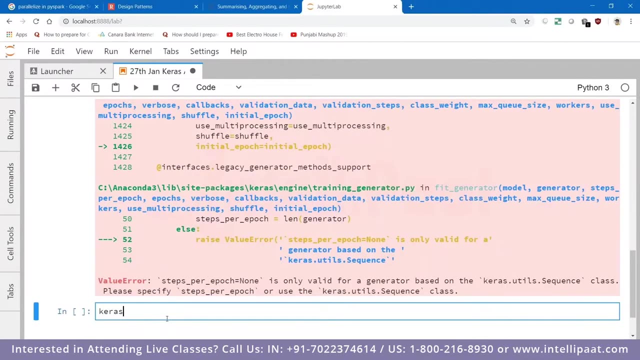 last. right, you get the concept of epochs and batches right. okay. now again it's saying something immediately, is not I disabled? okay, so, so gtm, please go for here. which version of Kiras am I using? one two point two: okay, this is one step ahead. okay, so my Kiras is a little. 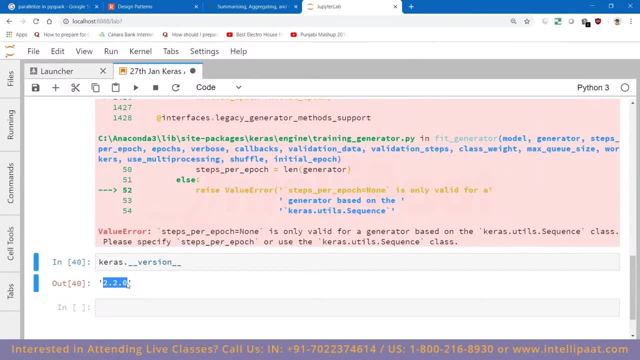 little step ahead. okay, so my Kiras is a little little step ahead. okay, so my Kiras is a little bit ahead of you guys. I think your would be Kiras one point two point. one. bit ahead of you guys. I think your would be Kiras one point two, point one. 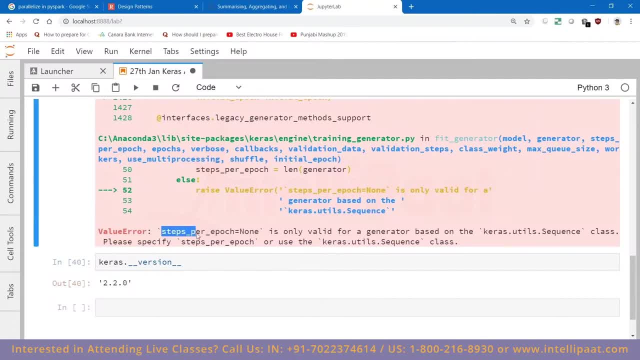 bit ahead of you guys, I think your would be Kiras. one point two point one. point four: mines is two point two point. oh so point four: mines is two point two point. oh so point four: mines is two point two point. oh so there might be something is give me. 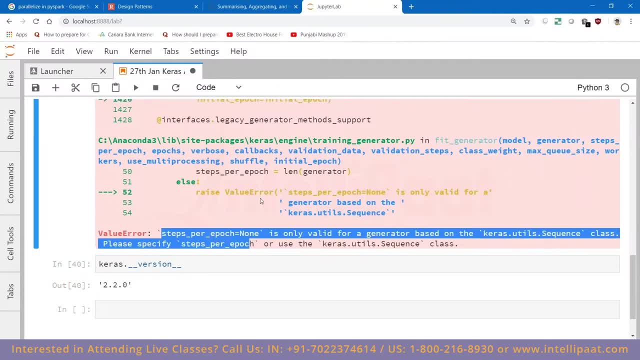 there might be something is: give me, there might be something is: give me just a second steps per epoch. none is not just a second steps per epoch. none is not just a second steps per epoch. none is not valid for generator type. you have to. valid for generator type, you have to. 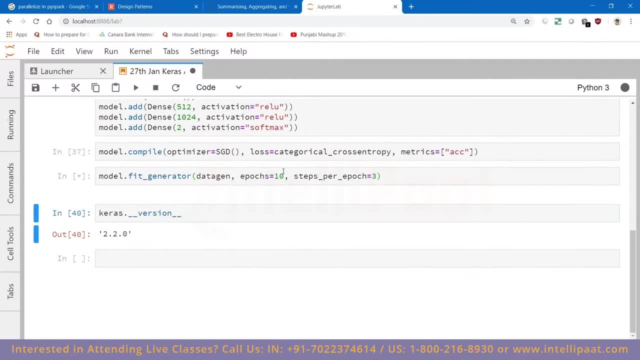 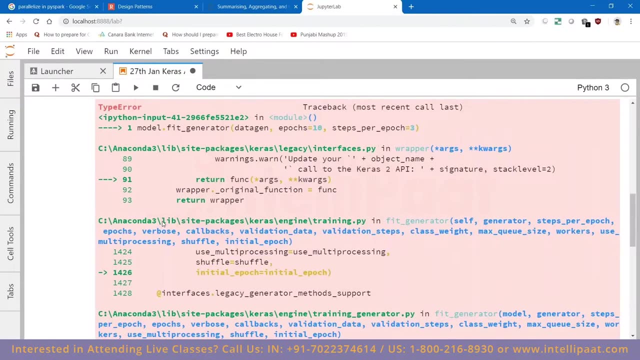 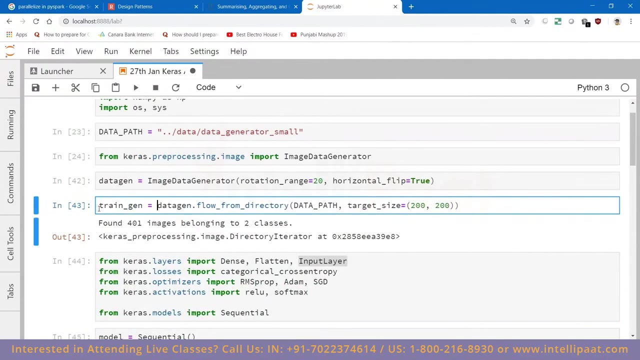 valid for generator type. you have to games and it says in which data games. and it says in which data games and it says in which data. generator object is not an iterator. why generator object is not an iterator. why generator object is not an iterator. why it's not an iterator now. 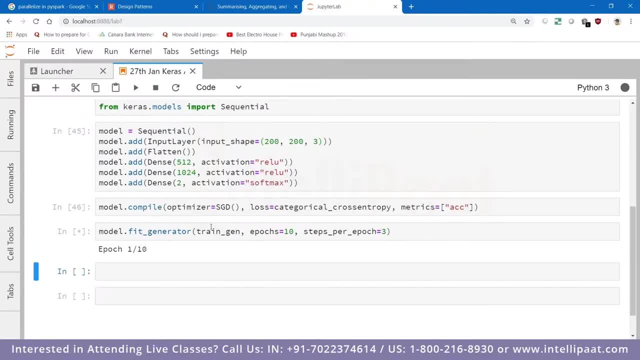 sorry my mistake, guys, so sorry okay. I sorry my mistake, guys, so sorry okay. I sorry my mistake, guys, so sorry okay. I was pushing this data generator object was pushing this data generator object was pushing this data generator object into that. you should let take the object into that. you should let take the object. 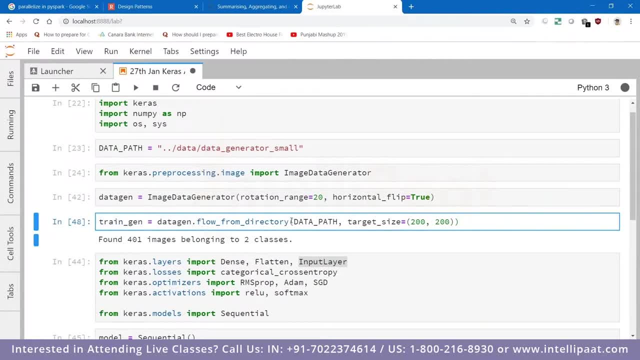 into that. you should let take the object out of this thing. you should take the out of this thing. you should take the out of this thing. you should take the return thing that is coming out and then return thing that is coming out, and then return thing that is coming out, and then you should use it. so this is going to 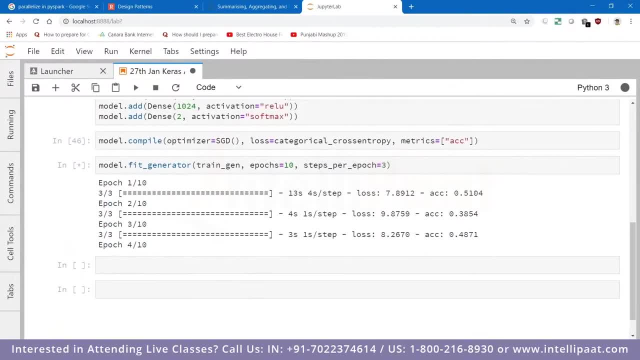 you should use it. so this is going to. you should use it. so this is going to run your model. you can see here your run your model. you can see here your run your model. you can see here your model is running. model is running. model is running. it will go till 3, 3 till 10 epochs and 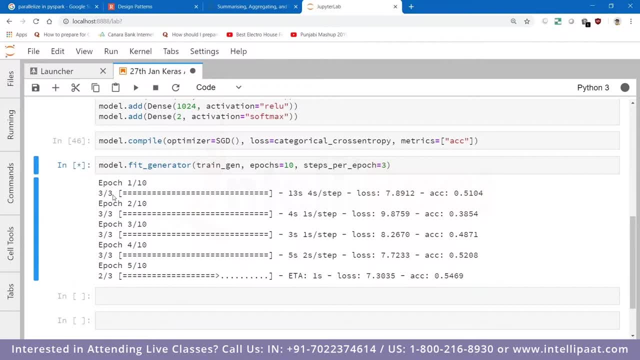 it will go till 3, 3 till 10 epochs and it will go till 3, 3 till 10 epochs. and you can see, here it is written 3 out of. you can see, here it is written 3 out of. you can see, here it is written 3 out of 3. it means that your one epoch is taking. 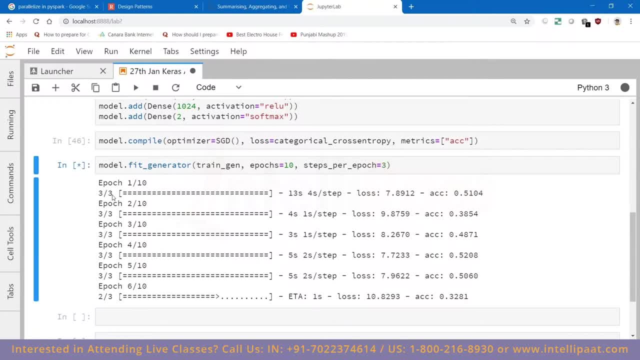 3. it means that your one epoch is taking 3. it means that your one epoch is taking 3 steps to complete one epoch now. if 3 steps to complete one epoch now. if 3 steps to complete one epoch now. if there are 401 images, how many images are? 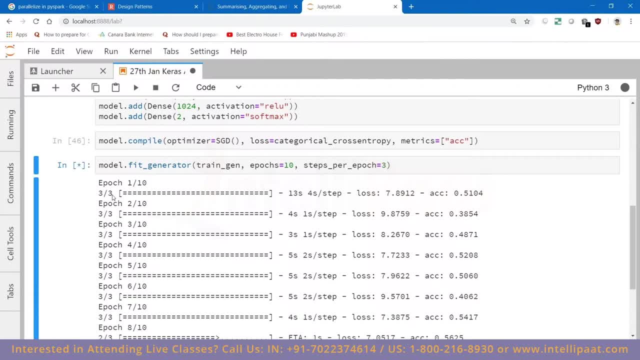 there are 401 images. how many images are? there are 401 images. how many images are going in one batch? going in one batch? going in one batch? 4 under divided by 3 right, these are a. 4 under divided by 3 right, these are a. 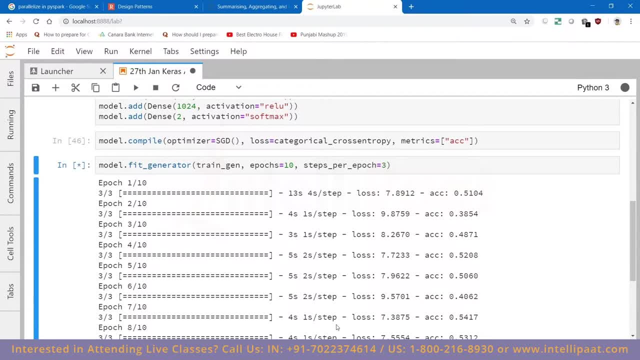 4, under divided by 3, right. these are a number of images that are going inside. number of images that are going inside. number of images that are going inside the model there is a. this is the only the model there is a. this is the only the model there is a. this is the only small change that you have to do. if you 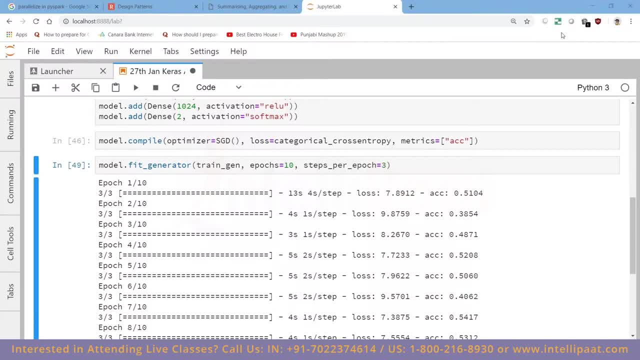 small change that you have to do, if you small change that you have to do, if you are doing, you're not doing the regular are doing. you're not doing the regular are doing. you're not doing the regular training rather than you are doing a training rather than you are doing a. 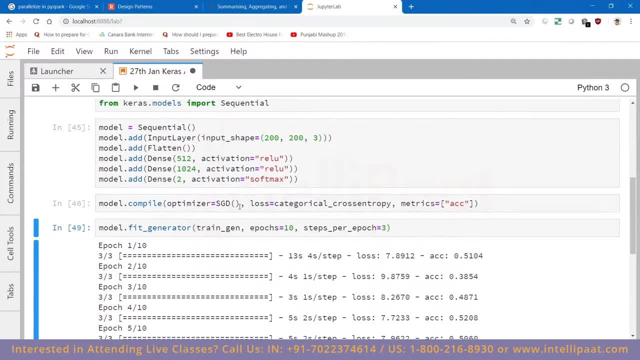 training rather than you are doing a batch training, right, okay, there is one batch training, right, okay, there is one batch training, right, okay. there is one more thing that I wanted to add. here is more thing that I wanted to add here is more thing that I wanted to add here is that there is this one step. it is called: 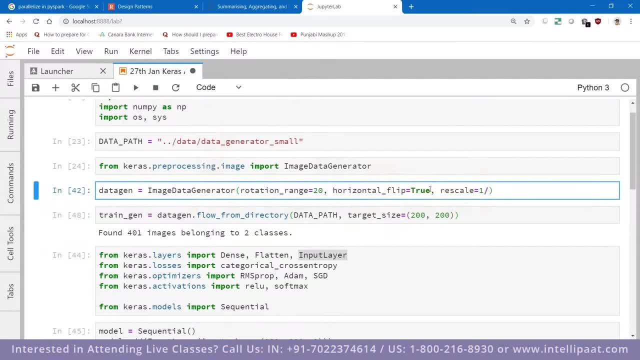 that there is this one step. it is called that there is this one step. it is called rescale now. rescale means that you want rescale now. rescale means that you want rescale now. rescale means that you want to divide your all the images with 0.25. 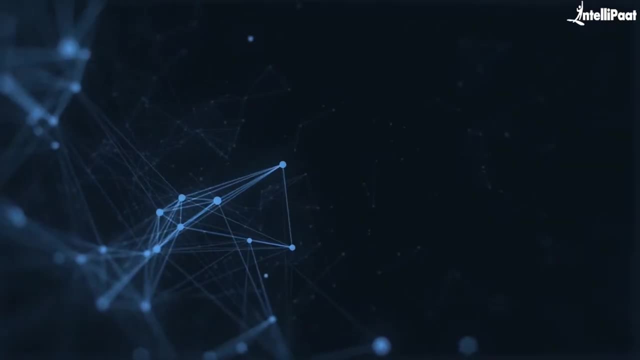 to divide your all the images with 0.25. to divide your all the images with 0.25- 5.0. why do we do this? just a quick info- 5.0. why do we do this? just a quick info, 5.0. why do we do this? just a quick info, guys. Intellipaat provides artificial 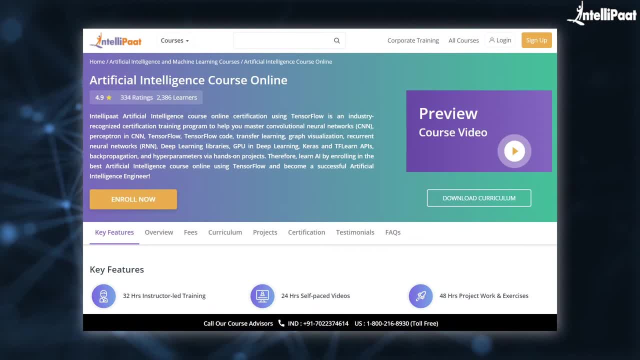 guys. Intellipaat provides artificial guys. Intellipaat provides artificial intelligence. online training mentored by intelligence. online training mentored by intelligence. online training mentored by industry experts. the course link of it industry experts, the course link of it industry experts, the course link of it, is given in the description below now, 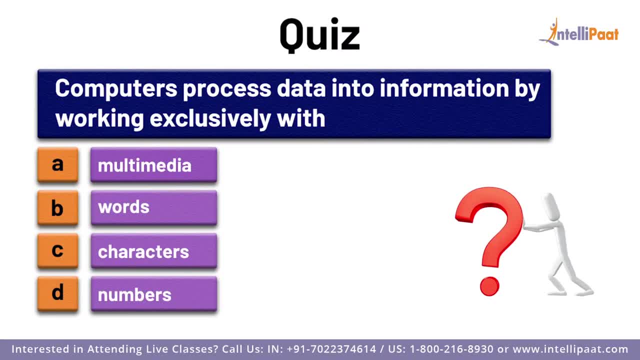 is given in the description below now is given in the description below. now let's continue with the session test. let's continue with the session test. let's continue with the session test: your knowledge of computer vision by your knowledge of computer vision. by your knowledge of computer vision by answering this question, computers process. 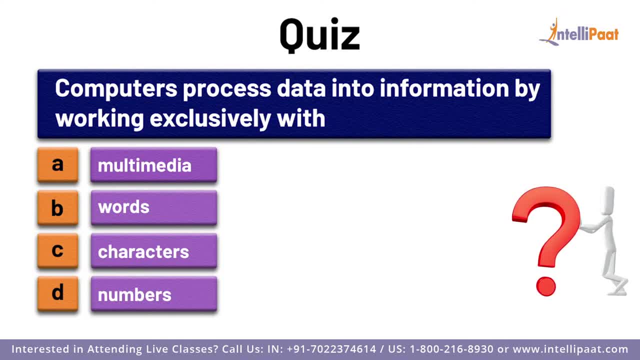 answering this question. computers process. answering this question. computers process: data into information by working data into information by working data into information by working exclusively with which of the following: a exclusively with which of the following: a exclusively with which of the following: a multimedia B words, C characters, D numbers. 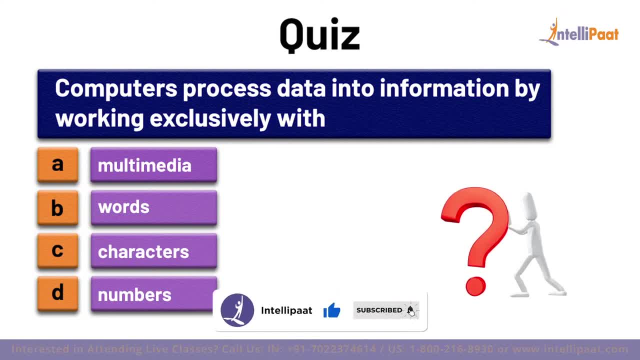 multimedia B words C characters D numbers. multimedia B words C, characters D numbers. comment. your answer in the comment comment. your answer in the comment comment. your answer in the comment section below: subscribe to Intellipaat to section below. subscribe to Intellipaat to section below. subscribe to Intellipaat. to know the right answer. now let's continue. 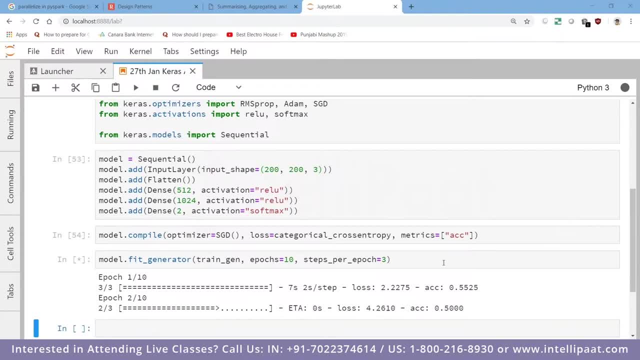 know the right answer now. let's continue. know the right answer now. let's continue with the session. this is actually with the session. this is actually with the session. this is actually normalization. if you remember, this is normalization. if you remember, this is normalization. if you remember, this is normalization of the model images that 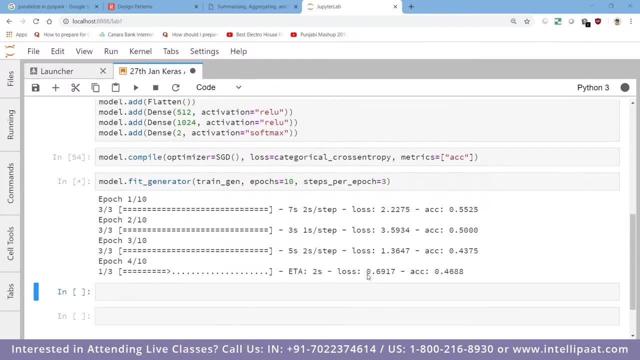 normalization of the model images, that normalization of the model images, that their image, the model should not look their image, the model should not look their image, the model should not look like that. there are some small images like that. there are some small images like that. there are some small images that are called zero. and then there are 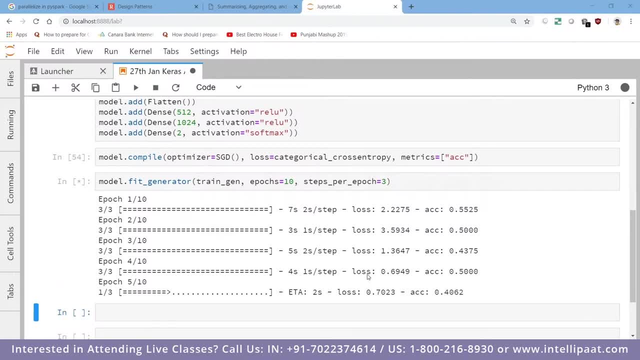 that are called zero, and then there are that are called zero, and then there are some big images called 255. so we some big images called 255, so we some big images called 255. so we normalize the data, we squeeze the data. normalize the data, we squeeze the data. 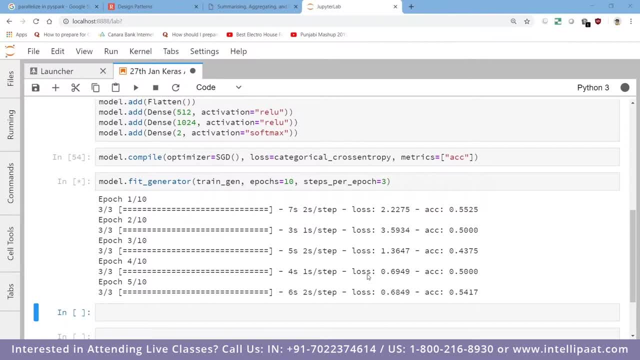 normalize the data. we squeeze the data between some range of 0 to 1, and how do? between some range of 0 to 1 and how do between some range of 0 to 1, and how do we do that? we do that. we do that. there are multiple ways of doing this. 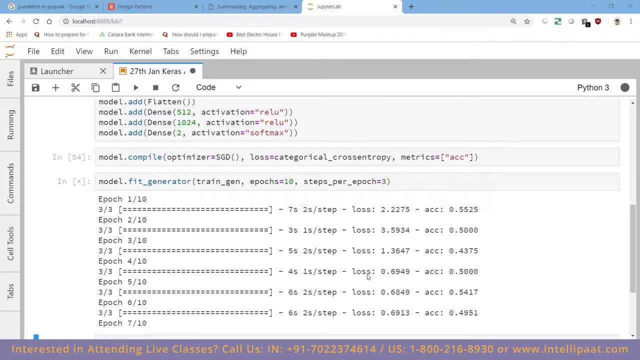 there are multiple ways of doing this. there are multiple ways of doing this: standard scalar- min max or scalar. and standard scalar- min max or scalar. and standard scalar- min max or scalar. and this was the min max scalar where you. this was the min max scalar where you. 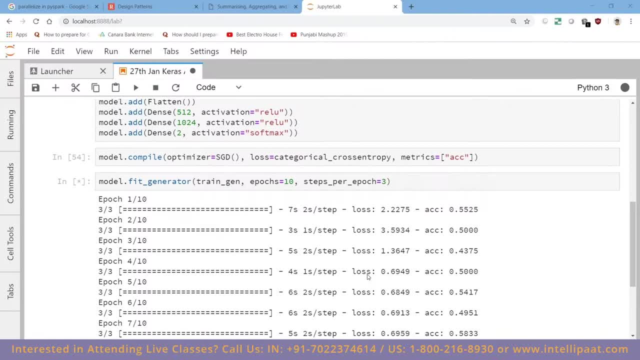 this was the min max scalar, where you divide your data with the largest pixel, divide your data with the largest pixel, divide your data with the largest pixel value the largest pixel where that can value. the largest pixel where that can value. the largest pixel where that can come is 255, so you divide all your data. 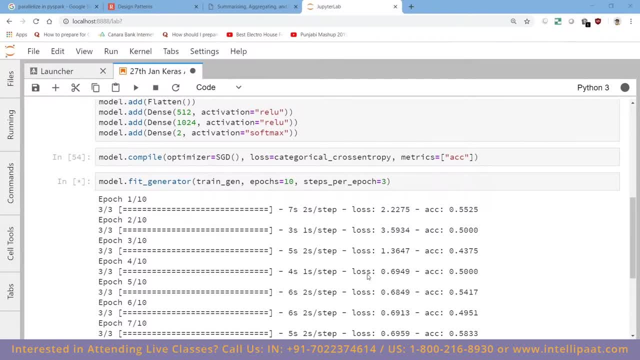 come is 255, so you divide all your data. come is 255, so you divide all your data with 255, and then you get your ranges with 255, and then you get your ranges with 255, and then you get your ranges from 0 to 1. right, correct, make sense. so 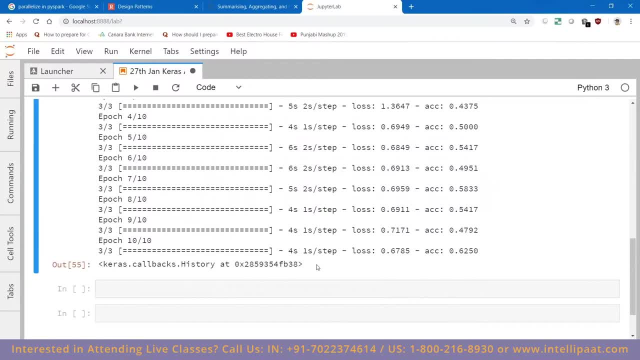 from 0 to 1 right- correct make sense. so from 0 to 1 right- correct make sense. so this was a. this was a small example this. this was a. this was a small example this. this was a. this was a small example. this was showing you that. how do you connect? 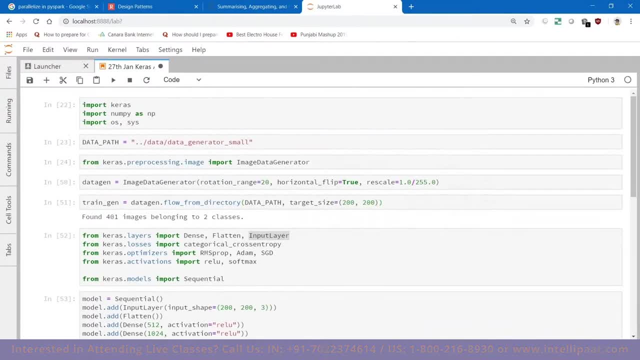 was showing you that. how do you connect? was showing you that how do you connect your augmented data inside your, inside your augmented data inside your, inside your augmented data inside your, inside your model right? this was all the step, your model right. this was all the step. your model right. this was all the step. so let's move to the next section of 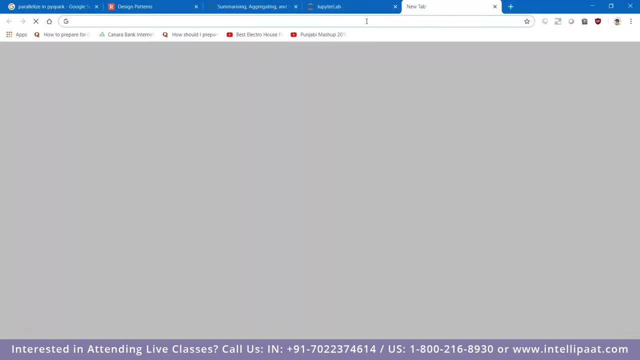 so let's move to the next section of. so let's move to the next section of this thing that is called the cnn's, this thing that is called the cnn's, this thing that is called the cnn's. now, cnn's are actually a new kind of a. 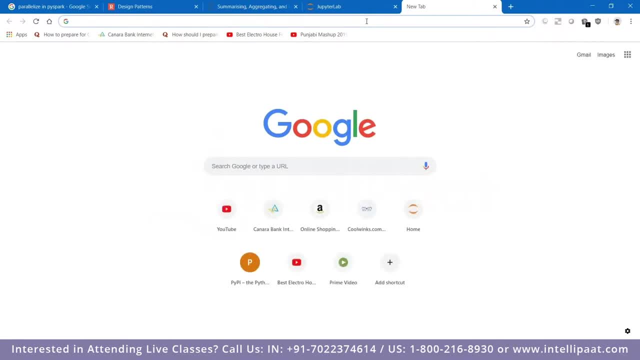 now cnn's are actually a new kind of a. now, cnn's are actually a new kind of a, not a new, but they are one of the most- not a new, but they are one of the most- not a new, but they are one of the most fascinating kind of architecture that you. 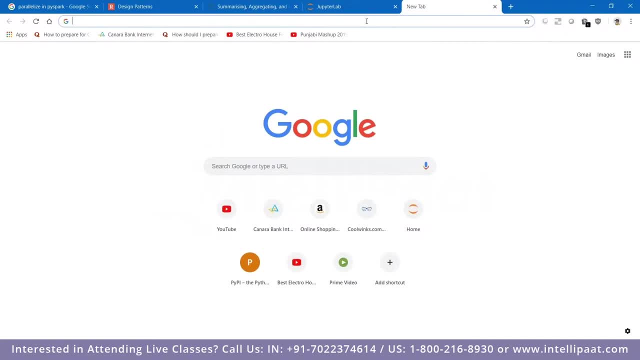 fascinating kind of architecture that you fascinating kind of architecture that you will ever learn in deep learning, will ever learn in deep learning, will ever learn in deep learning, especially in images. so till now, what, especially in images? so till now what, especially in images? so till now, what we have done is we have just seen that 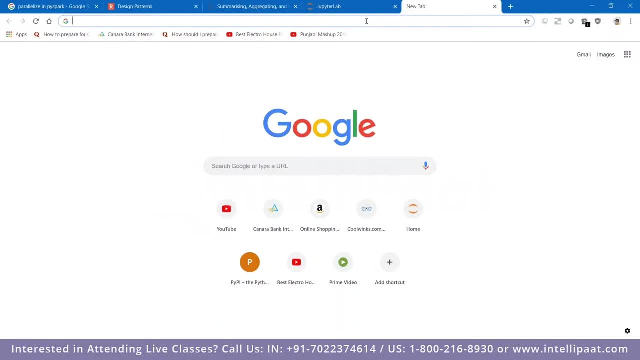 we have done is we have just seen that we have done is we have just seen that, okay, we are connecting some neurons to. okay, we are connecting some neurons to. okay, we are connecting some neurons to other neurons and other neurons to other other neurons and other neurons to other. 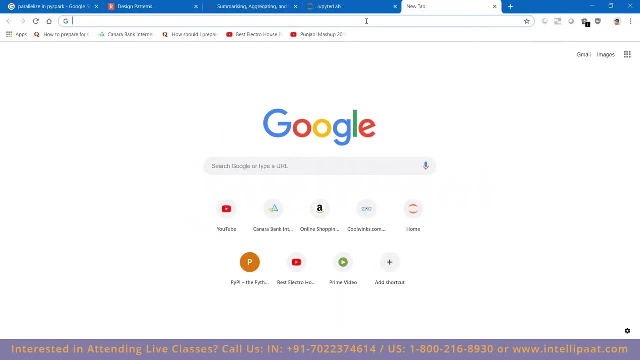 other neurons and other neurons to other neurons, and this is something the neurons and this is something the neurons and this is something the information is getting passed. and if you information is getting passed, and if you information is getting passed, and if you remember the maths behind this that we 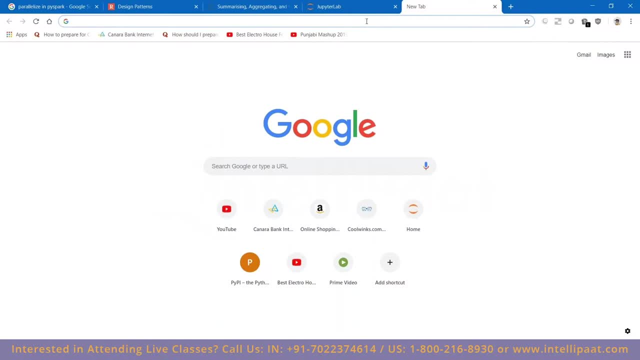 remember the maths behind this, that we remember the maths behind this. that we are just doing a fine, then we do. some are just doing a fine, then we do. some are just doing a fine, then we do some activation function. it means that we are activation function. it means that we are. 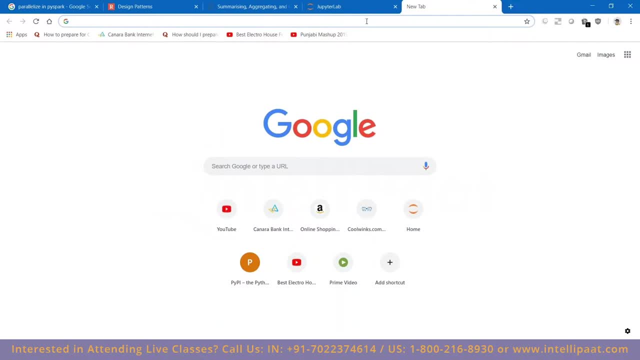 activation function. it means that we are bringing some non-linearity in the data, bringing some non-linearity in the data, bringing some non-linearity in the data, and then we are passing it through some, and then we are passing it through some, and then we are passing it through some activation function and then we are. 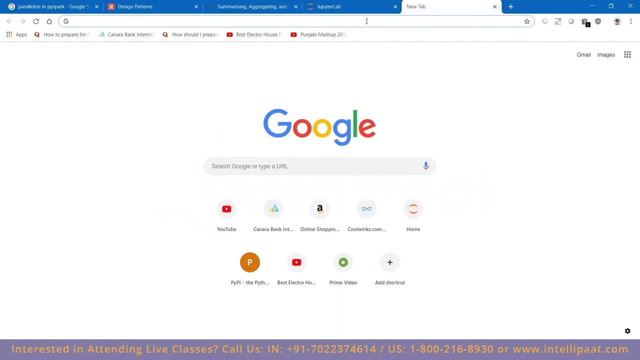 activation function, and then we are activation function, and then we are finally giving it to the next layer, finally giving it to the next layer, finally giving it to the next layer, and then the, and then this chain is going, and then the, and then this chain is going. 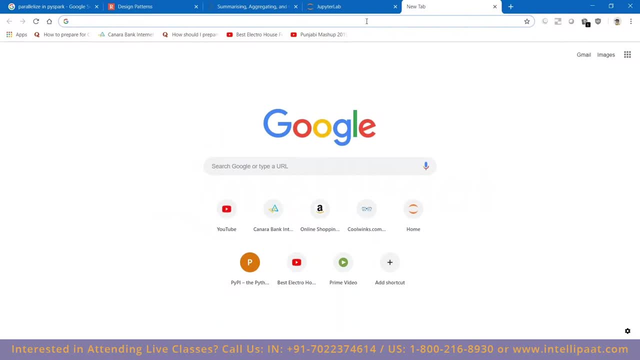 and then the, and then this chain is going on on on. things are coming in, going out, coming. things are coming in, going out, coming. things are coming in, going out, coming in, going out right in going out, coming in, going out right in going out, coming in, going out right. but how is this? how is this network? 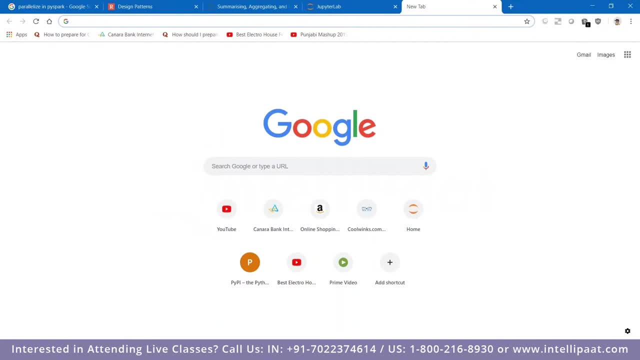 but how is this? how is this network? but how is this? how is this network helping the helping the helping the? how is this network helping the model to? how is this network helping the model to? how is this network helping the model to learn the key features? learn the key features. 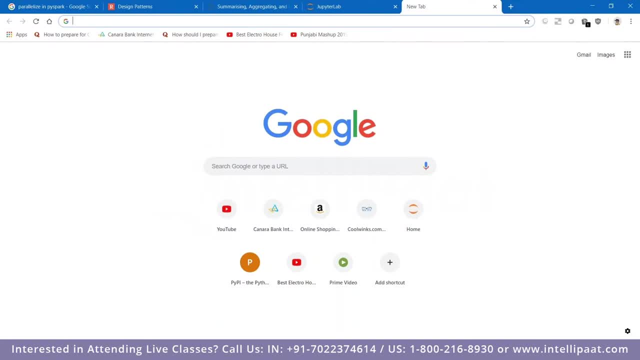 learn the key features right. so today we learn this new and right. so today we learn this new and right. so today we learn this new and very interesting, very interesting, very interesting. uh, neural network architecture is uh, neural network architecture is. uh. neural network architecture is called cnn, cnn, or commonly known as the 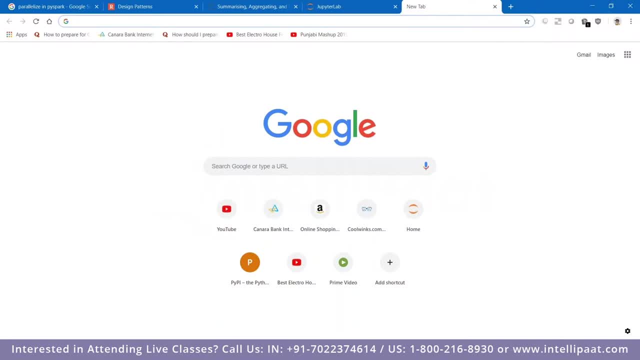 called cnn, cnn, or commonly known as the called cnn, cnn, or commonly known as the convolution neural network, convolution, neural network, convolution, neural network, so convolutional network. what will it? so convolutional network, what will it? so convolutional network? what will it will do? is? it is somewhat like uh. 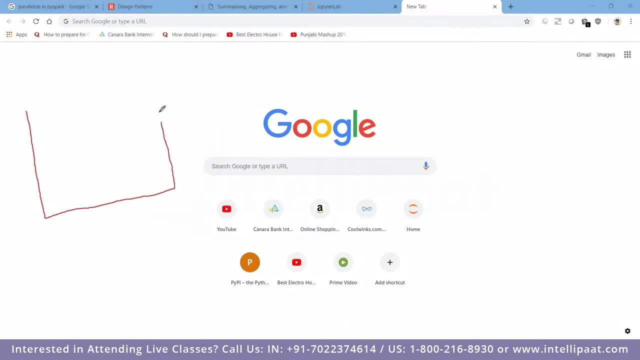 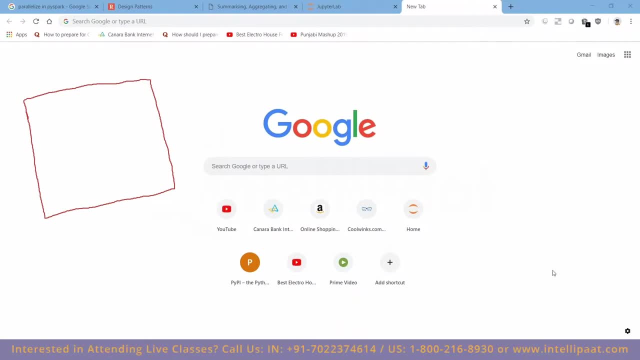 original image. original image then to find out the features inside it. then to find out the features inside it. then to find out the features inside it: cube, cube, cube, cube or square? sorry, not cube, cube or square, sorry, not cube, cube or square, sorry, not cube. you will take a, a small. 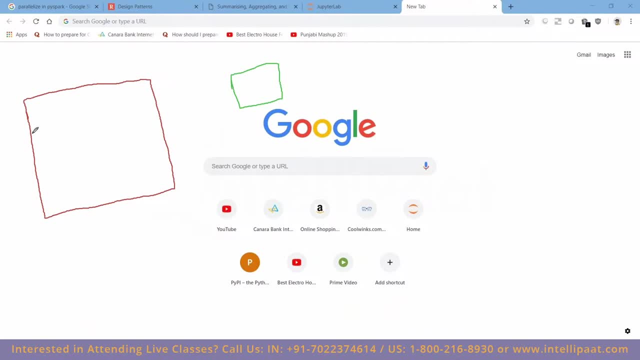 you will take a, a small. you will take a a small square green square, and then you'll apply square green square, and then you'll apply square green square, and then you'll apply this: you'll put this green, this, you'll put this green, this, you'll put this green here on the top. so it will somewhat cover. 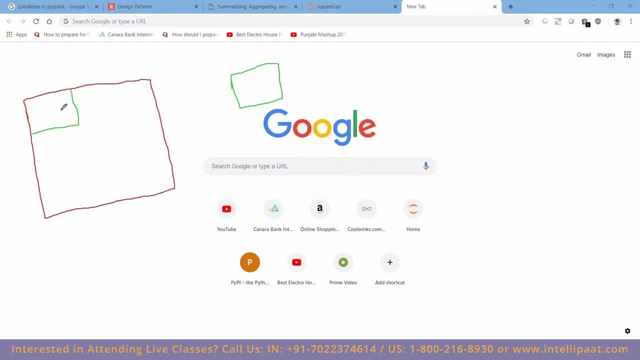 here on the top, so it will somewhat cover here on the top, so it will somewhat cover: like this right, like this right, like this right, then you will move this green spot to, then you will move this green spot to, then you will move this green spot to your right. 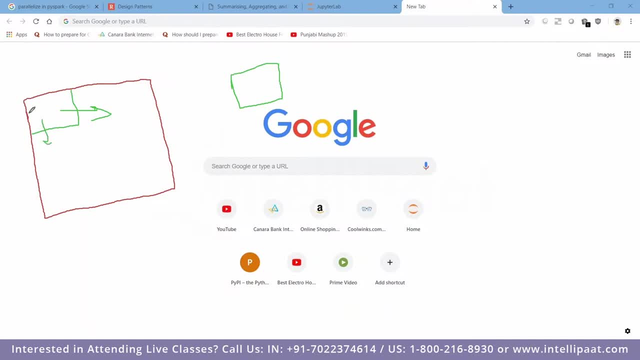 right, then one step down right, then one step down right, then one step down. so it will, so it will, so it will. it will come like this: again right, then one step down, then again right, then one step down, again right, and then one step down. eventually, this, this small, this small. 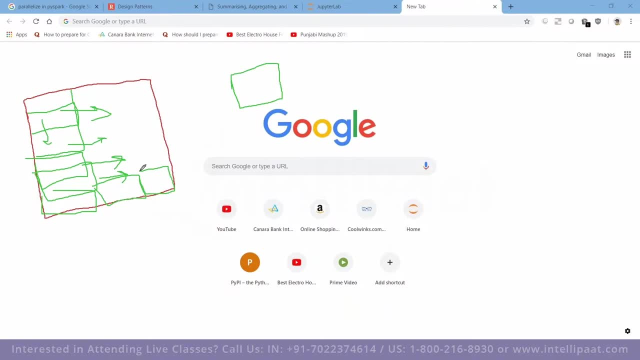 eventually this, this small, this small, eventually this, this small, this small, small image, or we call it as filter- small image, or we call it as filter small image, or we call it as filter- will like run over this whole image and will like run over this whole image and 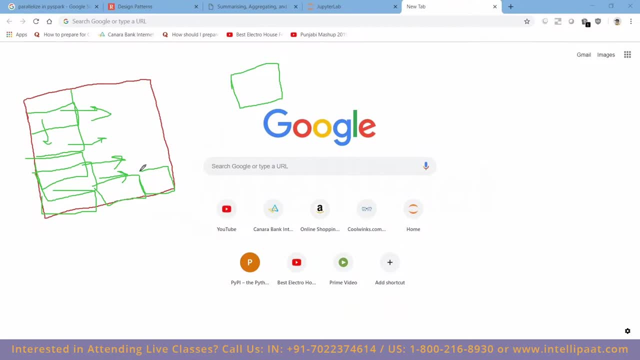 will like run over this whole image and it will learn the important features and it will learn the important features and it will learn the important features and the aspects of the, the aspects of the, the aspects of the of the image right now. how does this? of the image right now, how does this? 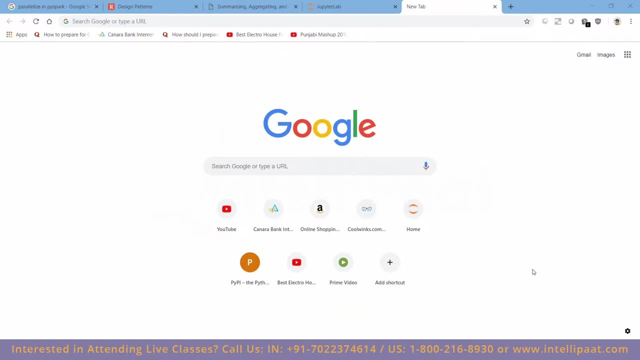 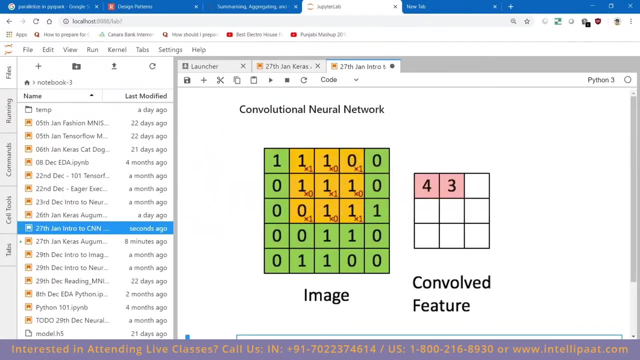 of the image right now. how does this is done? i'll show you a very intuitive is done. i'll show you a very intuitive is done. i'll show you a very intuitive. let me make a new jupiter notebook. see, this is somewhat what is happening. see, this is somewhat what is happening. 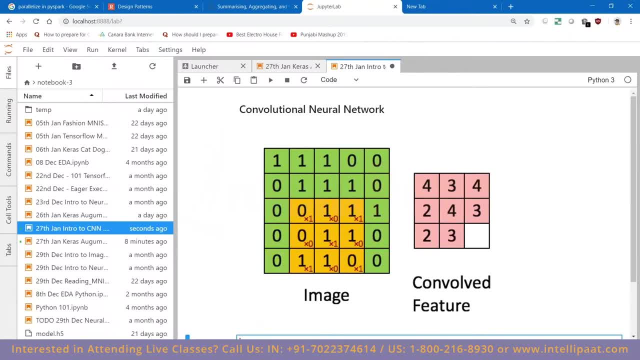 see, this is somewhat what is happening inside, here, inside, here, inside, here. so this green image that you are seeing, so this green image that you are seeing, so this green image that you are seeing right now, this is the big image right now. this is the big image. 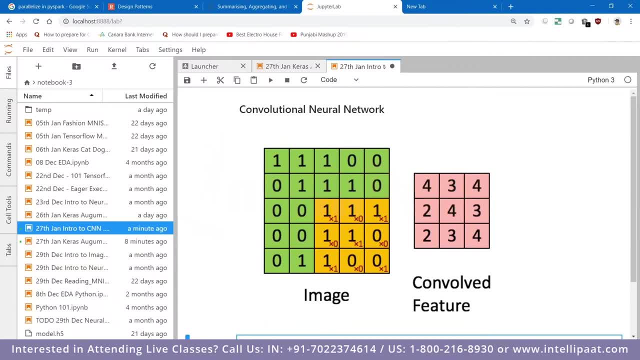 right now. this is the big image and the orange image that is moving is, and the orange image that is moving is, and the orange image that is moving is called the filter, called the filter, called the filter. so what you are doing is you are moving. so what you are doing is you are moving the filter on the image, one by one. 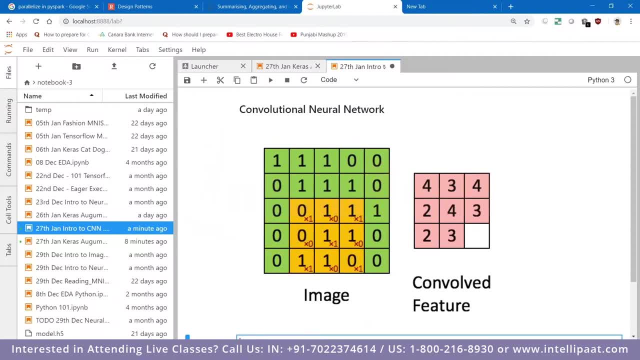 the filter on the image one by one. the filter on the image one by one. you're moving the filter by one by one. you're moving the filter by one by one. you're moving the filter by one by one. now, when i say when you are moving this, 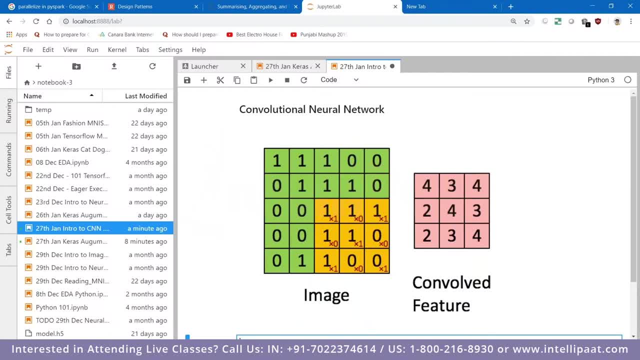 now, when i say when you are moving this, now, when i say when you are moving this, filter on the original image, what i mean filter on the original image. what i mean filter on the original image. what i mean is that you are doing a, is that you are doing a? 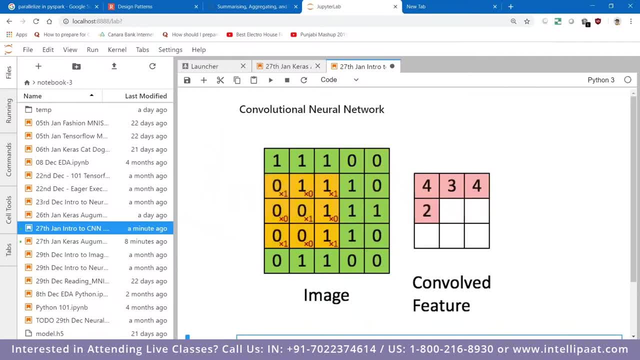 is that you are doing a element wise multiplication on this element, wise multiplication on this element, wise multiplication on this image, image, image, and then you are, and then you are, and then you are summing up all the things. so if i stop summing up all the things, so if i stop, 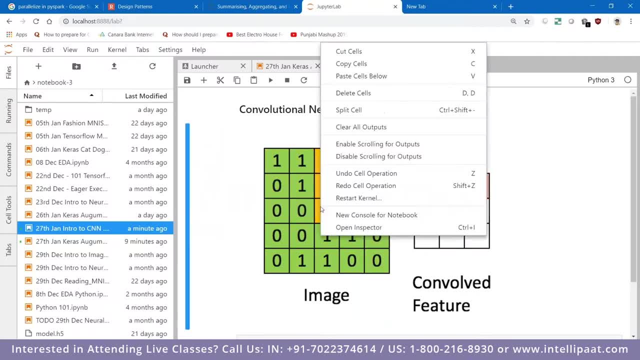 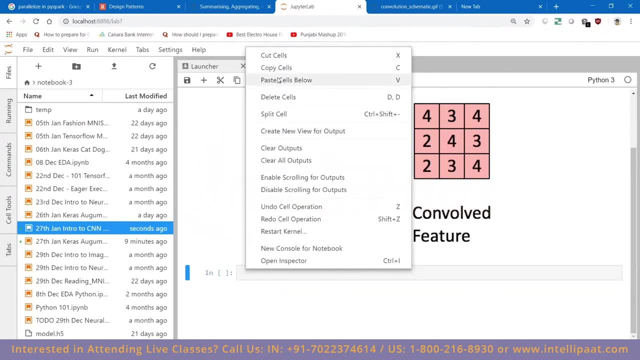 summing up all the things. so if i stop this thing here, this thing here, this thing here, okay, it doesn't stop. okay, it doesn't stop. okay, it doesn't stop. okay, if i put it here: cool, i have this picture already with me. cool, i have this picture already with me. 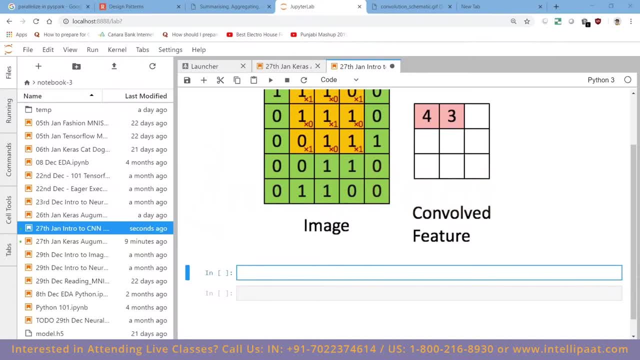 cool, i have this picture already with me: ctrl c, ctrl c, ctrl c. okay, so img src. okay, so img src. okay, so img src refer to: okay, see this image right now. right, you okay, see this image right now. right, you okay, see this image right now. right, you can see this image right now in front. 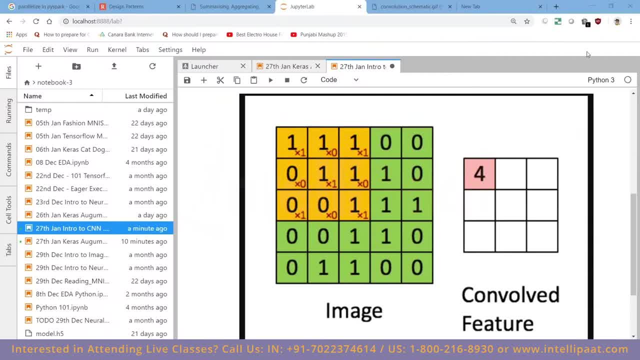 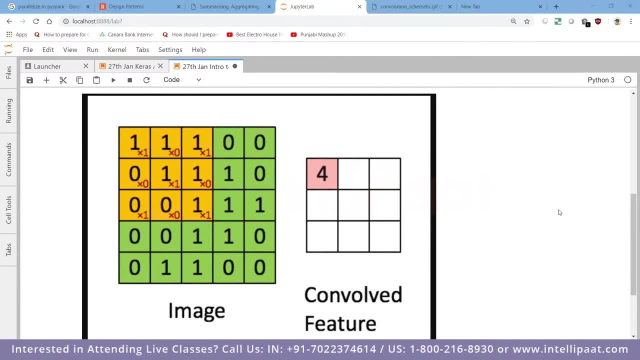 okay, so this green thing, this green, okay, so this green thing, this green image, and whatever this, this big thing image and whatever this, this big thing image and whatever this. this big thing is written here, these big numbers. one is written here, these big numbers, one is written here, these big numbers, one, one, z one, one one zero, zero, zero one. 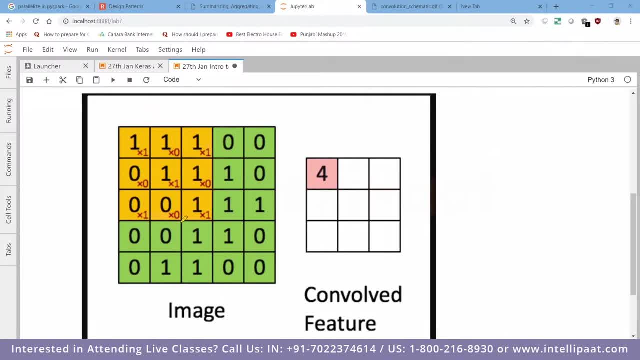 one z one one one zero, zero one one z one one one zero, zero, zero one one one, one one one zero, zero, zero one one one one one one zero, zero, zero one one. all these big numbers are what these are. all these big numbers are what these are. 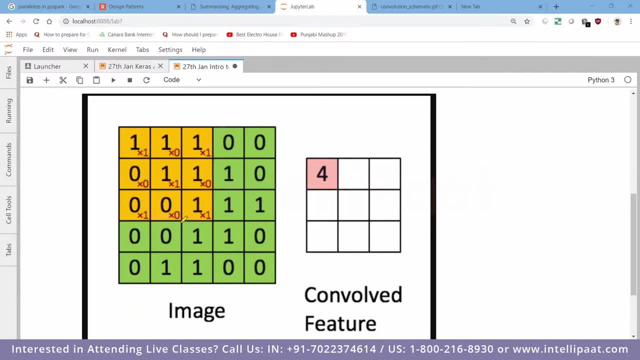 all these big numbers are what these are. let's say the pixel coordinates of the, let's say the pixel coordinates of the. let's say the pixel coordinates of the big image or the original image right big image, or the original image right big image, or the original image right. and then 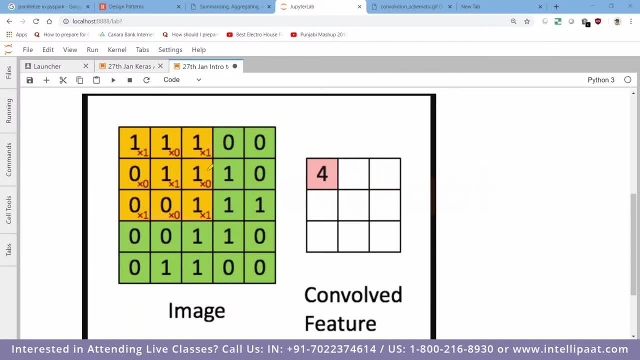 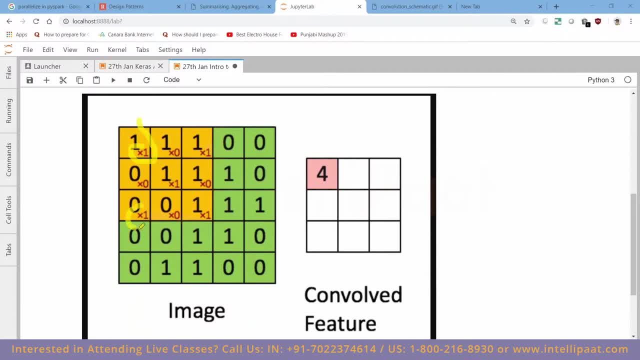 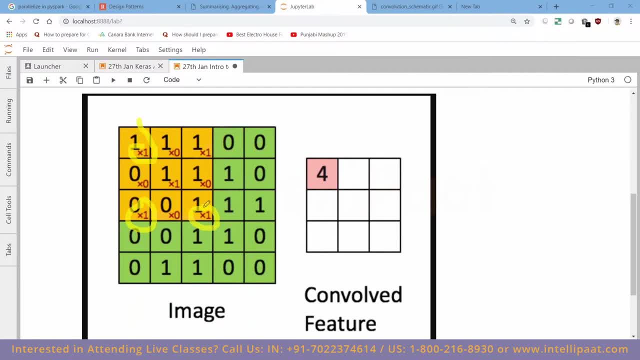 one one. these small numbers are the filter: filter, filter. these are the. these are the numbers for. these are the. these are the numbers for these are the. these are the numbers for the filter that is going to move over the, the filter that is going to move over the. 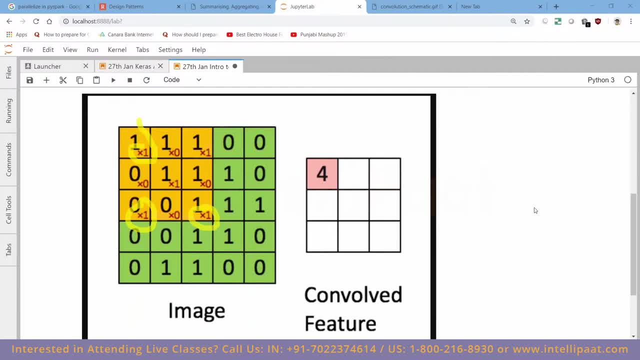 the filter that is going to move over the image right image, right image. right now, when this, when this thing is moving now, when this, when this thing is moving now, when this, when this thing is moving over this thing, it is doing a element. over this thing, it is doing a element. 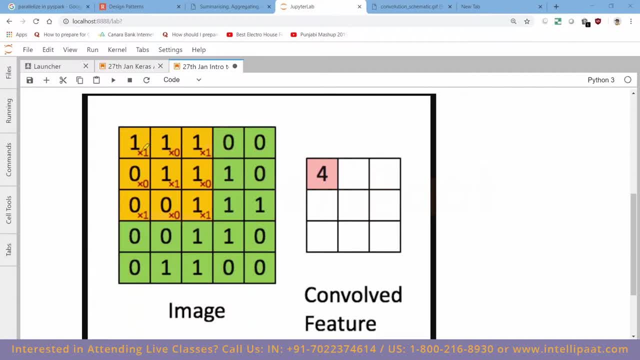 over this thing. it is doing a element wise, wise, wise, or you can say a scalar multiplication, or you can say a scalar multiplication, or you can say a scalar multiplication. element wise, one by one multiplication. element wise, one by one multiplication. element wise, one by one. multiplication means that this one is multiplied by one. 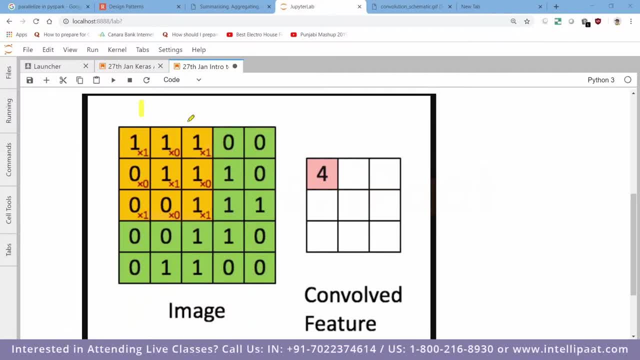 means that this one is multiplied by one. means that this one is multiplied by one called one, called one. called one. one multiplied by zero is zero. one plus one multiplied by zero is zero. one plus one multiplied by zero is zero. one plus one is one. one is one. 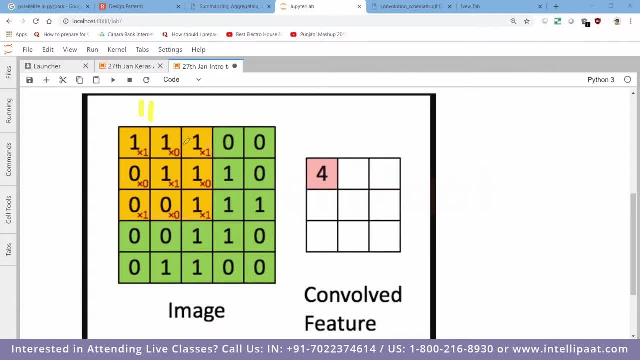 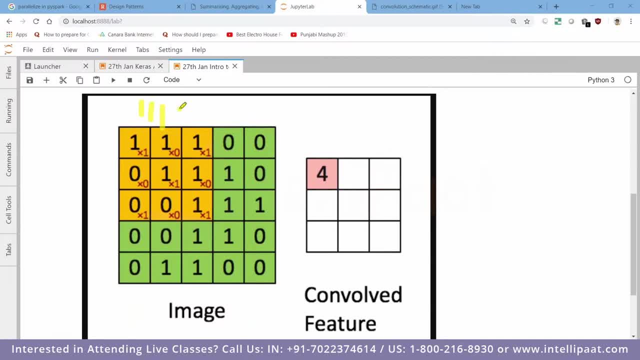 one plus zero is zero. zero plus one, zero plus one, and then one is two. one plus one, and then one is two. one plus one, and then one is two, one right. and then you have one more, so right. and then you have one more, so right, and then you have one more. so all these numbers, 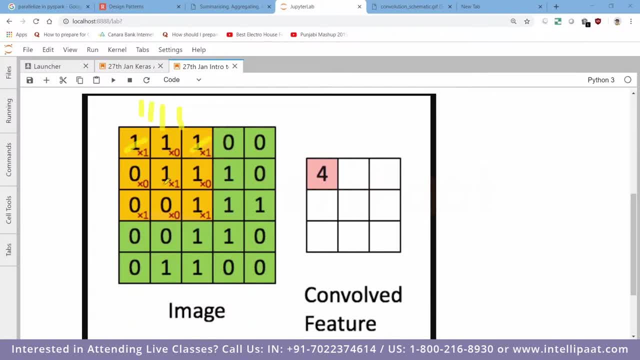 all these numbers, all these numbers: first for this one, second for this one, first for this one, second for this one, first for this one, second for this one, third for this one, third for this one, third for this one and fourth for this one and fourth for this one. 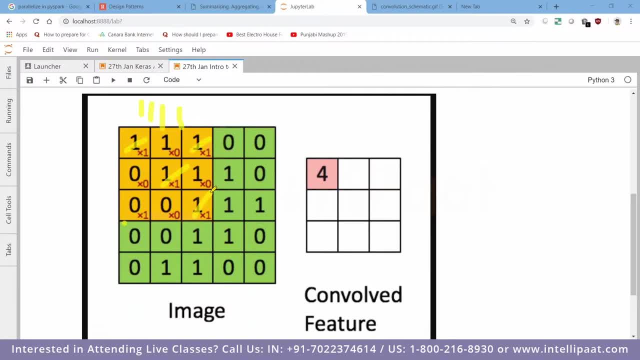 and fourth for this one, sorry this one, sorry this one, sorry this one. so these, these four, this number becomes so, these, these four, this number becomes so, these, these four, this number becomes four, and you write here four, and you write here four, and you write here four. similarly, what you'll do is you will 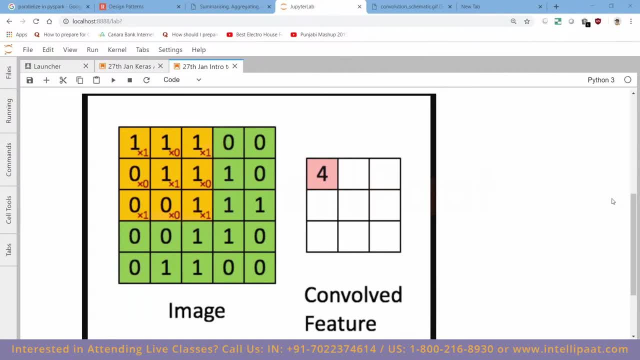 four. similarly, what you'll do is: you will four. similarly, what you'll do is you will shift the now shift the now shift the now this filter to to a little bit of your this filter, to to a little bit of your this filter, to to a little bit of your right. right, then you'll have a second. 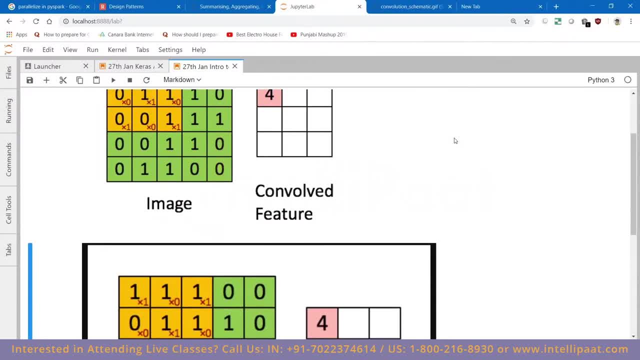 right right, then you'll have a second right right, then you'll have a second one, one one. if you move it to a little low, then it. if you move it to a little low, then it. if you move it to a little low, then it becomes your see. 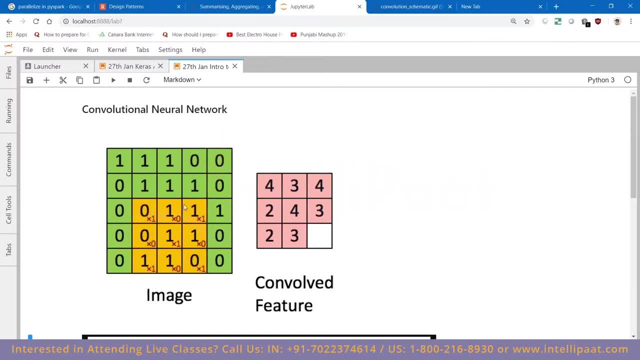 becomes your see, becomes your see. low and down. it becomes two, three, four. low and down, it becomes two, three, four, then four. two, three, four, then four. two, three, four, then four. two, three, four. this is how your convi convoluted. this is how your convi convoluted. 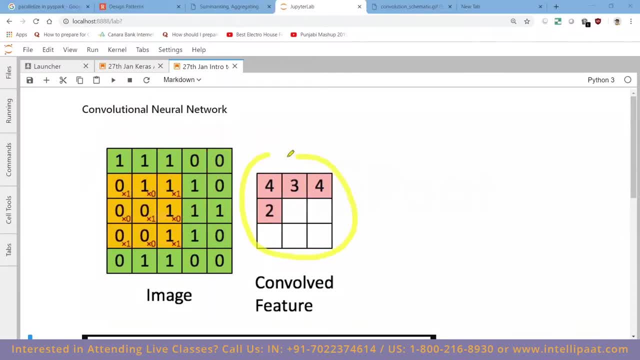 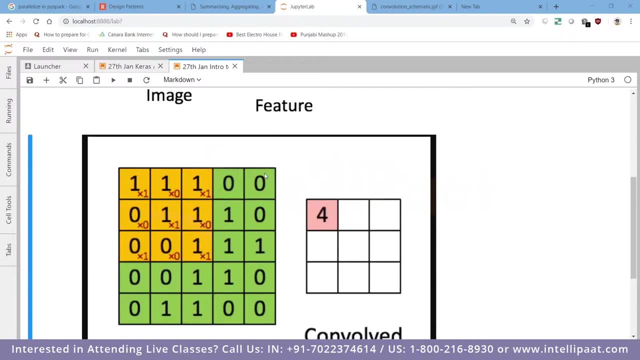 this is how your convi, convoluted filters, filters, filters, a features are calculated. everybody gets the idea, so now do you. everybody gets the idea. so now do you. everybody gets the idea. so now do you get the idea. get the idea, get the idea how this thing is coming. if you see this. 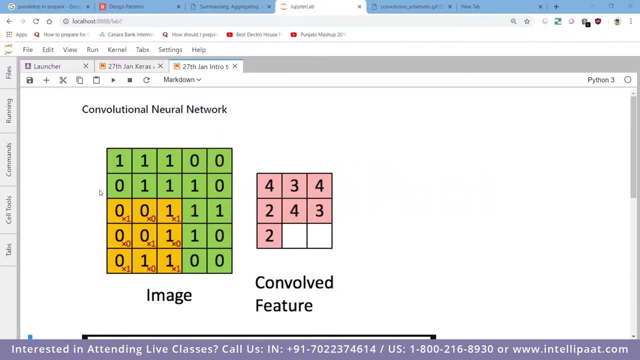 how this thing is coming if you see this, how this thing is coming if you see this. gif a little more. uh, once take your time, imagine how this. once take your time, imagine how this. once take your time, imagine how this thing is working. thing is working. thing is working. it goes on the right hand side, one by one. 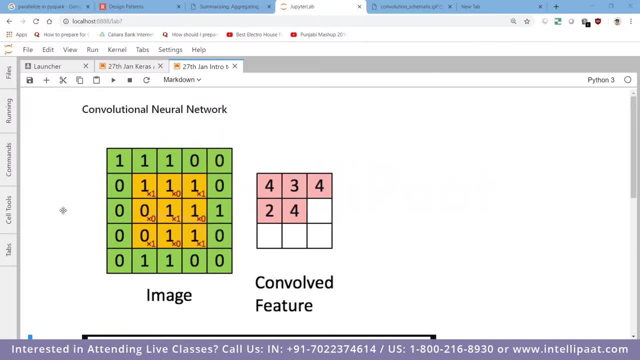 it goes on the right hand side, one by one. it goes on the right hand side, one by one. one is shifting, one is shifting, one is shifting, goes down. again, one shifting goes down, and this is how your final image is made. and this is how your final image is made. 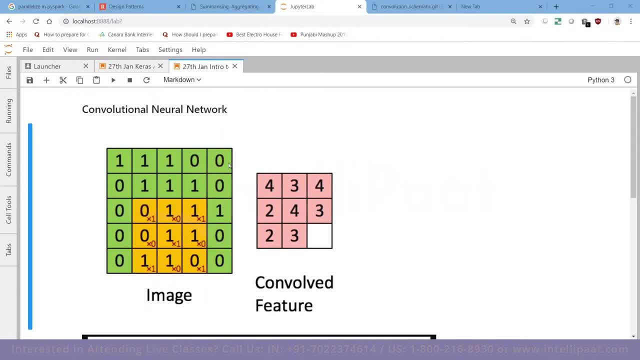 and this is how your final image is made. this, this pink image, is your final image. this, this pink image, is your final image. this, this pink image, is your final image. that is made, that is made. that is made because now i'll tell you what is, because now i'll tell you what is. 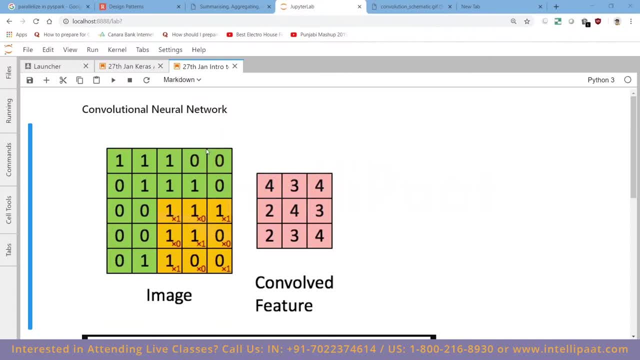 because now i'll tell you what is happening when you are doing this thing. happening when you are doing this thing, happening when you are doing this thing, so what is happening is right now here, so what is happening is right now here. so what is happening is right now here is that, if you 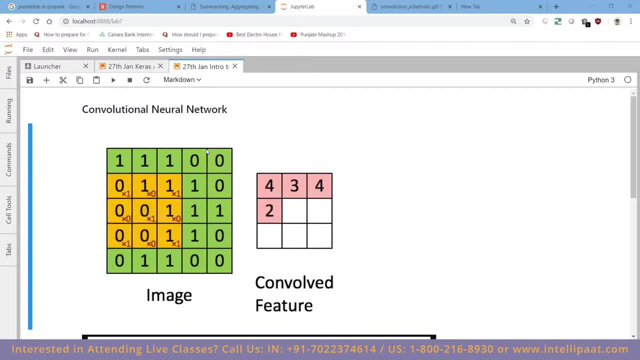 is that? if you is that, if you, so okay, just tell me this thing that. so okay, just tell me this thing that. so okay, just tell me this thing that let's say if. if you are standing, let's say if if you are standing, let's say if, if you are standing in front of something, right, and then so. 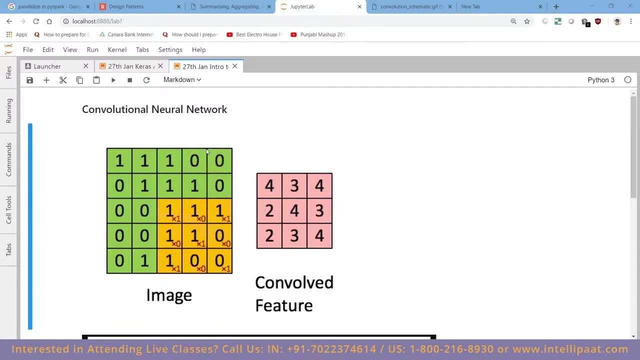 in front of something right and then so in front of something right and then so. how do you identify? how are your images? how do you identify? how are your images? how do you identify? how are your images identifying you as a body? i'll tell you so. there are pixel value. 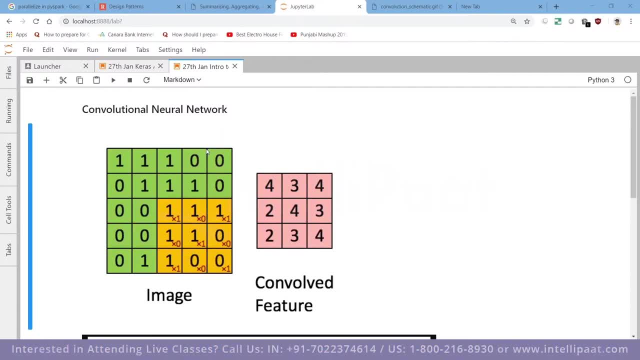 i'll tell you so there are pixel value. i'll tell you so there are pixel value that are changing, that are changing, that are changing at the border of of your body right, so at the border of of your body right, so at the border of of your body right. so let's say that you took a. 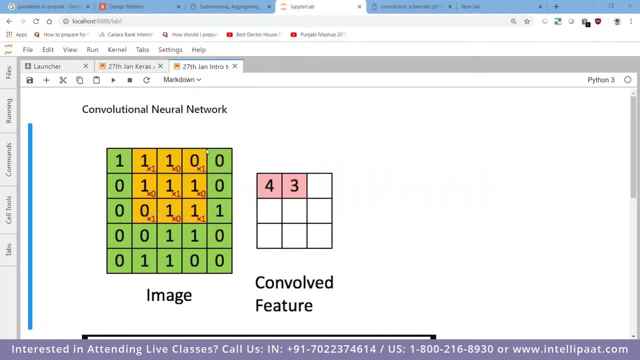 let's say that you took a. let's say that you took a. let's say you're standing in front of a. let's say you're standing in front of a. let's say you're standing in front of a white wall, white wall, white wall, a pure white wall. and then you are. 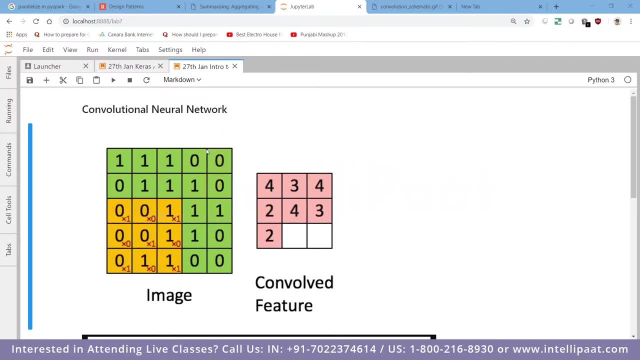 a pure white wall, and then you are a pure white wall and then you are standing, standing, standing. how are you differentiated from a wall? how are you differentiated from a wall? how are you differentiated from a wall? because, if you see, if you open up the, because if you see, if you open up the, 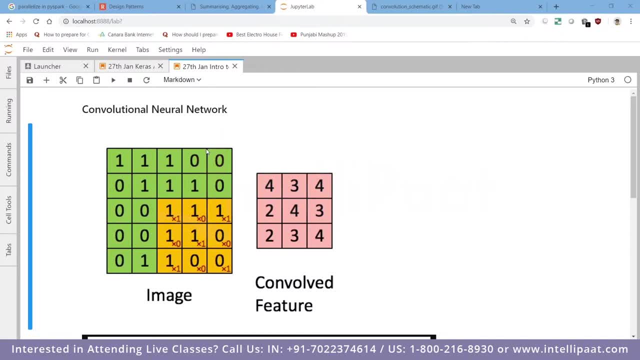 because if you see, if you open up the matrix of that image, if you open up the matrix of that image, if you open up the matrix of that image, if you open up the numpy array of the image, numpy array of the image, numpy array of the image, you'll see that your body will contain. 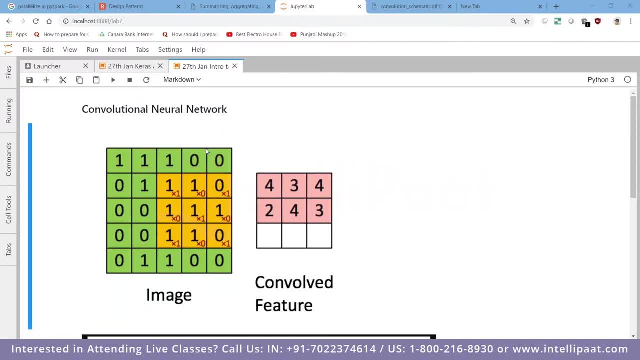 you'll see that your body will contain. you'll see that your body will contain a higher pixel value, a higher pixel value, a higher pixel value, and the white wall will contain zero and the white wall will contain zero and the white wall will contain zero pixel values. right. 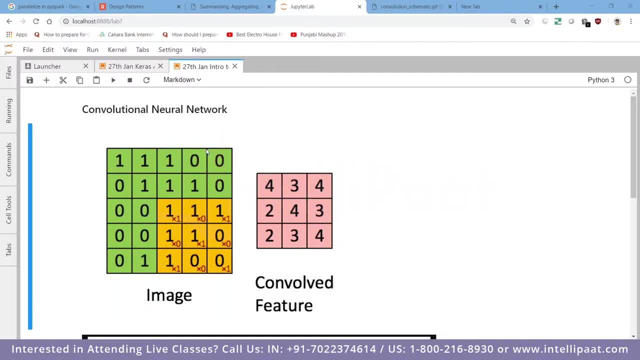 pixel values: right. pixel values, right now. whenever your body to wall is there now. whenever your body to wall is there now. whenever your body to wall is there, whenever the boundary of your body is, whenever the boundary of your body is. whenever the boundary of your body is there. 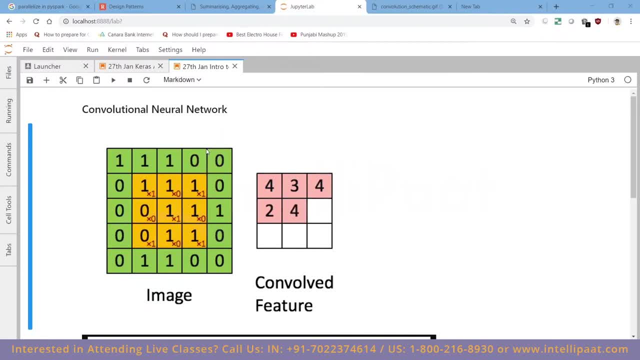 there, there, right at that particular instance, right at that particular instance, right at that particular instance, your pixel values will be changing right. your pixel values will be changing right, your pixel values will be changing right because your pixel value would be, because your pixel value would be, because your pixel value would be somewhat like 230 to 35, and then 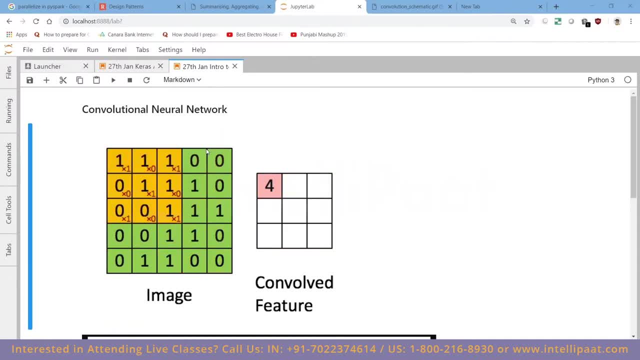 somewhat like 230 to 35, and then somewhat like 230 to 35, and then, suddenly, the image of white will be zero, suddenly the image of white will be zero. suddenly the image of white will be zero, right? so? whenever you will be running, right so, whenever you will be running, 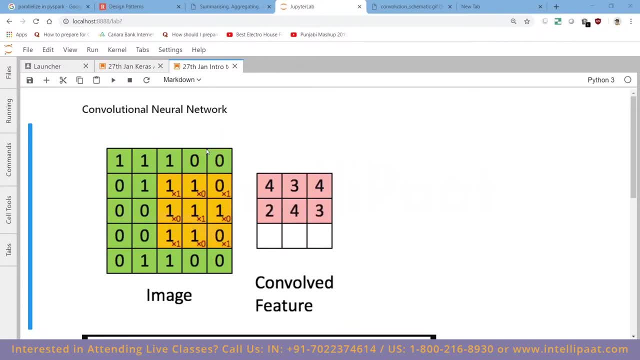 right. so whenever you will be running this, this filter over your image, and then this, this filter over your image, and then this, this filter over your image, and then doing this multiplication, what will doing this multiplication? what will doing this multiplication? what will happen that it will happen that it will. 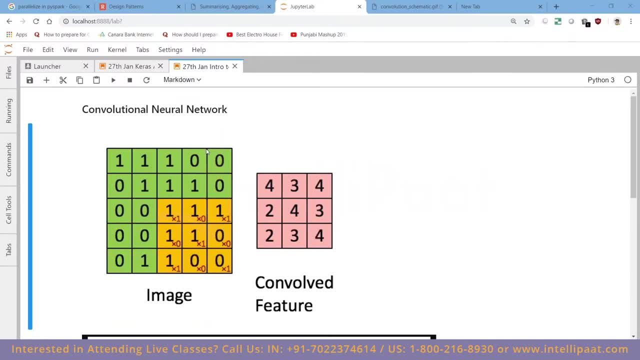 happen that it will large in up the uh the you know broaden large in up the uh the you know. broaden large in up the uh the you know. broaden up the areas. it will broaden up those up the areas. it will broaden up those up the areas. it will broaden up those border areas for you. 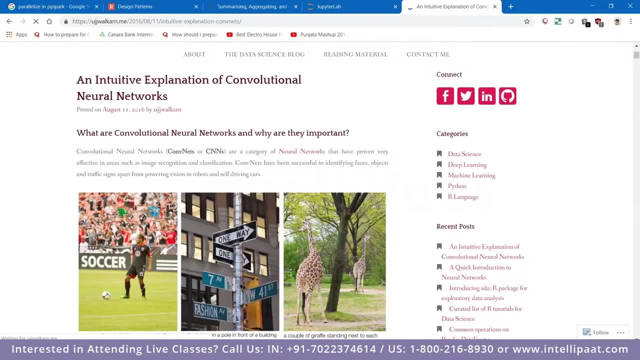 border areas for you, border areas for you, but this is this block actually, but this is this block actually, but this is this block actually. so, if you come down here, what is so? if you come down here, what is so if you come down here, what is happening here is. 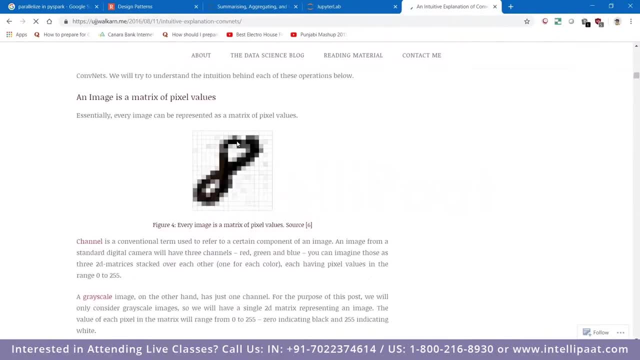 happening here is happening here is: this is what the image looks like, right. this is what the image looks like, right. this is what the image looks like, right. we have already discussed this thing. we have already discussed this thing. we have already discussed this thing: that 255 is sheer, black and white is. 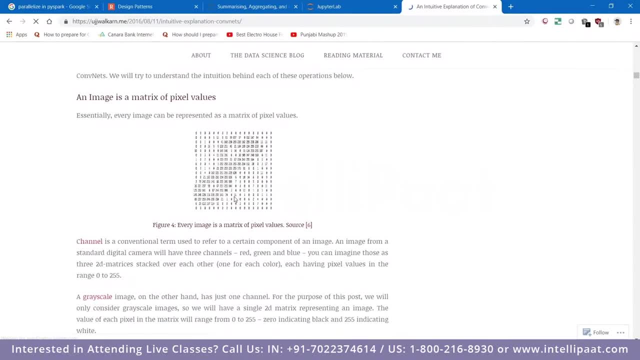 that 255 is sheer black and white, is that 255 is sheer black and white is almost like zero, right, almost like zero right, almost like zero right now. what is happening is: let's say this now: what is happening is: let's say this now: what is happening is: let's say: this green was your image, this green thing. 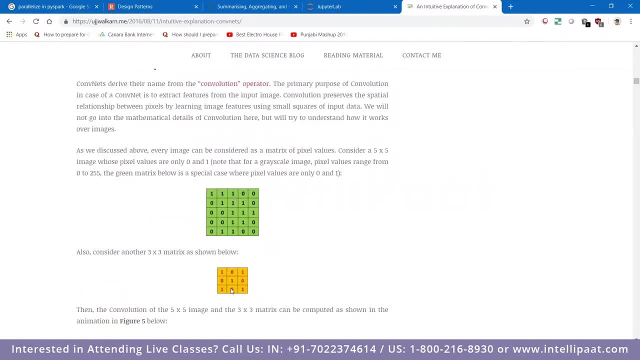 green was your image. this green thing, green was your image, this green thing was your image, and this uh was your image, and this uh was your image. and this, uh, orange one was your matrix right, or you. orange one was your matrix right, or you orange one was your matrix right, or you filter right. what you're going to do is: 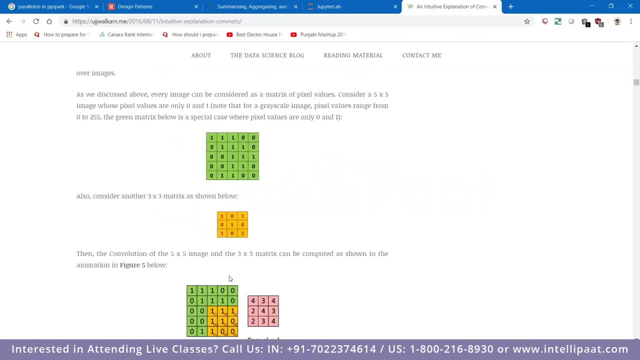 filter right. what you're going to do is filter right. what you're going to do is you're going to put this three cross. you're going to put this three cross. you're going to put this: three cross three. image over this: five cross five. three. image over this: five cross five. 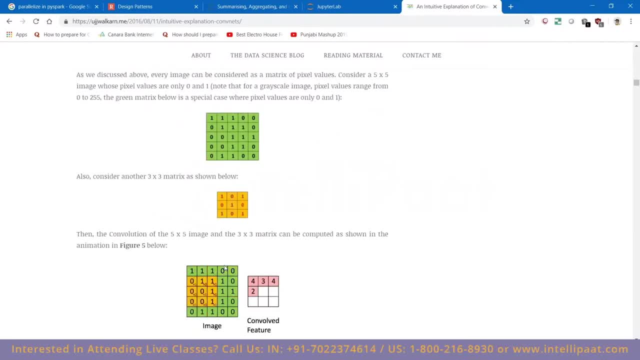 three image over this five cross five image, and then do a multiplication image, and then do a multiplication image and then do a multiplication, right, right, right, multiplication. say you will be getting a multiplication. say you will be getting a multiplication. say you will be getting a convoluted feature. 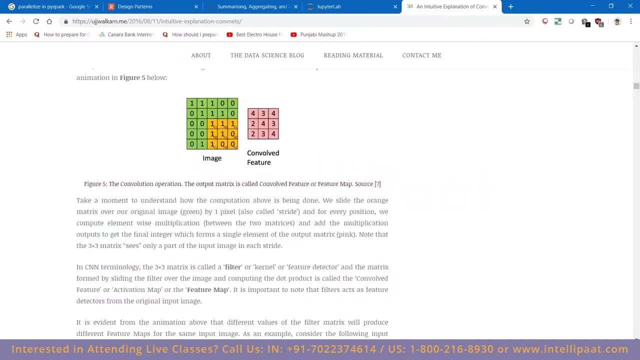 convoluted feature. convoluted feature right now. if you understand this thing right now, if you understand this thing right now, if you understand this thing, okay, so, first of all, you know this thing, okay, so, first of all, you know this thing, okay, so, first of all, you know this thing is called a filter. sometimes we call it. 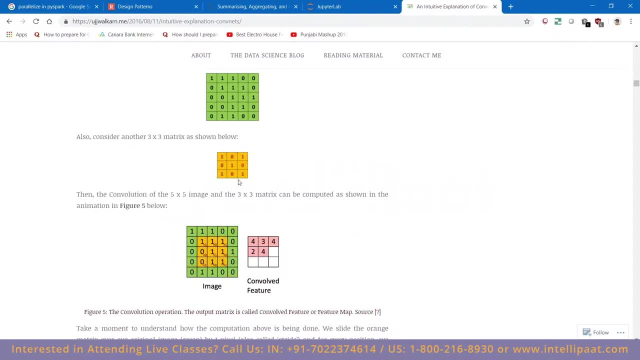 is called a filter. sometimes we call it is called a filter, sometimes we call it as a as a kernel. also this orange thing as a as a kernel, also this orange thing as a as a kernel, also this orange thing as a kernel or a filter also now see. 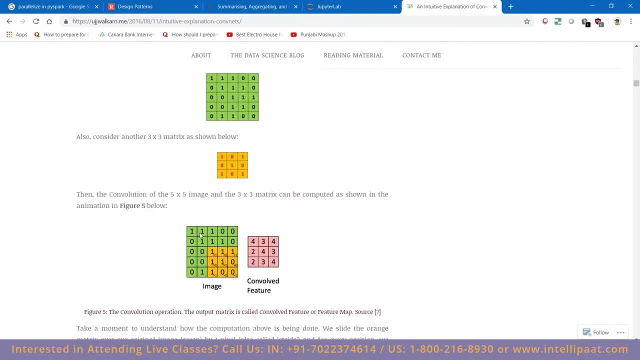 as a kernel or a filter also now see. as a kernel or a filter, also now see. imagine what you're doing. is that you are? imagine what you're doing is that you are? imagine what you're doing, is that you are. let's say, this image was not made up. 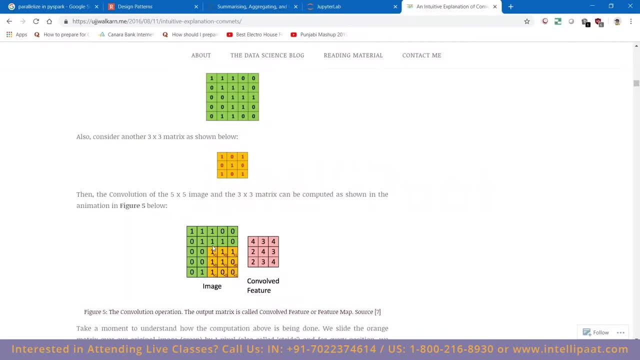 let's say this image was not made up. let's say this image was not made up of zero and one only, but it was made up of of zero and one only, but it was made up of of zero and one only, but it was made up of zero to two, five, five. now what would 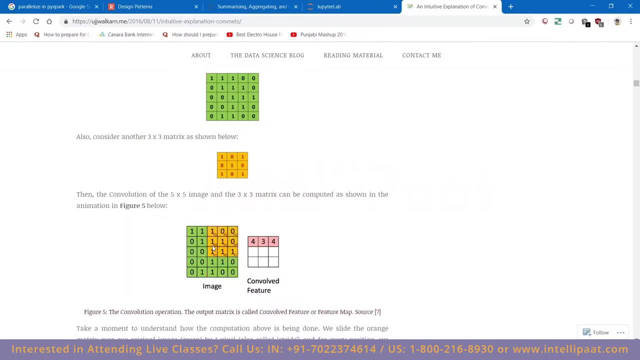 zero to two, five, five now. what would zero to two, five, five now, what would be happening is that the larger values be happening. is that the larger values be happening? is that the larger values, that the value that are two. so imagine that the value that are two. so imagine. 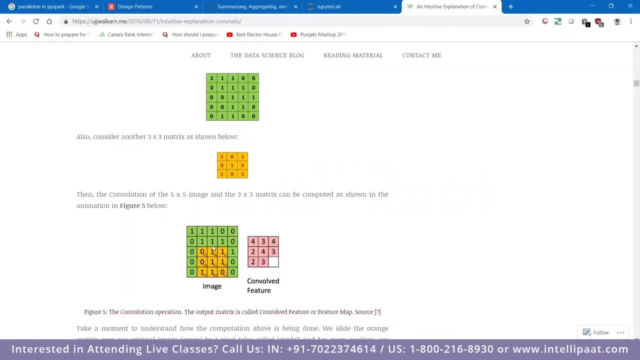 that the value. that are two. so imagine there are two numbers in front of you. there are two numbers in front of you. there are two numbers in front of you. one is called, let's say five. one is called, let's say five. one is called, let's say five, and another one is 230.. now, if you 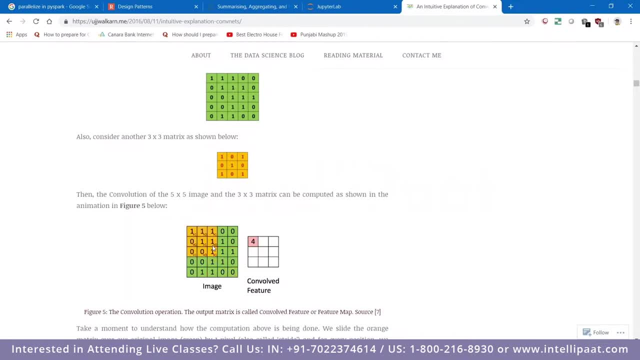 and another one is 230.. now if you and another one is 230.. now, if you multiply both the numbers with, let's say, multiply both the numbers with. let's say, multiply both the numbers with, let's say, 10, which one will become more larger? 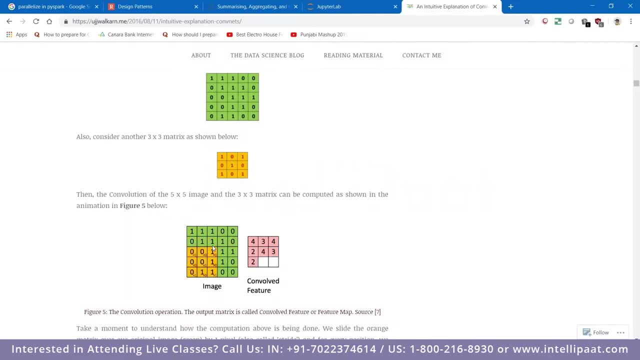 10 which one will become more larger. 10, which one will become more larger. there are two numbers five and another. there are two numbers five and another. there are two numbers five and another. one is 230.. one is 230.. one is 230.. 230 is the person, you, who are standing. 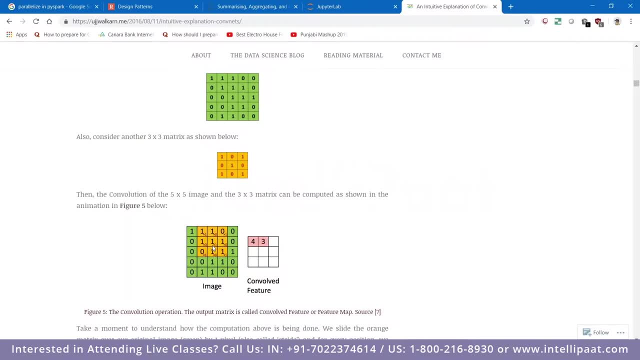 230 is the person, you who are standing. 230 is the person, you who are standing. this is your body. this is your body. this is your body. pixel right, but the white background. the pixel right but the white background. the pixel right but the white background. the white background will contain values. 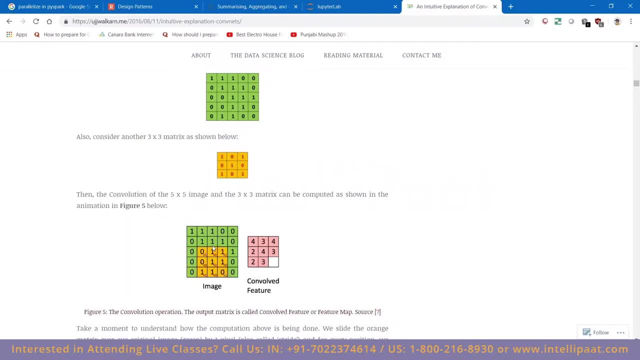 white background will contain values. white background will contain values: from zero to like 10. only right because, from zero to like 10, only right because, from zero to like 10, only right because this is a white wall, a pure white wall. this is a white wall, a pure white wall. this is a white wall, a pure white wall. so let's say, even if we say that there. so let's say, even if we say that there. so let's say, even if we say that there are some tents and something, so that are some tents and something, so that. 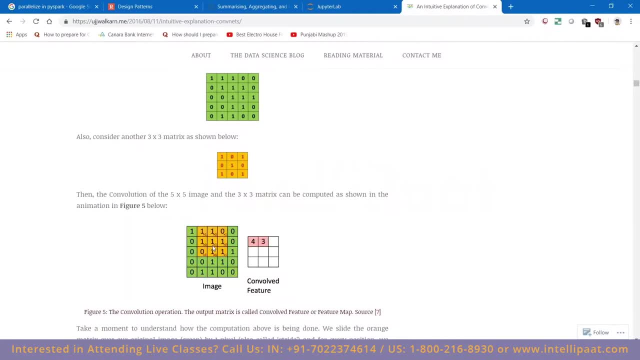 are some tents and something, so that 30 to try 2300, 30 to try 2300, 30 to try 2300. so what is going to happen is that we are. so what is going to happen is that we are. so what is going to happen is that we are going to do a matrix multiplication and 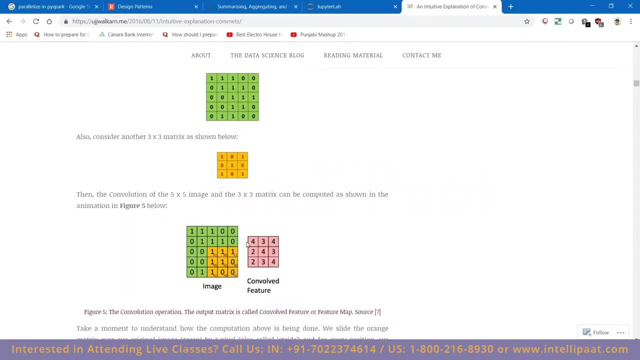 going to do a matrix multiplication and going to do a matrix multiplication and then sum up all the things, and these are then sum up all the things, and these are then sum up all the things. and these are gathered here, right, all the things are gathered here in. 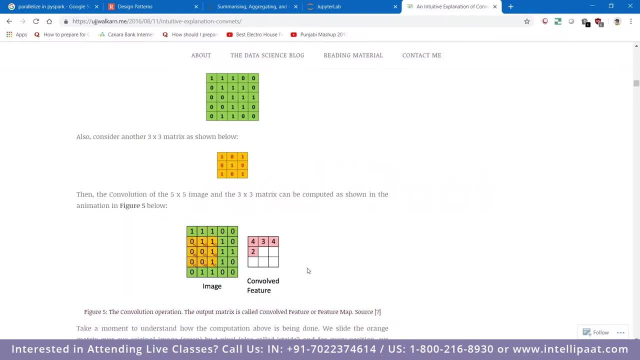 right. all the things are gathered here in right. all the things are gathered here in this area, this area, this area. now you might say that what has happened? now you might say that what has happened now. you might say that what has happened if you have gathered larger values and 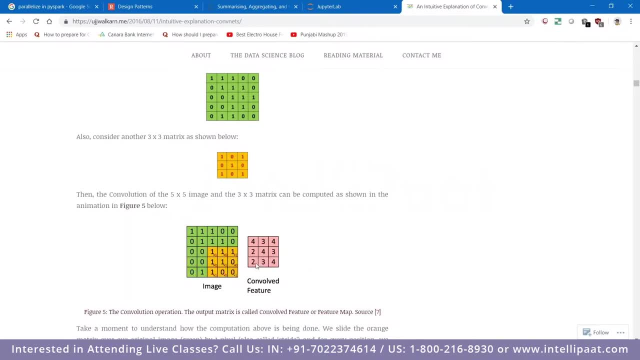 if you have gathered larger values, and if you have gathered larger values and then there might be some lower values, then there might be some lower values also, because if you are running this also, because if you are running this also, because if you are running this thing on a white, 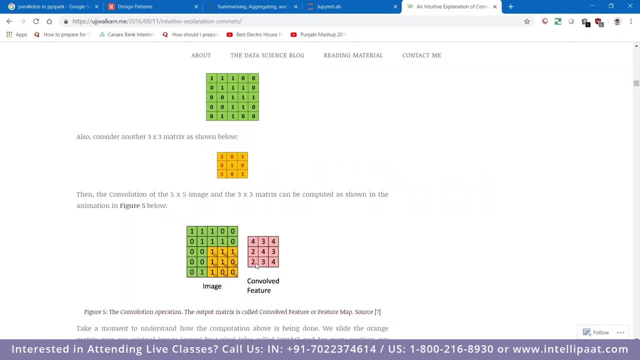 thing on a white thing on a white border also. let's say: if everything is border also. let's say: if everything is border also, let's say: if everything is five, five, five, five multiply by 10, everything is 50 right. five multiply by 10, everything is 50 right. 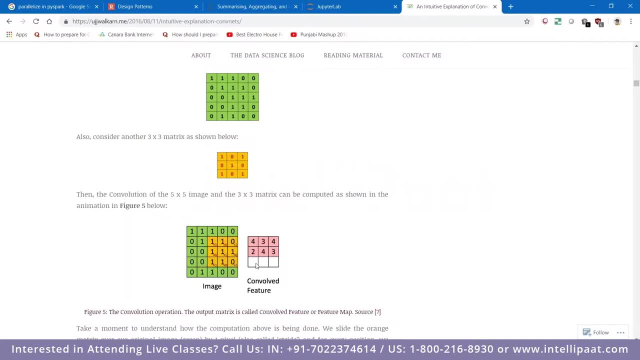 five multiply by 10, everything is 50, right, doesn't make sense. 50 go you add up. doesn't make sense, 50 go, you add up. doesn't make sense, 50 go, you add up. all it will become the same value, right? all it will become the same value, right. 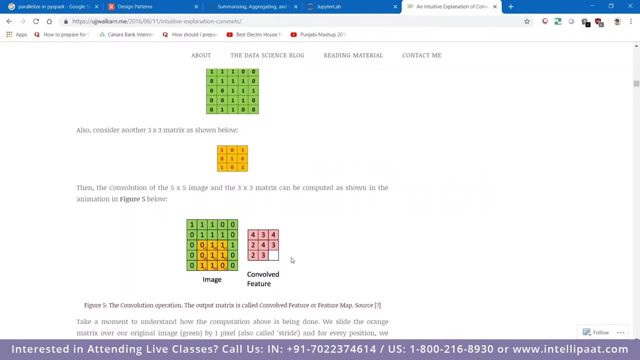 all it will become the same value. right now, i'll tell you how things change here. now i'll tell you how things change here. now. i'll tell you how things change here. when you run this, let's say this was. when you run this, let's say this was. 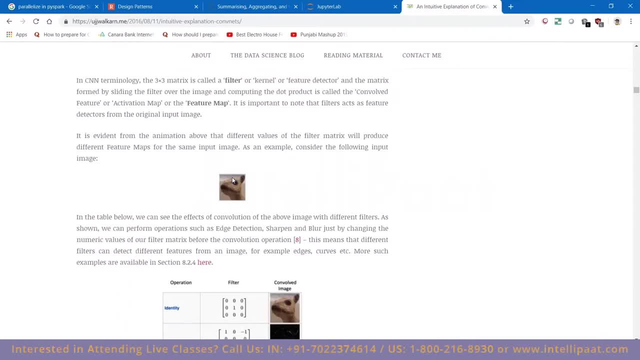 when you run this, let's say: this was your original image, this, this your original image. this this your original image. this, this dear, was your original image. if i zoom dear was your original image. if i zoom dear was your original image. if i zoom in a little bit to show you. 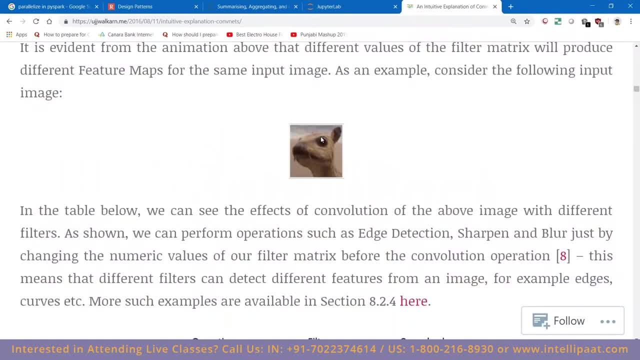 this was the image. if you see clearly on, this was the image. if you see clearly on, this was the image. if you see clearly on my screen, this was the, let's say, my screen, this was the let's say, my screen, this was the let's say image. right, and when you do a filter of 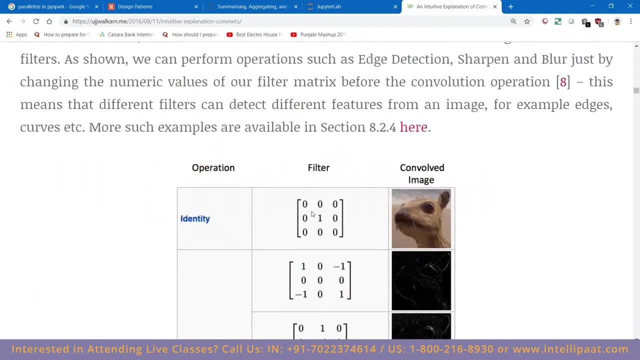 image right and when you do a filter of image right and when you do a filter of this, this, this identity filter, it will return you identity filter. it will return you identity filter. it will return you something like this, something like this, something like this: if you return this filter, it will return. 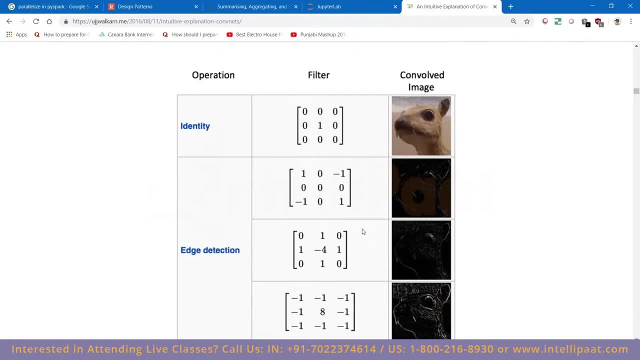 if you return this filter, it will return you something like this: you something like this, you something like this: if you return edge filter. this is: if you return edge filter. this is, if you return edge filter. this is something like this. if you return minus, something like this: if you return minus. 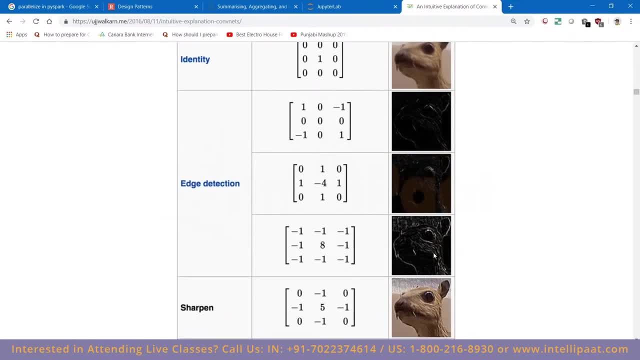 something like this: if you return minus one minus one minus one, one minus one minus one minus one, one minus one minus one, this is called blur sharpened blur, this is called blur sharpened blur. this is called blur sharpened blur, edge blur. then you have box blur. 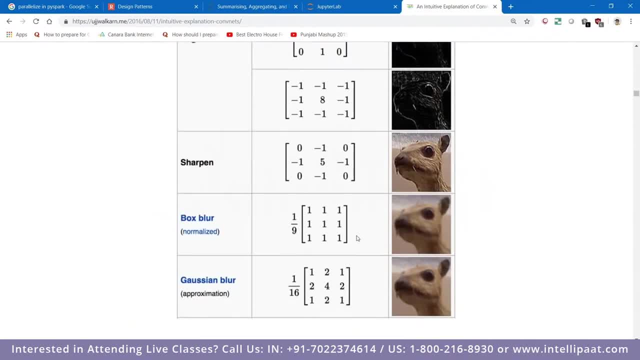 edge blur. then you have box blur, edge blur. then you have box blur, gaussian blur. so this will happen if you gaussian blur. so this will happen if you gaussian blur. so this will happen if you multiply your image with this filter and multiply your image with this filter and 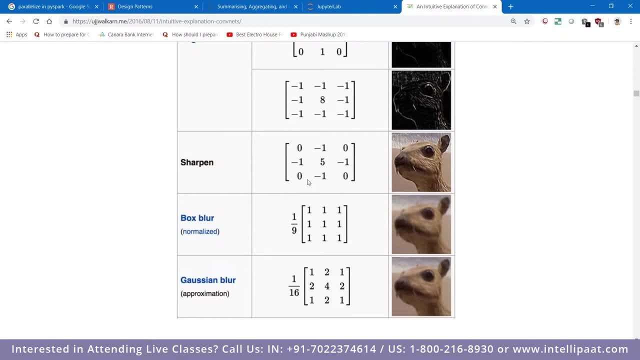 multiply your image with this filter and you run this filter on your image with. you run this filter on your image with. you run this filter on your image with style equal to one, style equal to one, style equal to one. so your original image from here. so your original image from here. 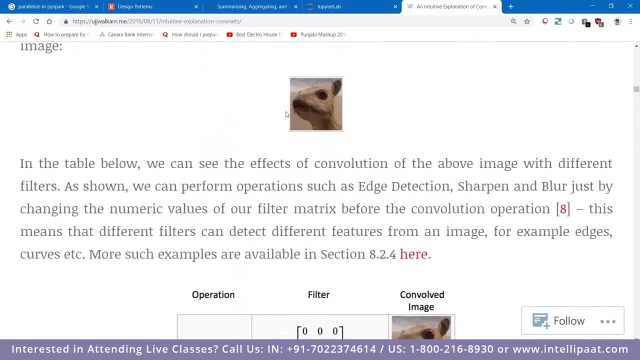 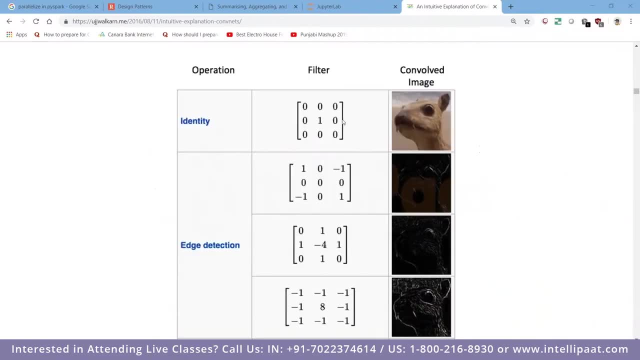 so your original image from here: this thing, this thing, this thing, this particular thing, this thing will this particular thing, this thing, will this particular thing, this thing will change, to change, to change to these things, depending on which which these things, depending on which which these things, depending on which which filter, through which filter you are. 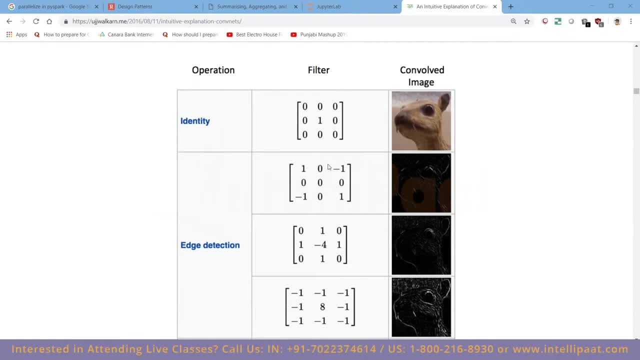 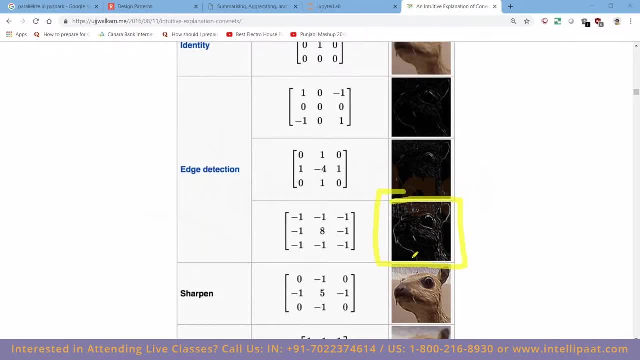 you are, if you are, if you are analyzing this thing, you are, if you are, if you are analyzing this thing, this image, what has happened? this image, what has happened this image, what has happened here is that you can easily see that here is that you can easily see that. 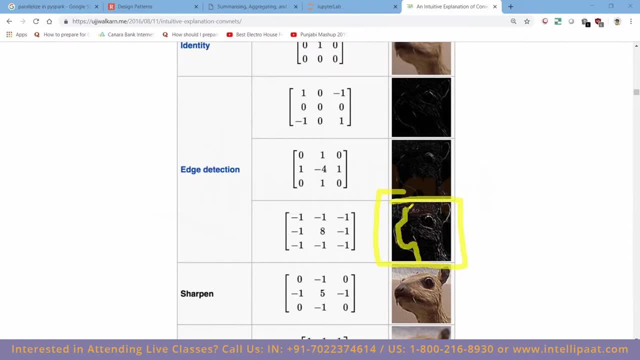 here is that you can easily see that the animals border are now created, or the animals border are now created, or the animals border are now created or sharpened here, right, you can more sharpened here, right, you can more sharpened here, right. you can more easily visualize the borders of the 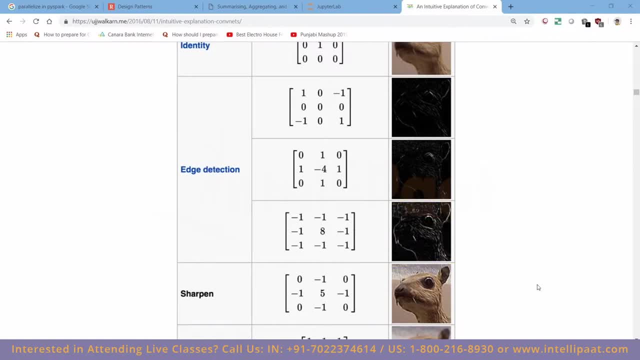 easily visualize the borders of the easily visualize the borders of the animal right, animal right, animal right. rather than with this, with this original, rather than with this with this original, rather than with this with this original. image at here, image at here. image at here, where the borders were not much uh. 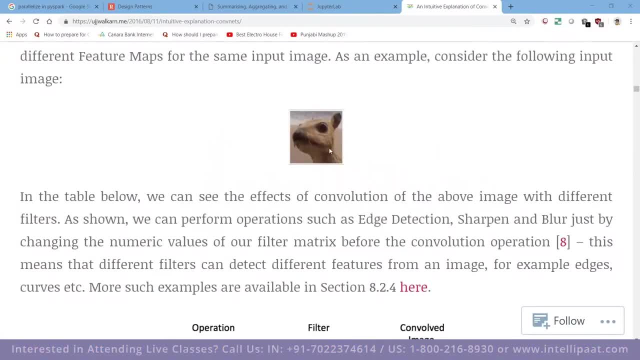 where the borders were not much. uh. where the borders were not much, uh, much they were not much in the same group. much they were not much in the same group, much they were not much in the same group. now you can easily do a spread out with. now you can easily do a spread out with. 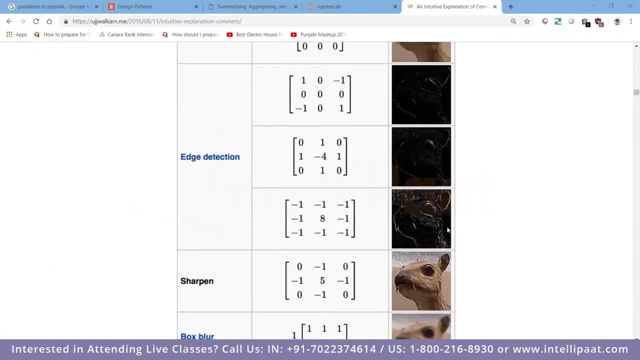 now you can easily do a spread out with just one convolution. just one convolution, just one convolution, and this is just one we will like. and this is just one we will like, and this is just one we will like. replicate it like multiple times to get. replicate it like multiple times to get. 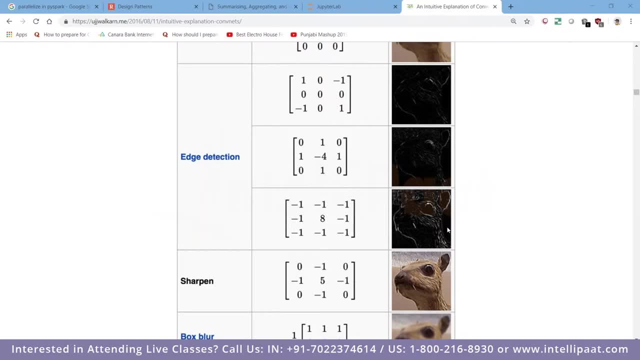 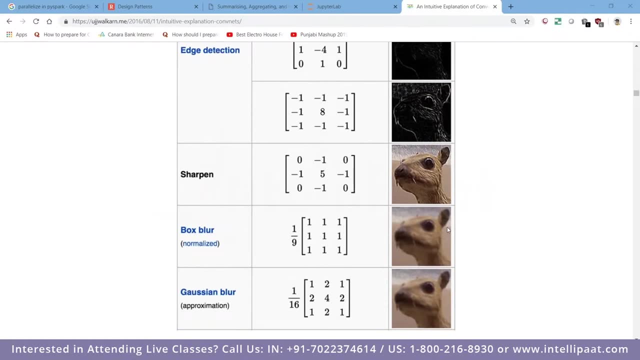 replicate it like multiple times to get more, more, more value out of it. make sense now you understand why we are make sense now you understand why we are make sense. now you understand why we are doing this, doing this, doing this, running a filter over the image. now this: running a filter over the image. now this: running a filter over the image. now, this depends that. what are the values that depends that? what are the values that depends that? what are the values that you're using inside your filter? your you're using inside your filter your. 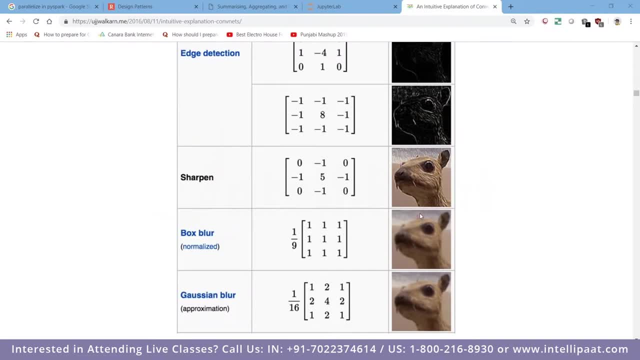 you're using inside your filter. your filter might do a blur of the image also. filter might do a blur of the image also. filter might do a blur of the image also and it might do a sharpening of your and it might do a sharpening of your. 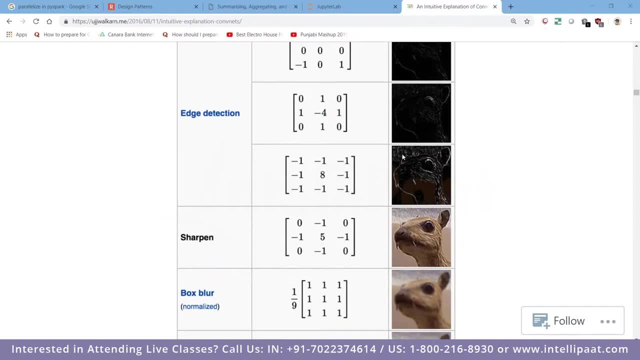 and it might do a sharpening of your image also, image also, image also, and these, this thing, this edge detection, and these, this thing, this edge detection, and these, this thing, this edge detection is the something that we want to do right, is the something that we want to do right. 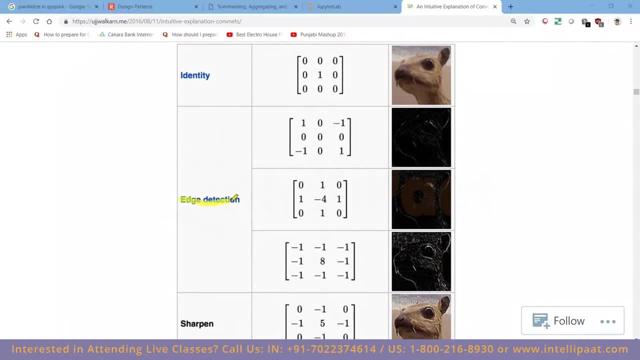 is the something that we want to do right now that we are very much interested to now that we are very much interested to, now that we are very much interested to know that what is the edge of that, know that what is the edge of that, know that what is the edge of that animal, so that we can differentiate if 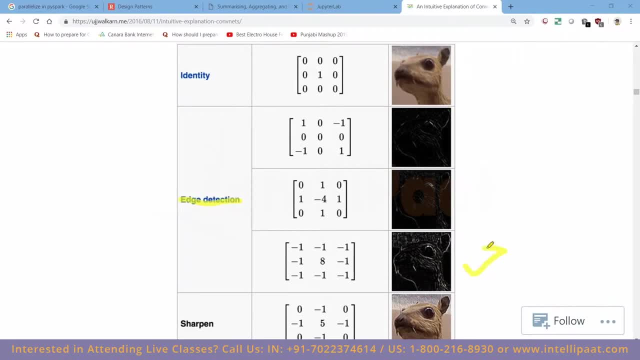 animal, so that we can differentiate if animal, so that we can differentiate if it's a cat or a dog, right, and this is a. it's a cat or a dog, right, and this is a. it's a cat or a dog, right, and this is a perfect example how things are working. 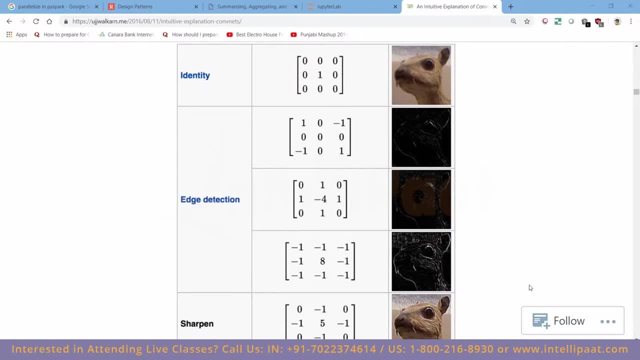 perfect example how things are working. perfect example how things are working for us, for us, for us, correct now. once you have done this correct now, once you have done this correct now, once you have done this filter, and you have got a very edgy filter, and you have got a very edgy. 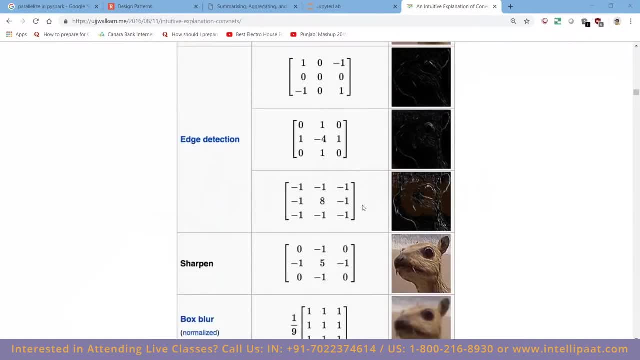 filter and you have got a very edgy image. now, what you want to do is still image now. what you want to do is still image. now. what you want to do is still on this edgy image you want to capture, on this edgy image you want to capture. 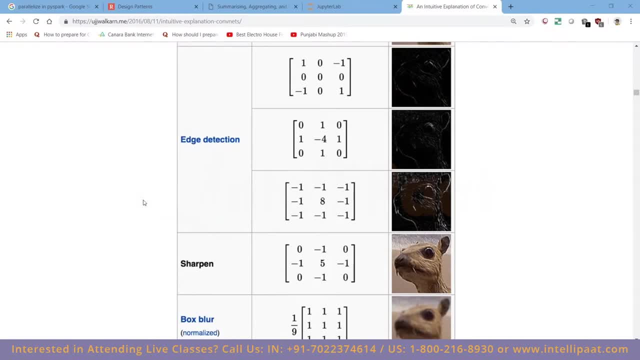 on this edgy image. you want to capture the maximum values, so you, so now the maximum values. so you, so now the maximum values. so you so now imagine that what you have done is. you imagine that what you have done is you imagine that what you have done is you have multiplied a larger number with a. 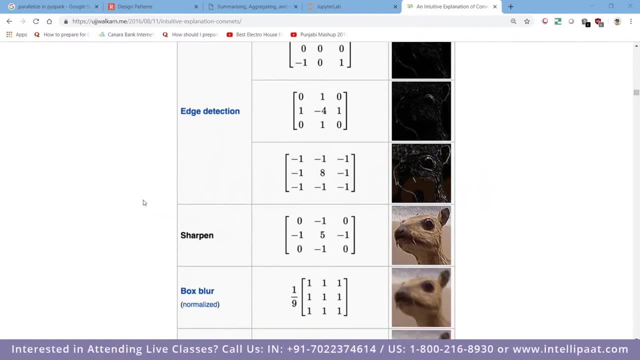 have multiplied a larger number with a. have multiplied a larger number with a more larger number. right, more larger number, right, more larger number, right. so your smaller number will become so your smaller number will become, so your smaller number will become smaller and larger number will become smaller and larger number will become. 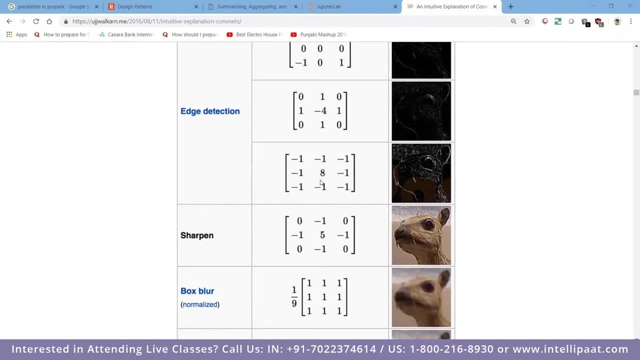 smaller and larger number will become more larger, and then also you are saying more larger, and then also you are saying more larger, and then also you are saying that you want to have the maximum, that you want to have the maximum, that you want to have the maximum values only. 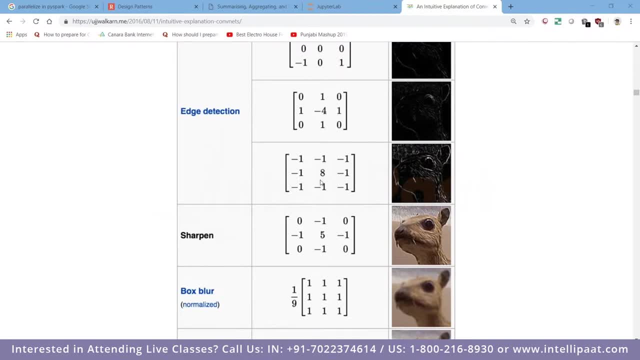 values, only, values only. this step is called as the second step. this step is called as the second step. this step is called as the second step in our cnn network, and this is called in our cnn network, and this is called in our cnn network, and this is called max pooling. this is called as max pooling. 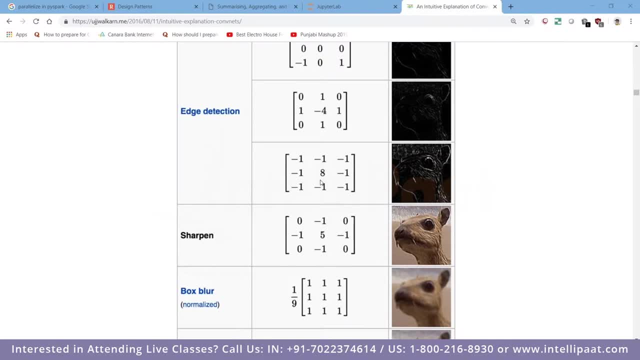 max pooling- this is called as max pooling. max pooling- this is called as max pooling. the first thing was running a filter over. the first thing was running a filter over. the first thing was running a filter over your images. right that you have already your images. right that you have already. 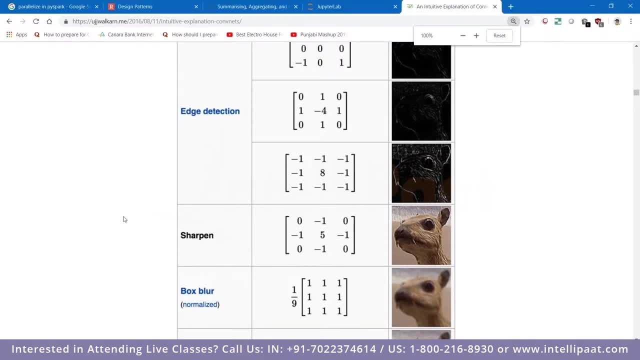 your images, right that you have already run successfully and you got everything run successfully and you got everything run successfully and you got everything out of your image, out of your image, out of your image. next, what you're going to do is: you are. next, what you're going to do is you are. 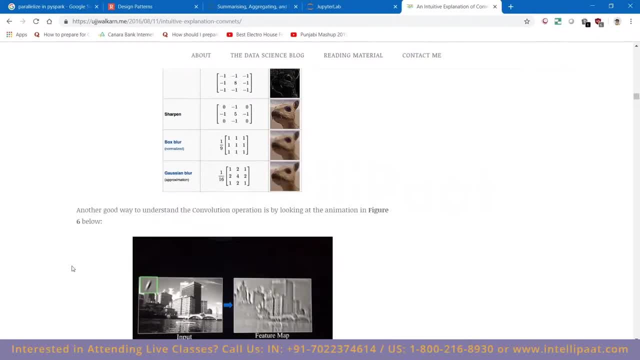 next, what you're going to do is you are going to do, going to do, going to do this thing. okay again, sorry, one more this thing. okay again, sorry, one more this thing. okay again, sorry. one more thing to show you thing. to show you thing to show you, let's see, with different, different. 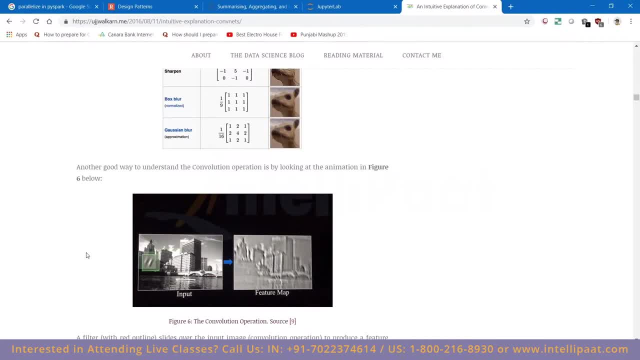 let's see with different, different. let's see with different, different filters. you have different, different filters. you have different, different filters. you have different, different feature maps available to you. let me zoom feature maps available to you. let me zoom feature maps available to you. let me zoom in so that you can see it more. 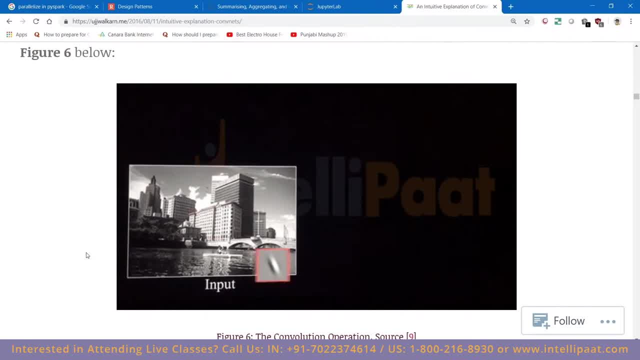 in so that you can see it more in, so that you can see it more efficiently. so what we are doing is we efficiently. so what we are doing is we efficiently. so what we are doing is we are trying to run a, are trying to run a, are trying to run a filter over this and through different 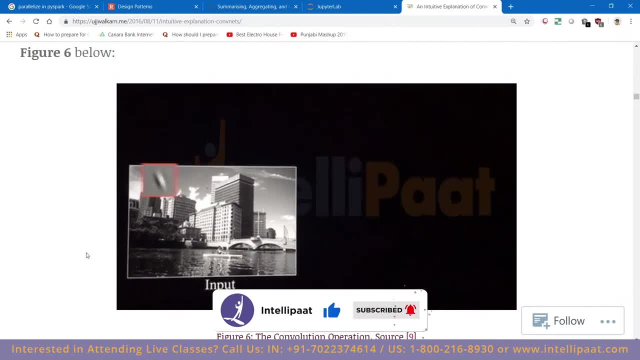 filter over this and through different filter over this and through different, different filters. you can see different, different filters. you can see different. different images are coming out. different, different images are coming out. different, different images are coming out. different. different outputs are coming out. different, different outputs are coming out. 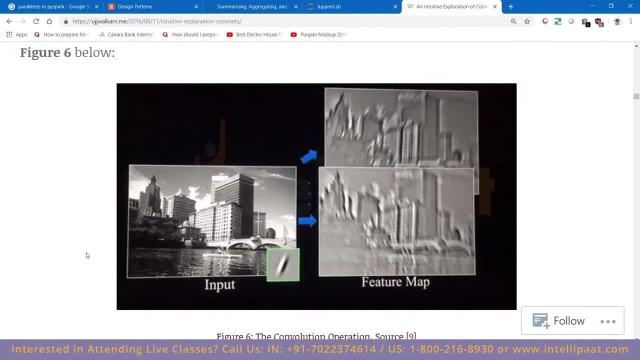 different, different outputs are coming out right right right makes sense. so what we are going to do makes sense. so what we are going to do makes sense. so what we are going to do is next: what we are okay now in this one is next: what we are okay now in this one: 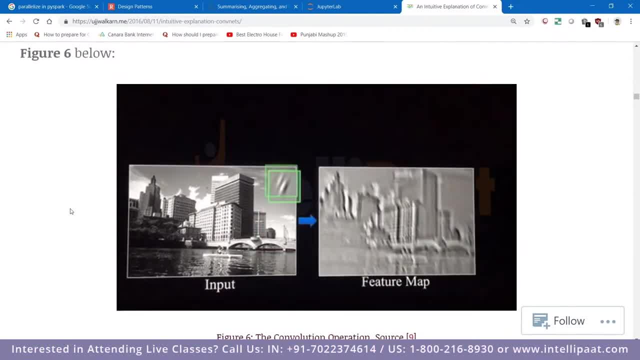 is next what we are okay now in this. one more thing i want to uh tell you, is that more thing i want to uh tell you, is that more thing i want to uh tell you is that you should have asked me this question. you should have asked me this question. 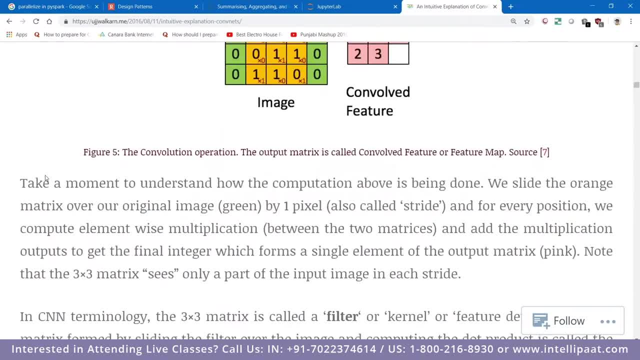 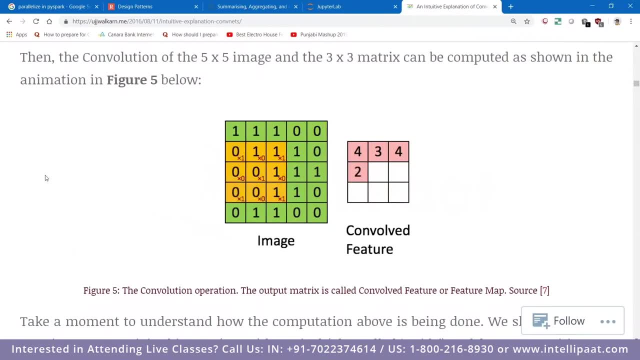 you should have asked me this question, that that that in this particular, in this particular, in this particular gif that we are seeing here, we are gif that we are seeing here, we are gif that we are seeing here, we are seeing. you might argue this to me that 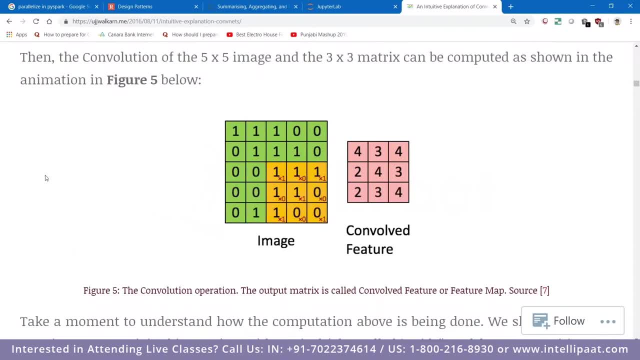 seeing you might argue this to me, that seeing you might argue this to me- that okay, this is also arbitrary right, we can. okay, this is also arbitrary right, we can. okay, this is also arbitrary right, we can. we can move it to two steps also. we can move it to two steps also. 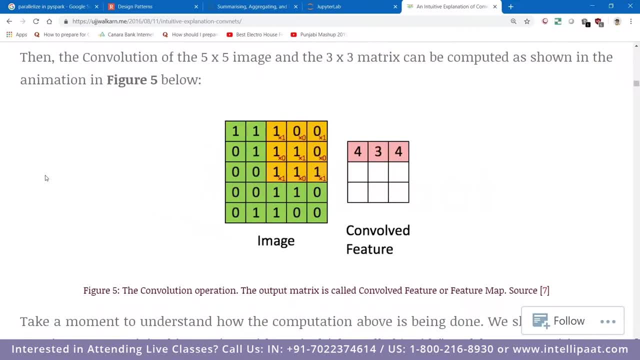 we can move it to two steps also, and my answer would be yes, you can move, and my answer would be yes, you can move, and my answer would be yes, you can move it two steps. you can move it three steps. it two steps. you can move it three steps. 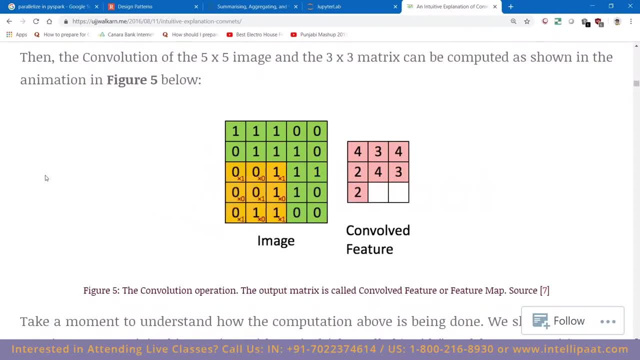 it two steps, you can move it three steps, and if it's a very large image, you can, and if it's a very large image, you can, and if it's a very large image, you can move it like, move it like, move it like more steps, right, so it depends on the 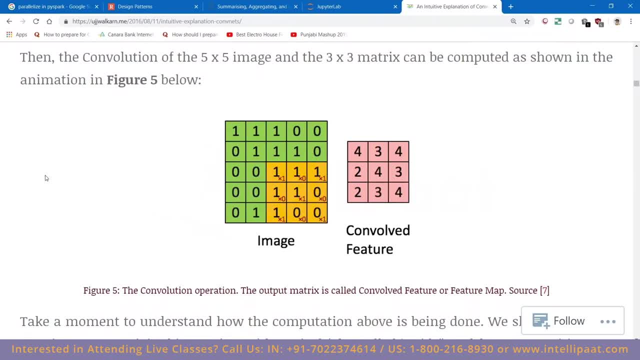 more steps right. so it depends on the more steps right. so it depends on the now the gif that you're seeing, the now the gif that you're seeing, the now the gif that you're seeing, the stride is equal to one. when you say: stride is equal to one when you say: 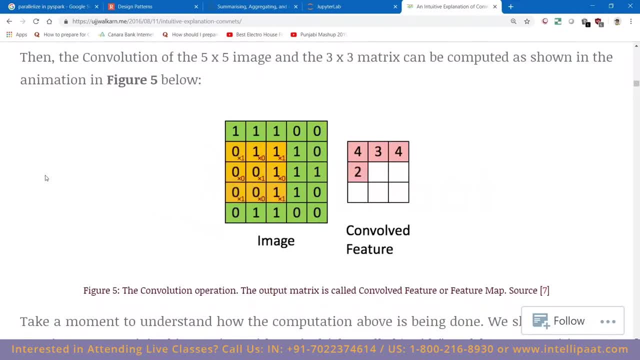 stride is equal to one. when you say stride is equal to one, it means that you stride is equal to one. it means that you stride is equal to one. it means that you will be moving your image. the kernel will be moving your image. the kernel will be moving your image, the kernel with one step ahead. 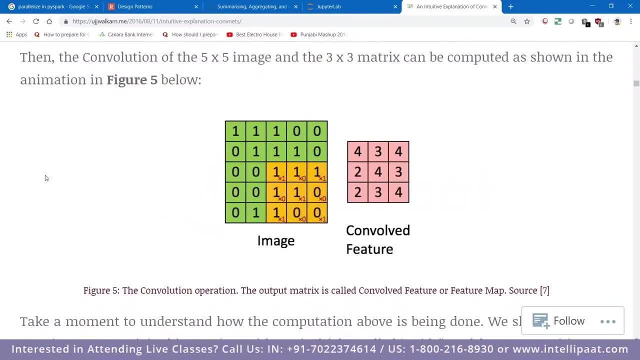 with one step ahead, with one step ahead from left to right. your kernel will be from left to right, your kernel will be from left to right, your kernel will be moving one step, and similarly for going moving one step, and similarly for going moving one step, and similarly for going down also. 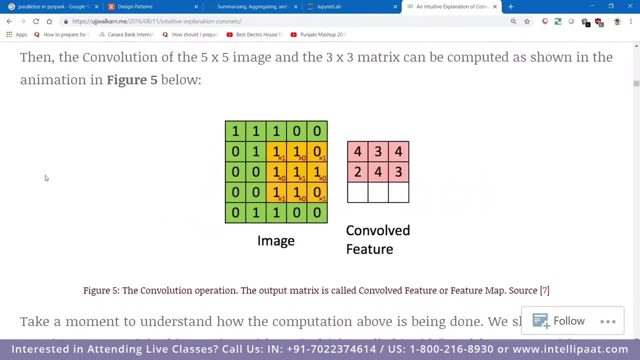 down, also, down, also. so it's. if you see, uh, if you quietly so it's. if you quietly so it's if you quietly observe that your kernel is shifting, observe that your kernel is shifting. observe that your kernel is shifting downwards, with just one row only. downwards, with just one row only. 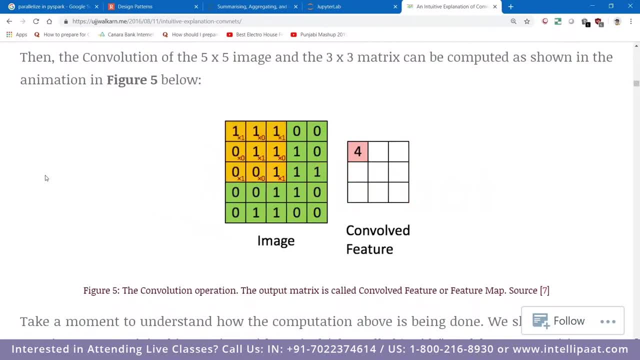 downwards with just one row only. it might have shifted to two rows also. it might have shifted to two rows also. it might have shifted to two rows also. right, right, right, but because you have set as strides as, but because you have set as strides as, but because you have set as strides as one comma one. one comma one means that 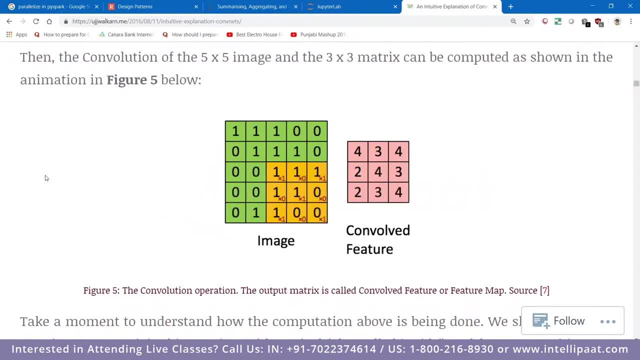 one comma one. one comma one means that one comma one. one comma one means that you will be shifting column to one, you will be shifting column to one, you will be shifting column to one. and to row also, you'll be shifting. and to row also, you'll be shifting. 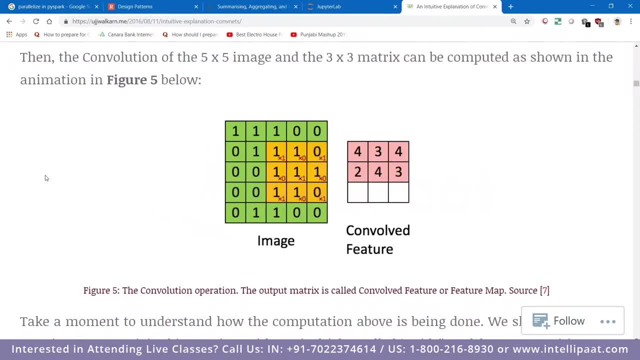 and to row also, you'll be shifting one. so till now, what we have done is we one. so till now, what we have done is we one. so till now, what we have done is we have taken some arbitrary arbitrary, have taken some arbitrary arbitrary, have taken some arbitrary, arbitrary matrix, called as the kernel matrix. 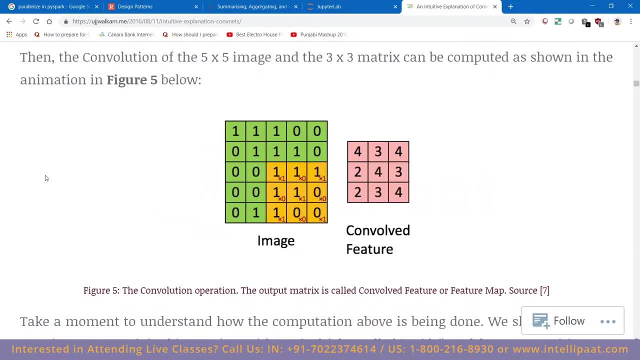 matrix called as the kernel matrix, matrix called as the kernel matrix. right then we took some arbitrary values. right then we took some arbitrary values. right then we took some arbitrary values inside it also inside it, also inside it, also some random values. then we have taken some random values. then we have taken 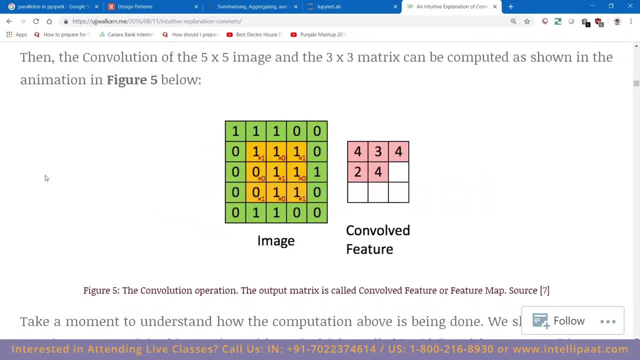 some random values. then we have taken this thing called strides, this thing called strides, this thing called strides, we have by default, we are giving it at. we have by default, we are giving it at. we have by default, we are giving it at one comma one. it means one row to the. 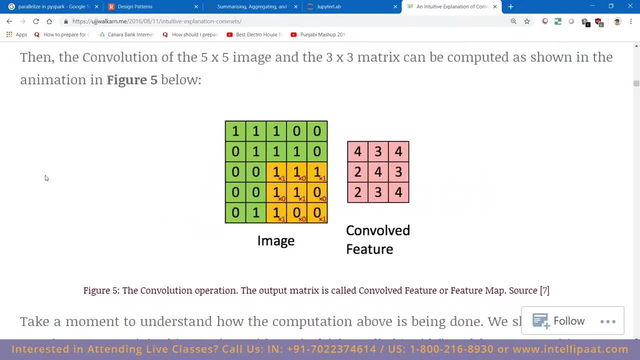 one comma one. it means one row to the one comma one. it means one row to the left and also right, and one to the left and also right, and one to the left and also right, and one to the down right, down right, down right. so we're cherishing all these things as. 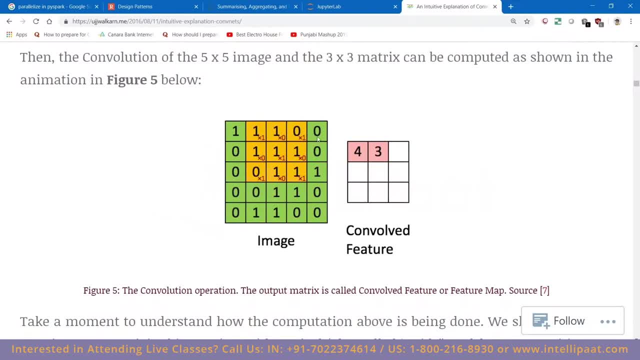 so we're cherishing all these things as. so we're cherishing all these things as of now, of now, of now, and then we have got out something that, and then we have got out something that, and then we have got out something that is called convoluted field. 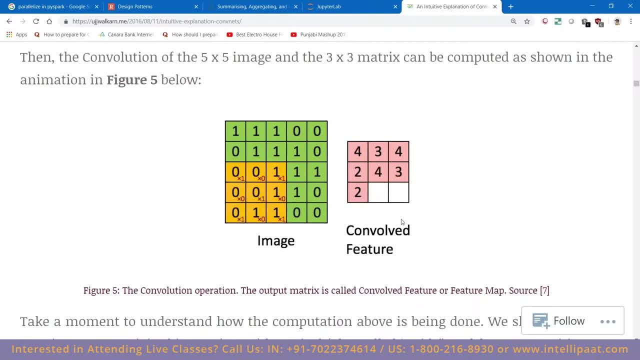 is called convoluted field is called convoluted field. feature right now. one thing is for sure: feature right now. one thing is for sure: feature right now. one thing is for sure: that your uh, that, your uh, that, your uh, that your output is going to shrink from. 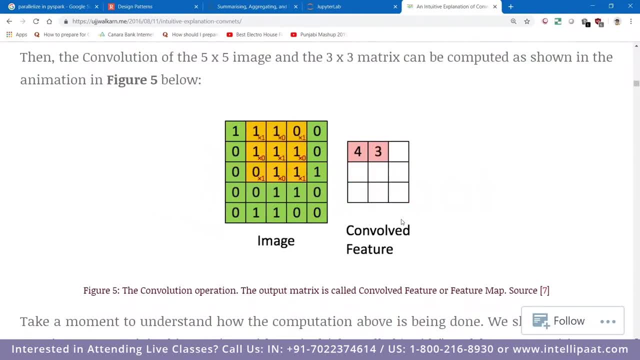 that your output is going to shrink from that. your output is going to shrink from the original image, the original image, the original image, right. so originally, if you see in your example right now, if you see in your example right now, if you see in your example, your image was around 5 cross 5. 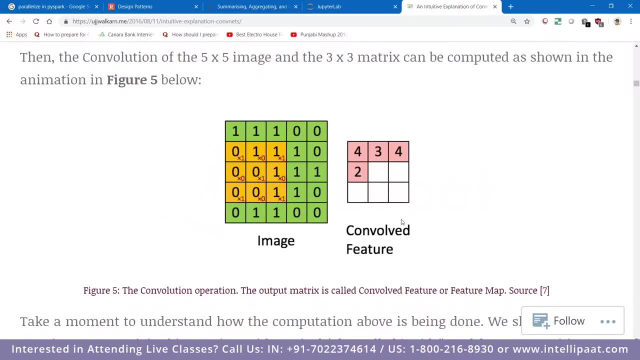 your image was around 5 cross 5. your image was around 5 cross 5, and now it has come into just 3 cross, and now it has come into just 3 cross, and now it has come into just 3 cross, 3. right, let's move to the next stage. 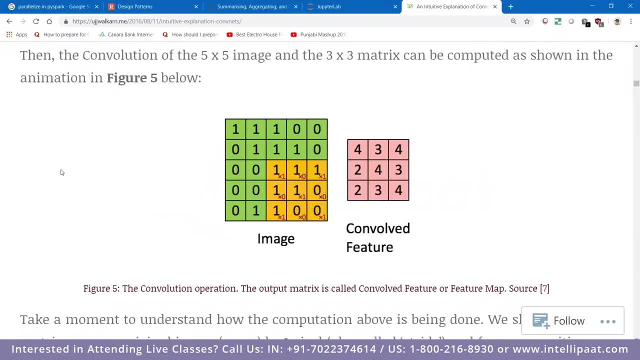 3- right, let's move to the next stage. 3- right, let's move to the next stage. where we have done this convolution, our where we have done this convolution, our where we have done this convolution, our next step would be. next step would be: next step would be to get more darker, i mean more edgy. 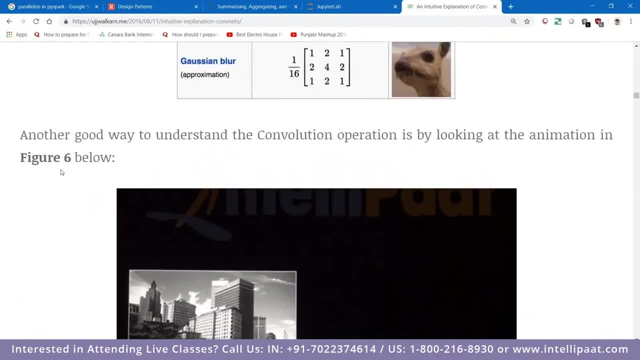 to get more darker, i mean more edgy. to get more darker, i mean more edgy. features out of it. features out of it. features out of it. so what we're going to do is after we. so what we're going to do is after we. so what we're going to do is after we have got this feature map here on the 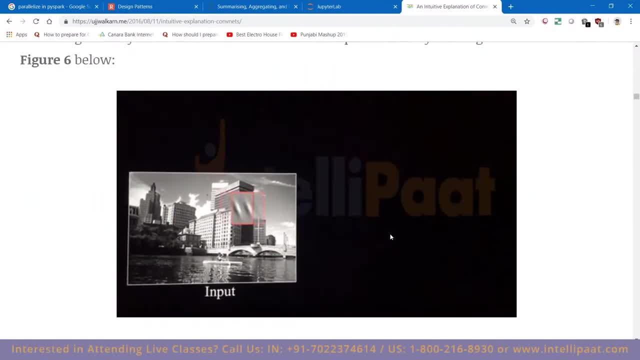 have got this feature map here on the. have got this feature map here on the. uh after once. we have got this feature. uh after once. we have got this feature. uh after once. we have got this feature. map on the left hand side, what we're map on the left hand side, what we're. 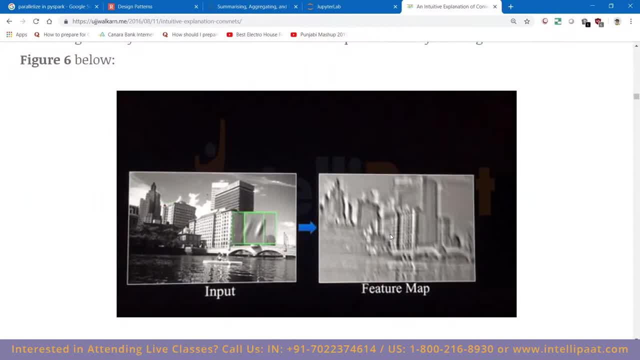 map on the left hand side. what we're trying to do is we'll again find out trying to do, is we'll again find out trying to do, is we'll again find out more maximum numbers out of it, more maximum numbers out of it, more maximum numbers out of it. so what i'll do, 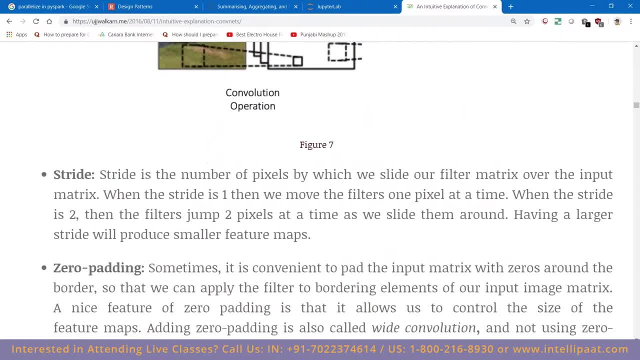 so what i'll do? so what i'll do, i'll do somewhat, i'll do somewhat, i'll do somewhat. let me show you where it is. let me show you where it is, let me show you where it is. this thing, this thing, this thing. so let's say, on the left hand side, that 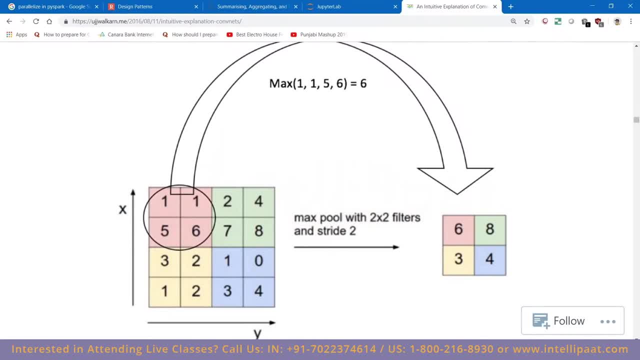 so let's say on the left hand side that. so let's say on the left hand side that you're seeing, is the you're seeing, is the you're seeing, is the convoluted filter. i mean this is the thing. convoluted filter. i mean this is the thing. 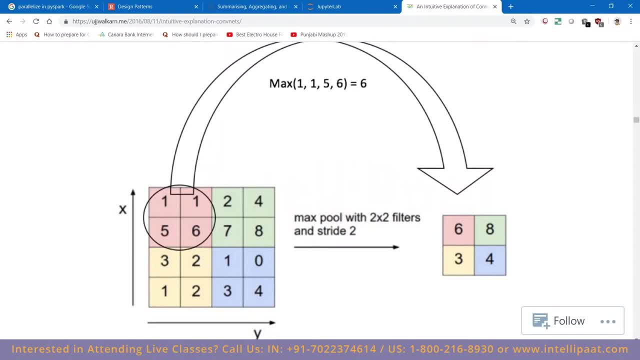 convoluted filter. i mean, this is the thing that they have returned you after that. they have returned you after that. they have returned you after you have done your. you have done your. you have done your uh feature mapping right, or your, or your uh feature mapping right, or your or your. 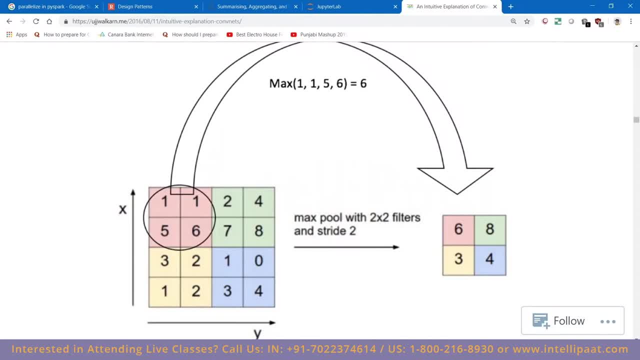 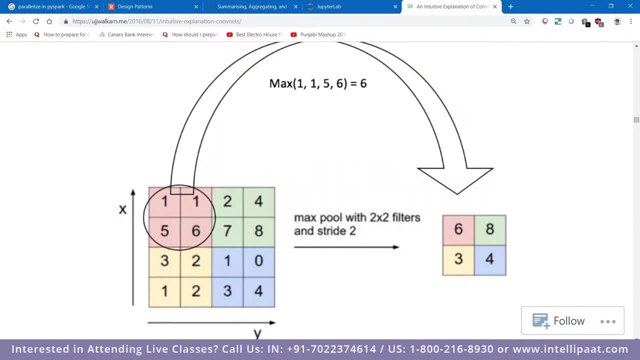 like mapping is done, you ran the filter over your image, and this is the output filter over your image, and this is the output filter over your image and this is the output that you see on the left hand side, that you see on the left hand side, that you see on the left hand side. now again, what you will do is you will. 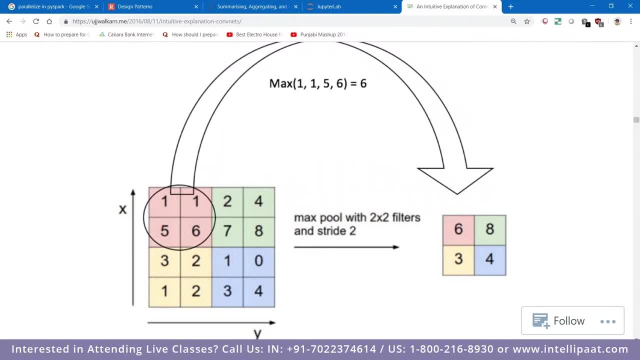 now again, what you will do is: you will now again what you will do is you will say that i will take a two by two. say that i will take a two by two, say that i will take a two by two, square, square, square right. i will take a two by two, square. 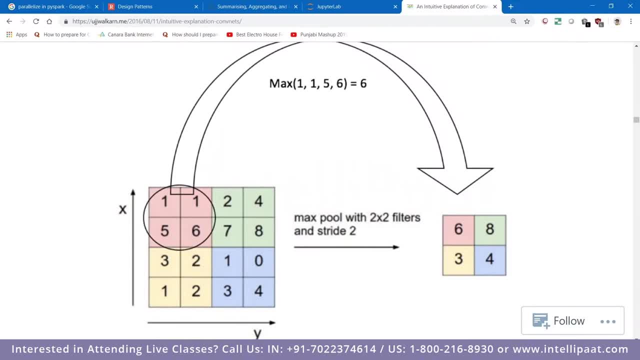 right, i will take a two by two square. right, i will take a two by two square and i'll pick up the maximum values and i'll pick up the maximum values and i'll pick up the maximum values that are present inside the image, that are present inside the image. 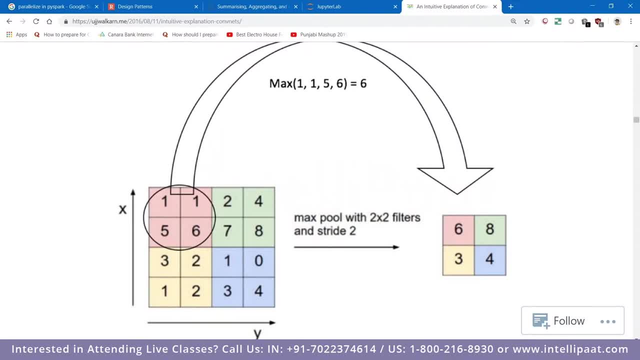 that are present inside the image. so what is going to happen is currently so. what is going to happen is currently so. what is going to happen is currently. your answer is in the. your answer is in the. your answer is in the shape of four cross, four right and then. shape of four cross four right, and then shape of four cross four right, and then four cross four, and let's say that you four cross four, and let's say that you four cross four and let's say that you are making a two cross two circle, are making a two cross two circle. 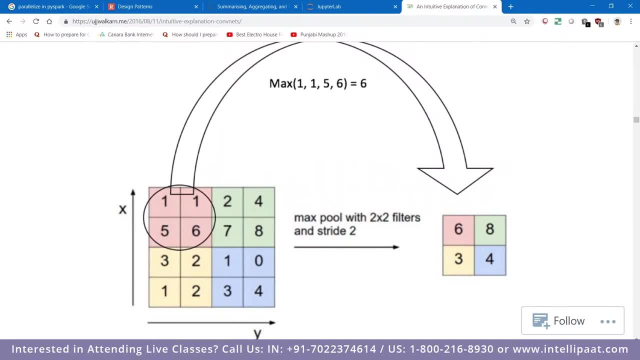 are making a two cross two circle and then you have to find the maximum, and then you have to find the maximum, and then you have to find the maximum value. so in the first two cross two, you value. so in the first two cross two, you value. so in the first two cross two, you find six. in the seven you have eight in. 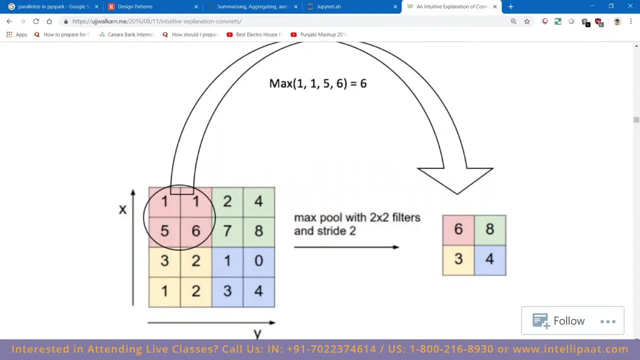 find six, in the seven, you have eight. in find six in the seven, you have eight. in the third, you have three, and in the, the third, you have three. and in the, the third, you have three. and in the fourth, you have four. fourth, you have four, fourth, you have four. makes sense even this max pooling thing. 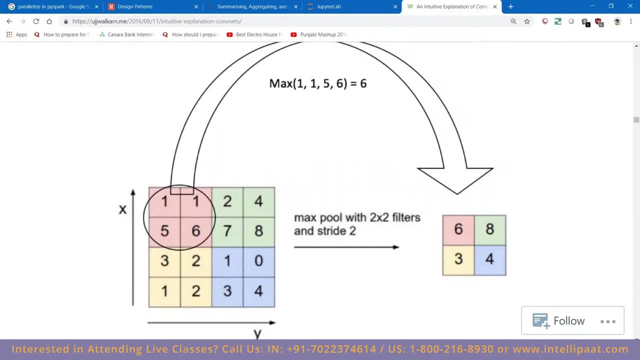 makes sense. even this max pooling thing makes sense. even this max pooling thing has this, has this, has this size that is called two, that you can see size that is called two, that you can see. size that is called two, that you can see right now it's two cross two. right now, it's two cross two. right now it's two cross two and it has strides equal to two. why and it has strides equal to two? why and it has strides equal to two? why? because you don't want to get the. because you don't want to get the. 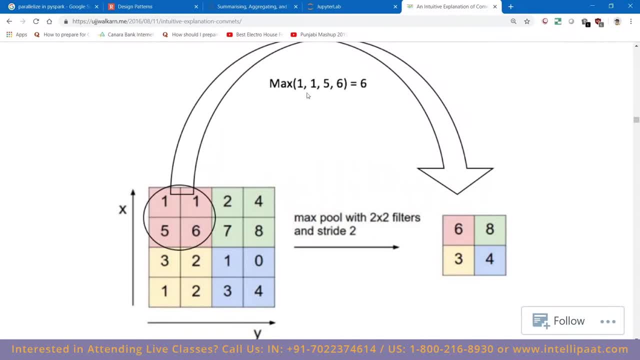 because you don't want to get the maximum number again and again, maximum number again and again, maximum number, again and again. so let's say: if you're taking this once, so let's say. if you're taking this once, so let's say. if you're taking this, once you have taken these values, you should. 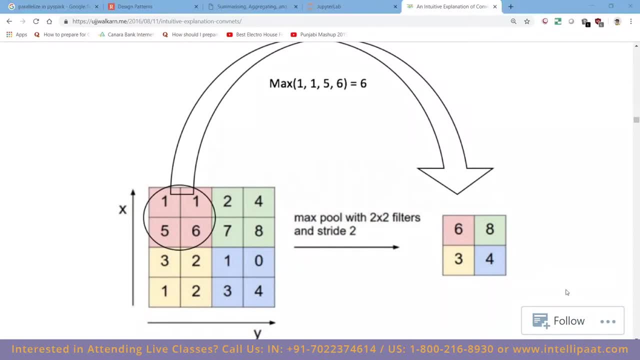 you have taken these values, you should. you have taken these values, you should move to the next move, to the next move, to the next right. so let's say this was the first right. so let's say this was the first right. so let's say this was the first filter of two cross two. and now you have. 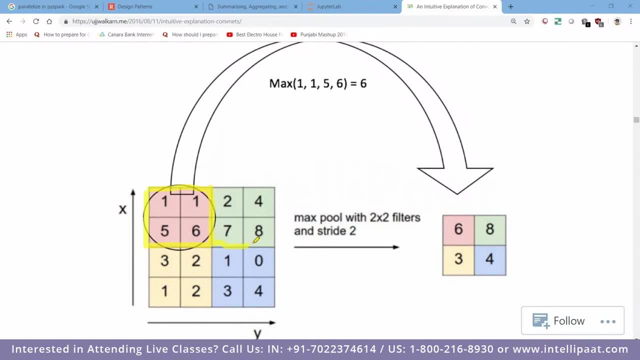 filter of two cross two, and now you have filter of two cross two, and now you have strides of two, which means it will shift strides of two, which means it will shift strides of two, which means it will shift to two to two, to two rows and two columns. so this will be your. 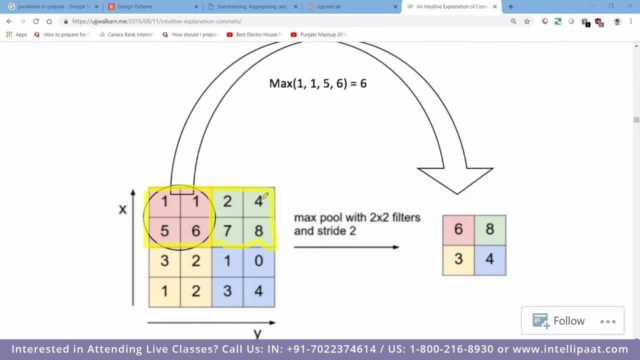 rows and two columns. so this will be your rows and two columns. so this will be your next row column. next question will be next row column. next question will be next row column. next question will be: who's the maximum? you'll say eight. so who's the maximum? you'll say eight. so 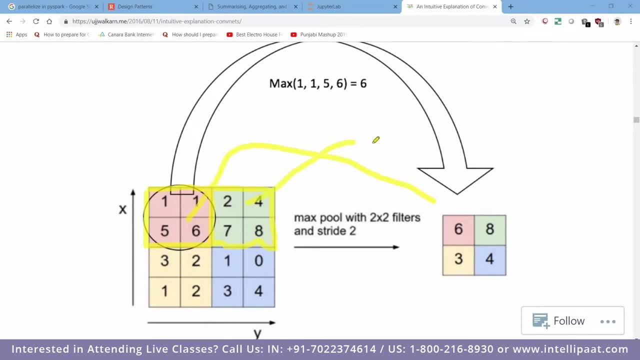 who's the maximum? you'll say eight, so you can see all the values are transferred. you can see all the values are transferred. you can see all the values are transferred from six, from six, from six then eight, then three, then eight, then three, then eight, then three and then four. 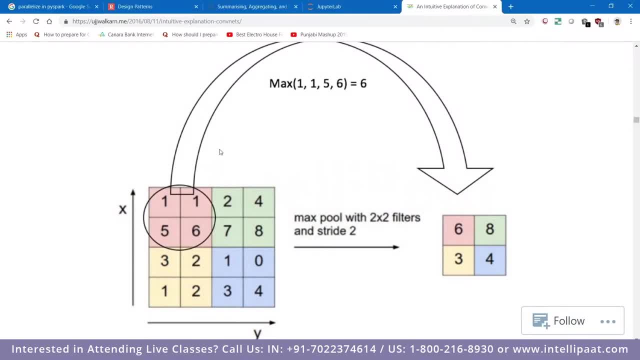 so see, the max pool thing is nothing. but so see, the max pool thing is nothing. but so see, the max pool thing is nothing. but let's say, if we go up again, let's say, if we go up again, let's say, if we go up again, if we go up again, till here where you just 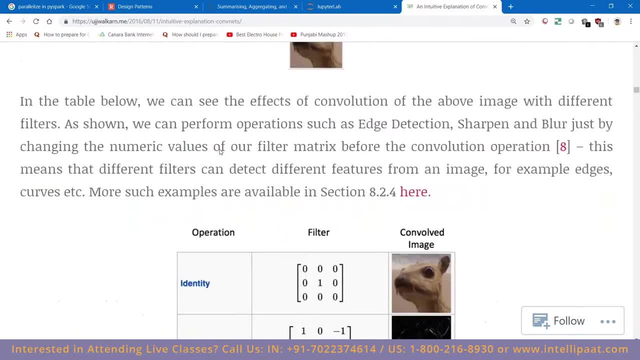 if we go up again till here where you just, if we go up again till here where you just got this new answer from your con. got this new answer from your con. got this new answer from your con. after you have run your filter over your. after you have run your filter over your. 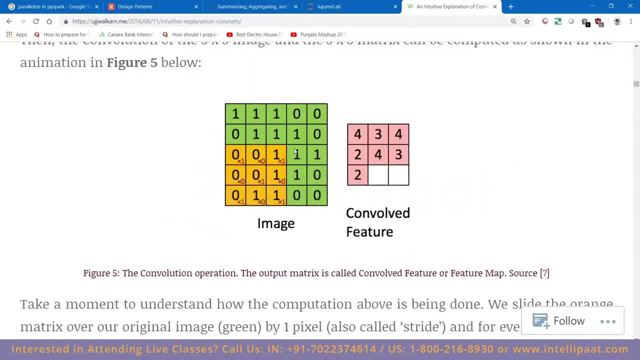 after you have run your filter over your image, image, image. this is called convoluted feature, right? this is called convoluted feature, right? this is called convoluted feature right now. this convoluted filter feature is now. this convoluted filter feature is. 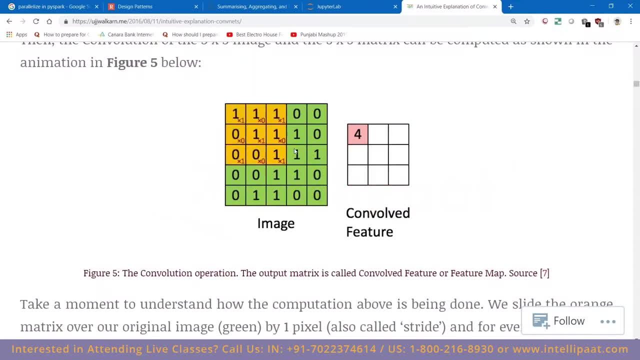 now, this convoluted filter feature is actually nothing but an edgy photograph. actually, nothing but an edgy photograph. actually nothing but an edgy photograph of your original photo, right of your original photo, right of your original photo, right. so it contains more edges, more clear. 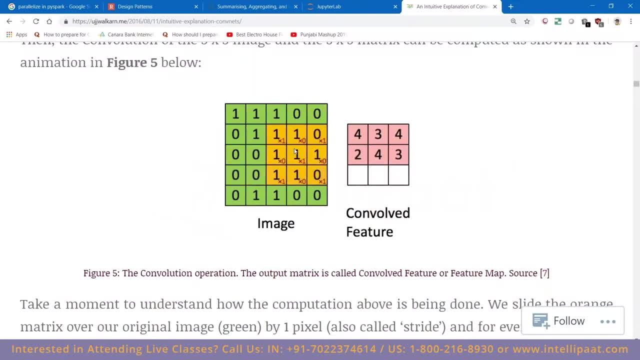 so it contains more edges, more clear. so it contains more edges, more clear edges and more edges and more edges and more things. but they're still not much clear things, but they're still not much clear to you, right? so then you want what do to you, right? so then you want what do. 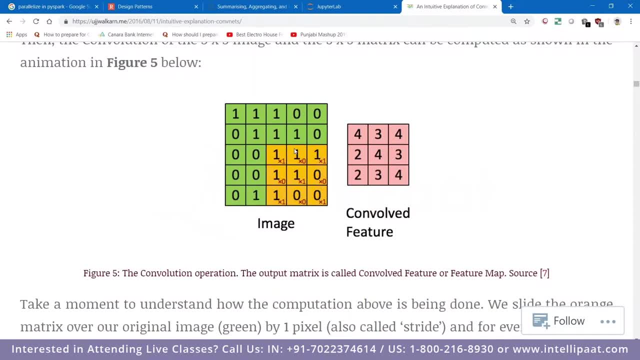 to you, right? so then you want, what do you want to say to the model? is you want to say to the model, is you want to say to the model: is that model, give me more. that model, give me more. that model, give me more, heavier amount of images, give me the. 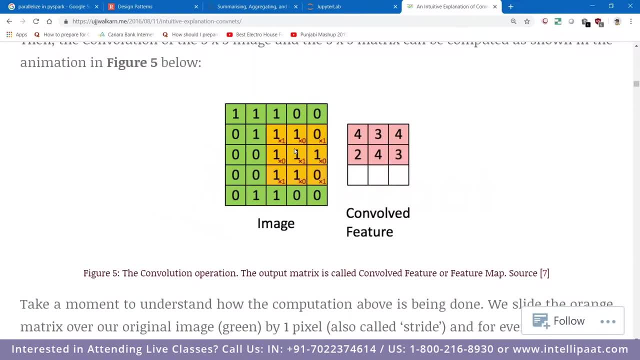 heavier amount of images. give me the heavier amount of images, give me the maximum maximum, maximum number of pixels in a particular area. so number of pixels in a particular area, so number of pixels in a particular area. so you say okay, you say okay, you say okay. so what you're going to do is the final. 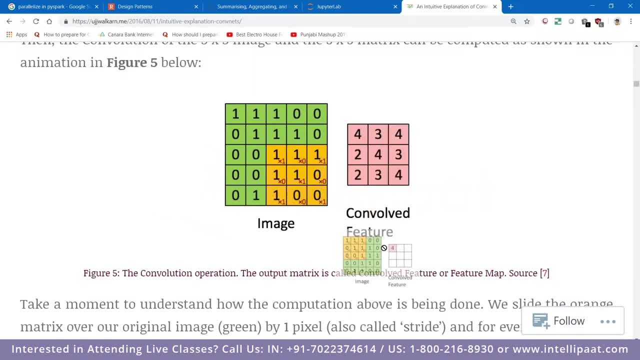 so what you're going to do is the final. so what you're going to do is the final thing that you have here right now in thing, that you have here right now in thing, that you have here right now in the pink, the pink, the pink: four, three, four, two, four, three, uh, 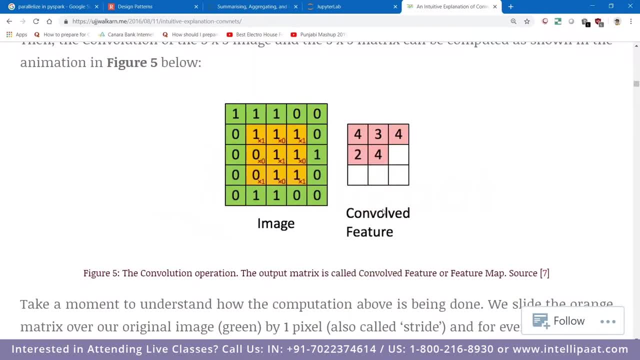 four, three, four, two, four, three, uh, four, three, four, two, four, three, uh, two, three, four. this thing is called a two, three, four. this thing is called a two, three, four. this thing is called a convoluted feature. now you'll go down. convoluted feature. now you'll go down. 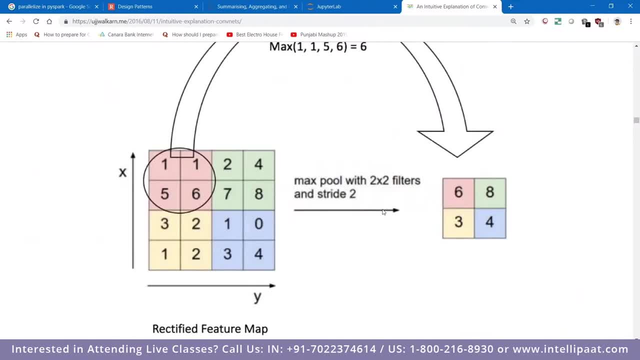 convoluted feature. now you'll go down now, once you have got this image, your now, once you have got this image, your now, once you have got this image, your second step is to take the image. second step is to take the image. second step is to take the image and run again a two cross, two filter over. 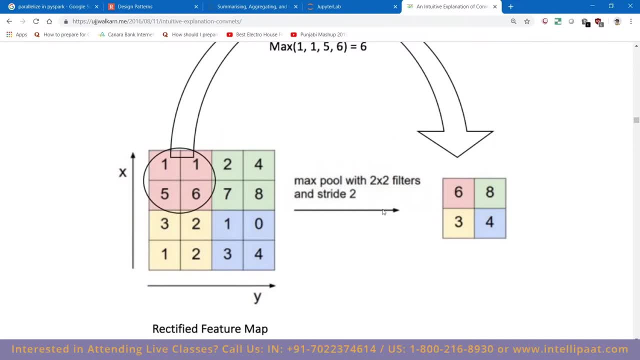 and run again a two cross, two filter over and run again a two cross two filter over it. it, it right, and then with the strides of two, it right, and then with the strides of two, it right, and then with the strides of two. it means the next step is not one step, but 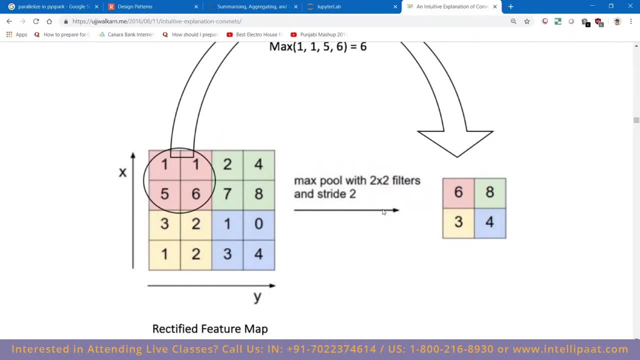 means the next step is not one step, but means the next step is not one step, but two steps right. so your first square: two steps right. so your first square, two steps right. so your first square will be one one, five, six right, this one will be one one five, six, right this one. 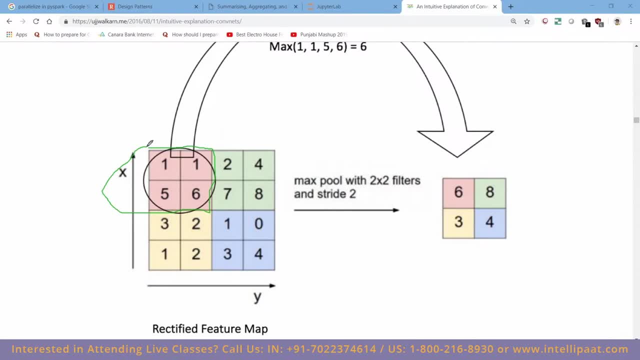 will be one. one, five, six, right. this one. right. this one is the first square. how right, this one is the first square. how right, this one is the first square. how. how much is your total uh maximum number? how much is your total uh maximum number? how much is your total uh maximum number in this one? one, five, six is six, right. 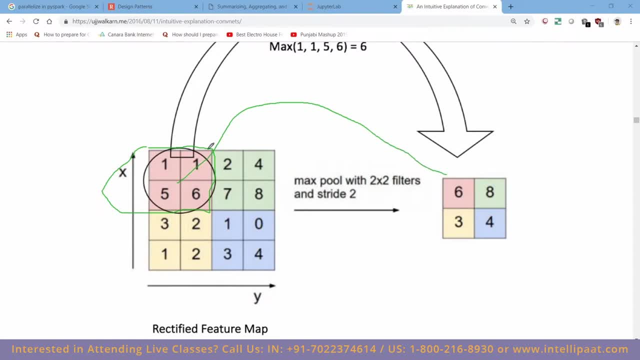 in this one, one, five, six is six right. in this one: one, five, six is six, right. so you give six here, so you give six here, so you give six here. then your second, because it's just tried, then your second, because it's just tried, then your second, because it's just tried, is two. so your next square will become: 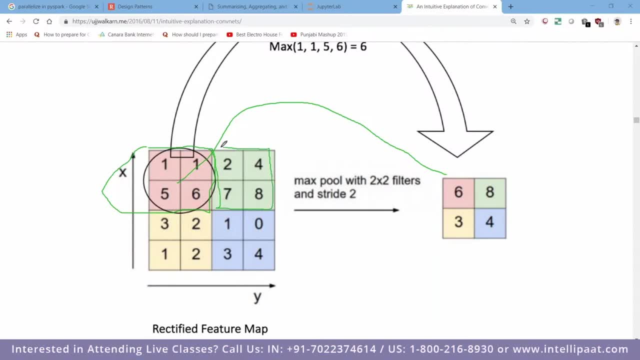 is two, so your next square will become is two, so your next square will become somewhat like this, somewhat like this, somewhat like this: two, four, seven, eight, right. two, four, seven, eight, right. two, four, seven, eight, right. maximum thing is eight, eight will come. maximum thing is eight, eight will come. 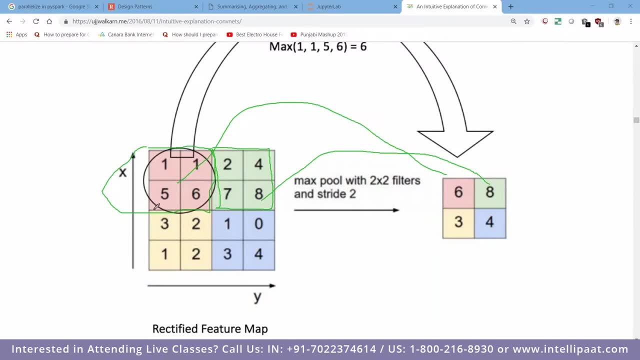 maximum thing is eight. eight will come here here. here you have next thing as three, two, two. you have next thing as three, two, two. you have next thing as three: two, two, one, two, one, two, one, two. then your three is equal to one. sorry, three is not equal to one, but three. 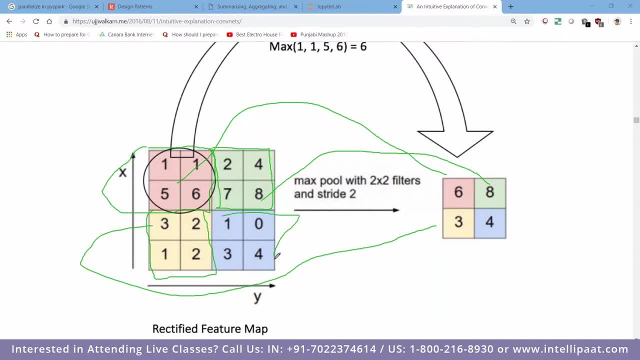 sorry, three is not equal to one, but three. sorry, three is not equal to one, but three. comes here right. comes here right, comes here right. then your fourth square. then this is a. then your fourth square, then this is a. then your fourth square, then this is a four square: one, zero, three, four, which is 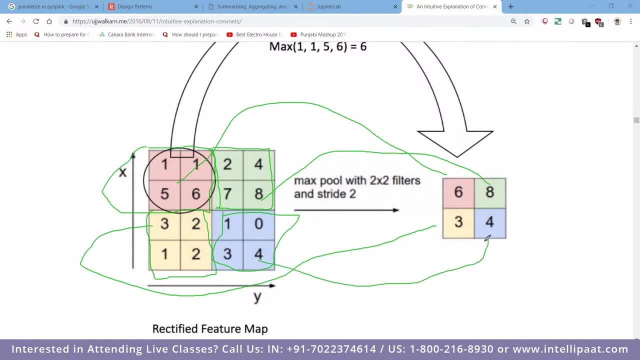 four square one, zero three. four, which is four square one, zero three. four, which is the maximum value four, the maximum value four, the maximum value four. four is shifted here. so let's four is shifted here. so let's four is shifted here. so let's zoom out of this and then let's try to. zoom out of this and then let's try to zoom out of this and then let's try to cover them one by one. what we have missed, cover them one by one. what we have missed, cover them one by one what we have missed till now, till now. 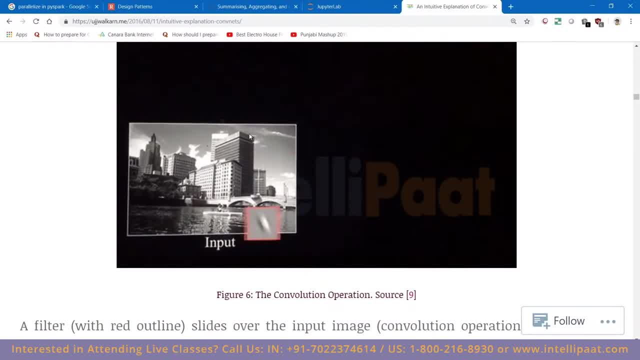 till now. so see whenever you're running this, this. so see whenever you're running this, this. so see whenever you're running this, this thing that you're seeing on your screen, thing that you're seeing on your screen, thing that you're seeing on your screen, this filter whenever you're running. 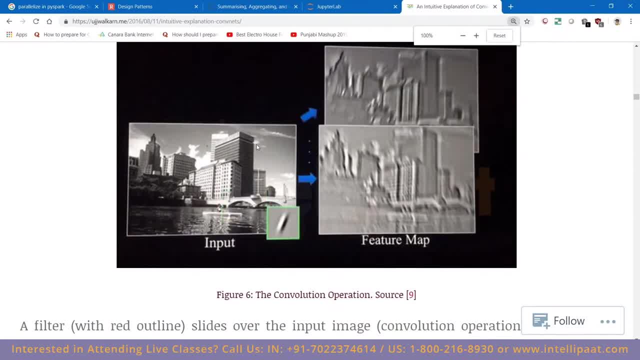 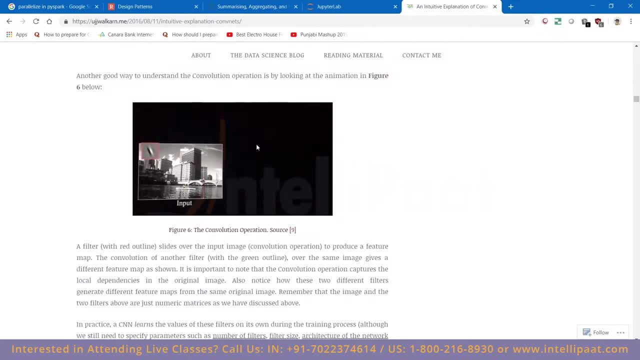 this filter whenever you're running this. you will never run a single filter. you will never run a single filter. you will never run a single filter on your image. this is what cnn is you will run. this is what cnn is you will run. this is what cnn is. you will run multiple filters with multiple different. 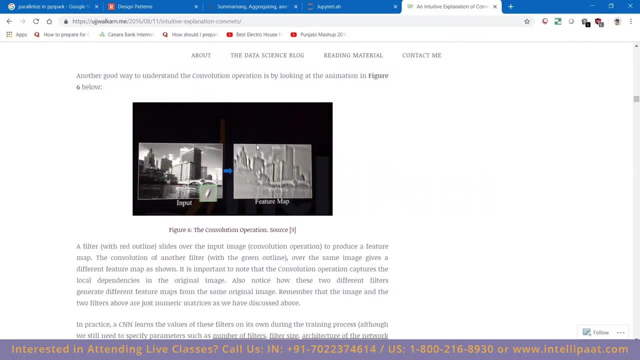 multiple filters with multiple different multiple filters with multiple different, different values, different values, different values, and that thing is known as the depth of, and that thing is known as the depth of, and that thing is known as the depth of the cnn, the cnn, the cnn. so, whenever you will say that from kiras, 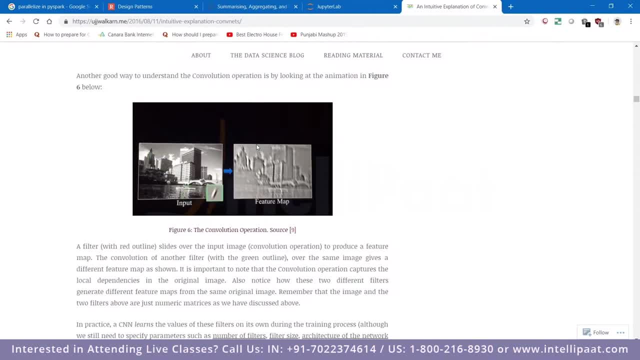 so whenever you will say that from kiras, so whenever you will say that from kiras, dot layers, import cnn dot layers, import cnn dot layers, import cnn. right or conf 2d, it's actually the name. right or conf 2d, it's actually the name. 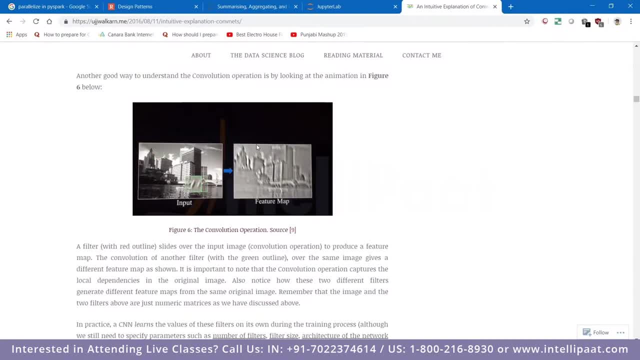 right or conf 2d. it's actually the name in the kiras library for this particular in the kiras library, for this particular in the kiras library, for this particular layer is called conv 2d- c-o-n-v layer is called conv 2d- c-o-n-v. 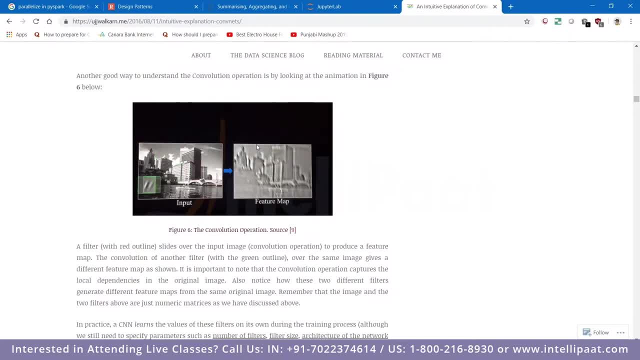 layer is called conv. 2d, c-o-n-v for convolution, c-o-n-v for convolution, c-o-n-v for convolution, c-o-n-v, and then 2d, so it means that you are, and then 2d, so it means that you are. 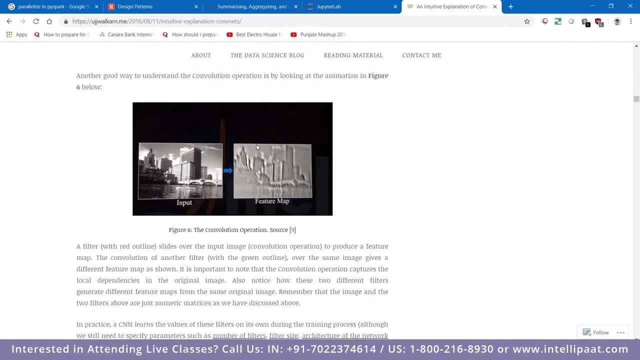 and then 2d. so it means that you are using convolution neural network for 2d, using convolution neural network for 2d, using convolution neural network for 2d. images right, images, right images right. so what you will do is at that instance. so what you will do is at that instance. 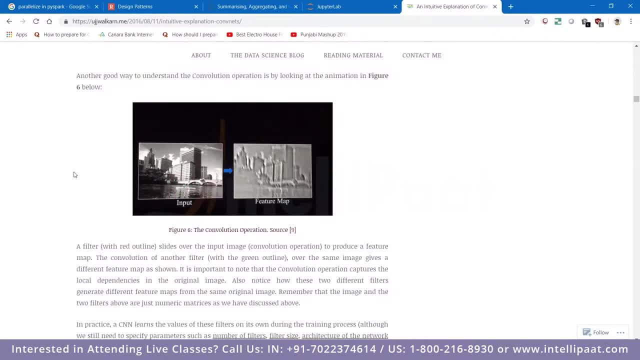 so what you will do is at that instance, it will ask you that how many filters do? it will ask you that how many filters do? it will ask you that: how many filters do you want to run on your? you want to run on your? you want to run on your image? how many random? 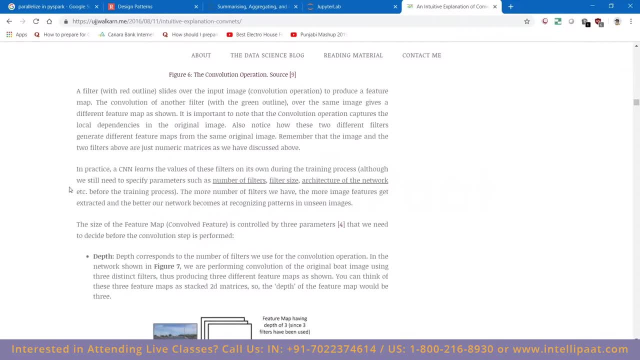 image. how many random image. how many random filters do you want to run? that is called filters. do you want to run that is called filters? do you want to run that is called the depth of the filter. the depth of the filter. the depth of the filter right now. imagine this photo here, that 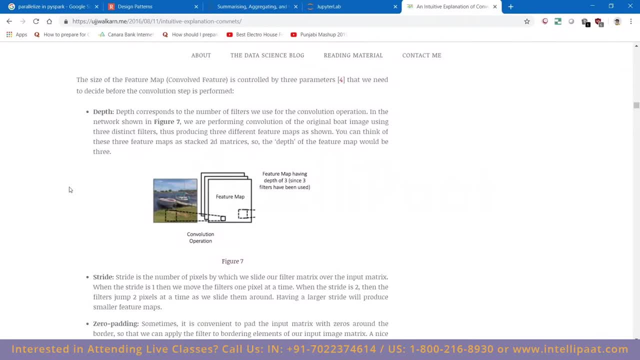 right now imagine this photo here. that right now, imagine this photo here that you're seeing here, is you're seeing here, is you're seeing here, is: this is a image of a boat that is: this is a image of a boat that is: this is a image of a boat that is standing somewhere near the deck. 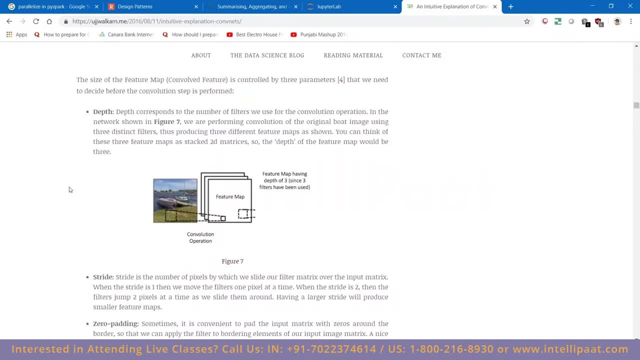 standing somewhere near the deck. standing somewhere near the deck and you can see water and some grass now, and you can see water and some grass now, and you can see water and some grass now. what it is is that right now, you have a. what it is is that right now you have a. 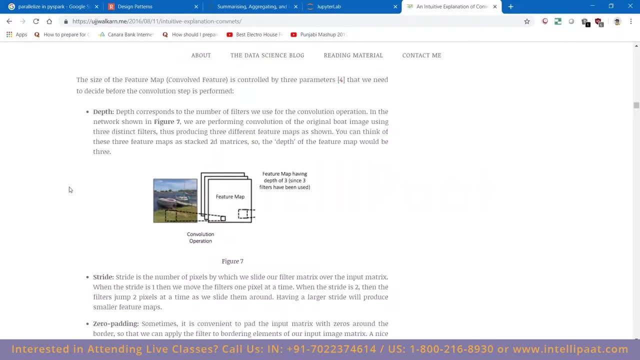 what it is is that right now you have a depth of three. it means three different depth of three. it means three different depth of three. it means three different filters will run on this image and they filters will run on this image and they filters will run on this image and they will produce three different convoluted. 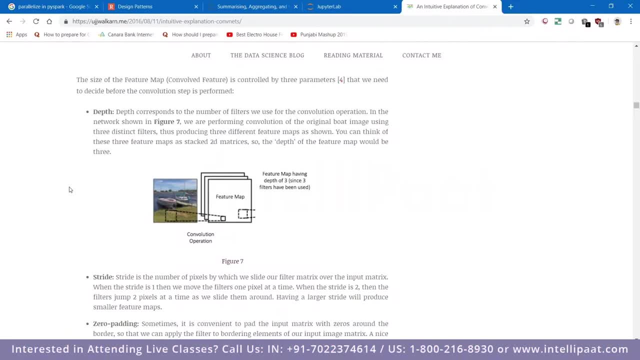 will produce three different convoluted, will produce three different convoluted images, images, images. did i make sense here? did i make sense here? did i make sense here? imagine that this thing is called as the imagine, that this thing is called as the imagine, that this thing is called as the depth of the convolution, now, depth of. 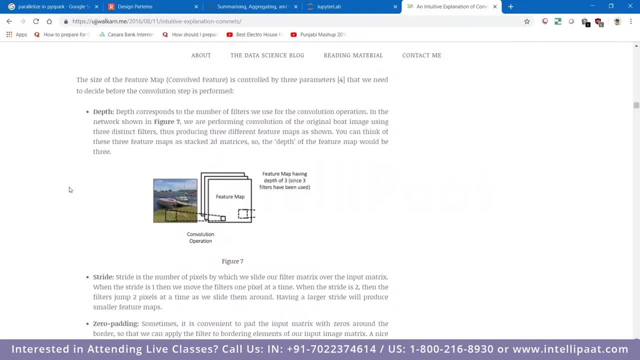 depth of the convolution, now, depth of depth of the convolution, now depth of the convolution, means that right now till the convolution, means that right now till the convolution, means that right now till till this- before this example, we were till this. before this example, we were till this. before this example, we were running only one convolution: right. 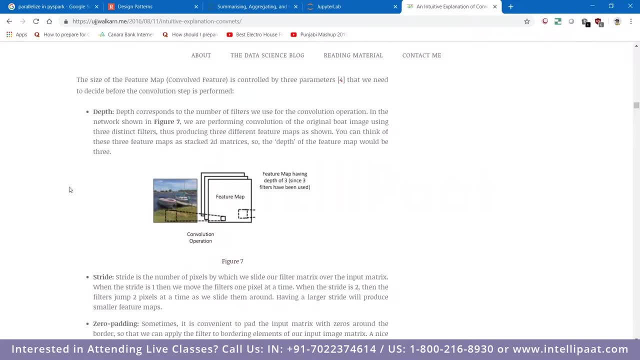 running only one convolution right. running only one convolution- right. we were running only one filter over the. we were running only one filter over the. we were running only one filter over the image and we were getting only one image. and we were getting only one image and we were getting only one output of that image, right. 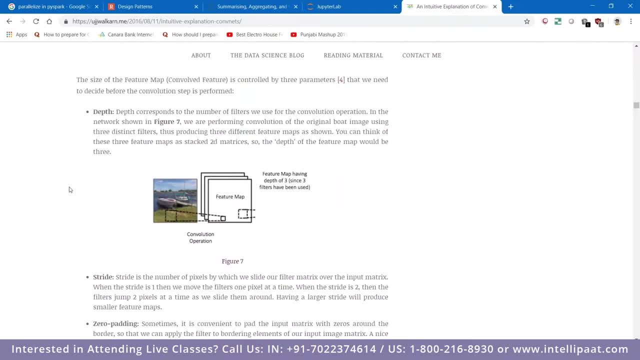 output of that image right. output of that image right now. what the model is saying that. we will now what the model is saying that we will now what the model is saying that we will not run one, but we will run multiple. not run one, but we will run multiple. 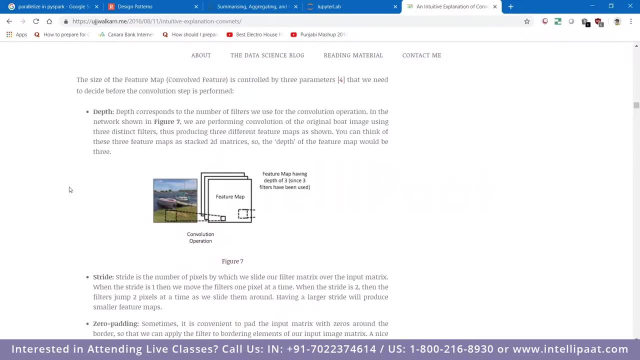 not run one, but we will run multiple. so in this example that you are seeing in, so in this example that you are seeing in, so in this example that you are seeing in front of your images, right in your front of your images, right in your front of your images, right in your screens, right now, where this you have a 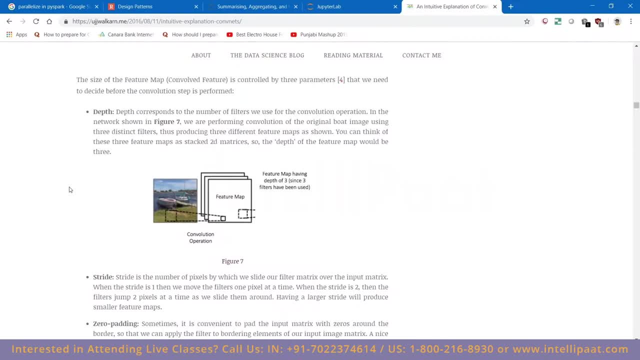 screens right now where this you have a screens right now where this you have a boat inside, where you have a boat near boat inside, where you have a boat near boat inside, where you have a boat near the near the surface of the earth, the near the surface of the earth. 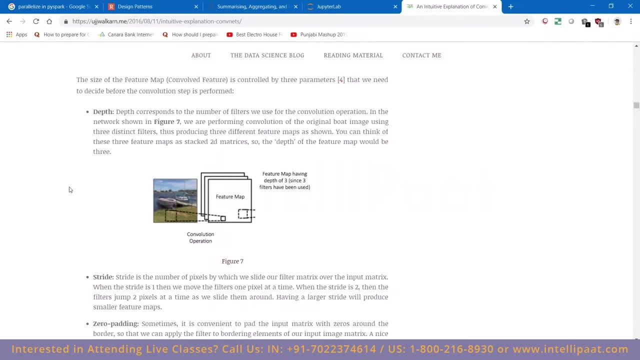 the near the surface of the earth. you are running three different filters. you are running three different filters. you are running three different filters. and for running three different filters. and for running three different filters and for running three different filters. you will get three different convoluted. 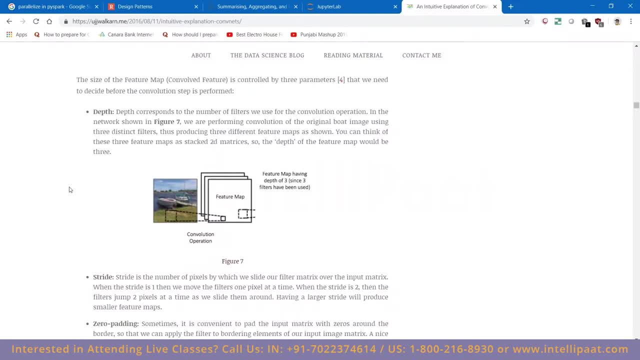 you will get three different convoluted. you will get three different convoluted features. features, features, right, right, right. so you cannot control the value that. so you cannot control the value that. so you cannot control the value that. what is going inside the? what is going inside the? 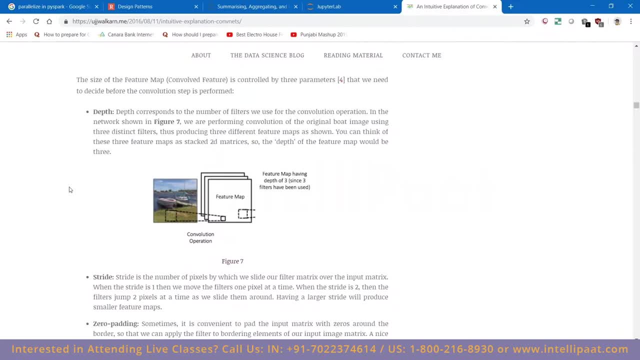 what is going inside the? i mean what is the value of those filters? i mean, what is the value of those filters? i mean, what is the value of those filters? but, yes, you have to definitely tell the but. yes, you have to definitely tell the but, yes, you have to definitely tell the model that i want to take these many 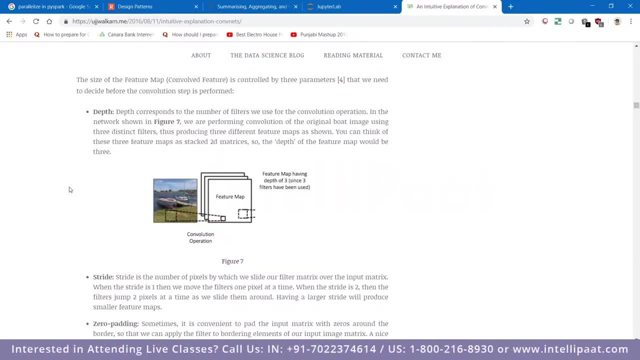 model that i want to take these many model that i want to take these many, uh, a number of filters, uh, a number of filters, uh, a number of filters, because this will increase the depth of, because this will increase the depth of, because this will increase the depth of your 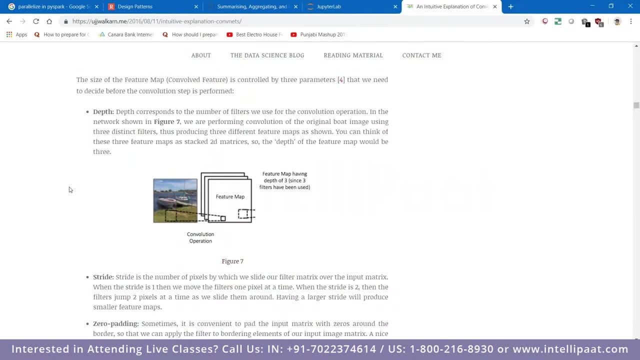 your, your model right. so you will say, let's say i model right. so you will say, let's say i model right. so you will say let's say i want to take 25, want to take 25, want to take 25 different depth of the model, or i want: 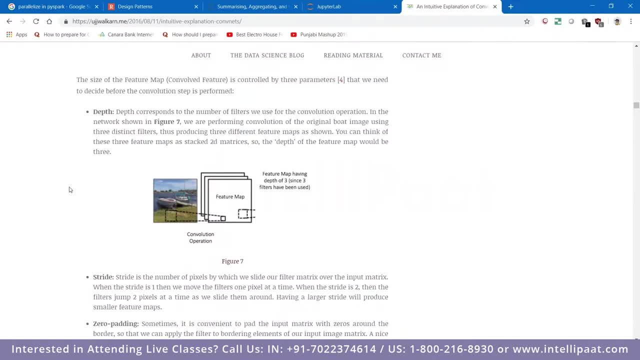 different depth of the model, or i want different depth of the model, or i want to take, to take, to take thousand depth. you know, for the first thousand depth, you know for the first thousand depth, you know, for the first image, i want to have thousand uh image. i want to have thousand uh. 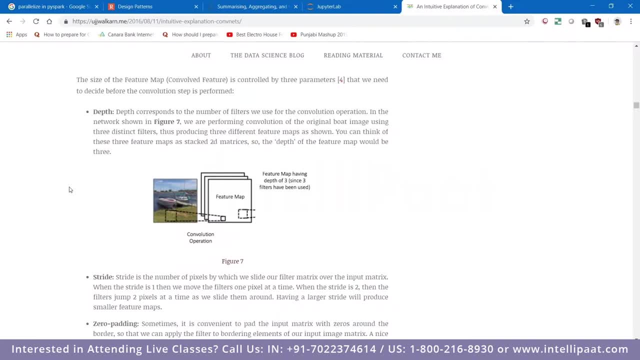 image. i want to have thousand, uh, different, different convolution filters, different, different convolution filters, different, different convolution filters, because eventually their size is, because eventually their size is, because eventually their size is decreasing, if you, if you see decreasing, if you, if you see decreasing, if you, if you see closely, if you, if you, if you remember the 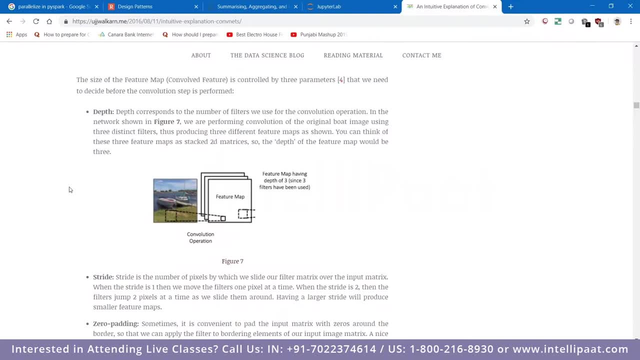 closely, if you, if you, if you remember the closely, if you, if you, if you remember the gif, gif, gif. the height and width of the image is going. the height and width of the image is going. the height and width of the image is going to decrease, right, but the depth is. 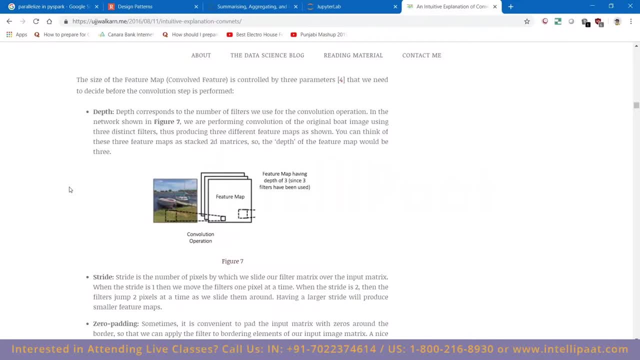 to decrease, right, but the depth is to decrease, right, but the depth is going to increase so earlier. let's say if going to increase so earlier. let's say if going to increase so earlier. let's say: if the image was of 1d, the image was of 1d. 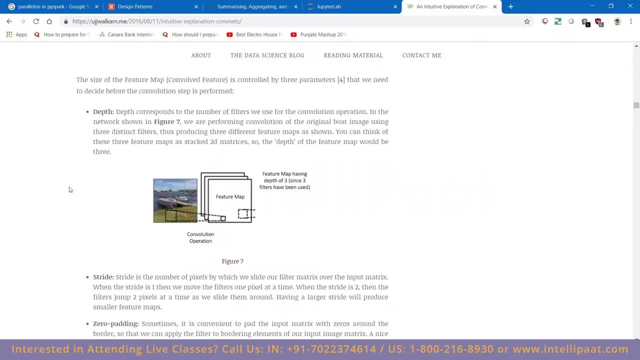 the image was of 1d. sorry with one channel. now it is going to sorry with one channel. now it is going to sorry with one channel. now it is going to convert it into three channel image. convert it into three channel image. convert it into three channel image because you have run three uh, three uh. 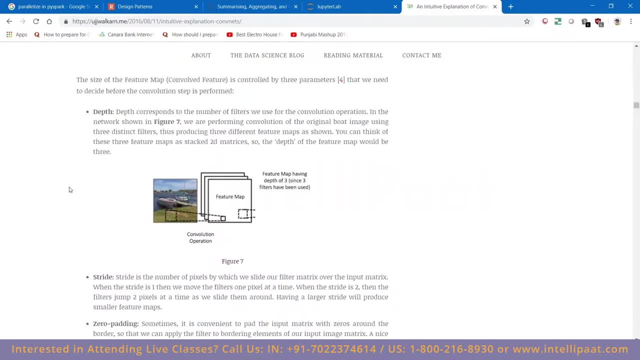 because you have run three uh, three uh, because you have run three uh three uh filters on it. let's say you ran 500 filters on it. let's say you ran 500 filters on it. let's say you ran 500 filters. so for one image you will have. 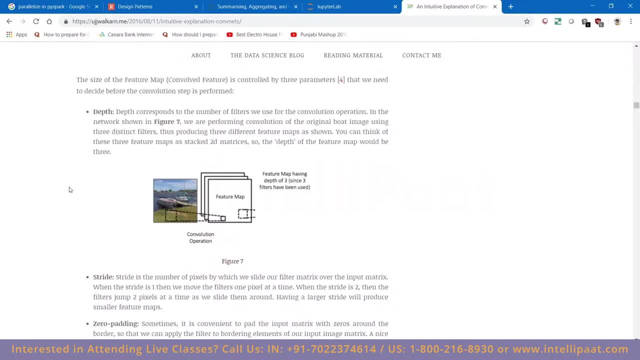 filters. so for one image, you will have filters. so for one image, you will have 500 different outputs, 500 different outputs, 500 different outputs, right? so see why we are increasing the right. so see why we are increasing the right. so see why we are increasing the depth is because the ultimately 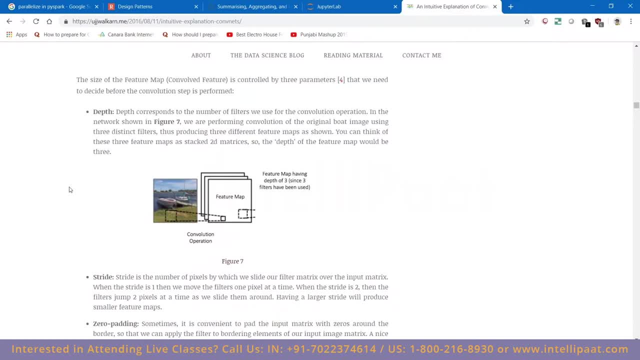 depth is because the ultimately depth is because the ultimately the model needs to get some or the other, the model needs to get some or the other, the model needs to get some or the other. uh, you know, final uh decision thing see. uh, you know, final uh decision thing see. 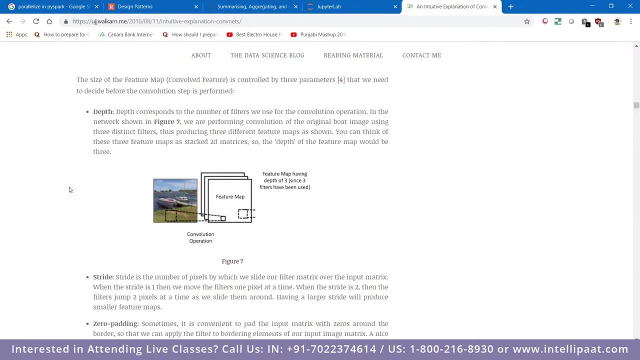 uh, you know, final, uh, decision thing, see, ultimately the decision is taken by the, ultimately the decision is taken by the, ultimately the decision is taken by the last layer right, last layer right, last layer right. and you remember that, you have to, and you remember that you have to. 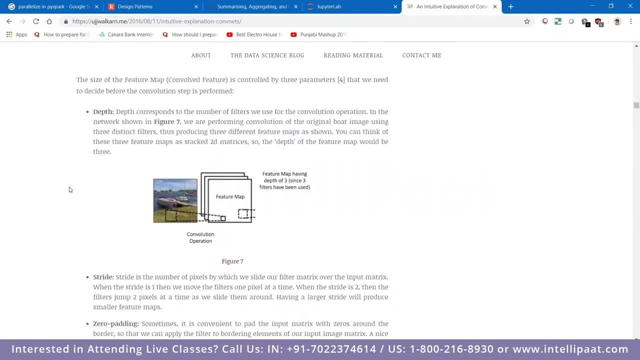 and you remember that you have to ultimately mold your model to take, to ultimately mold your model to take, to ultimately mold your model to take to the dense layer, the dense layer, and you remember the and you remember the and you remember the dense layer, are nothing but a single. 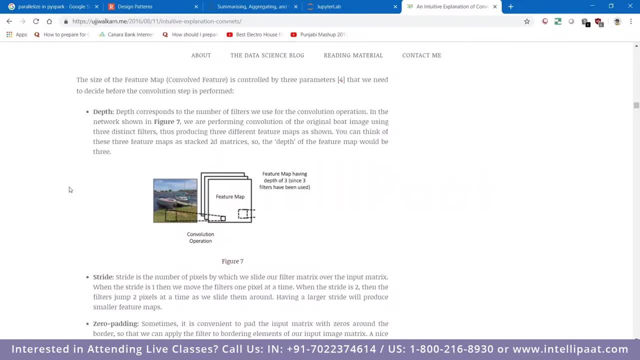 dense layer are nothing but a single dense layer are nothing but a single column, rows, column, rows, column, rows, right. so when i say dense 1024, it means right. so when i say dense 1024, it means right. so when i say dense 1024, it means that this is a one column. 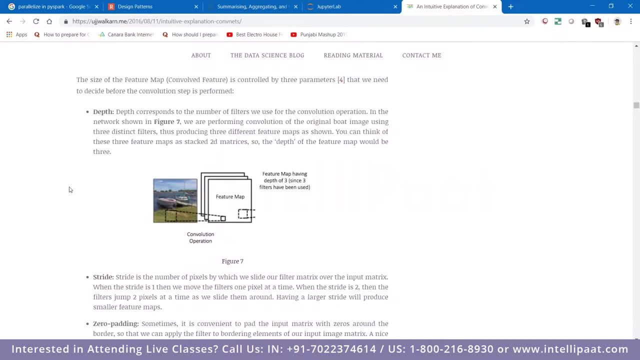 that this is a one column, that this is a one column, but 1024 different uh. but 1024 different uh. but 1024 different uh. 1024 different uh. rows are there standing, so you 1024 different uh rows are there standing, so you. 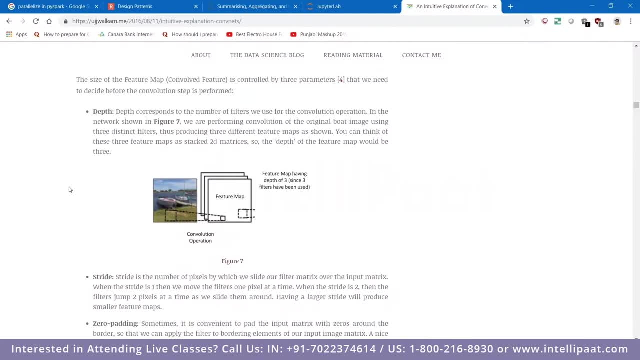 1024 different uh rows are there standing. so you can imagine 1024 blocks, can imagine 1024 blocks. can imagine 1024 blocks, one one over the above right. so you have one one over the above right. so you have one one over the above right. so you have to somehow. 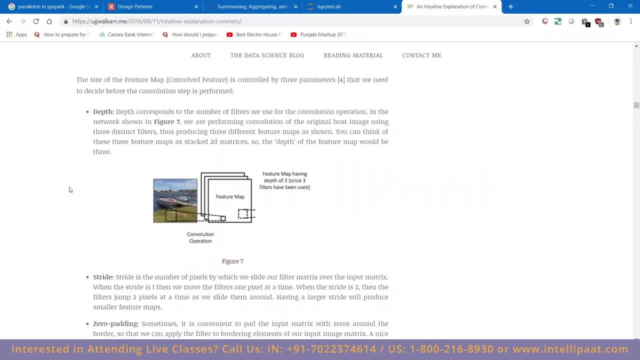 to somehow, to somehow, converge your model to have, so you're converge your model to have, so you're converge your model to have, so you're converging your 2d image which has height, converging your 2d image which has height, converging your 2d image which has height and depth. 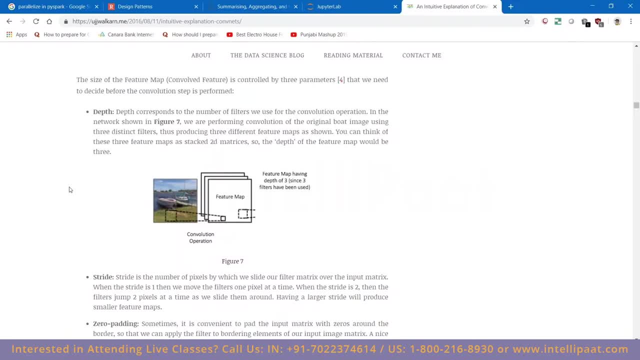 and depth and depth. when you want to convert it into a depth, when you want to convert it into a depth, when you want to convert it into a depth, only, only only thing right, so let's say that your image thing right, so let's say that your image. 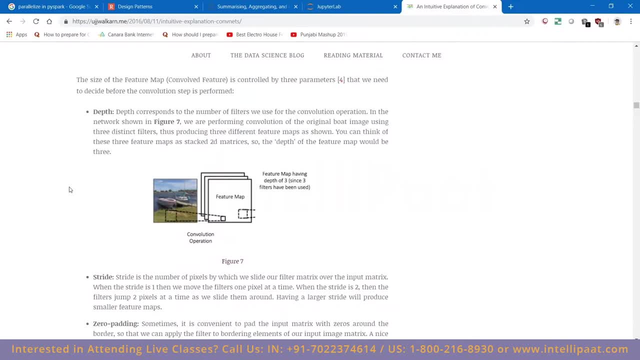 thing right. so let's say that your image was somewhat here, like 50 cross 15, was somewhat here like 50 cross 15, was somewhat here, like 50 cross 15. so what you're eventually doing is so. what you're eventually doing is so. what you're eventually doing is whenever you run a convolution filter. whenever you run a convolution filter. whenever you run a convolution filter, you're reducing its size to, let's say, 35. you're reducing its size to, let's say, 35. you're reducing its size to, let's say 35 plus 35 plus 35. 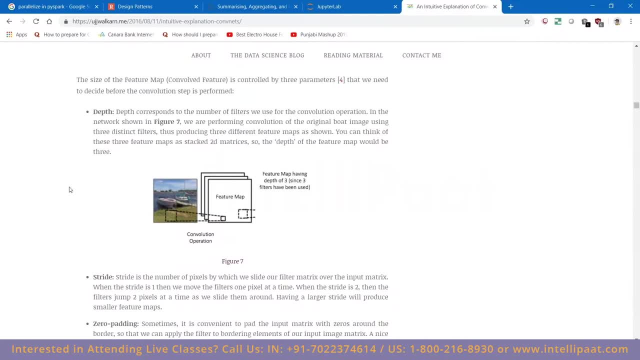 plus 35, but when that image is converted into 35, but when that image is converted into 35, but when that image is converted into 35 plus 35, you're increasing the depth of it plus 35. you're increasing the depth of it plus 35. you're increasing the depth of it because you're not running single. 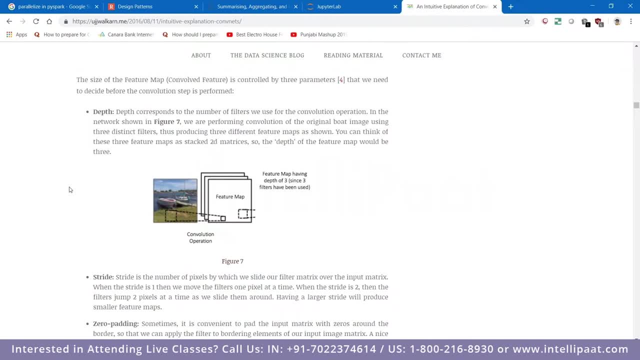 because you're not running single, because you're not running single convolution filter, because you're convolution filter, because you're convolution filter because you're running, let's say, 10 running, let's say 10 running, let's say 10. so so, if, if, the if, if the original size, 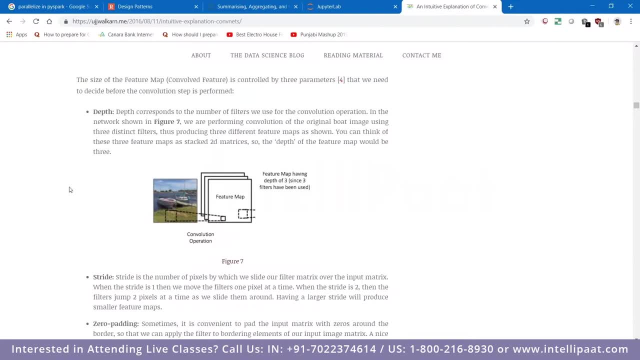 so. so, if, if the, if the original size, so so, if, if the, if the original size was 50 cross 50, now it was converted. was 50 cross 50, now it was converted. was 50 cross 50, now it was converted into 35, into 35, into 10. into 35, into 35, into 10, into 35, into 35, into 10. right, when you will run more, it will right. when you will run more, it will right. when you will run more, it will convert it into, let's say, convert it into. let's say: 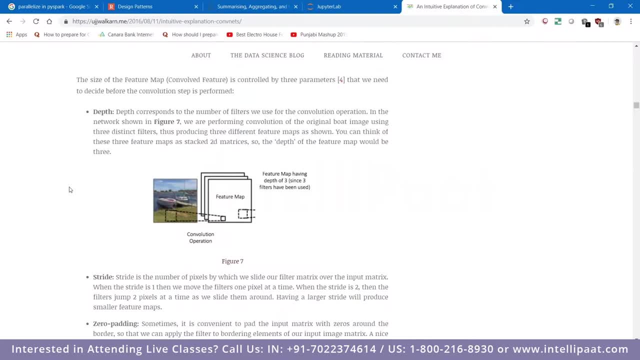 convert it into, let's say, 15 into 15 into 100 right, and then 15 into 15 into 100 right, and then 15 into 15 into 100 right, and then eventually, you will be having only one, eventually you will be having only one. 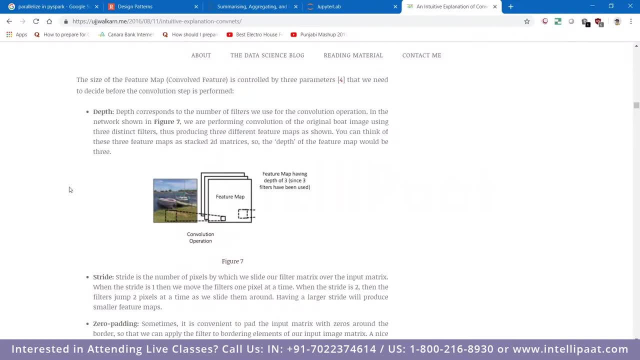 eventually, you will be having only one cross one cross hundred. cross one cross hundred. cross one cross hundred, rather than you know running one, rather than you know running one, rather than you know running one convolution filter, and having only one convolution filter and having only one convolution filter and having only one answer to the model, what we are doing is 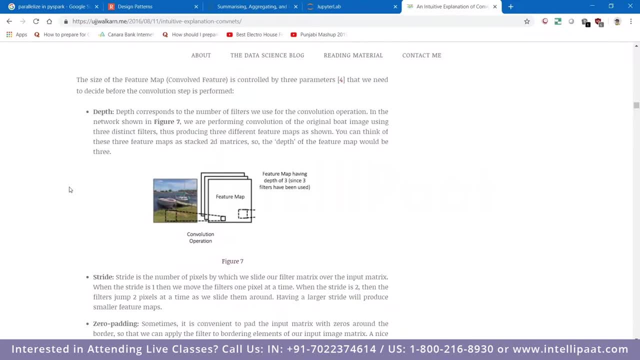 answer to the model. what we are doing is answer to the model. what we are doing is we are running 10 and hundreds of, we are running 10 and hundreds of. we are running 10 and hundreds of filters so that eventually we are like filters, so that eventually we are like. 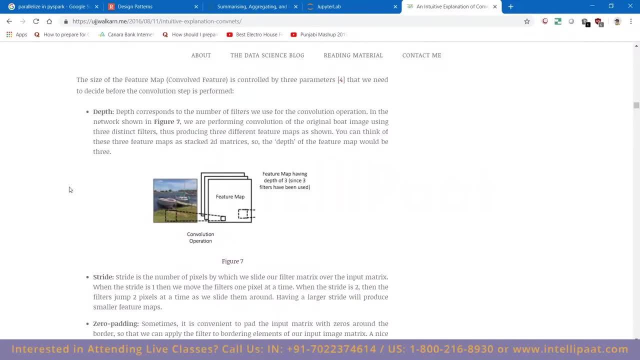 filters, so that eventually we are like, in the end we are clubbing them all. so in the end we are clubbing them all. so in the end we are clubbing them all so that we can. so if you have, if you, if that we can. so if you have, if you, if. 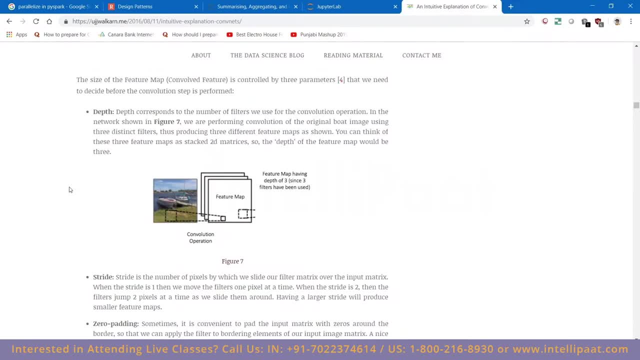 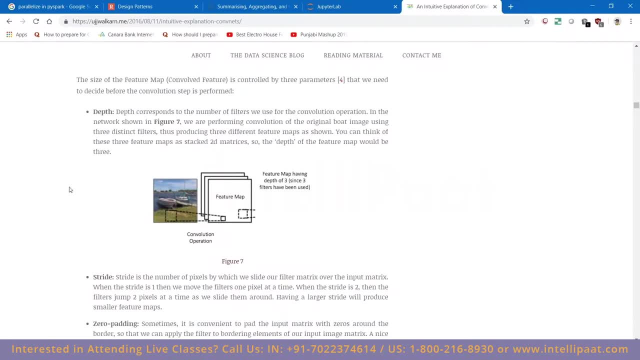 have heard of this thing called ensembling of all the models right. ensembling of all the models, right, ensembling of all the models, right. so let's say that you don't. you don't, so let's say that you don't. you don't, so let's say that you don't. you don't want to trust only one model, but you. 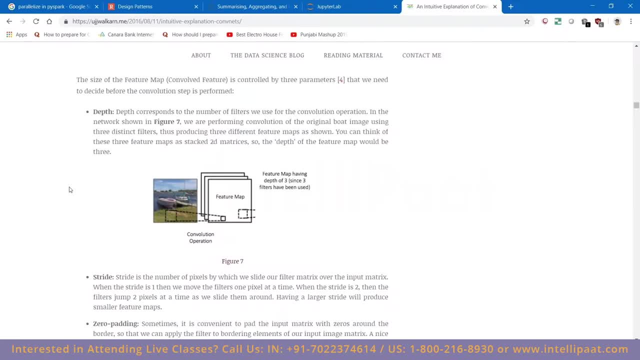 want to trust only one model, but you want to trust only one model, but you build three different models and then build three different models, and then build three different models, and then you club all these models. this is what you club all these models. this is what you club all these models. this is what is happening here also. we are not 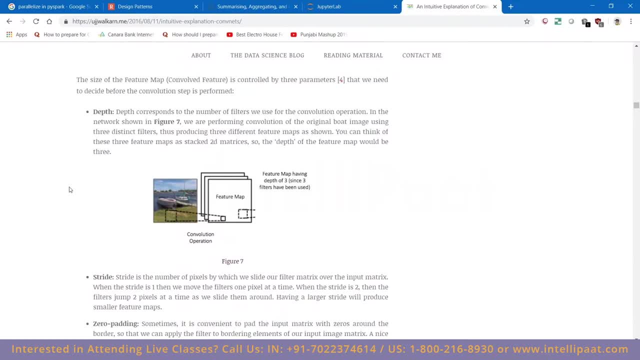 is happening here also. we are not is happening here also. we are not running only one filter, but we are running only one filter, but we are running only one filter, but we are running 100 different filters, and then at running 100 different filters, and then at 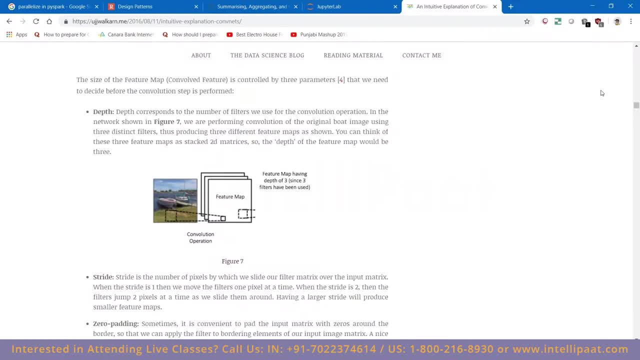 running 100 different filters and then at the end we are clubbing all their the end. we are clubbing all their the end. we are clubbing all their results, right? uh, let me just scroll it results, right? uh, let me just scroll it results, right? uh, let me just scroll it up. so when i say filter or feature, i 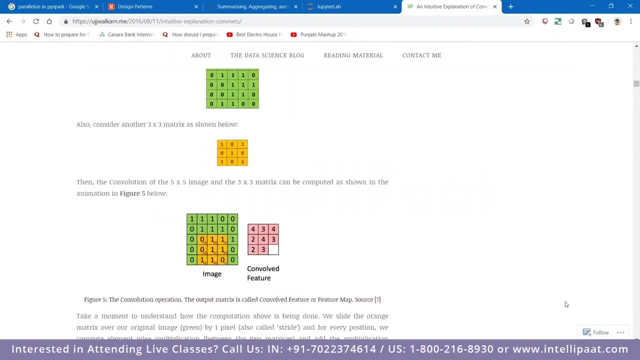 up. so when i say filter or feature, i up. so when i say filter or feature, i mean this thing, this uh, this small mean this thing. this uh, this small mean this thing, this uh, this small yellow thing that is not known to us, yellow thing that is not known to us. 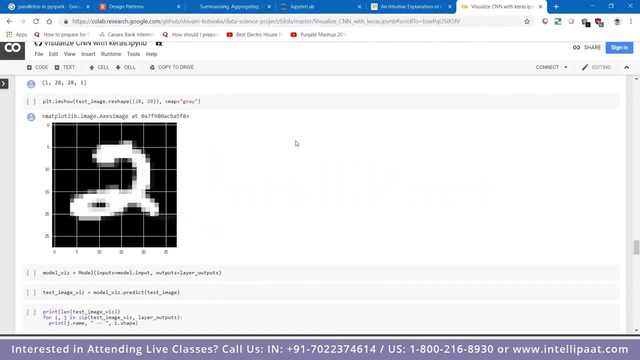 yellow thing that is not known to us. this is the random matrix that we know. this is the random matrix that we know. this is the random matrix that we know. okay, now coming back to the problem. okay, now coming back to the problem. okay, now coming back to the problem, where we were. that, if you are doing, where we were, that if you are doing where we were, that, if you are doing, let's say you have done the con. let's say you have done the con, let's say you have done the con. you have just ran a filter over your image. you have just ran a filter over your image. 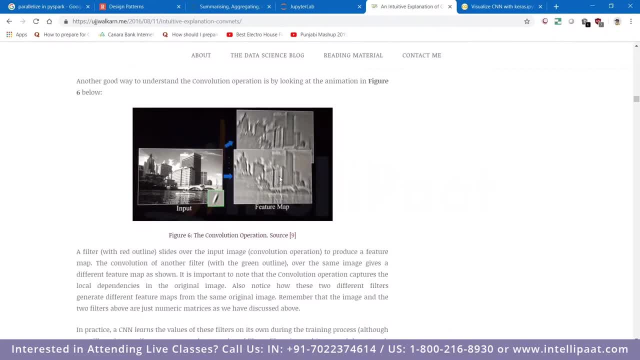 you have just ran a filter over your image and your image is converted from this and your image is converted from this, and your image is converted from this simple image to this simple image, to this simple image, to this more enhanced edgy image right. more enhanced edgy image right. 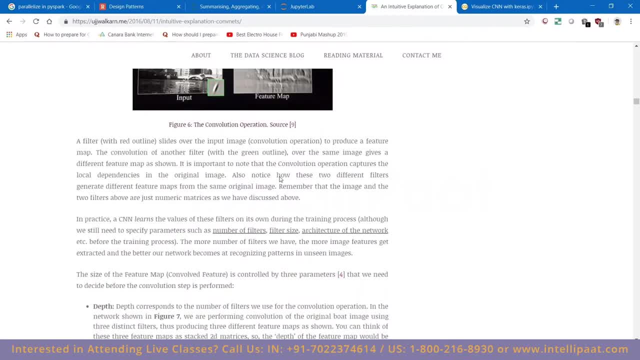 more enhanced edgy image right now, if you go more now, if you go more now, if you go more thing out. so first thing that you were thing out, so first thing that you were thing out, so first thing that you were doing, was what that was called depth. 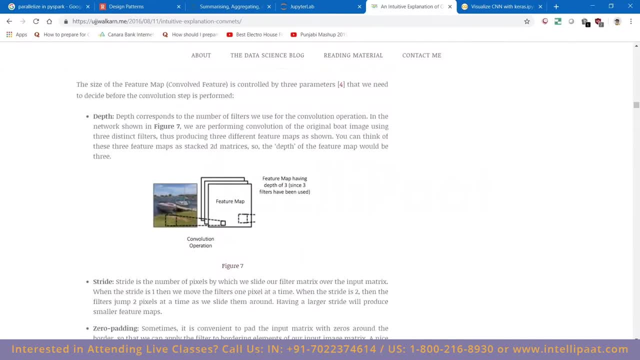 doing was what that was called depth. doing was what that was called depth. now, what is depth? depth means just that. now, what is depth? depth means just that. now, what is depth? depth means just that if you are running different, different, if you are running different, different, if you are running different, different types of convolution, filters of our on. 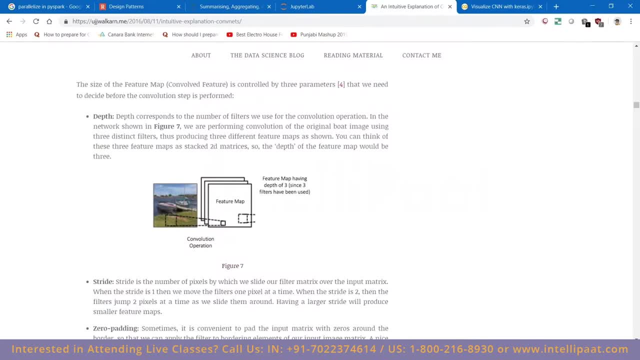 types of convolution filters of our. on types of convolution filters of our. on our images, our images, our images, then you'll get different results right. then you'll get different results right, then you'll get different results right. so if i'm saying i'm running a depth of 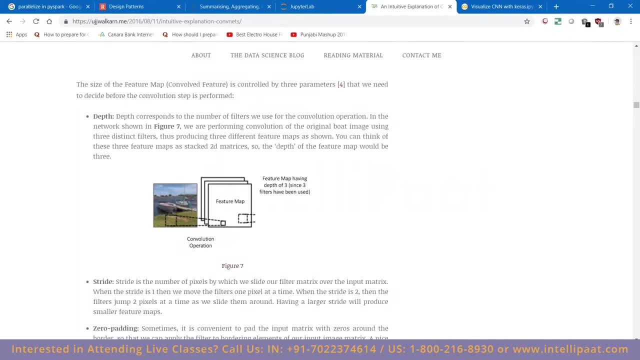 so if i'm saying i'm running a depth of so if i'm saying i'm running a depth of 64, i mean i have 64 different features. 64 i mean i have 64 different features. 64 i mean i have 64 different features which i ran over my image and they gave. 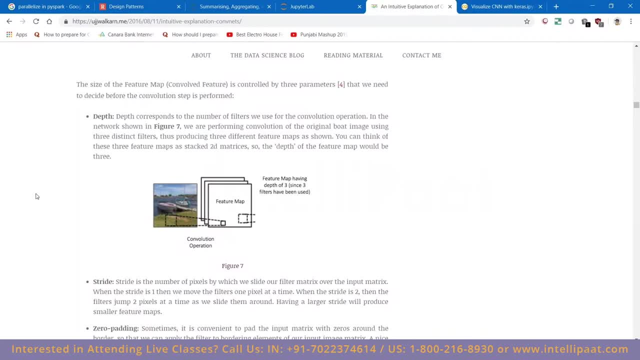 which i ran over my image and they gave which. i ran over my image and they gave me the output me, the output me, the output. right. second thing is strides, yes, strides. right second thing is strides, yes, strides. right second thing is strides, yes, strides. we already know, strides is what. 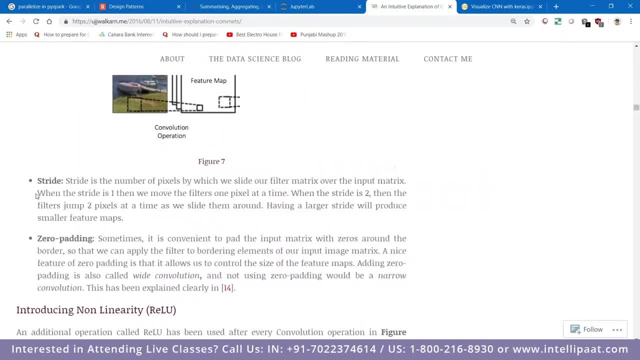 we already know. strides is what we already know. strides is what. strides is the step size. strides is the step size. strides is the step size that. how many jumps do you does? do you that? how many jumps do you does? do you that? how many jumps do you does? do you want your filter to move? 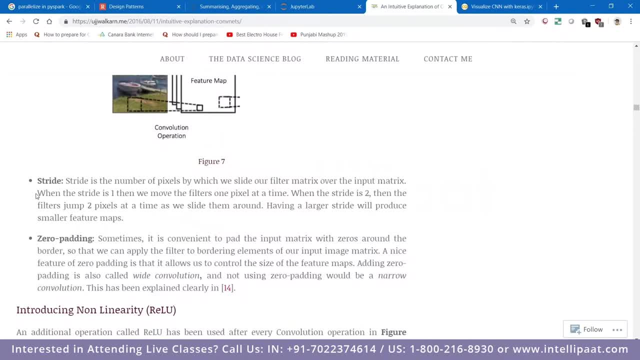 want your filter to move, want your filter to move. so in the gif we were seeing that our so in the gif we were seeing that our so in the gif, we were seeing that our model was shifting with model was shifting with. model was shifting with one space right, one space to the 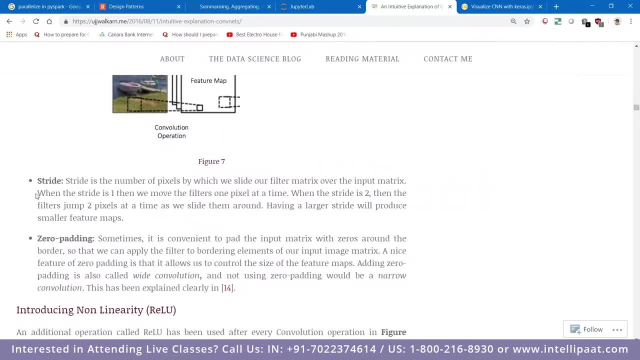 one space right, one space to the one space right, one space to the right. it was shifting so that time it right. it was shifting so that time it right. it was shifting so that time it was tried equal to one, but if you do was tried equal to one, but if you do. 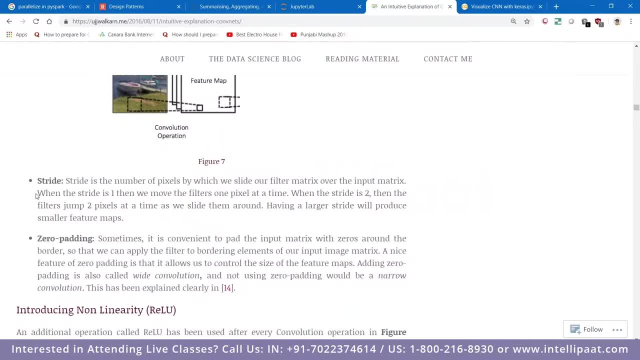 was tried equal to one. but if you do strike two, it means that which is going strike two. it means that which is going strike two. it means that which is going to jump. it is going to take two steps to jump. it is going to take two steps. 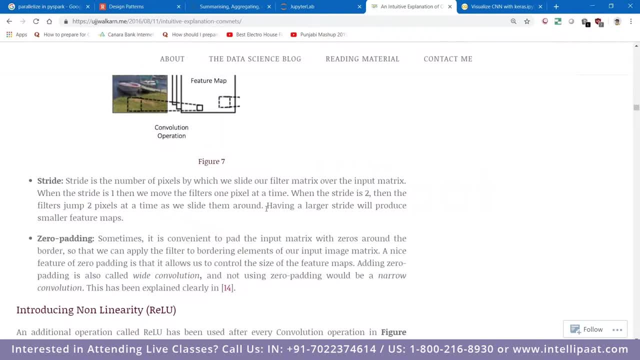 to jump. it is going to take two steps. right, right, right. oh then we have one of the important. oh, then we have one of the important. oh, then we have one of the important thing that is called padding. now you thing that is called padding, now you thing that is called padding, now you might. 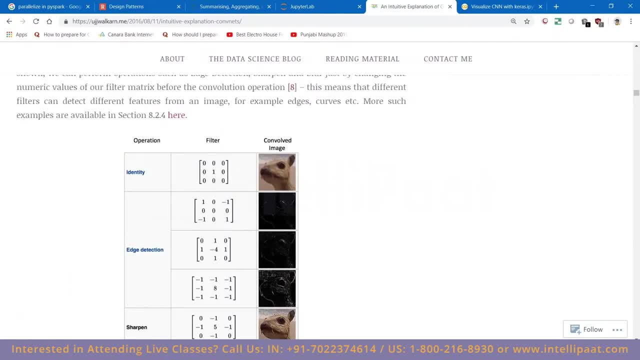 might, might if we go up again, if we go up again, if we go up again, if not, let's not go up again. but if if not, let's not go up again. but if if not, let's not go up again. but if you see this thing right here, 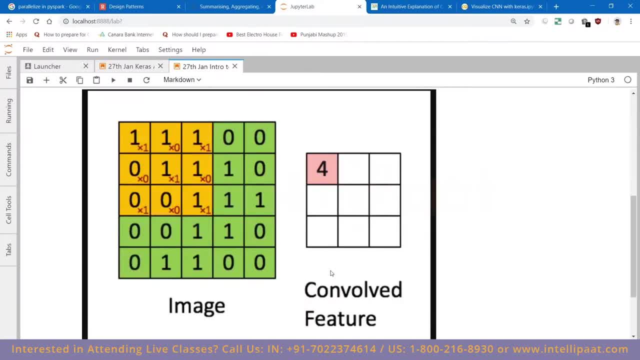 okay, okay, okay, this is the dynamic one, this is it. this is the dynamic one. this is it, this is the dynamic one, this is it. right, right, right. let's say: if you are here, and let's say: let's say: if you are here, and let's say: 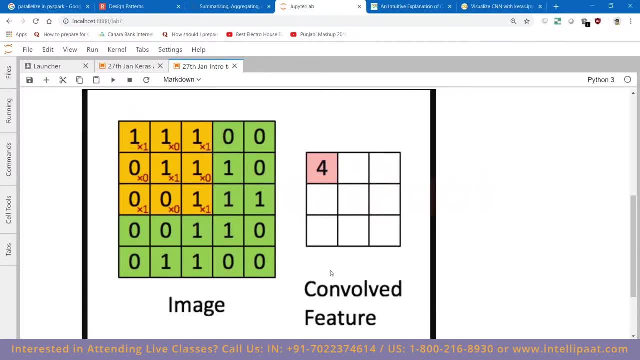 let's say, if you are here and let's say that this is the first step, right, it has that this is the first step, right, it has that this is the first step, right, it has completed, completed, completed. now let's say that you have a stride of. 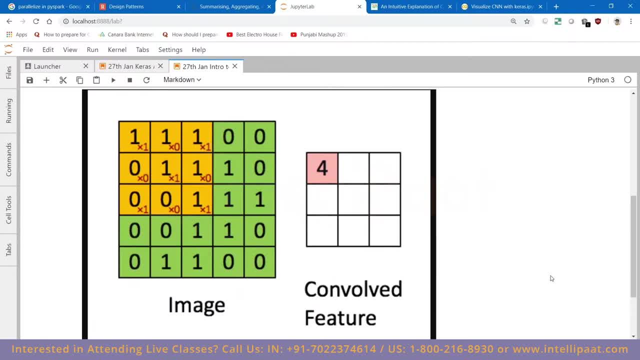 now, let's say that you have a stride of. now, let's say that you have a stride of two, two, two. where will be the next stride position? where will be the next stride position? where will be the next stride position will be stride position will be almost. 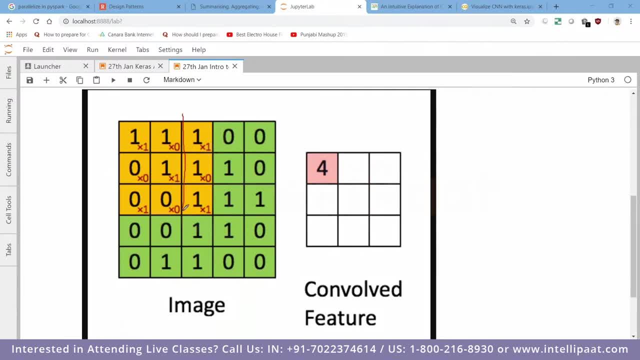 will be stride position will be almost will be stride position will be almost somewhat here, somewhat here, somewhat here, this, this, this and this and this right now, let's take an example that right now, let's take an example that right now, let's take an example that you again have a five cross, five image. 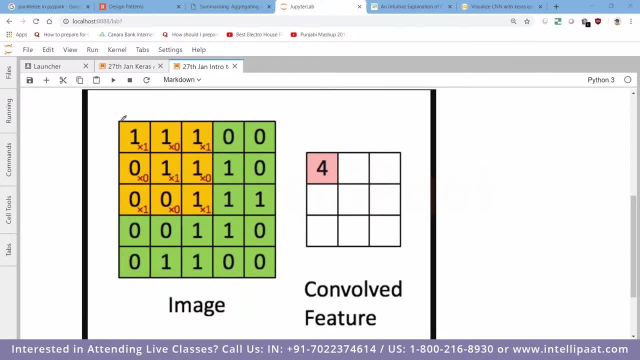 you again have a five cross five image. you again have a five cross five image, three cross three filter. but you have a three cross three filter. but you have a three cross three filter, but you have a stride of three cross three. what will stride of three cross three? what will? 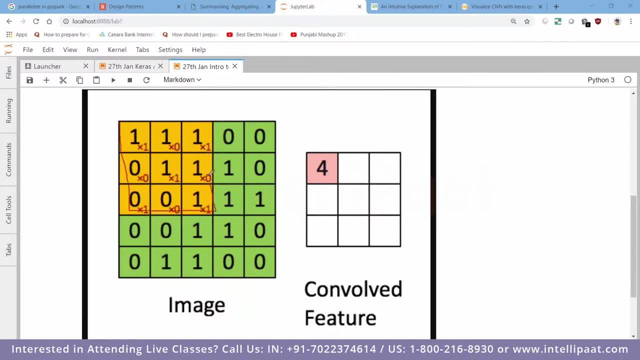 stride of three cross three. what will happen right now? happen right now. happen right now. first is here. i can draw it for you. first is here. i can draw it for you. first is here. i can draw it for you. first will be this. first will be this: 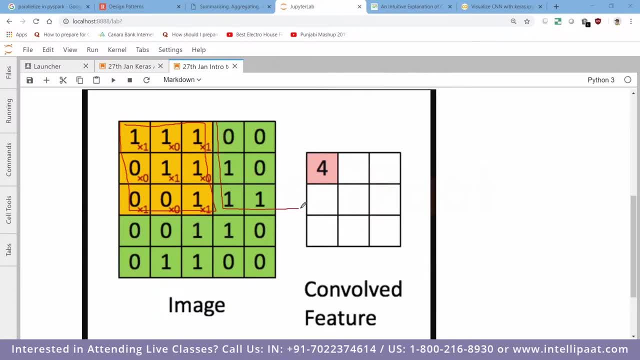 first will be this, the third one will be the second one, the third one will be the second one, the third one will be the second one will be here, but at this particular will be here, but at this particular will be here, but at this particular instance. you have only two columns where 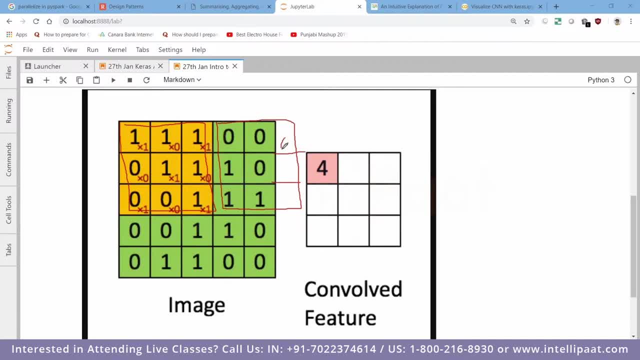 instance, you have only two columns. where instance, you have only two columns, where is this third column? is this third column, is this third column right? so what you do is you fill it with right. so what you do is you fill it with right. so what you do is you fill it with zeros. here. this is called zero padding. 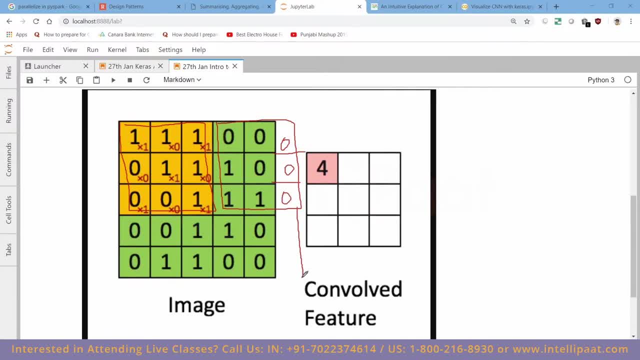 zeros- here this is called zero padding. zeros- here this is called zero padding. when you don't have enough number of, when you don't have enough number of when you don't have enough number of columns to fill your things what you do. columns to fill your things, what you do. 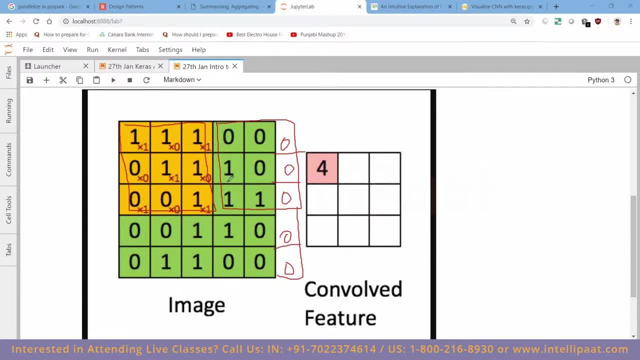 columns to fill your things, what you do. fill it with zeros, zero zeros, so that. fill it with zeros, zero zeros, so that fill it with zeros, zero zeros, so that now you can have a three cross three. now you can have a three cross three, now you can have a three cross three padding. just a quick info, guys. test your. 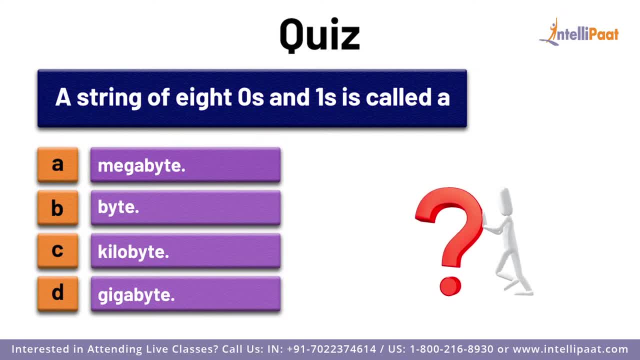 padding. just a quick info, guys test your padding. just a quick info. guys test your knowledge of computer vision by knowledge of computer vision, by knowledge of computer vision by answering this question. a string of eight answering this question, a string of eight answering this question, a string of eight zeros and ones is called. what a 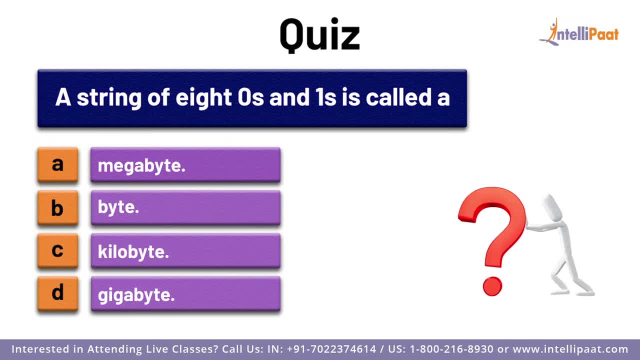 zeros and ones is called what a? zeros and ones is called what a megabyte B byte C. kilobyte D gigabyte. megabyte B. byte C. kilobyte D gigabyte. megabyte B byte C. kilobyte D, gigabyte. comment your answer in the comment. 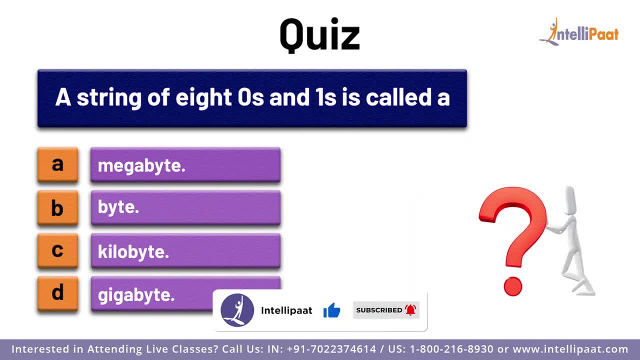 comment your answer in the comment. comment your answer in the comment section below: subscribe to Intellipaat. to section below: subscribe to Intellipaat to section below: subscribe to Intellipaat. to know the right answer now, let's know the right answer now, let's. 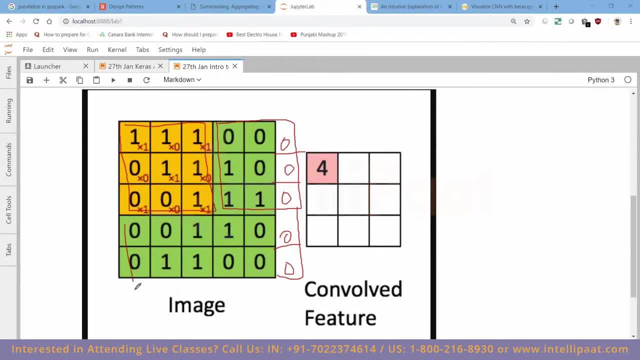 know the right answer now. let's continue with the session similarly. if continue with the session similarly, if continue with the session similarly, if you go down, you will have this problem. you go down, you will have this problem. you go down, you will have this problem here also. you won't have an extra row. 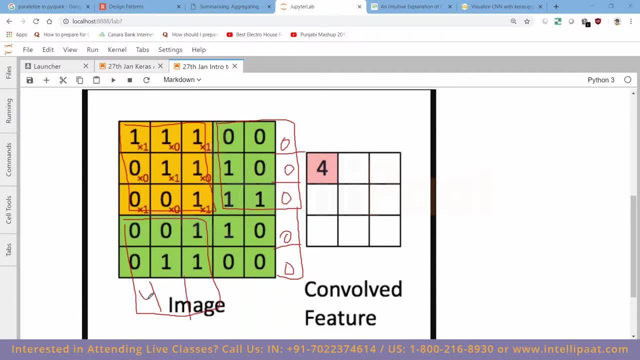 here also, you won't have an extra row. here also, you won't have an extra row. so what you will do is: again you will go. so what you will do is: again you will go. so what you will do is: again you will go. this will fill zero in this, zero, zero. 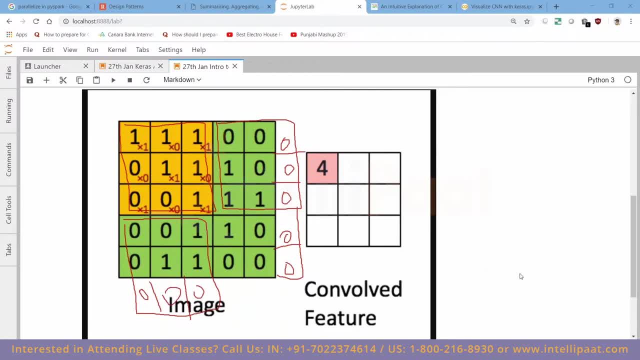 this will fill zero in this, zero, zero. this will fill zero in this, zero, zero and zero. this thing is called padding and zero. this thing is called padding and zero. this thing is called padding. what is called this is called zero. what is called this is called zero. 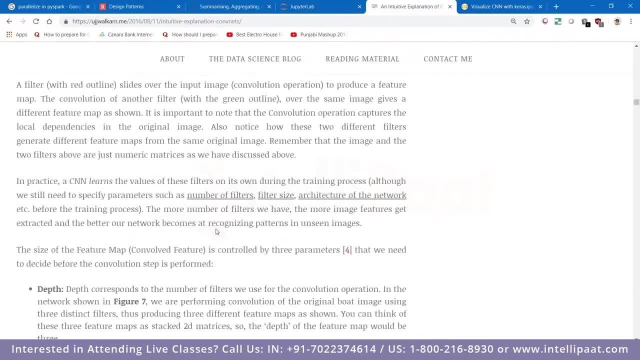 what is called? this is called zero padding right. smoke the next thing. this padding right, smoke the next thing. this padding right, smoke the next thing. this is called zero padding right now. once is called zero padding right now. once is called zero padding right now. once you have done all this, you know you have. 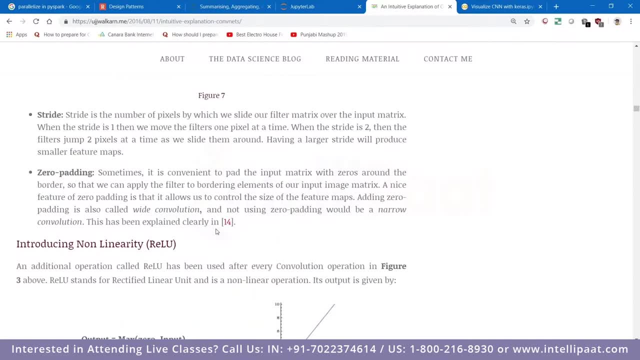 you have done all this. you know you have. you have done all this, you know you have run the feature with multiple depth and run the feature with multiple depth and run the feature with multiple depth and you have some padding or you have some. you have some padding or you have some. 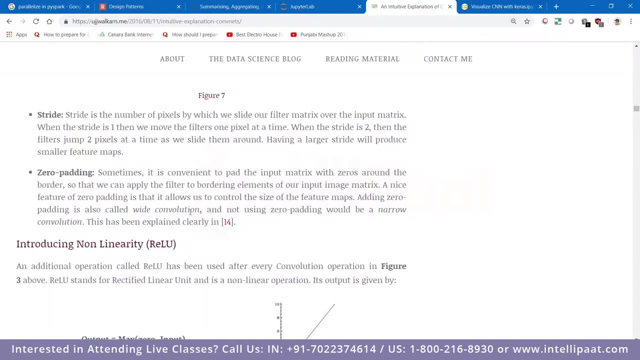 you have some padding or you have some strides right then you'll get some strides right. then you'll get some strides right. then you'll get some output out of the trade. similar like output out of the trade, similar like output out of the trade, similar like you've got something here like four, three. 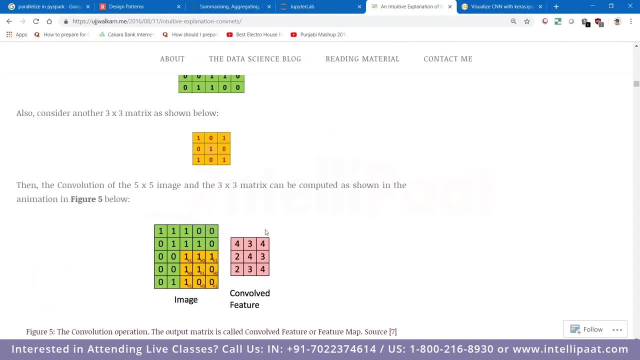 you've got something here like four, three. you've got something here like four, three, four, two, four, three and two, three, four, four, two, four, three and two, three, four, four, two, three, four, two, three, four. right, this pink answer, you'll get right. right, this pink answer, you'll get right. 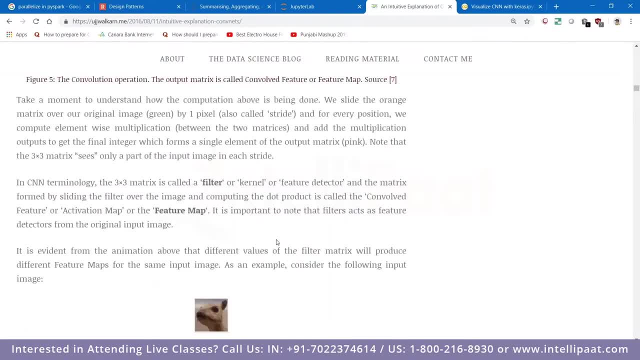 right, this pink answer you'll get right, so we'll get an image now if I say that. so we'll get an image now if I say that. so we'll get an image now if I say that, please run it through a relu now if you. please run it through a relu now if you. 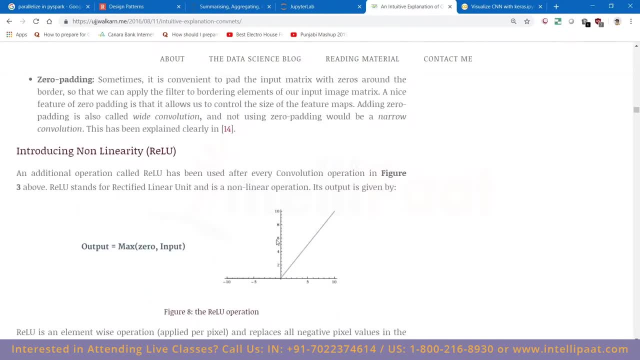 please run it through a relu now if you remember relu. what was relu? remember relu, what was relu? remember relu? what was relu? relu used to give you the answer, as it is relu used to give you the answer. as it is relu used to give you the answer as it is, if the number is greater than zero. 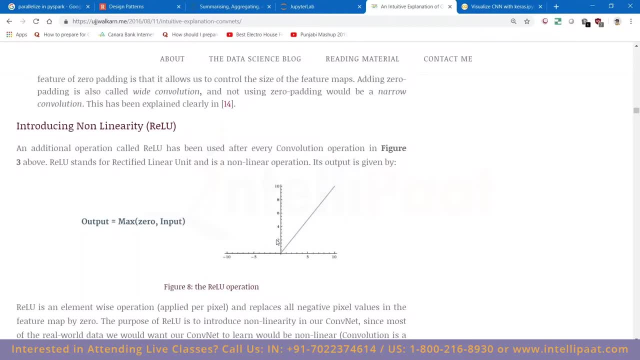 if the number is greater than zero. if the number is greater than zero, right. but if the number is less than zero, right. but if the number is less than zero, right. but if the number is less than zero, it will convert everything to zero. so it will convert everything to zero. so 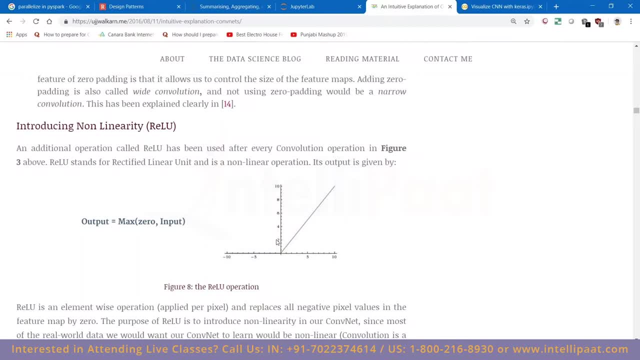 it will convert everything to zero. so what we are trying to say is that, if what we are trying to say is that, if what we are trying to say is that if there is a positive number, let it go, and there is a positive number, let it go, and 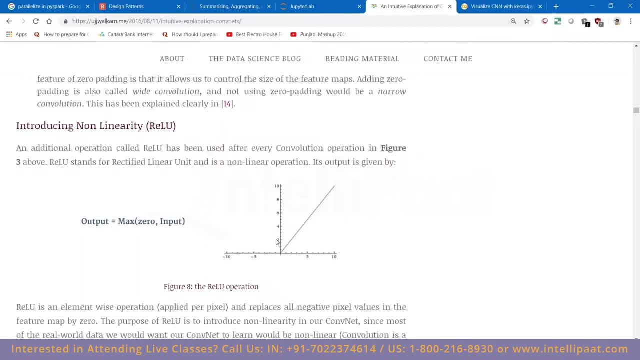 there is a positive number, let it go and fly. we don't care. but if something is fly, we don't care. but if something is fly, we don't care. but if something is negative, we are going to convert it to negative. we are going to convert it to. 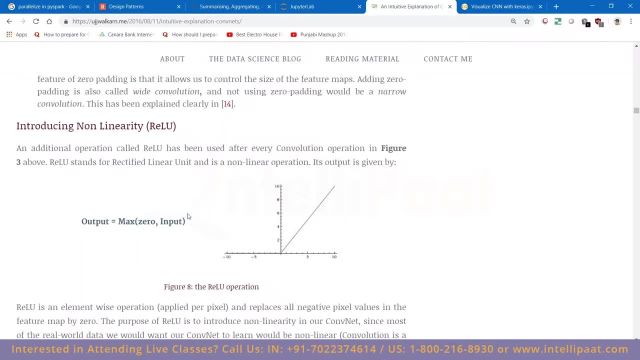 negative, we are going to convert it to zero. so what will happen is if you give zero. so what will happen is if you give zero. so what will happen is: if you give a image, see if this was your, if you can a image, see if this was your, if you can. 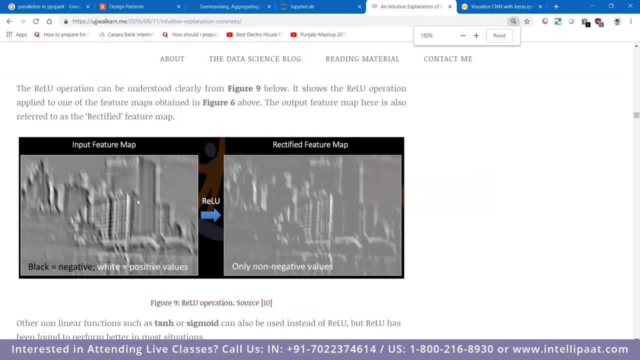 a image. see if this was your. if you can see clearly, let me go in. if you clearly see clearly, let me go in. if you clearly see clearly, let me go in. if you clearly see from here, you can see it right now. see from here, you can see it right now. 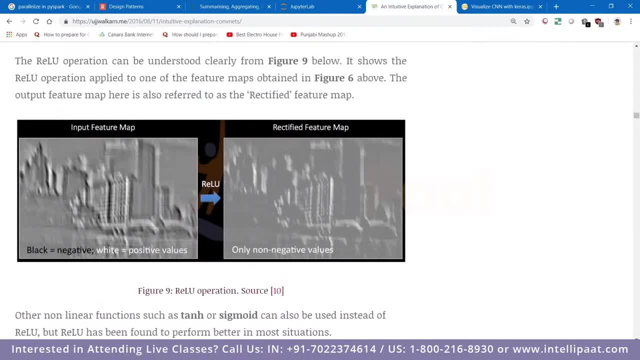 see from here. you can see it right now. if you clearly see from here on the left, if you clearly see from here on the left, if you clearly see from here on the left hand side. this was the output from the hand side. this was the output from the. 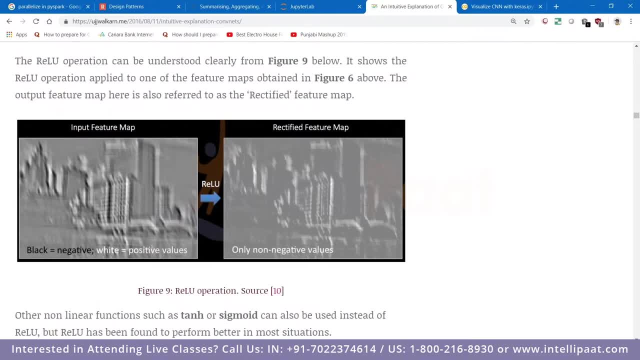 hand side. this was the output from the feature, one of the output from the feature, one of the output from the feature, one of the output from the feature. and then you ran this value feature, and then you ran this value feature, and then you ran this value thing. this is what has happened, only. 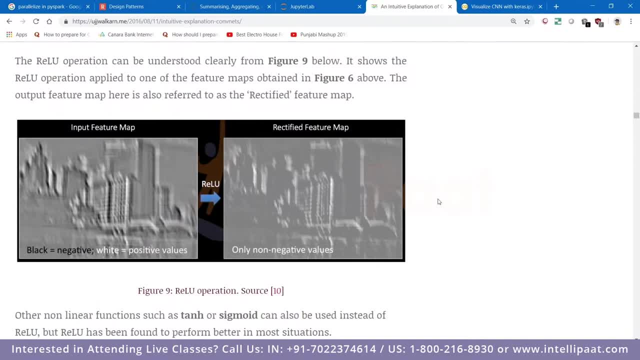 thing. this is what has happened. only thing: this is what has happened. only non-negative values are there. all the non-negative values are there. all the non-negative values are there? all the negative values are gone. negative values are gone. negative values are gone. you can read there also. it was written: 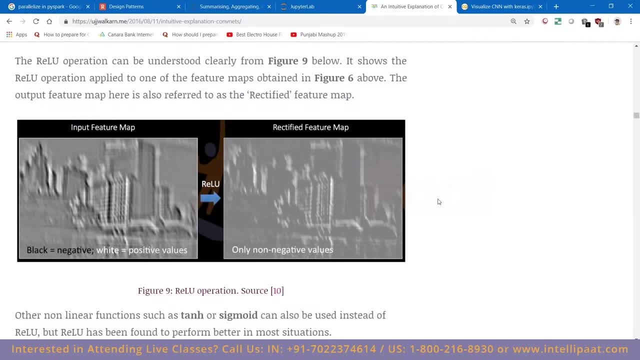 you can read there also. it was written. you can read there also. it was written: black is equal to negative, white is black is equal to negative. white is black is equal to negative. white is equal to positive value. so all the whites equal to positive value. so all the whites. 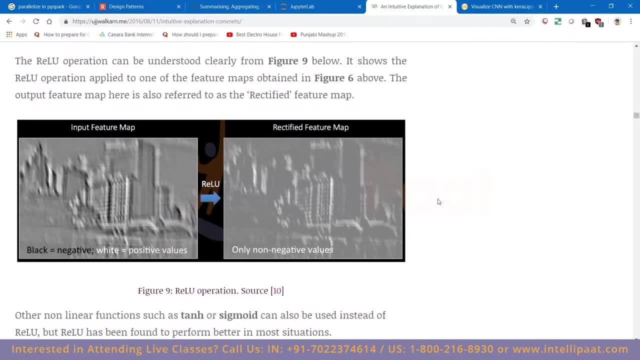 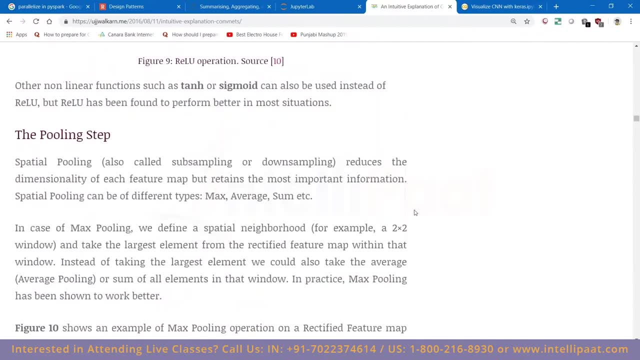 equal to positive value. so all the whites are there. blacks are all gone, right, are there? blacks are all gone, right, are there? blacks are all gone, right now. once you have done the pool, you have now, once you have done the pool, you have now, once you have done the pool, you have done the relu, then you have this thing: 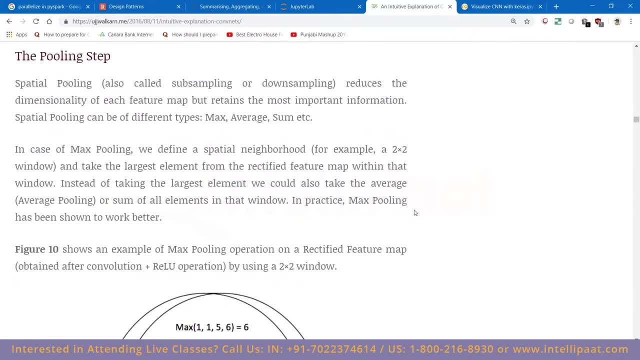 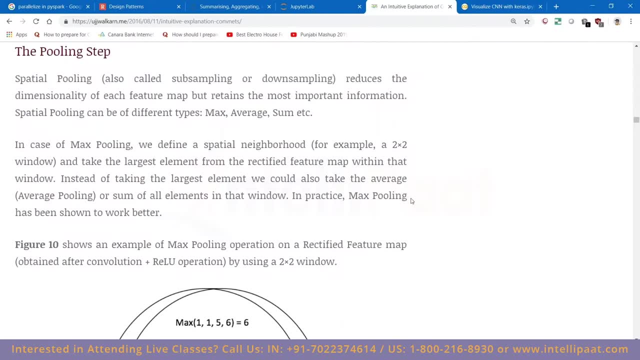 done the relu, then you have this thing done the relu, then you have this thing called pooling. that you were just called pooling that. you were just called pooling that. you were just using the most important features, using the most important features, using the most important features, and this one we were talking about that. 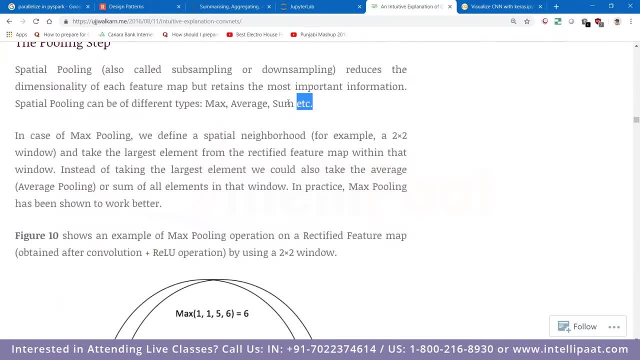 and this one. we were talking about that and this one- we were talking about that. the pooling can be of different types. the pooling can be of different types. the pooling can be of different types: max average, and some need it here. max average and some need it here. 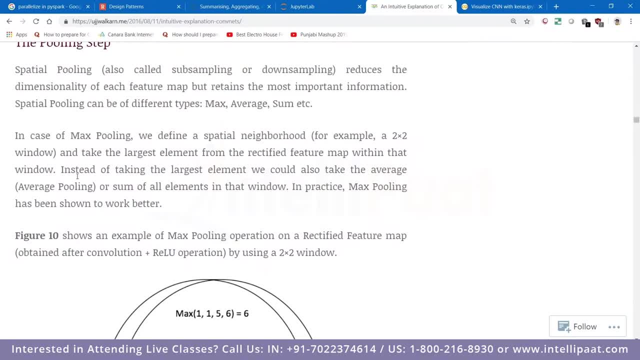 max average and some need it here. these three lines, this is one of the best. these three lines, this is one of the best. these three lines, this is one of the best right, and especially for you know new right, and especially for you know new right and especially for you know new people who just started learning how. people who just started learning, how people who just started learning, how deep learning- this is one of the best deep learning. this is one of the best deep learning. this is one of the best because it is not using any kind of a. because it is not using any kind of a. 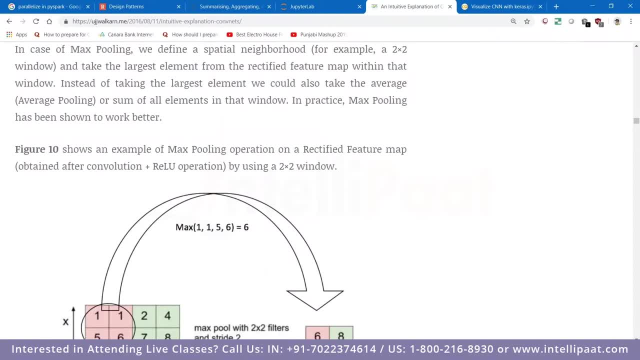 because it is not using any kind of a jargon word. you know otherwise people jargon word. you know otherwise people jargon word. you know otherwise people. they use like non-spatial locational. they use like non-spatial locational. they use like non-spatial locational. background of the image will not and 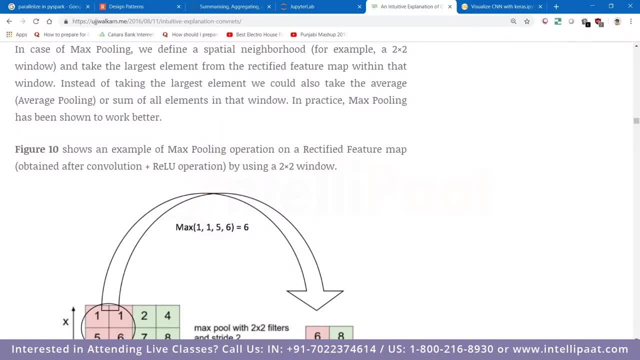 background of the image will not, and background of the image will not, and then you won't have any idea what is, then. you won't have any idea what is, then you won't have any idea what is going on right. so what is happening is going on right. so what is happening is. 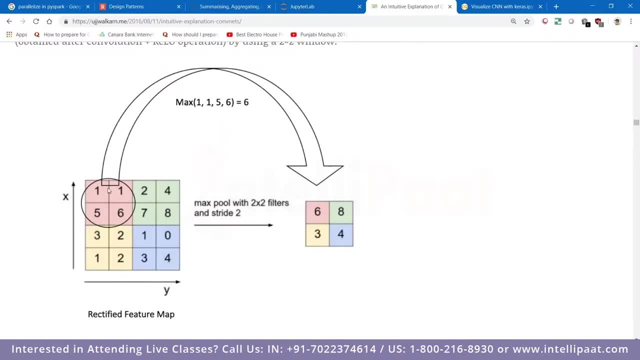 going on right. so what is happening is: this is a four cross four image you take this is a four cross four image you take this is a four cross four image. you take a two cross two matrix over it. you do a. a two cross two matrix over it. you do a. 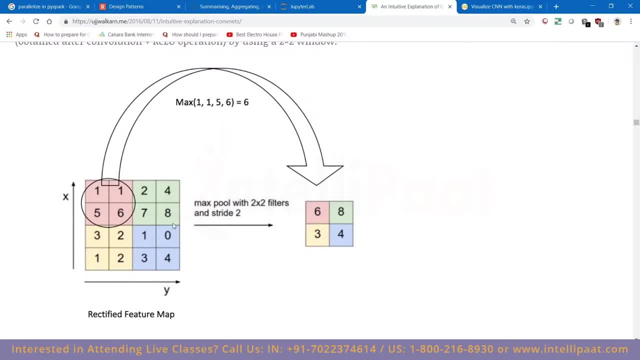 a two cross two matrix. over it you do a max pooling six is maximum. take six. eight. max pooling six is maximum. take six. eight. max pooling six is maximum. take six. eight is maximum. take eight here. maximum is is maximum. take eight here. maximum is is maximum. take eight here. maximum is three. here. maximum is four. take all this. three here, maximum is four. take all this. three here, maximum is four. take all this. so what you've done is you take your. so what you've done is you take your. so what you've done is you take your original picture. original picture: you do. original picture, original picture: you do. 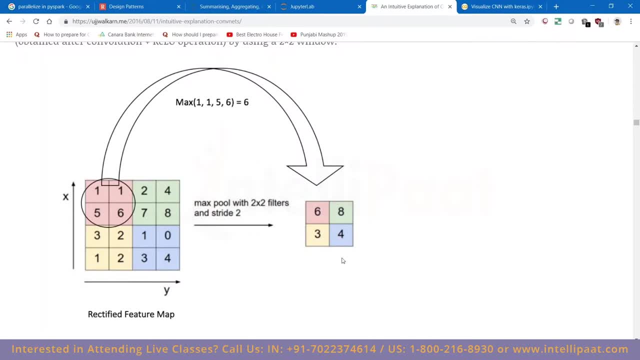 original picture: original picture: you do some feature of you, ran some filter you some feature of you, ran some filter you some feature of you, ran some filter. you got the converted filter, then you ran, got the converted filter, then you ran some value and then on the value you ran. 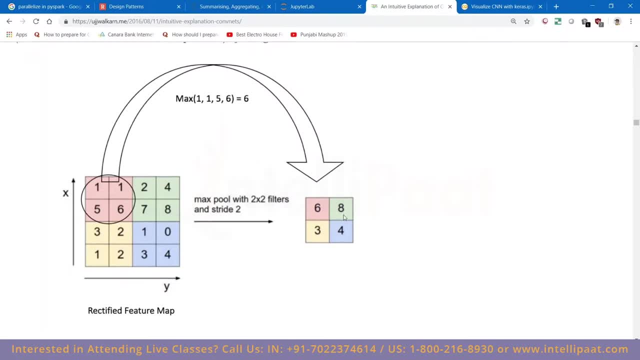 some value and then on the value, you ran some value. and then on the value, you ran a max pooling, a max pooling, a max pooling. so, eventually, what will happen? let's see. so, eventually, what will happen. let's see. so, eventually, what will happen. let's see if you ran the image on a max pooling. 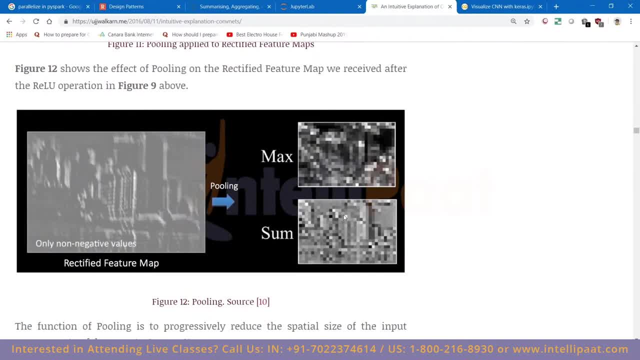 if you ran the image on a max pooling, if you ran the image on a max pooling, this is what will happen. this is what will happen. this is what will happen. but if you will see this thing for a. but if you will see this thing for a. 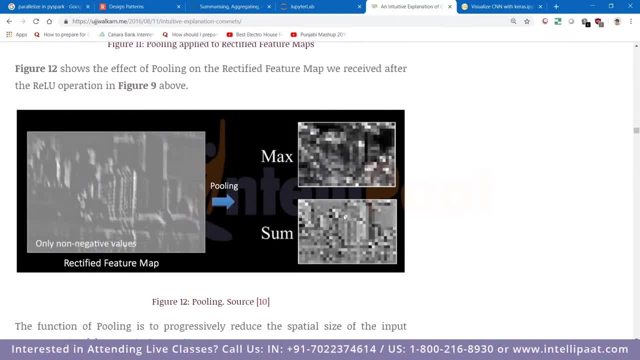 but if you will see this thing for a very large image, right, very large image, right, very large image, right, you will understand these things also. you will understand these things also. you will understand these things also. let's say, if you have an image of, let's say, if you have an image of, 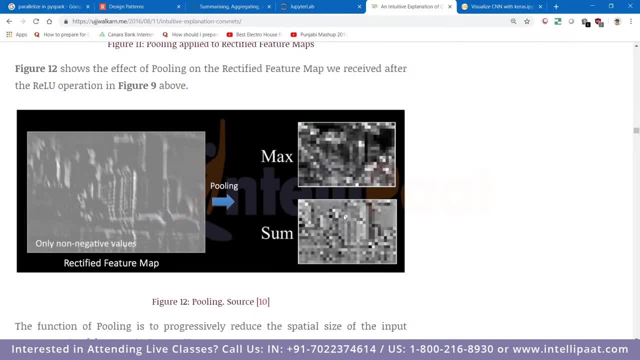 let's say, if you have an image of thousand plus thousand, and then you're thousand plus thousand, and then you're thousand plus thousand, and then you're running this thing, you will definitely running this thing, you will definitely running this thing, you will definitely capture these things. that what it is. 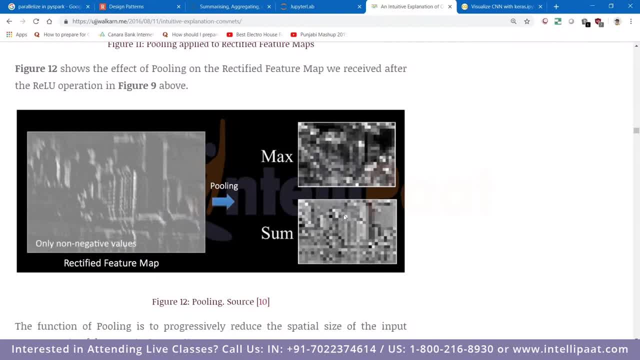 capture these things. that what it is. capture these things. that what it is doing is, ultimately, all these buildings doing is, ultimately, all these buildings doing is, ultimately, all these buildings are now reduced to a very lower level, are now reduced to a very lower level, are now reduced to a very lower level, has been now reduced to this small. 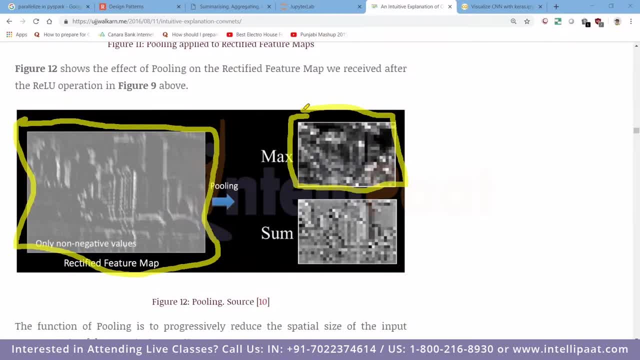 has been now reduced to this small has been now reduced to this small. image right, image right. image right. and now if this would have been a high, and now if this would have been a high, and now if this would have been a high quality image, you could have easily seen. 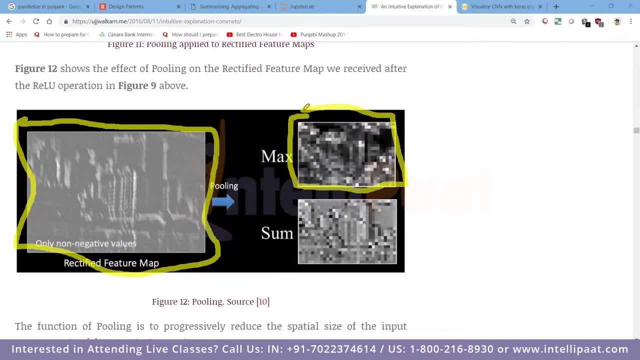 quality image. you could have easily seen quality image. you could have easily seen that all these tall buildings are, now that all these tall buildings are, now that all these tall buildings are now reduced to a smaller level in the things, reduced to a smaller level in the things. 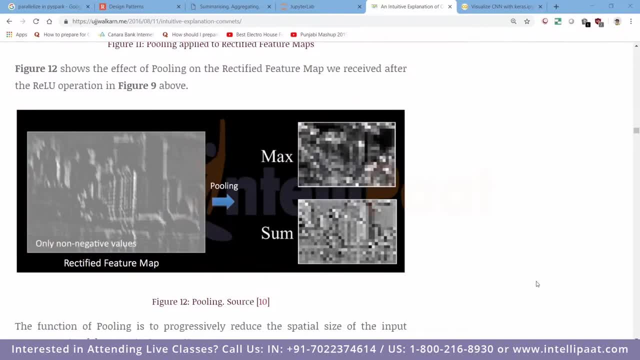 reduced to a smaller level in the things and we are reducing the dimensionality and we are reducing the dimensionality and we are reducing the dimensionality. right, this is all what we do in right. this is all what we do in right. this is all what we do in convolution. at the end, we get this. 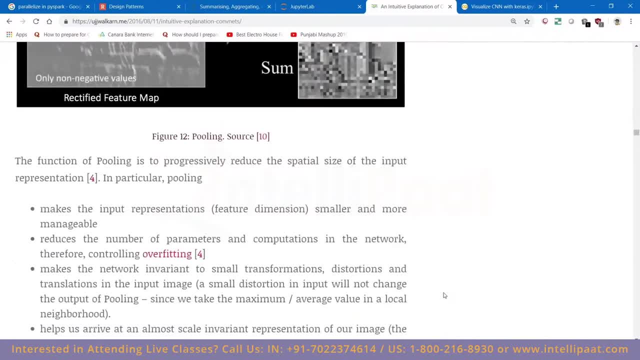 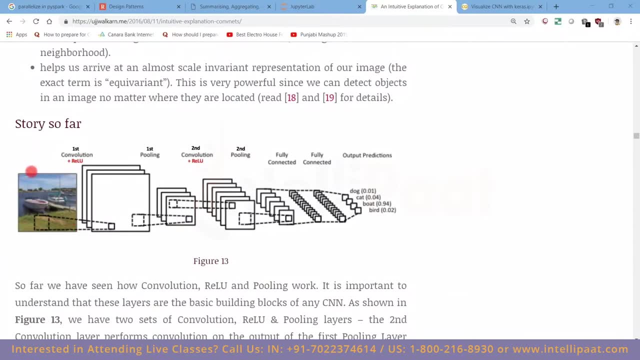 convolution. at the end, we get this convolution. at the end, we get this convolution and we get somewhat convolution and we get somewhat convolution and we get somewhat architecture like this architecture like this architecture like this: this extreme left was your, this extreme left was your, this extreme left was your original image. right then you ran some. 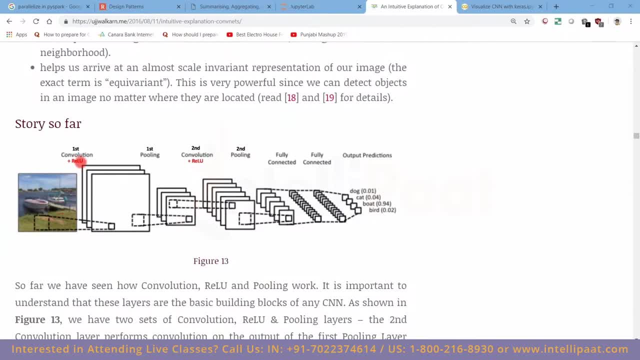 original image. right then you ran some original image. right then you ran some filters on it. let's say you ran three filters on it. let's say you ran three filters on it. let's say you ran three filters, filters, filters, so the size is three. filters are here now. 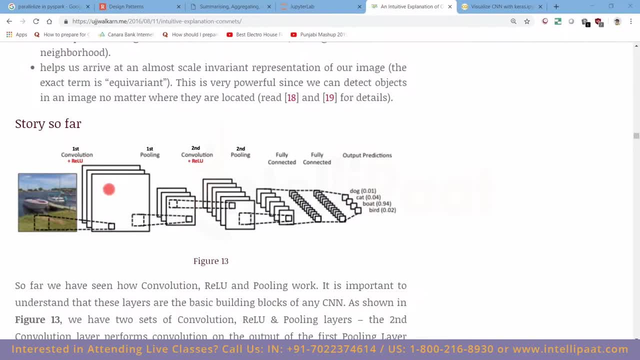 so the size is three. filters are here now, so the size is three. filters are here now. out of one image, you can get three. out of one image, you can get three. out of one image, you can get three images right, three different outputs. images right, three different outputs. 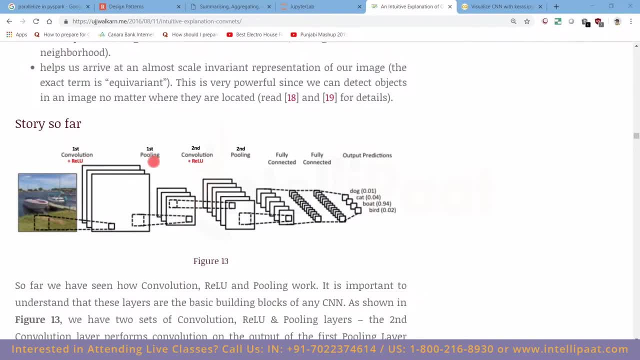 images: right, three different outputs for three different filters. now on for three different filters. now on for three different filters. now on these filters. you ran a pooling, now these filters. you ran a pooling, now these filters. you ran a pooling, now pooling, say you reduced the size of your. 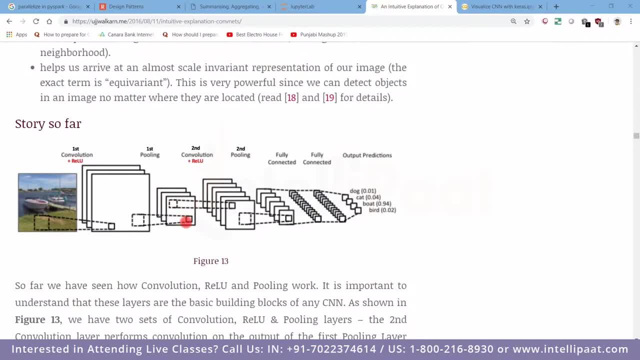 pooling. say you reduced the size of your pooling, say you reduced the size of your image. right again on this answer, that image. right again on this answer, that image. right again on this answer that. so you'll have nine images then again. so you'll have nine images then again. 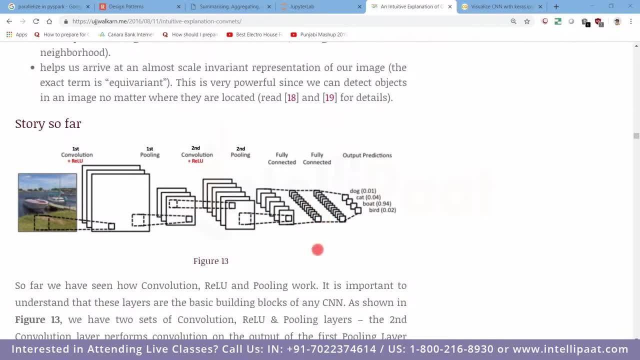 so you'll have nine images. then again you ran a max pool, then again you'll do, you ran a max pool, then again you'll do, you ran a max pool, then again you'll do pooling. so eventually, what will happen? pooling. so eventually, what will happen? pooling. so eventually, what will happen is your, your, your image size. if it was 50. 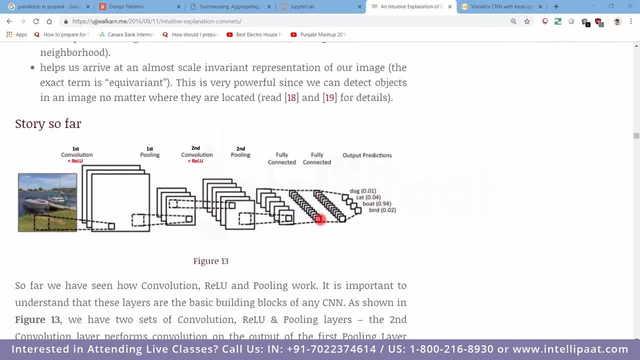 is your, your, your image size if it was 50? is your, your, your image size if it was 50 cross 50? this will end up to, let's say, cross 50. this will end up to, let's say, cross 50. this will end up to, let's say, seven cross seven. or let's say, one cross. 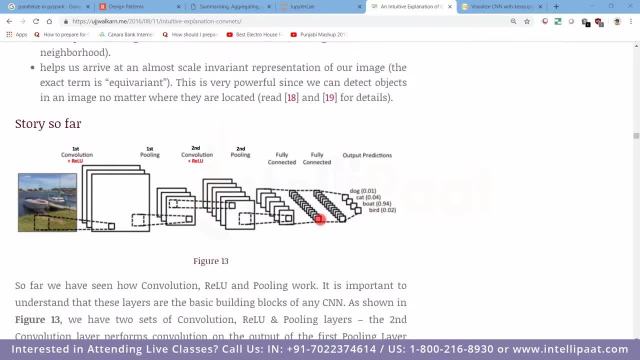 seven cross seven. or let's say one cross seven cross seven. or let's say one cross one, one one. but its depth will increase, but its depth will increase, but its depth will increase. its depth will increase to a very large level. its depth will increase to a very large level. 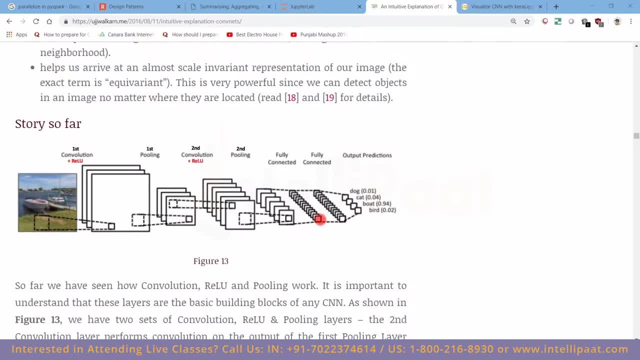 its depth will increase to a very large level, and this will ultimately convert it, and this will ultimately convert it, and this will ultimately convert it into a dense neural network, into a dense neural network, into a dense neural network, and this is what our idea is also make. 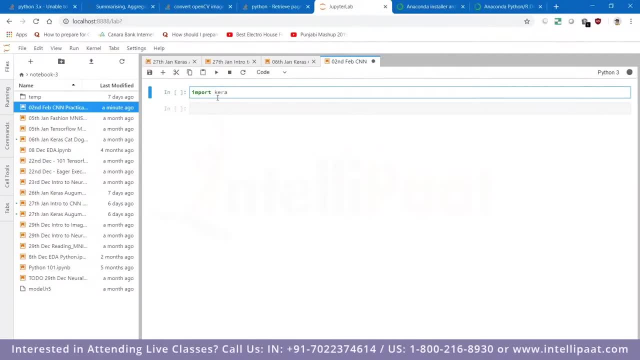 and this is what our idea is also make, and this is what our idea is also make sense, sense, sense. let's import the first thing first. let's import the first thing first. let's import the first thing first: import giras, import giras, import giras, our best friend. 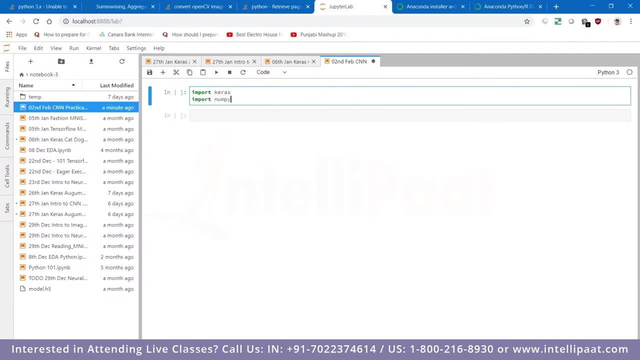 our best friend, our best friend. then we have numpy a second best friend. then we have numpy a second best friend, then we have numpy a second best friend. as envy, as envy, as envy. import: import: import: matplotlib dot, pyplot spld. let's go to giras dot. pre-processing. 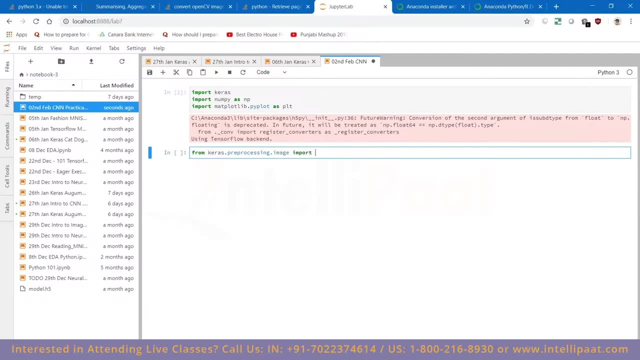 let's go to giras dot pre-processing. let's go to giras dot pre-processing, dot image, and then we have image data generator, then you have image data generator, then you have image data generator, then you have from from from giras, giras, giras. 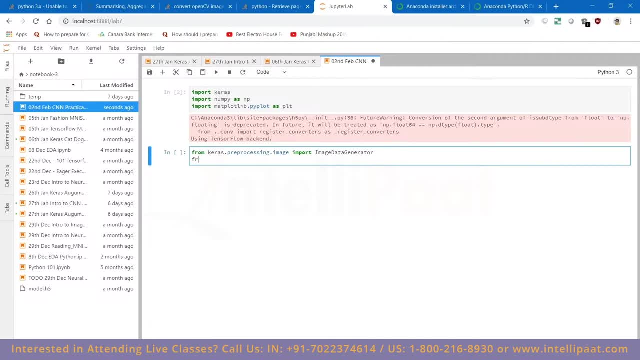 giras, dot, dot dot. okay, let's do the layer one, and okay, let's do the layer one, and okay, let's do the layer one, and afterwards, afterwards, afterwards, and let's make the data gen data and let's make the data gen data and let's make the data gen data generator. data generator is. 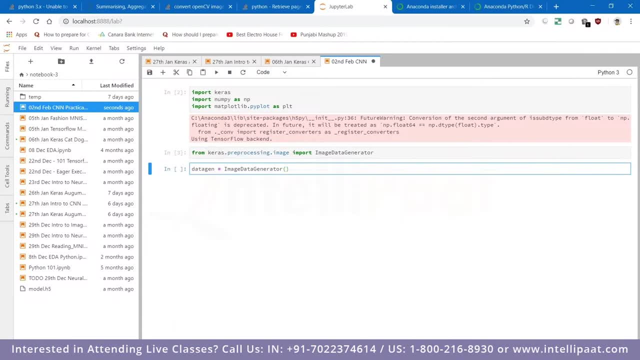 so okay, image data generator. what does so okay, image data generator. what does so okay, image data generator. what does it takes? it takes multiple things. how it takes. it takes multiple things. how it takes. it takes multiple things. how many things do you want to give? let's. 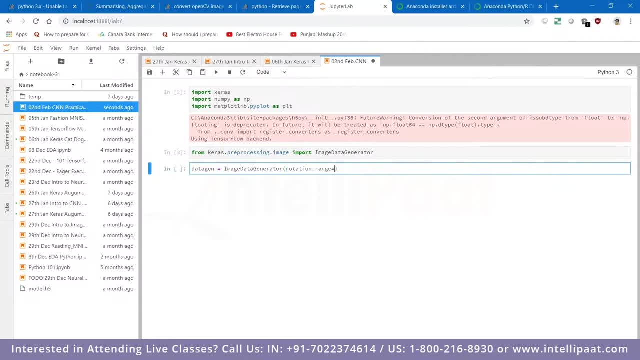 many things do you want to give? let's many things do you want to give. let's say, say, say, rotation range, rotation range. should rotation range, rotation range, should rotation range, rotation range should be what? 40. i'm so, i'm so, i'm so. sorry i have to see this thing with shift. 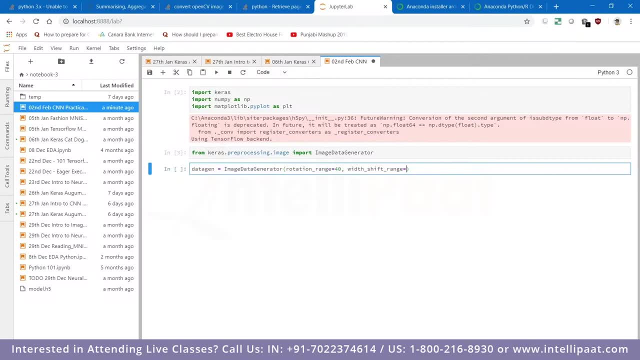 sorry, i have to see this thing with shift. sorry, i have to see this thing with shift. range, range, range, how much 0.2, how much 0.2, how much 0.2. then we have, then we have, then we have right, shift 0.2. 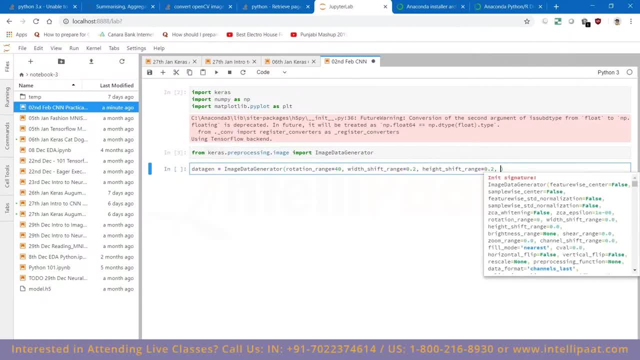 0.2, 0.2. right, we can what. what else do we have right, we can what? what else do we have right, we can what? what else do we have right with right with right with? and then okay, we can do a flip also. and then okay, we can do a flip also. 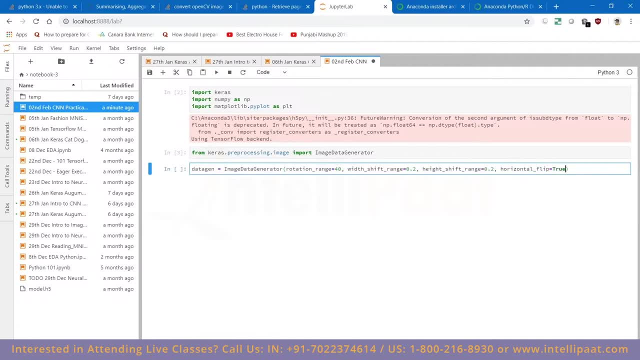 and then, okay, we can do a flip also. okay, horizontal, flip horizontal. okay, horizontal flip horizontal. okay, horizontal flip horizontal. equal to true, equal to true, equal to true. we can move this gt, we can move this gt, we can move this gt. i'm a little bit here. 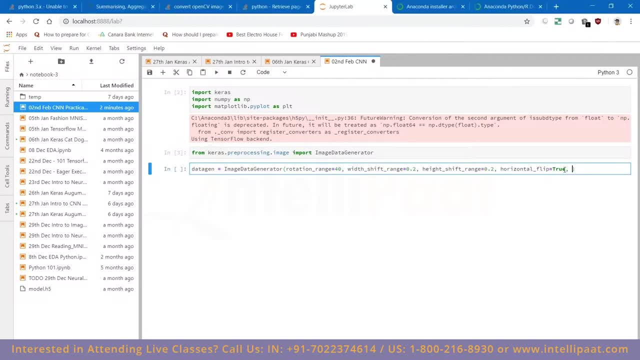 okay, then we have boom also zone range, boom also zone range, boom also zone range. let's do this as of now, only let's do this as of now, only let's do this as of now, only so our data generator is ready, so our data generator is ready. 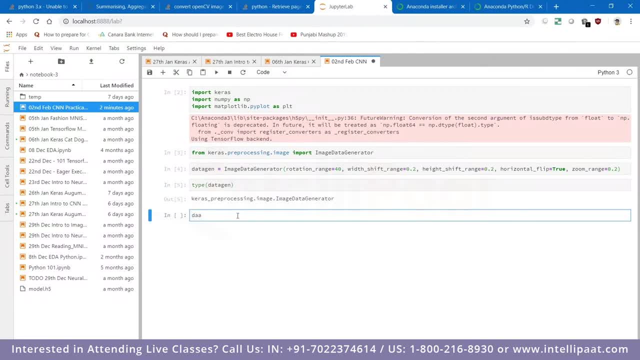 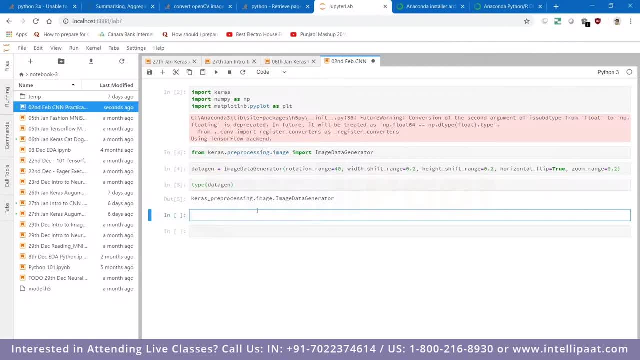 going here, it can tell you whatever. going here, it can tell you whatever. things, things, things you have taken, you have taken, you have taken it, you have taken. it will do, will do, will do, now, now, now, when you are using image data generator, when you are using image data generator, 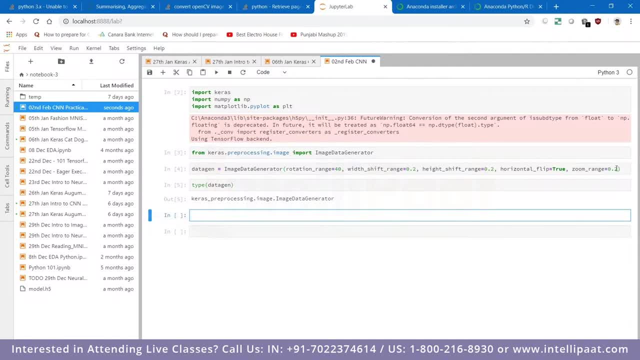 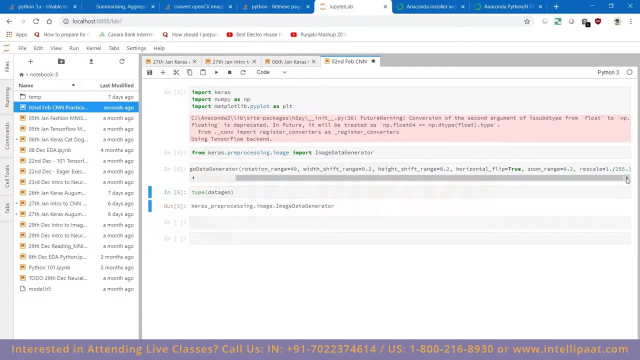 when you are using image data generator, you can do the same with just one thing. you can do the same with just one thing. you can do the same with just one thing. you just say rescale. so now, what will happen? all your images. so now, what will happen? all your images. 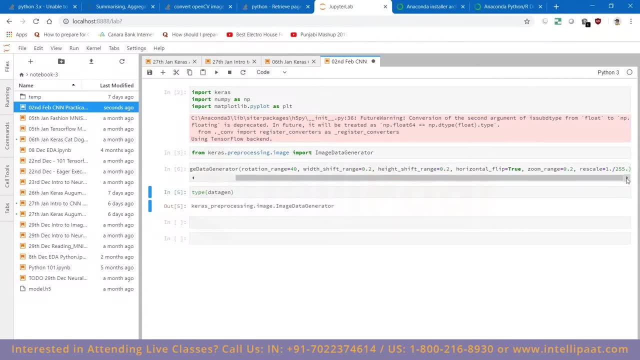 so now what will happen? all your images will be, will be, will be here through your, here through your, here through your. will be multiplied through divided. divided will be multiplied through divided. divided will be multiplied through divided divided by 255. right by 255. right by 255. right again, your data generator is: 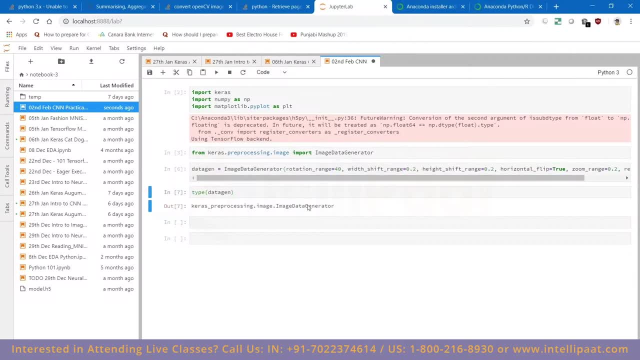 again. your data generator is again. your data generator is activated- see data generator- right saying activated. see data generator- right saying activated. see data generator- right saying it's a generator. so it will not give you. it's a generator. so it will not give you. it's a generator, so it will not give you all the values at one. 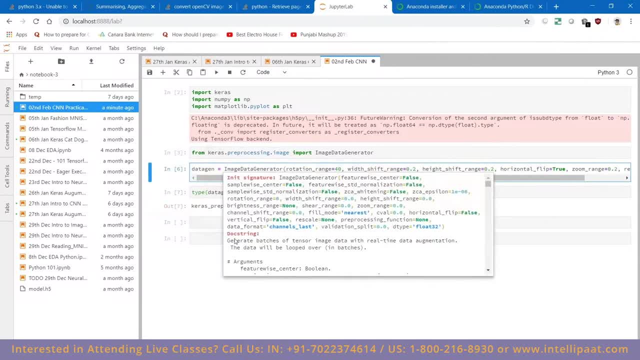 all the values at one. all the values at one. it will give you the results in batches. it will give you the results in batches. it will give you the results in batches where we read this. that generates where we read this. that generates where we read this. that generates batches of tensor images, data with. 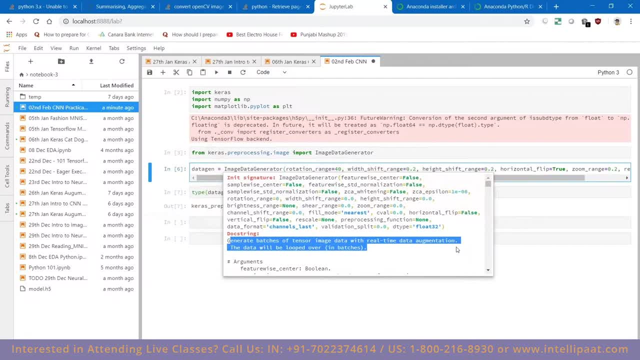 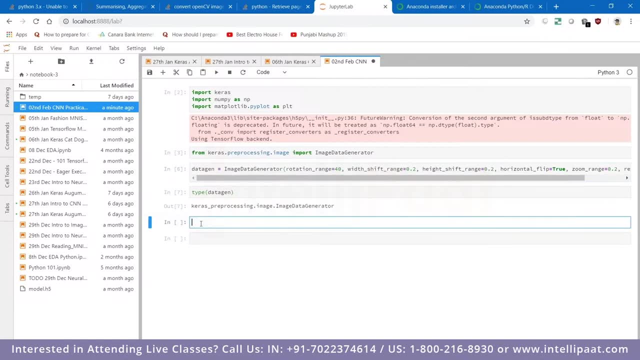 batches of tensor images. data with batches of tensor images. data with real-time augmentation: real-time augmentation. real-time augmentation. the data will be looped over in batches. the data will be looped over in batches. the data will be looped over in batches right. next we are going to do is that we have. 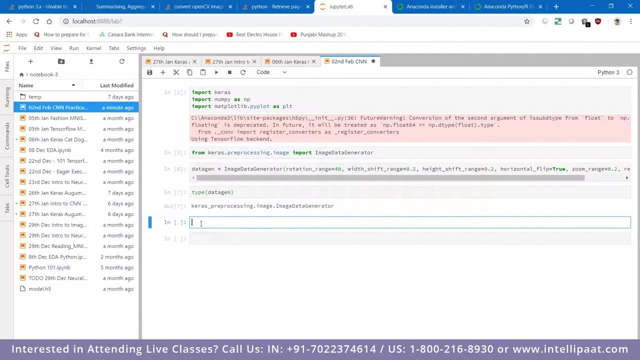 next we are going to do is that we have. next we are going to do is that we have made this generator here now. what we can made this generator here now, what we can made this generator here now, what we can do is we can directly start with our 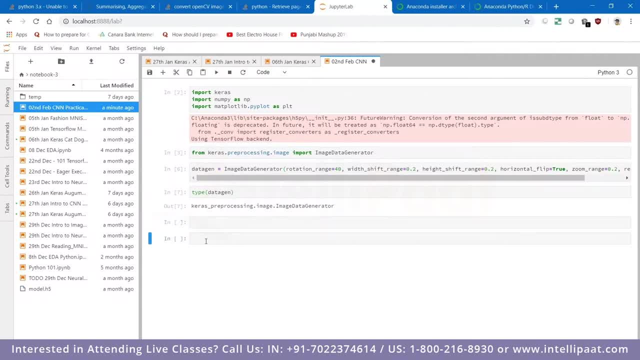 do is we can directly start with our do is we can directly start with our uh modeling part right from keras dot model. from keras dot model. from keras dot model import sequential right- import sequential right import sequential right from keras dot layers- keras dot layers, keras dot layers import. 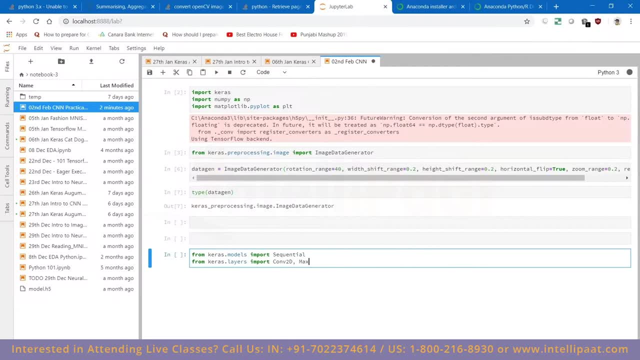 import: import conf 2d. today we're going to do is con conf 2d. today we're going to do is con conf 2d. today we're going to do is con 2d, 2d, 2d, then max pool: 2d. 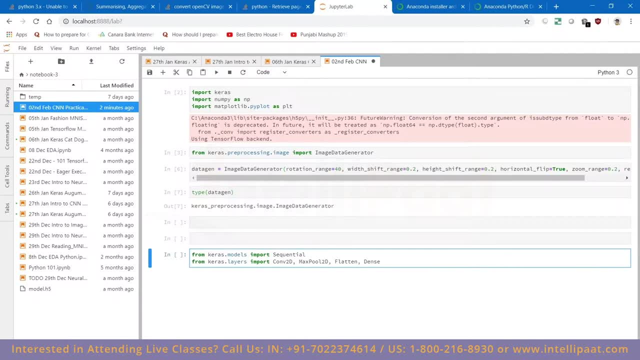 then max pool 2d, then max pool 2d, then we use flatten, then we will use, then we use flatten, then we will use, then we use flatten, then we will use dense, dense, dense. what else should we use? that's it. what else should we use? that's it. 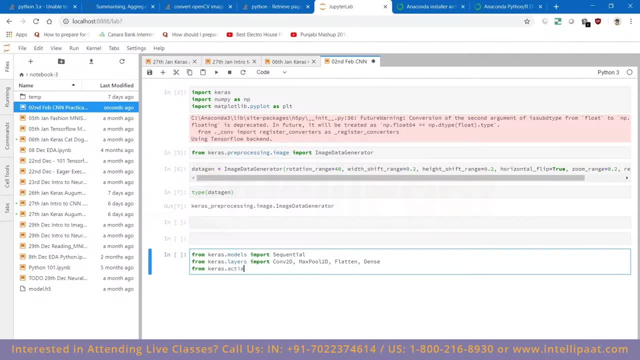 what else should we use? that's it right, right, right. and from kira's dot activation let's import activations. what kind of? let's import activations? what kind of? let's import activations? what kind of activation? do we know activation? do we know activation? do we know relo and softmax? 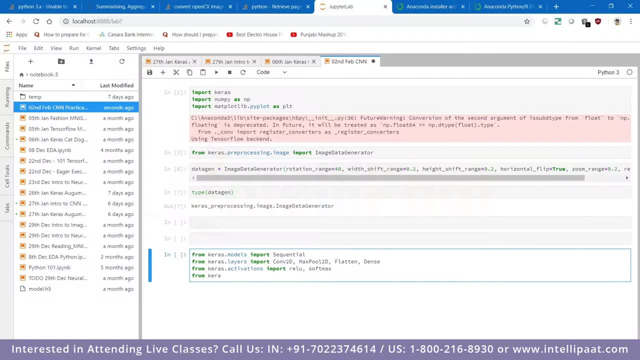 softmax, softmax, softmax. right then kira's softmax, right then kira's softmax, right then kira's dot, dot, dot, dot, dot, dot dot losses. maybe we'll use categorical losses. maybe we'll use categorical losses, maybe we'll use categorical cross entropy, cross entropy, cross entropy. right and from. 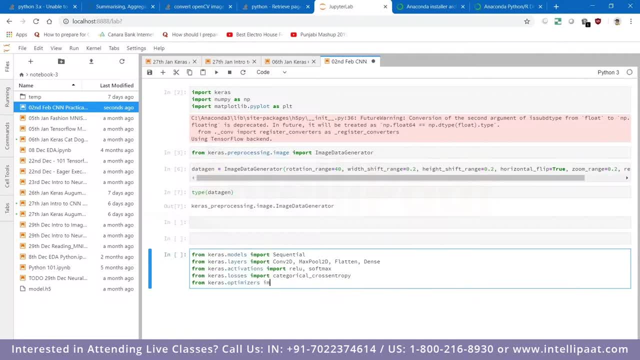 right and from right and from kira's dot optimizer. kira's dot optimizer. kira's dot optimizer. import hgd and rms prop. import hgd and rms prop. import hgd and rms prop- rms prop. okay, let's activate all these rms prop. okay, let's activate all these. 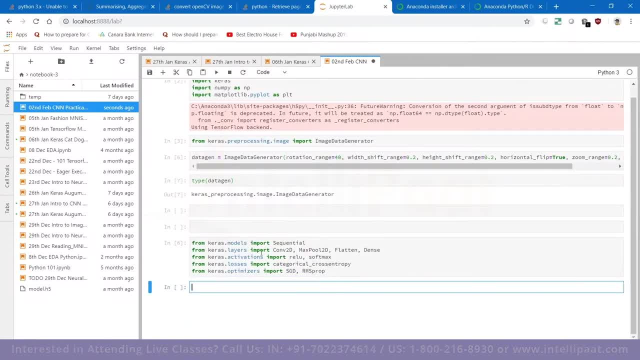 rms prop. okay, let's activate all these things, things, things. i think you're almost done. you've taken. i think you're almost done, you've taken. i think you're almost done. you've taken layers. you've taken activations, then layers. you've taken activations, then layers. you've taken activations, then you've taken losses, optimizers, nothing. 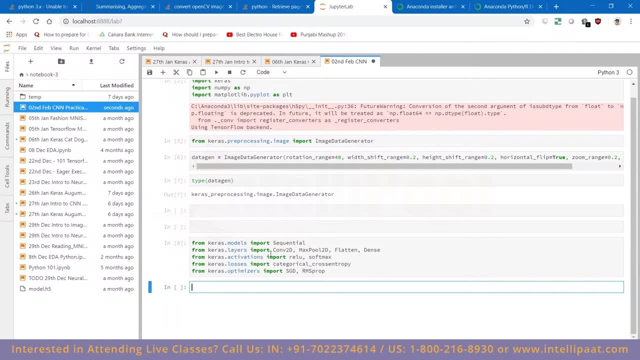 you've taken losses optimizers- nothing. you've taken losses optimizers- nothing else. right, let's make the model, and else right, let's make the model, and else right, let's make the model. and before we make the model, let me shift. before we make the model, let me shift. 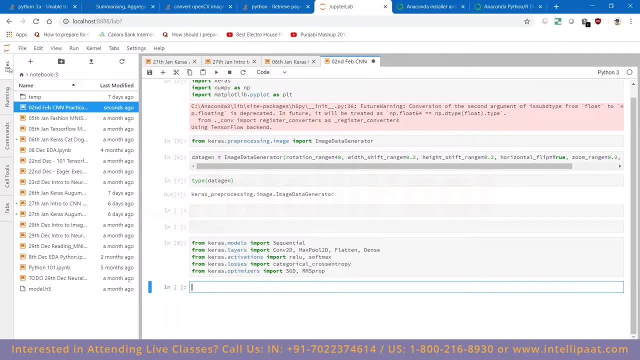 before we make the model, let me shift this track, this here and this, track this here and this, track this here, and close this thing out. you get more space, close this thing out. you get more space, close this thing out. you get more space. right now, let's make the model. model is: 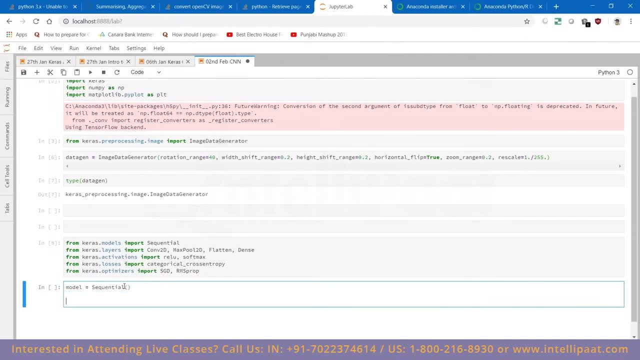 right now, let's make the model model is. right now, let's make the model. model is equal to sequential type of a model. equal to sequential type of a model. equal to sequential type of a model- right. sequential type of one, now, let's right. sequential type of one, now let's. 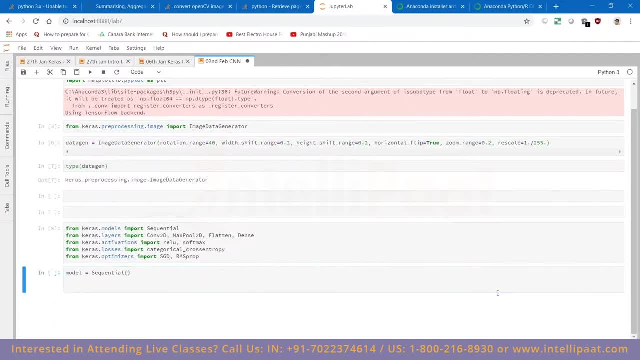 right, sequential type of one, now, let's pay a little bit attention. but how do we pay a little bit attention? but how do we pay a little bit attention? but how do we make a model out here, right, make a model out here, right, make a model out here, right. let's, let me give some space and then 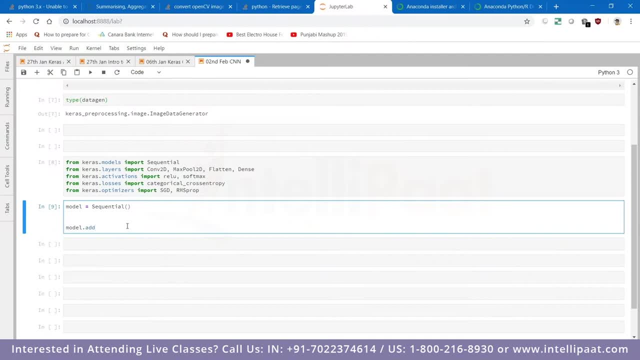 let's let me give some space, and then let's let me give some space and then okay, first of all, what i'll do is: i will okay, first of all. what i'll do is: i will okay, first of all. what i'll do is i will add a con player. i am not going to. 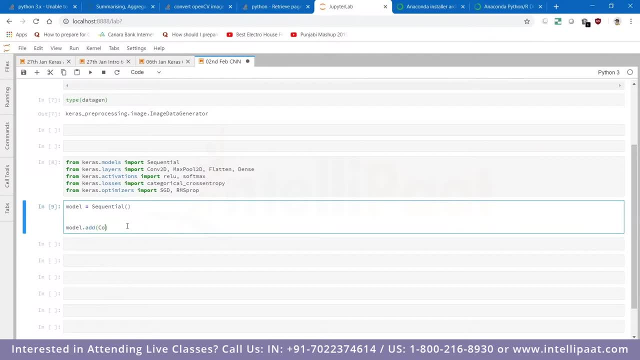 add a con player. i am not going to add a con player. i am not going to convert this image into a 1d image. by convert this image into a 1d image. by convert this image into a 1d image by doing a flattening. 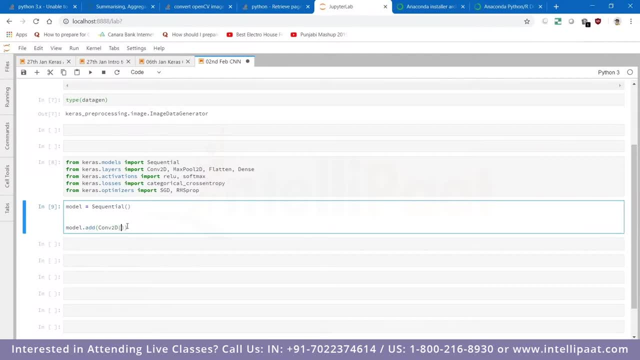 doing a flattening, doing a flattening this time i have to. i am going to give this time i have to. i am going to give this time i have to. i am going to give the images, the images, the images con 2d, as it is that when we were, 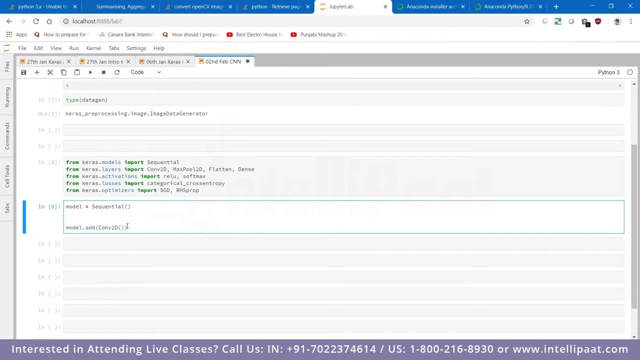 con 2d. as it is that when we were con 2d, as it is that when we were running the convolution in practical running, the convolution in practical running, the convolution in practical, we had this 2d image, we were not doing. we had this 2d image, we were not doing. 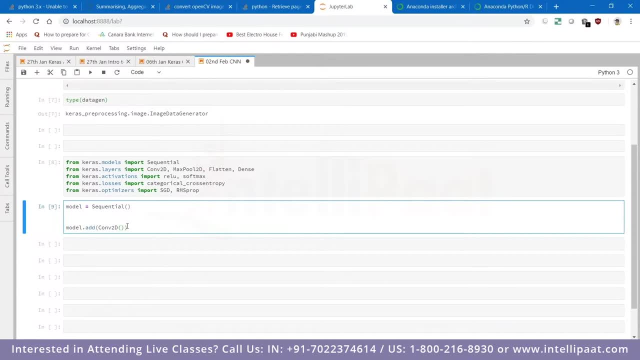 we had this 2d image. we were not doing it, flattening it, flattening it, flattening. we were not doing it row major. or we were not doing it row major. or we were not doing it row major or column major flattening right. column major flattening right. 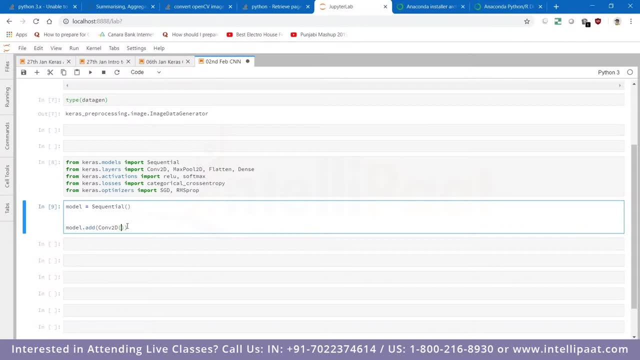 column- major flattening right. we took the image as it is right, so you, we took the image as it is right, so you, we took the image as it is right, so you are going to take this image, are going to take this image, are going to take this image. modeladd- convolution 2d. we are not. 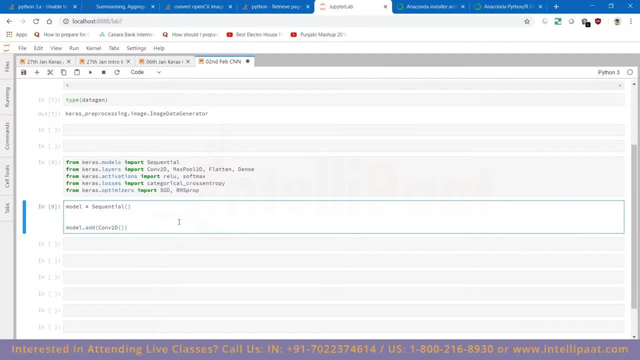 modeladd convolution 2d. we are not going to do the flattening part now. going to do the flattening part now. going to do the flattening part now. let's see that. what does this con 2d? let's see that. what does this con 2d? 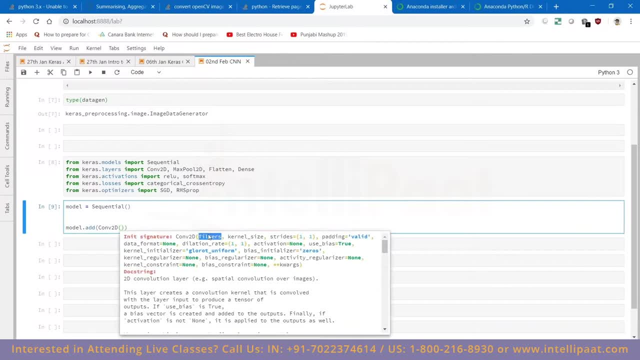 let's see that. what does this? con 2d takes place, takes place, takes place. now con 2d first takes place filters. now, con 2d first takes place filters. now con 2d first takes place filters. okay, let's see what filters is then we. 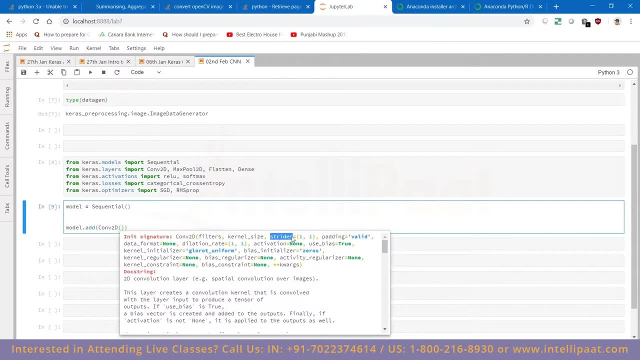 okay, let's see what filters is, then we? okay, let's see what filters is, then we. have kernel size, then we have strides. have kernel size, then we have strides. have kernel size, then we have strides. if you don't give strides, strides are by. if you don't give strides, strides are by. 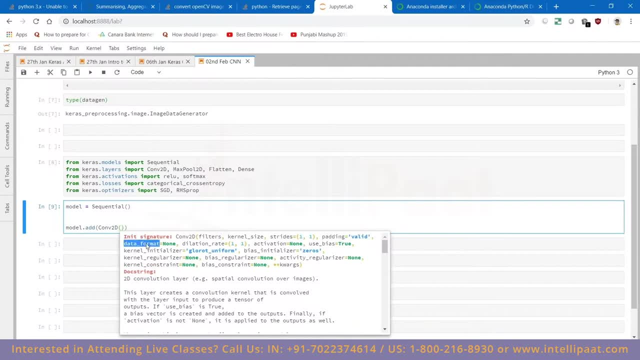 if you don't give strides, strides are by default one cross one, then you have default one cross one, then you have default one cross one, then you have padding, then you have data format, then padding, then you have data format, then padding, then you have data format, then you have dilation. now, after that all. 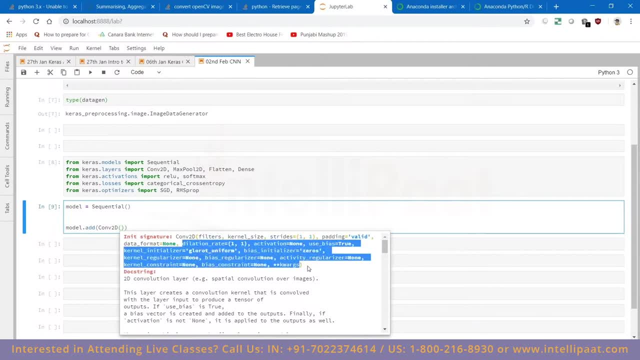 you have dilation now. after that, all you have dilation now. after that. all these are like uh, these are like uh, these are like uh, like default values. they already have like default values. they already have like default values. they already have some values. the only two things that it. 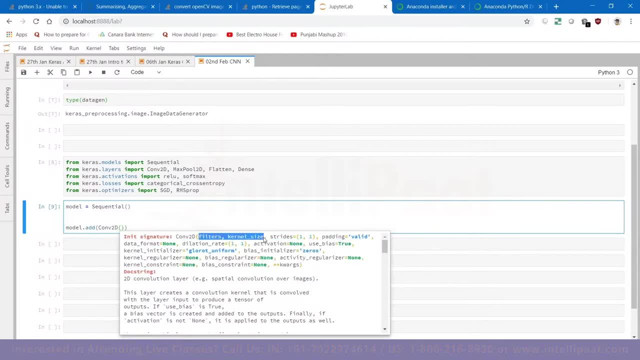 some values, the only two things that it some values, the only two things that it expects from you is: one is the filters. expects from you is: one is the filters. expects from you is: one is the filters and another one is the kernel size now and another one is the kernel size now. 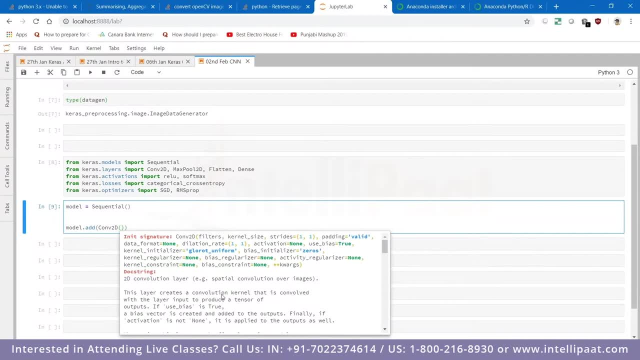 and another one is the kernel size. now, filters is nothing but it's the number. filters is nothing but it's the number. filters is nothing but it's the number of different types of filters, that you, of different types of filters, that you, of different types of filters, that you want, random filters that you want to run. 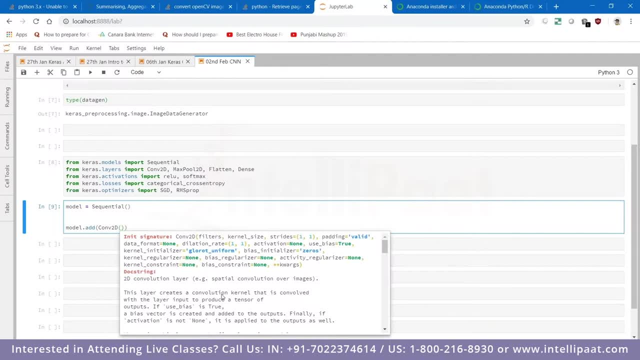 want random filters that you want to run, want random filters that you want to run on your image right and second is the on your image right and second is the on your image right and second is the kernel size. now, when you're making this kernel size, now, when you're making this, 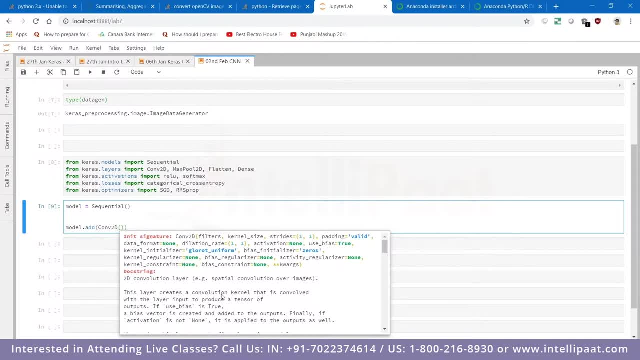 kernel size. now, when you're making this filter, how, what? what should be the size filter? how, what? what should be the size filter? how, what? what should be the size of the particular? you know, filter that of the particular. you know, filter that of the particular. you know, filter that you are going to run on the image, right? 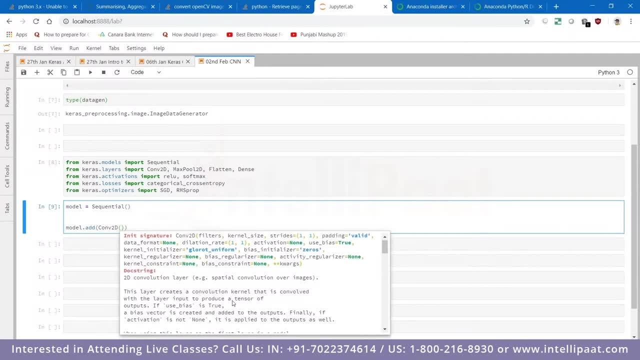 you are going to run on the image, right, you are going to run on the image, right. you're telling you, tell you will be, you're telling you, tell you will be, you're telling you, tell you will be telling the conv 2d kiras that these are. 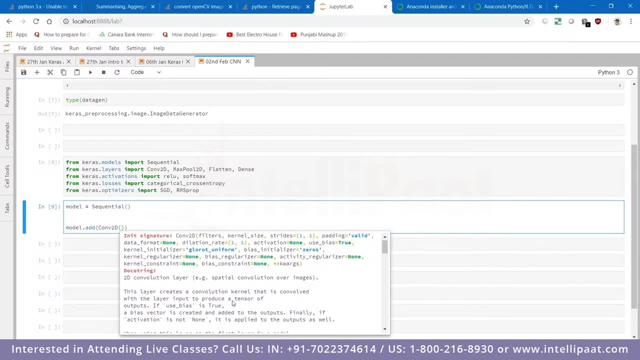 telling the conv 2d kiras that these are telling the conv 2d kiras that these are the number of filters that i will. let's the number of filters that i will. let's the number of filters that i will. let's say i use 64 filters and this should be. 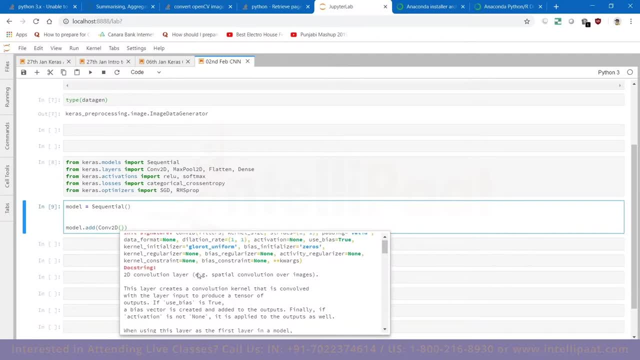 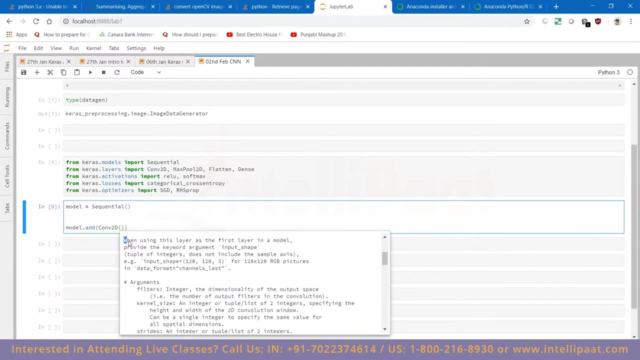 say i use 64 filters, and this should be say i use 64 filters, and this should be the size, the size, the size. let's see more deeper into this. see now one more important thing when- see now one more important thing, when- see now one more important thing- when you're using this layer as the first. 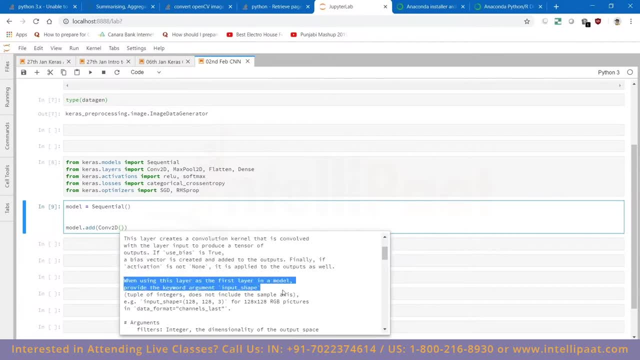 you're using this layer as the first. you're using this layer as the first layer in the model. provide the keyword layer in the model. provide the keyword layer in the model. provide the keyword input shape. so you have to make sure input shape. so you have to make sure. 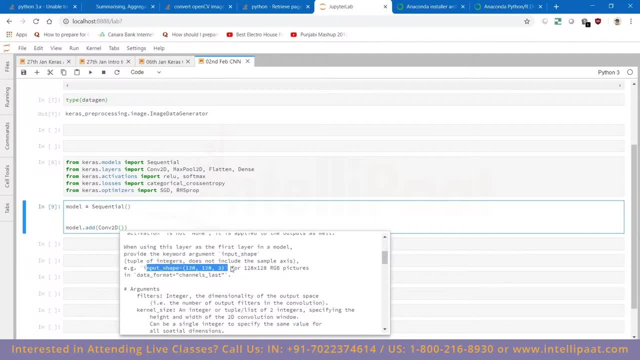 input shape. so you have to make sure that you're providing the input shape, that you're providing the input shape, that you're providing the input shape right and your input shape is equal to right and your input shape is equal to right and your input shape is equal to 20, 20, 28. 3 means that for uh, 20, 20, 28. 20, 20, 28, 3 means that for uh 20, 20, 28, 20, 20, 28, 3 means that for uh 20, 20, 28. rgb pictures: right, and you have to make. rgb pictures, right, and you have to make. 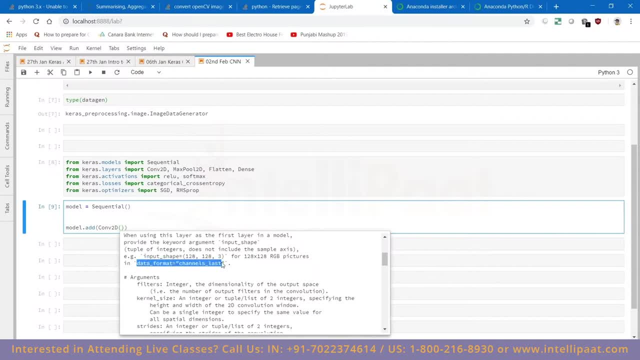 rgb pictures. right, and you have to make sure that your data format is equal to sure that your data format is equal to sure that your data format is equal to channel equal to last. it means that channel equal to last. it means that channel equal to last. it means that whenever you're specifying your 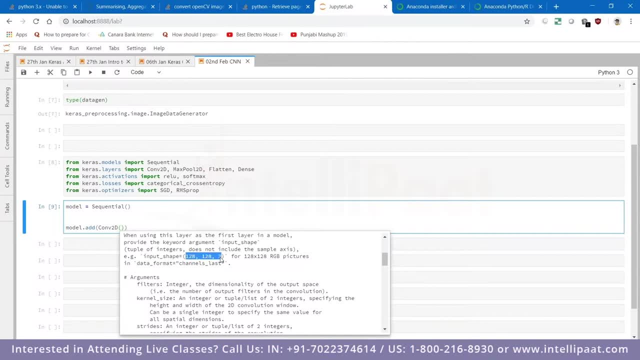 whenever you're specifying your, whenever you're specifying your dimension as 28 cross 28 cross 3. dimension as 28 cross 3. dimension as 28 cross 3. here 3 means that these are the number of here 3 means that these are the number of. 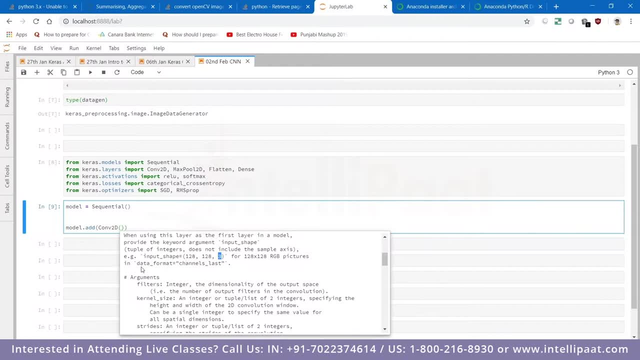 here, 3 means that these are the number of channels. but if you are giving 3 comma channels, but if you are giving 3 comma channels, but if you are giving 3 comma, 28, 28, make sure that you change your 28, 28, make sure that you change your. 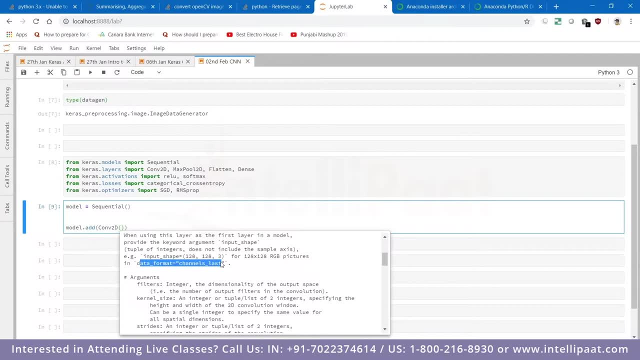 28, 28. make sure that you change your data format as channel first. so this data format as channel first, so this data format as channel first. so this used to happen a lot when there was. this used to happen a lot when there was. this used to happen a lot when there was this framework called. 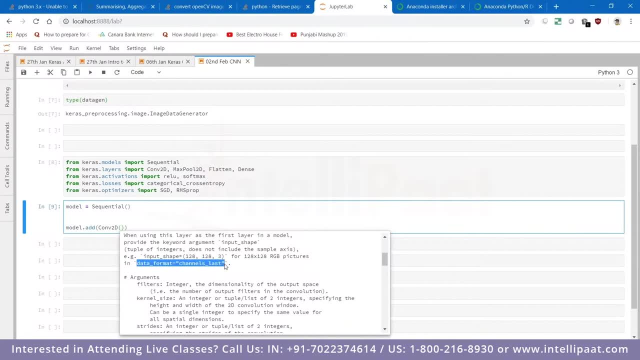 framework called framework called tiano. so tiano had this own format of tiano. so tiano had this own format of tiano. so tiano had this own format of having the channel first, then tensorflow, having the channel first, then tensorflow, having the channel first, then tensorflow came in. it said, no, i want the channel at. 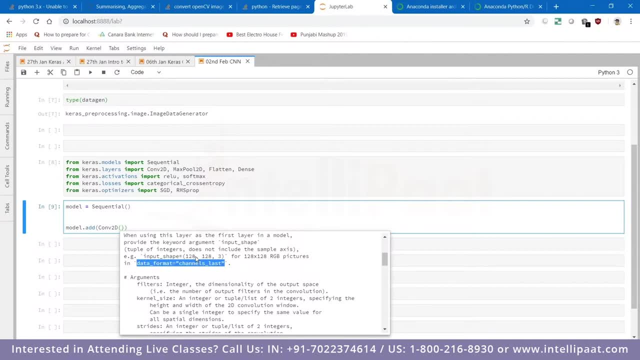 came in, it said no, i want the channel at. came in, it said no, i want the channel at the last. so there was this conflict a the last. so there was this conflict a the last, so there was this conflict a lot. so now you have to specify, because 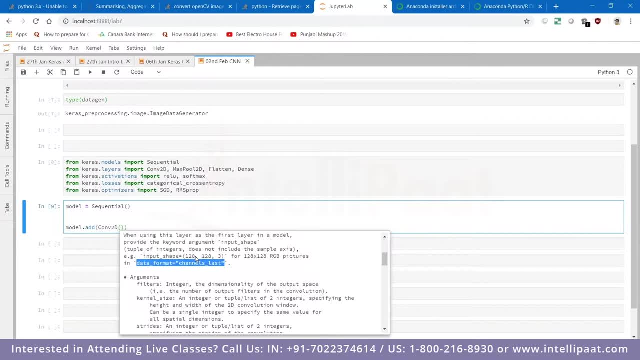 lot. so now you have to specify because lot. so now you have to specify because kia's used to support both tensorflow, kia's used to support both tensorflow. kia's used to support both tensorflow, and and and tiano backend. so it has this thing. 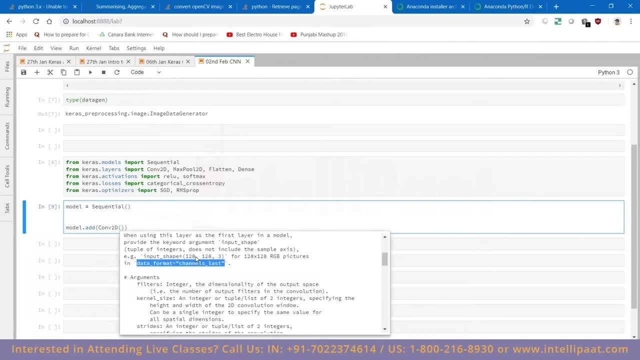 tiano backend, so it has this thing. tiano backend, so it has this thing called data format, where you can specify called data format, where you can specify called data format, where you can specify that that that you will be providing your channel, you will be providing your channel. 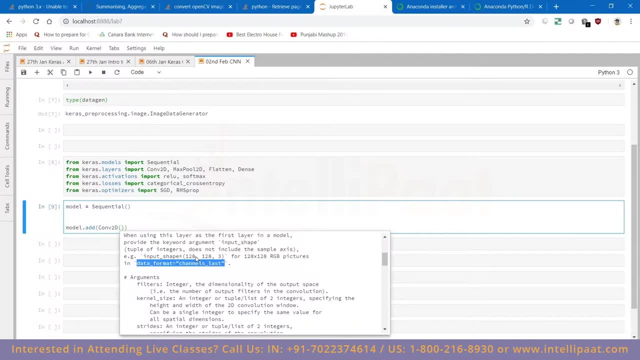 you will be providing your channel first, or channel last, right but first, or channel last, right but first, or channel last, right, but tiano ended in 2017, so 2017- yes. tiano ended in 2017, so 2017- yes. tiano ended in 2017, so 2017- yes, so you don't have to worry much about. 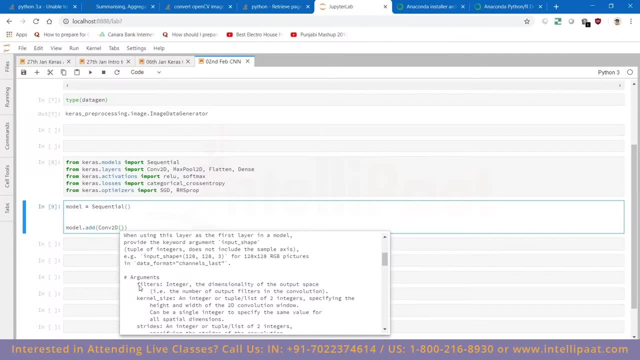 so you don't have to worry much about. so you don't have to worry much about data format. data format should be data format. data format should be data format. data format should be channel last, only channel last, only channel last, only filters. now, this filter, you are expected. 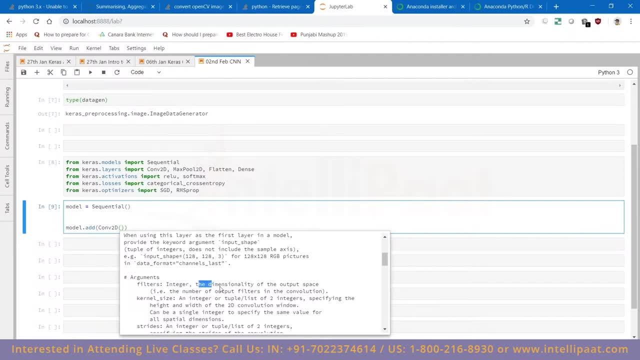 filters, now this filter. you are expected filters, now this filter. you are expected to enter a integer here. to enter a integer here. to enter a integer here, now integer, it means that the now integer, it means that the now integer, it means that the dimensionality of the outer space. dimensionality of the outer space. dimensionality of the outer space, that is the number of the output filter, that is the number of the output filter, that is the number of the output filter. and the convolution. it means, let's say: and the convolution, it means, let's say: 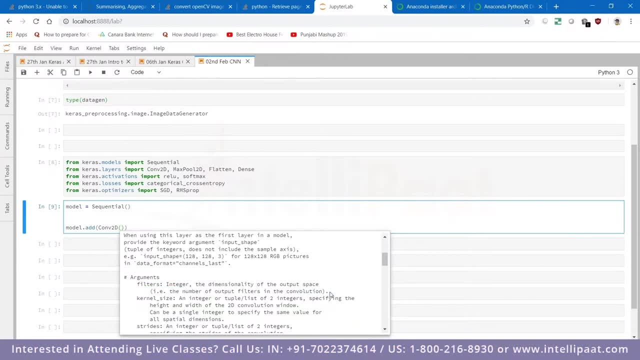 and the convolution. it means, let's say, if you give it numbers 32, it means there. if you give it numbers 32, it means there. if you give it numbers 32, it means there are 32 different filters. are 32 different filters, are 32 different filters, random filters that will run on the 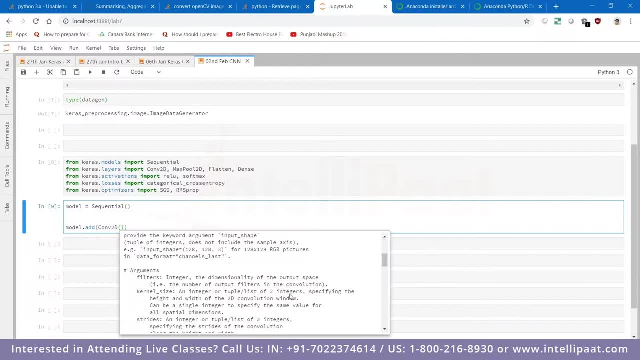 random filters that will run on the random filters that will run on the image and they will produce the image, and they will produce the image and they will produce the convoluted image. convoluted image, convoluted image. second, is the kernel size and integer or? 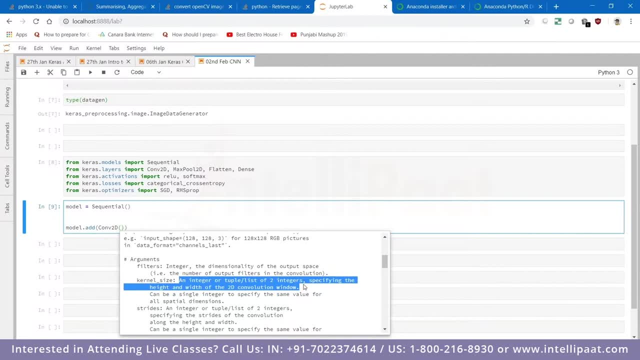 second is the kernel size and integer, or. second: is the kernel size and integer or tuple list of integer 2. specifying the tuple list of integer 2. specifying the tuple list of integer 2. specifying the height and width of the 2d convoluted. 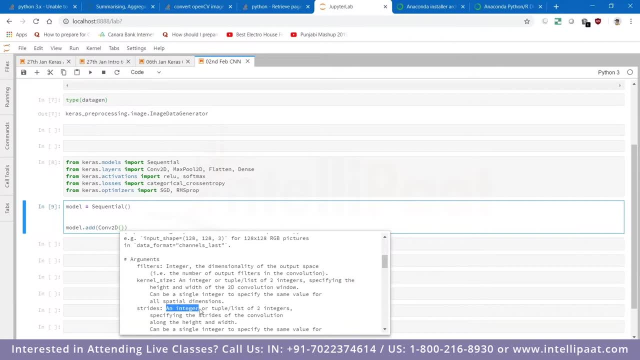 height and width of the 2d convoluted height and width of the 2d convoluted window. sides can be integer or double same as sides can be integer or double. same as sides can be integer or double same as above. uh, if you don't specify by default. 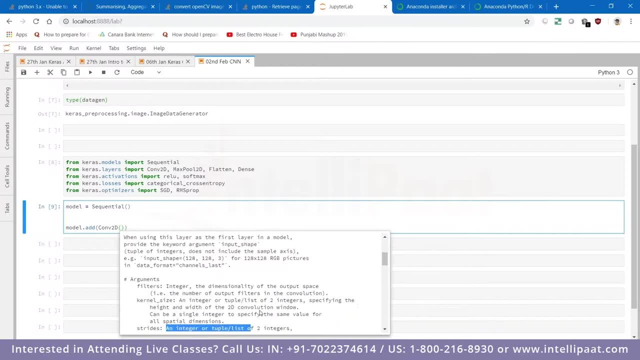 above uh. if you don't specify by default above uh. if you don't specify by default, it is uh, it is uh, it is uh. one one cross one, one, one cross, one, one, one cross one. right, then you have padding. padding is right, then you have padding padding is. 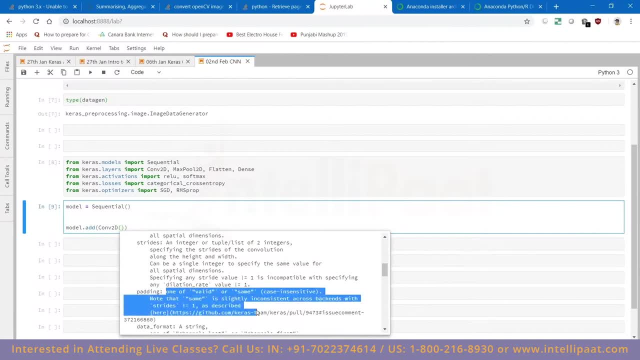 right. then you have padding. padding is either valid or same. either valid or same, either valid or same. right the right the right the. you know it is saying that same is. you know it is saying that same is. you know it is saying that same is slightly inconsistent across back end. 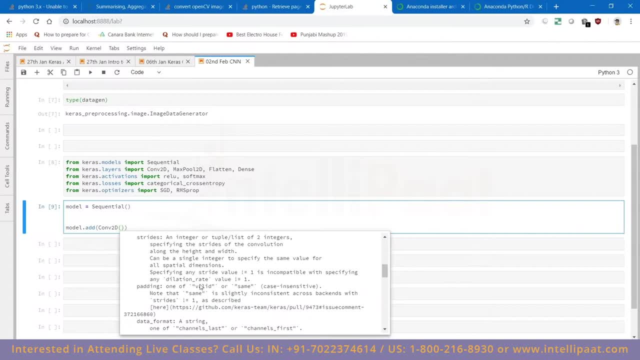 slightly inconsistent across back end. slightly inconsistent across back end. with side is equal to one as described with side is equal to one as described with side is equal to one as described here. so you should always take it as a here. so you should always take it as a. 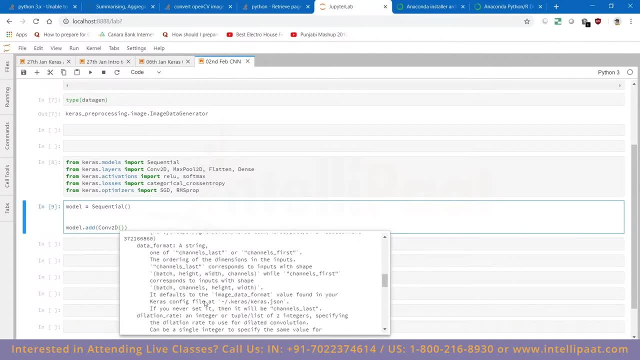 here. so you should always take it as a valid one, valid one. valid one works better then your data format. these works better then your data format. these works better then your data format. these are all like numbers that are already. are all like numbers that are already. are all like numbers that are already predefined. you don't have to look much. 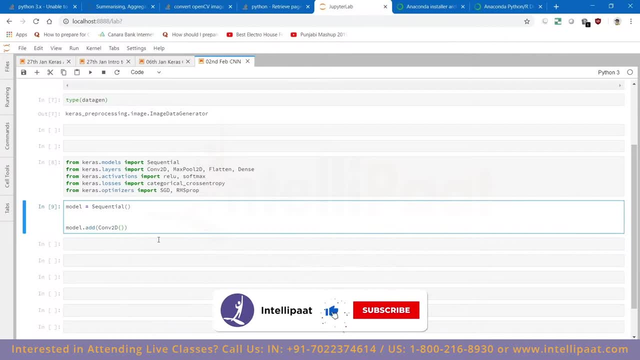 predefined, you don't have to look much predefined, you don't have to look much about it. but let's start with the about it. but let's start with the about it. but let's start with the convolution uh 2d. convolution uh 2d. convolution uh 2d. that we have to make right. just a quick. 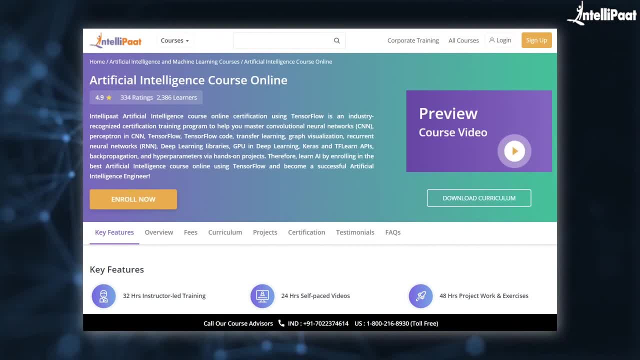 that we have to make right just a quick, that we have to make right just a quick. info guys, info guys, info guys. intellipaat provides artificial intellipaat provides. artificial intellipaat provides artificial intelligence. online training mentored by intelligence. online training mentored by. 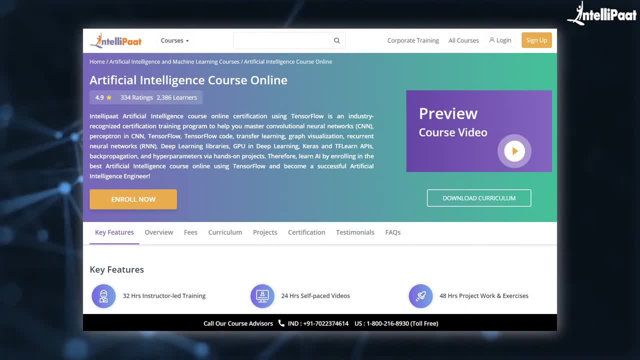 intelligence online training mentored by industry experts, industry experts, industry experts, the course link of which is given in the, the course link of which is given in the, the course link of which is given in the description below: description below, description below. now let's continue with the session. let's. 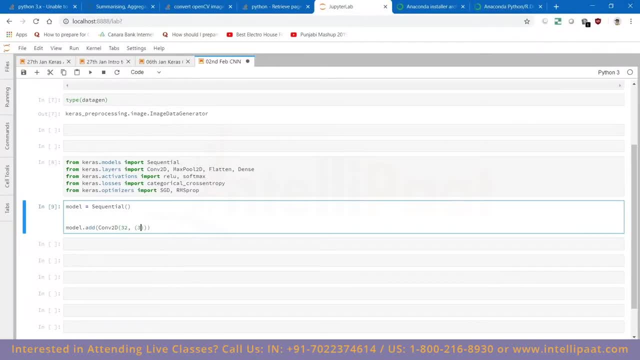 now let's continue with the session. let's now let's continue with the session. let's say that we want 32, say that we want 32, say that we want 32. 32 images of 3 cross 3. 32 images of 3 cross 3. 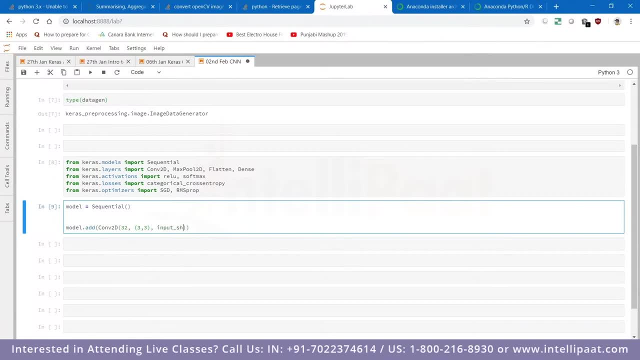 32 images of 3 cross, 3, right, right, right. next it: you have to give it as a input. next it, you have to give it as a input. next it, you have to give it as a input: shape, shape, shape, input, shape. let's say that we are going. 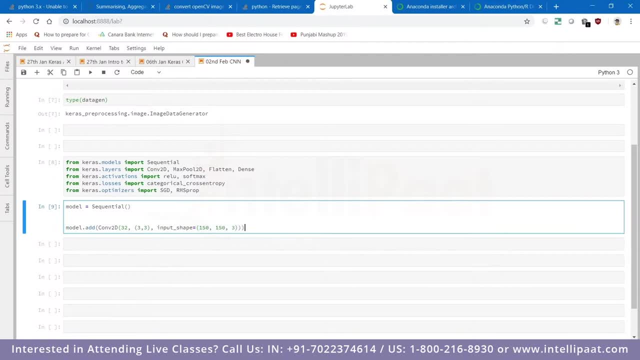 input shape. let's say that we are going. input shape. let's say that we are going to give 150 cross, 150 cross 3. to give 150 cross, 150 cross 3. to give 150 cross, 150 cross 3. we are going to give, we have still not. 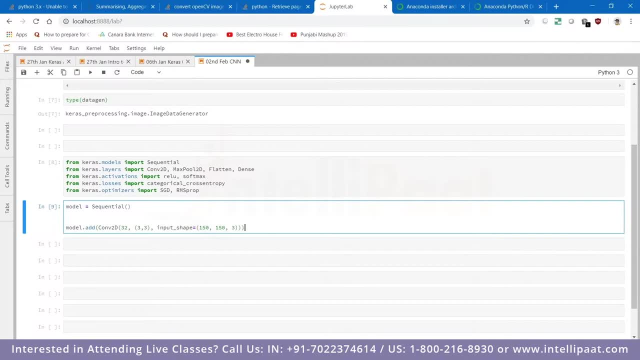 we are going to give. we have still not. we are going to give. we have still not given. we have still not decided how our given. we have still not decided how our given. we have still not decided how our shapes of the input will look like. but shapes of the input will look like, but. 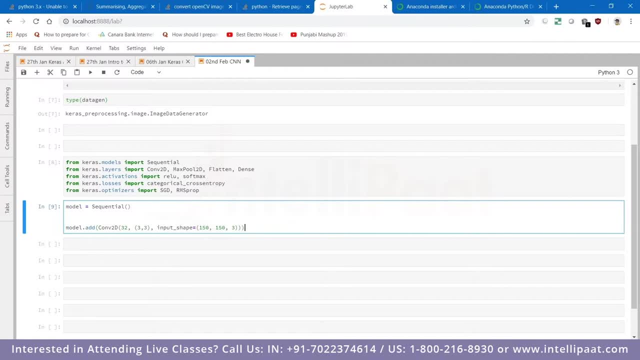 shapes of the input will look like. but we have decided, let's, we'll go with 150. we have decided, let's, we'll go with 150. we have decided, let's, we'll go with 150 cross, 150, cross, cross, cross, 3. now, once you have specified this, 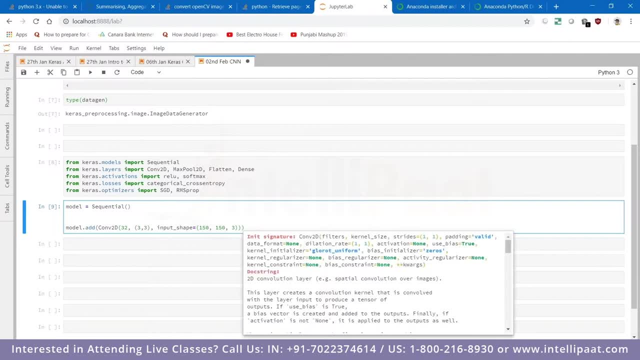 3: now, once you have specified this 3, now, once you have specified this convolution, you have to specify a convolution. you have to specify a convolution. you have to specify a activation function also right. either you activation function also right, either you activation function also right, either you can specify here only in this: 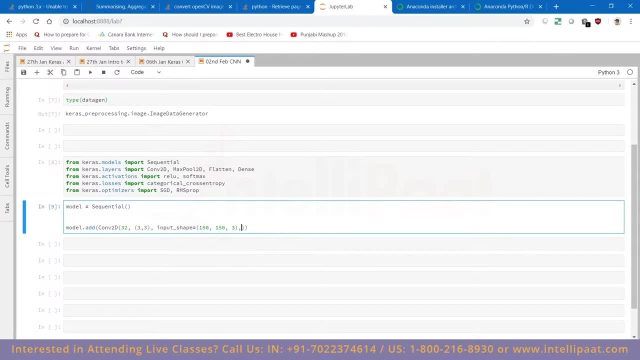 can specify here, only in this. can specify here, only in this. con thing. you can just go and say con thing. you can just go and say con thing. you can just go and say activation is equal to, or you can activation is equal to, or you can activation is equal to, or you can specify uh by again saying here: model. 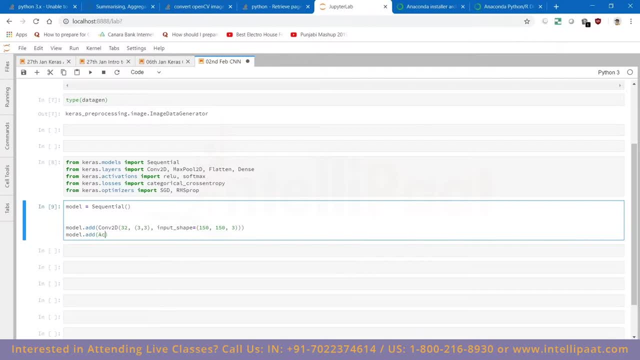 specify uh by again saying here: model. specify uh by again saying here: model, dot add, and then you can have a dot add, and then you can have a dot add, and then you can have a activation is equal to okay, we have not. activation is equal to okay, we have not. 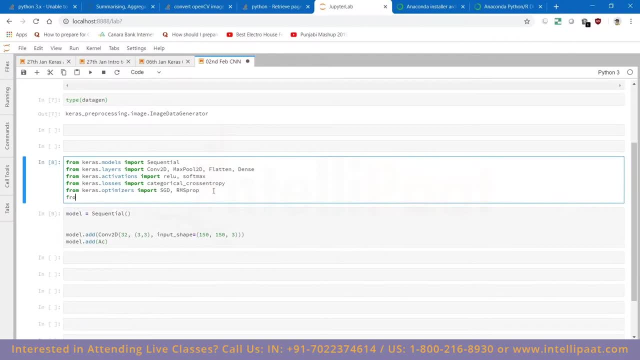 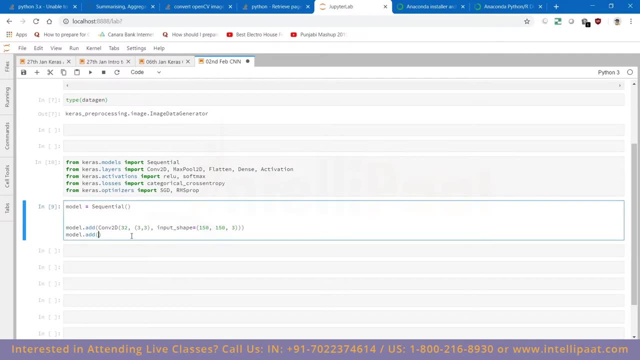 activation is equal to okay. we have not gone here from, gone here from gone here from okay. so you can add an activation layer here. so you can add an activation layer here. so you can add an activation layer here also also. also, i generally don't like this, i just add. 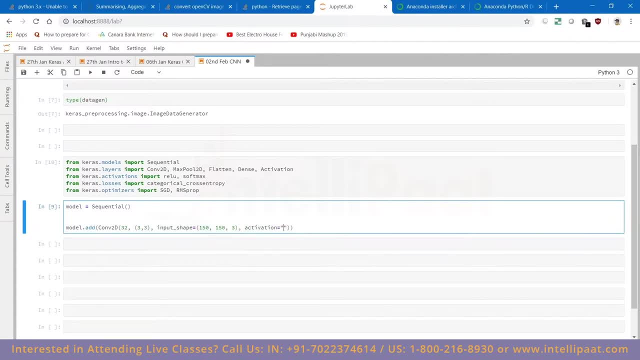 i generally don't like this, i just add: i generally don't like this, i just add it here, only it here. only it here, only activation activation. we love relo, we'll activation activation. we love relo. we'll activation activation. we love relo. we'll go with relu only. 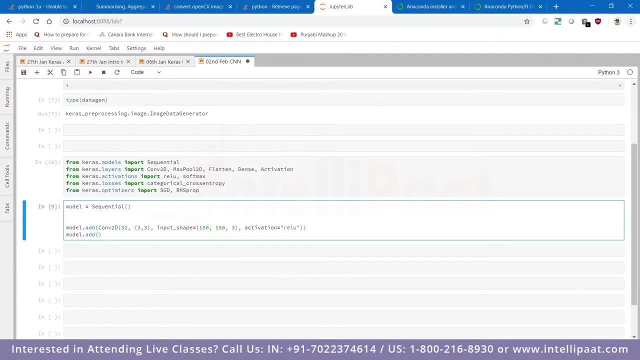 go with relu, only go with relu, only relu is the most important thing. okay, now, relu is the most important thing. okay now, relu is the most important thing. okay now, after convolution, and then doing an after convolution, and then doing an after convolution and then doing an activation. what was the next step that we 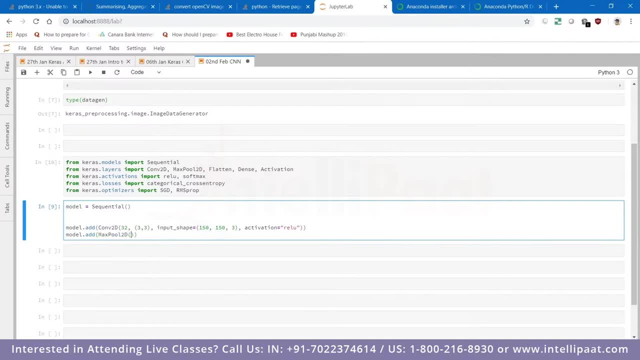 activation. what was the next step that we activation? what was the next step that we used to do, used to do, used to do? we used to have a max pool, max pool. we used to have a max pool, max pool. we used to have a max pool, max pool. again, let's go. 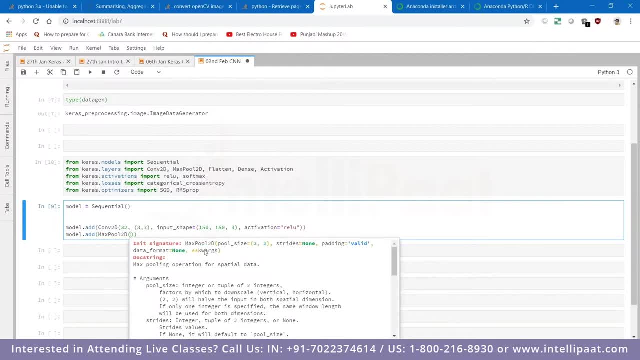 again. let's go again. let's go. max pool. what was max pool doing? max pool, max pool. what was max pool doing? max pool, max pool. what was max pool doing? max pool was doing nothing, but it was was doing nothing, but it was was doing nothing, but it was bifurcating your image into. 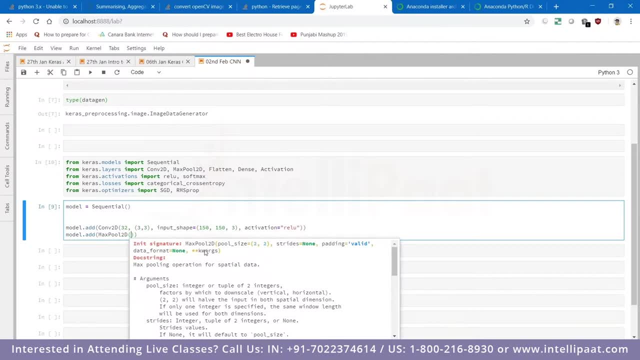 bifurcating your image into bifurcating your image into parts that you specify, and then picking parts that you specify, and then picking parts that you specify and then picking up, the up, the up, the maximum value out of it. right so it's maximum value out of it, right so it's. 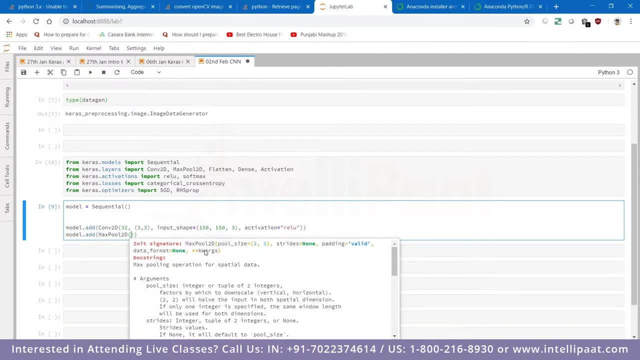 maximum value out of it, right? so it's saying that your image, let's say the saying that your image, let's say the saying that your image. let's say the pool size is two cross two. it means that pool size is two cross two. it means that 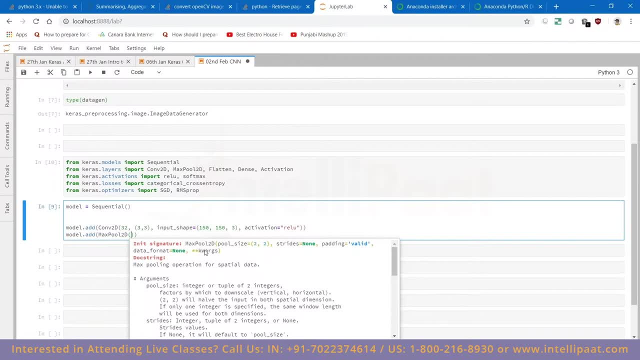 pool size is two cross two. it means that the? the image will start from the the the image will start from the the the image will start from the kernel size of two cross two, and then kernel size of two cross two, and then kernel size of two cross two, and then out of that four values, it is going to 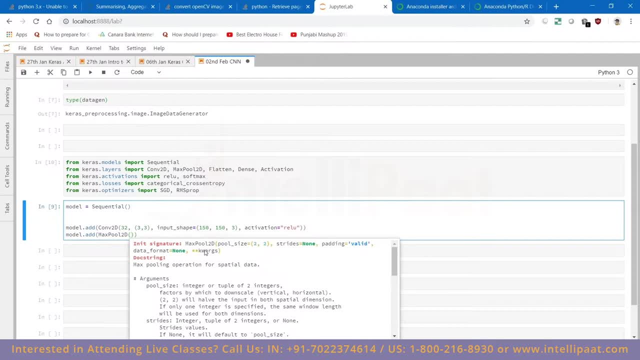 out of that four values. it is going to. out of that four values, it is going to take the one which is the maximum number. take the one which is the maximum number. take the one which is the maximum number, right? but let's say we want to change. 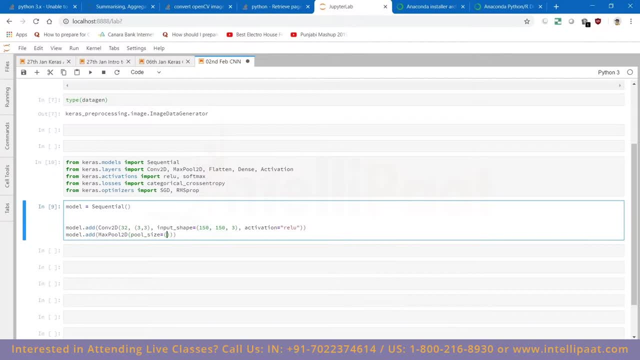 right, but let's say we want to change right. but let's say we want to change this. how to change this? you say: pool this. how to change this? you say: pool this. how to change this? you say: pool size. pool size is equal to, let's say, we. 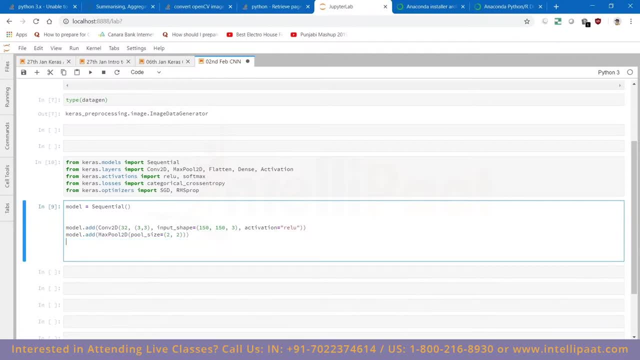 size. pool size is equal to: let's say we size. pool size is equal to: let's say we take it two cross two ones now this. take it two cross two ones now this. take it two cross two ones. now this thing that we have written till these. 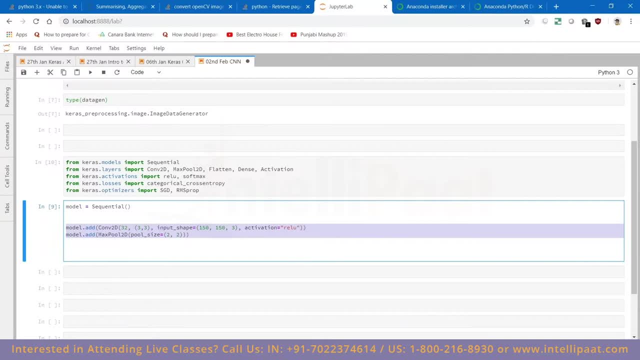 thing that we have written till, these thing that we have written till these three lines, these two lines, which three lines, these two lines, which three lines, these two lines which contain three specific operations. this contain three specific operations. this contain three specific operations. this thing is called as the chunk. 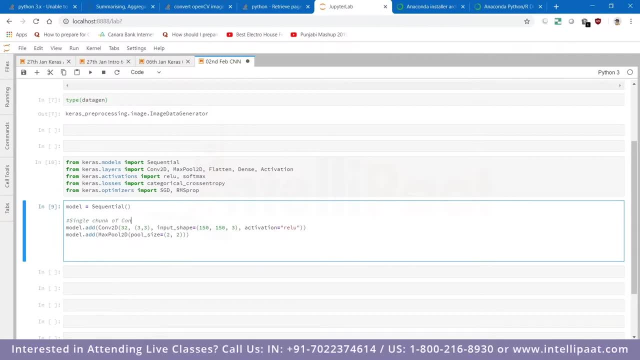 single chunk of convo solution. single chunk of convo. single chunk of convo, these three steps, uh, what, which one is these three steps? uh, what, which one is these three steps? uh, what, which one is? the one one is conv, the one one is conv, the one one is conv. then you have activation and then you have 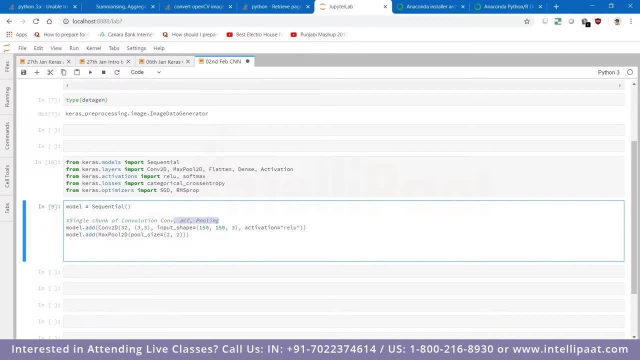 then you have activation and then you have, then you have activation and then you have pooling, pooling, pooling. these three things together are called. these three things together are called. these three things together are called as the chunk of now. what you can do is as the chunk of now. what you can do is: 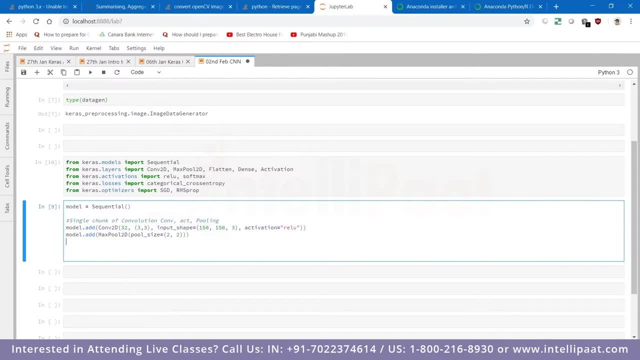 as the chunk of now. what you can do is you can just copy paste these things and you can just copy paste these things and you can just copy paste these things, and then you can have more chunks, but this, then you can have more chunks, but this, then you can have more chunks, but this time you have to make sure that you are. 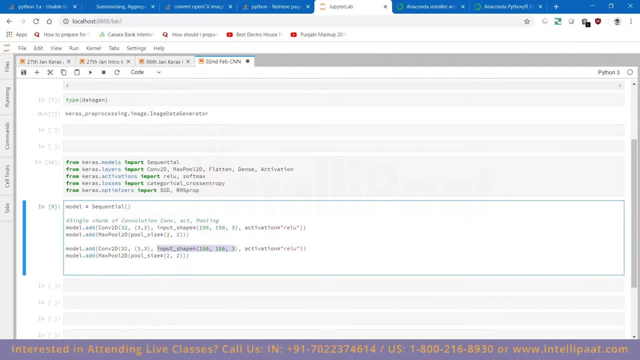 time. you have to make sure that you are time. you have to make sure that you are not using this input size because input not using this input size, because input not using this input size, because input size should always be inside your size, should always be inside your. 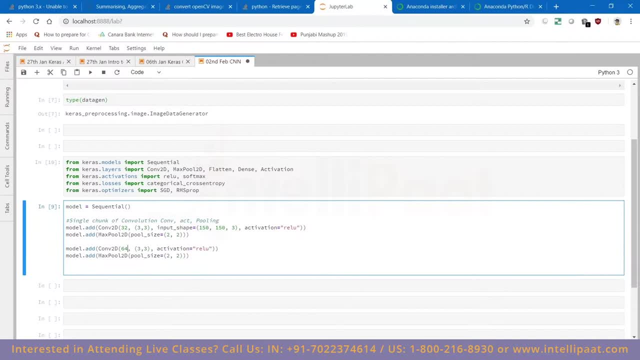 size should always be inside your first thing, only first thing, only first thing only. i'll increase this number to 64 here, or i'll increase this number to 64 here, or i'll increase this number to 64 here, or let's say: let's keep it 32 only. 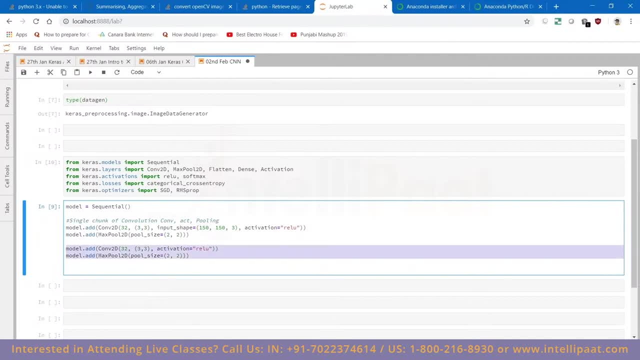 let's say: let's keep it 32 only. let's say: let's keep it 32 only. again, i will copy this thing again. i will copy this thing again. i will copy this thing. let's make three chunks because our data. let's make three chunks because our data. 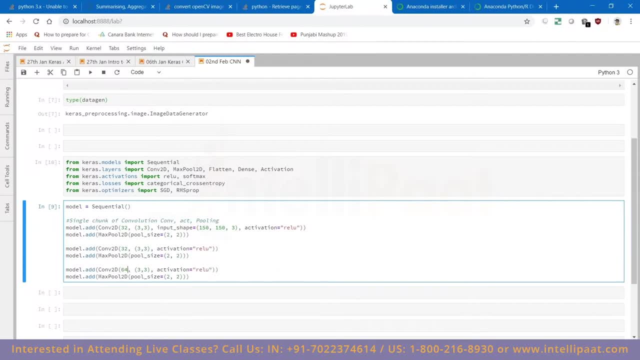 let's make three chunks, because our data is not that much complex. is not that much complex? is not that much complex? let's have 32 34 64, let's have 32 34, 64, let's have 32 34 64, and then come here and then you have. 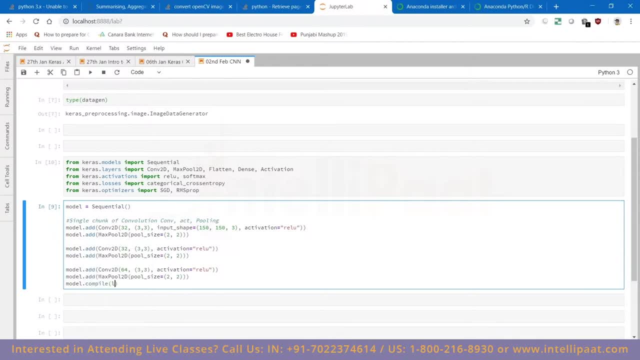 and then come here, and then you have, and then come here, and then you have modelcompile, modelcompile, modelcompile, right, compile me you have. loss is equal right. compile me you have. loss is equal right, compile me you have. loss is equal to categorical cross entropy, to categorical cross entropy. 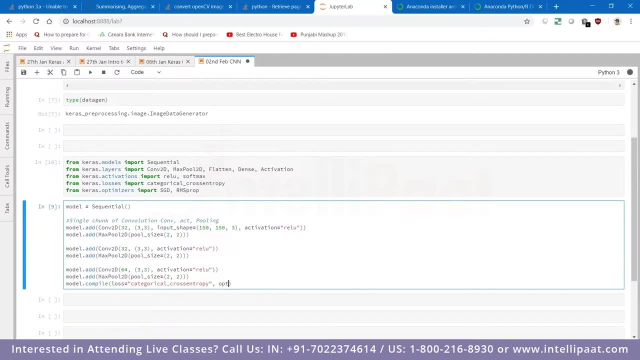 to categorical cross entropy. let's find it in double quotes, then you, let's find it in double quotes, then you, let's find it in double quotes, then you have have, have optimizers. let's use sgd only. this is the optimizers. let's use sgd only. this is the. 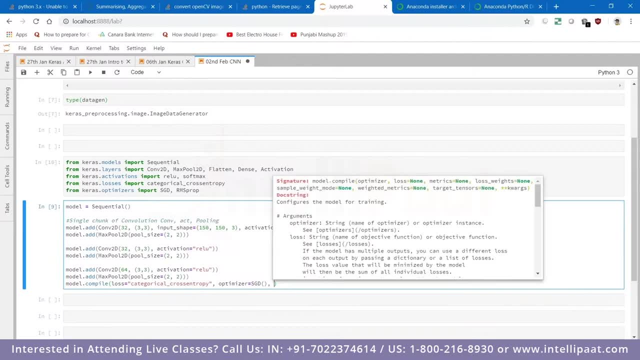 optimizers. let's use sgd. only. this is the one that converges, one that converges, one that converges the fastest, then you have matrix, the fastest, then you have matrix, the fastest, then you have matrix, matrix. let's use accuracy, matrix. let's use accuracy. 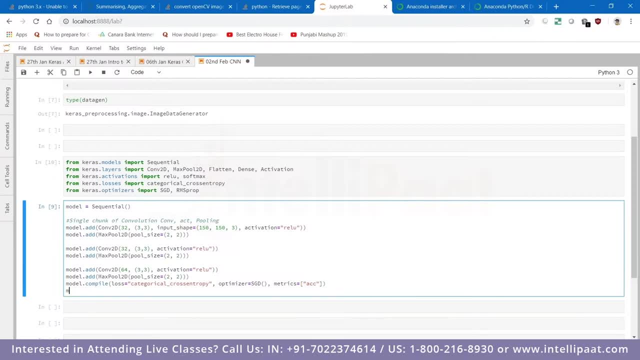 matrix. let's use accuracy, right, and then we'll do modelfit, but right, and then we'll do modelfit, but right, and then we'll do modelfit, but as of now, we don't have any uh input. as of now, we don't have any uh input. 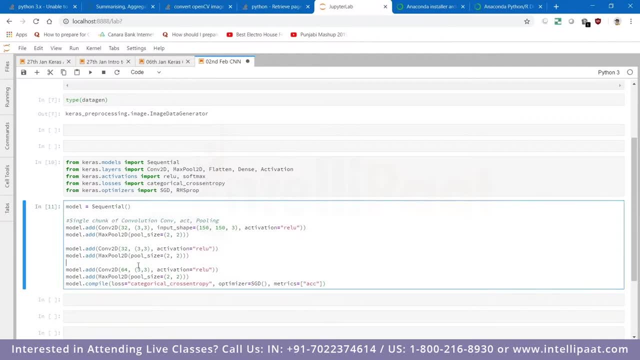 as of now, we don't have any uh, input, outputs, outputs, outputs. let's just make the model sit here, only. let's just make the model sit here. only let's just make the model sit here, only, right. nothing much to do so what we did, right, nothing much to do so what we did. 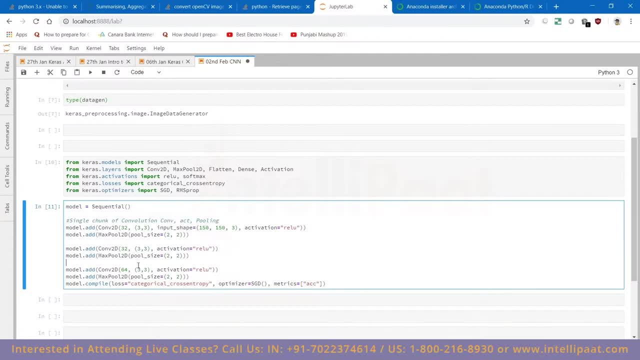 right, nothing much to do. so what we did actually here is we just made three. actually here is we just made three. actually here is we just made three convolution filters. one is this 32 when convolution filters. one is this 32 when convolution filters. one is this 32 when we started this off. 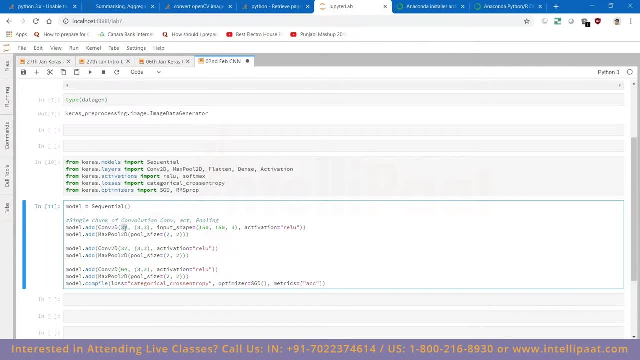 we started this off. we started this off 32. we said 32 numbers of different, 32. we said 32 numbers of different, 32, we said 32 numbers of different, different, different, different. so one let imagine this one image will. so one let imagine this one image will. 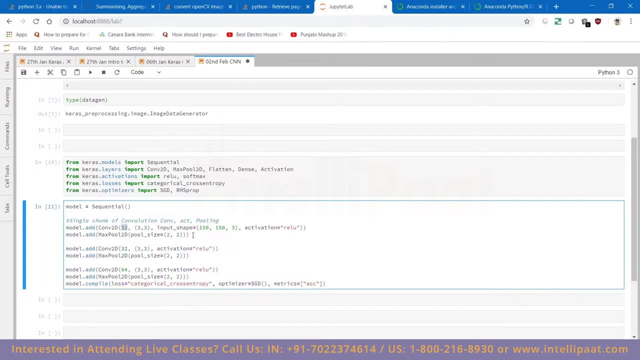 so one let imagine this one image will now become 32 images, but the size will now become 32 images. but the size will now become 32 images. but the size will drop due to max pooling right drop, due to max pooling right drop, due to max pooling right again, these 32 images will now become 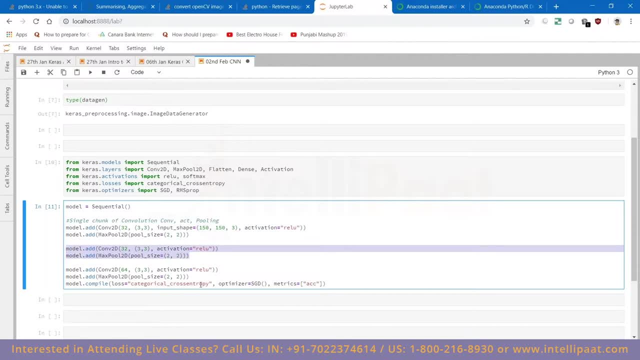 again. these 32 images will now become again. these 32 images will now become into 32, but their size will decrease into 32, but their size will decrease into 32, but their size will decrease again. the height width will decrease again. the height width will decrease. 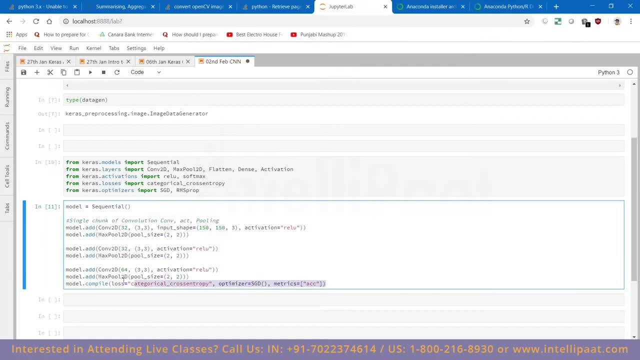 again. the height, width will decrease. now. these 62 will become now. these 62 will become now. these 62 will become almost like uh, almost like uh, almost like uh. what will they become? they'll become 64. what will they become? they'll become 64. 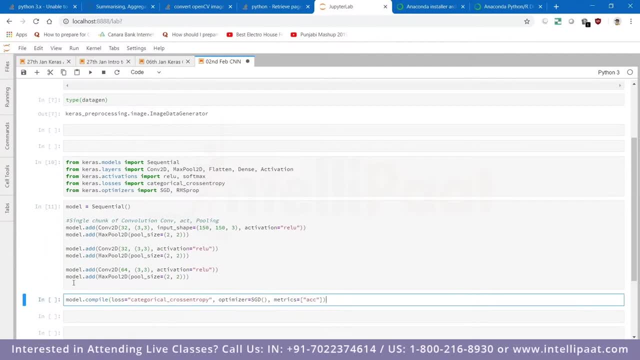 what will they become? they'll become 64, 64, so they'll become more. and that, so they'll become more, and that, so they'll become more. and that their uh, their height width will again their uh, their height width will again their uh, their height width will again decrease. a lot. one thing that i forgot: 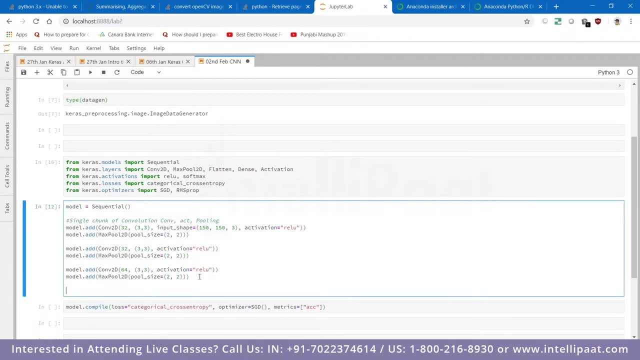 decrease a lot. one thing that i forgot decrease a lot. one thing that i forgot to tell you is that this is not the end. to tell you is that this is not the end. to tell you is that this is not the end. right, our end will be somewhere where. 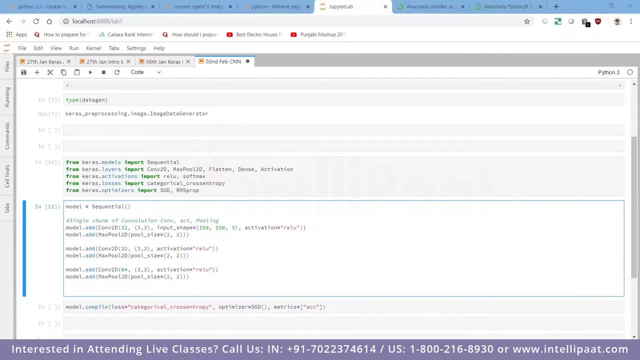 right, our end will be somewhere where. right, our end will be somewhere where the output will be only two units. the output will be only two units. the output will be only two units. right, this is not the output, right we? right, this is not the output, right we? 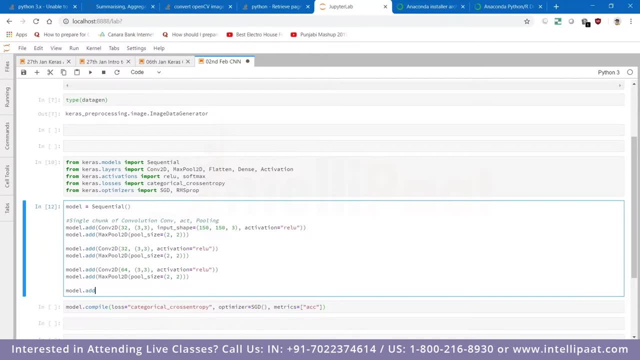 right, this is not the output. right, we have to do a flatten here, have to do a flatten here, have to do a flatten here. remember, because ultimately see our answer will, because ultimately see our answer will, because ultimately see our answer will not add once is flattening, we have done. 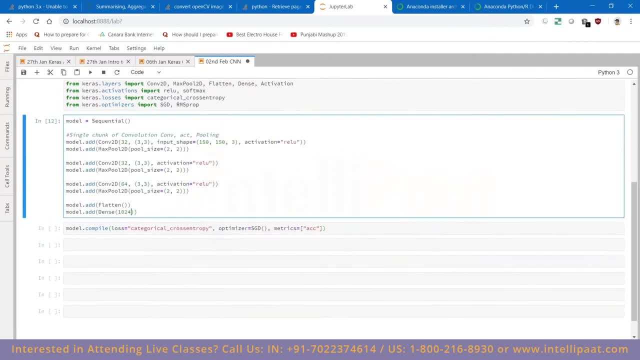 not add once is flattening we have done, not add once is flattening, we have done the flattening. then we might use a dense the flattening. then we might use a dense the flattening. then we might use a dense layer, layer, layer and slayer. let's say we take 1024, then 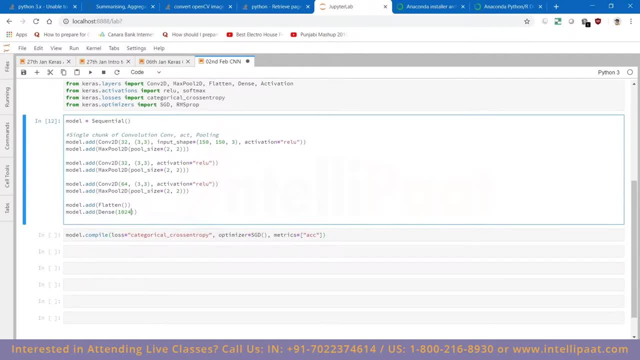 and slayer, let's say we take 1024, then and slayer, let's say we take 1024, then let's add, let's add, let's add activation. let me add it here, only in activation. let me add it here, only in activation. let me add it here only in this thing. 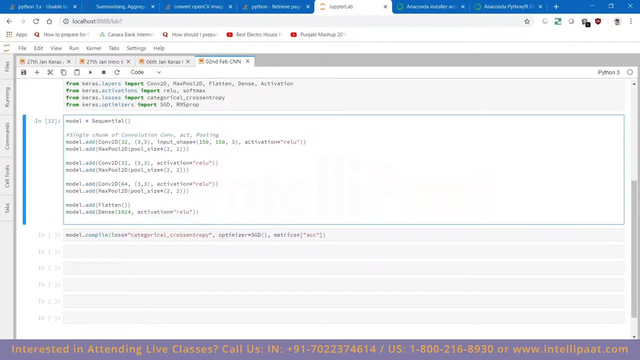 this thing, this thing: activation is equal to relu, activation is equal to relu, activation is equal to relu. then let's decrease this by then, let's decrease this by then, let's decrease this by, let's say, let's say, let's say: oh, five, one, two again have activation of. 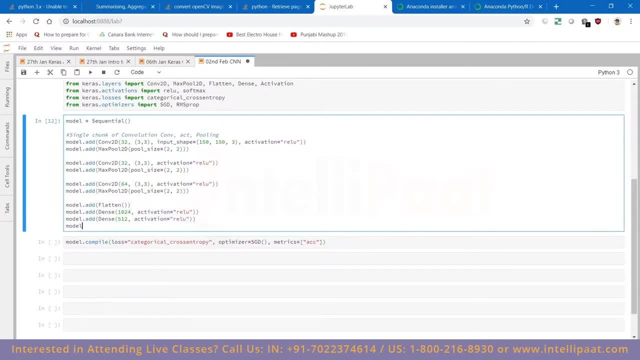 oh, five, one, two again have activation of. oh, five, one, two again have activation of relu, and then in the end let's have relu, and then in the end let's have relu, and then in the end let's have the final one. will have how many? only. 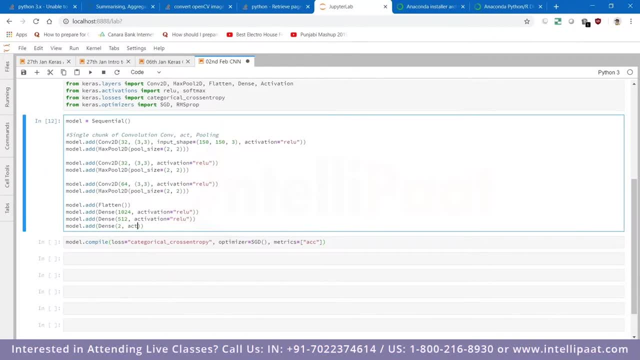 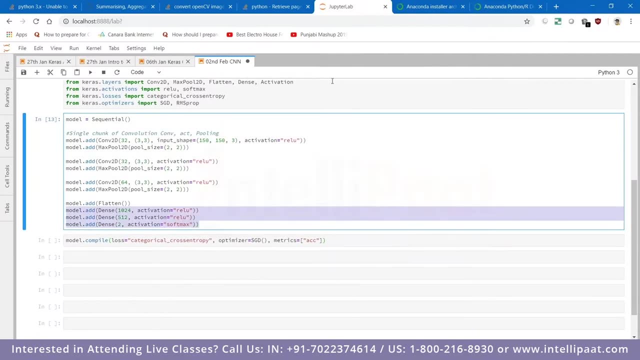 the final one will have how many? only the final one will have how many? only two, two, two dense and two, and this time the dense and two, and this time the dense and two, and this time the activation will be activation will be, activation will be softmax, right. so this will almost become like 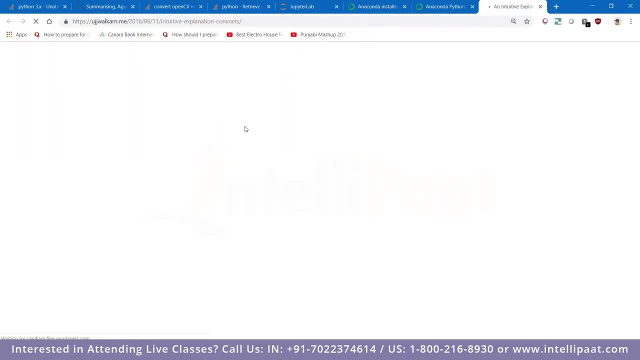 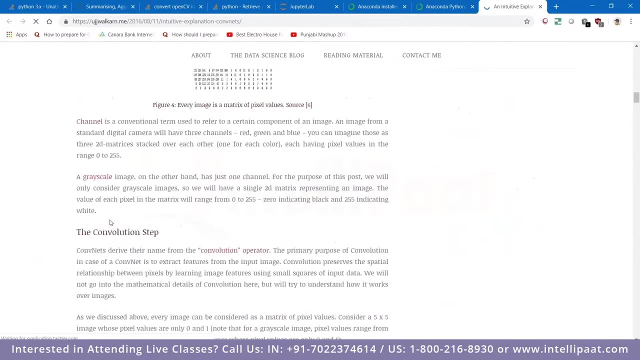 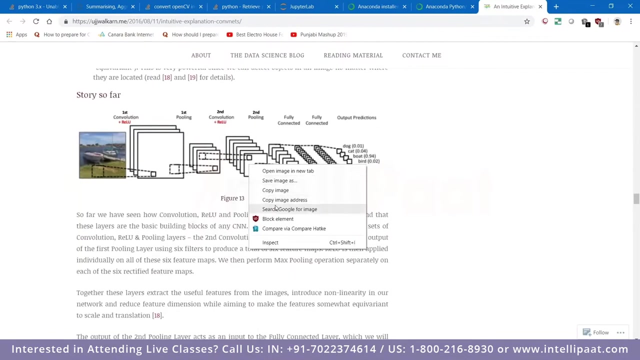 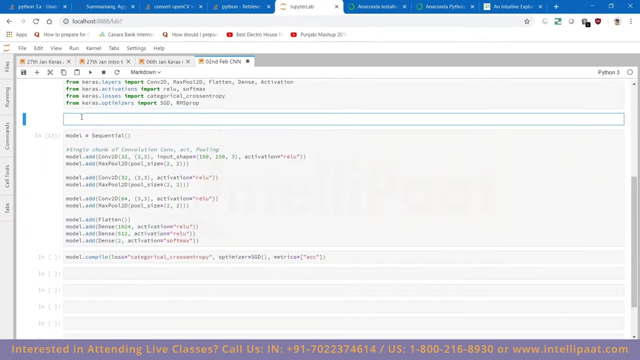 right, so this will almost become like right, so this will almost become like this. so our model should almost look like. so our model should almost look like. so our model should almost look like like this, like this, like this. just a second, does this look like the same? so first, 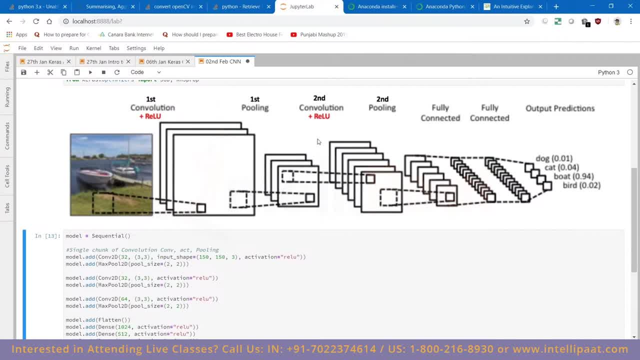 does this look like the same? so first does this look like the same? so first convolution, convolution, convolution, then boolean, then convolution, then boolean, then convolution, then boolean, then second convolution, then pooling, then second convolution, then pooling, then second convolution, then pooling. then imagine we have a third convolution also. 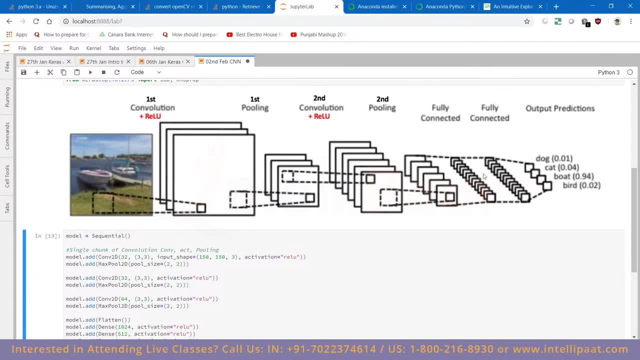 imagine we have a third convolution also. imagine we have a third convolution also. then we have a fully connected dense, then we have a fully connected dense, then we have a fully connected dense, layer, layer, layer, and then we are reducing the number of, and then we are reducing the number of. 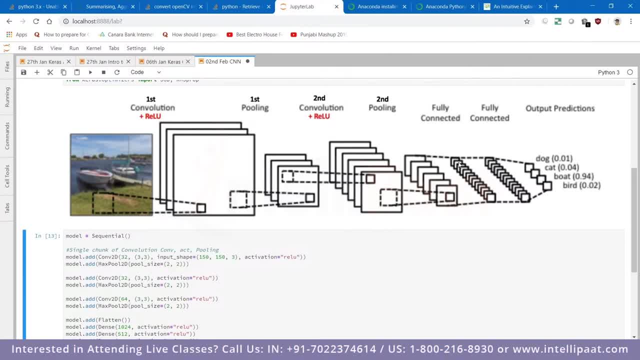 and then we are reducing the number of dense layers, dense layers, dense layers, from one one zero, two, four and five. one from one, one, zero, two, four and five. one from one one, zero, two, four and five, one, twelve and then immediately two, twelve and then immediately two. 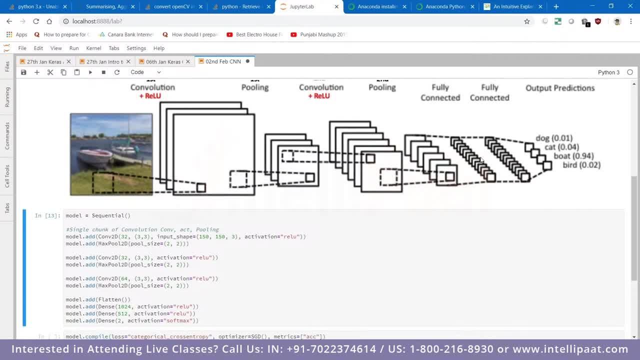 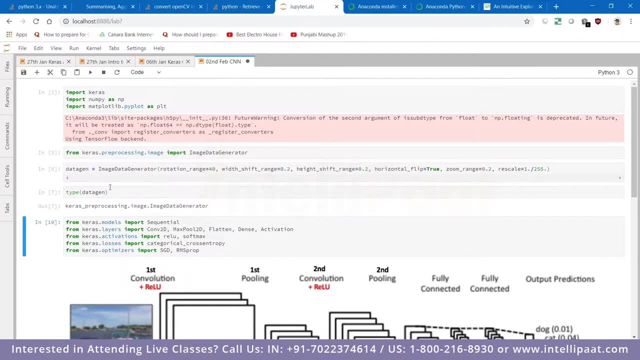 twelve and then immediately two. so this example has more, but this is so. this example has more, but this is so. this example has more, but this is somewhat like what, somewhat like what, somewhat like what. we have an inspiration code, right data generator. now what we have to do is: 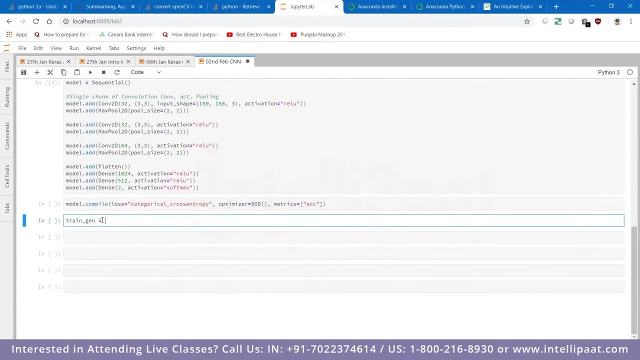 data generator. now, what we have to do is data generator. now, what we have to do is that we have to make a, that we have to make a, that we have to make a train generator. train gen is equal to train generator. train gen is equal to train generator. train gen is equal to data gen. dot flow from directory. 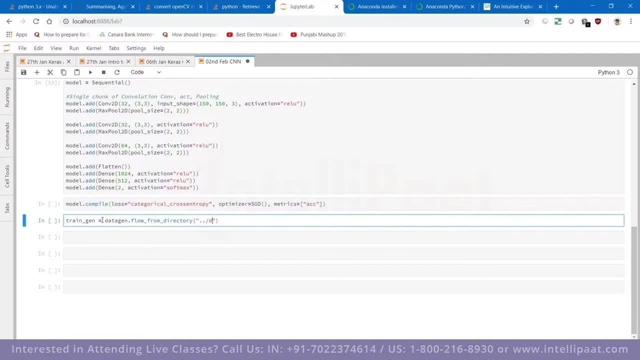 data gen dot flow from directory. data gen dot flow from directory. right flow from directory. where is where right flow from directory? where is where right flow from directory? where is, where is our data? our data is just behind. this is our data. our data is just behind this. 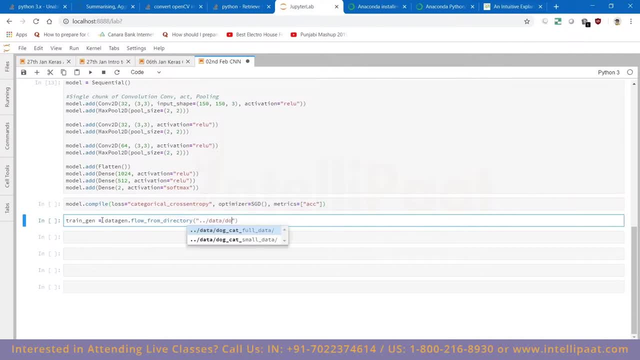 is our data, our data is just behind this. then we have, then we have, then we have cat top cat: yes, top cat. small cat top cat. yes, top cat. small cat top cat. yes, top cat small. uh-huh, we have more. uh-huh, we have more. 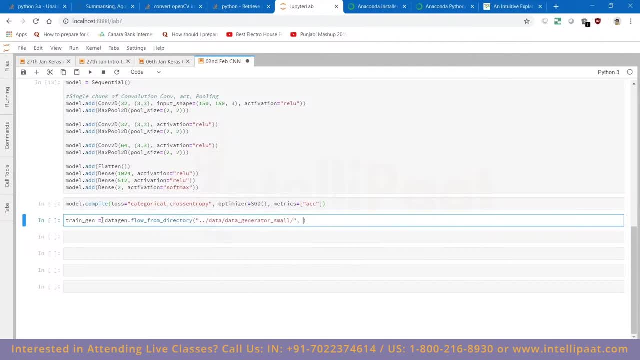 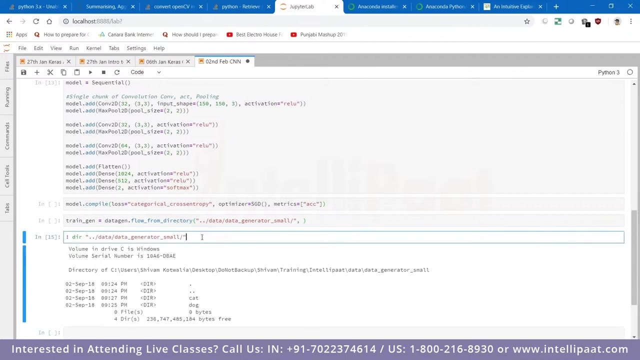 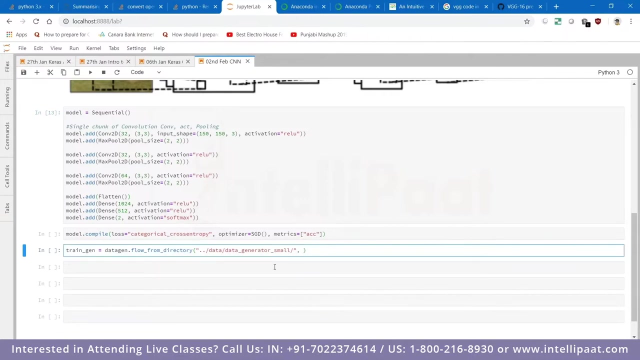 uh-huh, we have more generator, small generator, small generator, small. the format of this folder should pair. the format of this folder should pair. the format of this folder should pair. let me show you, let me show you, let me show you. you all know how the folder looks like. 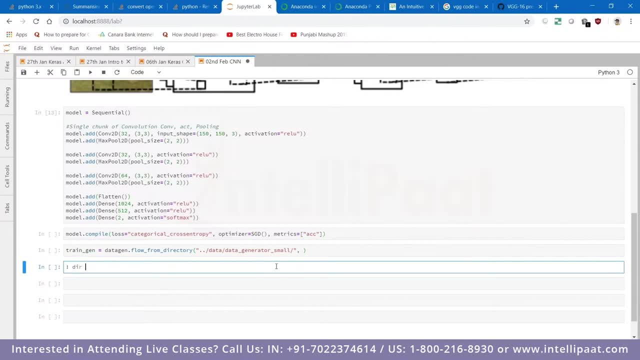 you all know how the folder looks like. you all know how the folder looks like right, right, right l dir is equal to. if i show you what is l dir is equal to. if i show you what is l dir is equal to. if i show you what is inside. 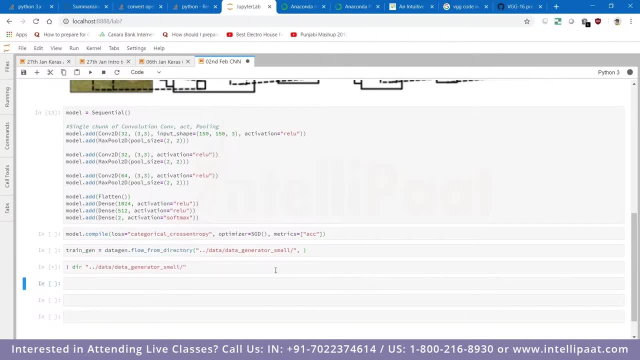 inside, inside. data generator small, then this is nothing. data generator small, then this is nothing. data generator small, then this is nothing. but the two folders category wise. but the two folders category wise. but the two folders category wise folders, right, these are category wise folders, right, these are category wise. 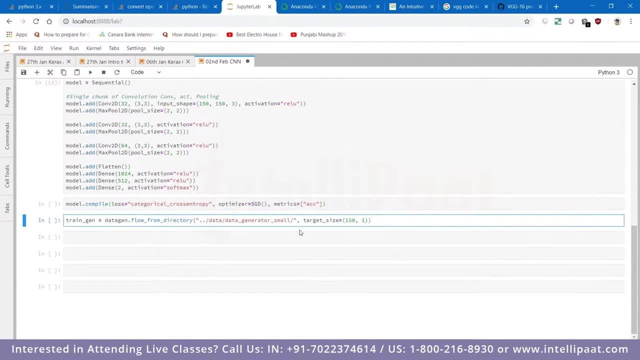 folders: right, these are category wise folders, okay, so let's move back here again. so we okay, so let's move back here again. so we okay, so let's move back here again. so we have a data generator here already. we have a data generator here already we. 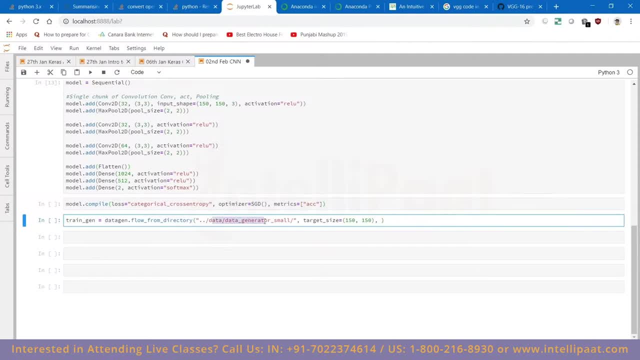 have a data generator here already. we will say that please go to this, will say that please go to this, will say that please go to this directory data generator- small directory data generator, small directory data generator, small- and then flow these images from this and then flow these images from this. 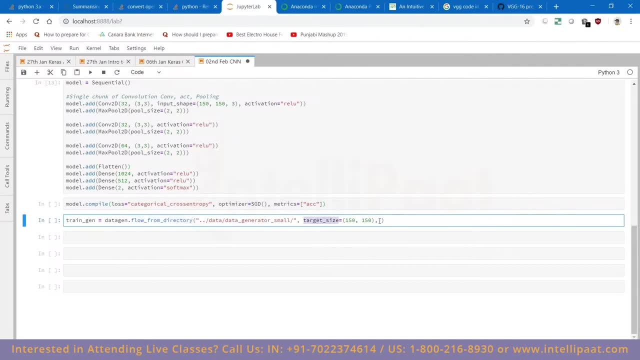 and then flow these images from this directory right, directory right, directory right. i am also telling it that you should. i am also telling it that you should. i am also telling it that you should have a target size of 150, so whatever. have a target size of 150, so whatever. 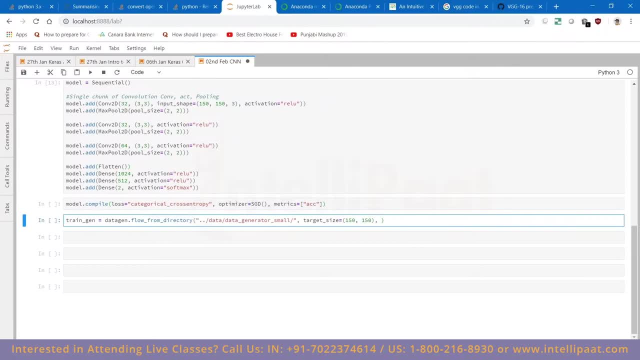 have a target size of 150. so whatever the size of the images, resize that the size of the images. resize that the size of the images. resize that image. say if your image was one zero image. say if your image was one zero image. say if your image was one zero: five, six, cross something, something. 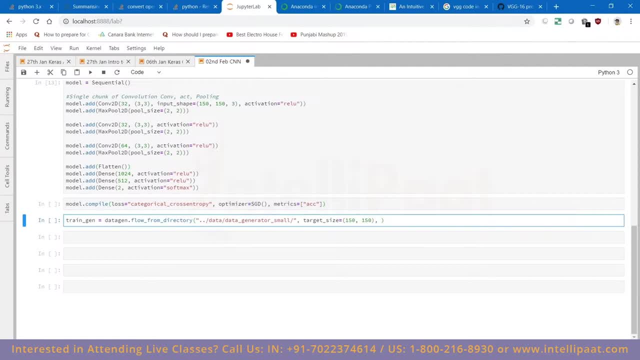 five, six cross something, something. five, six cross something, something, something. this is not getting cropped. this, this is not getting cropped. this is resizing the image right, so you are is resizing the image, right? so you are is resizing the image right? so you are saying that you want to convert your? 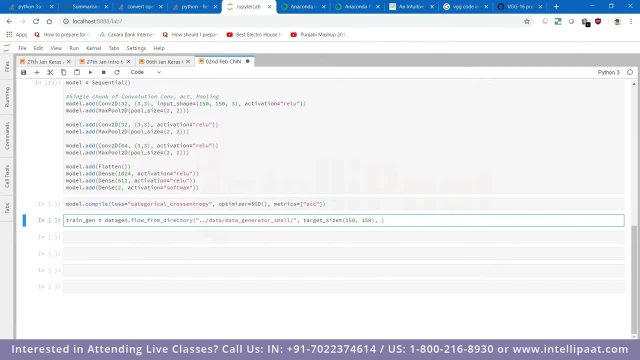 saying that you want to convert, your saying that you want to convert your image into this, then you have to give image into this. then you have to give image into this. then you have to give the batch size at how many images that the batch size at how many images that? 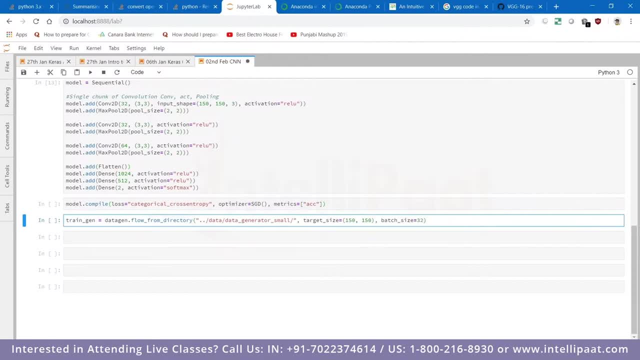 the batch size, at how many images that you want to read, right? let's say i want you want to read. right, let's say i want you want to read. right, let's say i want to read 32 images per batch. to read 32 images per batch. 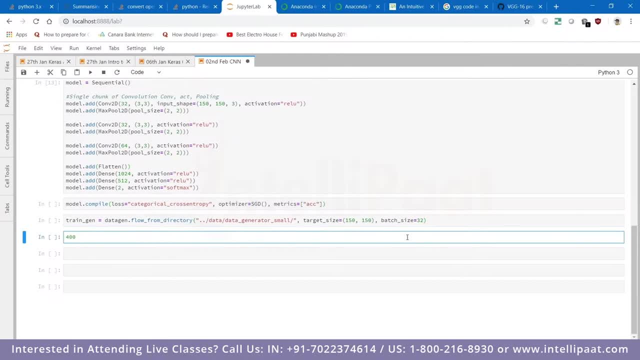 to read 32 images per batch. now, you remember, we have 400 images for now, you remember, we have 400 images for now, you remember, we have 400 images for all the classes, for all the two classes. now i am saying 32 batch size, 32 batch. 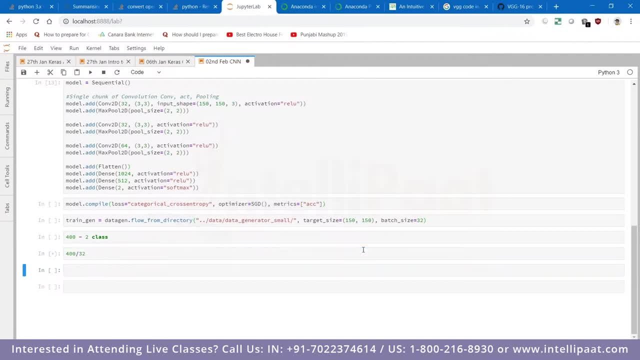 now i am saying 32 batch size, 32 batch. now i am saying 32 batch size. 32 batch size means that if i divide 400 with 32 size means that if i divide 400 with 32 size means that if i divide 400 with 32, it will give me around around 12. 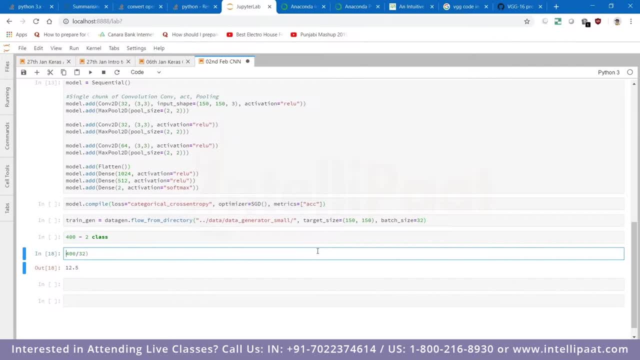 it will give me around around 12. it will give me around around 12, 12.5 or let's say 13, so this is always 12.5. or let's say 13, so this is always 12.5. or let's say 13, so this is always ceiling. 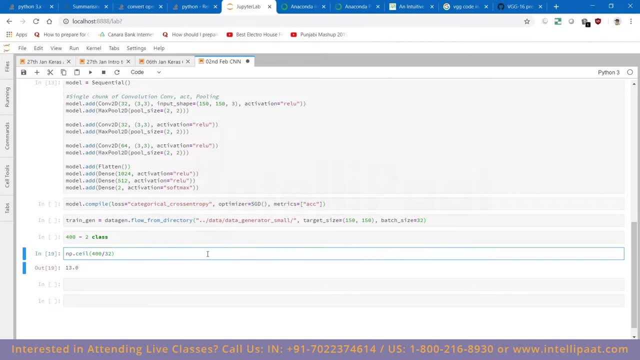 so this is all. this will always be a 13. so this is all. this will always be a 13. so this is all. this will always be a 13. to to to 13 buckets: we will have, so our epoch: 13 buckets we will have, so our epoch. 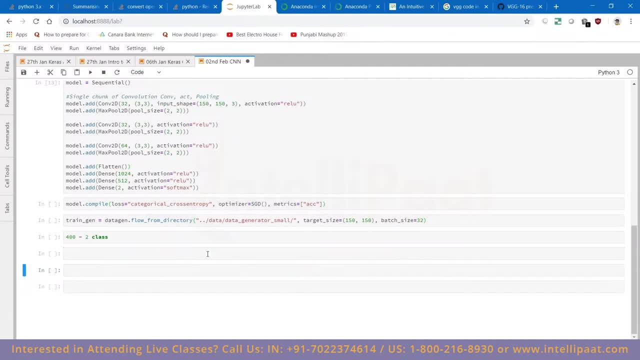 13 buckets we will have. so our epoch will show a count, will show a count, will show a count from 0 to 13, right batch size 32, and then we have batch size 32, and then we have batch size 32, and then we have. then what do we have? we have data. 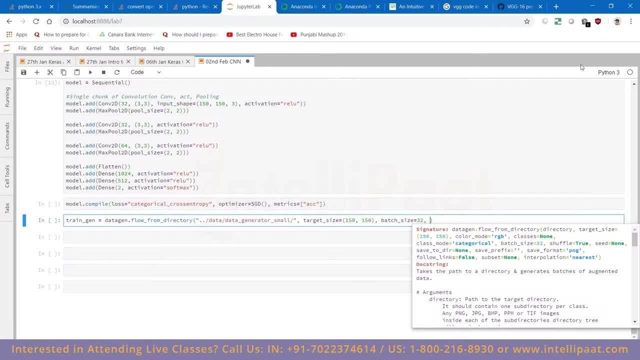 then what do we have? we have data. then what do we have? we have data generator. then we have color mode it's generator. then we have color mode it's generator. then we have color mode. it's already rgb, then we have classes is already rgb, then we have classes is. 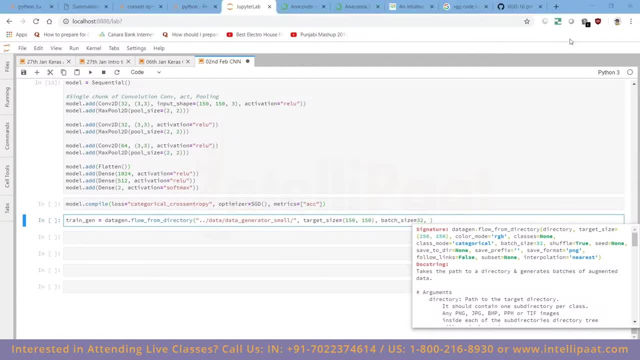 already rgb. then we have: classes is equal to none, we need to keep it. none equal to none, we need to keep it. none equal to none, we need to keep it none. then class mode is categorical. yes, we then. class mode is categorical. yes, we then class mode is categorical- yes, we want it categorical. only we have batch. 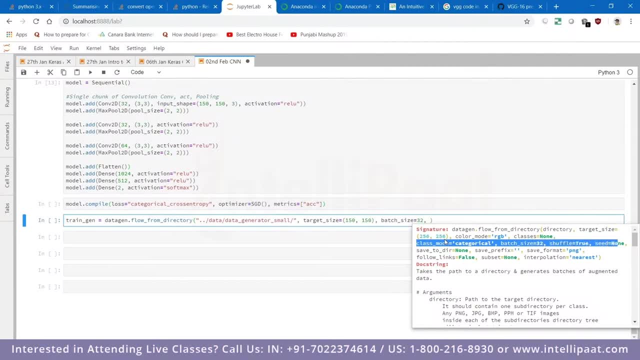 want it categorical: only we have batch. want it categorical: only we have batch size of 32. it's by default, shuffle size of 32. it's by default shuffle size of 32. it's by default: shuffle. equal to true- yes. seed equal to none. we. equal to true- yes. seed equal to none- we. 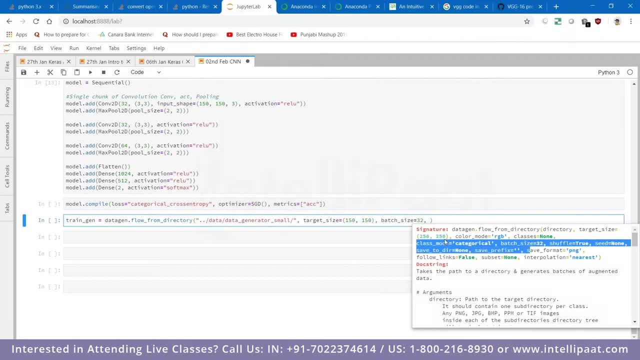 equal to true. yes, seed equal to none. we don't want seeding- we save directory. no, don't want seeding, we save directory. no, don't want seeding, we save directory. no, we don't want to save, we don't want to save, we don't want to save nothing. 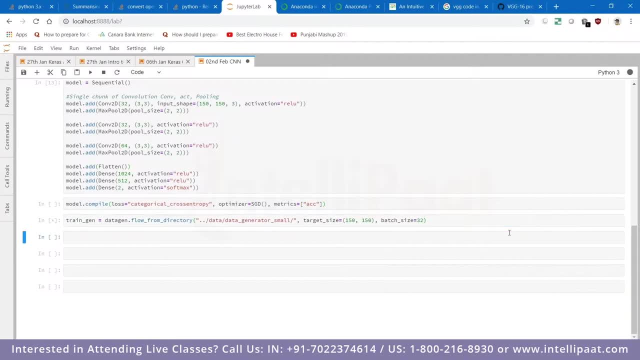 nothing, nothing. we don't want to save, we want to just. we don't want to save, we want to just. we don't want to save, we want to just start the thing it says that it found. start the thing it says that it found. start the thing it says that it found 401 images belonging to two classes and. 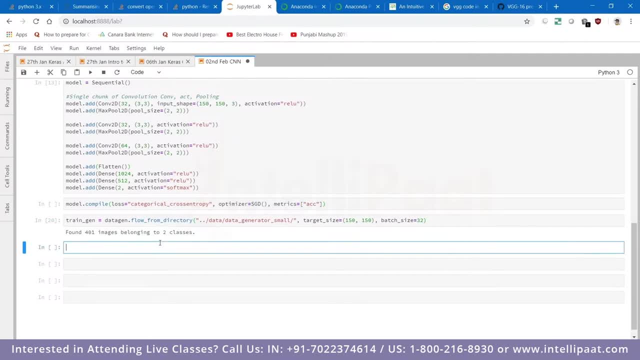 401 images belonging to two classes and 401 images belonging to two classes, and that was correct. we had only two classes. that was correct. we had only two classes. that was correct. we had only two classes. right after we have got our train gen, right after we have got our train gen. 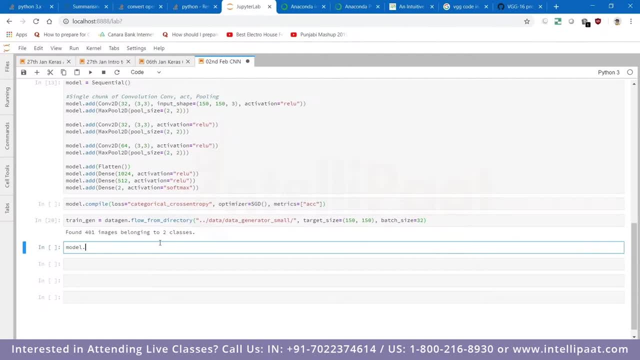 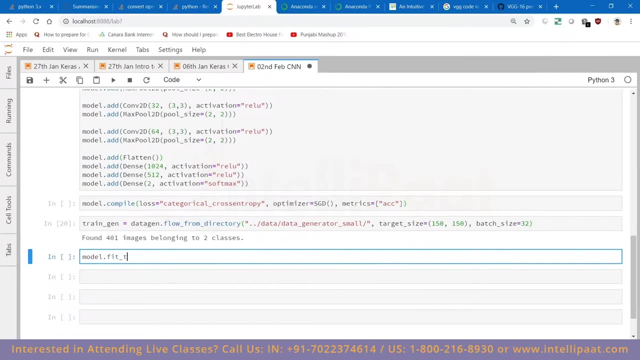 right after we have got our train gen ready. we should use the model dot fit ready. we should use the model dot fit ready. we should use the model dot fit right. so fit will not work here, we will use fit. so fit will not work here, we will use fit. 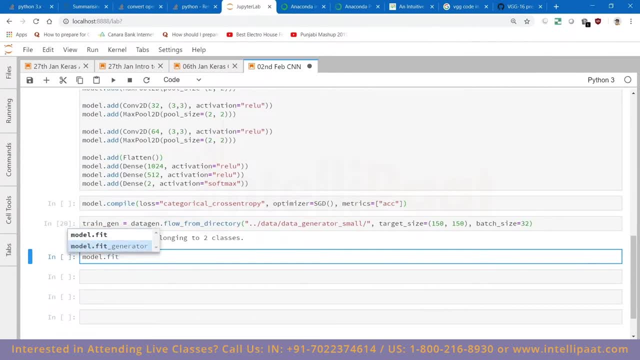 so fit will not work here. we will use fit transform, transform transform model dot model dot, model dot fit generator. sorry, not transform fit generator. sorry, not transform fit generator. sorry, not transform generator. generator generator, modelfit generator. you have to give it. modelfit generator. you have to give it. 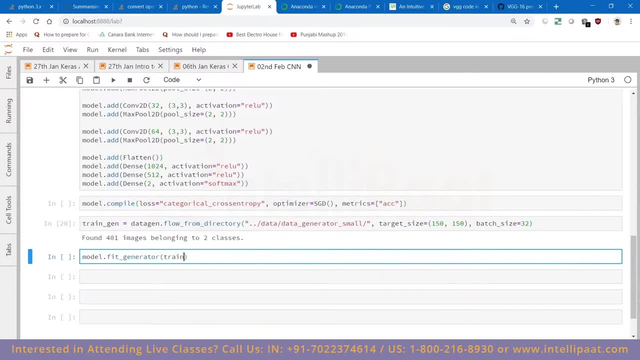 modelfit generator. you have to give it. what a train gen that you have just made. what a train gen that you have just made. what a train gen that you have just made. next, you have a step per epoch, step per. next, you have a step per epoch, step per. 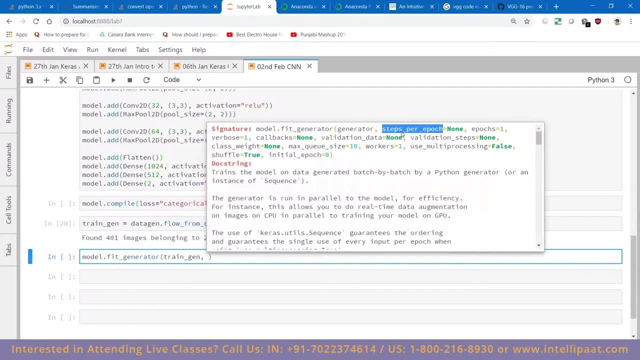 next, you have a step per epoch. step per epoch is none by default, but this is epoch is none by default, but this is epoch is none by default, but this is what you think right. steps per epoch is what you think right. steps per epoch is what you think right. steps per epoch: is what that? how many buckets will come? what that? how many buckets will come what that? how many buckets will come here. so you get the idea right. what was here? so you get the idea right. what was here? so you get the idea right. what was the number that we just calculated? that, the number that we just calculated that. 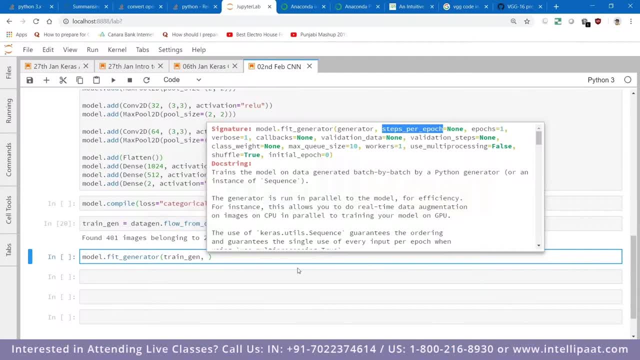 the number that we just calculated. that was 13.. i'll tell you again how it came was 13.. i'll tell you again how it came was 13.. i'll tell you again how it came 13.. so you have 401 images in total. 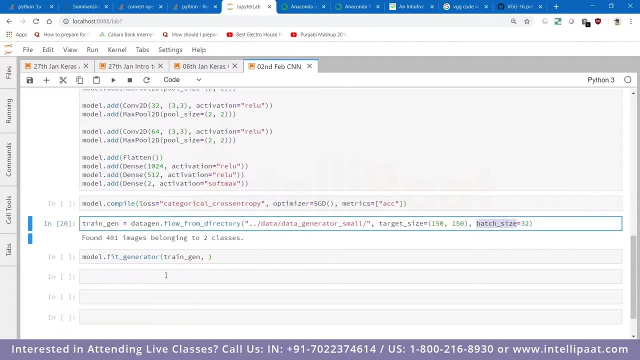 13. so you have 401 images in total- 13. so you have 401 images in total. right, and you are saying that you will right, and you are saying that you will right, and you are saying that you will have a batch size of 32. 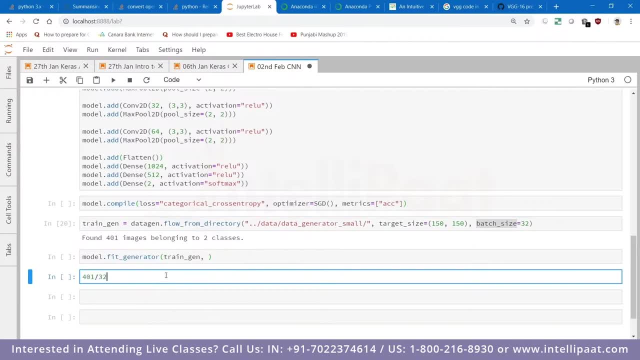 have a batch size of 32, have a batch size of 32. batch size of 32 means that in each bucket, batch size of 32 means that in each bucket, batch size of 32 means that in each bucket you will have 32 images. you will have 32 images. 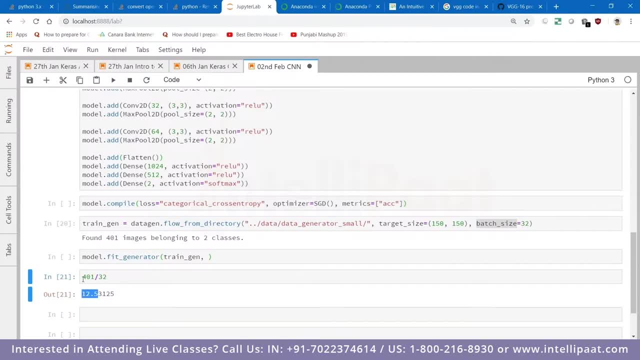 you will have 32 images. then how many buckets will you have? 12.53? then how many buckets will you have 12.53? then how many buckets will you have? 12.53? now, bucket can be an integer only. so now bucket can be an integer only so. 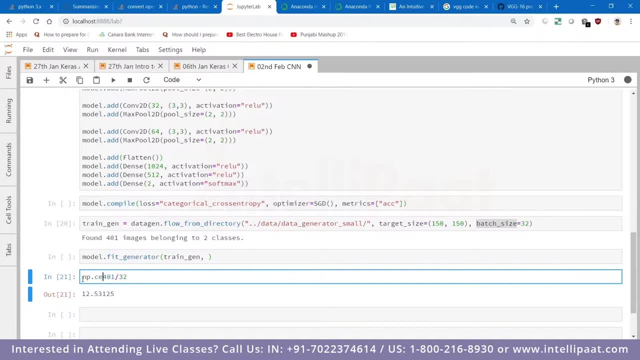 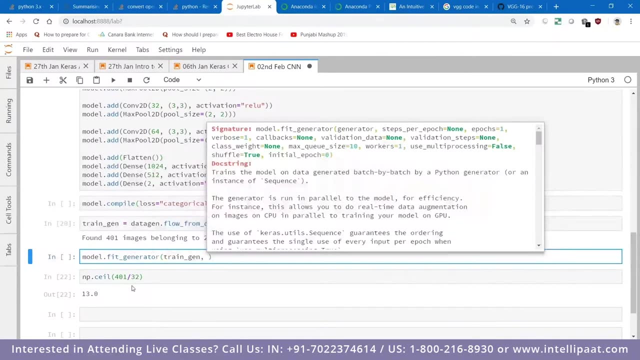 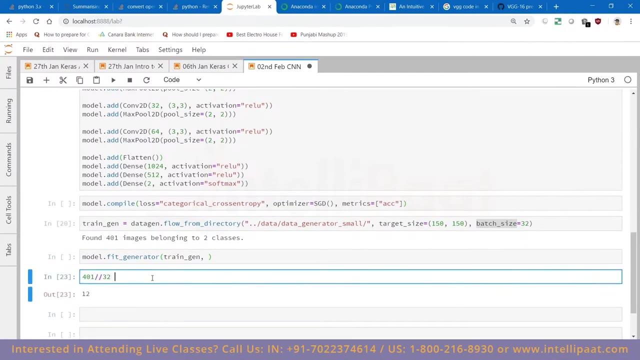 now, bucket can be an integer only. so what you will do is you will do np dot. what you will do is you will do np dot. what you will do is you will do np dot ceiling, ceiling, ceiling, plus one that gives you the idea right, plus one that gives you the idea right. 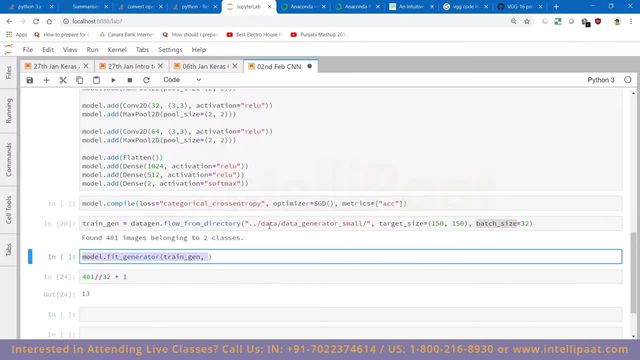 plus one that gives you the idea right. so what we are going to do is we can. so what we are going to do is we can. so what we are going to do is we can write here that steps per epoch will be. write here that steps per epoch will be. 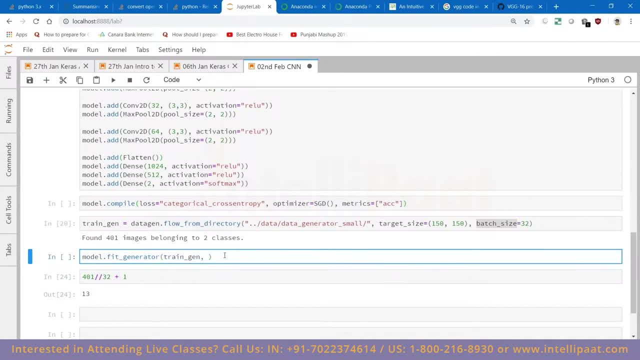 write here that steps per epoch will be, so one epoch is what when all your so one epoch? is what when all your so one epoch is what when all your images are gone from the model forward images are gone from the model forward images are gone from the model forward and backward once. 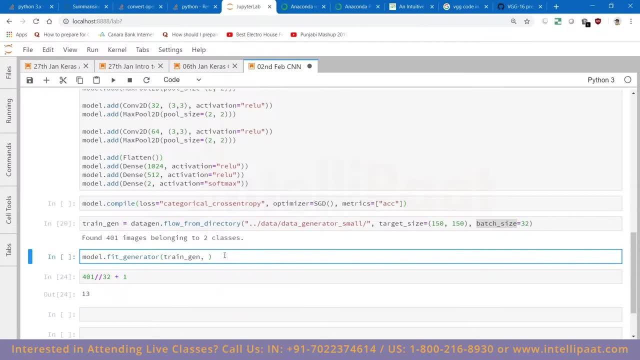 and backward, once and backward once. that is one epoch. now you have 400. that is one epoch. now you have 400. that is one epoch. now you have 400 images, images, images. you are only taking 32 once at a time. you are only taking 32 once at a time. 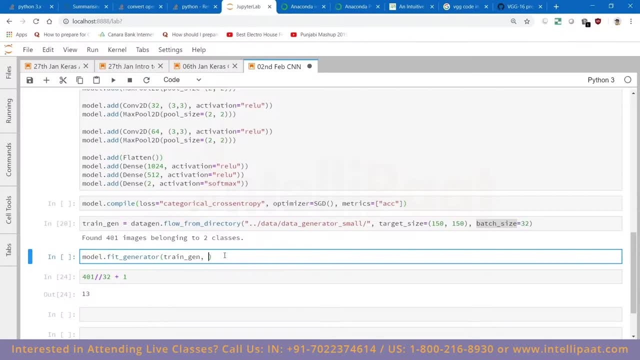 you are only taking 32 once at a time, so your model will be your model will, so your model will be your model will, so your model will be your model will be taking 13 times each bucket of 32. be taking 13 times each bucket of 32. 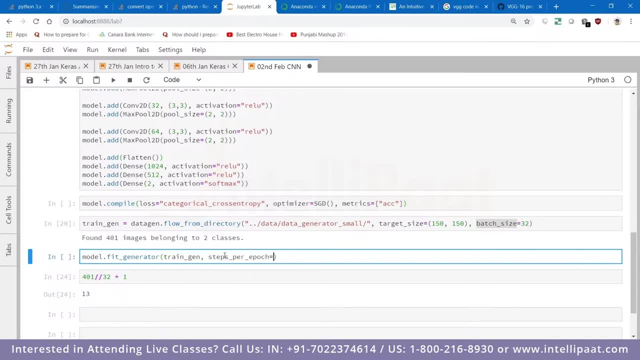 be taking 13 times each bucket of 32 images, images, images, and then it will cover 400. so your steps, and then it will cover 400, so your steps, and then it will cover 400, so your steps. per epoch will be what. per epoch will be what. 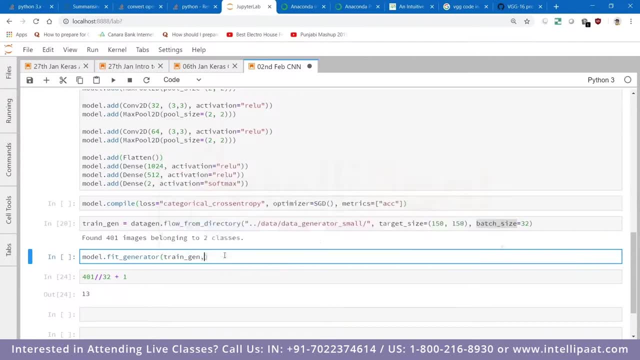 per epoch will be what? 32? then you have epochs. let's say 10 epochs, then you have epochs. let's say 10 epochs, then you have epochs. let's say 10 epochs. only right now, only right now, only right now. i had- i don't have much as i am in this- 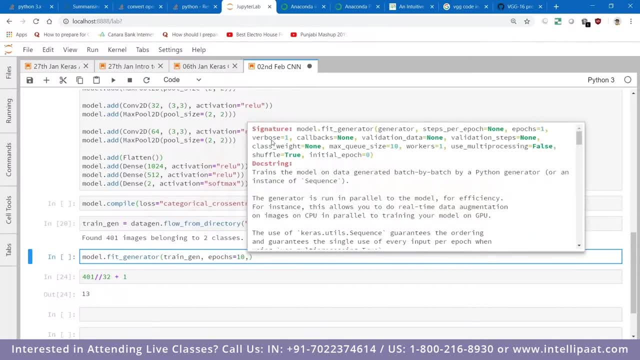 i had. i don't have much as i am in this. i had. i don't have much as i am in this, but okay, and then you can say verbose, but okay, and then you can say verbose, but okay, and then you can say verbose equal to one. one was equal to one means. 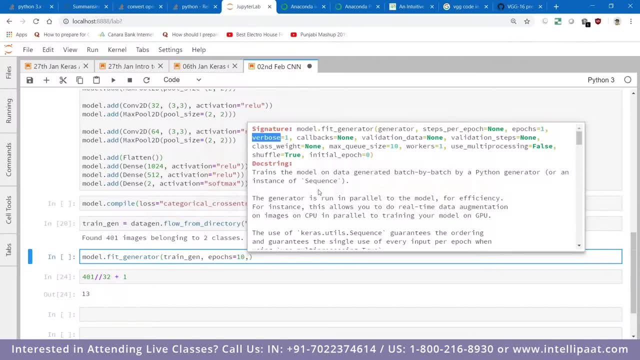 equal to one. one was equal to one means equal to one. one was equal to one means that you want the output to be printed, that you want the output to be printed, that you want the output to be printed. yes, we want. you can have zero or one. 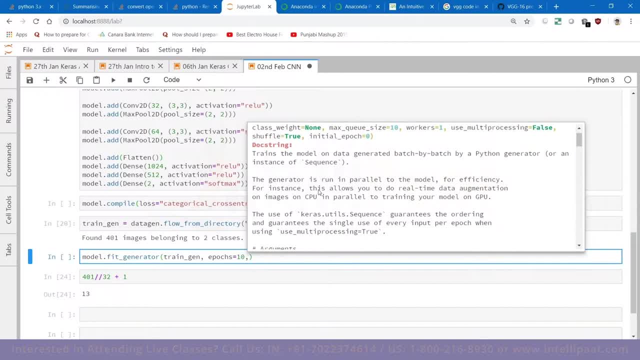 yes, we want you can have zero or one. yes, we want you can have zero or one, dependingly, and i have they. they have dependingly and i have they. they have dependingly and i have they. they have two also, if i remember, yes, verbose is two also, if i remember, yes, verbose is. 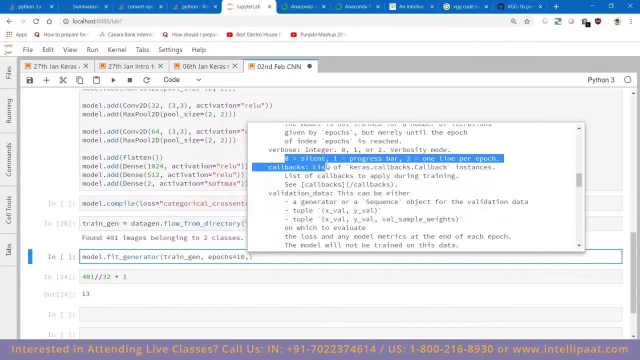 two. also, if i remember, yes, verbose is equal to zero. one two zero is like equal to zero. one two zero is like equal to zero. one two zero is like totally silent. you don't want anything. totally silent, you don't want anything. totally silent, you don't want anything. one is with the progress bar and two is 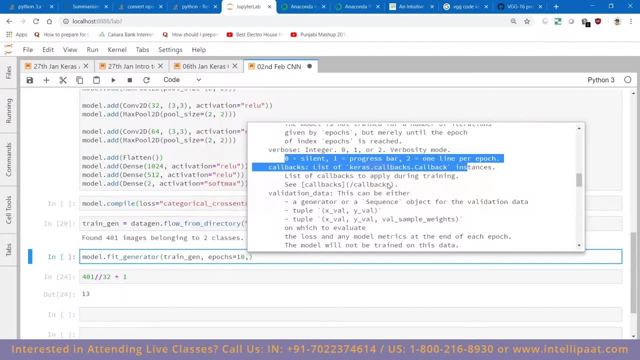 one is with the progress bar and two is: one is with the progress bar and two is with the one line each per, with the one line each per, with the one line each per. one line per epoch. one line per epoch, one line per epoch, right, okay, then you have these things. 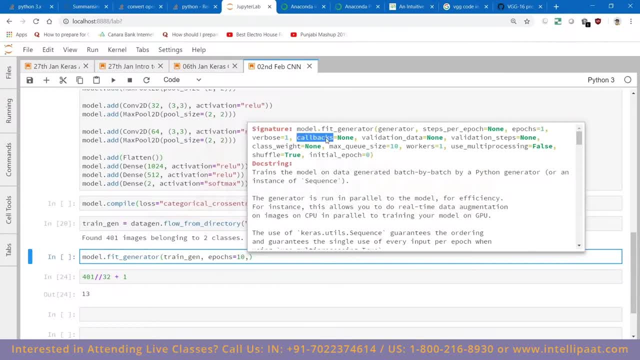 right. okay, then you have these things right. okay, then you have these things called uh, called uh, called uh, this class callbacks this class callbacks. this class callbacks right. how, when you are running a very right, how, when you are running a very right, how, when you are running a very large model, how do you see the losses? 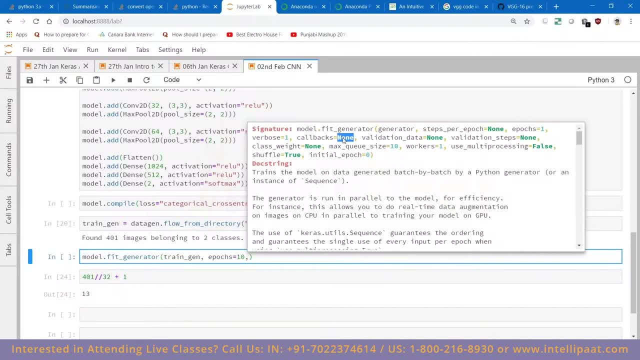 large model. how do you see the losses large model. how do you see the losses and the and the and the accuracy of this right? similarly, you can accuracy of this right. similarly, you can accuracy of this right. similarly, you can have validation data if you have. have validation data if you have. 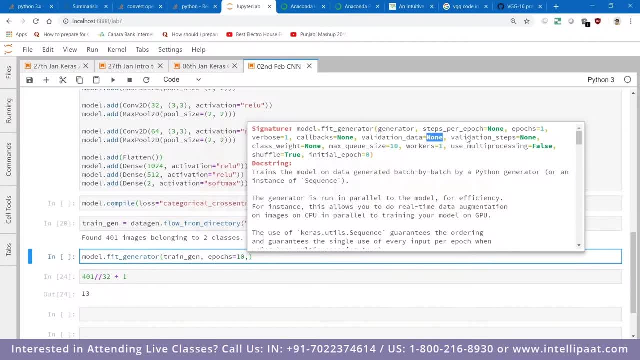 have validation data. if you have validation data, you give your validation validation data. you give your validation validation data. you give your validation data where it is data, where it is data, where it is right validation steps: how many steps do right validation steps? how many steps do right validation steps? how many steps do you want? and then you can further give. 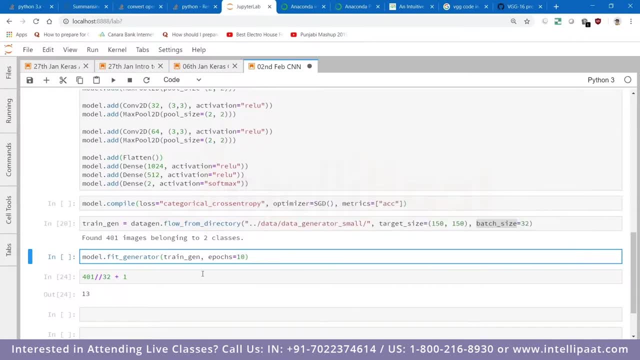 you want and then you can further give you want and then you can further give this thing, this thing, this thing. we don't have much, we will say we will. we don't have much, we will say we will. we don't have much, we will say we will remove this thing. 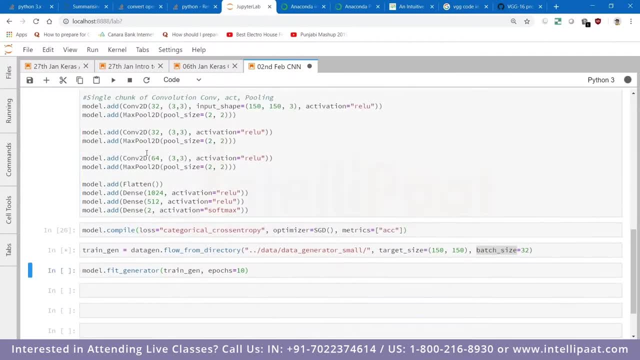 remove this thing, remove this thing. we will run this again, again, again, and we will run this again, again, again, and we will run this again, again, again. and our model is started and my cpu, our model, is started and my cpu- our model is started and my cpu has started heating up. 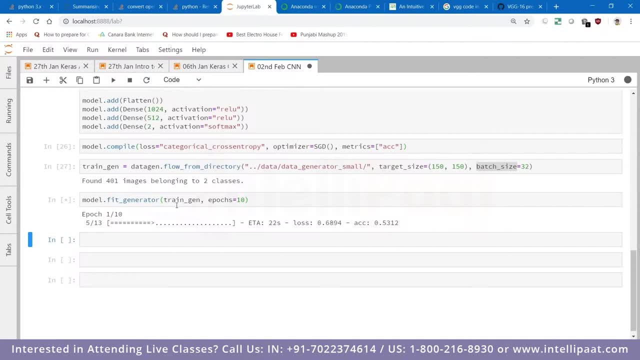 has started heating up, has started heating up. okay, let me stop it here. okay, let me stop it here. okay, let me stop it here. i forgot to do one thing here that you i forgot to do one thing here that you i forgot to do one thing here that you have to. 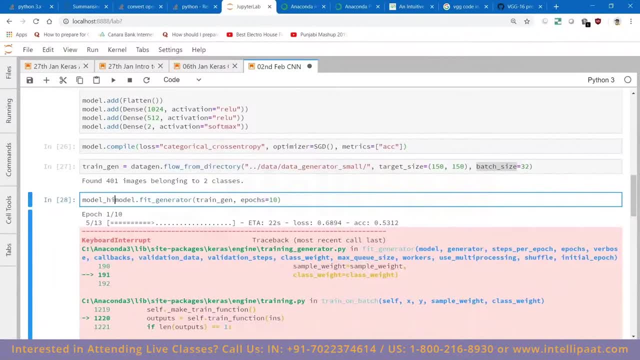 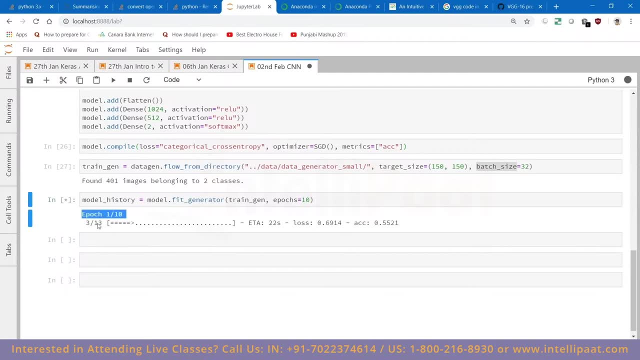 have to have to take this thing in. some take this thing in, some take this thing in some. output, output, output history, history, history. now we will start this. see, i told you, now we will start this. see, i told you, now we will start this. see, i told you, this number is going to be 13, right, 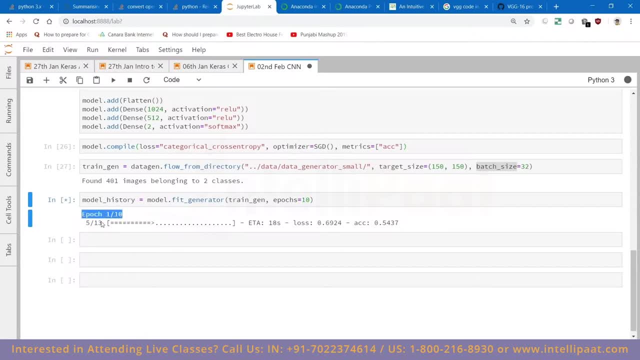 so we are saying that we want 10 epochs. so we are saying that we want 10 epochs, so we are saying that we want 10 epochs, that is a different story, but in each that is a different story. but in each that is a different story. but in each epoch, how many times it is going to run? 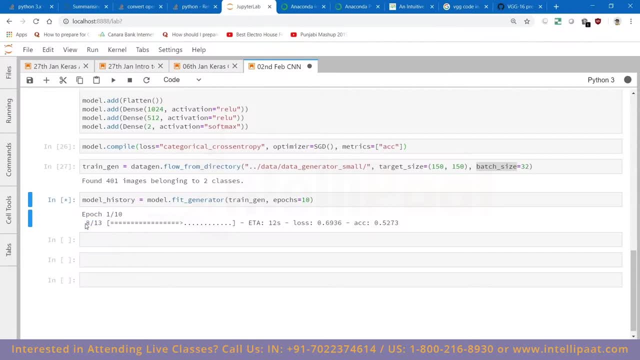 epoch. how many times it is going to run epoch? how many times it is going to run? 13 times, 13 times forward, backward, 13 times. 13 times forward, backward, 13 times, 13 times forward, backward, forward, backward, forward, backward. 13 times forward, backward, forward, backward, forward, backward, 13 times. 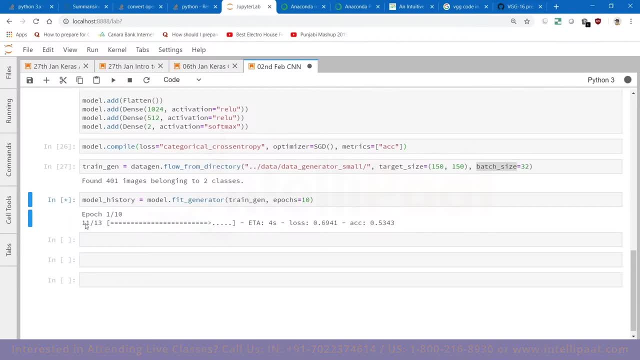 forward, backward, forward backward, forward backward, 13 times and each forward backward is taking how and each forward backward is taking how and each forward backward is taking how many images? many images, many images, 32 images. now you can see your model is giving 54. now you can see your model is giving 54. 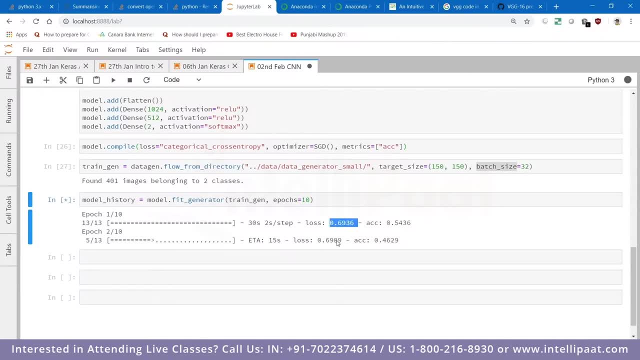 now you can see your model is giving 54 percent accuracy losses are decreasing percent accuracy losses are decreasing percent accuracy losses are decreasing 0.69, 0.69, 0.69, oh, 70 increased, 69, decreasing again. okay, this was a very bad line we had. 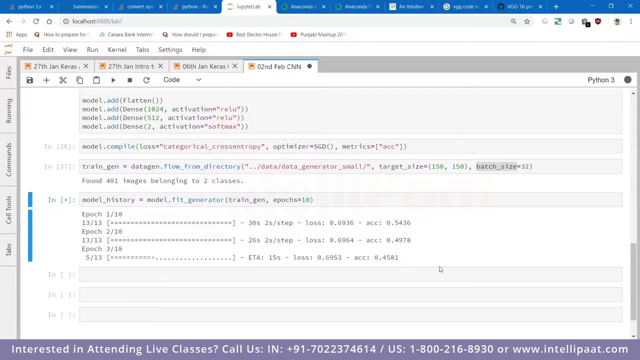 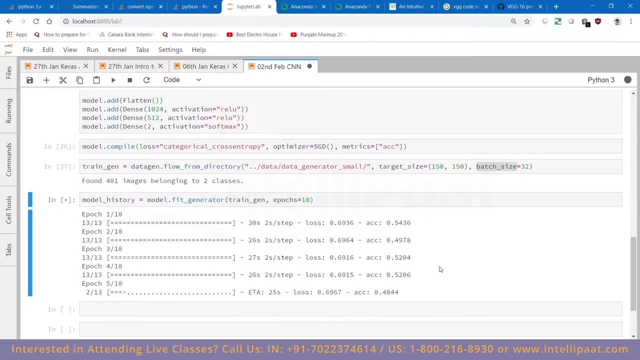 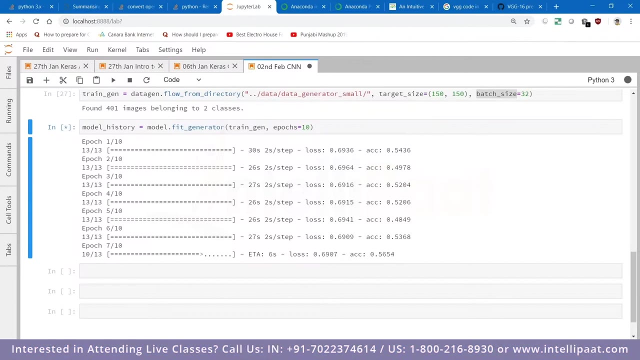 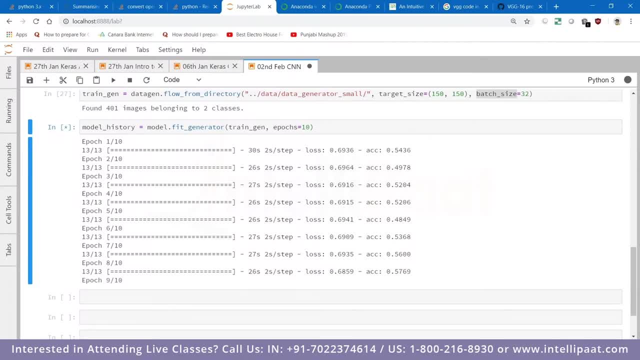 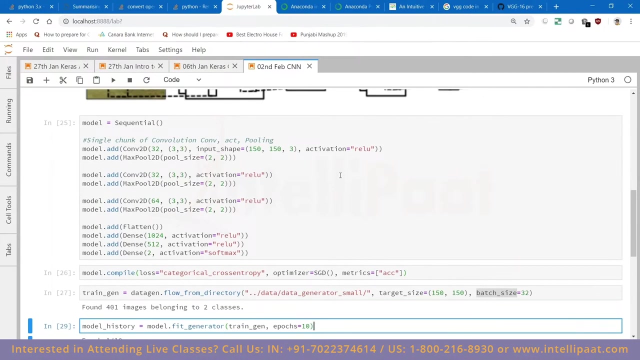 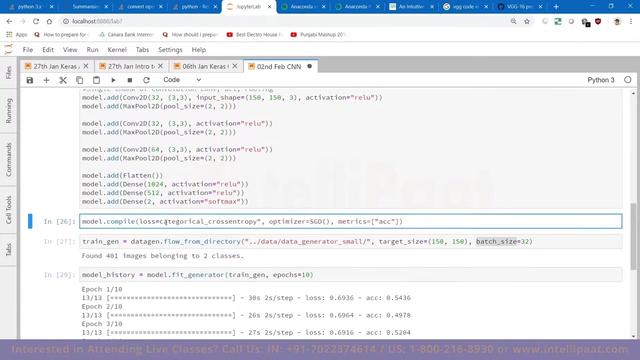 be done, be done, be done. this is how we do. this is how we do. this is how we do. now let me check one thing. because now, let me check one thing. because now let me check one thing, because i think i did something, because this is not what the accuracy i 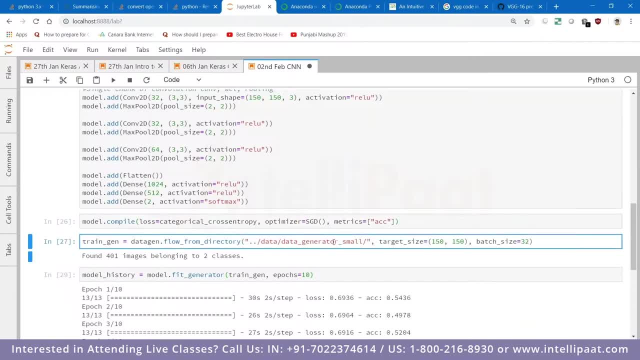 because this is not what the accuracy i- because this is not what the accuracy i was expecting the accuracy should be like. was expecting the accuracy should be like. was expecting the accuracy should be like: okay, so we have a data set also. okay, so we have a data set also. 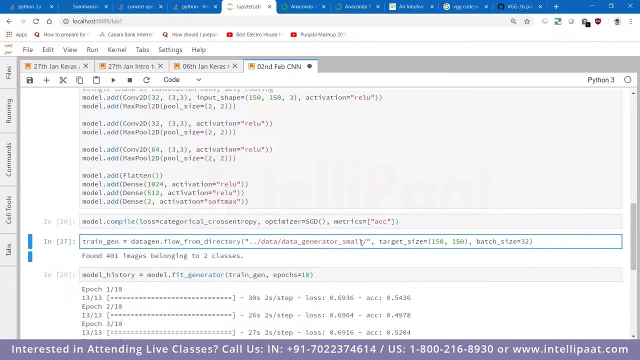 okay, so we have a data set, also small one. if i give it the big one, small one if i give it the big one, small one if i give it the big one. let's try it, let's try it, let's try it, then it should work better. 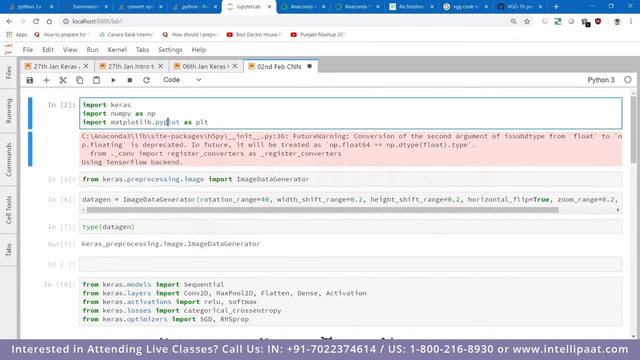 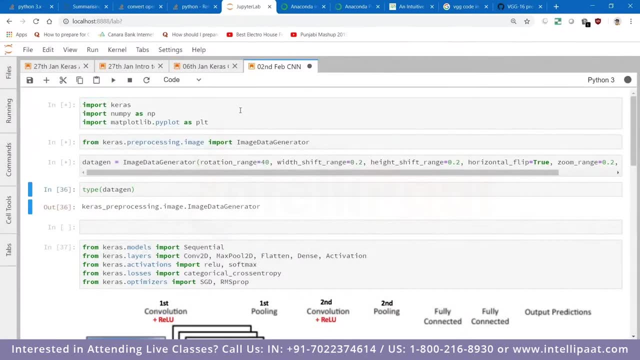 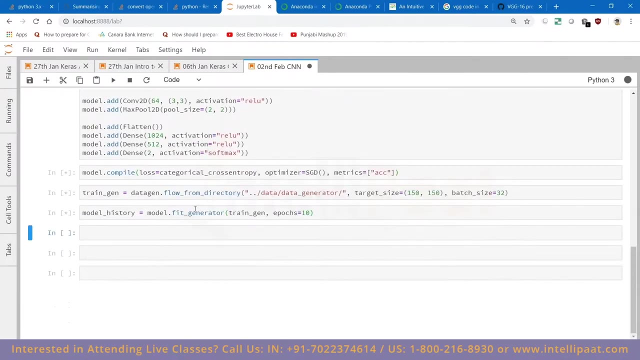 then it should work better. then it should work better. okay, let me run this again. let me run this again. let me run this again. let me restart the one. currently, epochs are also less, so you might try to. epochs are also less, so you might try to. epochs are also less, so you might try to increase the epochs also. 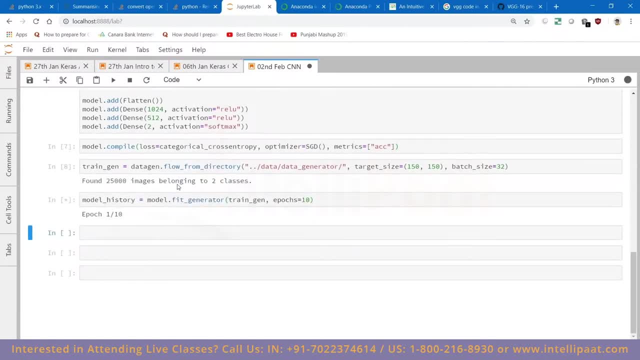 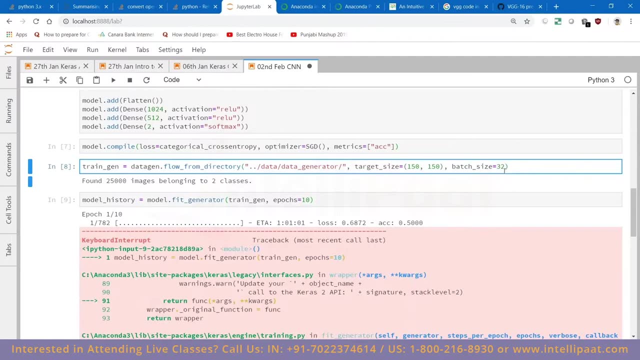 increase the epochs also. increase the epochs also. and i might need to do one more thing. i and i might need to do one more thing. i and i might need to do one more thing: i might need to increase the might need to increase the might need to increase the batch size. 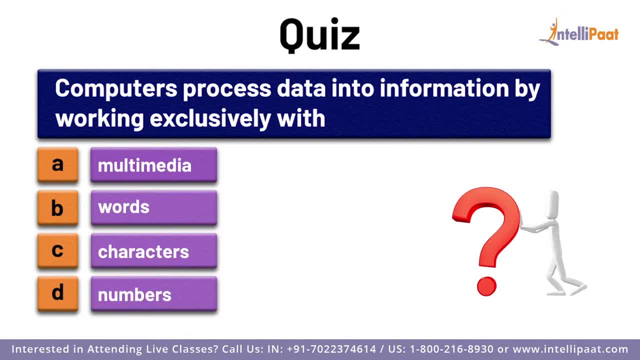 batch size. batch size: just a quick info guys. just a quick info guys. just a quick info guys. test your knowledge of computer vision. test your knowledge of computer vision. test your knowledge of computer vision by answering this question. by answering this question, by answering this question, computers process data into information. 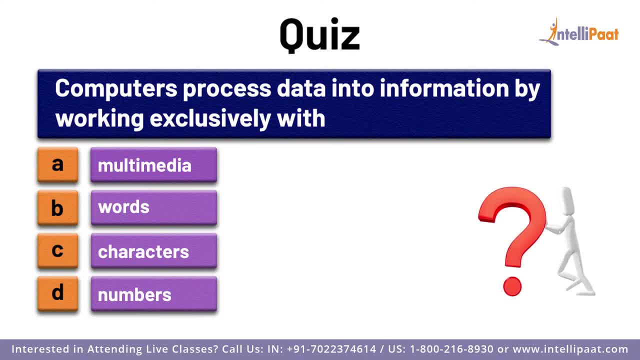 computers process data into information. computers process data into information by working exclusively with which of the by working exclusively with which of the by working exclusively with which of the following following following: a multimedia, a multimedia, a multimedia d words, d words, d words c, c, c, c, characters, d numbers. 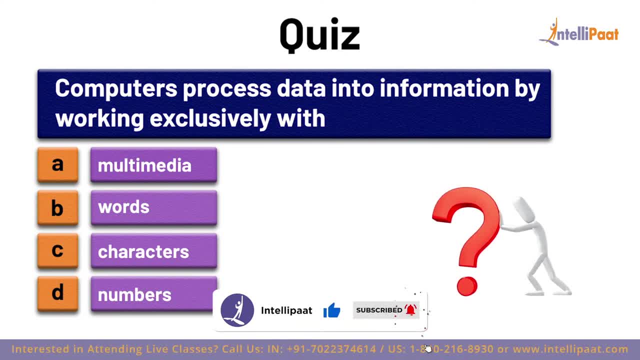 characters d numbers. characters d numbers- comment. your answer in the comment comment. your answer in the comment comment. your answer in the comment section below, section below. section below: subscribe to intellipaat to know the right. subscribe to intellipaat to know the right. subscribe to intellipaat to know the right answer. 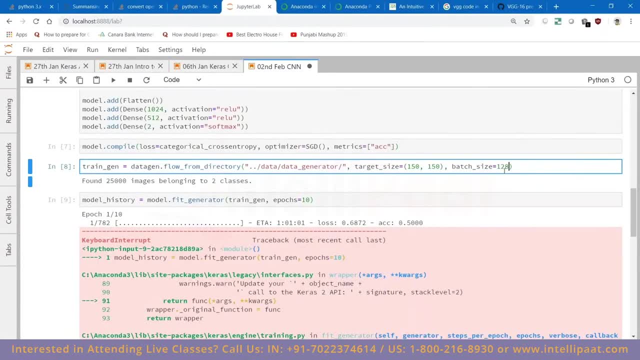 answer. answer. now let's continue with the session. how is now let's continue with the session. how is now let's continue with the session. how is the batch size, the batch size, the batch size, uh effecting the model one. is that okay? it uh effecting the model one, is that okay it? 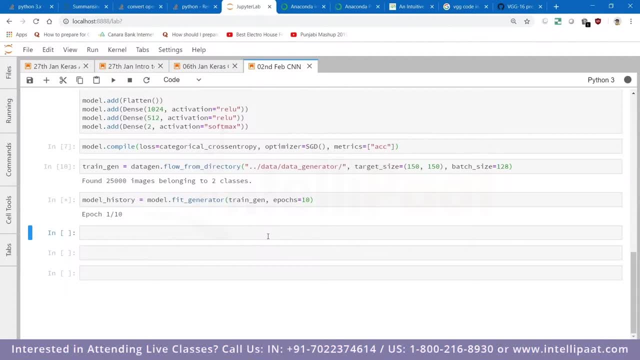 uh, effecting the model. one. is that, okay, it is using the ram, right, because 128 is using the ram. right because 128 is using the ram. right, because 128 images are now going inside the model images are now going inside the model images are now going inside the model. but what else it is doing? 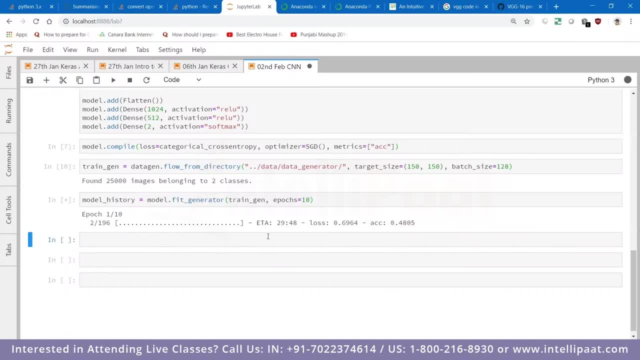 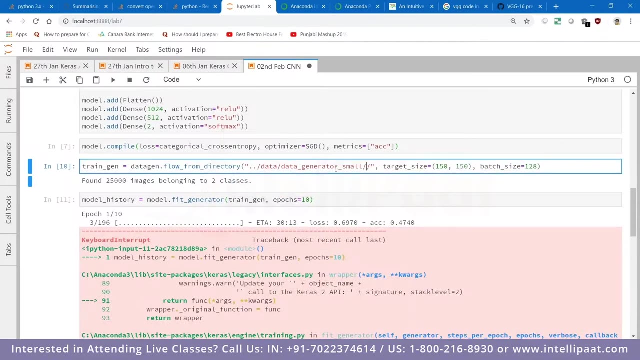 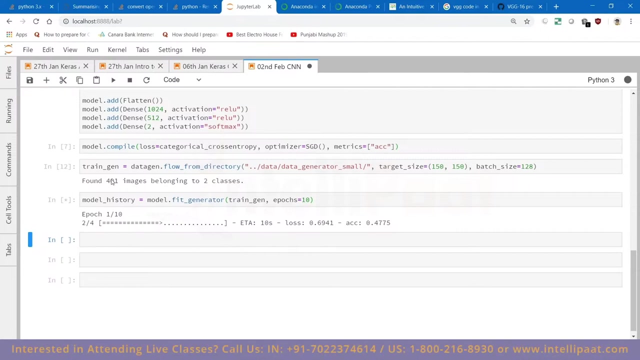 but what else it is doing, but what else it is doing, so. so let's say: i give you this example, so. so let's say: i give you this example, so so let's say: i give you this example. let's say that, let's say that, let's say that there are two animals that are not known. 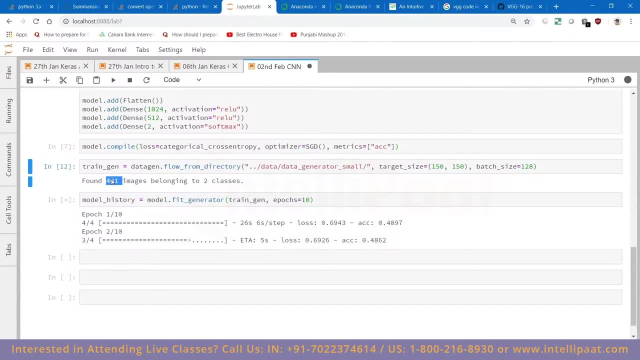 there are two animals that are not known. there are two animals that are not known to you, right to you, right to you, right. i am giving you the images that this one, i am giving you the images that this one, i am giving you the images that this one is, uh. 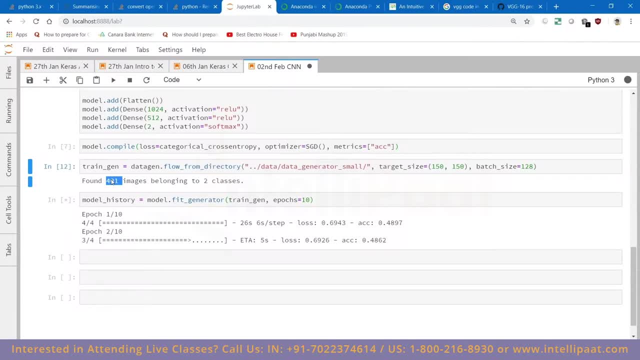 is uh, is uh animal a, and this one is animal b, right animal a, and this one is animal b, right animal a and this one is animal b right now. if i show you only one now, if i show you only one now, if i show you only one image at a time, and then i ask you to, 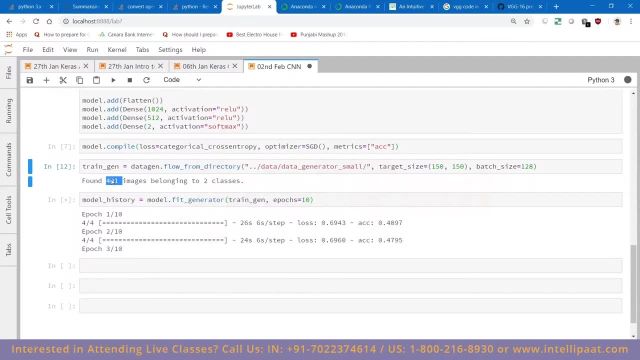 image at a time, and then i ask you to image at a time, and then i ask you to tell me who this thing is. or another, tell me who this thing is. or another, tell me who this thing is. or another case is when i'm giving you 100 images. 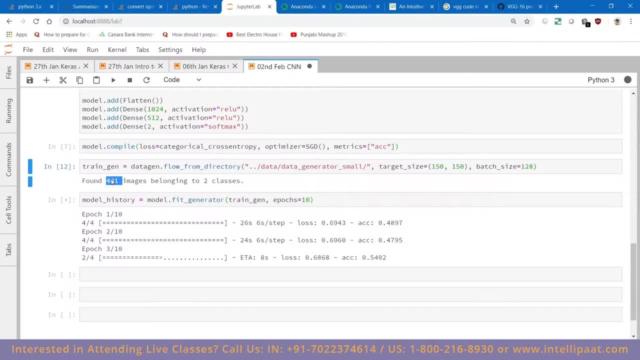 case is when i'm giving you 100 images. case is when i'm giving you 100 images and then i'm saying 50 are the 50 others, and then i'm saying 50 are the 50 others, and then i'm saying 50 are the 50 others, and then you see all those, okay, 50 the. 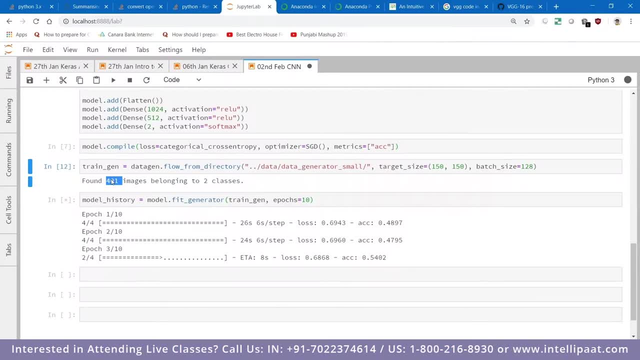 and then you see all those okay, 50 the. and then you see all those okay, 50 the, 50 animal a, 50 animal b, and then in 50 animal a, 50 animal b, and then in 50 animal a, 50 animal b, and then in which state you will be able to give. 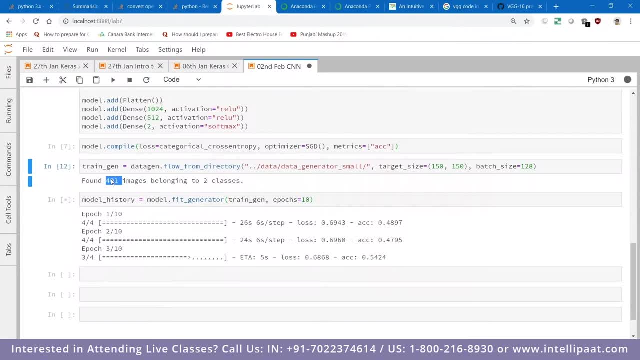 which state you will be able to give, which state you will be able to give when i give you next image in which, when i give you next image in which, when i give you next image, in which state you will be give you can give me, state you will be give you can give me. 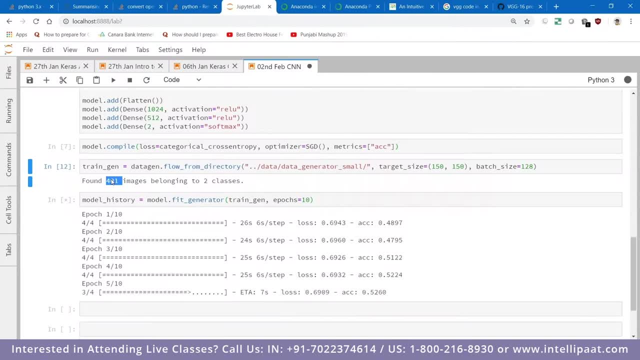 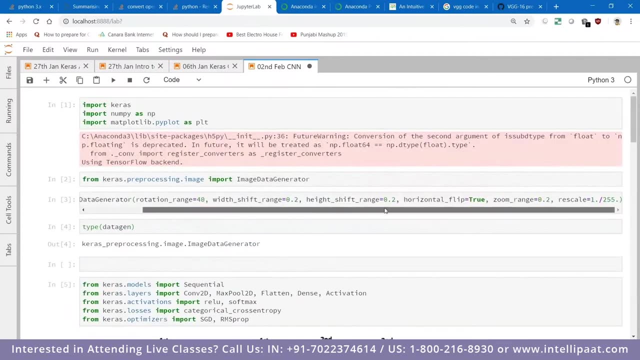 state you will be give you can give me better answer, because i want to show you one more. because i want to show you one more, because i want to show you one more thing here is that we have two classes. thing here is that we have two classes. 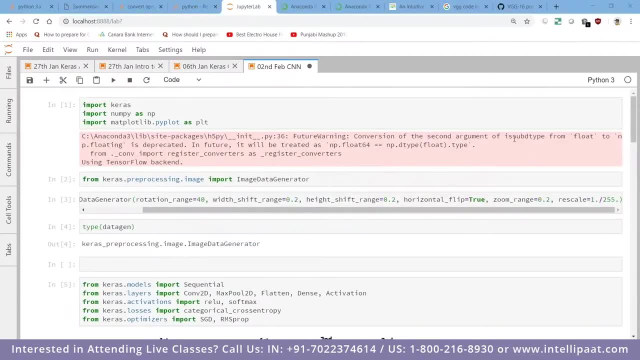 thing here is that we have two classes right now, right, right now, right right. we could have done one more thing. we, we could have done one more thing. we, we could have done one more thing. we could have asked it here that we have. no, not here. we could have come here and 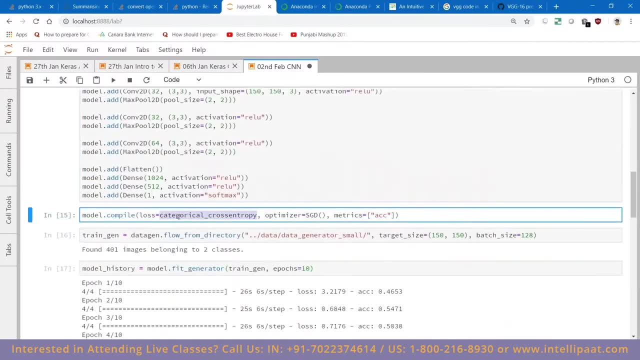 no, not here. we could have come here and no, not here. we could have come here and say that this is only one, say that this is only one, say that this is only one, and rather than saying that this is, and rather than saying that this is, and rather than saying that this is cross entropy, we could have said: 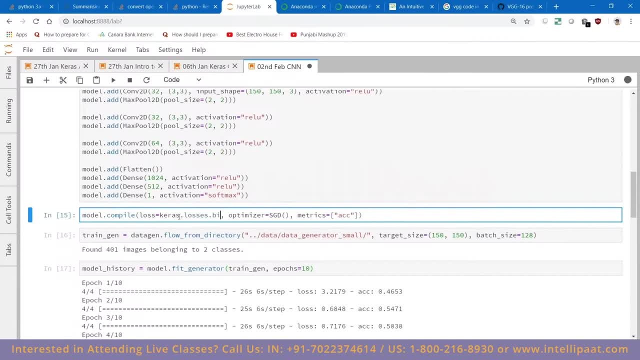 cross entropy. we could have said cross entropy. we could have said: kiraz dot losses dot binary cross. kiraz dot losses dot binary cross. kiraz dot losses dot binary cross. entropy right. how i'm showing you that entropy right, how i'm showing you that entropy right, how i'm showing you that. what is the difference between? 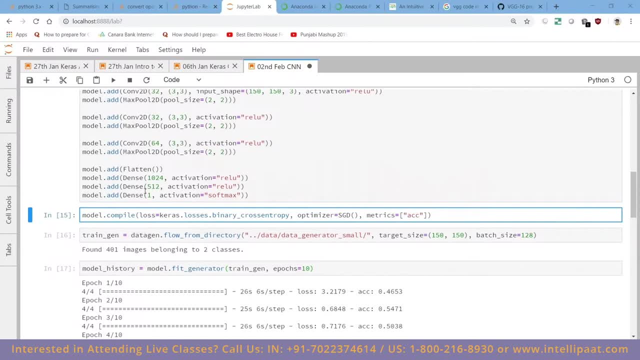 what is the difference between? what is the difference between categorical and binomial? so what i'm categorical and binomial. so what i'm categorical and binomial. so what i'm saying is why i took one. only because saying is why i took one, only because saying is why i took one, only because now my answer will be in zero and one. 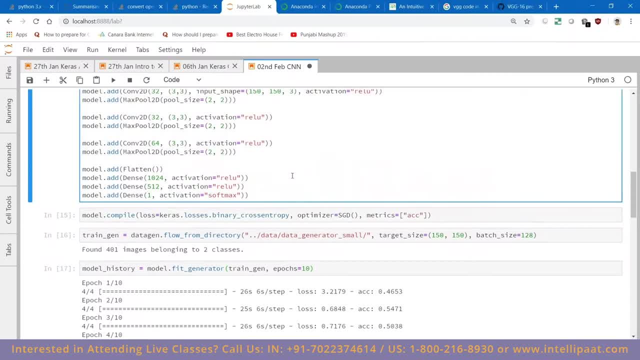 now my answer will be in zero and one. now, my answer will be in zero and one. and why zero and one? because, if it's not. and why zero and one because, if it's not? and why zero and one? because if it's not a cat, it is a dog actually, right. so 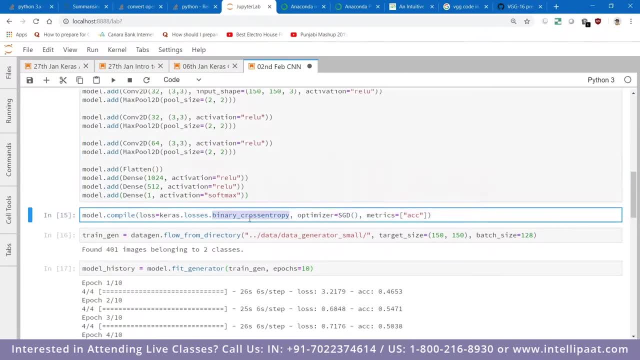 a cat, it is a dog, actually right, so a cat, it is a dog, actually right, so it's actually. it's so how i've converted. it's actually it's so how i've converted. it's actually. it's so how i've converted two problem, two, uh, categorical problem. 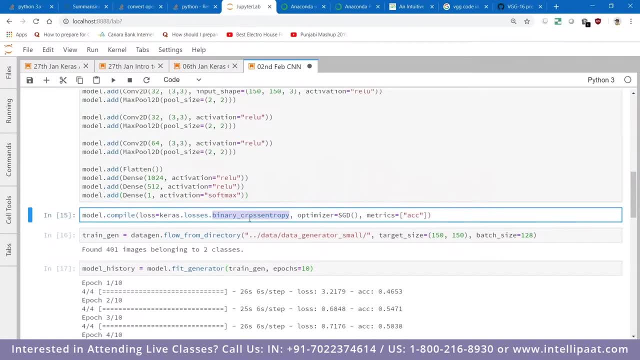 two problem two: uh, categorical problem. two problem two: uh, categorical problem into a binary problem. binary problem is into a binary problem. binary problem is into a binary problem. binary problem is: what zero or one right, what zero or one right, what zero or one right? let's say one is dog, then zero will. 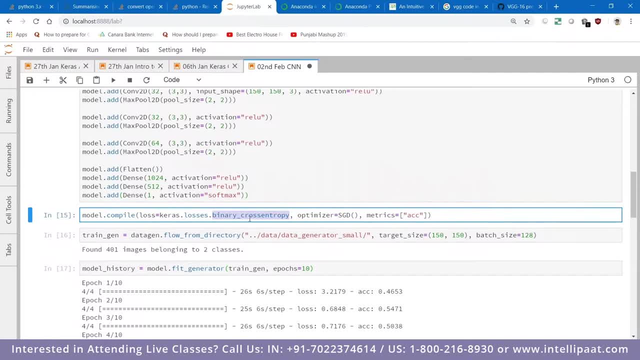 let's say one is dog, then zero will. let's say one is dog, then zero will eventually become, eventually become, eventually become. not dog and not dog. in our case is cat not dog and not dog. in our case is cat not dog and not dog. in our case is cat, and this is one thing that you should. 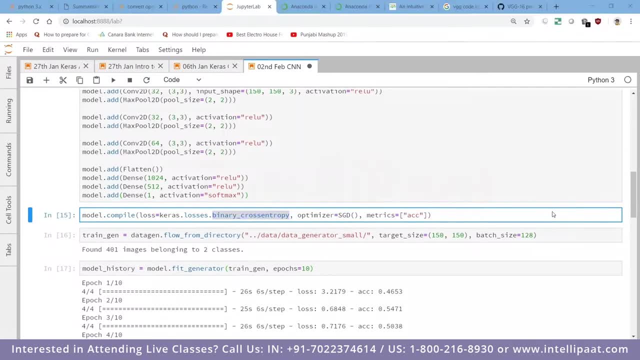 and this is one thing that you should, and this is one thing that you should always understand, always understand, always understand. let's say that, if your model is trying, let's say that. if your model is trying, let's say that, if your model is trying to predict three things: 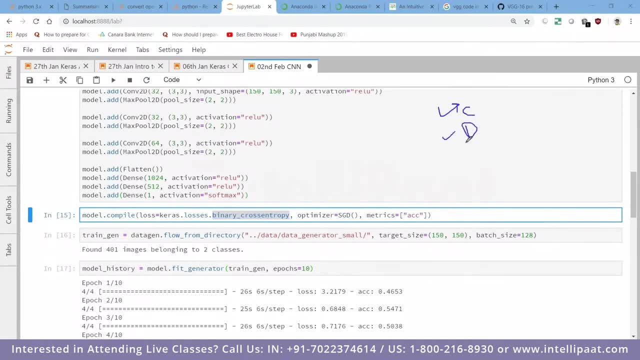 to predict three things. to predict three things: one is cat dog, one is cat dog. one is cat dog, an elephant, let's say, and let's say: you an elephant. let's say, and let's say you an elephant. let's say, and let's say you give a image of. 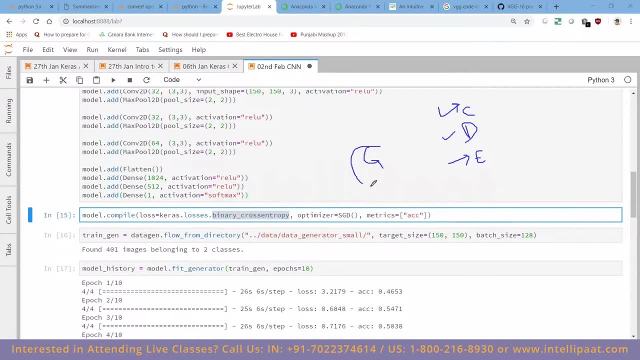 give a image of, give a image of giraffe here. right, you have drained your model on cat dog. you have drained your model on cat dog. you have drained your model on cat dog and and and elephant, and now you're giving it an elephant, and now you're giving it an. 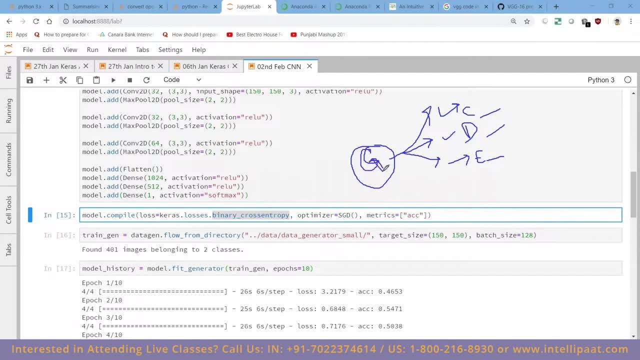 elephant and now you're giving it an image of giraffe. what will it predict? image of giraffe? what will it predict? image of giraffe? what will it predict? zero, zero, zero. okay, one answer is zero, zero, zero. okay, one answer is zero, zero, zero. okay, one answer is zero, zero, zero. 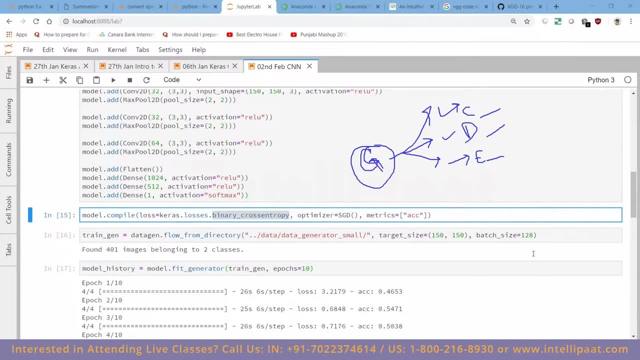 zero, zero, zero, that it will say zero for each zero, zero, zero, that it will say zero for each zero, zero, zero, that it will say zero for each probability, right, probability, right, probability, right. so one thing that you should always so, one thing that you should always so, one thing that you should always remember, is that the sum of the 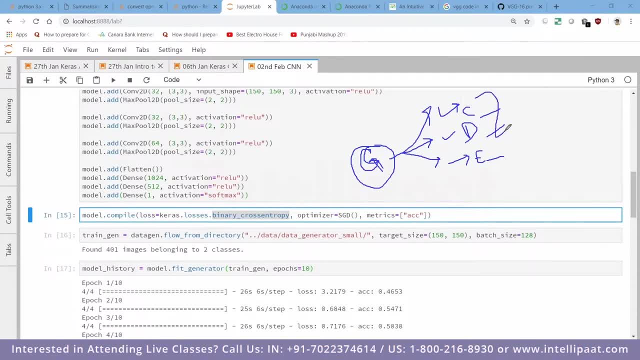 remember is that the sum of the remember is that the sum of the probability for the three glasses will probability for the three glasses, will probability for the three glasses will be equal to be equal, to be equal to one, one one and the softmax. we always use a softmax. 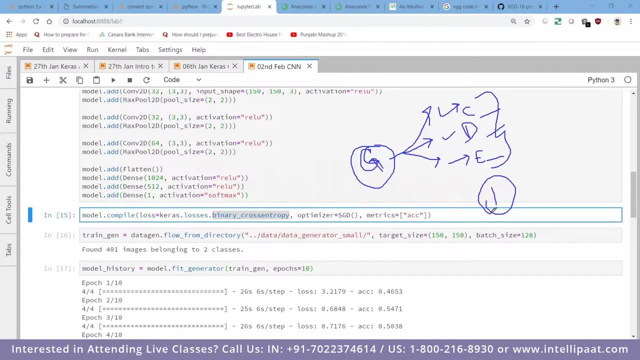 and the softmax. we always use a softmax and the softmax, we always use a softmax in the last layer. and what is the in the last layer and what is the in the last layer? and what is the responsibility of softmax that it will, responsibility of softmax that it will. 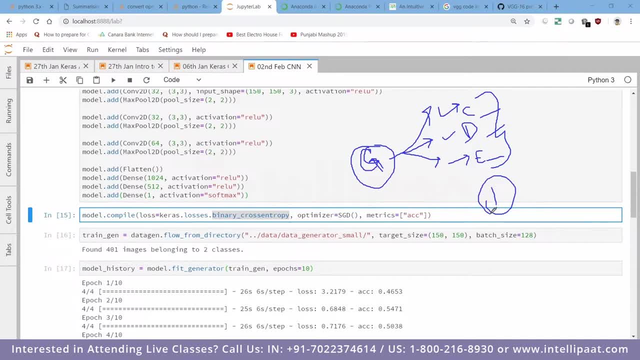 responsibility of softmax, that it will give you the, give you the, give you the. how many probabilities it will give you. how many probabilities it will give you. how many probabilities it will give you the probability that much classes that, the probability that much classes that, the probability that much classes that you have. so, if you have three classes, it. 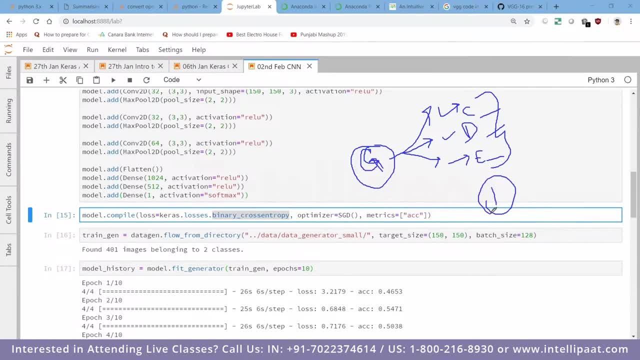 you have. so if you have three classes, it you have. so if you have three classes, it will give you three probabilities and the will give you three probabilities and the will give you three probabilities and the sum of all the probabilities will be. sum of all the probabilities will be: 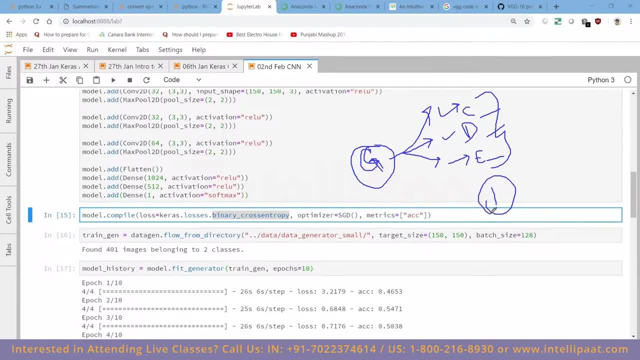 sum of all the probabilities, will be trained on this and the elephant is not trained on this. and the elephant is not trained on this. and the elephant is not matching. it's not matching even to your matching. it's not matching even to your matching. it's not matching even to your dog, not cat. 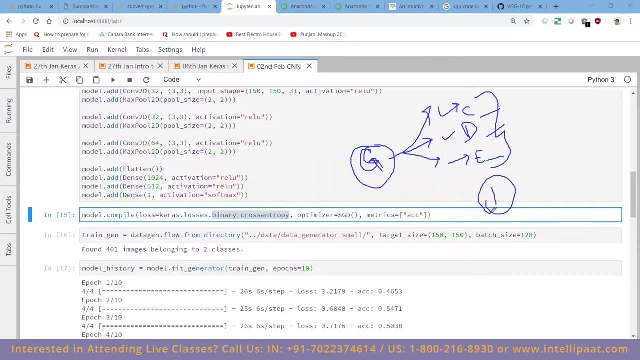 dog, not cat. dog not cat, but softmax. what it will try to do, even but softmax. what it will try to do even but softmax. what it will try to do, even if it is giving very less accuracy, for if it is giving very less accuracy, for if it is giving very less accuracy for each, it will. 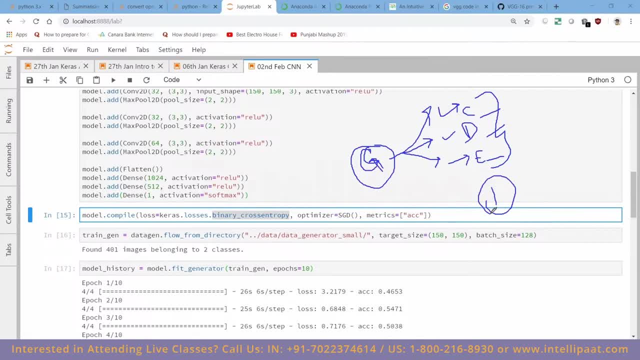 each, it will each, it will, based on the percentile it will give, based on the percentile. it will give, based on the percentile. it will give you the probability which will sum up to you the probability which will sum up to you the probability which will sum up to one that it might not give high probability. 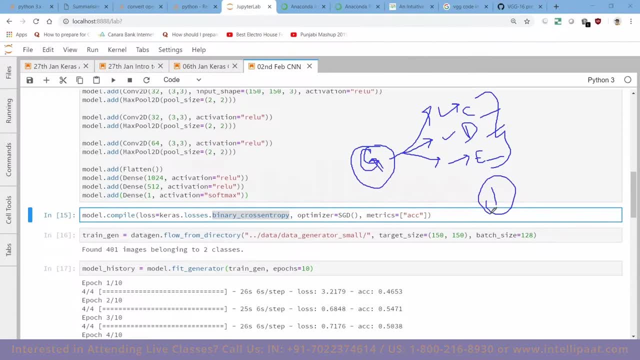 you the probability, which will sum up to one that it might not give high probability for cat and dog, but it might give some for cat and dog, but it might give some for cat and dog, but it might give some probability for elephant and probability for elephant, and 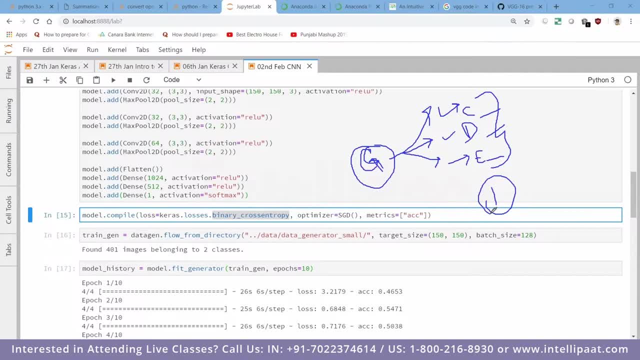 probability for elephant and dog also, and it might not cross 60 or dog also. and it might not cross 60 or dog also. and it might not cross 60 or above for any one of the category, so it above for any one of the category, so it. 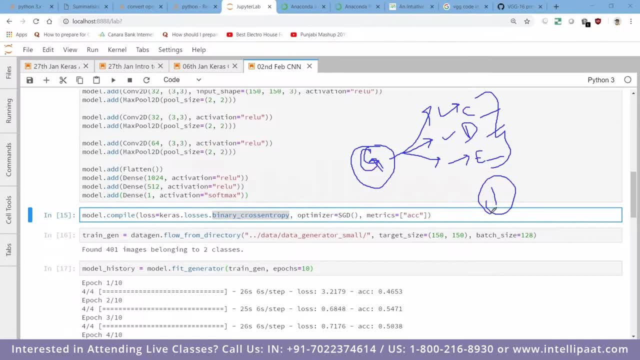 above for any one of the category. so it might be like 30, might be like 30, might be like 30, 20 for cat, 20 for cat, 20 for cat, 30 for 30 for 30 for dog and 34 elephant. i mean, i mean the. 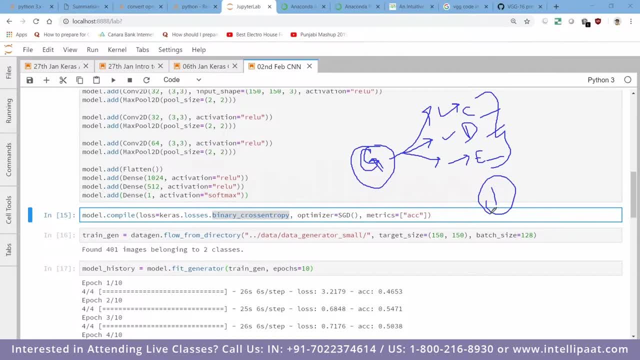 dog and 34 elephant. i mean, i mean the dog and 34 elephant. i mean i mean the sum will be one. it will try to do somewhat. sum will be one. it will try to do somewhat. sum will be one. it will try to do somewhat, like this. so always remember your model. 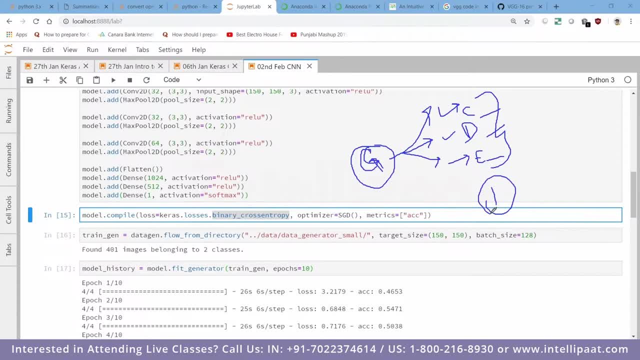 like this. so always remember your model. like this, so always remember your model: will never, will, never, will never, will always predict from only what you are, will always predict from only what you are, will always predict, from only what you are trying to tell it. trying to tell it. 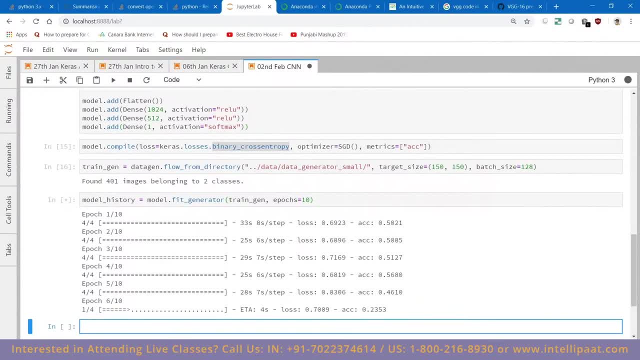 trying to tell it right and i will like to start with right and i will like to start with right and i will like to start with callbacks, because i have this sheet callbacks, because i have this sheet callbacks, because i have this sheet one six jan, where we did this history. 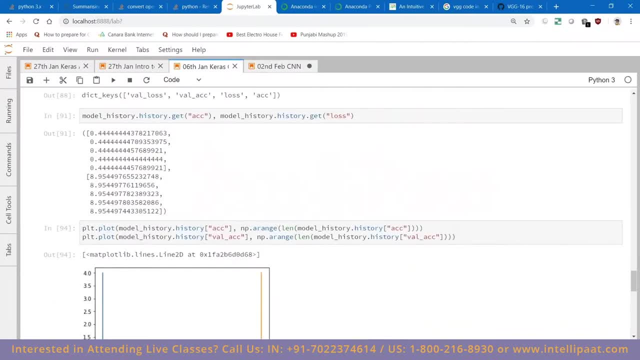 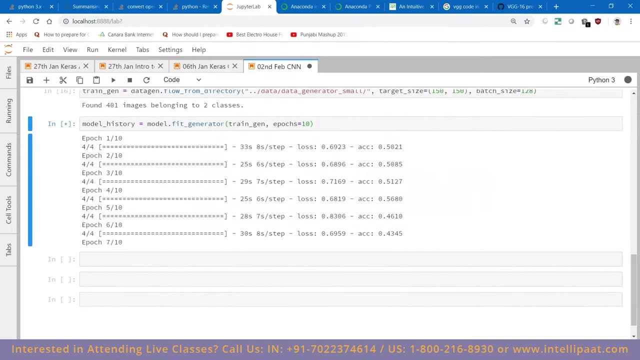 one six jan where we did this history, one six jan where we did this history thing out there thing, out there thing, out there history thing. we did all this plotting history thing, we did all this plotting history thing. we did all this plotting and all and all and all. so i think we should go with callbacks. 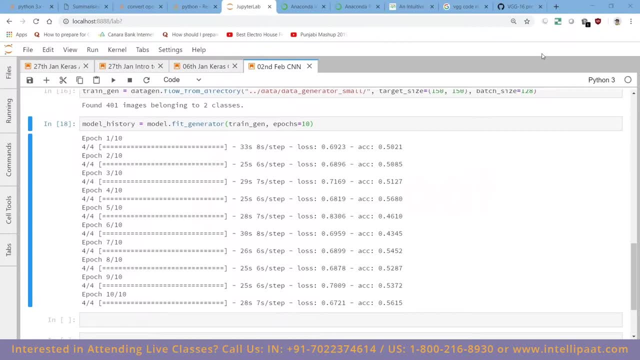 so i think we should go with callbacks. so i think we should go with callbacks. okay, so callback is actually a function. okay, so callback is actually a function. okay, so callback is actually a function that you can execute after every epoch, that you can execute after every epoch. 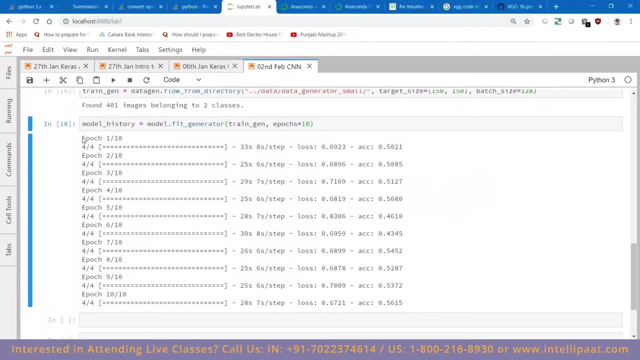 that you can execute after every epoch is run, is run, is run. so let's say that your line is somewhat so, let's say that your line is somewhat so, let's say that your line is somewhat. here, here, here, epoch, here, and then you come here, your 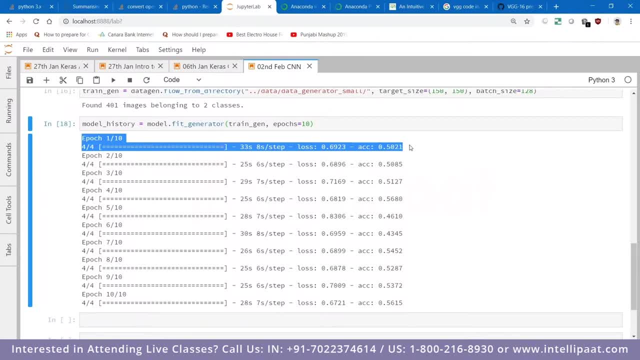 epoch here, and then you come here, your epoch here, and then you come here. your accuracy- final accuracy is printed- accuracy- final accuracy is printed. accuracy, final accuracy is printed. your validation accuracy is printed and your validation accuracy is printed and your validation accuracy is printed. and then, whatever you want to do, you can do. 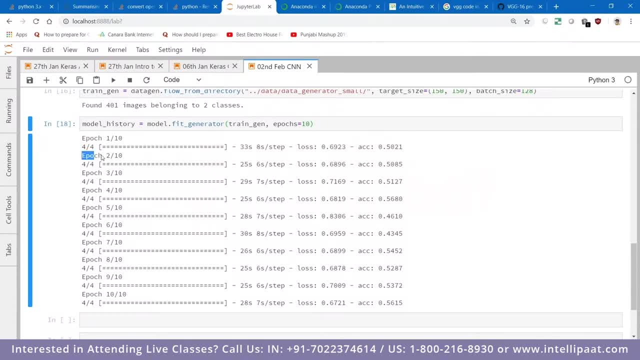 then whatever you want to do, you can do at this stage is called a callback at this stage is called a callback at this stage is called a callback again. this will be executed when your again. this will be executed when your again. this will be executed when your second epoch is completed, with all the 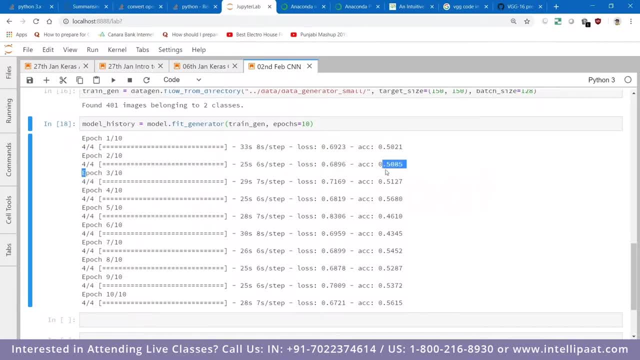 second epoch is completed with all. the second epoch is completed with all the four batches. four batches, four batches, then again at the third end after this, then again at the third end after this, then again at the third end after this, and similarly after each iteration of an. 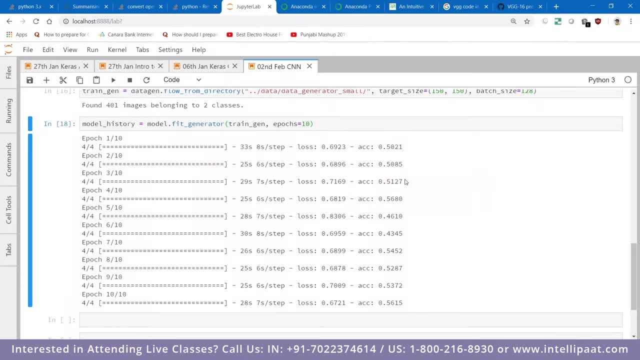 and similarly after each iteration of an, and similarly after each iteration of an epoch. if you want to run something epoch, if you want to run something epoch. if you want to run something, you get this thing inside your insider. you get this thing inside your insider. you get this thing inside your insider: callbacks. now, how do you get callbacks? 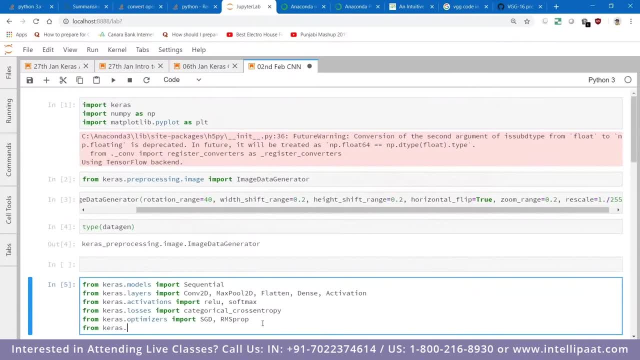 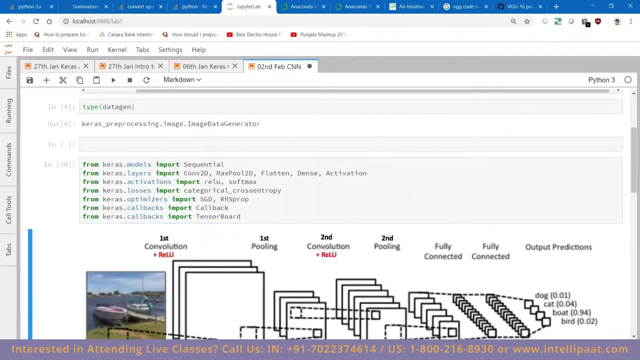 callbacks. now, how do you get callbacks? very easy, you just say from giras dot. very easy, you just say from giras dot. very easy, you just say: from giras dot. callbacks, callbacks, callbacks, import callback see import callback, see. import callback, see. callbacks is nothing but callback is. 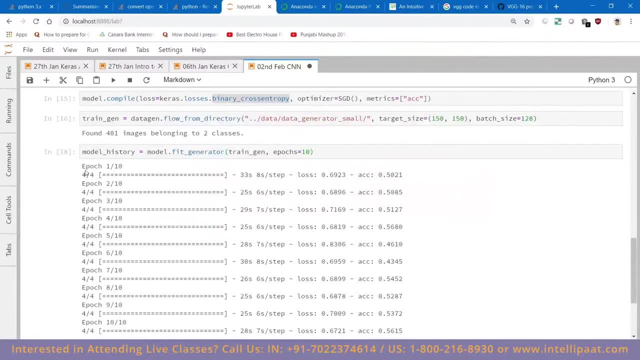 callbacks is nothing, but callback is. callbacks is nothing, but callback is that let's say that after every epoch, that let's say that after every epoch, that let's say that after every epoch, once a epoch is run, and if you want to, once a epoch is run, and if you want to, 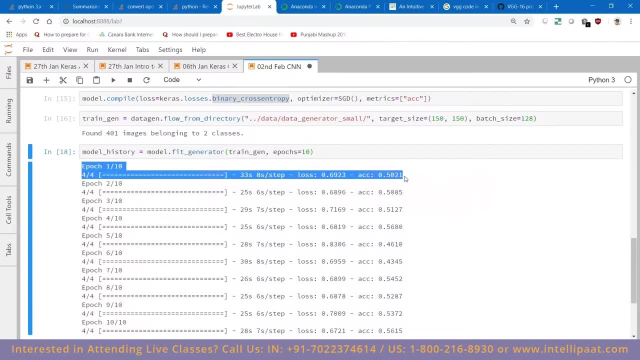 once a epoch is run, and if you want to perform some operation after every epoch, perform some operation after every epoch, perform some operation after every epoch, you can call that function inside a. you can call that function inside a. you can call that function inside a callback. that's simple. so there are 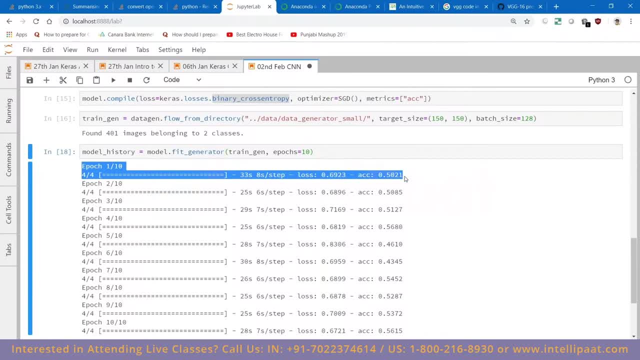 callback. that's simple, so there are callback. that's simple, so there are results. or let's say you're writing your results, or let's say you're writing your results. or let's say you're writing your own custom laws. or let's say you are own custom laws, or let's say you are. 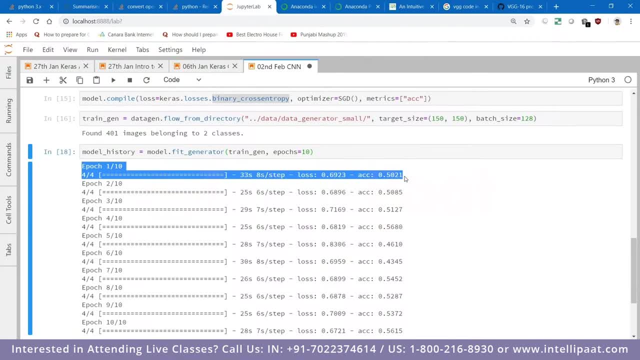 own custom laws. or let's say you are writing your own custom, writing your own custom, writing your own custom. uh, let's say um. uh, let's say um. uh. let's say um optimizer right. or let's say you are you optimizer right? or let's say you are you. 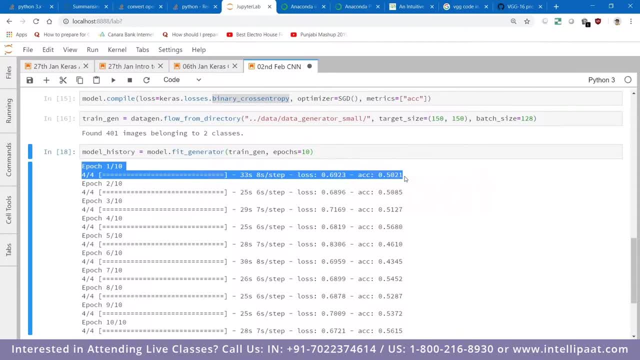 optimizer right, or let's say you are. you are decreasing your learning rate based are decreasing your learning rate based are decreasing your learning rate based on some particular, on some particular, on some particular parameters. so then you can write, i can- parameters. so then you can write, i can. 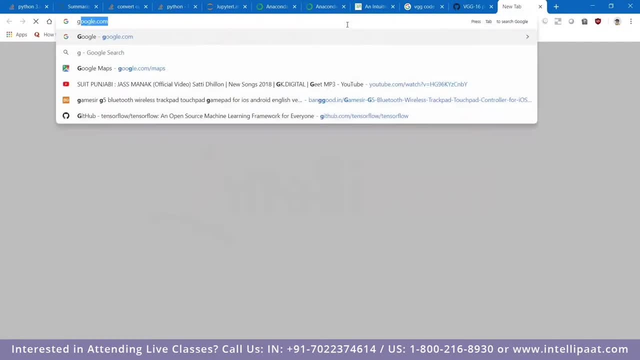 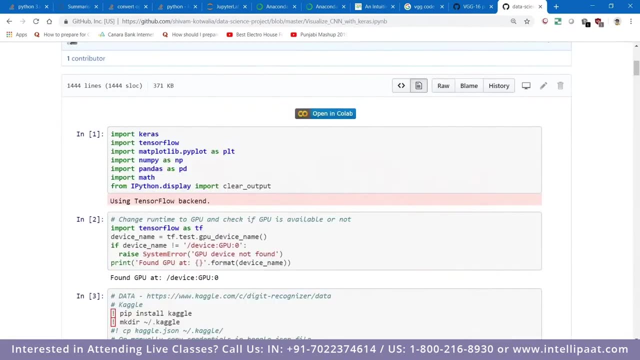 parameters. so then you can write, i can show you. i wrote this code. show you, i wrote this code. show you. i wrote this code somewhat long time ago and this contains a very good callback. and this contains a very good callback and this contains a very good callback thing. i'll let me show you. 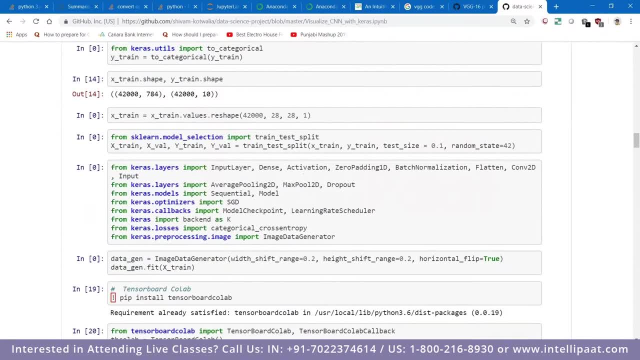 thing i'll let me show you, thing i'll let me show you. so if i show you here, so if i show you here, so if i show you here callbacks- here i'm using model callbacks, here i'm using model callbacks, here i'm using model checkpoint and learning rate scheduler. 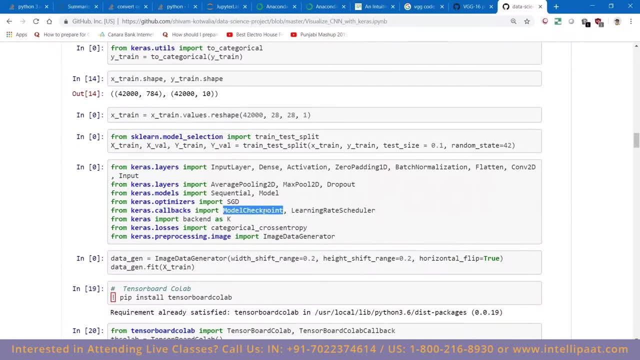 checkpoint and learning rate scheduler. checkpoint and learning rate scheduler. right, so i'm using two things. one is right. so i'm using two things. one is right. so i'm using two things. one is called tensor, one is called model called tensor. one is called model called tensor, one is called model checkpointing, another one is called 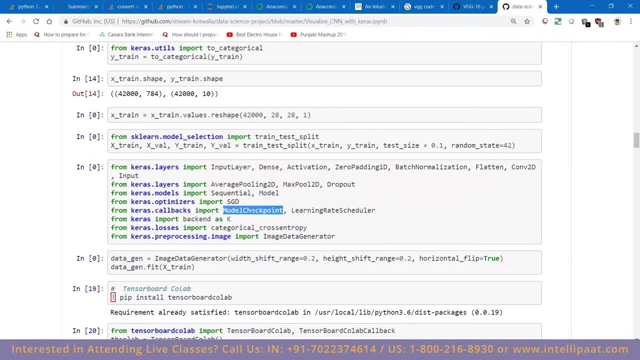 checkpointing. another one is called checkpointing, another one is called learning rate scheduler. now what this learning rate scheduler, now what this learning rate scheduler. now what this model checkpointing is doing. this model model checkpointing is doing this model model checkpointing is doing. this model checkpointing is saving the weights after. 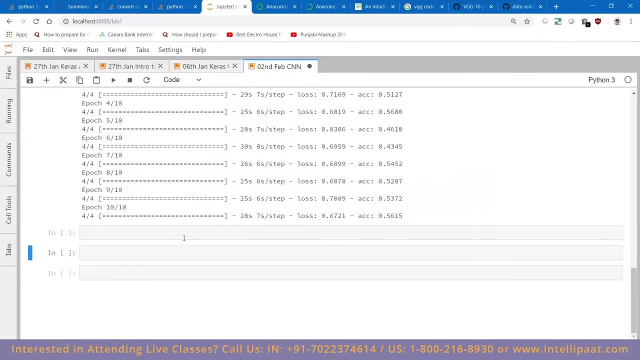 checkpointing is saving the weights after checkpointing is saving the weights after every epoch, every epoch, every epoch. so what it is is it is that after every. so what it is is it is that after every. so what it is is it is that after every epoch. if you want to run any kind of a 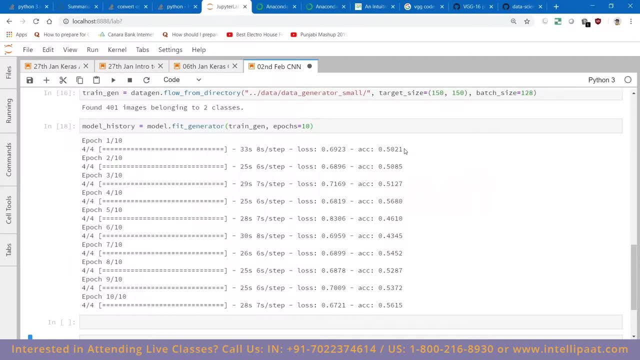 epoch, if you want to run any kind of a epoch, if you want to run any kind of a function, any kind of a function, any kind of a function, any kind of a method, then you can specify them here. method, then you can specify them here. method, then you can specify them here in the callbacks, then they will be. 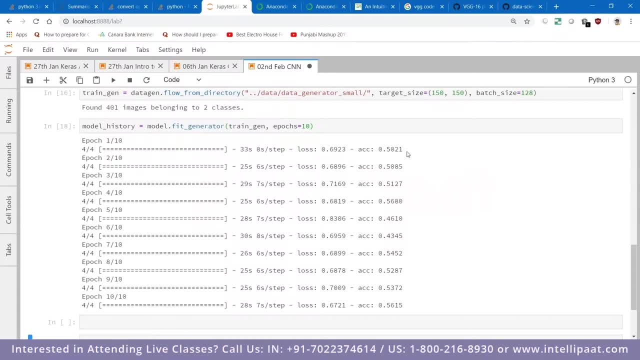 in the callbacks, then they will be in the callbacks, then they will be executed and they will be recorded in executed and they will be recorded in executed and they will be recorded in the tf dot event files, the tf dot event files, the tf dot event files. again, after the second epoch is completed: 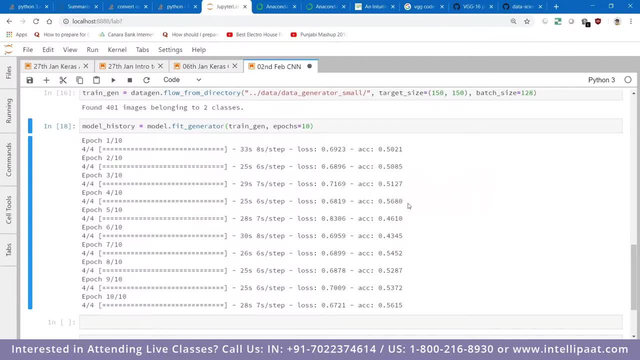 again after the second epoch is completed. again after the second epoch is completed, you run the callback. you run the callback. you run the callback after third. you run the callback after after third. you run the callback after after third. you run the callback after fourth. you run the callback function. so 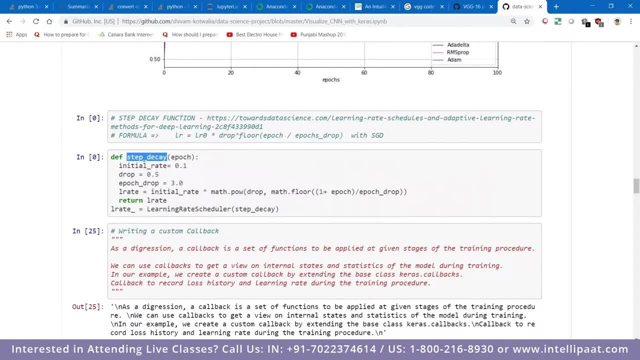 fourth, you run the callback function. so, fourth, you run the callback function. so we were here at this thing, that let's. we were here at this thing, that let's. we were here at this thing that let's say that you define your own custom step. say that you define your own custom step. 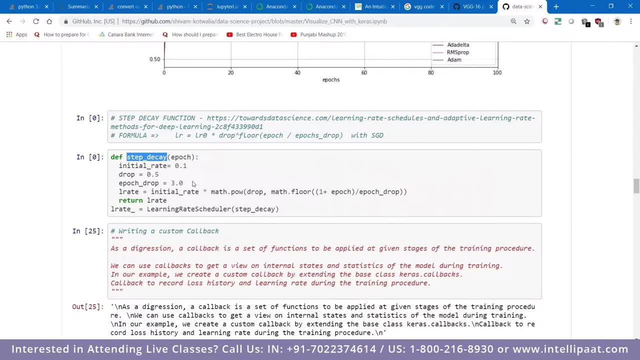 say that you define your own custom step decay function after you have done with decay function, after you have done with decay function, after you have done with the step decay. the step decay, the step decay. how do you call it? you make it your loss. how do you call it? you make it your loss. 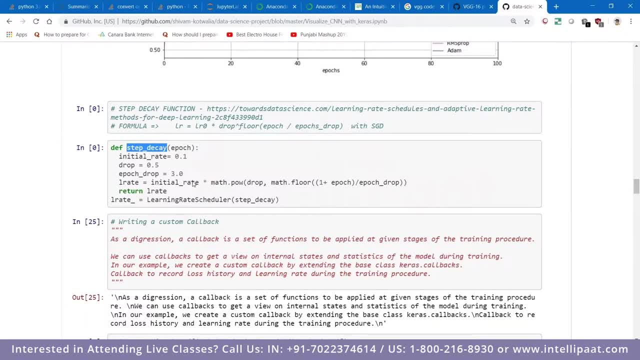 how do you call it? you make it your loss history. and when you are doing a dot fit history. and when you are doing a dot fit history. and when you are doing a dot fit, you call your callback here. you call your callback here. you call your callback here. right, so we will do the same thing out. 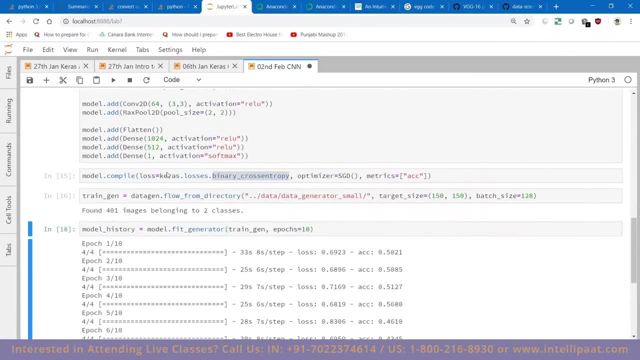 right, so we will do the same thing out right, so we will do the same thing out here. what we'll do here, what we'll do here, what we'll do. we have this thing called tensor board. we have this thing called tensor board. we have this thing called tensor board. so, if you see, i have imported this thing. 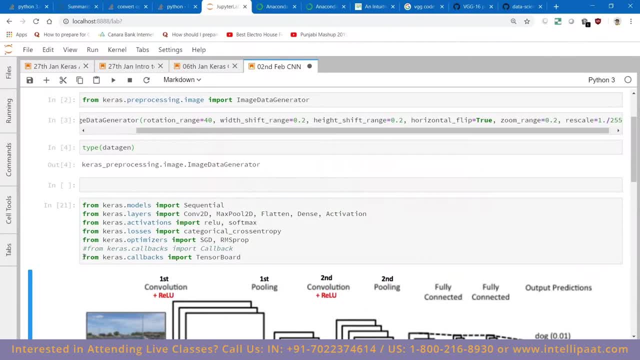 so if you see i have imported this thing, so if you see i have imported this thing, called this one is not needed. called this one is not needed. called this one is not needed. from kirazcallbacks import tensor board. from kirazcallbacks import tensor board. from kirazcallbacks import tensor board. so what i've taken is tensor board is. 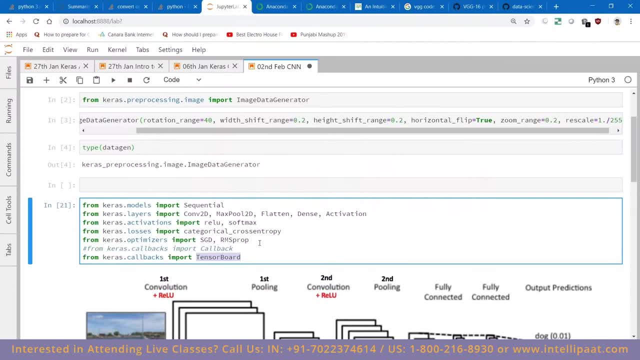 so what i've taken is tensor board is. so what i've taken is tensor board is. i'll show you what tensor board is, but i'll show you what tensor board is. but i'll show you what tensor board is, but let's first implement it at what tensor. 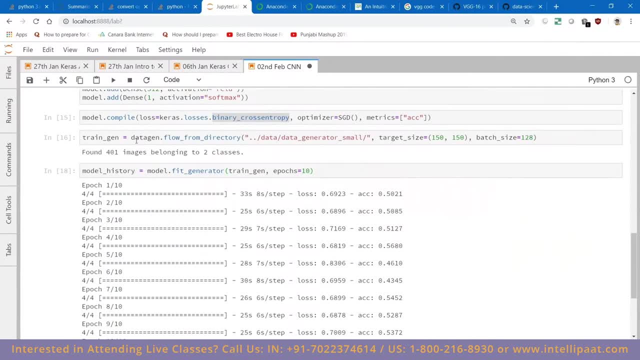 let's first implement it at what tensor? let's first implement it at what tensor board is. board is board is, before you are doing your training, you, before you are doing your training, you, before you are doing your training, you have to have to have to do a tensor. board is equal to tensor. 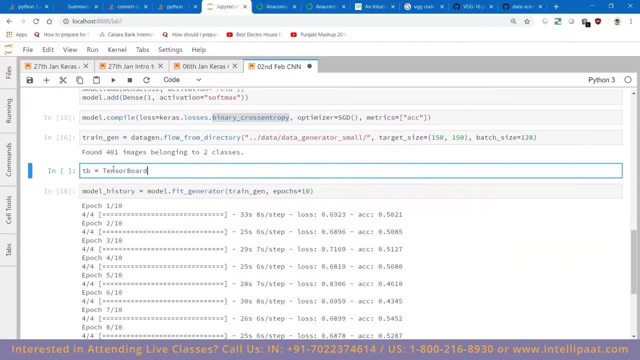 do. a tensor board is equal to tensor board board board. if it is in capital, it's a class class. if it is in capital, it's a class class. if it is in capital, it's a class class where you have to instantiate, where you have to instantiate. 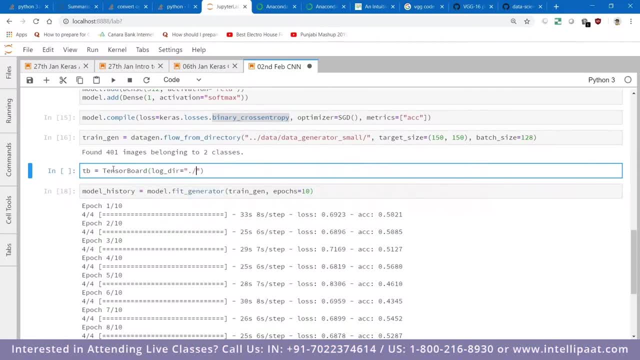 where you have to instantiate, you have, let's say log dir is equal to. you have. let's say log dir is equal to. you have. let's say log dir is equal to. let's say here only. or let's say that, let's say here only. or let's say that: 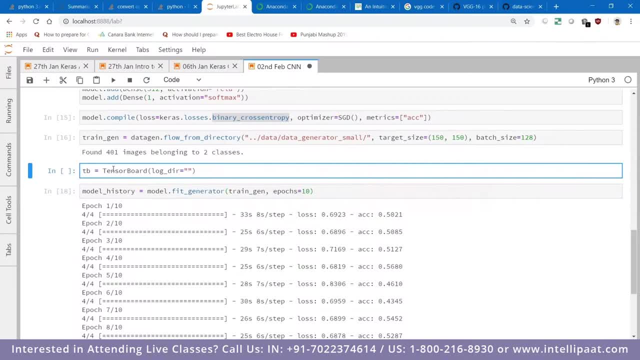 let's say here only, or let's say that you want to make it as a logs- okay, you want to make it as a logs- okay, you want to make it as a logs- okay. so what it will do, it will create a. so what it will do, it will create a. 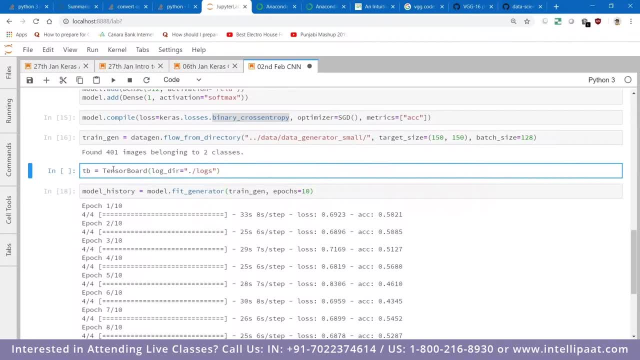 so what it will do: it will create a folder called logs in my current folder called logs in my current folder called logs, in my current directory, and then it will store all the directory, and then it will store all the directory and then it will store all the information there, right, what it will do. 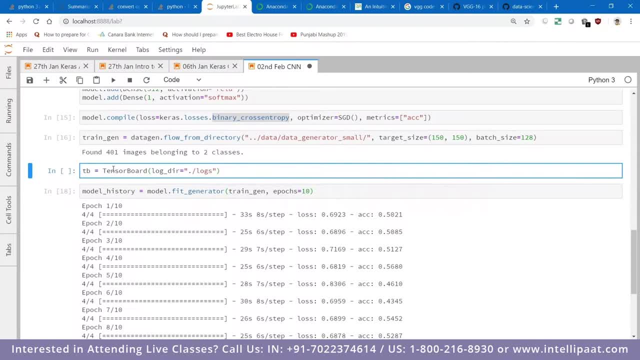 information there- right what it will do. information there- right what it will do. it will store all the information there. it will store all the information there. it will store all the information there. let's say i don't want to go in the logs. let's say i don't want to go in the logs. 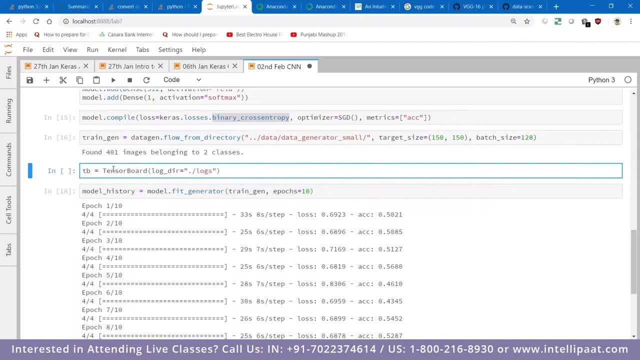 let's say, i don't want to go in the logs for the folder, i just want to stay in my for the folder. i just want to stay in my for the folder. i just want to stay in my dot folder, only stay wherever my jupiter dot folder, only stay wherever my jupiter. 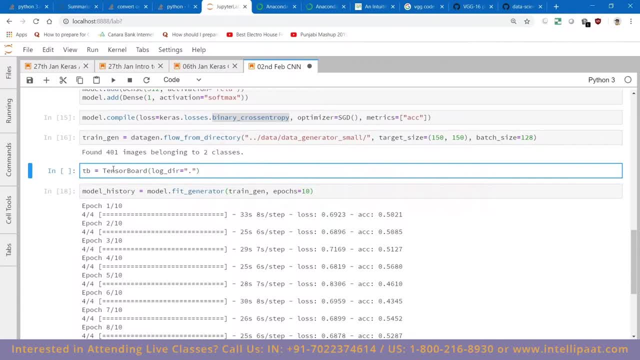 dot folder only stay wherever my jupiter notebook is: just create the file there. notebook is: just create the file there. notebook is: just create the file there. already right, but you can specify- already right, but you can specify- already right. but you can specify wherever you want to go. 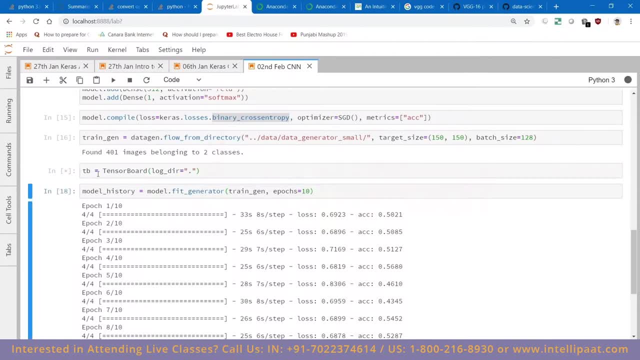 wherever you want to go. wherever you want to go, now, once you have done this, this will now, once you have done this, this will now, once you have done this, this will start this thing, tensor board, and then start this thing, tensor board. and then start this thing, tensor board. and then, while you are in your fit, generator, you. 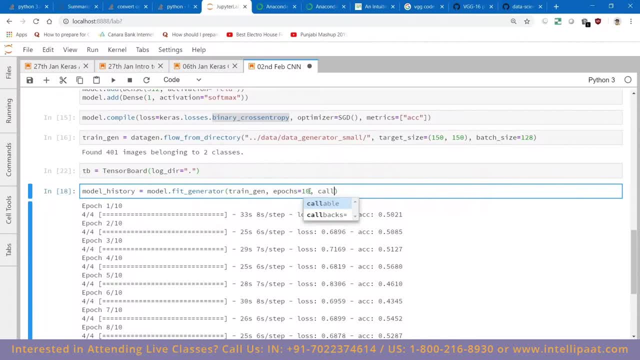 while you are in your fit generator, you, while you are in your fit generator, you will call the callbacks, will call the callbacks, will call the callbacks. let it complete callbacks, let it complete callbacks, let it complete callbacks and then it will be a list list, may, and then it will be a list list may. 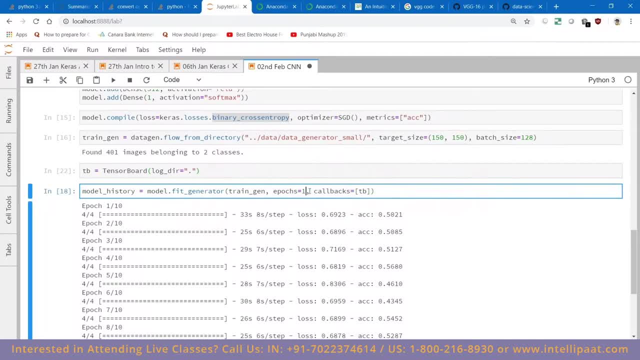 and then it will be a list list. may you give your tb? you give your tb. you give your tb, right. and let me increase this uh to 15, right, and let me increase this uh to 15, right, and let me increase this uh to 15 for now. 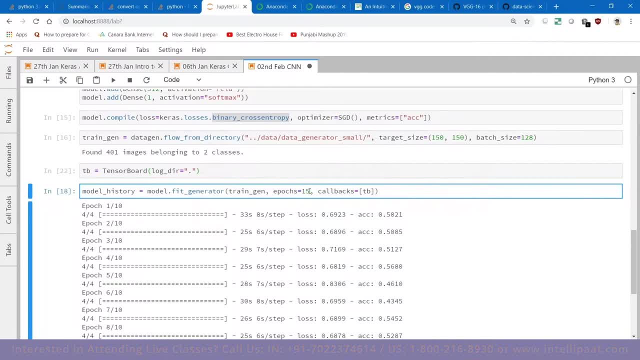 for now, for now, right. and let's let's start the model right. and let's let's start the model right, and let's let's start the model: dot, fit again, dot, fit again, dot, fit again. now, while we are doing this thing, what now, while we are doing this thing, what? 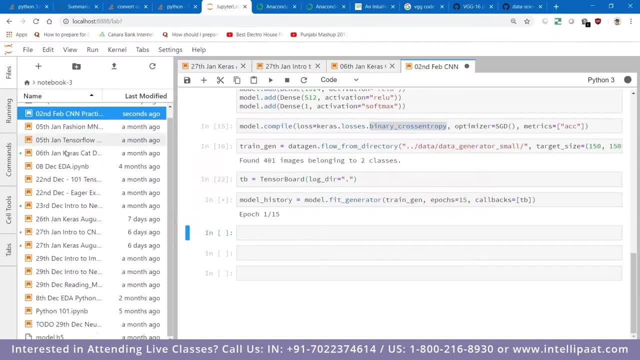 now, while we are doing this thing, what will happen is: let me show you if you go will happen is let me show you if you go will happen is let me show you, if you go in the files, in the files, in the files you see here, there is this thing that 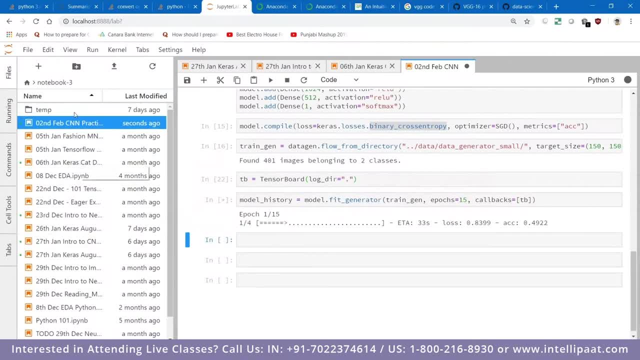 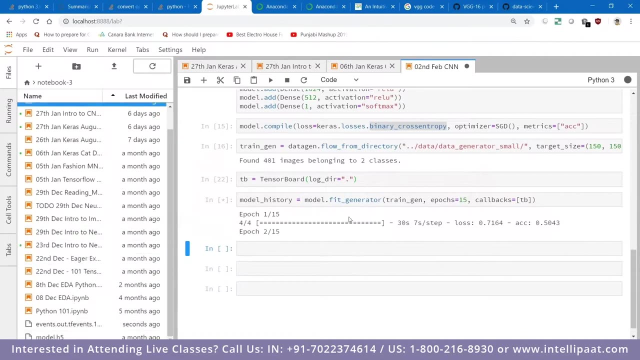 you see here. there is this thing that you see here. there is this thing that has started building up, has started building up, has started building up tfevent files after this first epoch tfevent files. after this first epoch tfevent files. after this first epoch. okay, as you can see here, 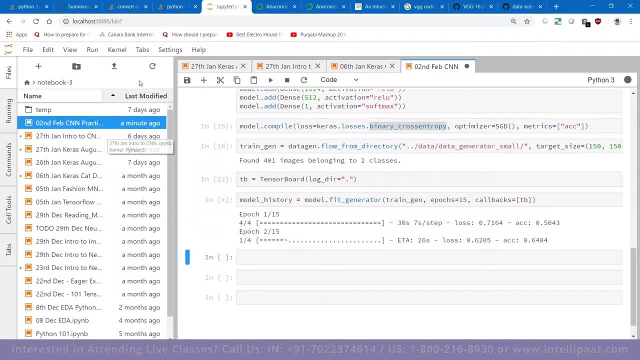 okay, as you can see here. okay, as you can see here, if i do a last modified above, if i do a last modified above, if i do a last modified above, okay, it's not coming, then you have to go. okay, it's not coming, then you have to go. 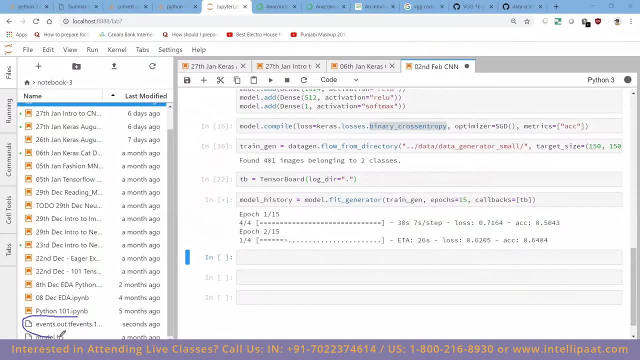 okay, it's not coming, then you have to go down and let me show you down, and let me show you down and let me show you see if you can read this thing called: see if you can read this thing called. see if you can read this thing called here on the down side, i'm just marking. 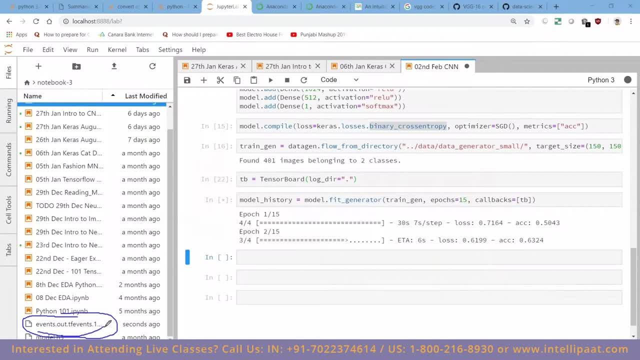 here on the down side. i'm just marking here on the down side, i'm just marking it with the blue marker, it with the blue marker, it with the blue marker. this is called eventsouttf event. this is called eventsouttf event. this is called eventsouttf event file. so what it is generating is the. 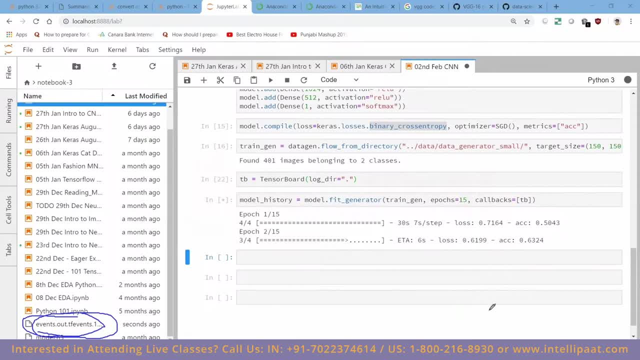 file. so what it is generating is the file. so what it is generating is the tensorflow is generating its event file. tensorflow is generating its event file. tensorflow is generating its event file, and they are stored here. and they are stored here and they are stored here. now, how can you open a tensor board? 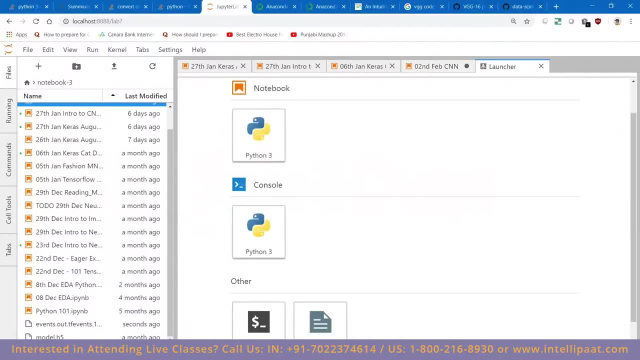 now, how can you open a tensor board now? how can you open a tensor board? very simple, very simple, very simple: open up your console console. you go there, open up your console console. you go there, open up your console console. you go there in the console, in the console. 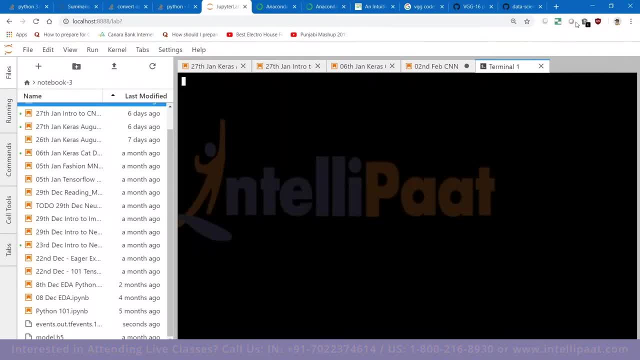 in the console. click on the console. okay, this is windows. click on the console. okay, this is windows. click on the console. okay, this is windows. this will take a little bit time. this will take a little bit time. this will take a little bit time enter and you have to just say tensor. 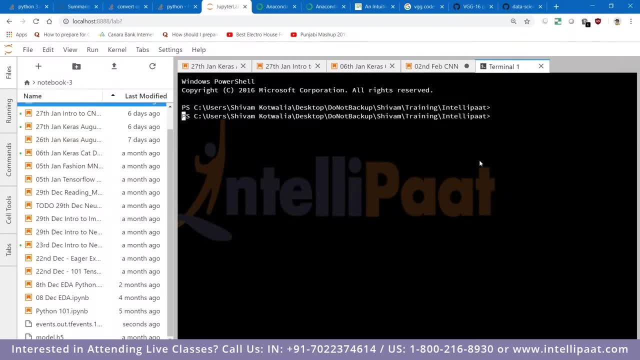 enter and you have to just say tensor enter and you have to just say tensor board. tensor board is by default board. tensor board is by default board. tensor board is by default, installed when you are installing tensor. installed when you are installing tensor. installed when you are installing tensor flow also. 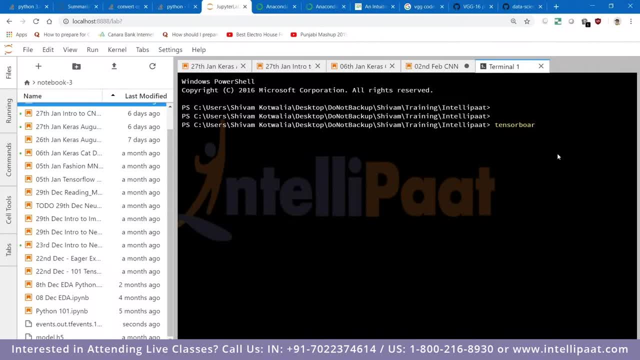 flow also flow also. the tensor b o a r b tensor board. the tensor b o a r b tensor board. the tensor b o a r b tensor board. hyphen hyphen log dir is equal to or i. hyphen hyphen log dir is equal to or i. 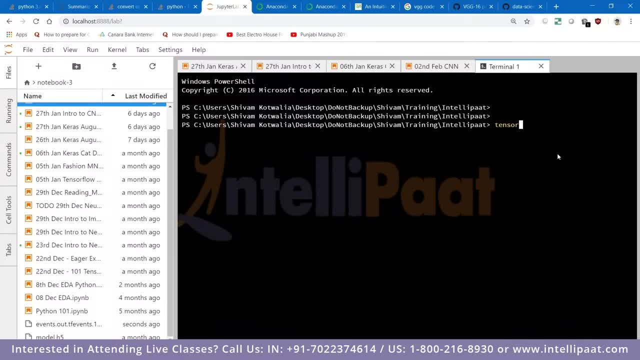 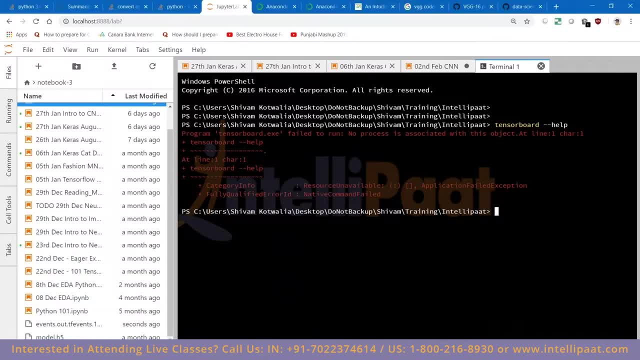 let me run it in this. let me run it in this: simple environment, simple environment, simple environment, just a second, just a second, just a second. this is here in telepath working. this is here in telepath working. this is here in telepath working. directory: directory directory. we are in notebook three. 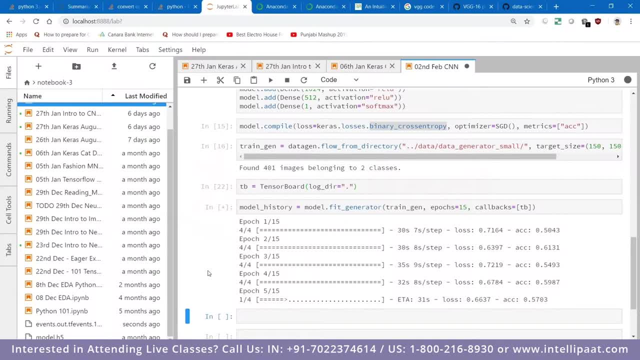 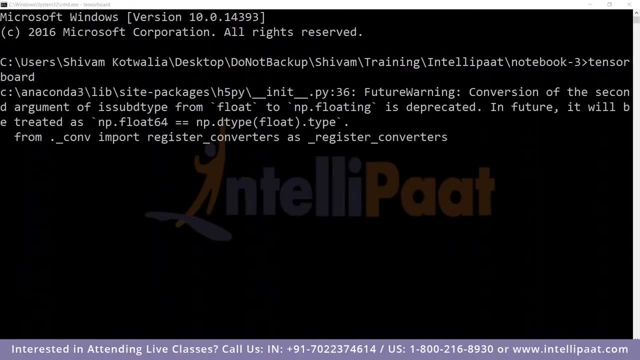 we are in notebook three. we are in notebook three, we are opening the cmd. let me open it up. let me open it up. let me open it up. so see what i ran. i just simply said so see what i ran. i just simply said. so see what i ran. i just simply said: tensor board. 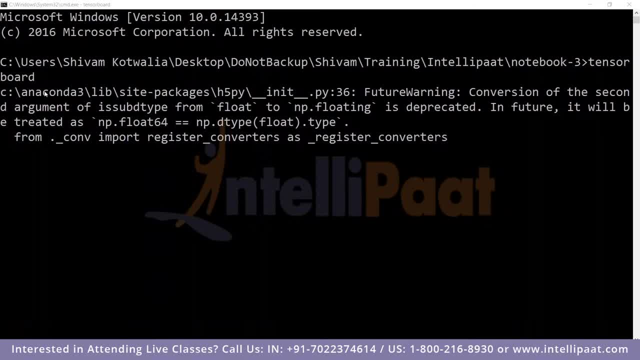 tensor board, tensor board. and this will start the tensor board and this will start the tensor board and this will start the tensor board inside the directory, inside the directory, inside the directory, right now, once, right now, once, right now, once, okay, okay, okay, i did a miss. i should. 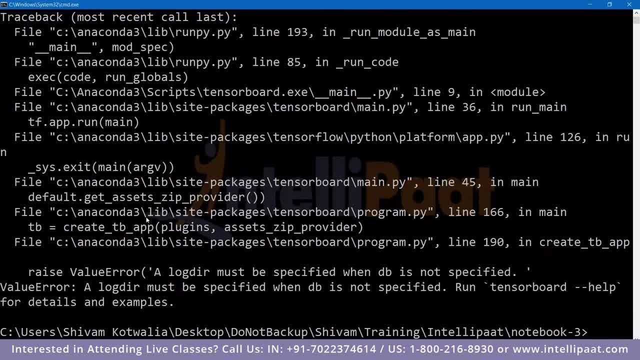 okay, okay, okay, i did a miss, i should okay, okay, okay, i did a miss. i should have specified this thing, but okay, have specified this thing. but okay, have specified this thing. but okay, first thing first. i should show you the first thing first. i should show you the. 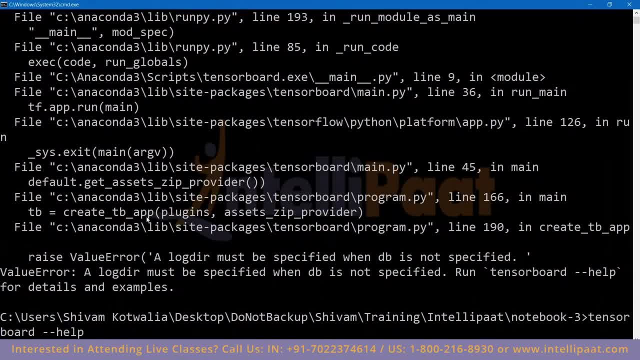 first thing. first, i should show you the help. hyphen hyphen help that. what are help? hyphen hyphen help that. what are help hyphen hyphen help that. what are the different different parameters, that the different different parameters, that the different different parameters that you can give? 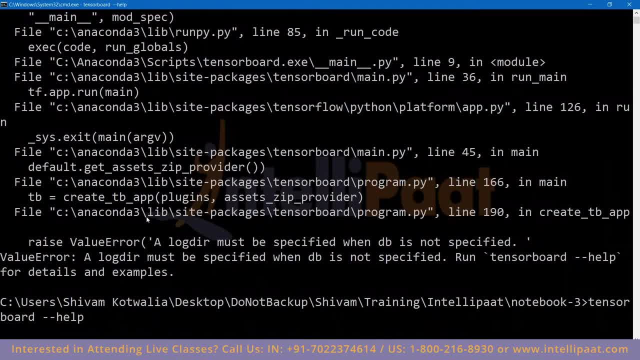 you can give, you can give. there's one parameter that's called log. there's one parameter that's called log. there's one parameter that's called log dir that you have to definitely give dir. that you have to definitely give dir. that you have to definitely give that where your logs are kept. 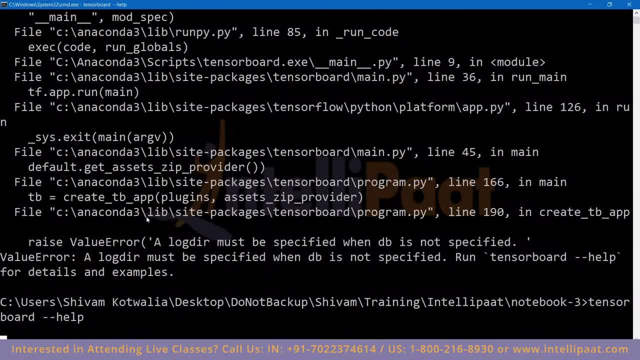 that where your logs are kept. that where your logs are kept. right where your logs are kept inside. right where your logs are kept inside. right where your logs are kept inside. which directory, which directory, which directory? okay, this is taking a small time. okay, this is taking a small time. 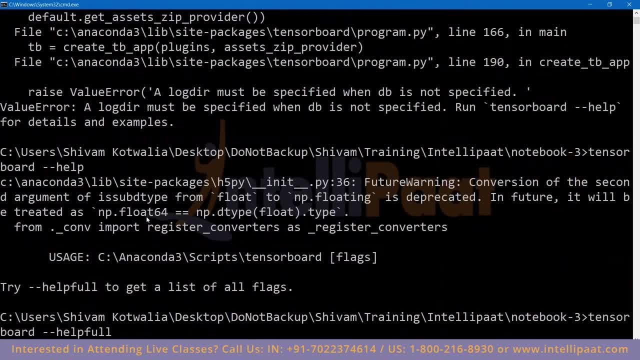 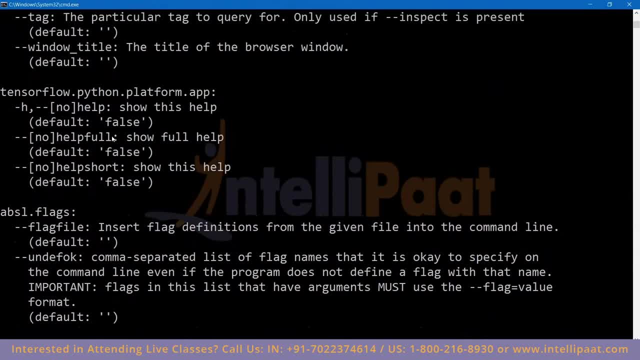 okay, this is taking a small time, so now they have changed it to helpful. so now they have changed it to helpful. so now they have changed it to helpful. it's not help, okay. so these are the different different. okay, so these are the different different. okay, so these are the different different flags that you can give. you can give a. 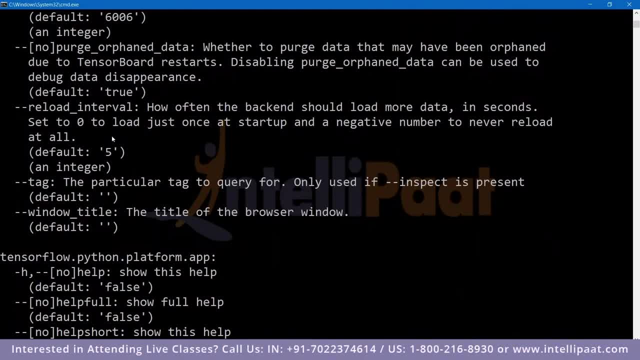 flags that you can give. you can give a flags that you can give. you can give a tag. if you're running multiple, you can tag. if you're running multiple, you can tag. if you're running multiple, you can give port number. which port do you want give port number? which port do you want? 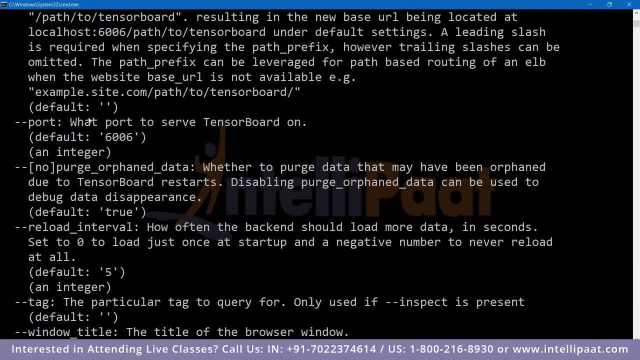 give port number. which port do you want to run, to run, to run? but the most important one is this, but the most important one is this, but the most important one is this: hyphen, hyphen loud dir. this one is the. hyphen hyphen loud dir, this one is the. 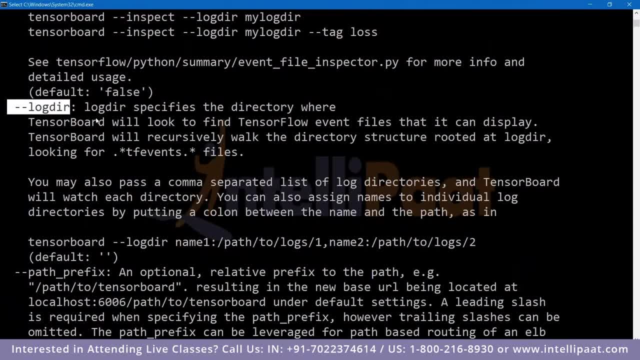 hyphen, hyphen, loud dir. this one is the one that is the most important, that you one that is the most important that you one. that is the most important that you have to give. there are multiple things have to give. there are multiple things have to give. there are multiple things that you can do with tensor board, but 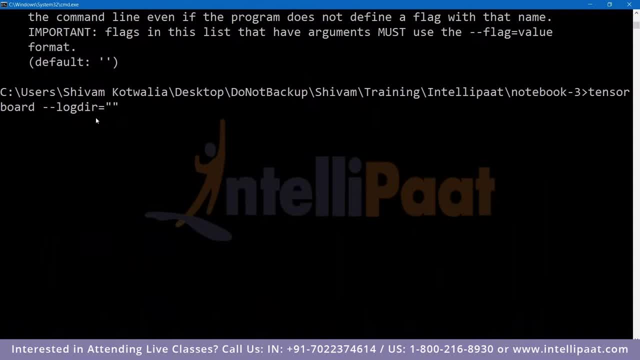 that you can do with tensor board, but that you can do with tensor board, but the most important is when you open. the most important is when you open. the most important is when you open tensor board and where you are, so i'm tensor board and where you are, so i'm. 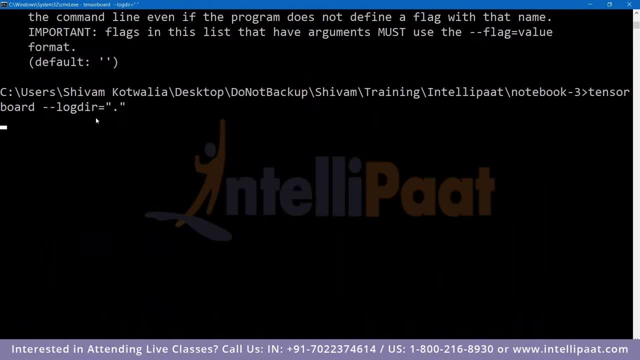 tensor board and where you are. so i'm saying dot dot means wherever you are saying dot dot means wherever you are saying dot dot means wherever you are present, that log files are present there. present that log files are present there. present that log files are present there. only let's go to our browser again and 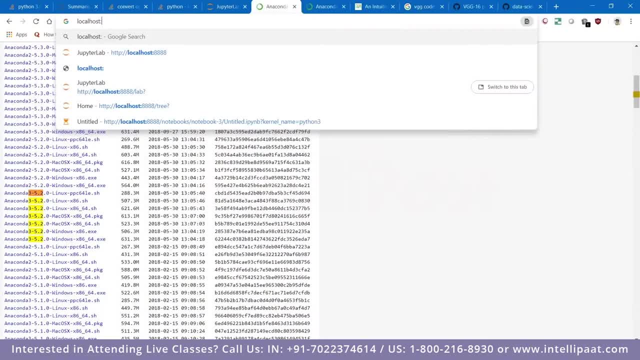 only let's go to our browser again, and only let's go to our browser again. and in the browser, let's open up our. in the browser, let's open up our. in the browser, let's open up our localhost localhost, localhost 6006. that is the by default port that we. 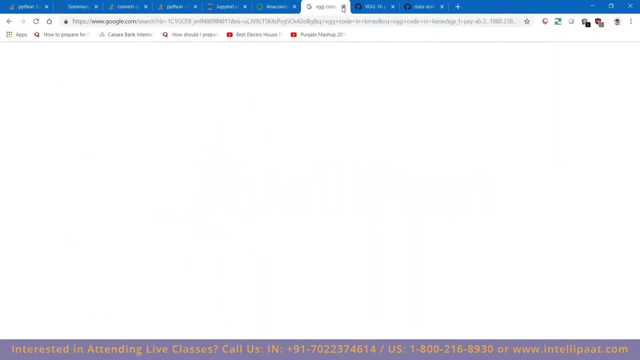 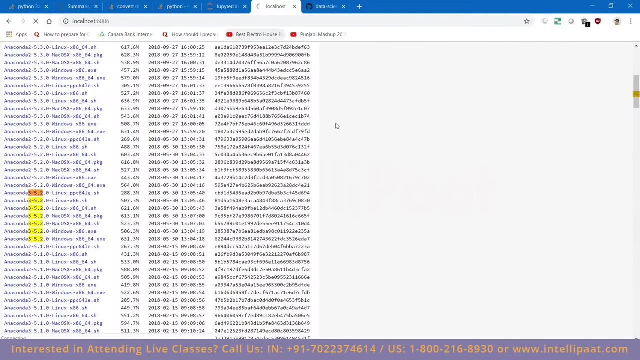 6006, that is the by default port that we- 6006, that is the by default port that we have have have takes time to run this thing. let me check, let me check, let me check. okay, so it runs on this thing. okay, so it runs on this thing. 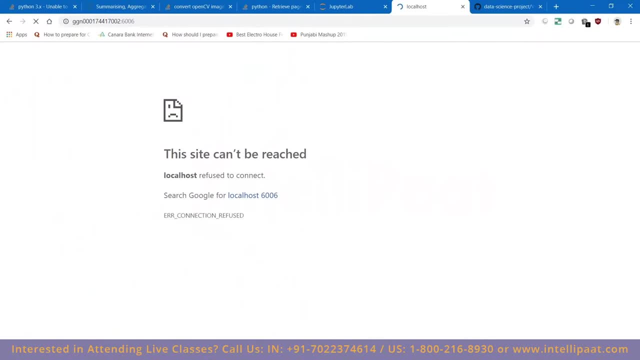 okay. so it runs on this thing, change to change to change to. so here, what you can see is the beautiful. so here, what you can see is the beautiful. so here, what you can see is the beautiful. tensor board, tensor board, tensor board. it's loading, it's loading. 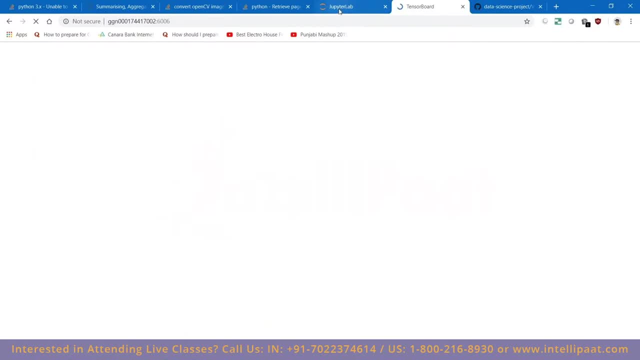 it's loading, it has multiple tabs, and let's if we see it has multiple tabs. and let's if we see it has multiple tabs. and let's if we see our model is running on. our model is running on, our model is running on 11th epoch, so you will have all the 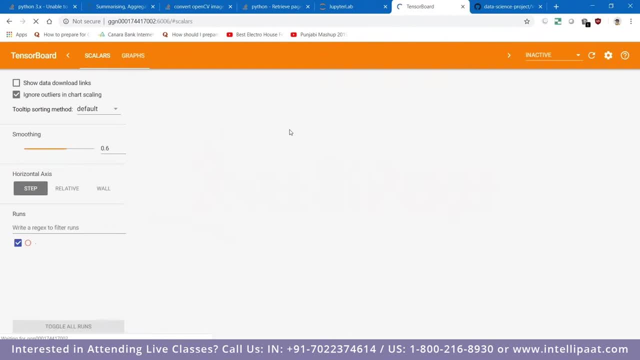 11th epoch. so you will have all the 11th epoch. so you will have all the information till 10th epoch in this thing. information till 10th epoch in this thing. information till 10th epoch in this thing. so you can see, the dashboard is here. 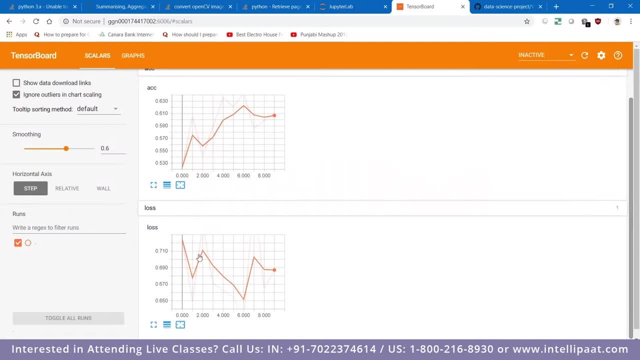 so you can see the dashboard is here, so you can see the dashboard is here and these are the loss and the accuracy, and these are the loss and the accuracy, and these are the loss and the accuracy. function, function, function. these are the same numbers that you have. 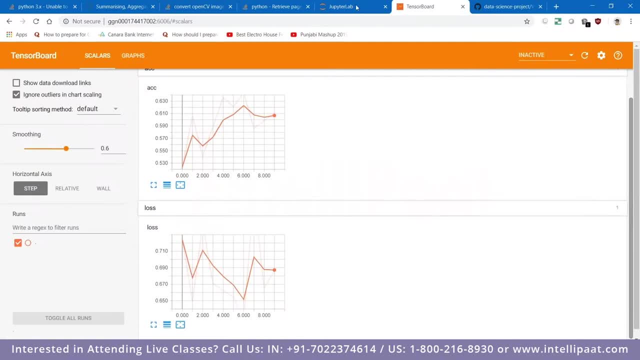 these are the same numbers that you have. these are the same numbers that you have here. so you have something that is here. so you have something that is here. so you have something that is greater than 7.1.0, greater than 7.1.0. greater than 7.1.0, and if we go back to our model, and if we see, and if we go back to our model, and if we see, and if we go back to our model, and if we see, what is the accuracy on the first? 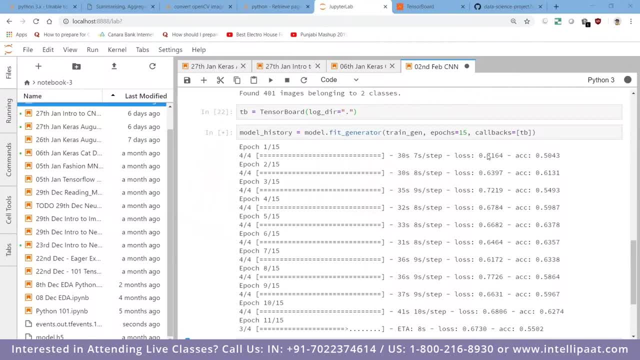 what is the accuracy on the first? what is the accuracy on the first epoch that is 50.3 sorry. this is the epoch that is 50.3 sorry. this is the epoch that is 50.3 sorry. this is the loss: 71.6 sorry. sorry. it's correct, it's. 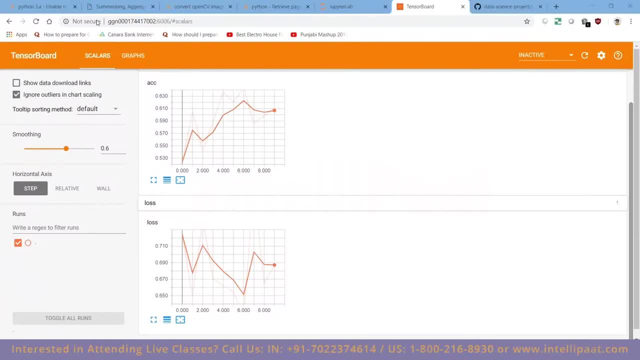 loss: 71.6. sorry, sorry, it's correct, it's loss 71.6. sorry, sorry, it's correct, it's correct, correct, correct. so it's showing you the accuracy on the. so it's showing you the accuracy on the. so it's showing you the accuracy on the top and losses at the below. so your loss. 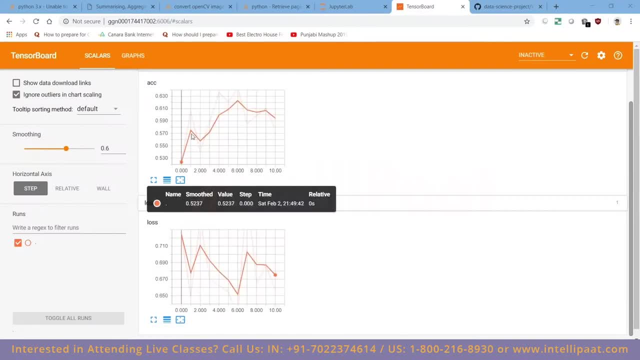 top and losses at the below. so your loss top and losses at the below, so your loss was greater than 7.10. if you go on, the was greater than 7.10. if you go on, the was greater than 7.10. if you go on the mouse, if you put it somewhere, it will. 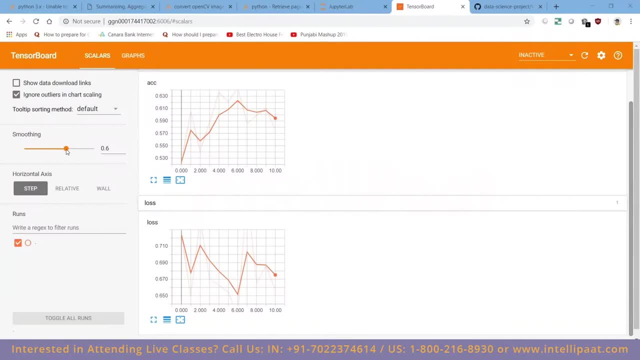 mouse. if you put it somewhere, it will mouse. if you put it somewhere, it will show you, show you, show you each and everything right. you can each and everything right. you can each and everything right. you can smoothen it up more to see the exact. smoothen it up more to see the exact. 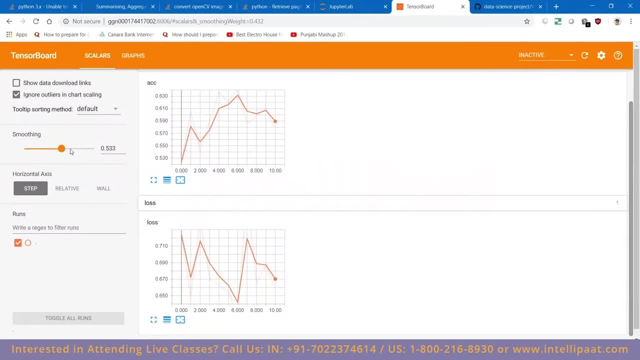 smoothen it up more to see the exact accuracy number. accuracy number. accuracy number if you're running larger- accurate if you're running larger- accurate if you're running larger accurate numbers and you want to smoothen it up. numbers and you want to smoothen it up. 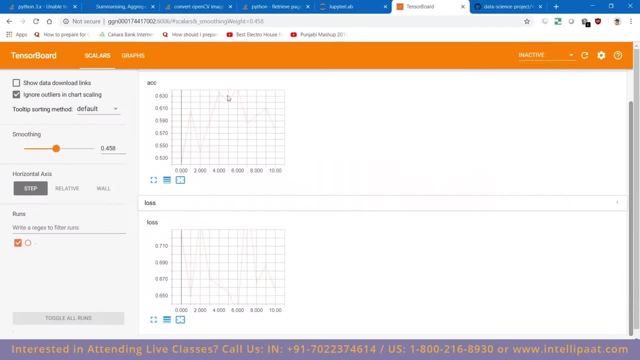 numbers and you want to smoothen it up and you can smoothen it up with here, right, right, right, and this is for loss whatever different, and this is for loss whatever different, and this is for loss whatever different kind of kind of kind of if you would have validation, accuracy. 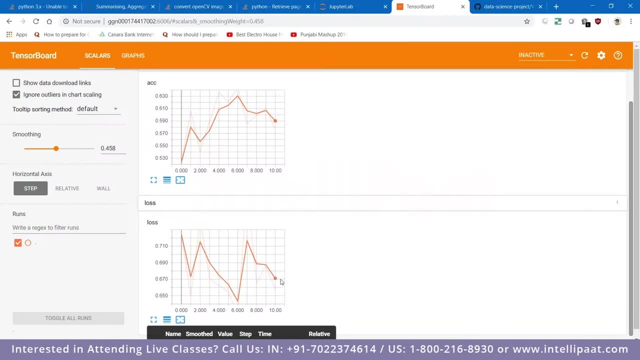 if you would have validation accuracy, if you would have validation accuracy or validation load they, or validation load they, or validation load they- they would have also been uh plotted here. they would have also been uh plotted here. they would have also been uh plotted here. these are the two things that you can. 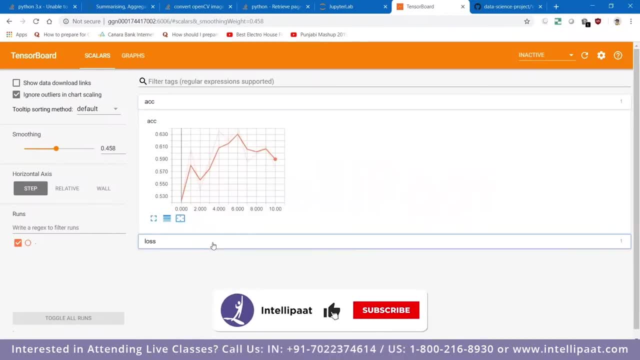 these are the two things that you can. these are the two things that you can definitely see here, definitely see here, definitely see here. so you don't have to actually view this, so you don't have to actually view this, so you don't have to actually view this, this thing here. 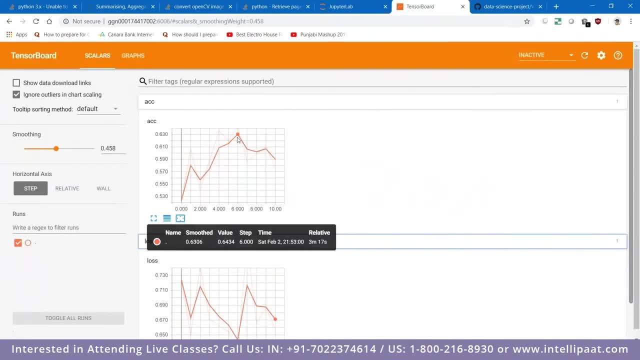 this thing here, this thing here. so what you can do is that you can. so what you can do is that you can. so what you can do is that you can quickly come up here and you can say: quickly come up here. and you can say: quickly come up here and you can say: okay, my step number six. 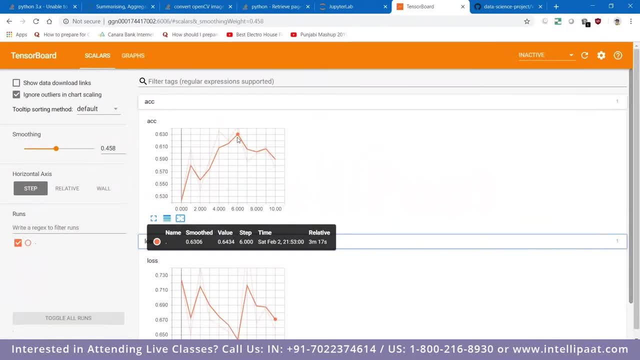 okay, my step number six. okay, my step number six is the best. this is performing the best is the best. this is performing the best is the best. this is performing the best. i will take its weight, i will take its weight, i will take its weight right. same here also for the sixth step. 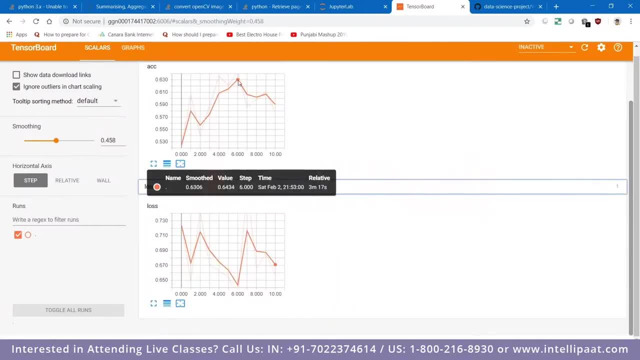 right same here also for the sixth step. right same here also for the sixth step. you had the lowest, you had the lowest, you had the lowest loss and the highest accuracy. so you'll loss and the highest accuracy. so you'll loss and the highest accuracy. so you'll say i'll take the this one. 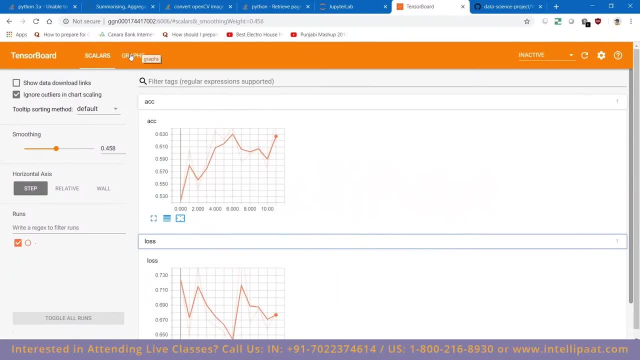 say i'll take the this one, say i'll take the this one right now. the most important thing is right now. the most important thing is right now. the most important thing is visualizing your model. so if you click, visualizing your model, so if you click, 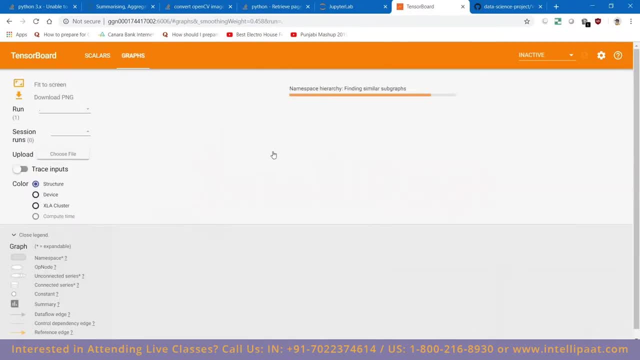 visualizing your model. so if you click on this graph button, on this graph button, on this graph button, you will see your model here, how it. you will see your model here, how it. you will see your model here how it looks like, looks like, looks like. this is how your model is actually. 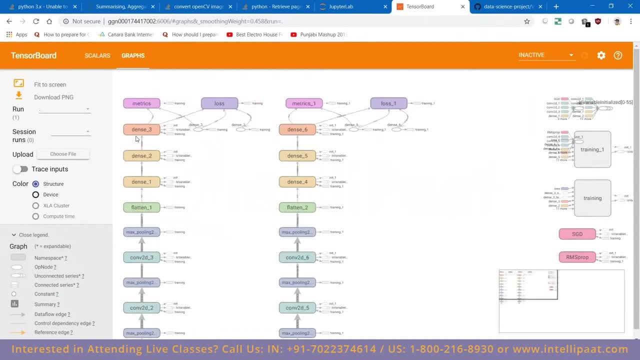 this is how your model is actually. this is how your model is actually. so if you can zoom in, you can zoom in. so if you can zoom in, you can zoom in. so if you can zoom in, you can zoom in and see and see and see how these things are you first, you had 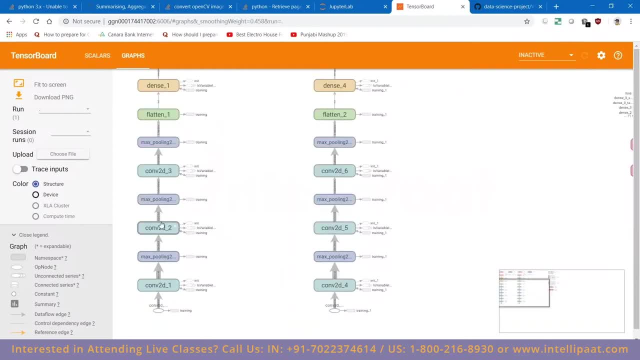 how these things are you first. you had: how these things are you first. you had this convolution one right. then you had this convolution one right, then you had this convolution one right. then you had a max pooling, then con, then max pooling. a max pooling, then con, then max pooling. 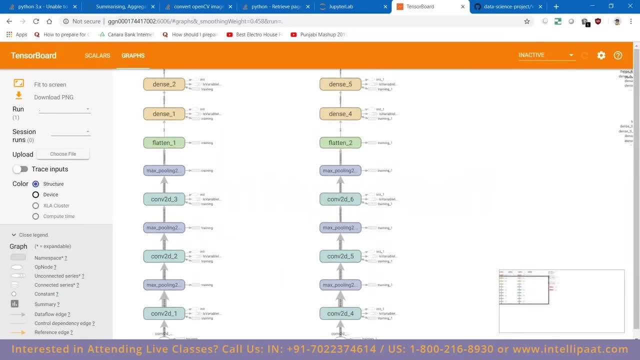 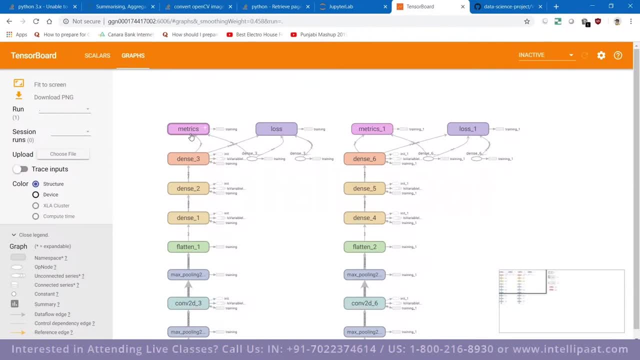 a dense layer, then again a dense, a dense layer, then again a dense layer, and then you had some a matrix to layer, and then you had some a matrix to layer, and then you had some a matrix to identify what kind of a matrix it uh. identify what kind of a matrix it uh. 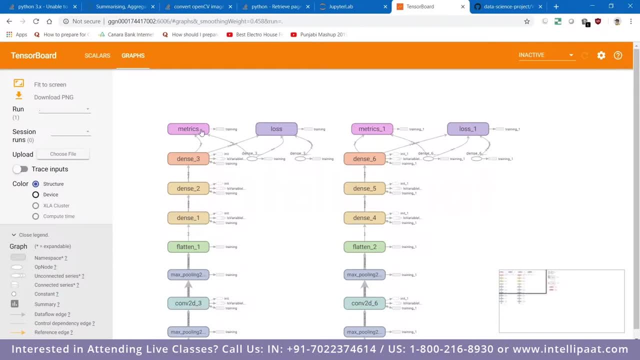 identify what kind of a matrix it uh, what kind of accuracy it is. and then you what kind of accuracy it is, and then you what kind of accuracy it is, and then you had the loss here, had the loss here, had the loss here. if you click on this loss here, you will. 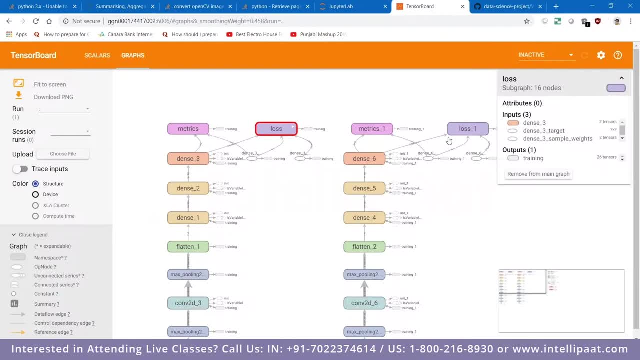 if you click on this loss here, you will. if you click on this loss here, you will be taken to the loss section on the be taken to the loss section on the be taken to the loss section on the right. you can see that this is giving right. you can see that this is giving. 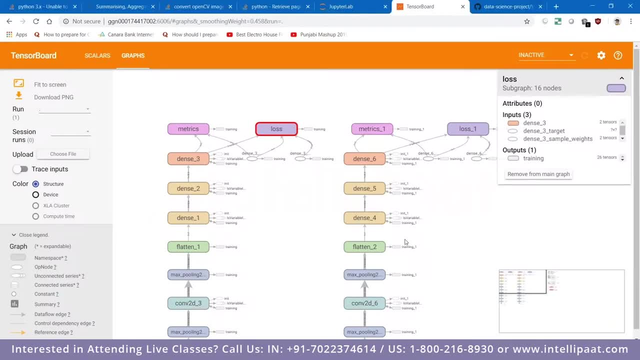 right, you can see that this is giving you all the things out here. you can also you all the things out here. you can also you all the things out here. you can also shift your model here, and then you can shift your model here, and then you can. 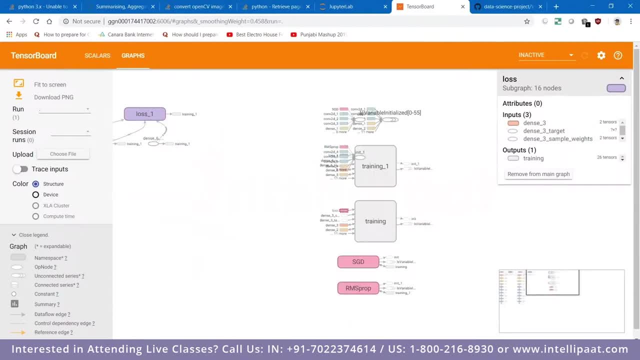 shift your model here and then you can see, see, see. this is how you're assumed in variable. this is how you're assumed in variable. this is how you're assumed in variable as as as: sorry, so if you click on each thing, then sorry. so if you click on each thing, then sorry. so if you click on each thing, then you can have this. let's say, i click on, you can have this. let's say i click on, you can have this. let's say, i click on this dense layer, then you have this thing, this dense layer, then you have this thing. 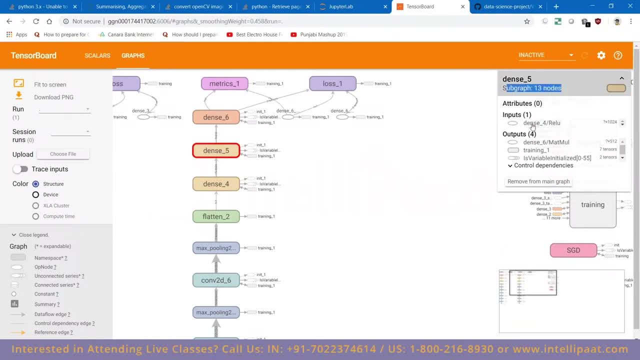 this dense layer. then you have this thing on dense sub node, 13th node. this is on dense sub node, 13th node. this is on dense sub node, 13th node. this is the 13th node. the input is coming from the 13th node. the input is coming from. 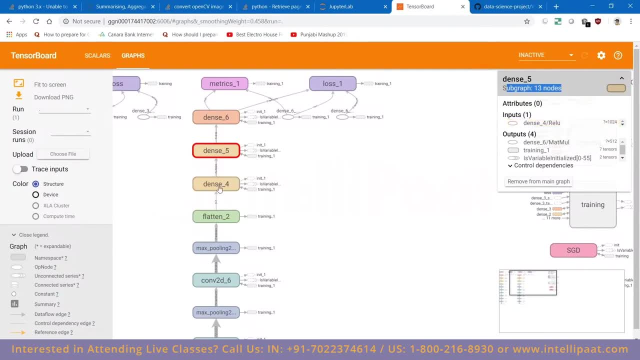 the 13th node, the input is coming from dense 4. that is absolutely right, because dense 4, that is absolutely right, because dense 4, that is absolutely right, because then this 4 is there and then you have, then this 4 is there and then you have. 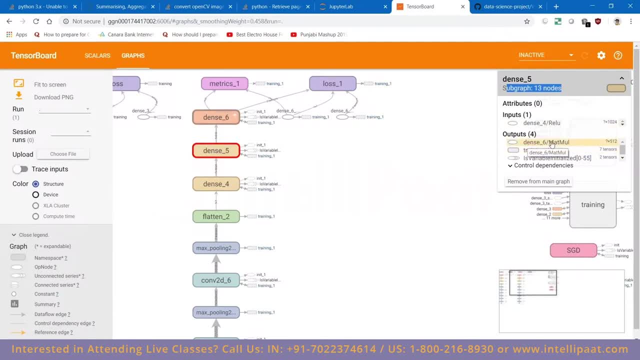 then this 4 is there, and then you have dense 5, and then the output is going in dense 5, and then the output is going in dense 5, and then the output is going in dense 6 for the matrix multiplication, dense 6 for the matrix multiplication. 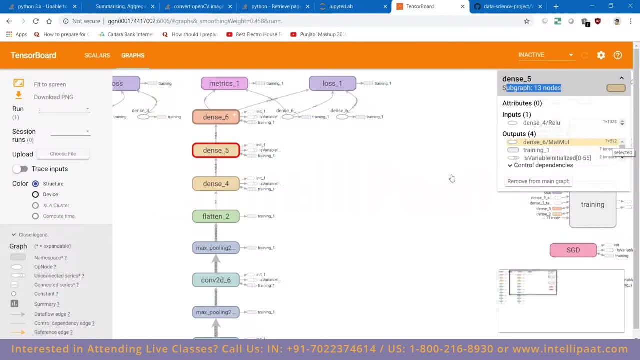 dense 6 for the matrix multiplication with 512 variables, and that is with 512 variables, and that is with 512 variables. and that is absolutely right, because in the first we absolutely right, because in the first we absolutely right, because in the first we had 1024, then we had 512 and then the 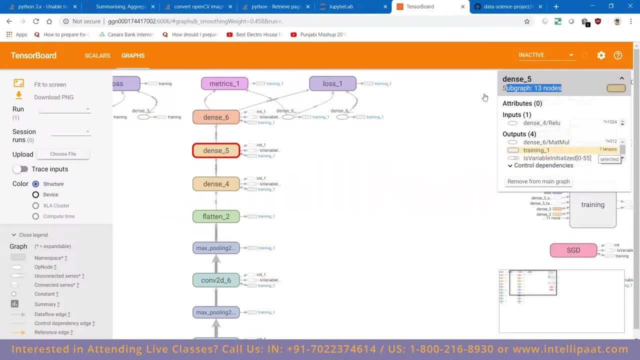 had 1024, then we had 512, and then the had 1024, then we had 512, and then the output will be in the form of seven. output will be in the form of seven. output will be in the form of seven tensors. absolutely correct, if you go this. 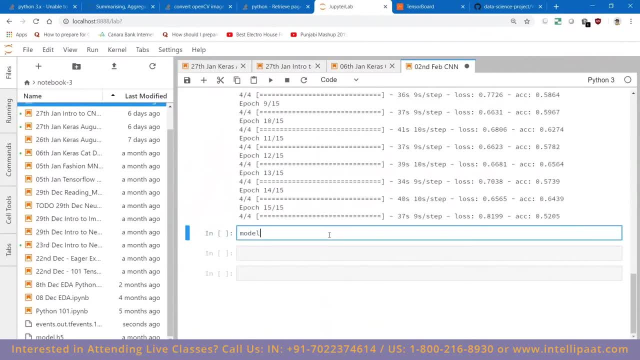 tensors absolutely correct. if you go this tensors absolutely correct. if you go this thing and if you just do a model dot thing, and if you just do a model dot thing and if you just do a model dot, history, history, history, it will model dot summary, it will be. 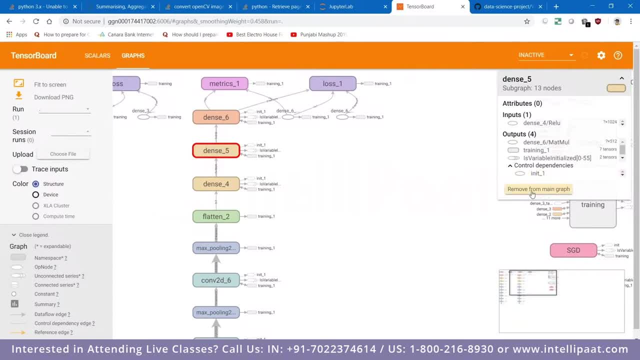 it will model dot summary: it will be multiple dependencies. if you want to multiple dependencies, if you want to multiple dependencies, if you want to have more information on the graph, then have more information on the graph, then have more information on the graph, then you should definitely show this to. 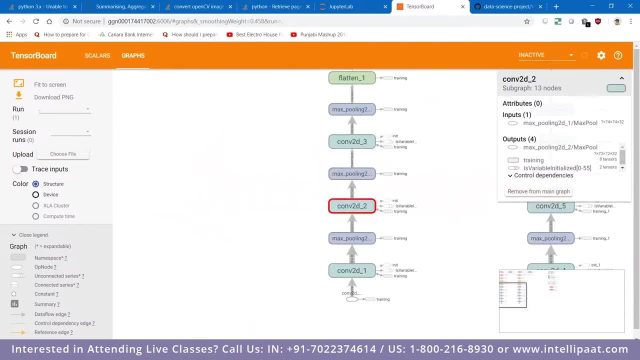 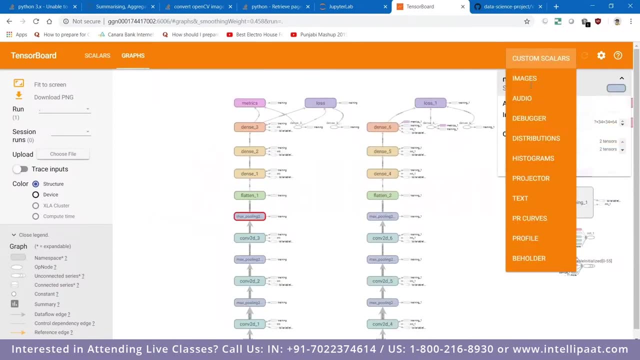 you should definitely show this to. you should definitely show this to client, client, client. these are like showing: here you can go. these are like showing here you can go. these are like showing: here you can go, anytime you can go there. it has multiple things, multiple things. it has multiple things, multiple things. 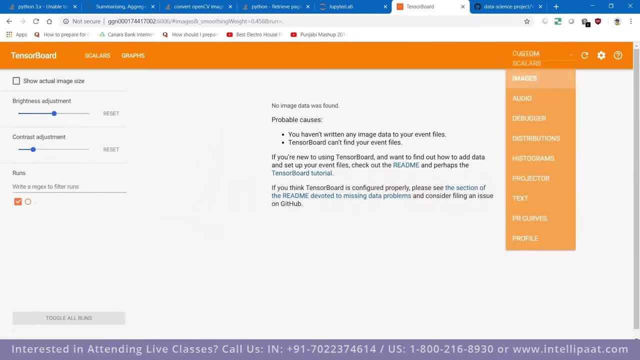 it has multiple things, multiple things. you can even see images inside it. so you can even see images inside it. so you can even see images inside it. so right now we are not given, but if you, right now we are not given, but if you, right now we are not given, but if you would have given, you can see your. 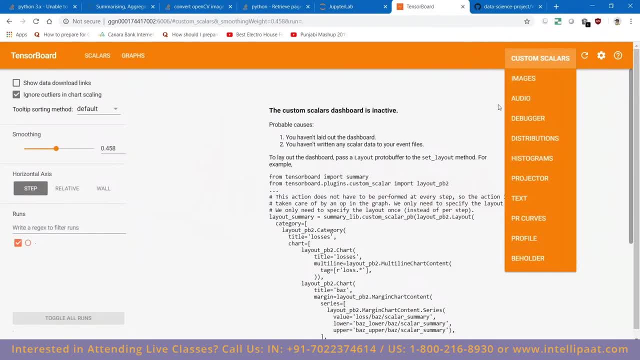 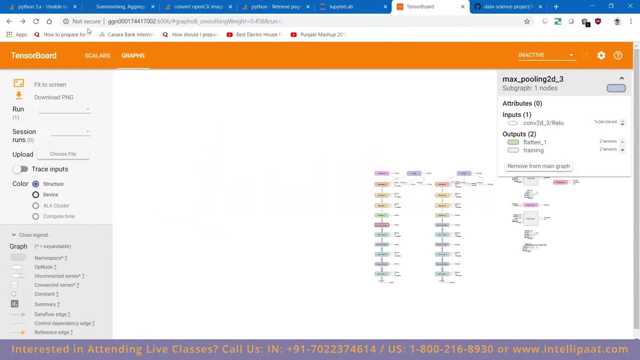 would have given. you can see. your would have given, you can see your uh things out there also. i'm so sorry, you have multiple things in here. you can you have multiple things in here. you can you have multiple things in here. you can download this graph also by clicking on. 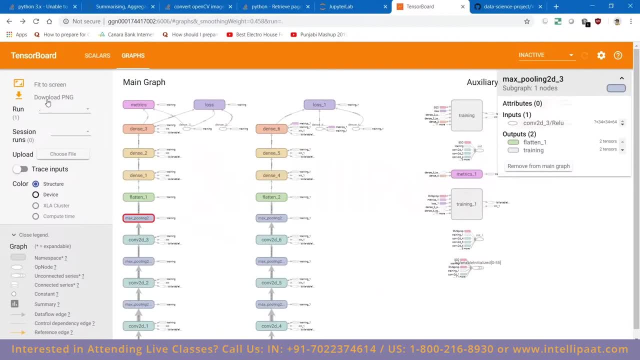 download this graph also by clicking on. download this graph also by clicking on this fit to this, fit to this, fit to screen, and then you could have download screen, and then you could have download screen and then you could have download this also. this also, this also session. you can see multiple devices also. 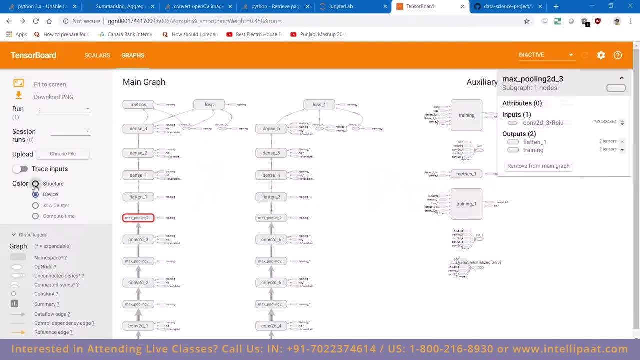 session: you can see multiple devices also. session: you can see multiple devices also. let's say i have only one device. let's say i have only one device. let's say i have only one device. you could have multiple devices. and then you could have multiple devices. and then 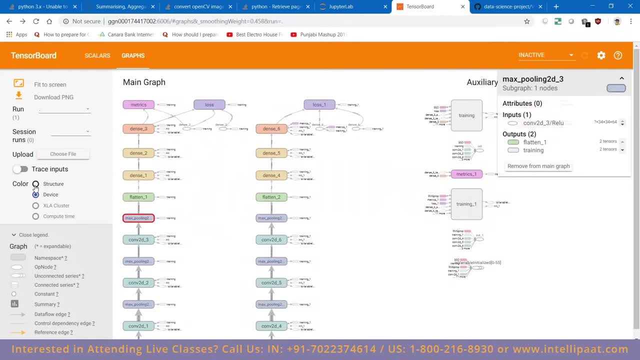 you could have multiple devices and then also you could have taken also. you could have taken also, you could have taken trace inputs. so you want to see where trace inputs, so you want to see where trace inputs, so you want to see where your inputs are going till now. 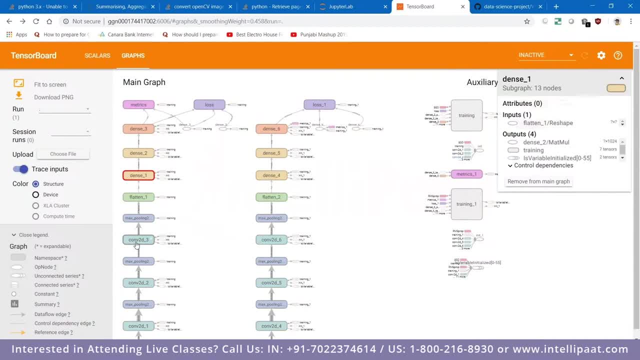 your inputs are going till now. your inputs are going till now. let's say: if i click on this, it will. let's say: if i click on this, it will. let's say: if i click on this, it will show me how is my input working for this. 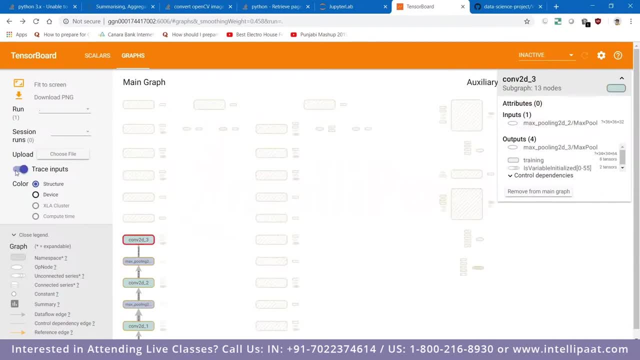 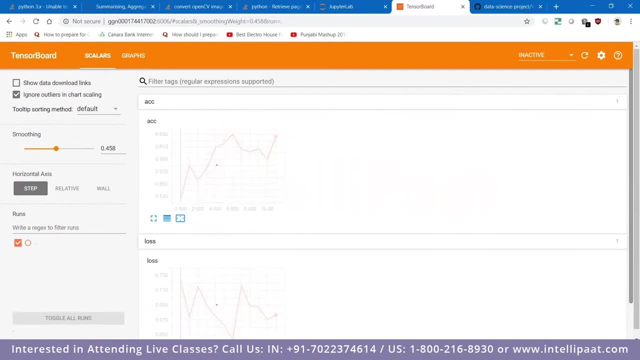 show me how is my input working for this. show me how is my input working for this particular section, particular section, particular section: right, right, right, choose lesions, whatever you want to have. choose lesions, whatever you want to have. choose lesions, whatever you want to have. right, it's a very, very useful thing. 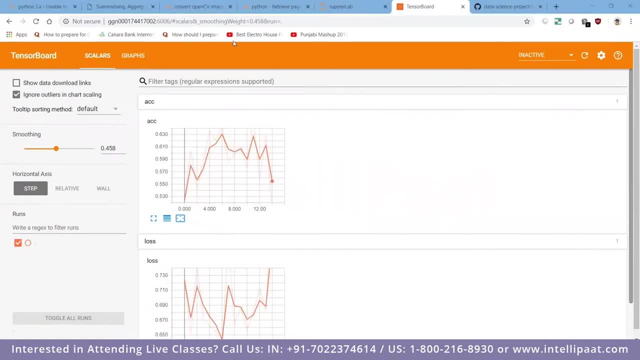 right, it's a very, very useful thing. right, it's a very, very useful thing. you will come to know more about this. you will come to know more about this. you will come to know more about this when you're training. you know very large. when you're training, you know very large. 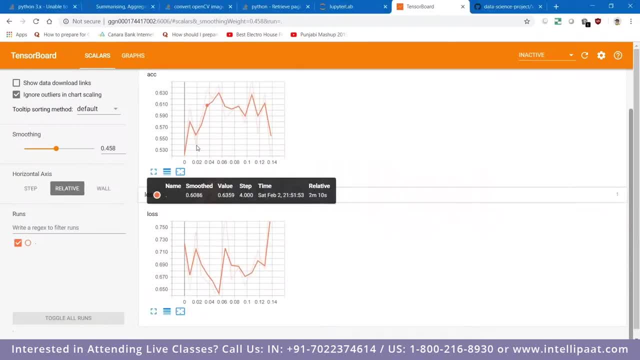 when you're training, you know very large layer networks, layer networks, layer networks. you have a relative number relative. you have a relative number relative. you have a relative number. relative number means what is the difference number means? what is the difference number means? what is the difference between the previous and the past one? so 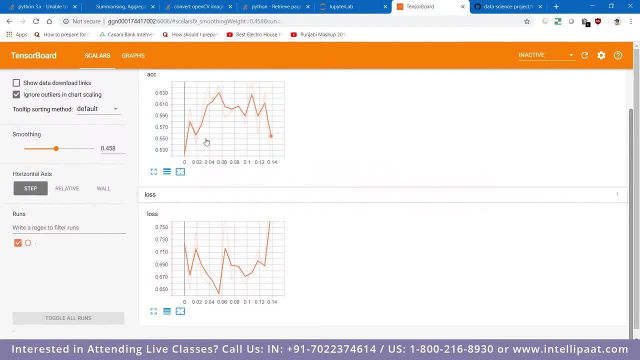 between the previous and the past one. so between the previous and the past one. so it's like a step function that you're it's like a step function that you're it's like a step function that you're doing, doing, doing. then you have the step. step is the. 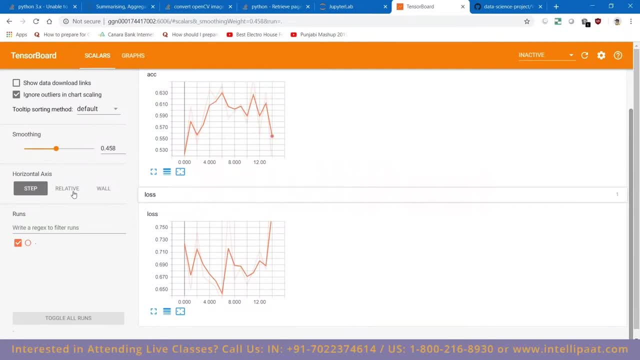 then you have the step step. is the. then you have the step step. is the exact one? that the exact one, that the exact one, that the recording for each epoch and relative is recording for each epoch and relative is recording for each epoch and relative. is that you're trying to get the number? 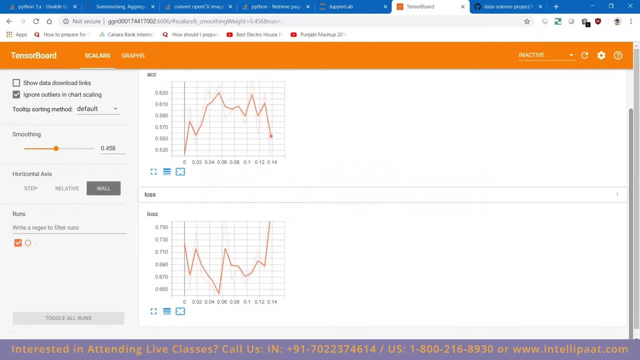 that you're trying to get the number, that you're trying to get the number from the previous one, how it is changing from the previous one, how it is changing from the previous one, how it is changing from the previous one, from the previous one, from the previous one. but the only thing, extra idea- to do two. 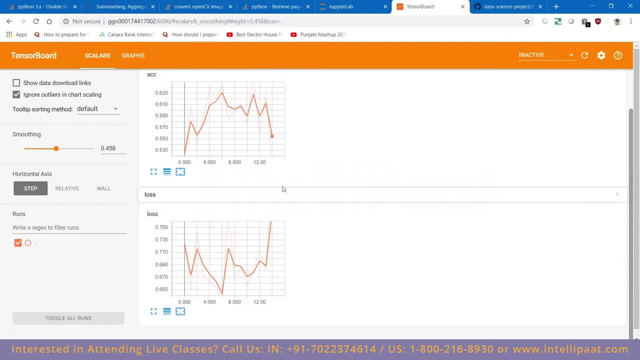 but the only thing extra idea to do two, but the only thing, extra idea to do two things, that extra idea to do to bring things, that extra idea to do to bring things, that extra idea to do to bring tensor board, was that first of all that tensor board, was that first of all that. 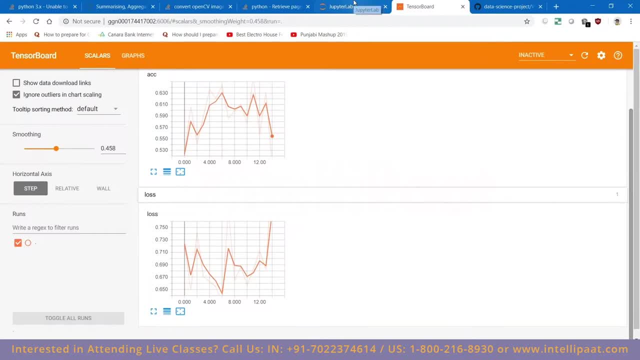 tensor board. was that, first of all, that you have to tell that you, you have to tell that you, you have to tell that. you have to tell the model that model, please have to tell the model that model, please have to tell the model that model, please, after every, after every epoch you have. 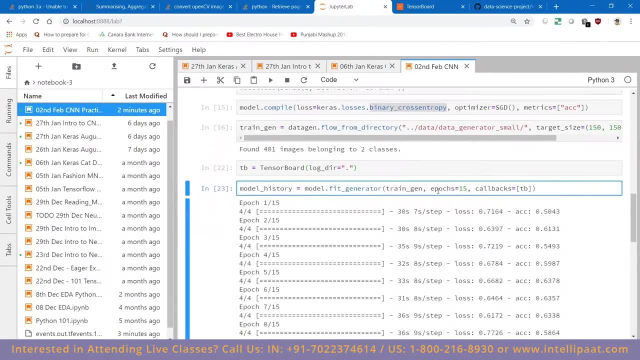 after every, after every epoch you have, after every, after every epoch you have to to to save those things for me inside this, save those things for me inside this, save those things for me inside this: filed call, callbacks, callbacks. so you filed call, callbacks, callbacks. so you filed call, callbacks, callbacks. so you have given a list. list me i've given tv. 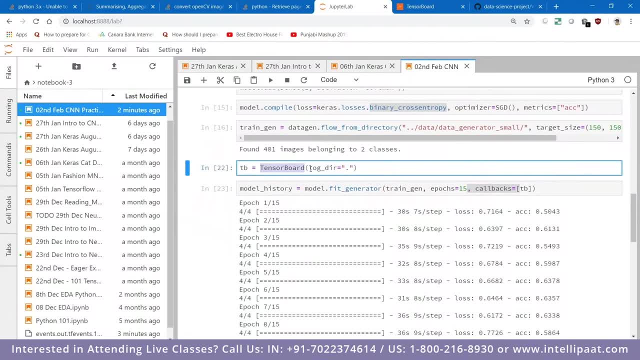 have given a list list me i've given tv. have given a list list me, i've given tv. tv is actually what it's- an instance of. tv is actually what it's an instance of. tv is actually what it's: an instance of tensor board and tensor board. how did 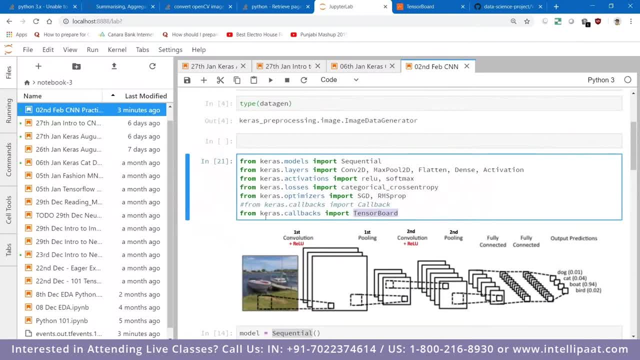 tensor board and tensor board. how did tensor board and tensor board? how did you declare it? you declared it from, you declared it. you declared it from, you declared it. you declared it from kirazcallbackstensorboard, now once. kirazcallbackstensorboard, now once. kirazcallbackstensorboard, now once. you are done with this tensor board, how? 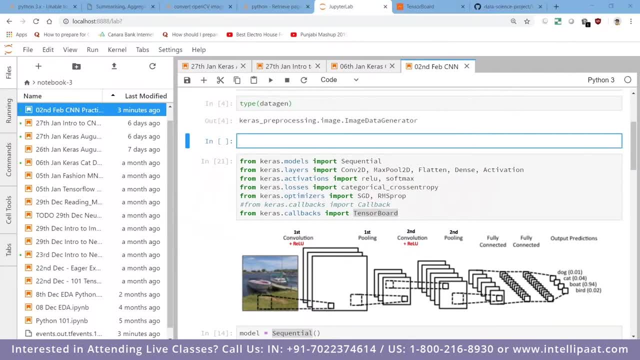 you are done with this tensor board. how you are done with this tensor board. how did you open the tensor board tensor? did you open the tensor board tensor? did you open the tensor board tensor board? you opened in the command prompt board. you opened in the command prompt. 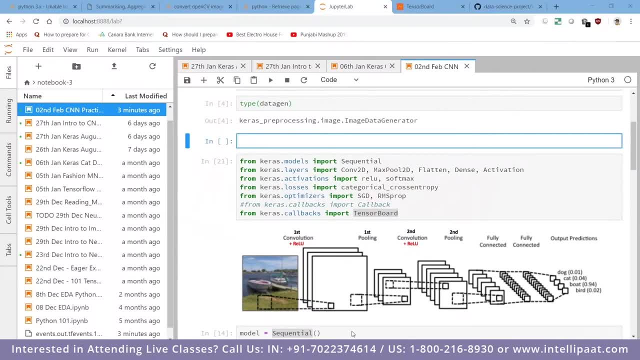 board. you opened in the command prompt, you went to the folder where you are, you went to the folder where you are, you went to the folder where you are running this thing, and then you just running this thing, and then you just running this thing, and then you just write: tensor board- hyphen, hyphen, log dir. 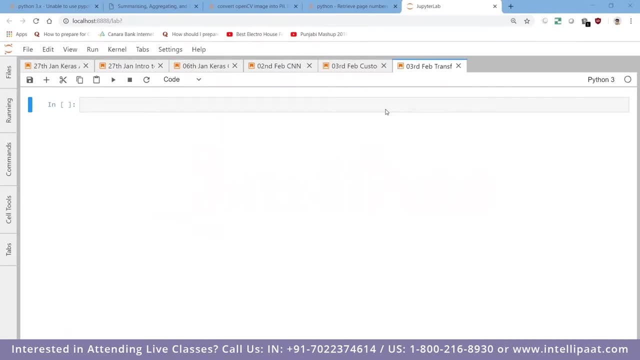 transfer learning now. what is this transfer learning now? what is this transfer learning now? what is this transfer learning and how does it matter? transfer learning, and how does it matter to me and how does it matter to the to me and how does it matter to the to me and how does it matter to the world? now, if you are working in 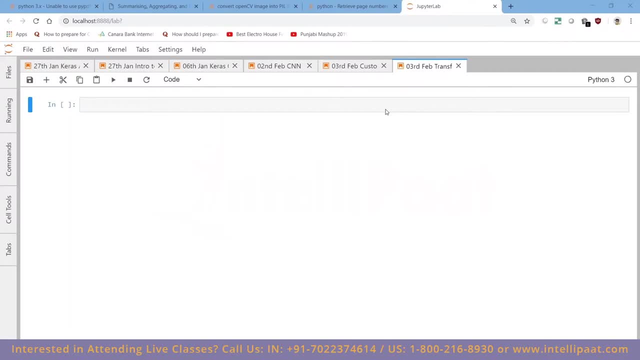 world now. if you are working in world now, if you are working in computer vision, you should have heard computer vision, you should have heard computer vision. you should have heard this name like multiple times, not from this name, like multiple times, not from this name, like multiple times, not from me, but from the world. also enter. 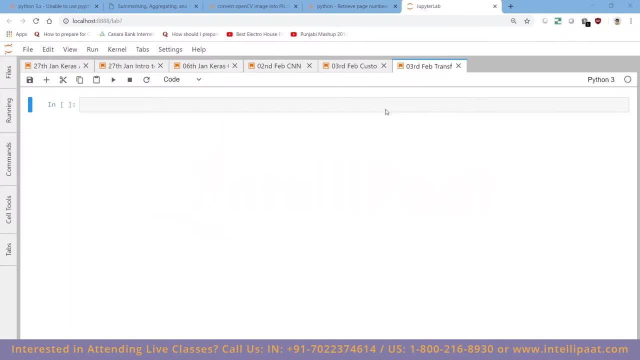 me, but from the world also enter me, but from the world also enter karpati. so he just said one thing: you karpati. so he just said one thing: you karpati. so he just said one thing: you know, you don't try to be an hero now. 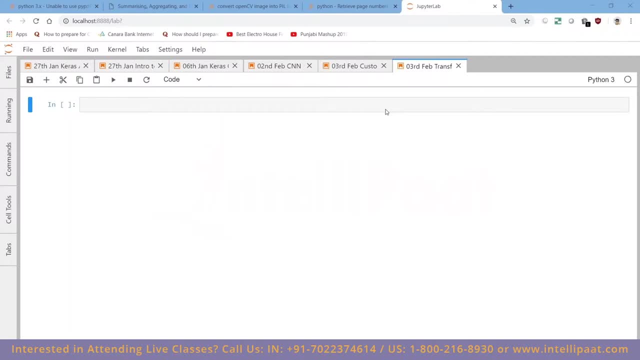 know you don't try to be an hero now. know you don't try to be an hero now. what does it mean? means that let's say: what does it mean? means that let's say: what does it mean? means that let's say that you're working for a client problem. 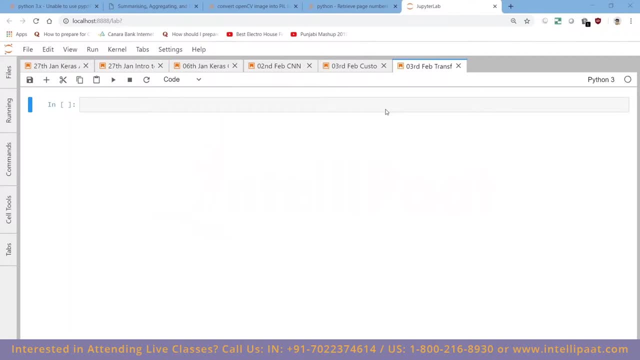 that you're working for a client problem, that you're working for a client problem which has very less data. now one thing which has very less data. now, one thing which has very less data. now, one thing is that you can learn everything from. is that you can learn everything from. 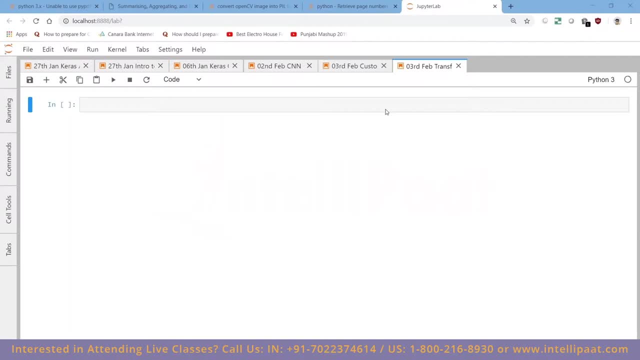 is that you can learn everything from scratch for the model. so there he says scratch for the model. so there he says scratch for the model. so there he says that do not try to be a hero if there that do not try to be a hero if there. 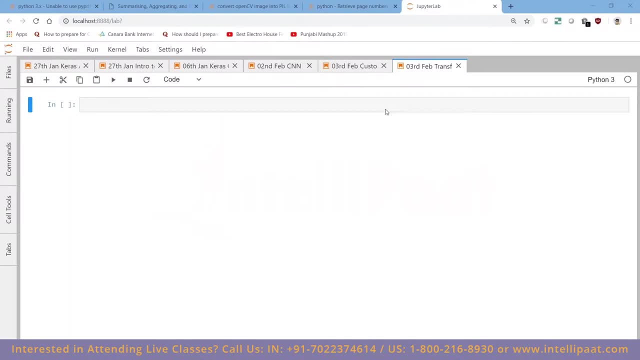 that. do not try to be a hero if there are things already made for you. do not. are things already made for you? do not. are things already made for you? do not. try to reinvent the wheel. this is what. try to reinvent the wheel. this is what. 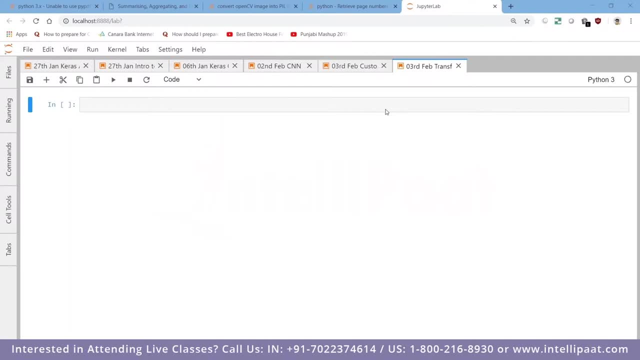 try to reinvent the wheel. this is what the concept of transfer learning is now. the concept of transfer learning is now. the concept of transfer learning is now. transfer learning says that. let's say: transfer learning says that. let's say: transfer learning says that. let's say that you have something already pre-built. 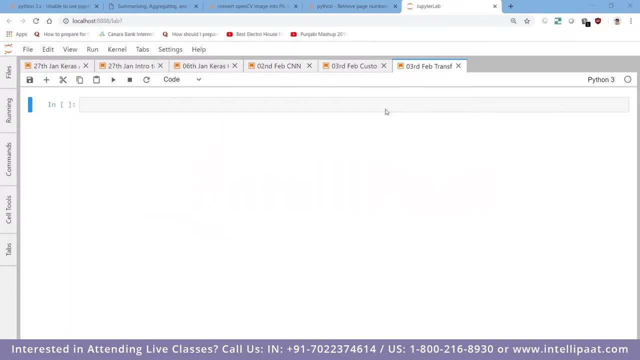 that you have something already pre-built, that you have something already pre-built. something has learned all the features. something has learned all the features. something has learned all the features already. and why are you trying to learn already? and why are you trying to learn already and why are you trying to learn this? so every year there is this. 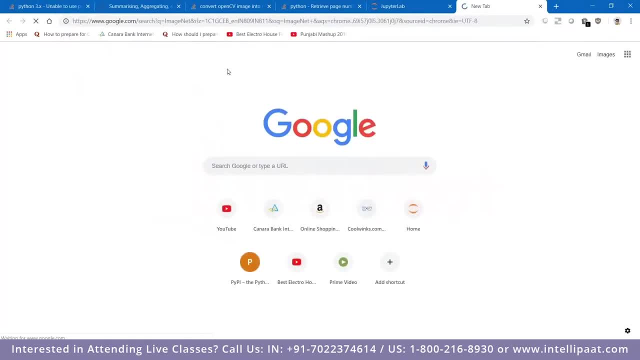 this. so every year there is this, this, so every year there is this competition that is called as the image competition, that is called as the image competition, that is called as the image net competition. you might have heard of net competition. you might have heard of net competition. you might have heard of this multiple times. so what? this image? 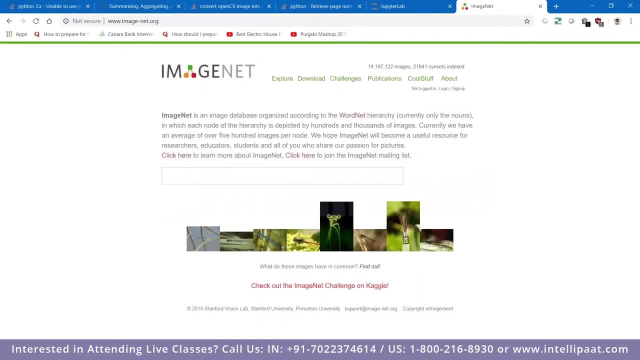 net competition. you might have heard of this multiple times. so what this image net competition. you might have heard of this multiple times. so what this image net is. i would definitely encourage net is. i would definitely encourage net is. i would definitely encourage you all to also access this thing. this. 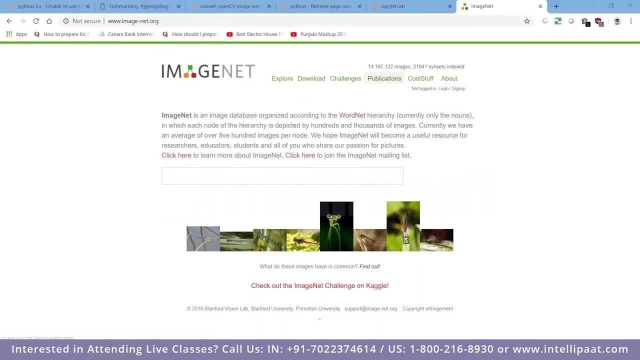 you all to also access this thing, this, you all to also access this thing, this image net. i can give you the url in the image net. i can give you the url in the image net. i can give you the url in the chart. this is actually a data set of one. 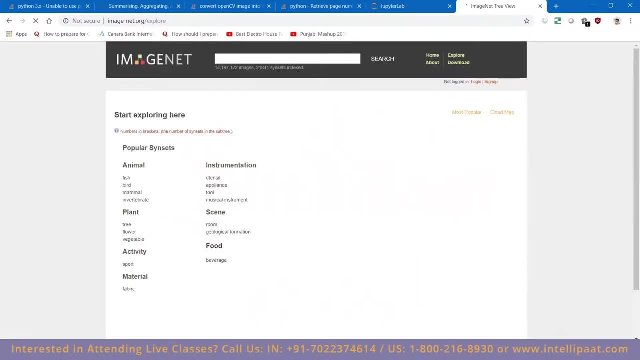 chart. this is actually a data set of one chart. this is actually a data set of one million images, million images, million images in thousand categories. now they have in thousand categories. now they have in thousand categories. now they have increased the images, they are increased the images, they are. 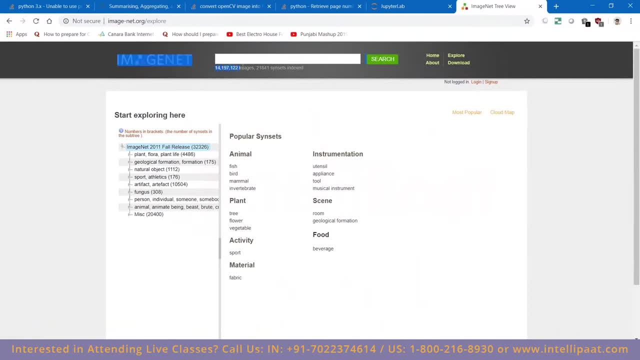 increased the images. they are more than like. oh yeah, they say they more than like. oh yeah, they say they more than like. oh yeah, they say they have 14 million images and 21 841 have 14 million images and 21 841 have 14 million images and 21 841. syntax means these are the different. 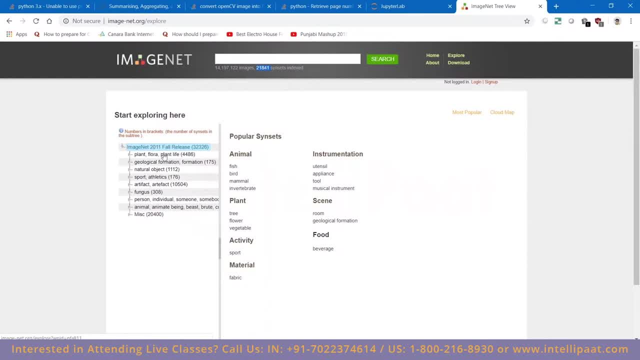 syntax means: these are the different syntax means. these are the different different categories. now the data set- different categories. now the data set different categories. now the data set that you are seeing is of 2011. that you are seeing is of 2011. that you are seeing is of 2011. here you can click on any of the 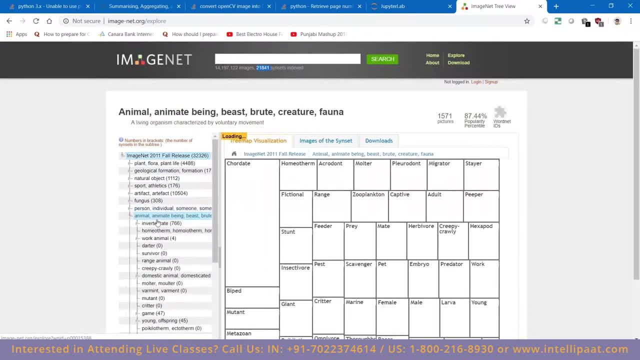 here you can click on any of the. here you can click on any of the particular category and it will take you particular category and it will take you particular category and it will take you sub categories and then sub more sub categories and then sub more sub categories and then sub more categories. so you can see if i click on. 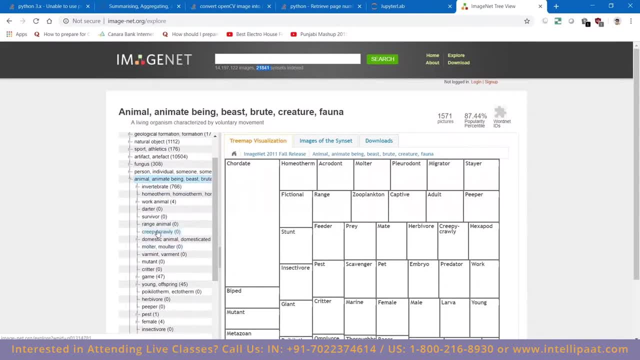 categories. so you can see if i click on categories. so you can see if i click on animals. i have these ranges, creepy animals. i have these ranges, creepy animals. i have these ranges creepy crawling, crawling, crawling. they are like multiples, like games. they are like multiples like games. 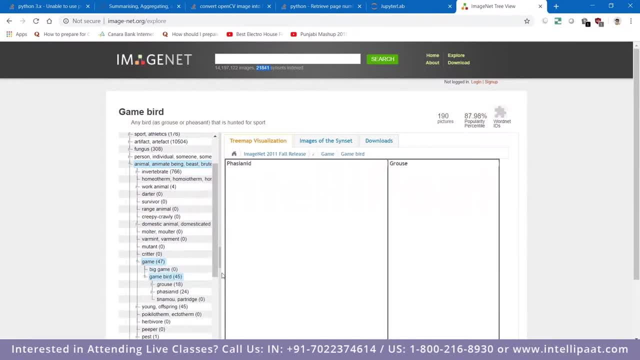 they are like multiples, like games, animal games. you have game birds there, animal games, you have game birds there, animal games. you have game birds. there are multiple uh subcategories also. you are multiple uh subcategories also. you are multiple uh subcategories also. you can, can, can. you can view these things, so you can. 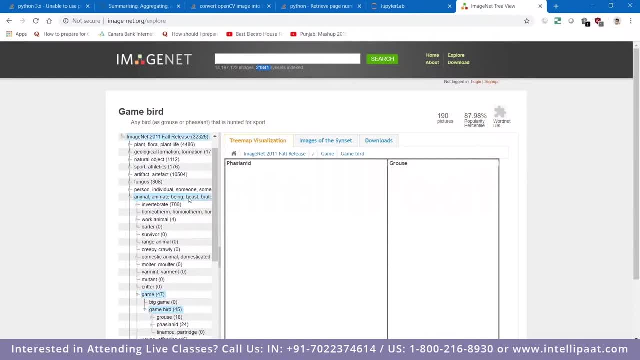 you can view these things, so you can. you can view these things so you can imagine what kind of a diverse data. imagine what kind of a diverse data. imagine what kind of a diverse data: character right from ranging from animals. character right from ranging from animals. character right from ranging from animals to fungus. 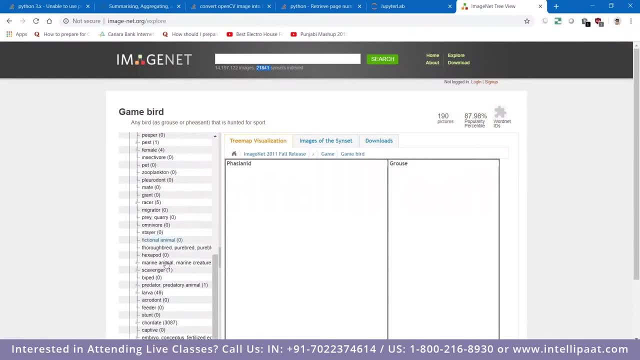 to fungus. to fungus. natural objects- plants- geographical natural objects- plants. geographical natural objects- plants- geographical formation formations, formation formations, formation formations, larva. you can have images for larva larva. you can have images for larva larva. you can have images for larva also, so you can have a. 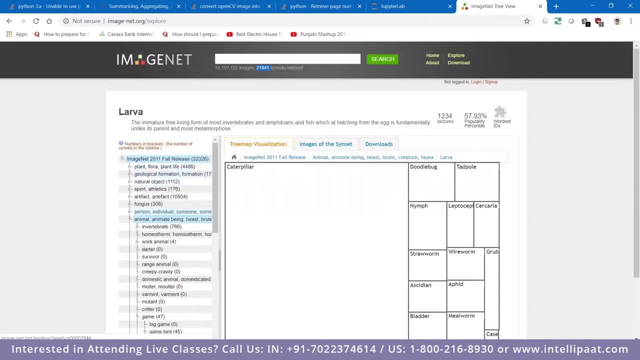 also, so you can have a also, so you can have a. a very diverse category inside this earlier, a very diverse category inside this earlier, a very diverse category inside this earlier it used to have it used to have it used to have. so you can see, even for like when i 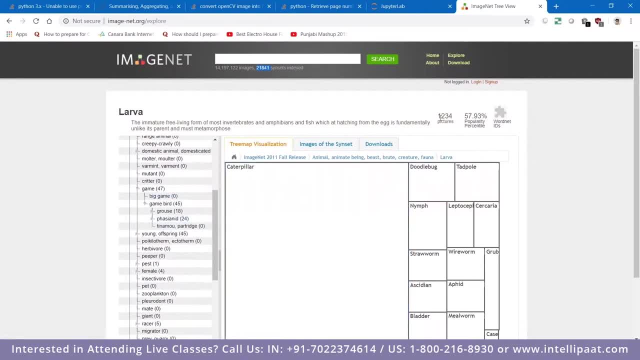 so you can see, even for like when i- so you can see, even for like when i- clicked on this thing called, clicked on this thing called. clicked on this thing called. this is actually larva larva, maybe you. this is actually larva larva, maybe you. 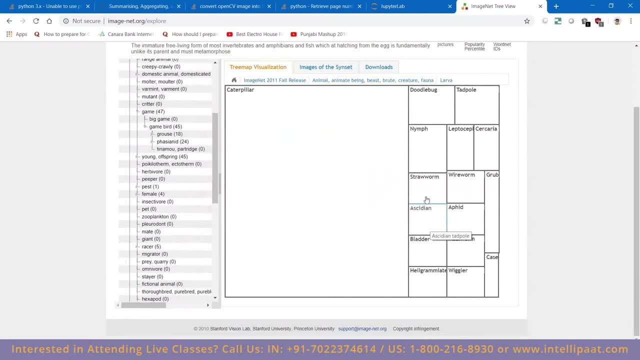 this is actually larva, larva. maybe you have one, two, three, four images. have one, two, three, four images. have one, two, three, four images. you can further go inside this thing larva. you can further go inside this thing larva. you can further go inside this thing larva also. then you can have like tadpoles. 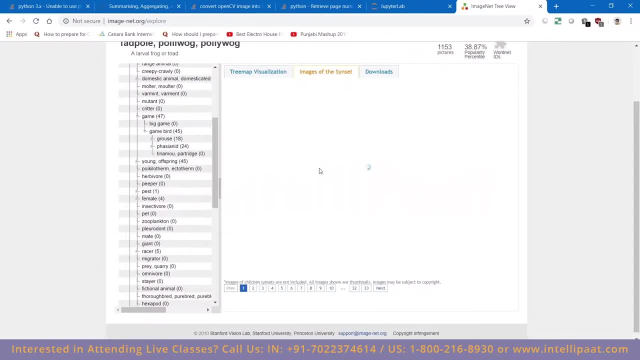 also, then you can have like tadpoles also, then you can have like tadpoles, let's click on tadpoles, tadpoles. when let's click on tadpoles, tadpoles, when let's click on tadpoles, tadpoles. when you have one, one, five, three images. so 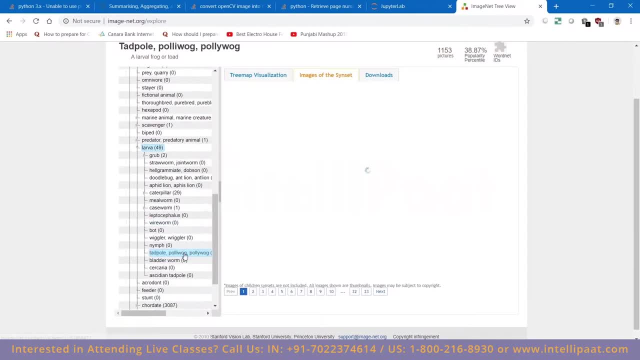 you have one, one, five, three images. so you have one, one, five, three images. so it's like a. it's like a, it's like a moving inside thing when i click on moving inside thing, when i click on moving inside thing, when i click on tadpoles. tadpoles means you have like. 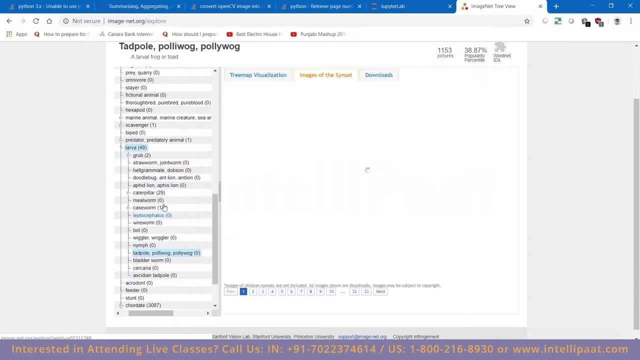 tadpoles. tadpoles means you have like tadpoles, tadpoles means you have like zero subcategories inside this. so the zero subcategories inside this, so the zero subcategories inside this. so the number zero here it means that number zero here it means that. 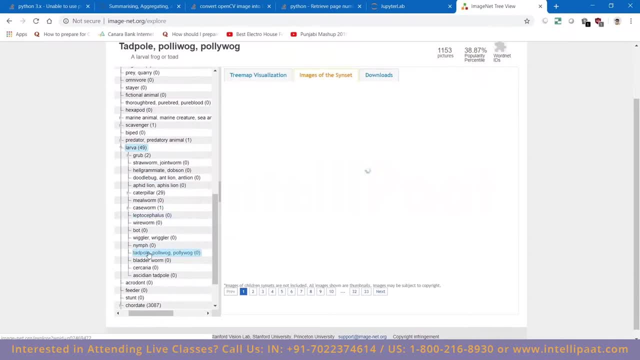 number zero here. it means that: how many subcategories does it contain? how many subcategories does it contain? how many subcategories does it contain? or is it the last child, so tadpole is? or is it the last child? so tadpole is? or is it the last child? so tadpole is the last chance? it has no subcategory. 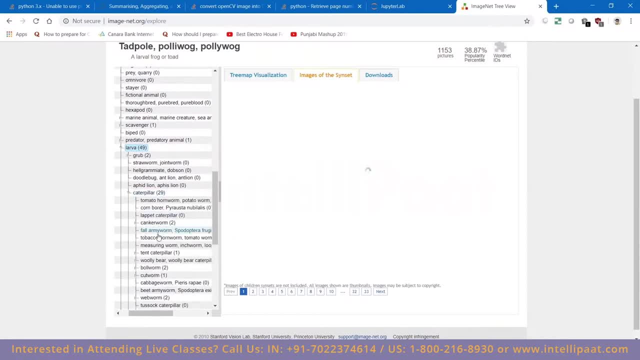 the last chance. it has no subcategory. the last chance: it has no subcategory. but if you go for caterpillar it has 29, but if you go for caterpillar it has 29. but if you go for caterpillar it has 29 more subcategories inside it and kenner. 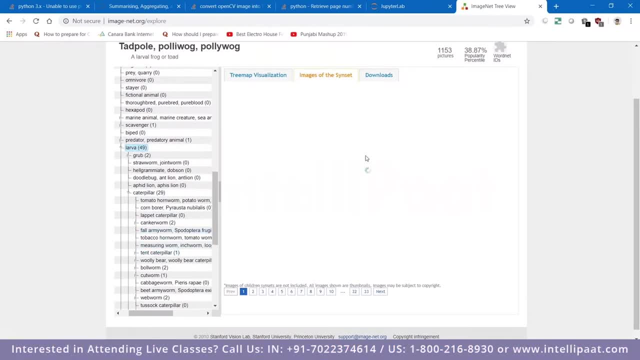 more subcategories inside it and kenner more subcategories inside it and kenner worm has more, another more. two worm has more, another more. two worm has more, another more. two categories, categories, categories. my internet sucks otherwise it would my internet sucks otherwise it would. my internet sucks otherwise it would have opened. you can go for the tree view. 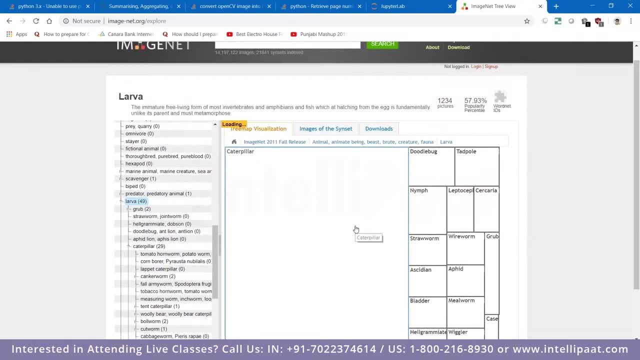 have opened, you can go for the tree view. have opened, you can go for the tree view. okay, if i click on larva here, you can. okay, if i click on larva here, you can. okay, if i click on larva here, you can have the tree view of this whole thing. 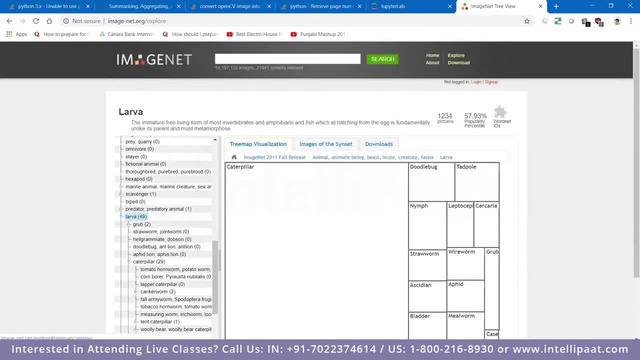 have the tree view of this whole thing, have the tree view of this whole thing. you can download them also download, but you can download them, also download, but you can download them also download. but this is like a, this is like a. this is like a. download is only available if you, uh, if. download is only available if you uh, if download is only available if you uh. if you like one by one image, it's not you like one by one image. it's not you like one by one image. it's not available like a bulk image of all the. 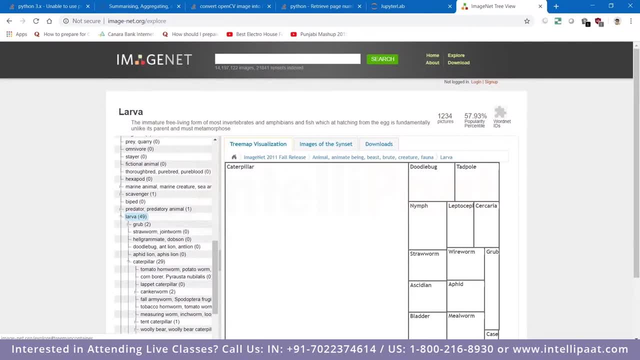 available like a bulk image of all the available, like a bulk image of all the things. to download the data set for things. to download the data set for things. to download the data set for image net, you have to be from some image net, you have to be from some. 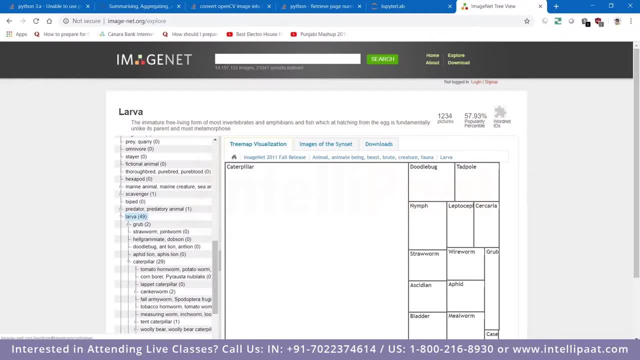 image net. you have to be from some academy, academy, academy, and you have to provide them some. and you have to provide them some and you have to provide them some proofs. then they give you the download proofs, then they give you the download proofs, then they give you the download link. for that also, you can download the. 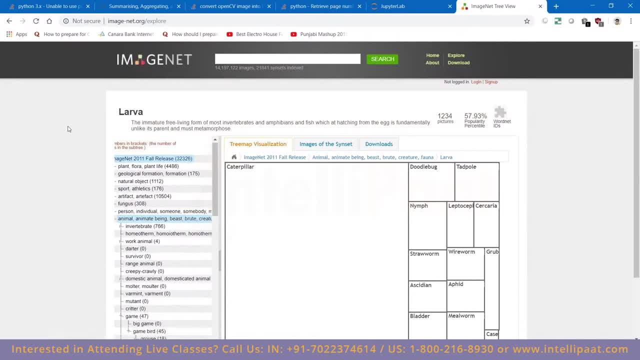 link for that also. you can download the link for that also. you can download the things from here now every year. they things from here now every year, they things from here now every year. they have this, you know, have this, you know, have this, you know things out here and there are like major 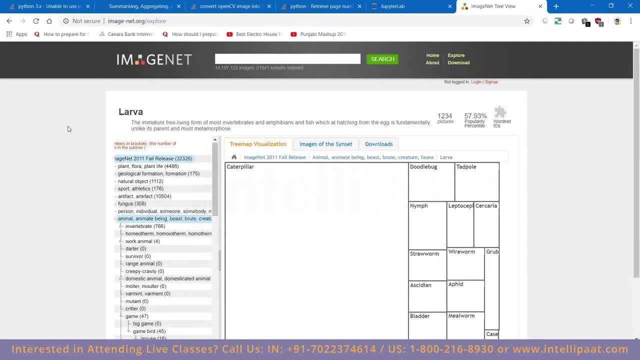 things out here and there are like major competition is being held on this- that if you can train your model, now, when these models are trained on data like this, now just imagine how diverse the data sets become right. they learn multiple things, not only just cat and dog features like how it is or how is that, but buildings. 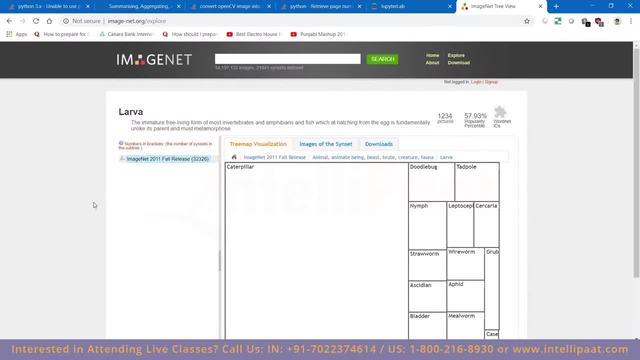 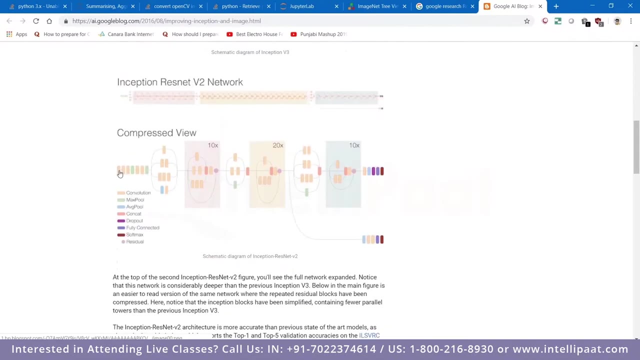 airplanes, vehicles, mobiles, microwaves. so they're learning almost everything, almost everything. so they are learning edges and functions for everything. now, in this paper, now they are telling that what are the things that they are learning inside this thing? so they are telling you that you know, this slight yellow part is actually the convolution, the green one is the. 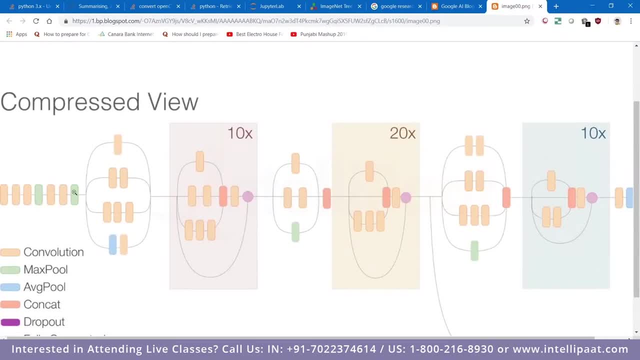 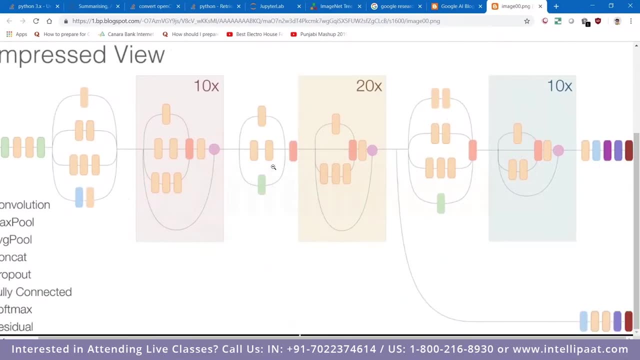 max pool. so you can see there are three convolutions, three conversions then a max pool, three: two convolution then a max pool, then they have a ring of convolution. blues are average pool. so this is how they describe their model right and if you go there they have provided the weights also for this. 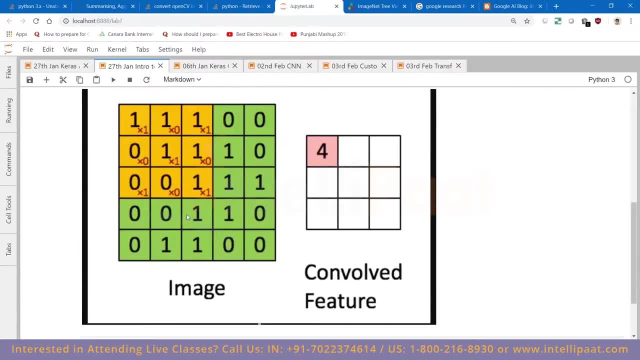 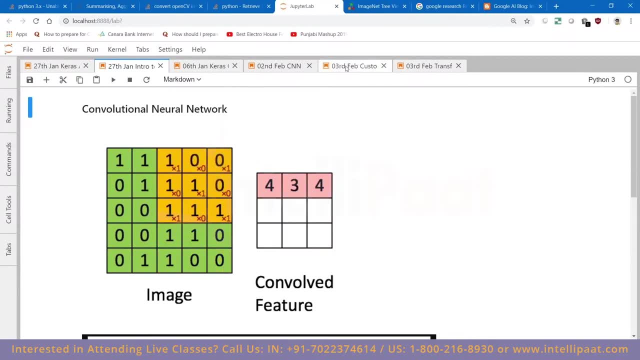 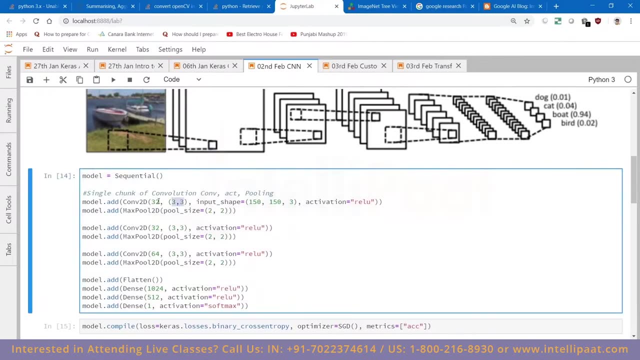 so when this filter, this orange filter, whenever this orange filter is moving, we didn't knew the values of this orange filter right. we randomly took the values of this kernel feature right. so when you were making your own, this convolution, and you said that you want to have a size of 3, cross 3 and you want to have 32 different kinds of these small yellow, these yellow, 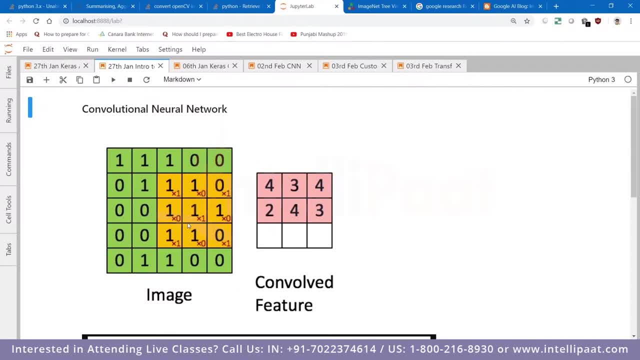 metrics. now, what was the value that was initially taken? it was random values, right, but when your model started training itself forward, backward, forward backward to minimize the error, it certainly came out of the box. so that's how you know that this filter is moving. so that's how you know that. 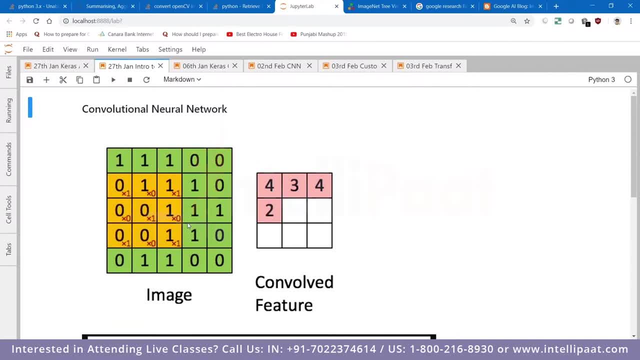 this filter is moving. so that's how you know that this filter is moving, so that's how you know that- to a point where it has optimized the value of this orange filter that is moving right. and these are the optimized value that are saved and called as the weights of the model, and you know what every 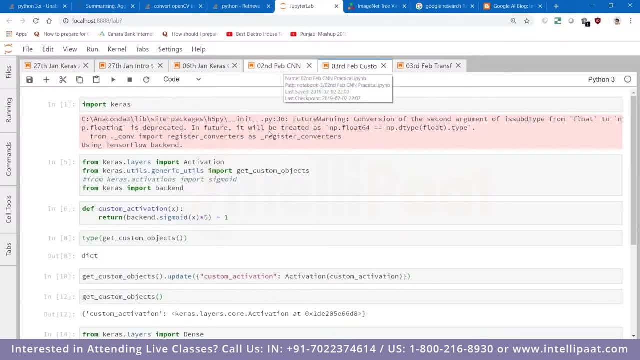 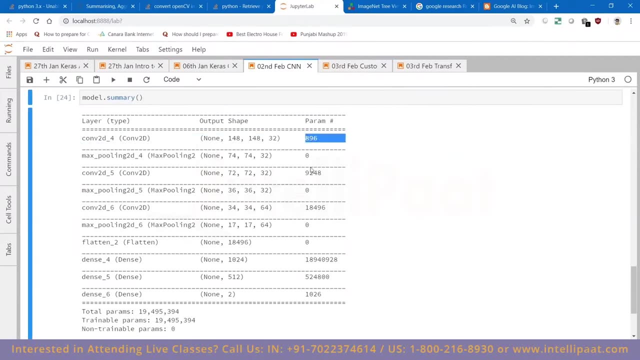 time we do this thing, every every time we do this thing called model dot summary, it tells you this thing: that it, at this particular layer, you had 896 values that are to be saved at this particular day. if you have 9 000 values to be saved at this particular layer, you have 18 000 values, and then 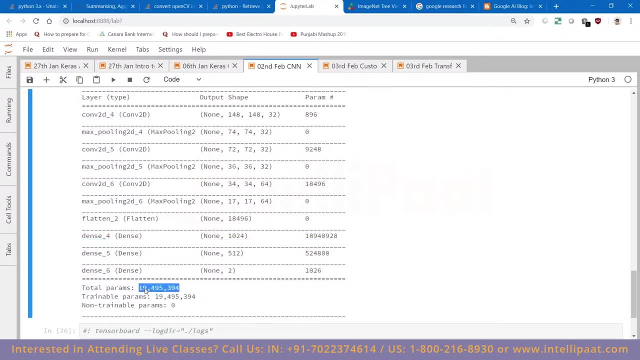 you have similarly these values and then you add up. these are called total trainable parameters. these 19 million parameters are actually saved inside your modelsave bit. so just imagine deep learning. what it is doing is, let's say: this is your input, this is your input image. let's say that: 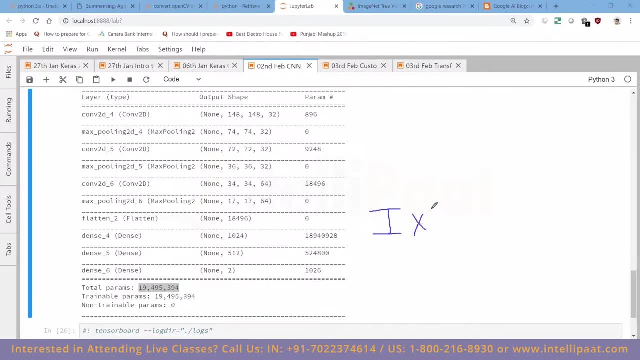 this is a simple operation, that you have to multiply it with something called, let's say, alpha, and then your answer will be output, right, so you have to convert your input to output, and then you don't know the value of this alpha. so what you do? you do a deep learning training and you want to 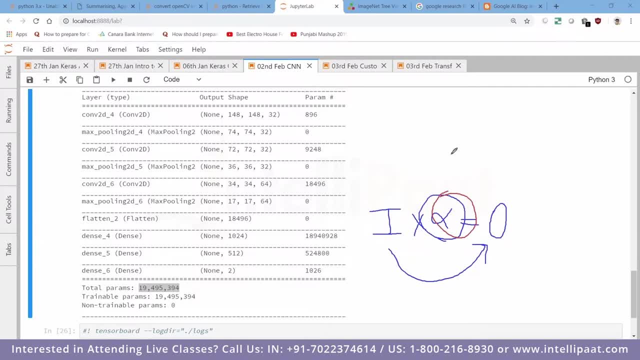 calculate the value, you learn the value of alpha. now you have the value of alpha, you save this value of alpha whenever someone gives you the input. you are going to simply do a multiplication and then you get the output right. so this alpha thing is actually these 19 000 uh parameters. 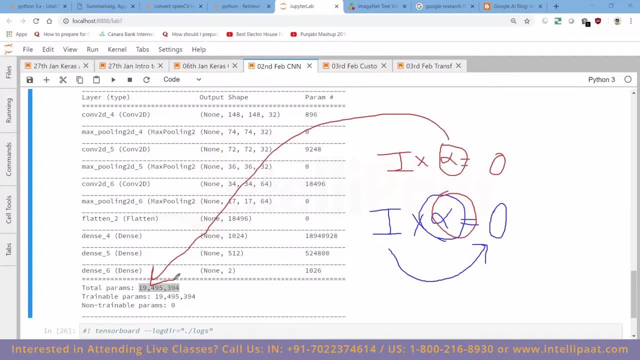 did that make sense to you? simply right? this is what we do in machine learning also and deep learning also. what we're trying to do is- it's a simple equation- that you have to do some or the other operation with the input to produce the output. now i am just simply saying: 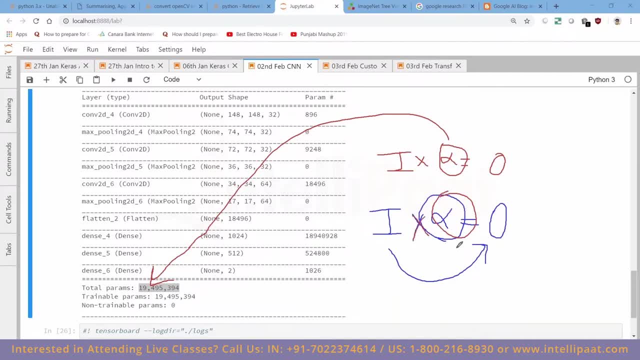 this is a multiplication, but no, it's not multiplication. it's like a very complex thing. but just to simplify this thing, let's say that there is some kind of a relationship, some kind of a function, with some kind of a function with input, so you have some kind of an input function, for i 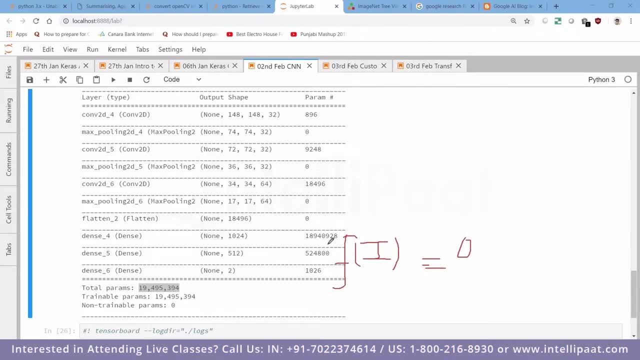 that is giving you the output. now you have to find this function. only this is your only job, that you have to find that. what is this function? once you have this function, next time, whenever you input, you just pass it into this function and then you will get the output right. this is what is. 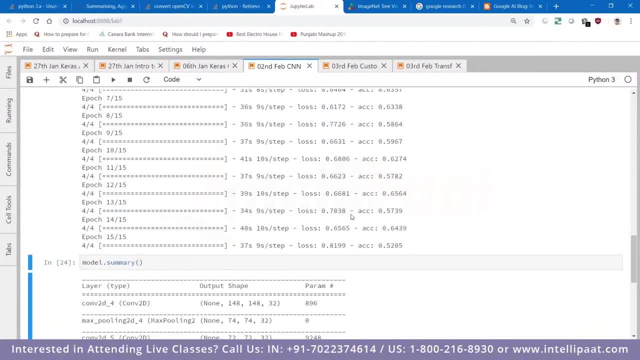 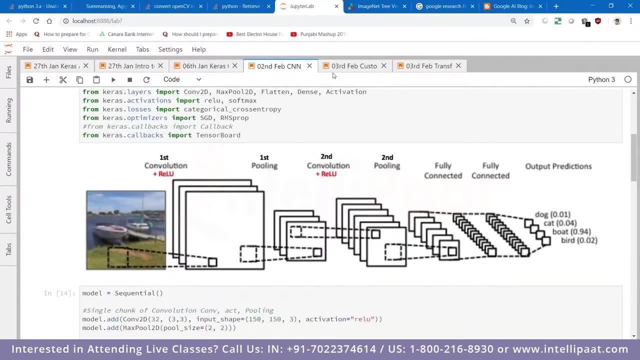 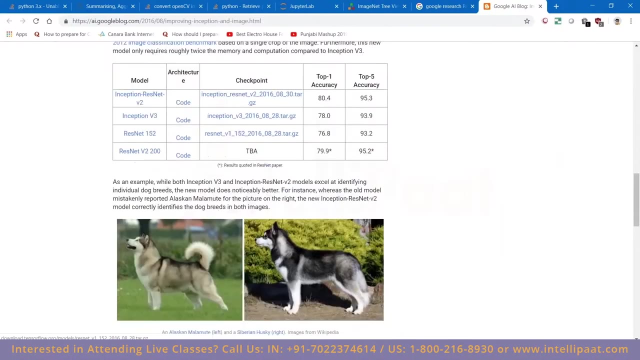 called as the weights of the weights of the model, nothing but the optimized value of all these 32, 64, 32, 64 combinations. this was all about weights and all. so these are all the values that are saved in your weights, right? so this is, uh, so what they do. they give you, they will give you the code also. 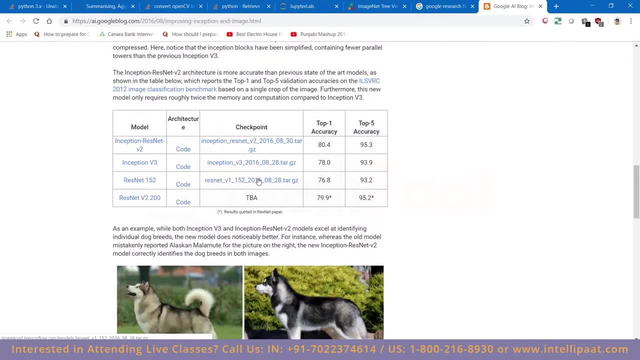 and then they will give you the uh weight also. so when they are giving you the weight, it means that they have given you everything. they you have now the trained values of those things, of which things, these things, these convolution that are here, these convolution, now you don't. 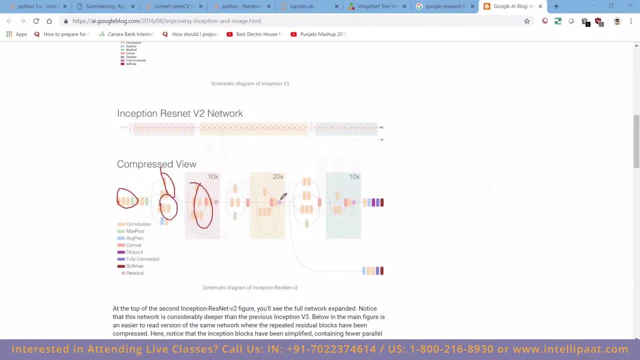 have to train to get the values. you already have the optimized value for all these convolutions, right, all these convolutions? you have the exact optimized value, so you don't have to train them when, when they give you the value, your model is, like, already filled up with the optimized number. 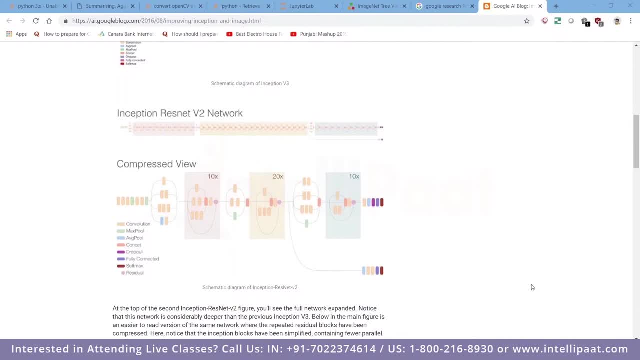 now, if i say, in theoretical terms, what it is happening is, let's say that you have this thing already in your uh. if i tell you what it is actually, uh, so, this was a mathematical thing, right? so what is happening is that, uh, your model has, let's say that you, you just copy pasted this. 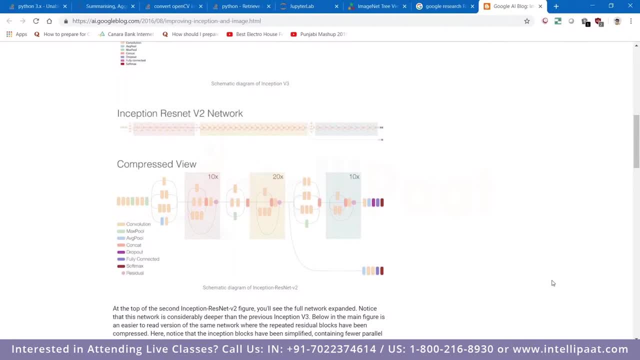 particular model and then in the end, rather than in the end. so see, if i am saying that this uh resnet was trained for thousand classes, can anybody tell me what will be the last of the dense layer? this last dense layer will give you how many probability if i say that there are thousand categories on which this, this resnet model. 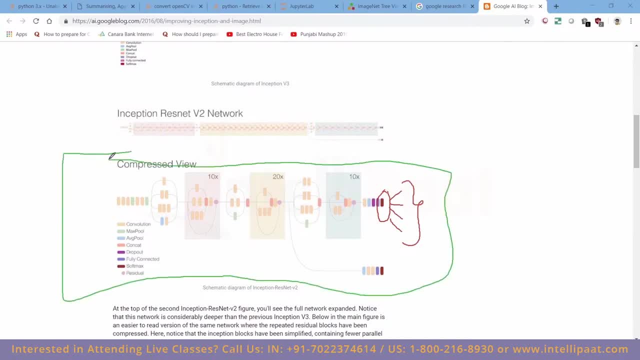 is trained. there are thousand categories on which this model is trained. what will be the number of dense layer at the end? what will be the value of the dense layer at the end? thousand only because you want to have variability for each class. right, you want to use this particular model only, but you 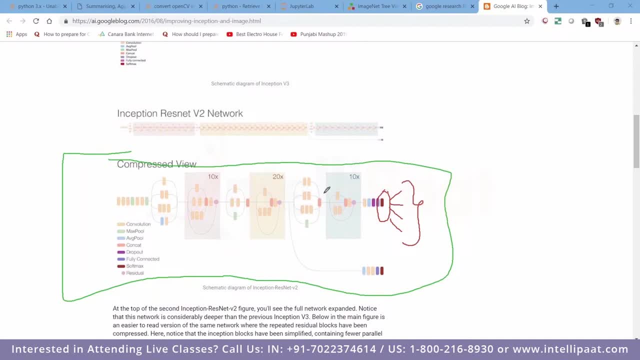 want to use your cat dog image data set. now, you cannot have these thousand layers at the end, right? you need to convert this thousand to two, or what thousand will be home? you have to cross this thousand. you have to cross this thousand and make it to two, only right. so now this is something that is called. 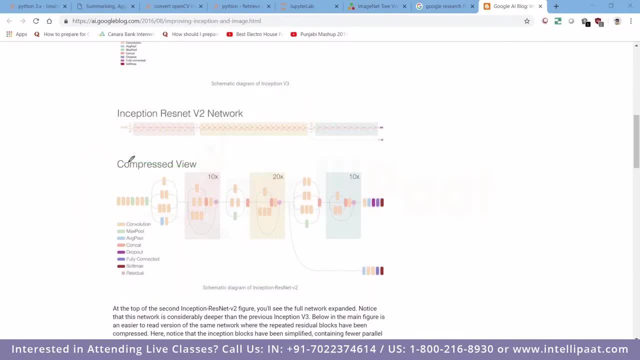 transfer learning. now what is happening is that you have every. you have this structure already. you have this structure net already made. let's call this as net, this thing as net and the weights as the weight. you already know, right. so what are what we are doing is that we already have a model. 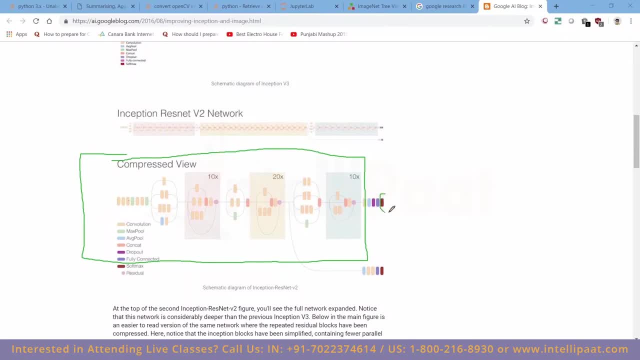 we already have a net prepared with us. thing that we have to do is that we have to remove this last layer, remove the thousand and put the two layer model there correct. and because we have the weights already filled in them, we have all the weights filled in them. so what we will do, we will not run the model, we will not back. 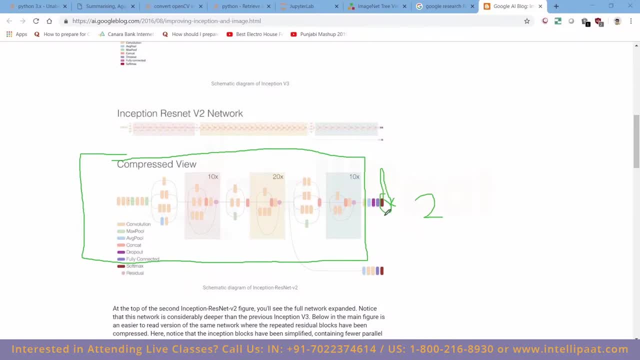 propagate everything like back and forth, back and forth. what we will do is we will just run the last layer, we will just run the last layer to be trained, because everything is already trained right, these layers are already trained. they are like super best layers in their nature. 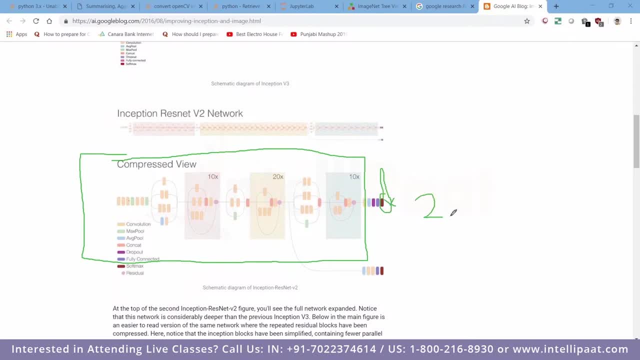 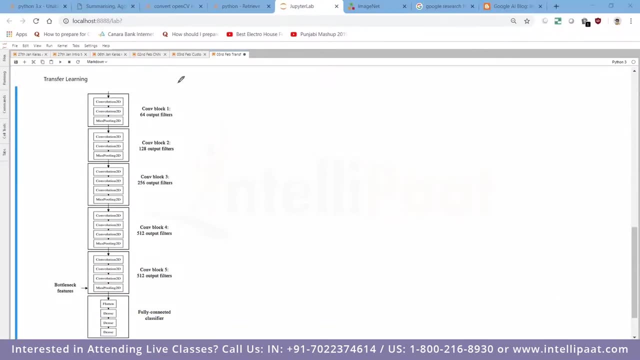 what you have just doing is you're just removing the thousand layer, putting a two layer and then training this layer transfer learning way. what you are doing is this is your vgg, uh, vgg- model, right? so it is saying: do not touch this green part, let it is as it is, just train your this part. lower part. 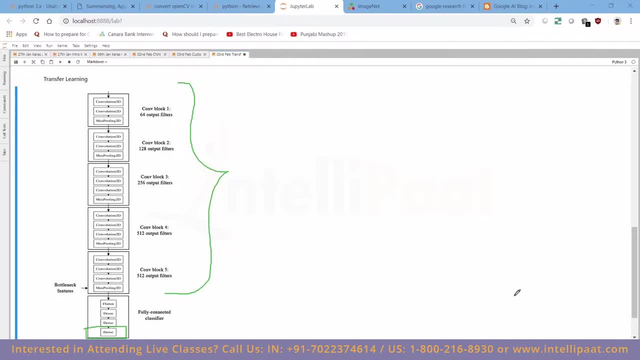 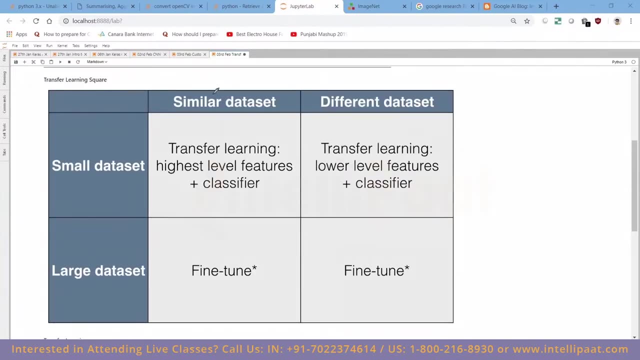 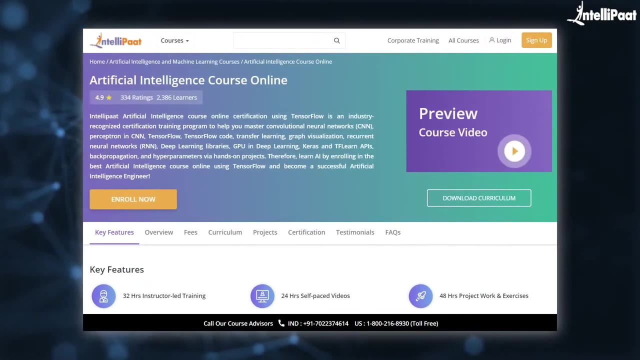 dense layer part and then change it from thousand to two. right, that's it. now let's come to the second example, where let's say you have a very similar data set and you have a large data set also. just a quick info, guys: intellipaat provides artificial intelligence online training, mentored. 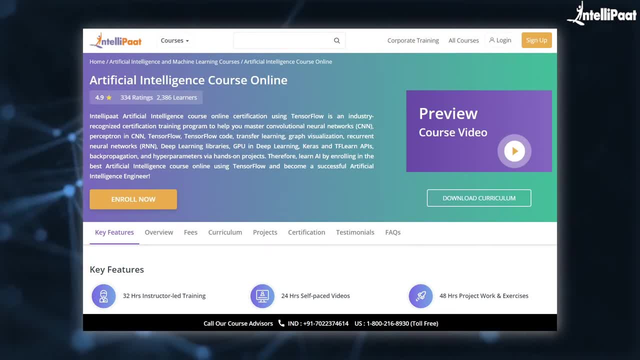 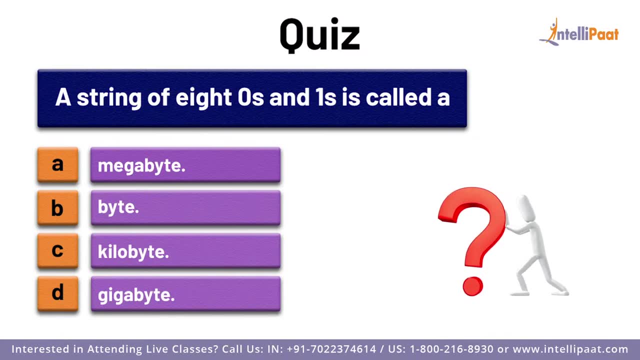 by industry experts, the course link of which is given in the description below. now let's continue with the session. test your knowledge of computers vision by answering this question. a string of eight zeros and ones is called what? a megabyte b, byte c, kilobyte d, gigabyte? comment your answer in the comment section below. 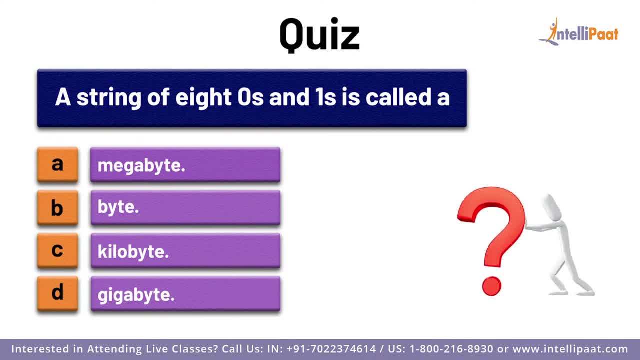 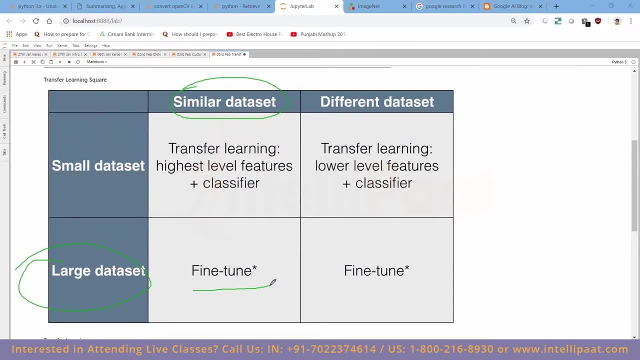 subscribe to intellipaat to know the right answer. now let's continue with the session. then you have to go with fine tune. fine tune, i'll. i'll explain you what this fine tune is, don't worry. so let's for for both the examples. if your data set is different or similar, you have to use fine tune. 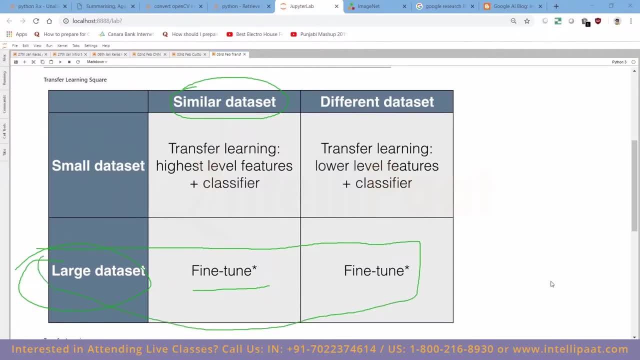 don't worry, i'll tell you fine tune also. but let's jump to the second second part that you are asking, right, that you are asking this right now, that let's say that data set is very different. it is not equal to, it is not equal to somewhat like, uh, somewhat like what you have seen. so what you want, 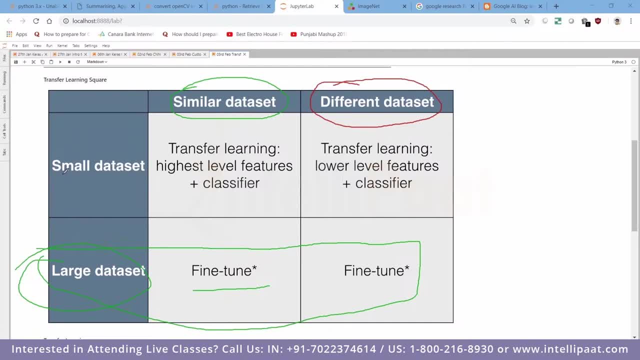 to get from your older model is, or from the vgg or resident. what you want is you just want a generic part right and all the generic information. you just want a generic part right and all the generic informations are present on the top layers on the this top list. this 64 con 128, convert to 56 count. 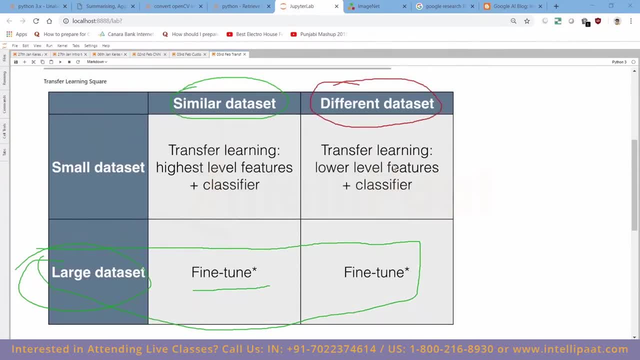 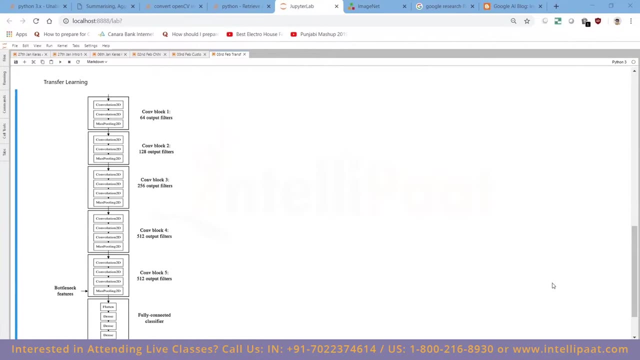 right. so what it is saying? it is saying that you use the transfer learning, that you use the transfer learning, but with low level features and classifiers. so what does this mean? now, this is saying you that please, please, go here and then freeze the model till here, or or, or at least. 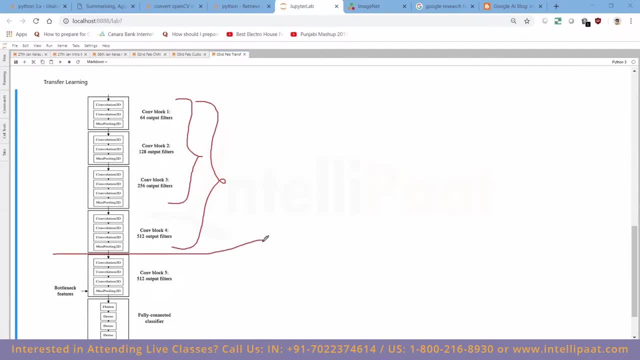 still here, but train your model below this, this line. so you are not only remodeling your classifier from 1000 to 2, but you're also training this last layer of convolution also. so these are different, different kinds of combinations: that where do you want to freeze your model and then where you want 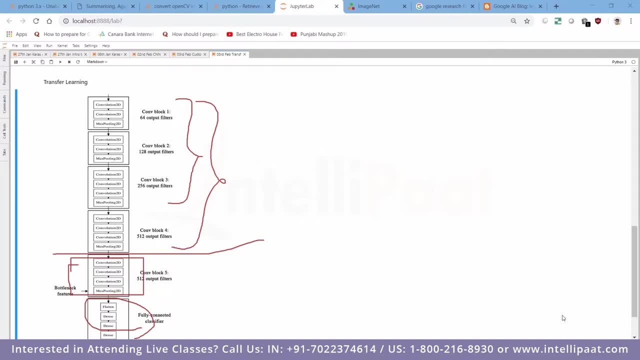 to retrain right and then, whenever you are trying to do this thing, whenever you are trying to, you know, uh, let's say, if i remove this thing, and let's say if i say: whenever you are trying to train something below this or below this, this thing is also called as fine tuning. this is the 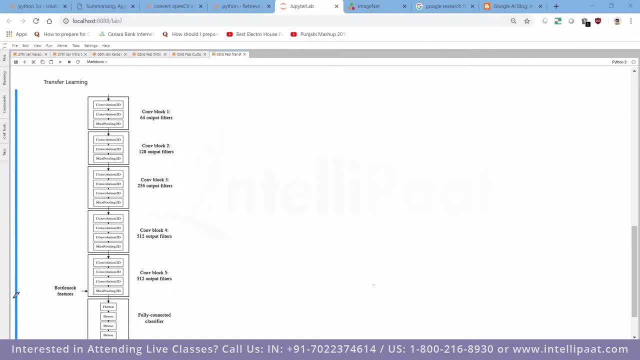 same thing. so if you are doing something that is below this line- below this line, this is this is somewhat like you're just changing the dense layer and the uh below something that is flattened. that is called uh transfer learning- if you are retraining your con blairs here or here, then 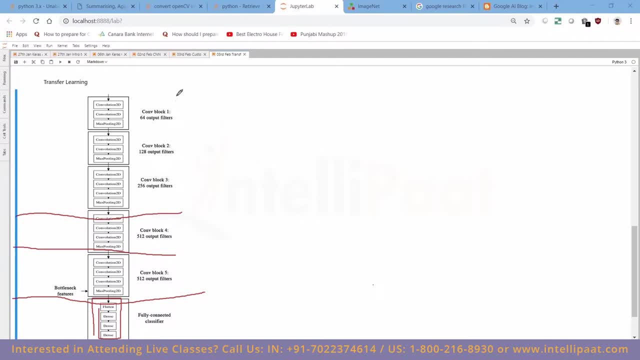 this is called fine tuning- nothing much fancy. so what you're trying to say- that you are trying to freeze your model till here- it means that you are not going to run the model till here. you are not. this part you're going to keep as it is, and then you're, you're going to train this section. 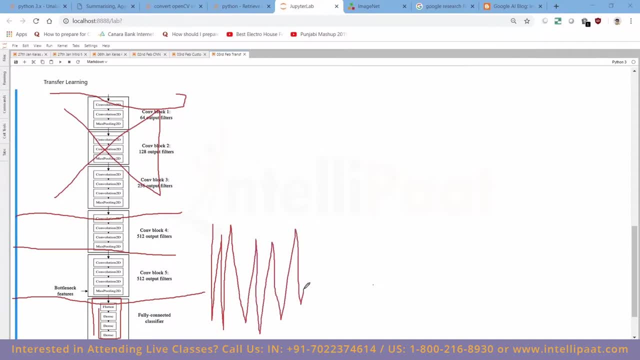 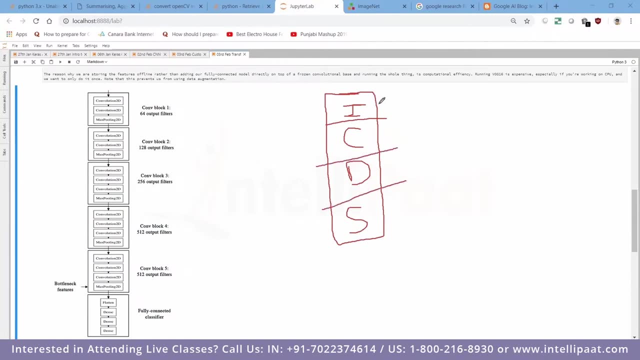 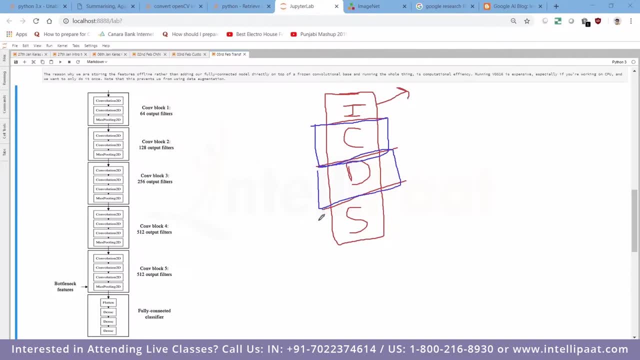 now, what i am trying to ask you to change is this softmax layer, and you have weights for all the things, right one, you agree with me, right, because we have weights for everything. now what i am trying to say is that please do not lower the weights for the last softmax layer. 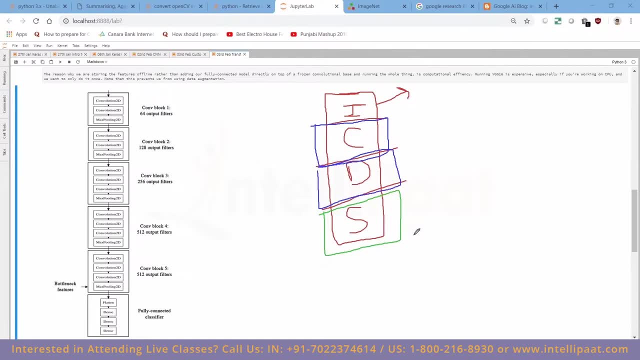 right and unfreeze this green layer and other, all these in the blue, let them freeze. when i say there, please do not lower the weights for the last softmax layer freeze, i am saying that all the forward and backward propagation is not going to happen there. right, the model is already. you know your, your model is already, you know it is. uh, it is having. 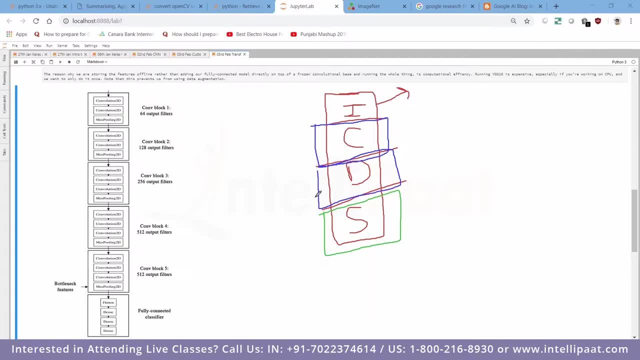 weights there and what you are trying to say is that you freeze the upper layer and you have unfreeze the lower layers and you will train them only. and this is how you will see now. now did you get the time? what i'm trying to say, the training, all the forward and backward propagation is going. 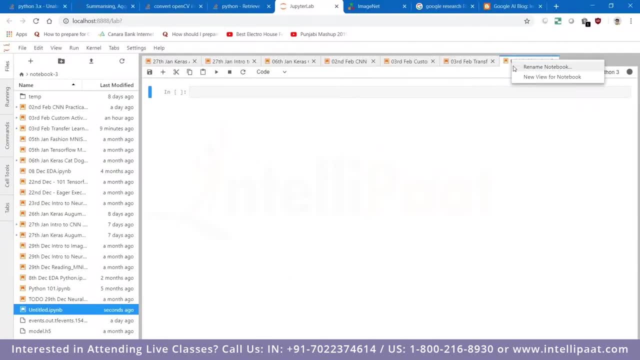 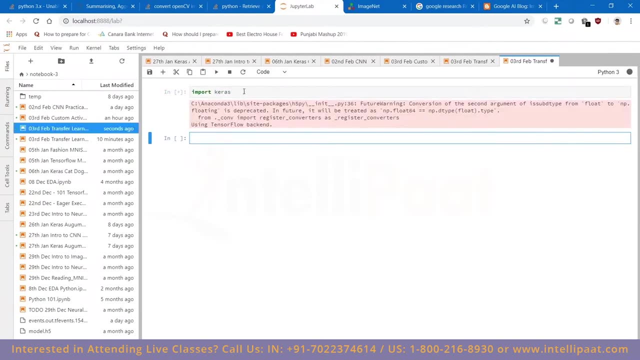 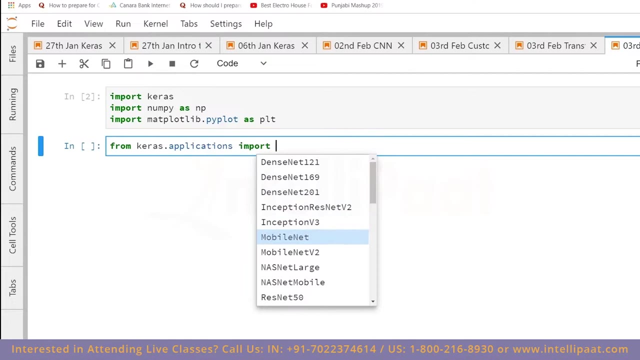 to happen till here only, and let's call it as article this time. let's do, and let me show you how to do the magic import. now you have multiple things: dense one, two, one. dense one six, nine. dense one, two, one. then inception, resnet, depending on the nature of intensity that you want. 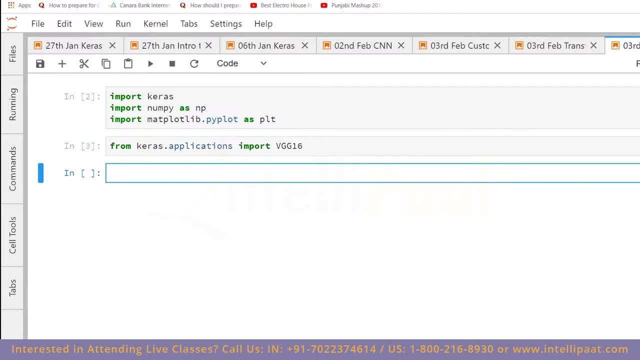 you can use, i love with you 16. this is a very small network, small in weights, because this is just a 16 layer. you can. you can just easily compare that we have done till now that if you go and see in this, uh, if you go in our class, only this. 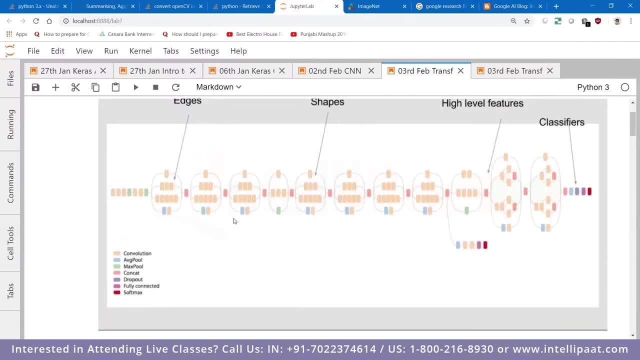 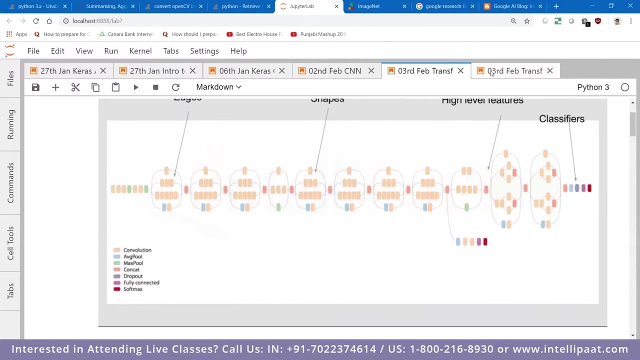 is the vgg. right, this is the vgg, but this one is resnet. now imagine the number of things going inside this thing. how many, uh, convolutions are there? one, two, three, four, five, and there are 100. so it's a resnet. there are two types of model. one is resonant- 51, another one is reset, 101. 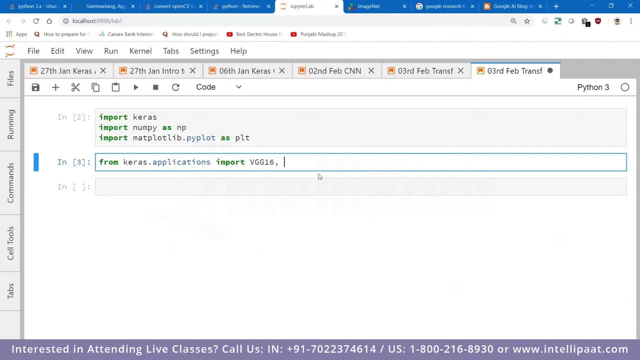 and i think both are inside now. resonance 50 is there only in this. inception has two. inception has version two and three both inside it. they are like literally heavy, and when i say heavy i mean very heavy. so what you can do is you can call your model. let's call it model vgg model. 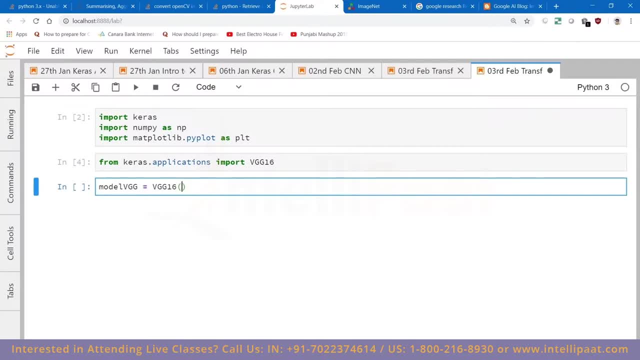 vgg is what vgg? and then you have to give your that you want to have now, depending on the thing. now, see, now, depending that you want to do the that you want to do the fine tuning or transfer learning, depending on that you have to. you have this option called including. 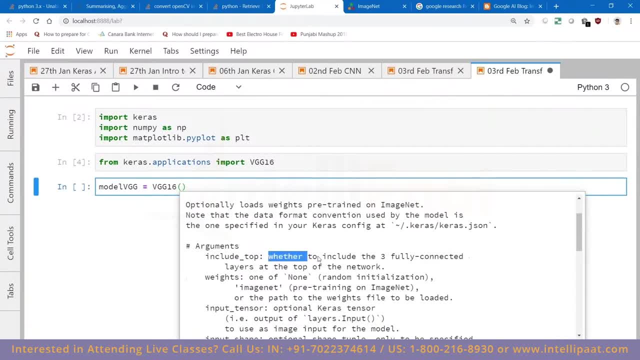 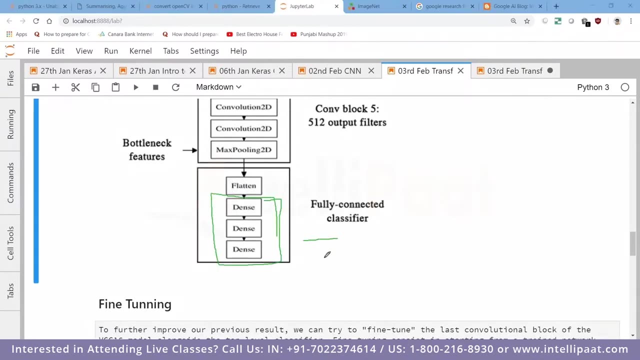 top. now, what does this include? top means whether to include the three fully connected layers at the top of the model. what are these three fully connected layers? these are the one that i was talking about, this thing, do you want these three? this is called the top part of the, so generally. 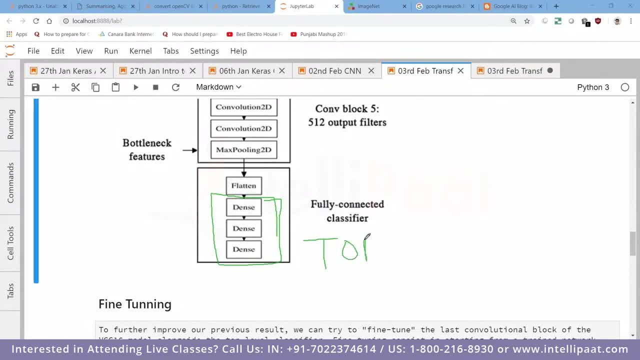 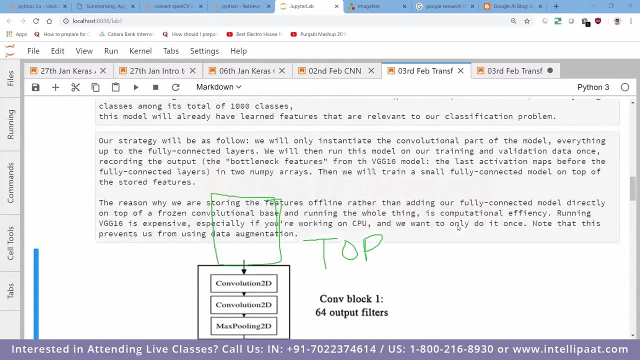 people get confused- i also, i- i was the first person who got confused in this thing also- that this is, this is the top, or or or this is the top, this convolution is the top, but but uh, kiras say this is the top part because this is giving you the output. so they say this is top. 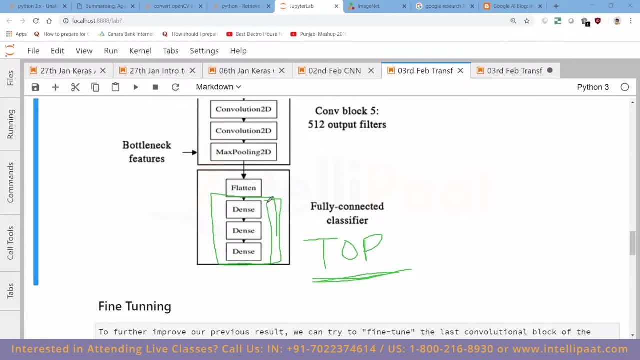 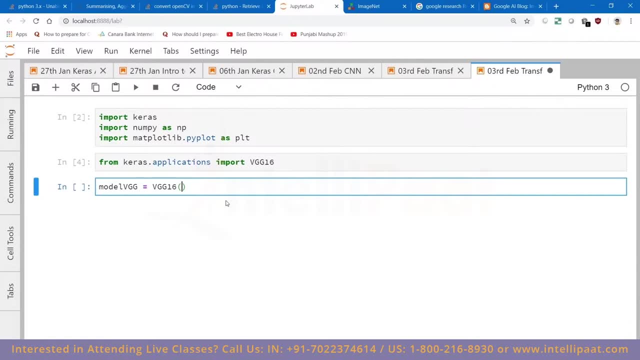 so, kiras, when it says include top, it means do you want to get these three dense layer output also right. so let's say that you want to get it or not. let's say, no, we don't want, we will, we will do it our own, we will make our own. uh, top three layers. right, then you have the second thing that is called 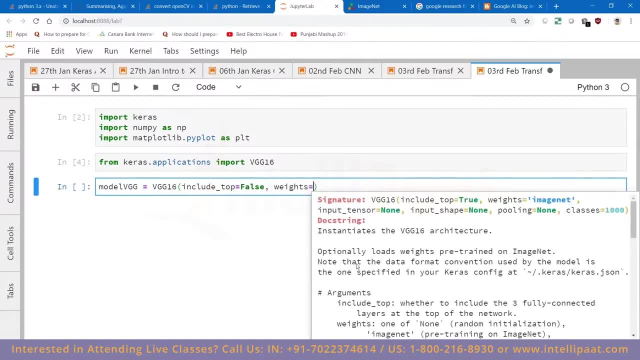 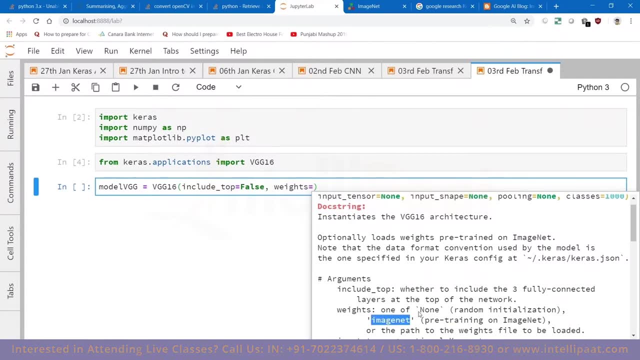 weights. now weights, which weights do you want to get? if you see it is one is called none, that is. or another one is the image net. if you see i've selected this one image net is the one that you will. that that is from the uh, this challenge, image net challenge, right? or if you have your, 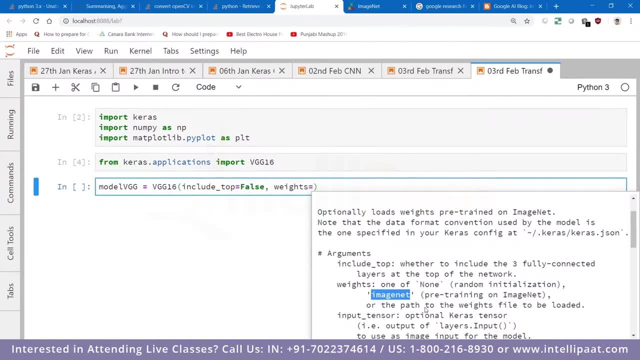 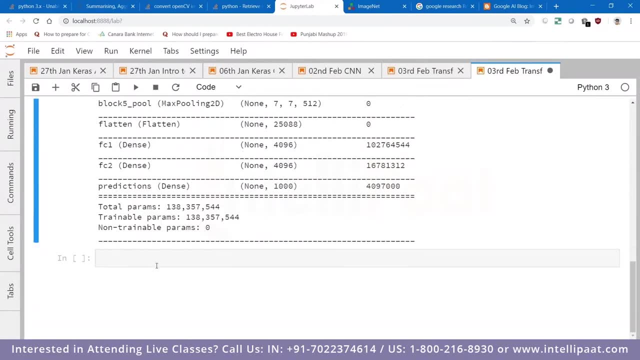 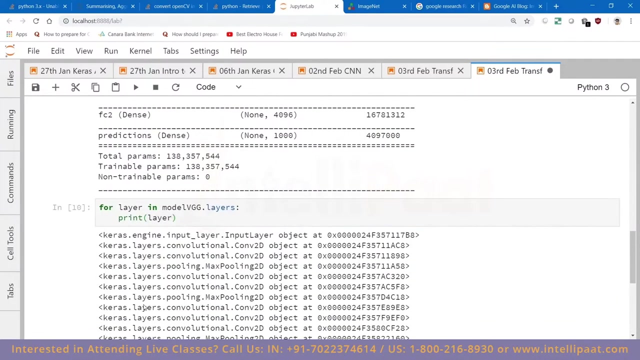 own custom weights also. you can give them here. right, let's say that we will train the top layer also. so what you can do is you can see here for i in for layer, in model vgg dot layers. you can see all the layers here, print layers. these are all the layers, layer dot trainable. it will give you. 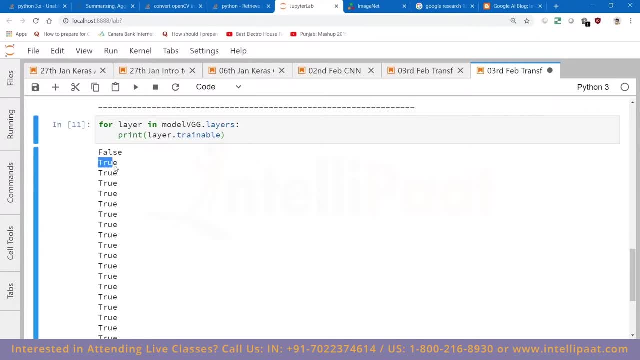 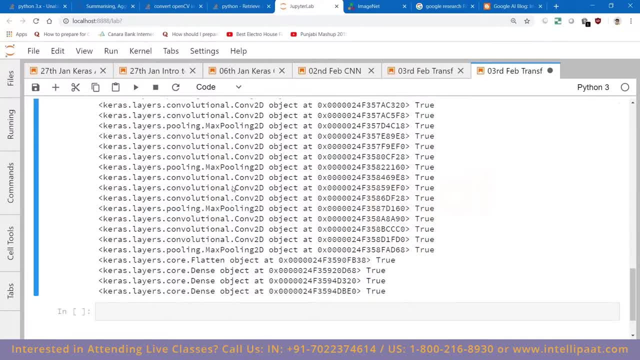 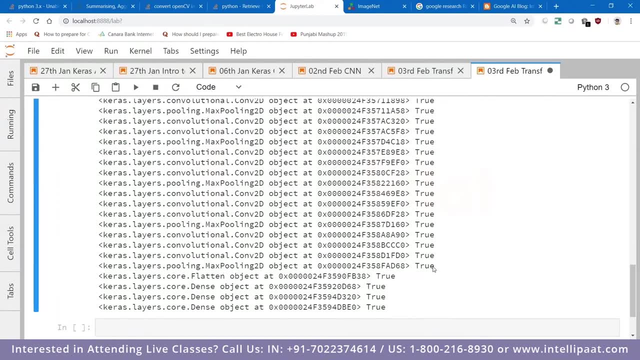 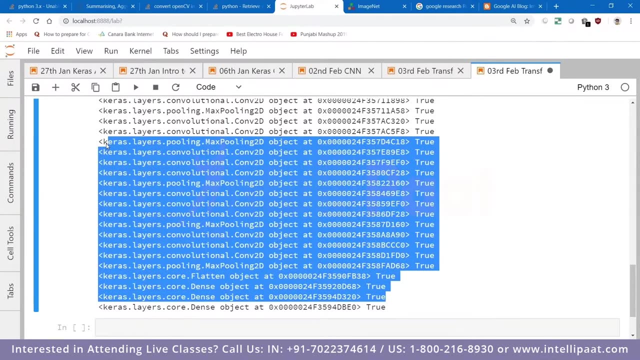 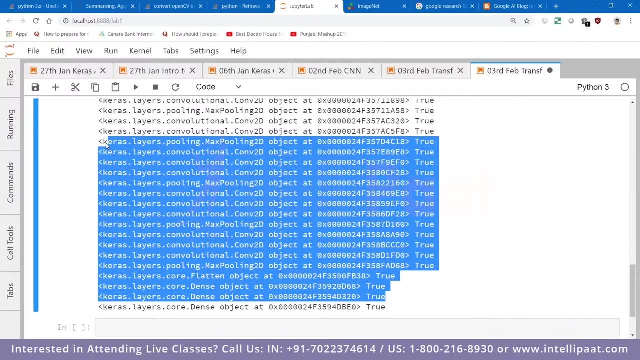 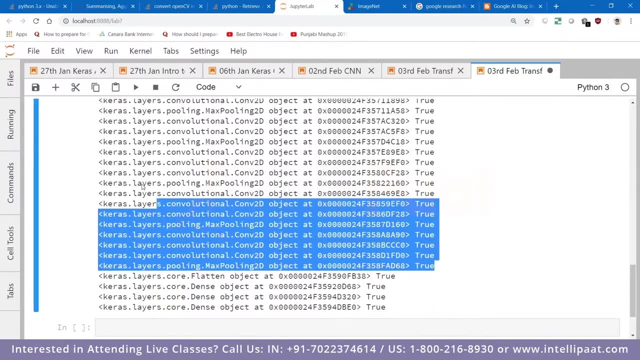 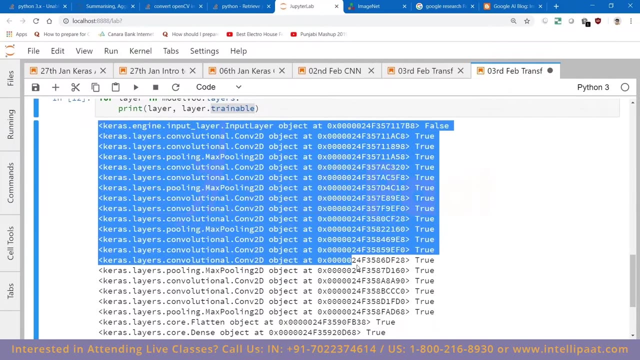 right, and then you can have your thing out. so let's say that we, we keep this till here, we keep this till here, and then we keep everything, and then we say that we don't want to train it till here. so if i get this number, this number should come out to be max. pool 2d is the last. 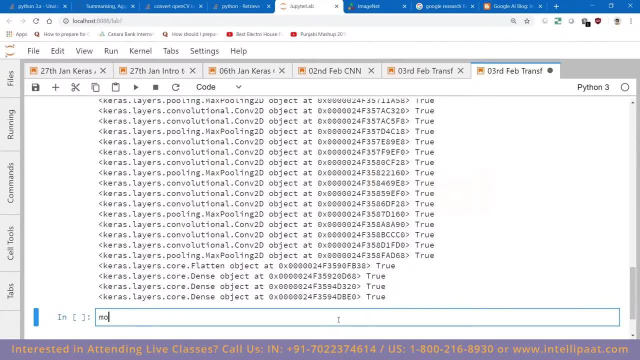 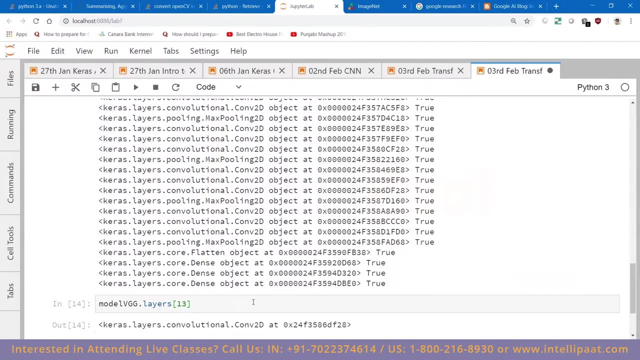 number. so layer model, ggg, dot layer, and this number should be 10th number. 10th number is what? uh, 160, no, it's still down. 13, 13, 13 is gone. 14, 160, no, 15, 15 is again gone to 16. 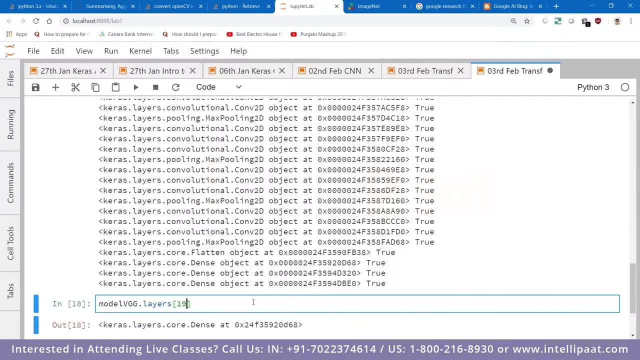 what dance? 9, 19, 19, 7, 18, so till 18. this is the fad: 6, 8. fad 6, 8. you can see, you can match this number: fad 6, 8 till 18. you want to say that we don't want to train you, sir? 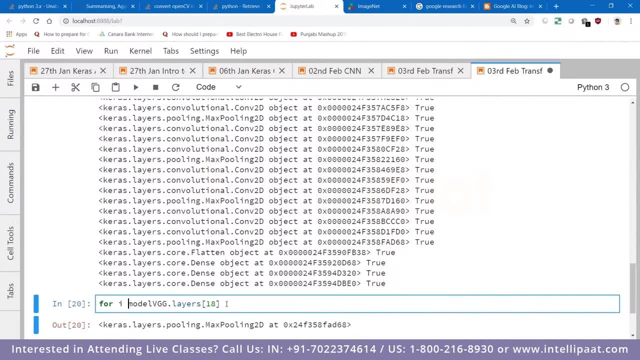 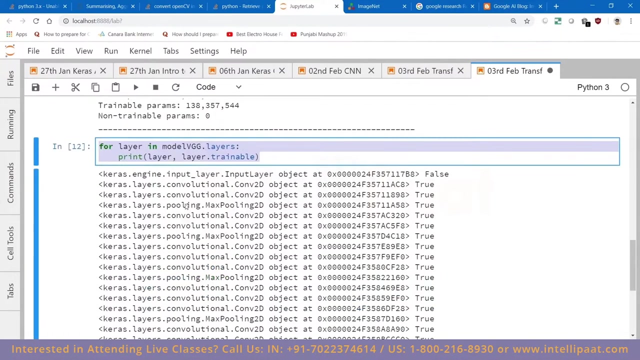 right. so what you will do, you will say for i, for layer in model vgg till 18, let's say 19, because you want to get one layer dot trainable equal to false right now, what we will do. we will again recheck that we have done the good things or bad things. let's check everything: is trainable equal to false? 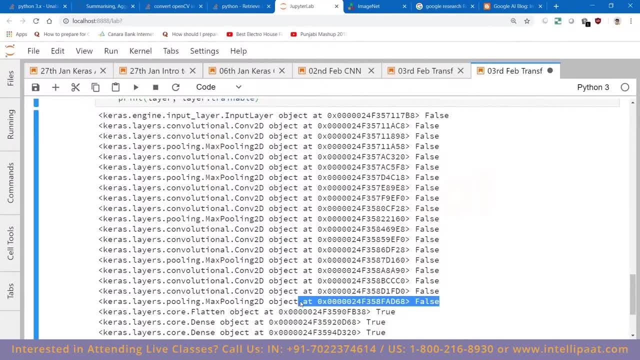 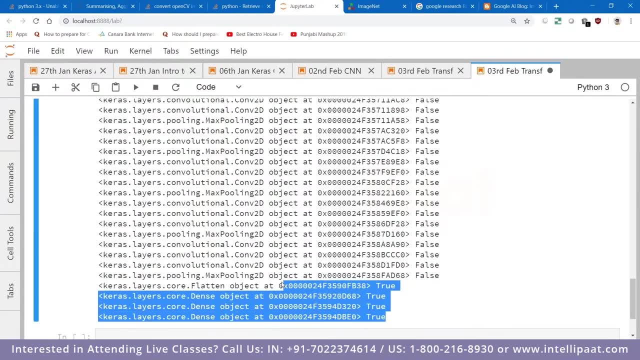 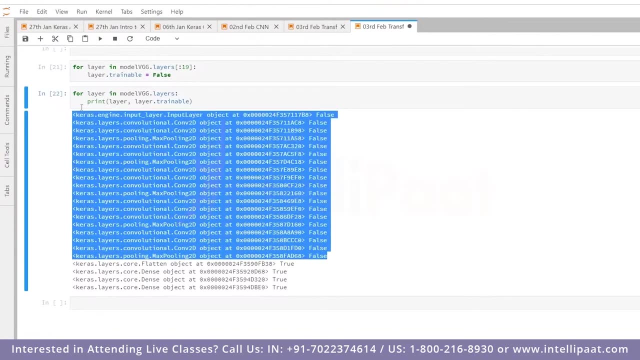 false, false, false, false, false, false. still here. see CourTale layer: we are going to train train is equal to true. so now what we can do is we can move our layers. and we have got the layers. we have got them fall. still here. right, we have got them falls. 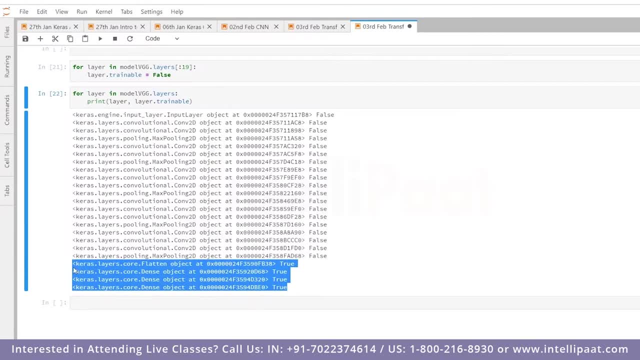 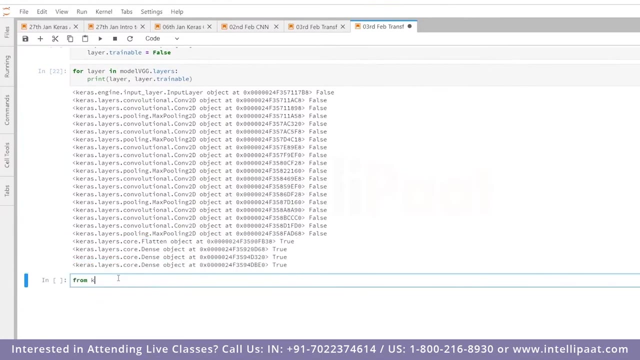 still here. they are not trained. we will train this still flatted till flatten. what we have done is we have made them as true left trou. now what we will do is we will add our own layer, right, we will add our own layer, let's say, from these: 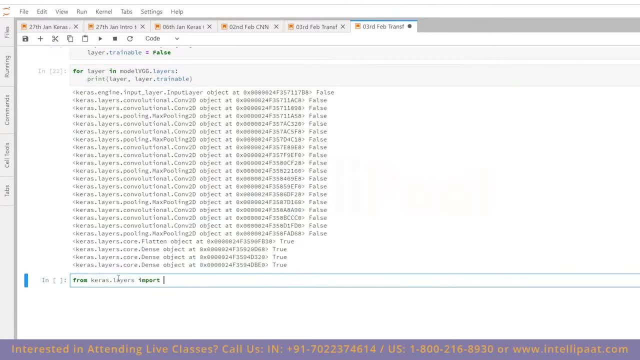 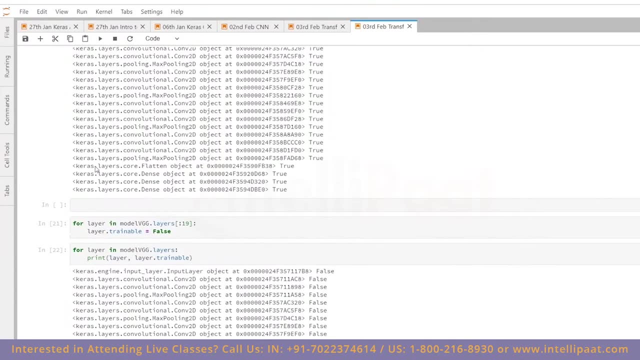 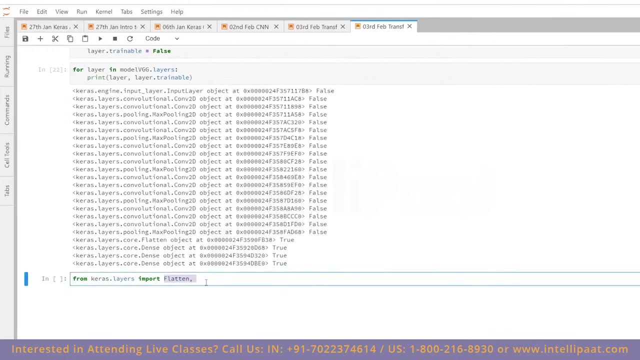 are not layers, import flatten, okay. so what I'm trying to do is I have this flatten, this dance, dance, dance, dance, dance, right, and then we will put another dense here. right now, what I will do is I will say that what I have got from that output X is equal to model BGG dot output. now what will happen? everything. 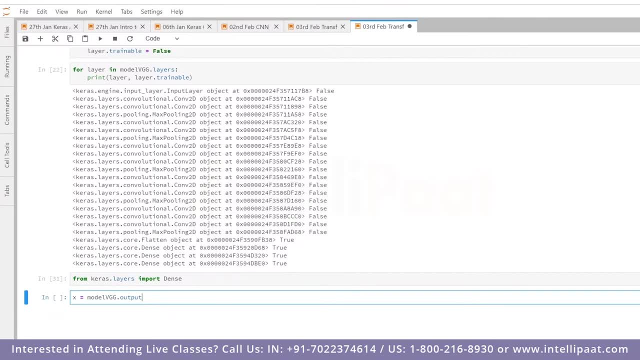 that is being till there will be outputted to me, right, and then I will say: X is equal to model. BGG dot. add model. what is happening? this is, let's say, dense, you add dense and add dense to what x, right? so what is happening? i have given. 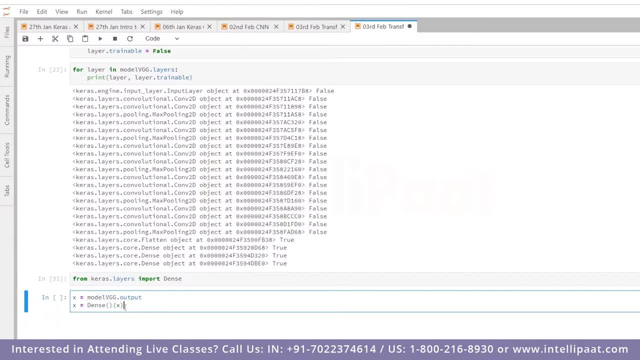 this output to what x, then x go. what i am doing, i am giving a dense to x, right? or what i can do is i can do, i can do this and then i can say: type of x is what tensor. okay, so x is equal to dense i. 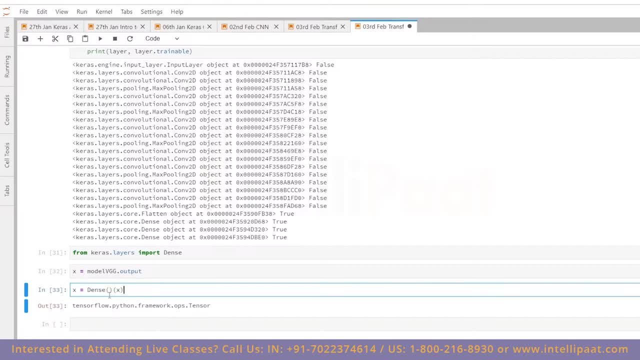 will say: make a dense, but where to attach the dense? attach it to x, only back again right, and how many. let's say: reduce it to five, one, two and then again copy this thing and this time make it to two, only correct. let me copy paste this line in this line only, so that we are not playing with. 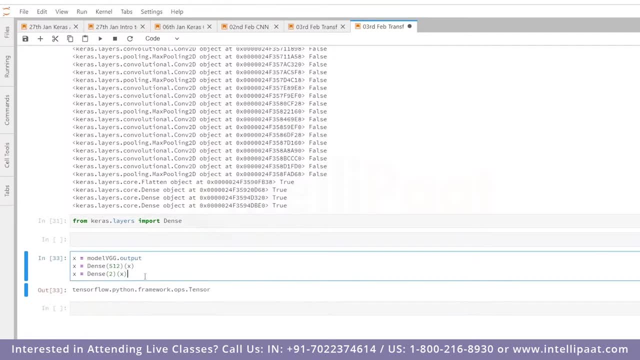 x again and again, because this will hurt the model a lot. right, and if i check now, x, x will be a obstensor. cool, what i did was i just added this one more, two layers after this dense layer. so i know this dense layer was of thousand categories. now i have reduced it to five, one, two and then two. i had to. 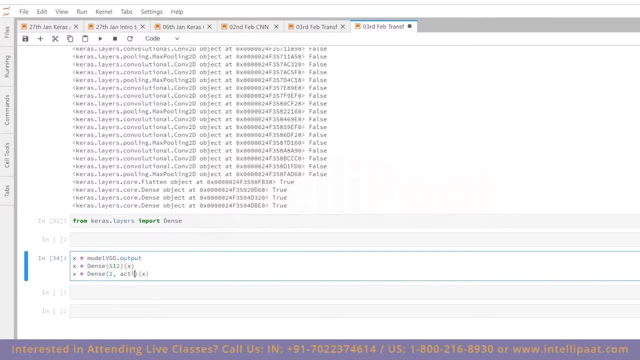 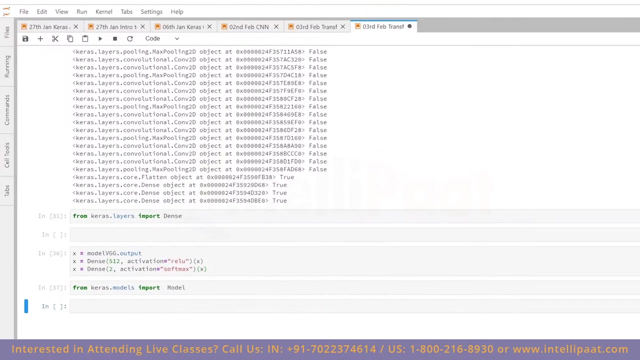 do one more thing. you guys forgot that here i have to add activation, also activation. let me add soft max, soft max and here also soft max. here i will add relu right now. once you have made this thing, you will say: you from keras dot model, import model. now what i will do? i will pass this x through model right, i will say: final model. 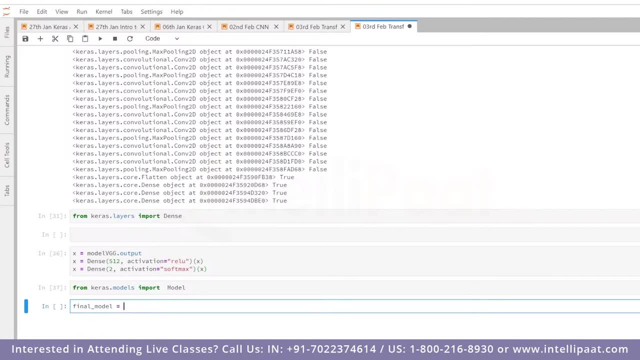 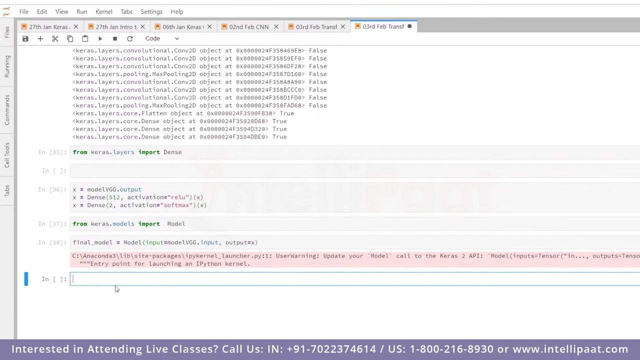 final model is equal to model. model will take two things. first is the input. who is giving you the input? so input is from what model? vgg, dot input right. and who is giving you the output? output is given by x. correct what i'm trying to say. i'm trying to make a final model, this final. 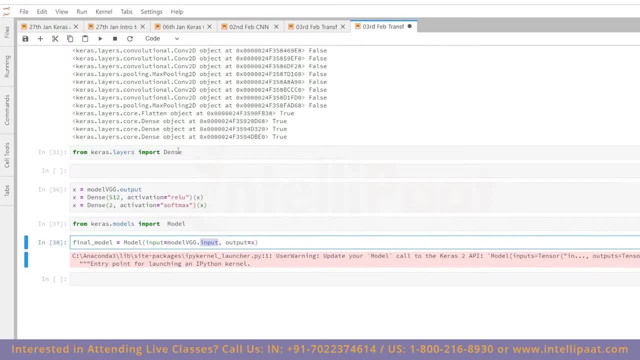 model has the input from model vgg, dot input, i mean this layer, right, and then you have output at x. x was what this dense two bit softmax, right? i showed that we have done one small error here. I will tell you. if you have got that error, then it's very good now. 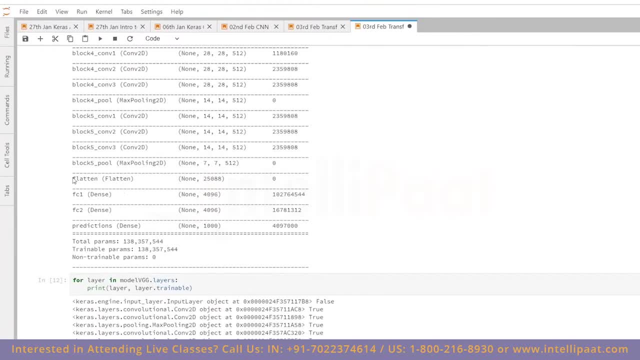 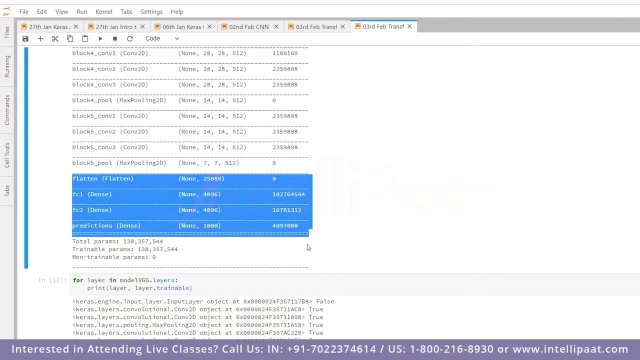 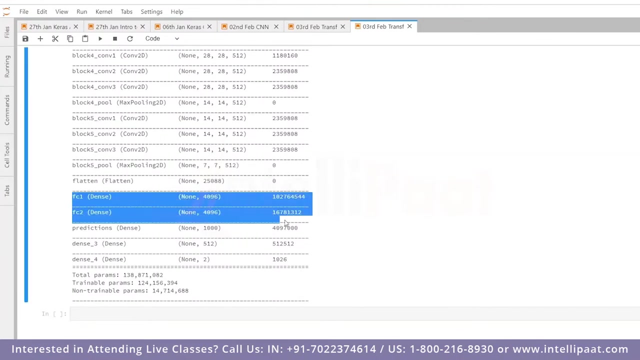 see eventually, how many FC layers did you have? you had a final FC layer, then you have a prediction layer. right now, let's see what you have. you have a flat FC layer, then I have see layered and a prediction layer, and then you have dense two layers. do you see this? this is how you are connecting your models, do you? 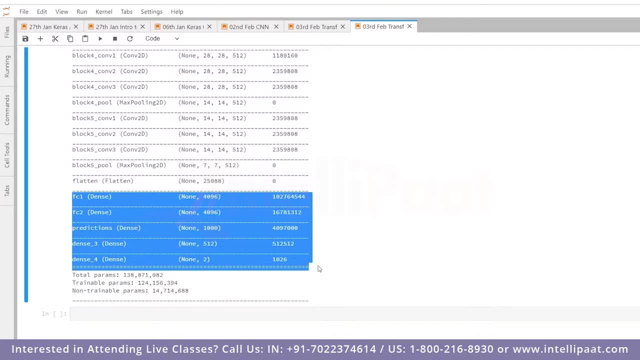 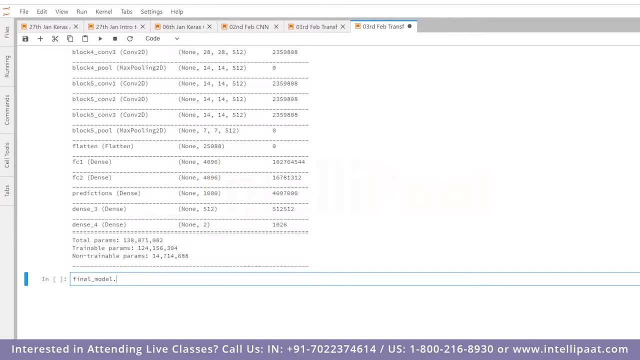 get the idea everybody, then you have to do nothing. you have to save model dot compile. so in final model dot combine, final model dot compile optimizers is equal to Kira's taught losses taught categorical cross entropy you have, then you have optimizers is equal to Kira's taught optimizers taught SGD. 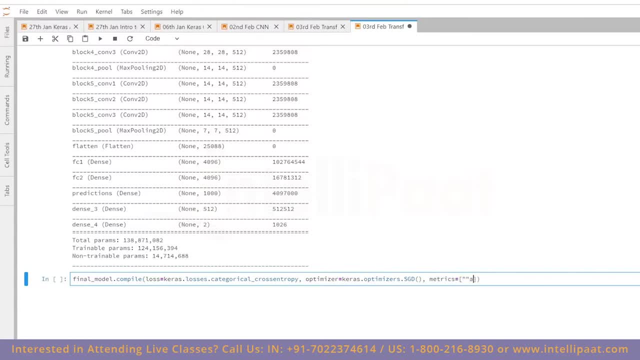 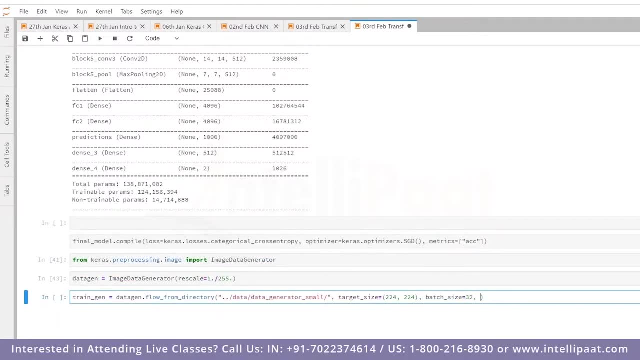 right, and then you have: matrix is equal to accuracy, right, and then you can run your final 32 images for it and class mode is categorical. I think it's categorical by default. yes, class mode is categorical. you don't have to give. this is your generator, it's ready. then later is. 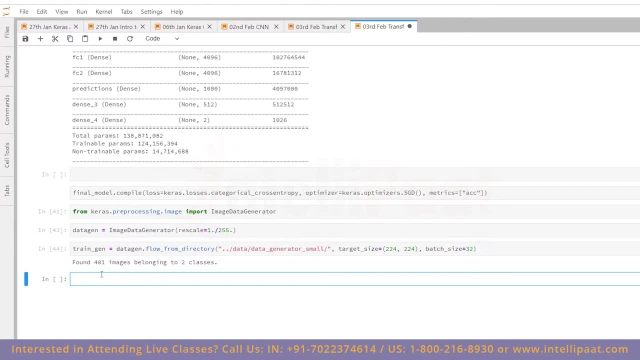 ready, ready. now you have to do nothing, you have to just say to your model what you have to say to your model: that model, final model, final model, dot fit generator. then you have to give range and a park. I will give only two- and then start this thing. this will start your modeling. quite easy, right, practical. 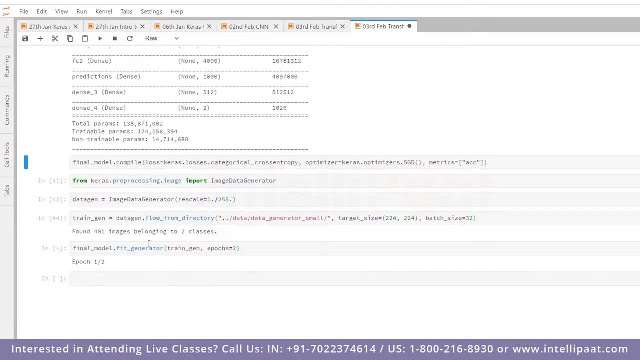 point of view. it's very easy. you don't have to do anything. this is will just will blow my laptop. I will not run it much because it's like a can go back to 500 MB of weights running in and out and my laptop is very, very, very, very short. 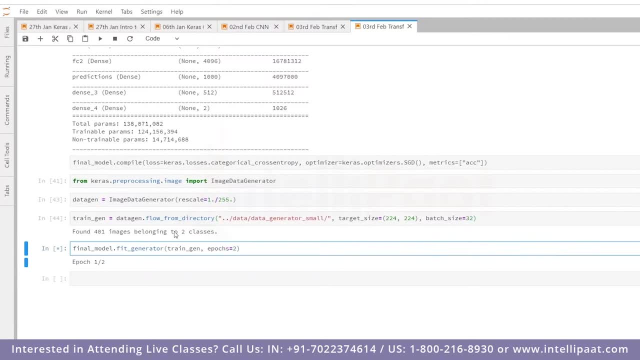 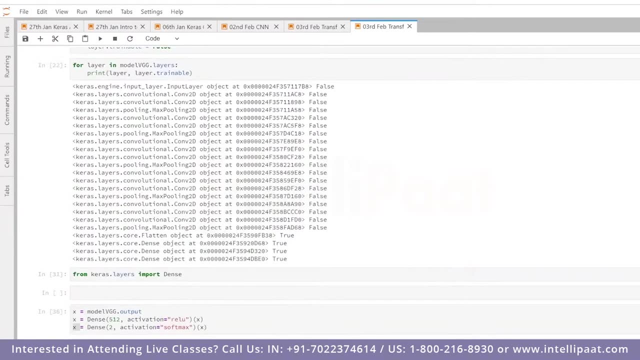 to taking time. it froze, okay, but this is how you can run and I think this is the best thing. you can run it as in collab. you should definitely run this thing in collab, collab. it will run really fast, it will like, will start see, you can see. 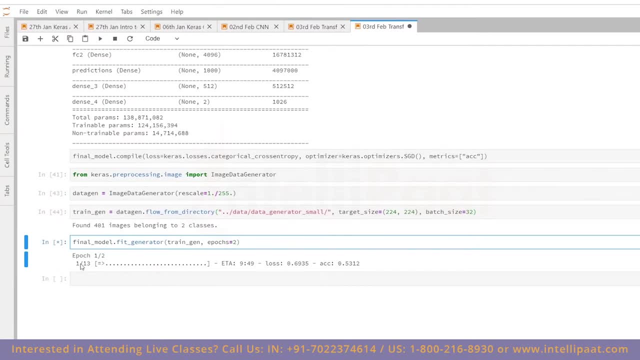 even with the first, even with like the first, what do you say? a batch only, you have got an accuracy of 53. if you run it for like 20 or 30 epochs, you will get an accuracy of around like 80- 86 percent in the starting only. so this is the 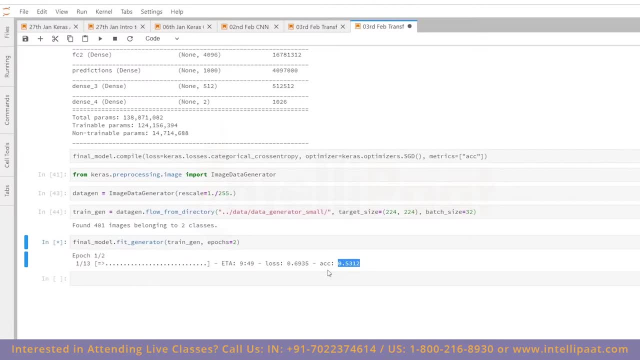 advantage of you know doing transfer learning. your model was still, it's, it will stick. it still take time to learn these things right, but here you can see it's learning. see 54 eight minutes to complete one epoch for me. but important point is that is giving. 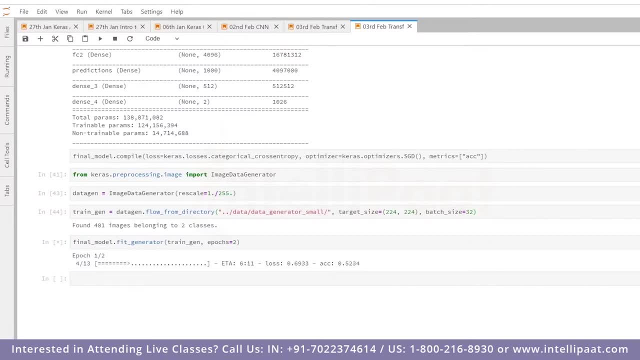 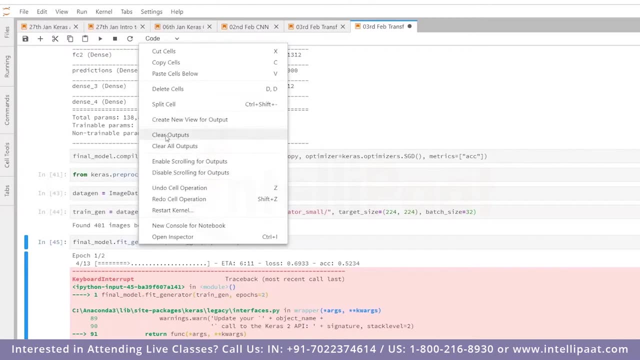 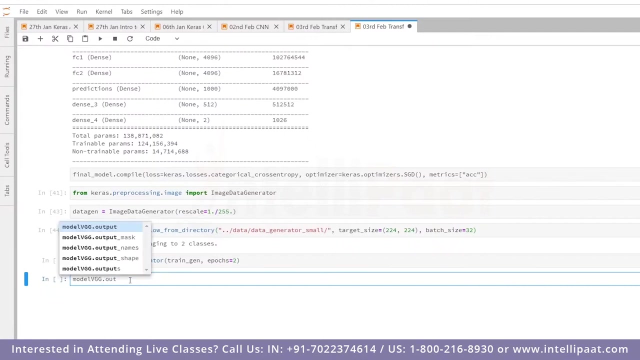 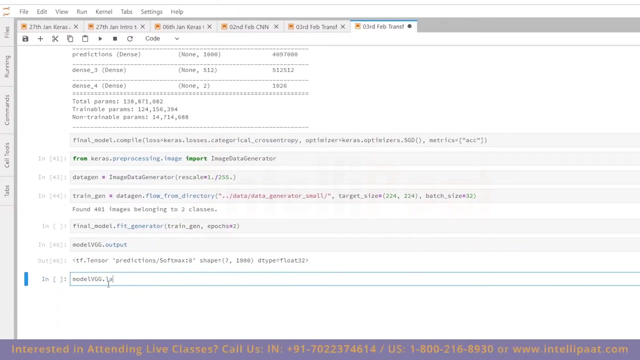 me the accuracy right. okay, stopped, let us do okay. so model VGG, model VGG dot output. if you print this thing, this is this right, softmax cup addiction. and if you do model VGG dot layers and if you do minus 1 and then you do output, this will be also the same right. 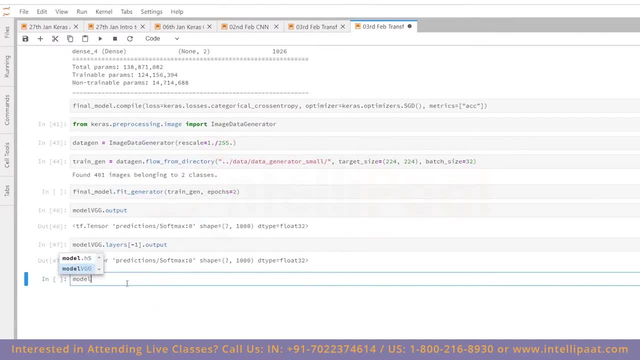 so, rather than doing this, we could have said the model, that model VGG dot layers, and then we could have said minus 2, minus 2 dot output. so what it would have taken it? it could have taken the answers from the FC 2 layer, right where it has. 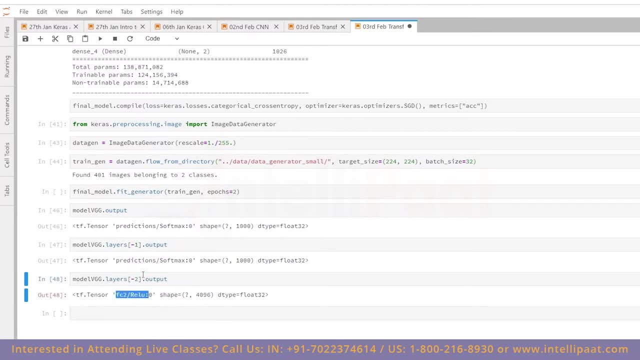 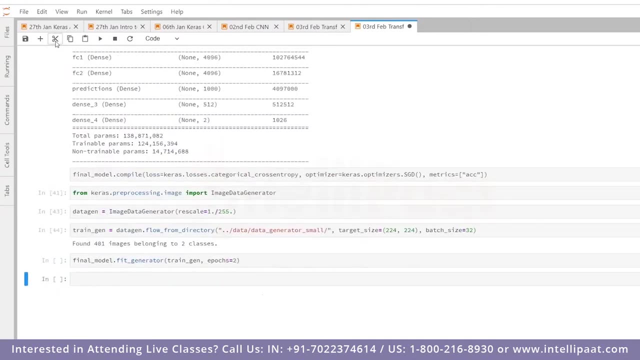 the relu activation function. you can see here FC to with relu activation where, as the last layer has predictions, softmax. let's me show you this thing so that you don't have doubts. but just replace this. but what I have to do is I have to rerun the whole thing. 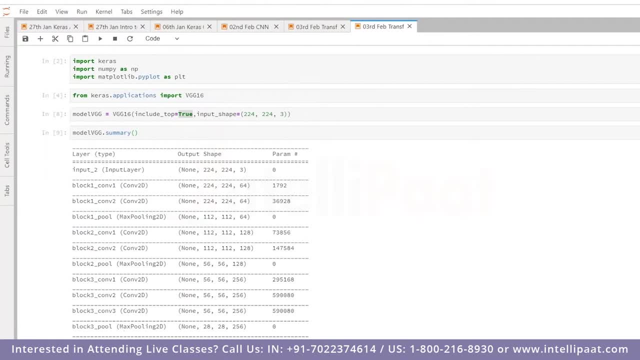 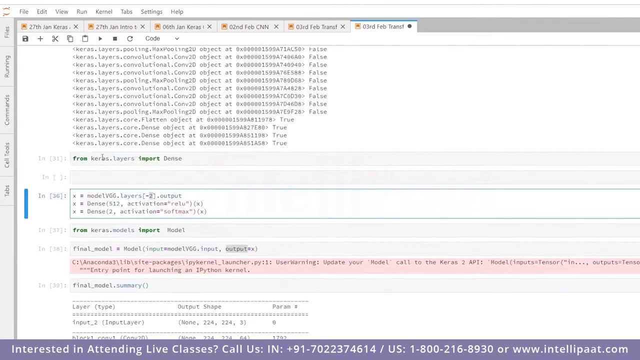 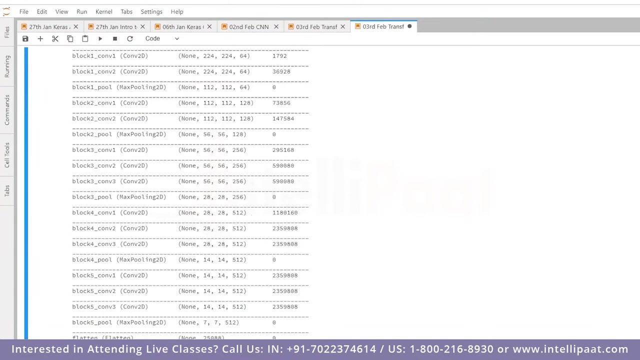 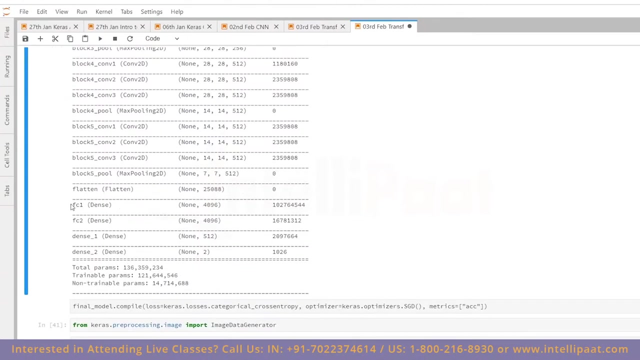 now we start the kernel, then read on everything. very easy, won't take much time, right, this, you run this also. then you go on: this, this and this and this. so right now, see, right now you are getting in the final summary. you were getting a prediction layer also, but now you won't see. right, see, you have only FC, then FC.